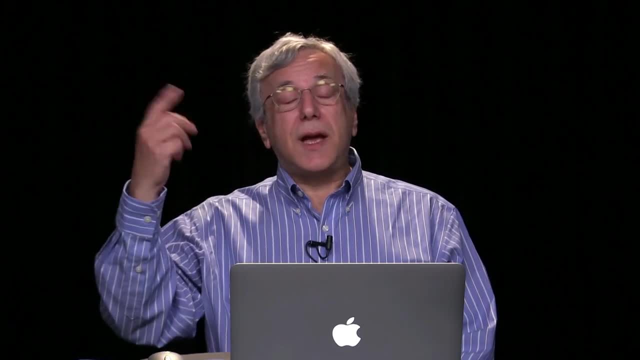 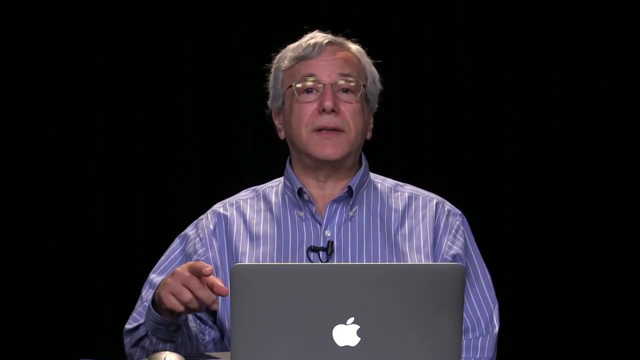 Now, then, maybe you would get to statement 50 again and jump somewhere else, or maybe, before you got back to statement 50, you'd encounter an if statement that sent you to another go-to statement that would sending you to line 2013.. It was a confusing 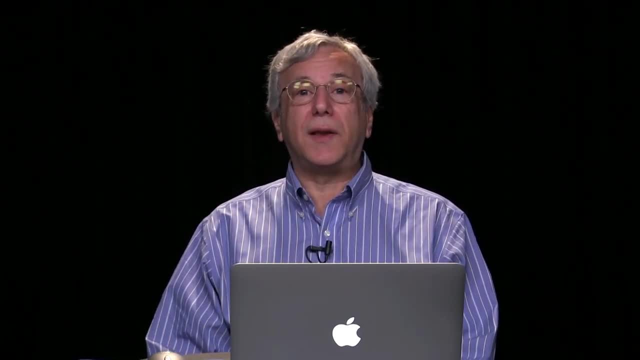 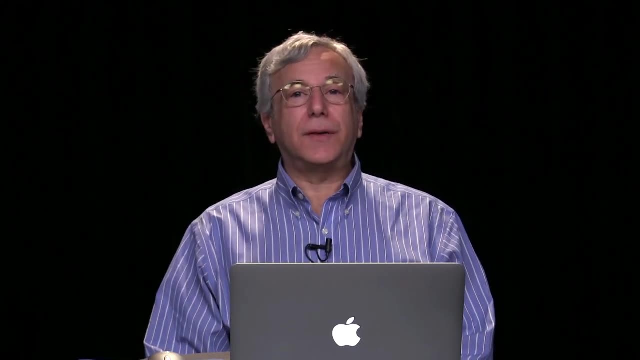 mess. It was called spaghetti code because it reminded people of code that's entangled the way strands of spaghetti are No good, No good. And Edgar Dykstra wrote the line379. this letter that said we shouldn't be doing this, we shouldn't be jumping from. 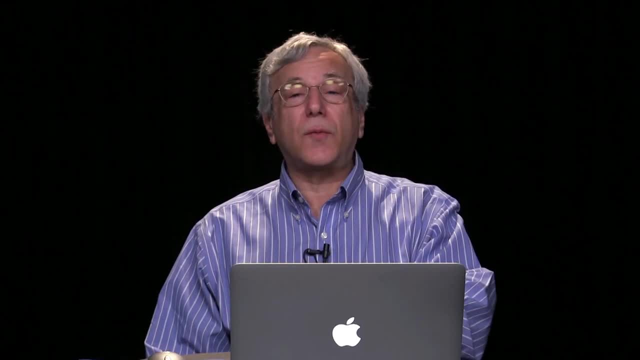 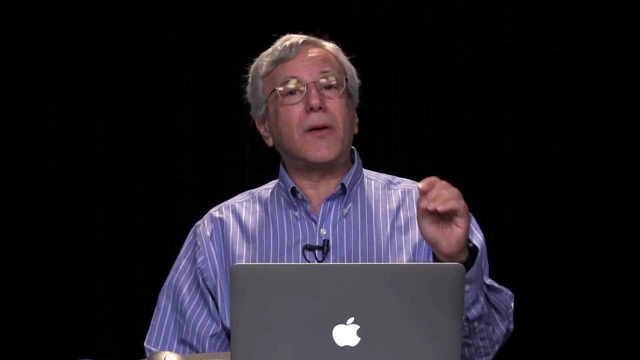 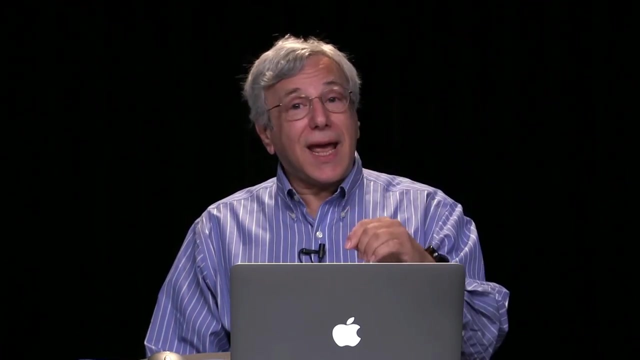 one part of a program to another part, to another part to another part. it makes the code very confusing. now, if you've never programmed with go-to statements, you don't know exactly how confusing this could be. this could actually make a program what we would consider today to be unreadable for all practical purposes. 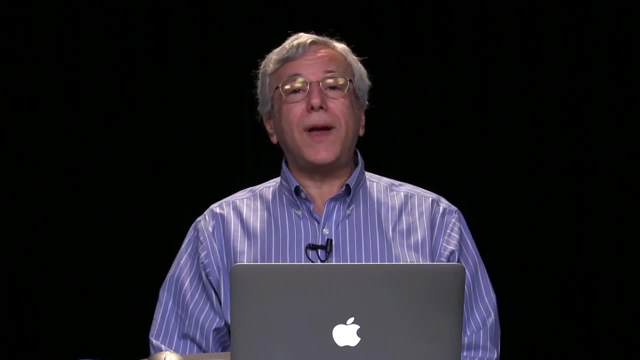 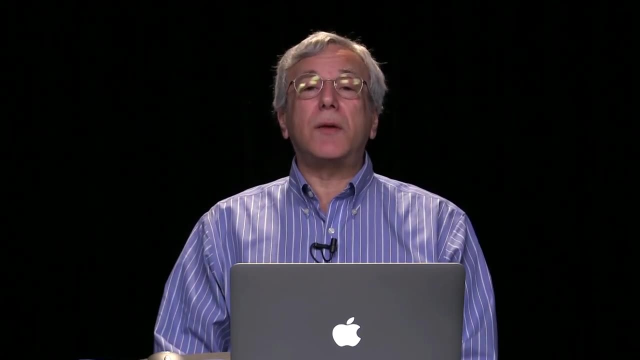 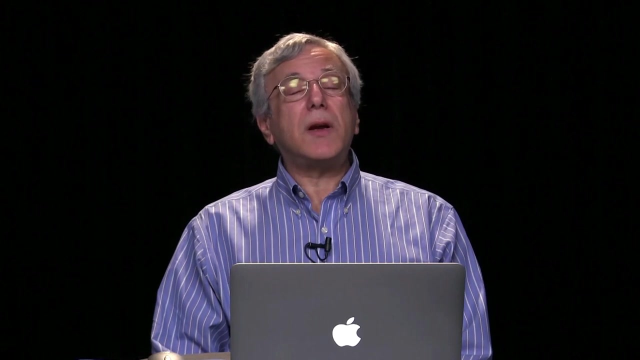 well, we've gotten rid of go-to statements, but now we have steps through programs that are more orderly. start with statement number one, then go to statement number two, then number three. ah, here we are at statement number four. at statement number four we encounter an if statement: the if. 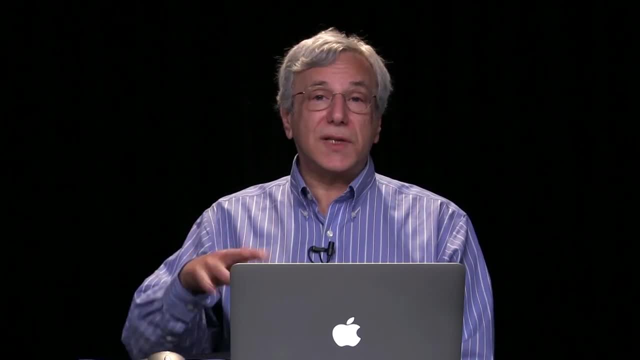 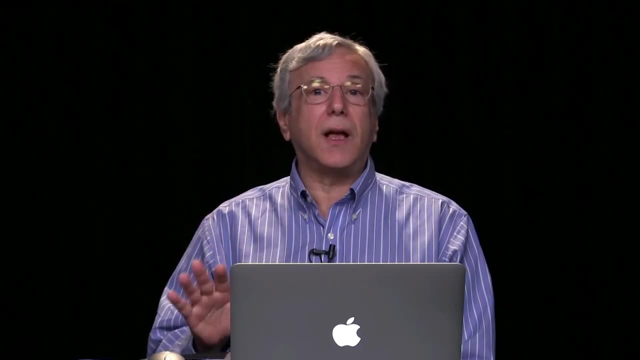 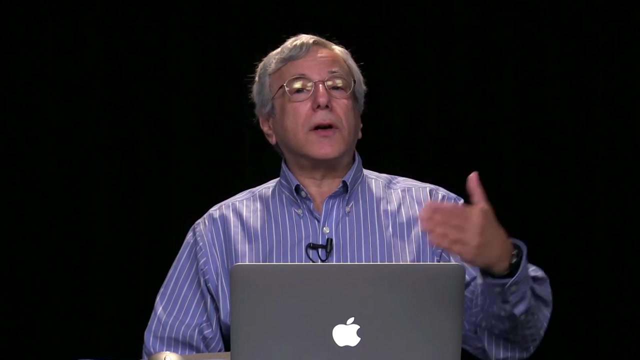 statement says: if a certain condition is true, then do this block of statements, otherwise do some other block of statements. okay, that's a little bit more discipline, actually a lot more discipline than a go-to statement. and then maybe later on in the program we encounter another, what we call control structure, a loop, and 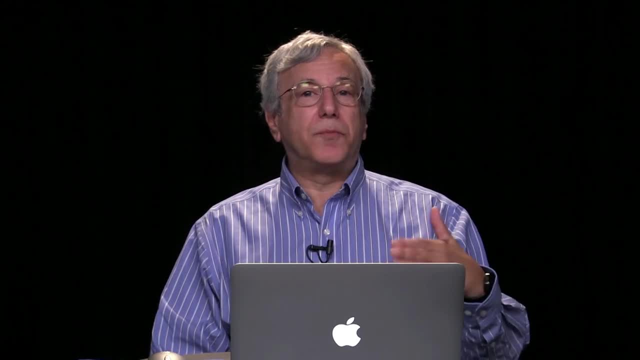 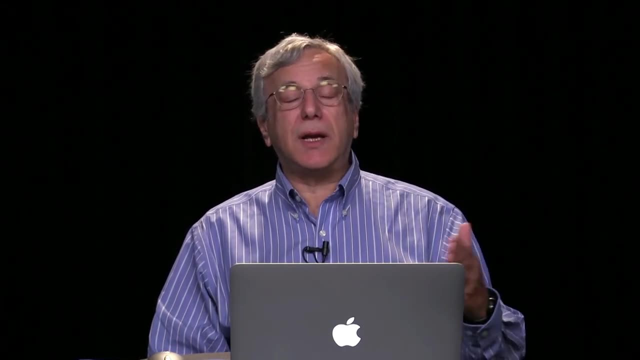 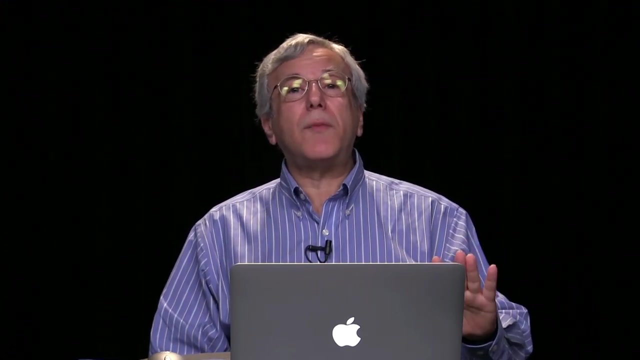 what the loop says is: do this block of statements once, and then, when you're done, do it again, and then, when you're done, do it again. keep testing conditions and make sure that you should do it again, and again and again. eventually jump out of it. oh wait, a minute, now we've got an. 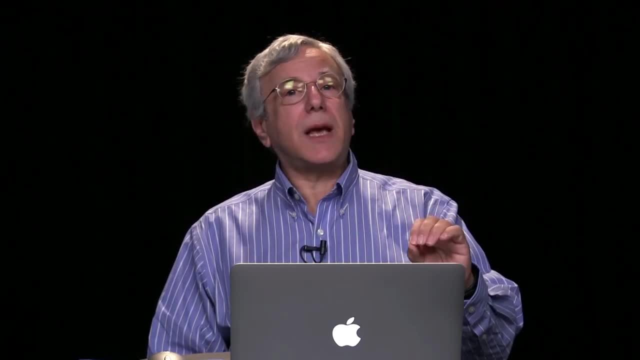 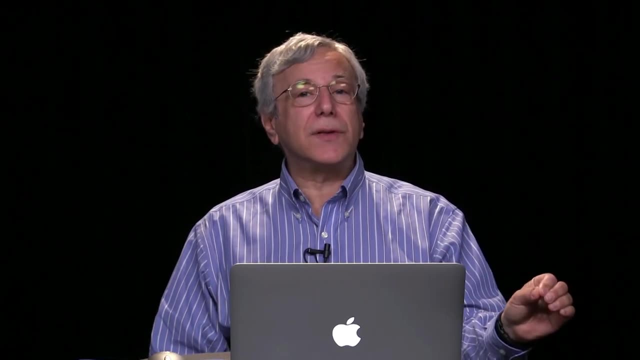 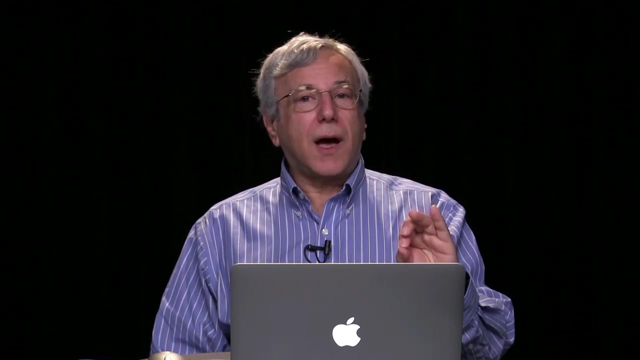 accessibility an exception handler. get into the exception handler and try to do a bunch of statements and when something goes wrong, jump out of those statements. whoops, I just used the word jump. sounds a little bit like a go-to. okay, the jumping that we've got in our current programming structures is much more. 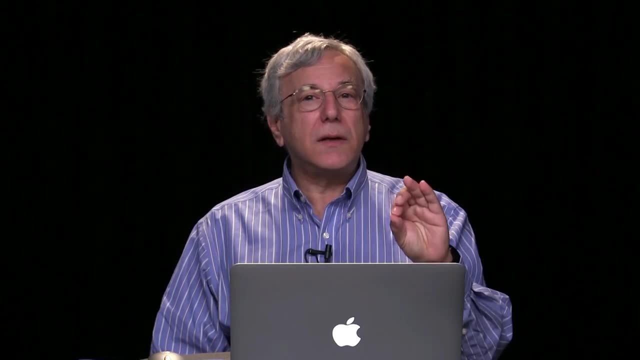 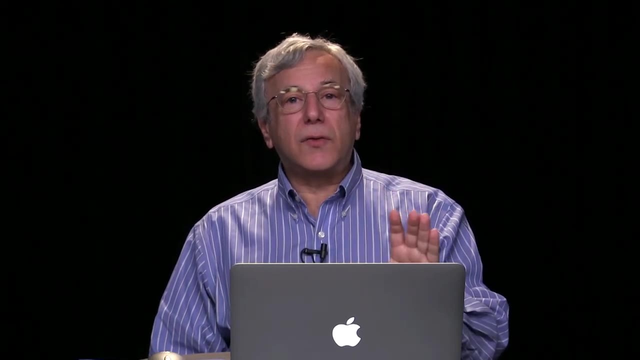 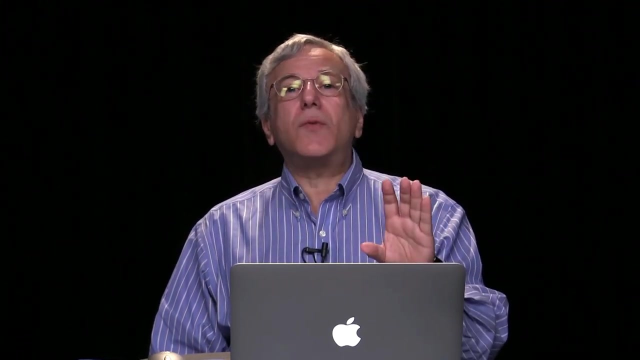 disciplined than a go-to statement, but it's still some sort of jumping. it's still some sort of sequencing. i'm going to make, at the start of this course, a very radical proposal. my proposal is going to be: any sequencing of statements in a program is to be: 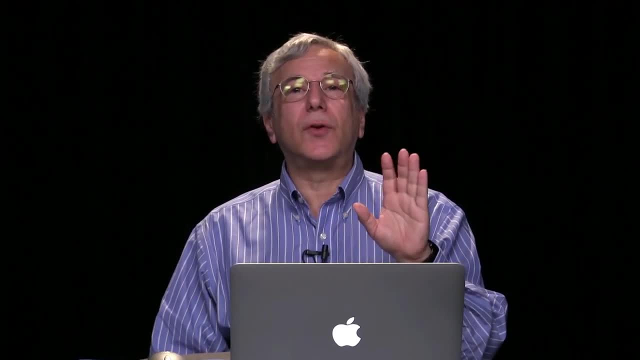 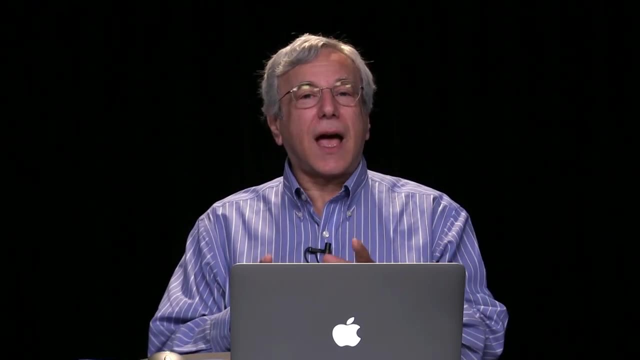 considered harmful. now I know that most computer scientists won't agree with me about that, but that's because i'm taking the very extreme approach here. what i'm saying is that it's not a good idea in a computer program to say: do this, then do that, then do that. 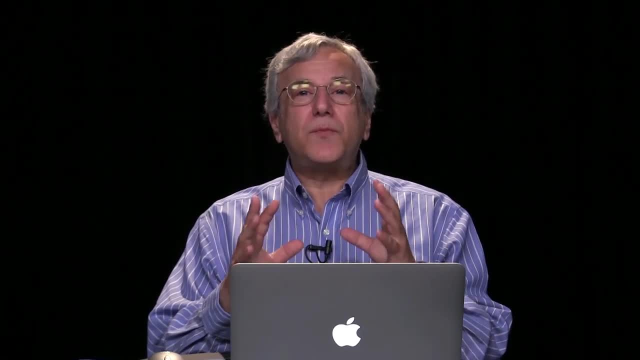 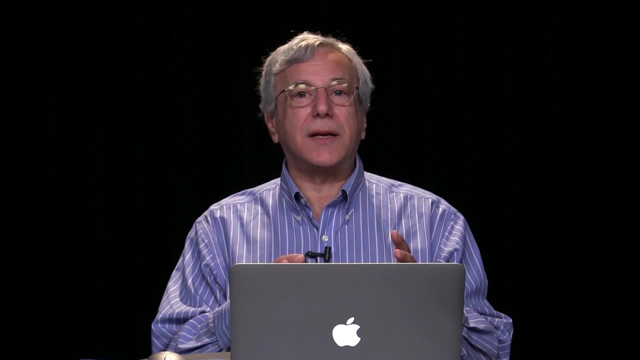 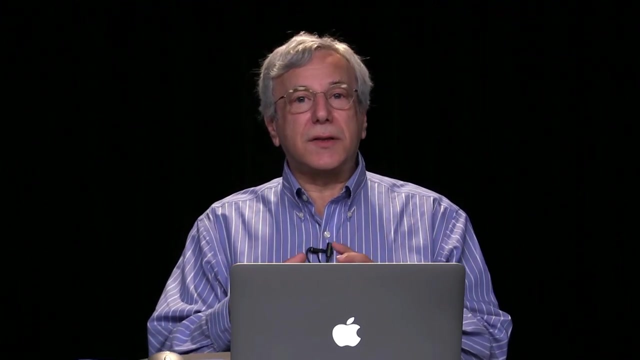 than do something else. Instead, it's better to think of solving a problem in terms of the mechanism, the tried and true mechanism in mathematics called functions. What happens when you have a function? You take a value and you apply a function to it. 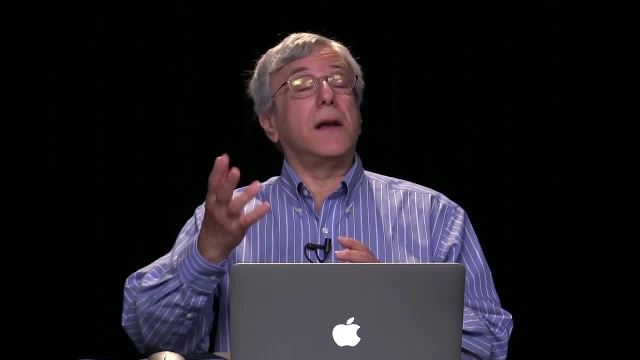 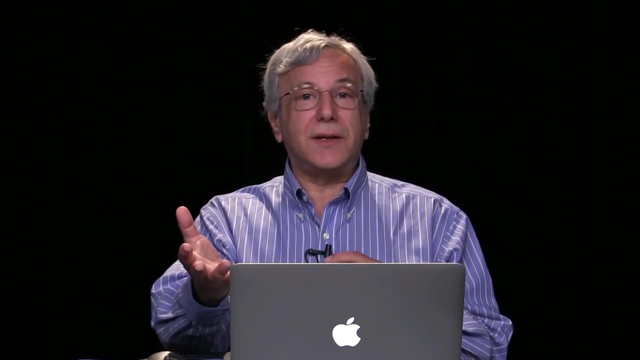 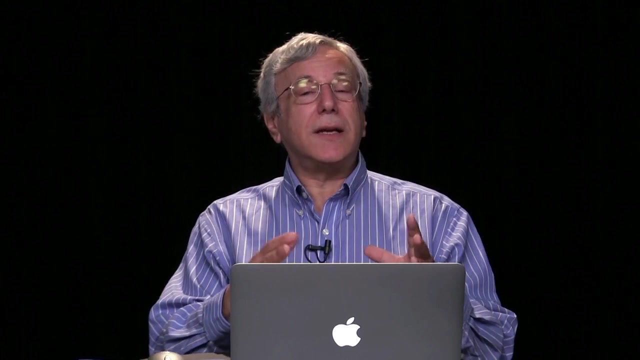 and you get another value, And then you apply another function to that result value and you get yet another value, And then maybe you apply yet another function to that value and get another value. I'm going to propose that that's a more disciplined way. 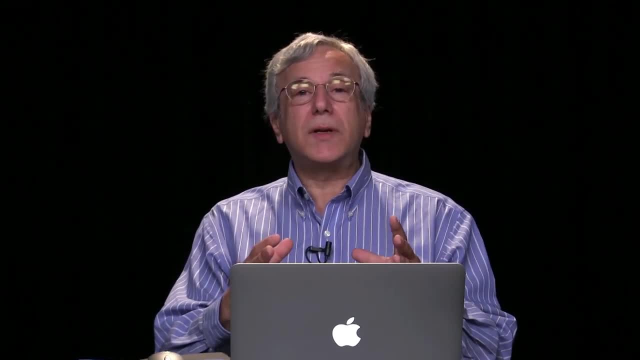 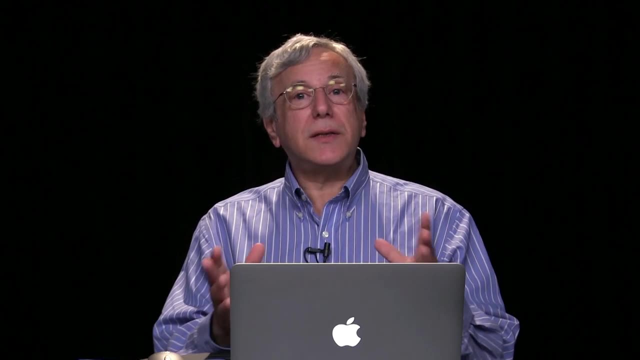 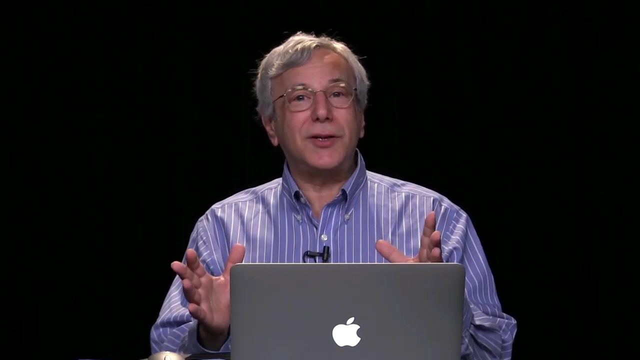 to look at solving problems and that that more disciplined way will lead us to programs that are more reliable, more correct, easier to work with. Am I correct or am I incorrect? Well, it'll be up to you to judge, and I'll give you all the equipment to judge. 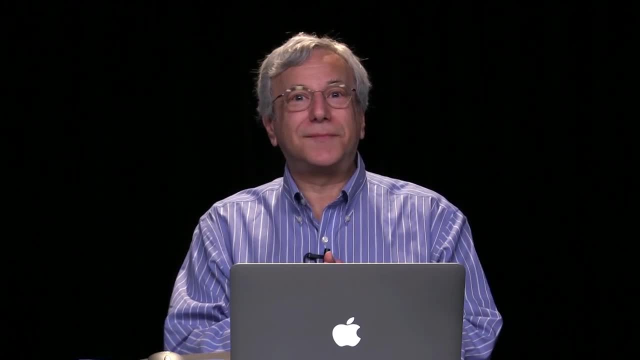 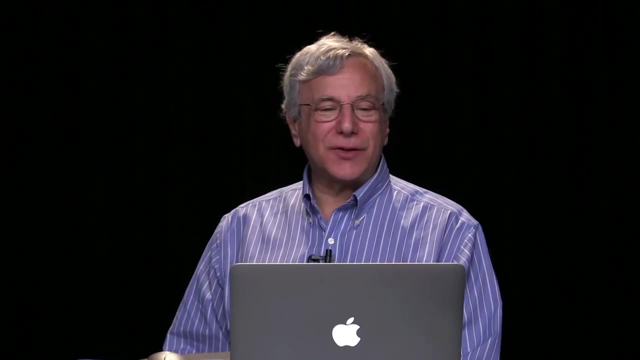 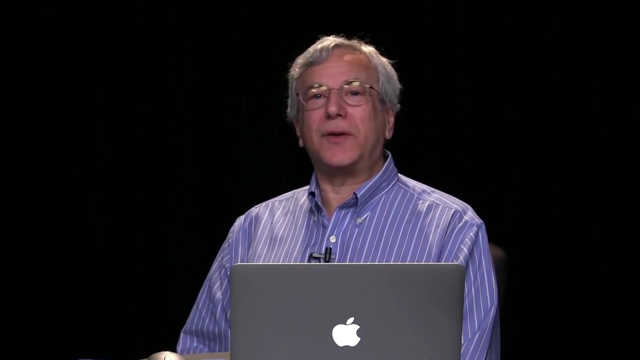 as this course goes on, I hope you enjoy it. So in this section, what I want to do is introduce the notion of functions and solving a problem in a functional style, rather than in the style that you're probably more familiar with: the imperative style. 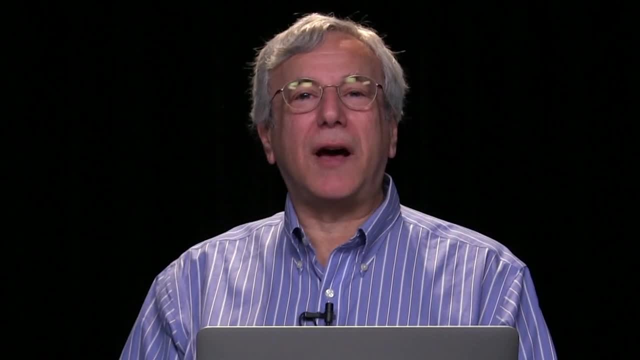 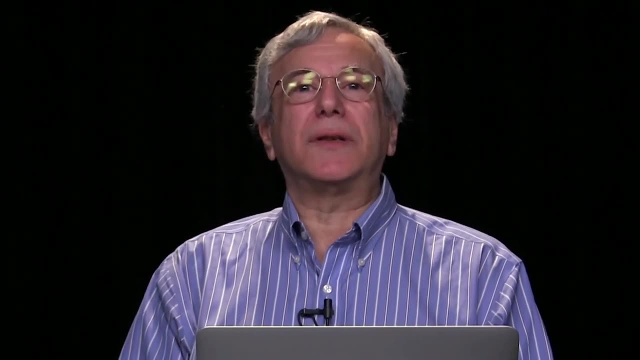 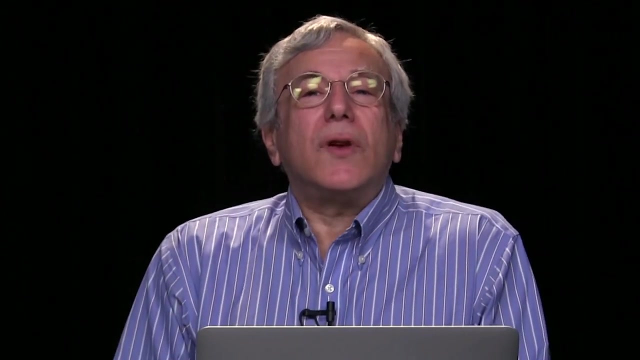 In the first section, I introduced the notion of an imperative program, that is, a step-by-step program and a functional program, one in which you apply functions to the results of other functions. In this section, what I want to do is make it more clear what you can do with functions. 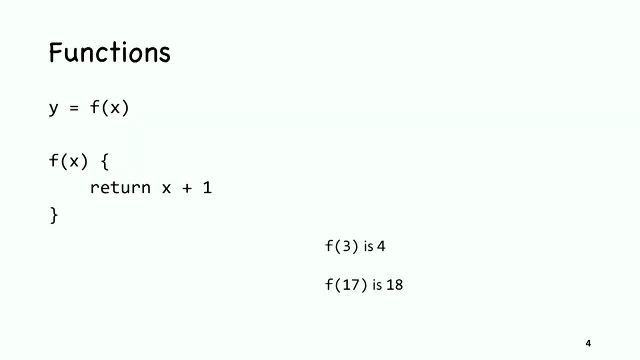 So let's take a look at one problem and see how we can solve it in two different ways. First, what is a function? Well, you've seen functions, even in imperative languages. So a function is something that takes a value. in this case, 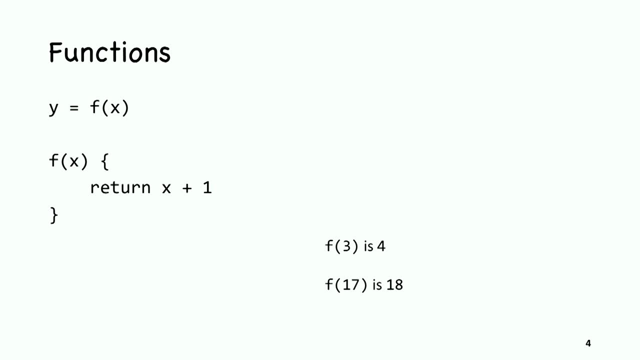 x or 3, or 17.. And returns another value, in this case x plus 1, or 4, or 18.. If I plug the number 105 into this function, then I get back the number 106.. 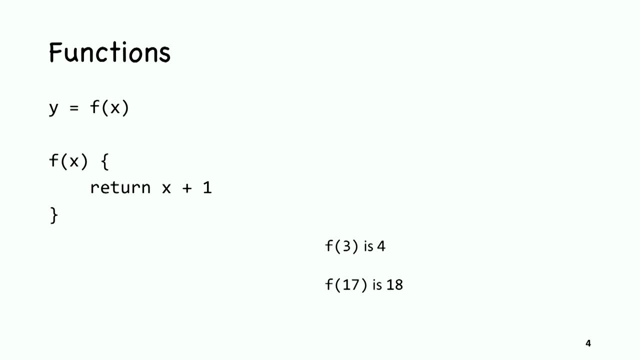 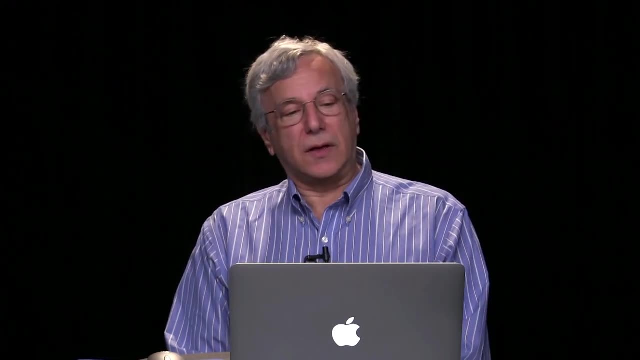 And the function in the language that you use most often doesn't have to look exactly like this. I intend to write my functions in a style that looks a little bit like Java, a little bit like JavaScript, a little bit like many other languages. 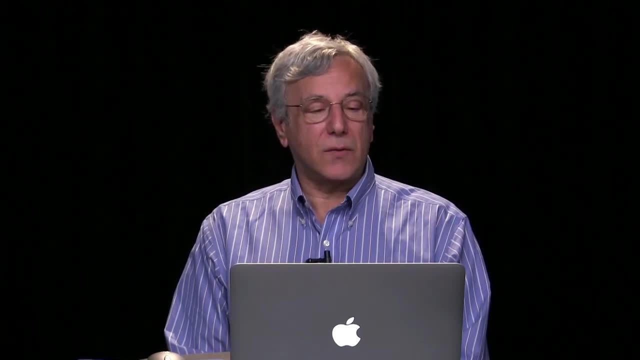 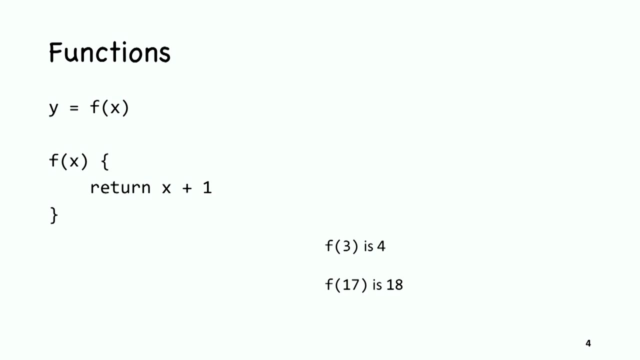 But we're not going to worry here about the syntax of the language, Just think I've got some sort of a function. That function is called in this case f. It takes an argument which, for the sake of argument, 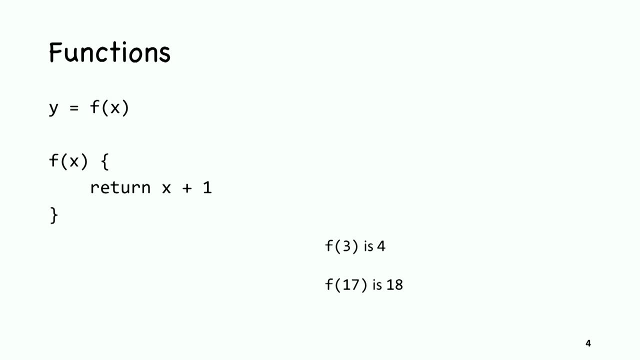 I'm calling x And it returns something else which is one more than that value: x. The y equals f of x and the f of x return x plus 1, that's just pseudocode. That's just meant to remind you of what kind of an animal. 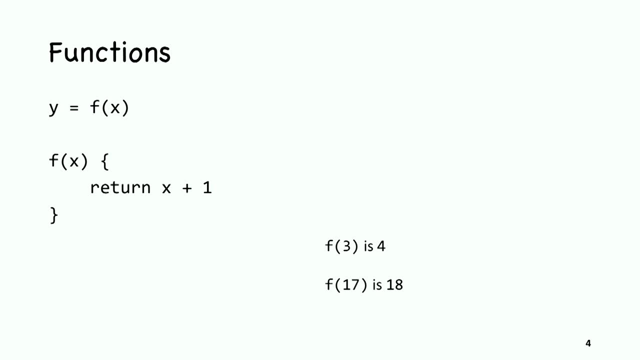 we have, And note that f of 3 is 4, f of 17 is 18.. I can create thousands and thousands of different functions of this sort, And I can use any notation that I want in order to describe how the function works. 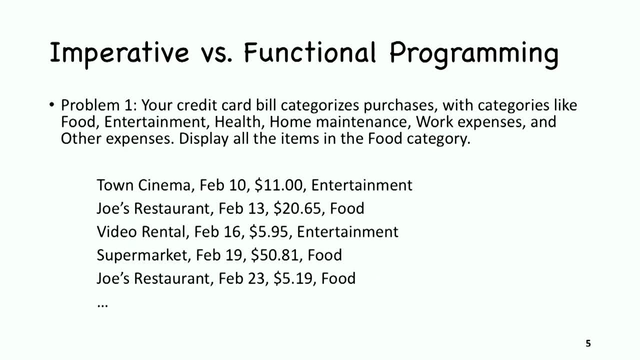 Let's take a look at a program that represents a sort of a typical program that you might want to solve in a programming language. We'll call it problem one. Your credit card bill categorizes purchases with categories like food, entertainment, health, home. 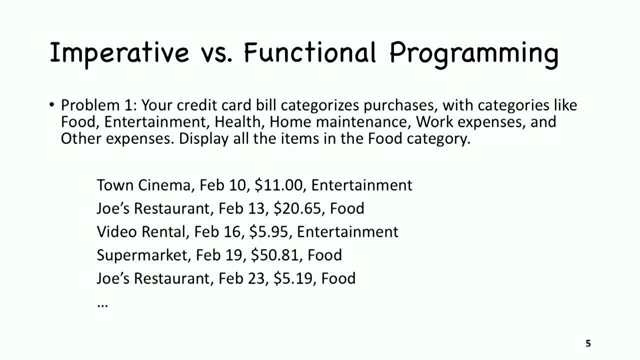 maintenance, work expenses and other things. Display all the items in the food category. You might not be working with credit card bills, You might be working in some other problem domain, But this kind of a problem in which you want to sift out all the things in a particular category. 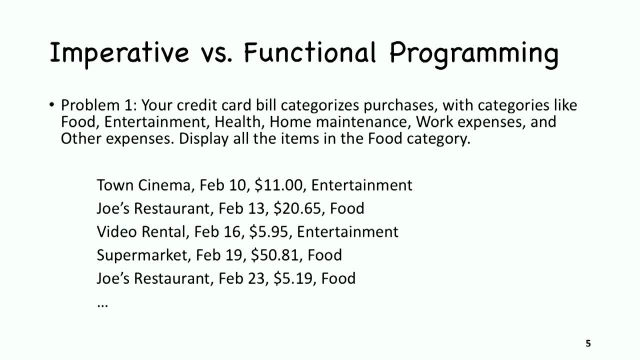 is not unusual in the computer processing world. And so, in concert with this particular problem, we've got a list of purchases: Town Cinema, Joe's Restaurant, and so on and so forth. Now what we want to do is solve the problem of displaying. 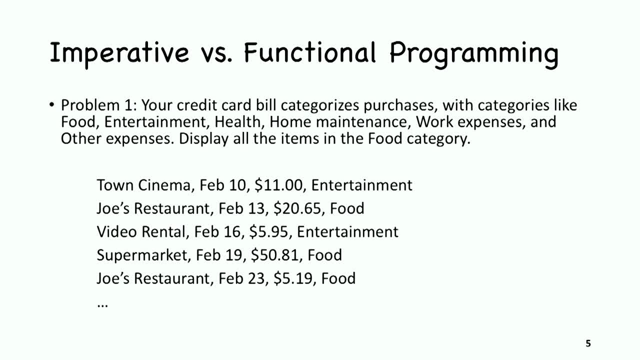 the items that are food items. Let's see how we would do it in a do this, then do that, step-by-step language, the kind of language that you're most likely familiar with. We call it the imperative style of processing, And we're going to do that. 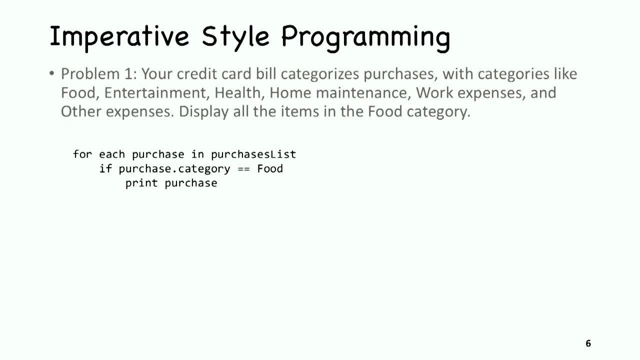 OK. So what we're going to do is we're going to do the imperative style of programming We would say for each purchase in the purchase list. if the purchase has the category food, then print the purchase. So we've got a kind of a loop for each purchase. 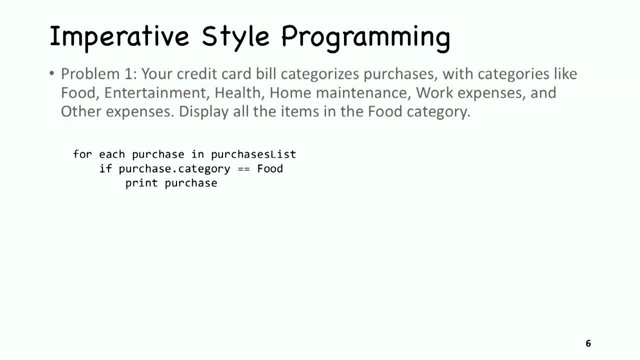 We've got a kind of a decision-making statement. If purchase category is food, then print the purchase. We've got several steps here that we have to go through. We're going to do the if statement several times. We're going to decide either, yes, print the purchase or no. 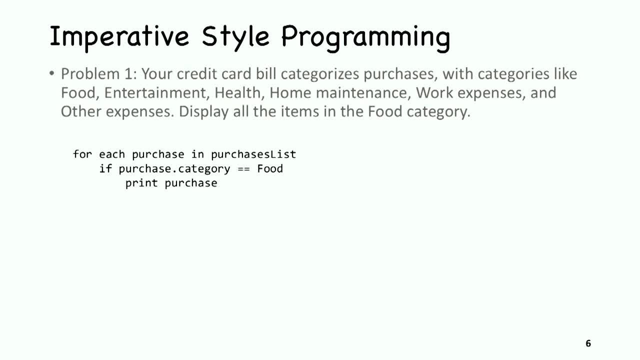 don't print the purchase. Now, I want to emphasize again that this code that you see in front of you, the imperative style programming code, is not meant to be a particular kind of language code. Well, yes, it's the imperative style programming. 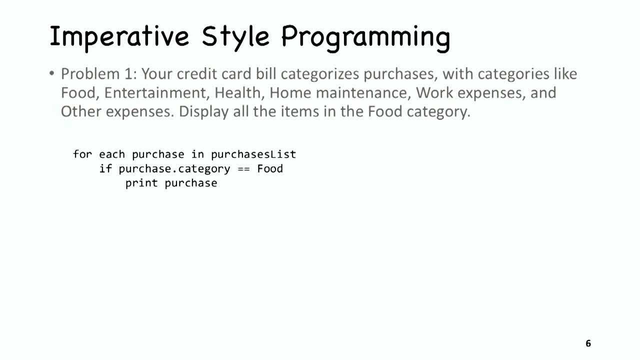 but it's not meant to be Java, It's not meant to be F sharp, It's not meant to be Groovy, It's not meant to be JavaScript, It's meant to be pseudocode and the dot doesn't indicate some kind. 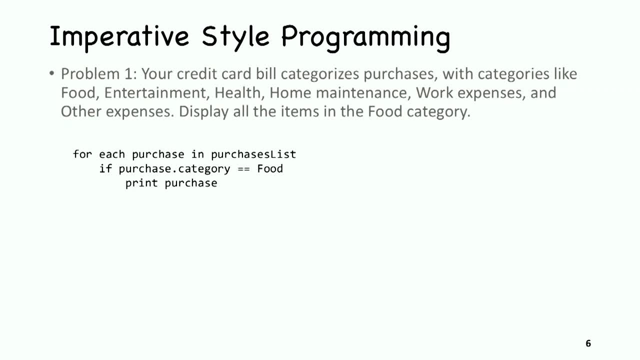 of an object or class, the way object-oriented programming languages use that terminology. I just mean to suggest here that we're going to have some sort of a loop, We're going to have some sort of a decision-making branch and we're going to have some way of checking the category. 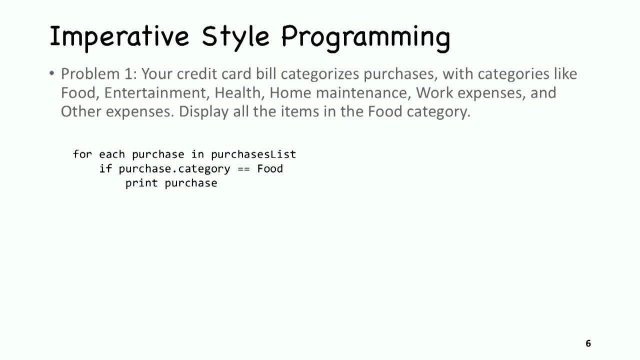 of a particular purchase And once we've checked that, we'll compare it with the category food and we'll decide: yes, we want to print the purchase or no. we don't want to print the purchase. That's the imperative way of solving the problem. 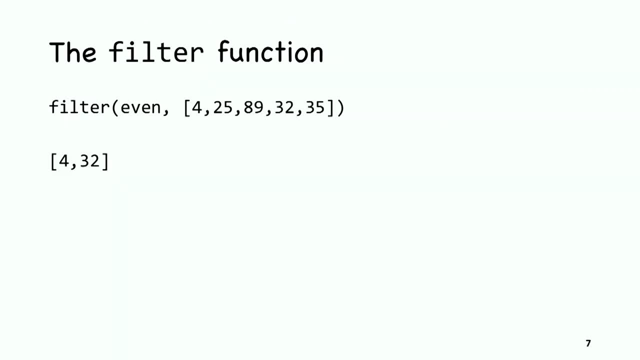 Let's take a look at how we might solve the problem in a functional manner. In a functional manner, we might have a function whose name is filter. Now again, this is the name of a function in several functional languages, but some functional languages. 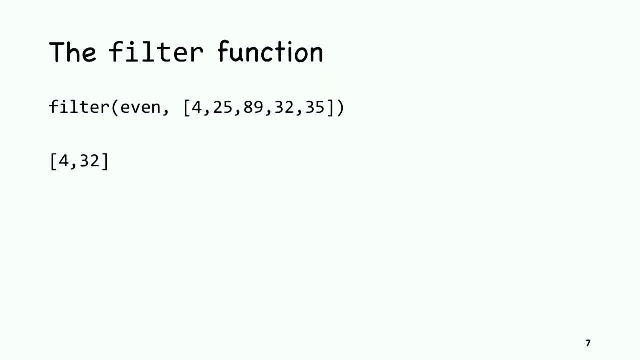 don't use the word filter. They use other words instead of the word filter. I'm not talking about a particular functional language here. I'm talking about functional languages in general. I'm going to define a filter function and the filter function is going to take two arguments. 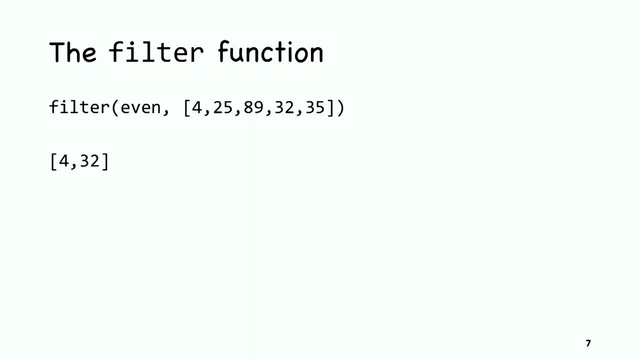 The first argument, in this case even, is a property, a property that a particular number may or may not have. And the second argument to the filter function is a list, in this case a list of numbers. So I'm going to denote a list in this course, with square brackets. 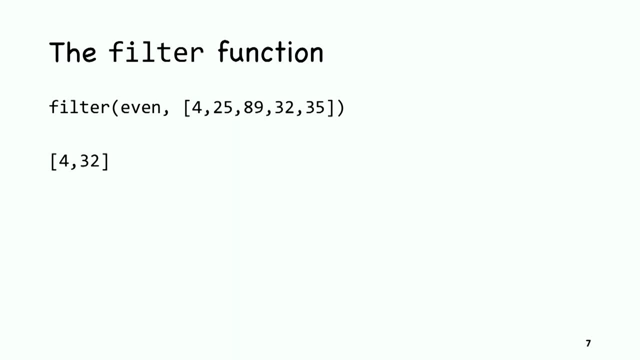 And this list will contain, in this example, the numbers 4,, 25,, 89,, 32, and 35.. And when I apply the filter function to the even property and to the list 4,, 25,, 89,, 32,, 35,, I get a brand new list. 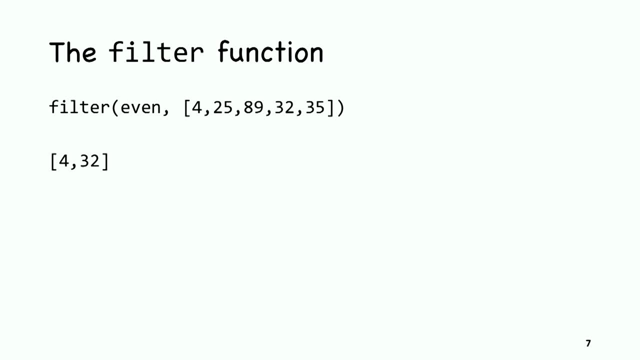 And in this case the list is the list containing only the numbers 4, 32.. So I filtered out the numbers that don't satisfy The property of being even. In this case, I get a brand new list, and that new list has only the numbers that are even. 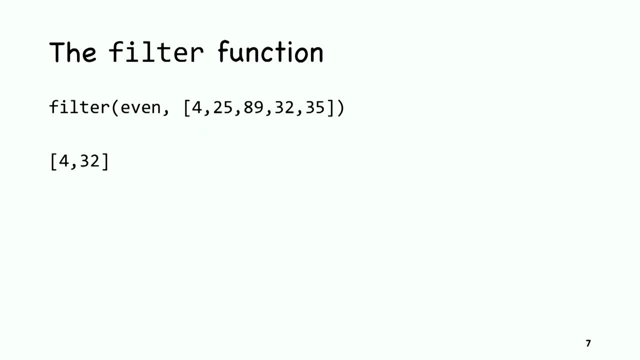 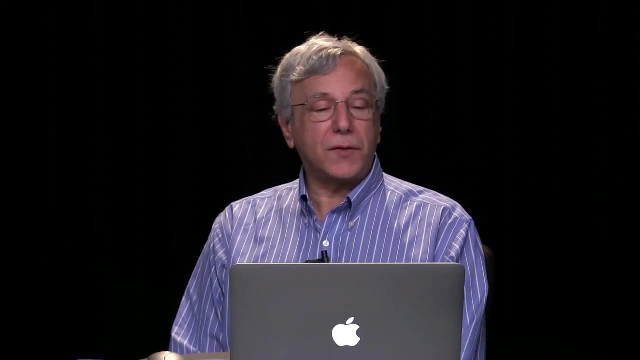 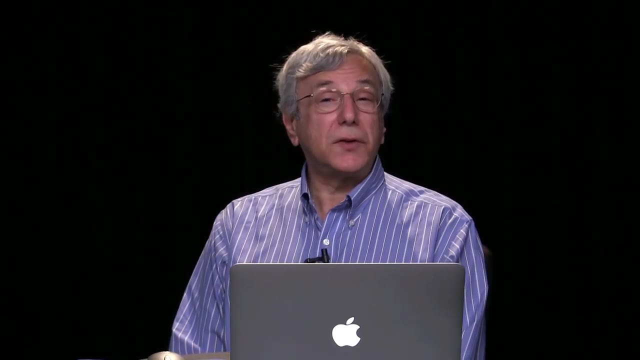 the numbers 4 and 32.. That's my filter function. The filter function- or a function with a similar purpose, maybe not named- filter is one that you'll find in almost every functional programming language. So how does the filter function help? 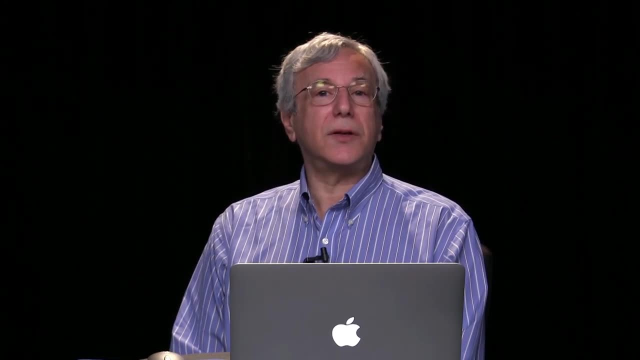 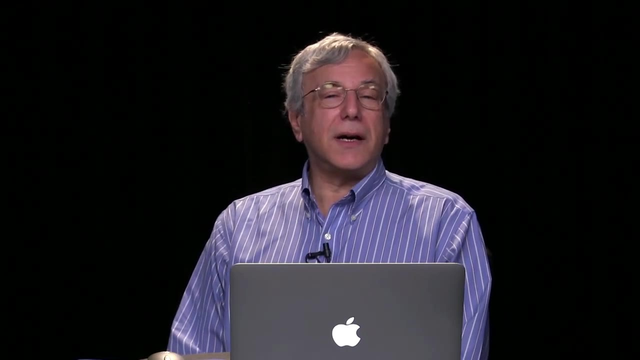 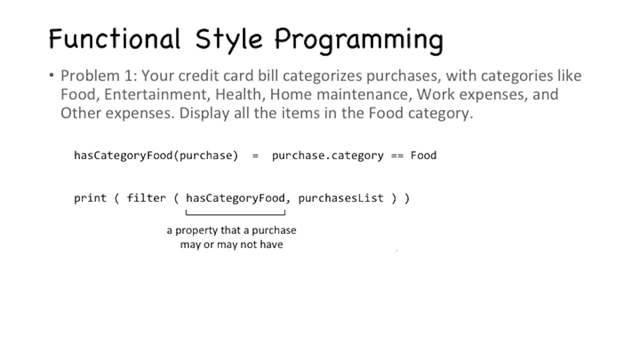 me solving the credit card category. Well, the filter function is a function that kind of does what an if statement does in an imperative language. Let's take a look at a functional style programming solution to the credit card categorization problem. I'm going to filter the purchase list for only those purchases. 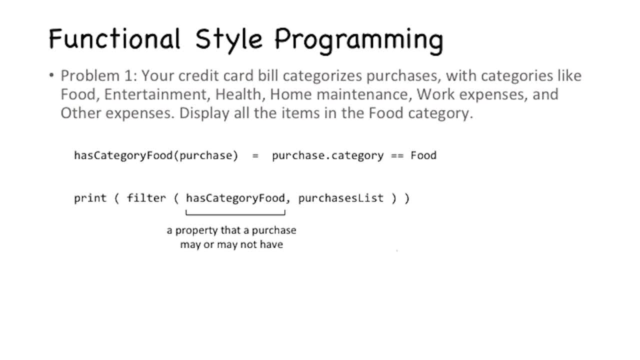 that have the category of food. OK, OK, OK, OK, OK. Of course I have to define another function here And, as you see on the slide, I've already done that. When I call has category food on a purchase. 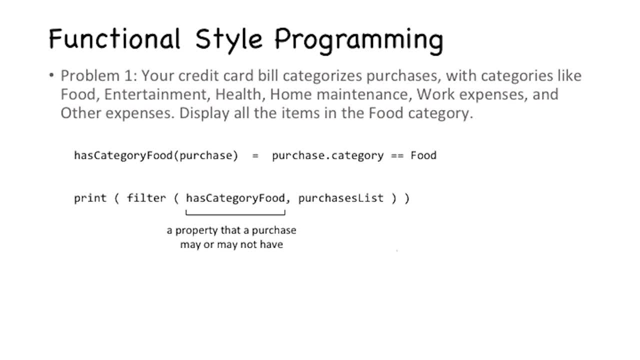 it gives me true or false. Is that purchase's category food Or is that purchase's category not food? OK, Instead of even I have has category food And instead of 4 comma 25, or whatever that list numbers had, I have a purchase list. 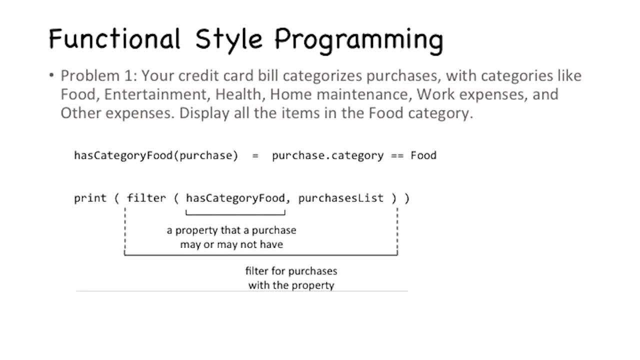 And now what I'm doing is applying the filter function to the property has category food and to the list of purchases, And what I get back is a new list with only those purchases that have the category of food, And to that new list I apply yet another function. 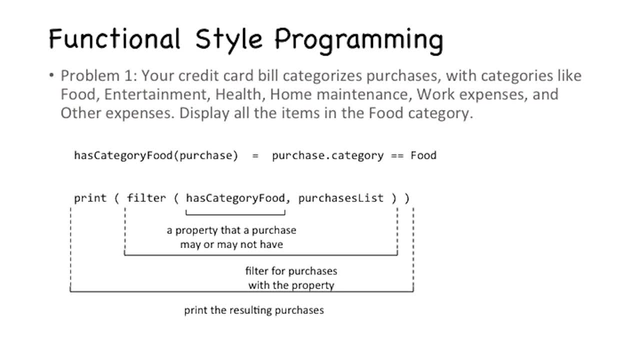 which, in this case, I'm calling the print function. And what that print function does is. it says: take all the elements in the filtered list, the list of purchases with food category, and display the results on the screen. So now what I've got is: I've got a way of solving the problem. 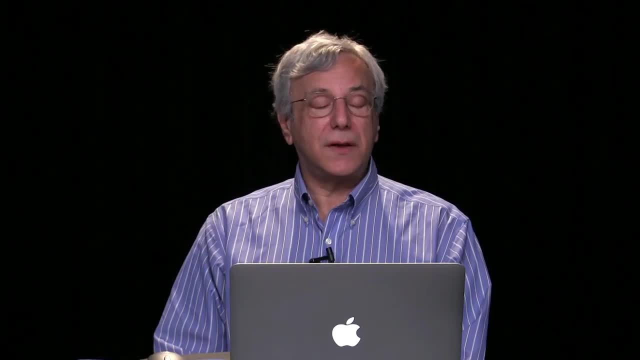 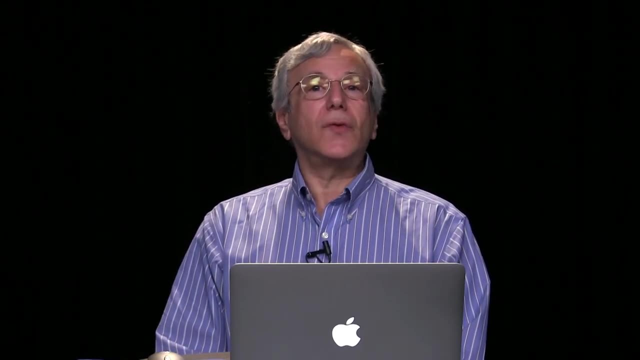 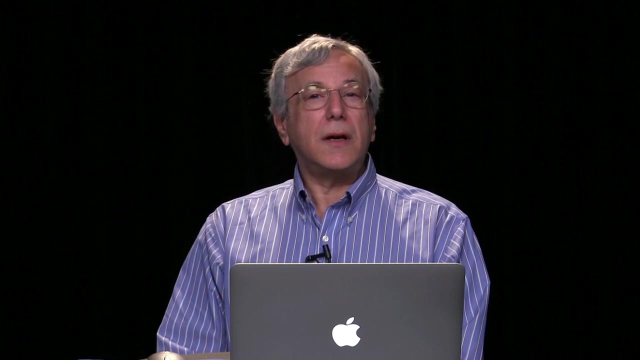 where I'm thinking about it in terms of functions rather than in terms of looping through a bunch of things and choosing: if this, then do that, otherwise do something else. And that's just a brief hint. It's just a brief hint about what we can do with functions. 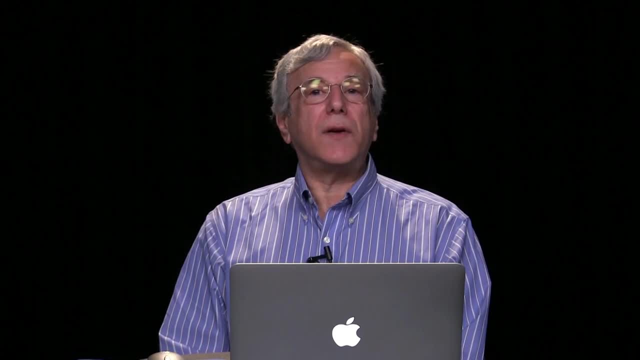 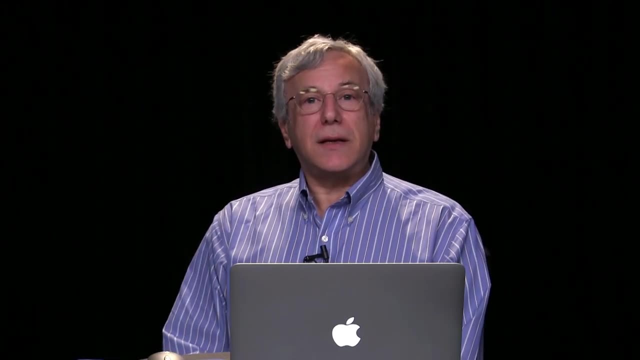 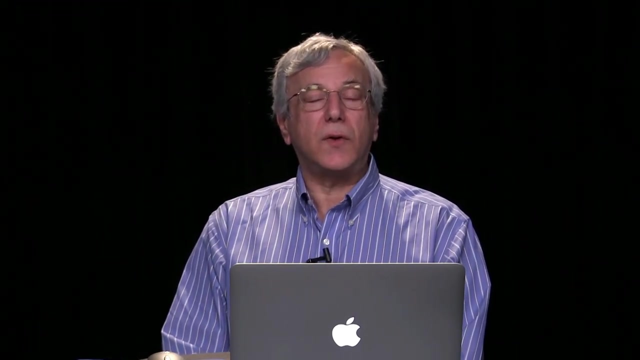 and the way that we can solve a problem with functions instead of solving it with step by step, imperative programming. In the next set of slides, in the next part of the course, we'll refine these notions and talk more about how we apply functions to one another. 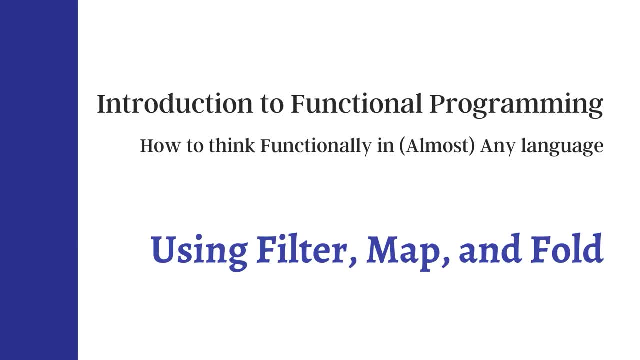 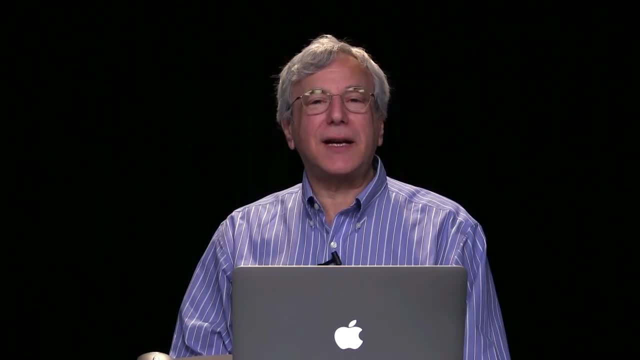 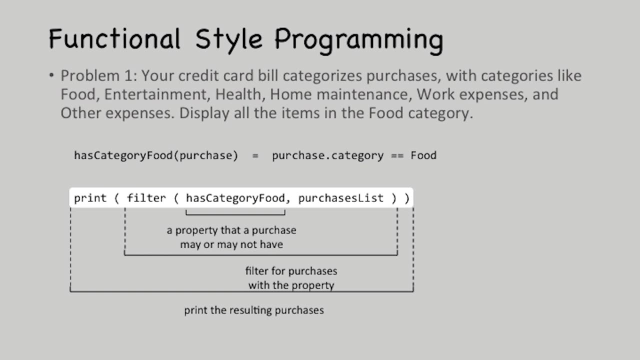 to solve important programming problems. So how will we solve the credit card categorization problem? Let's take a look at the slide that we finished off with in the previous segment. We have a filter function. We apply it to two arguments. the has category food function. 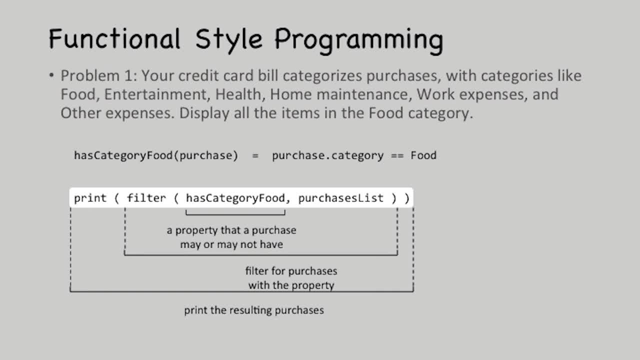 and the purchases list. When we've applied the filter function to those two arguments, we get a brand new list, a list of purchases whose category is food. Then, to that result, we get a new list, a list of purchases whose category is food. 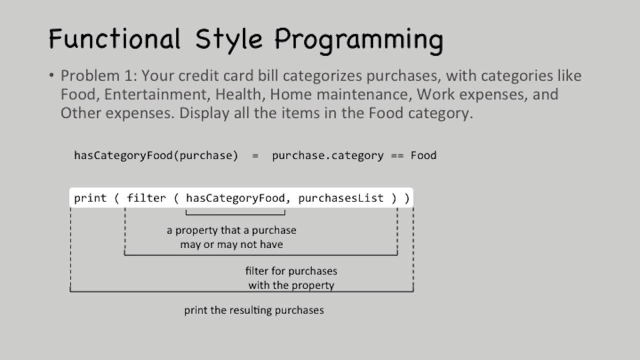 Then we apply the print function. What I didn't talk about in the previous segment was this: has category food criterion: Has category food. one student asked me during one run of this course: is that built into a language? No, it can't possibly be built into a language. 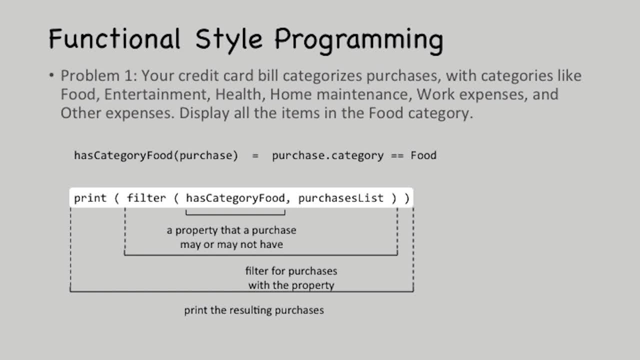 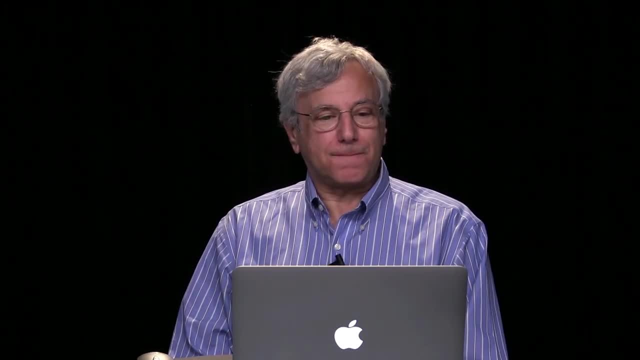 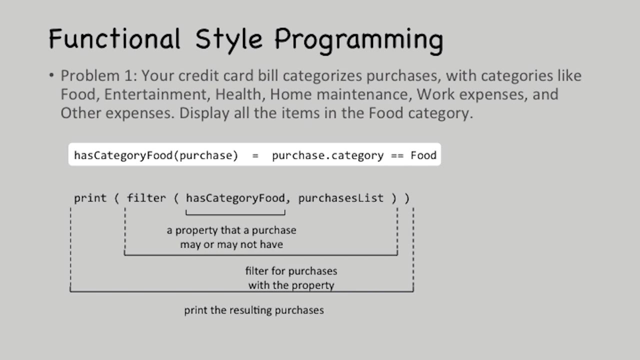 because languages don't have special functions for food. So what we have to do is define a function, to define a has category food function. So what I'm going to define- and I define it just above the place where I solve the problem- is I'm going to define a has category food function. 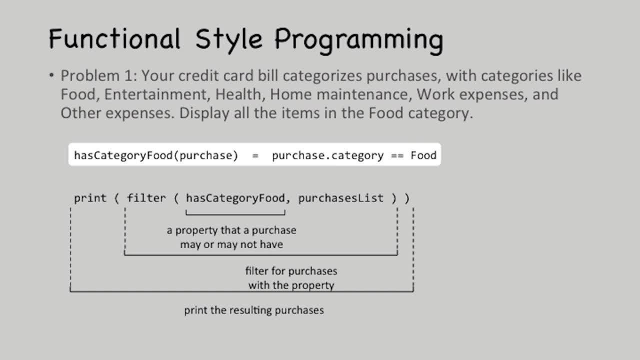 and it applies to an argument which I'm calling purchase And the value of has category food. purchase is true if a particular purchases category is food and false if a particular purchases category isn't food. So now, instead of a one line program, I really have a two line program. 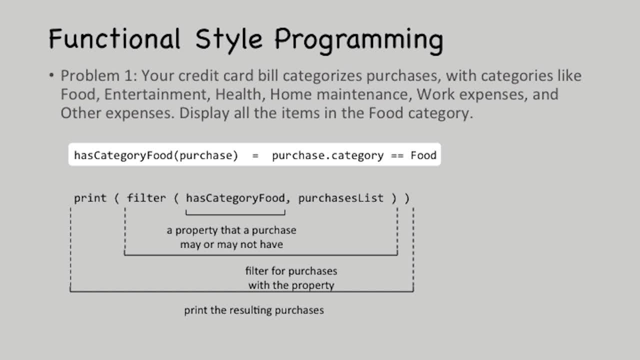 It would be handy to be able to turn it into a one line program. Not because we don't like typing and not because we want our programs to be as short as possible, but because if we can turn this into a one line program, it represents a facility, a dexterity that we have. 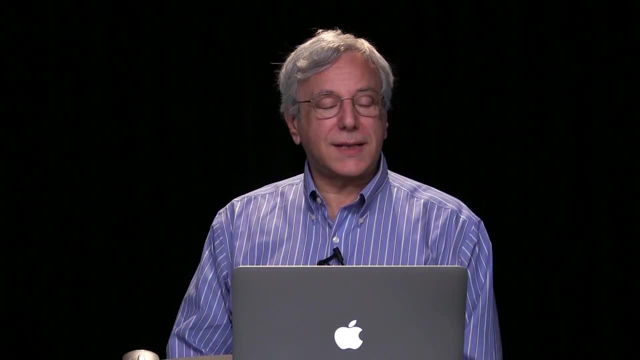 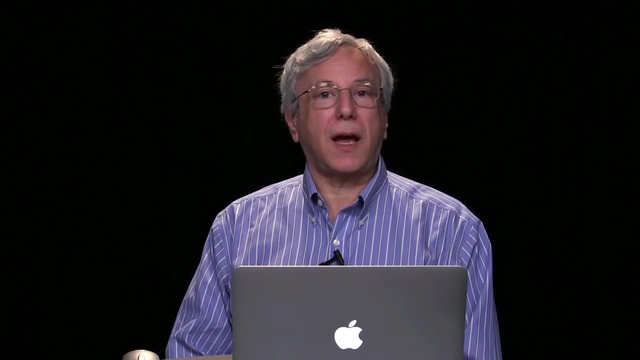 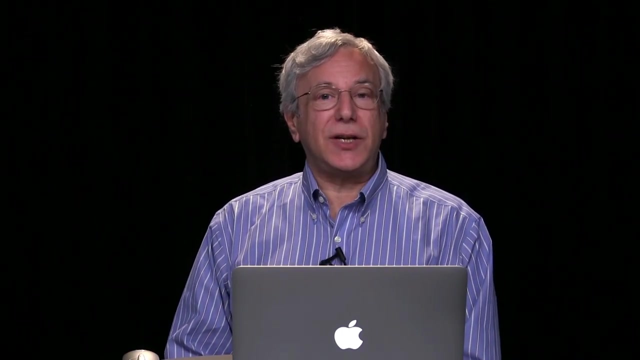 with functions That will be useful later on. Let's take a look at a new way of defining the has category food function. Remember that our new way of defining the has category food function will define the same has category food function. We'll simply be using a different notation to define it. 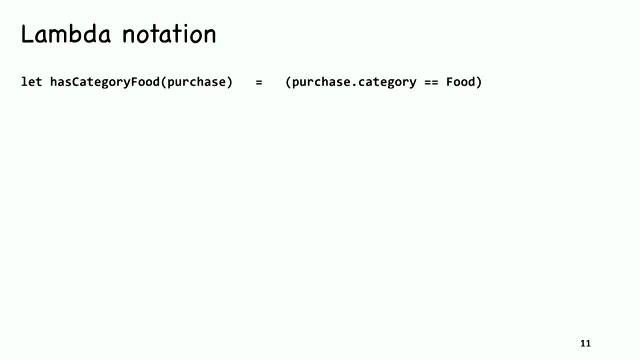 Here's the way has category food normally looks when it's defined. I'm going to let: has category food purchase equal, true or false, depending whether the purchases category is food or isn't food. That's sort of standard notation. It's the notation that you might have seen in a mathematics course here and there. 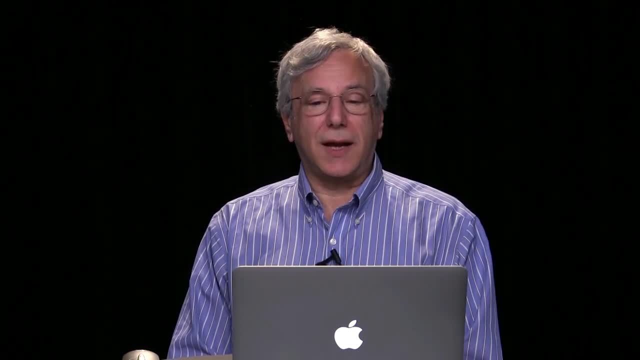 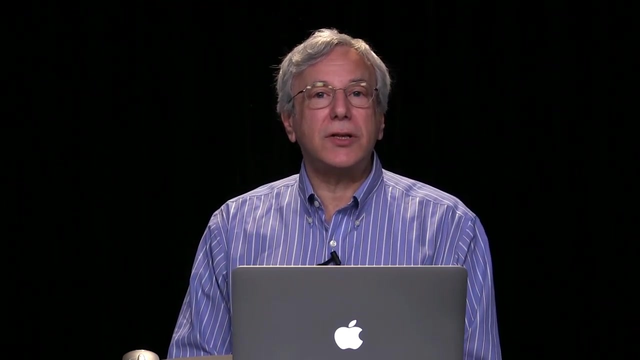 And it's certainly a notation that you can use in certain programming languages. Well, there was a fellow in the 1930s named Alonzo Church who defined what he called the lambda calculus. Lambda is a Greek letter and the lambda calculus uses a slightly different notation. in order, 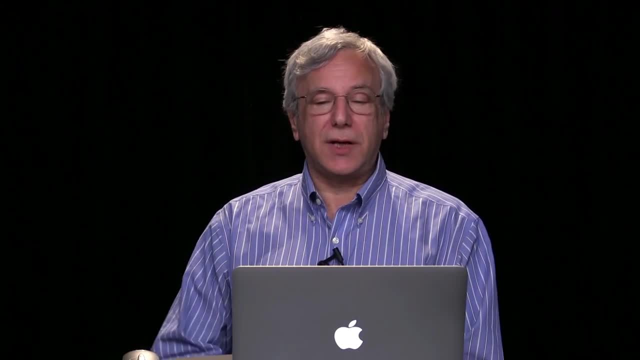 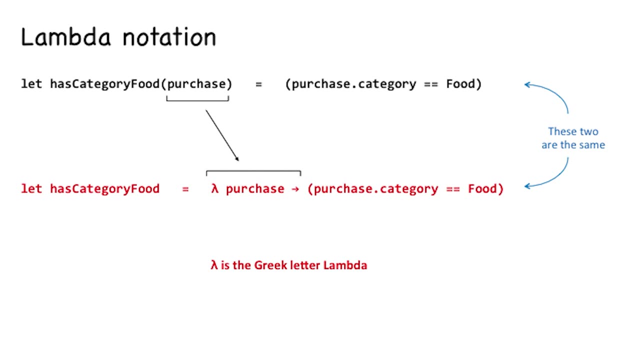 to define a function Turns out to be a really useful notation for our purposes. Here's what it looks like: Instead of saying has category food parentheses purchase, I'm going to say let has category food equal. I'm going to move the word purchase- the argument- to the other side of the equal sign. 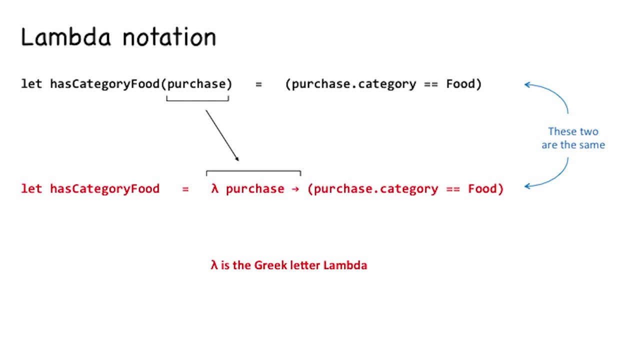 And it's going to simply say lambda, purchase arrow and then, of course, purchase dot. category equals food. The equation I read defines exactly the same function as the notation in black. The only difference is that now the word has category. food is the only thing on the left. 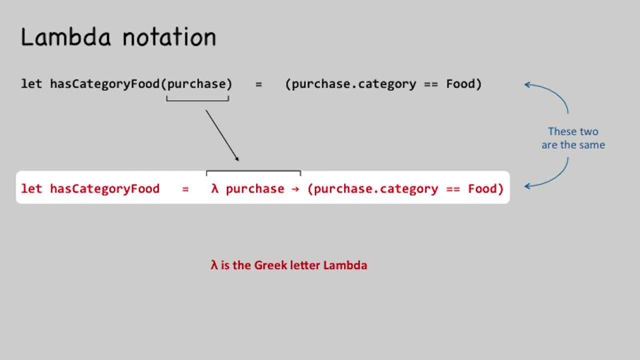 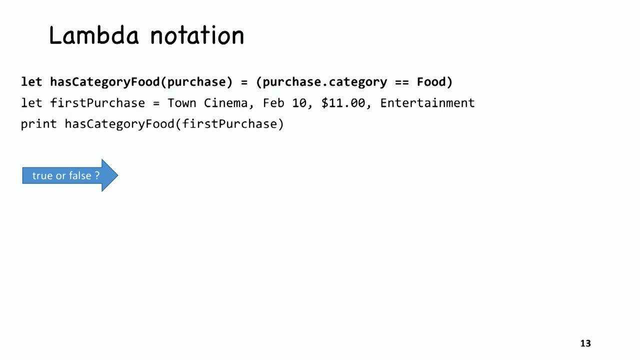 side of the equation and everything else is on the right-side of the equation. What in the world does that gain us? What does that gain us? We start off with: Has category food purchase equals东 purchase? dot category food dużo нет defined the way we see it in most programming languages. 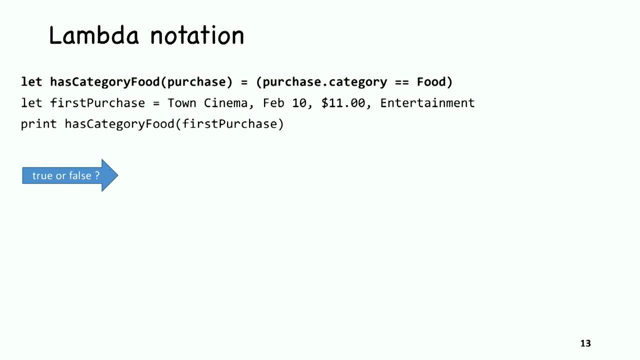 or in a mathematics course, And then we let first purchase be town cinema, so on and so forth- entertainment. If I decide that I want to print, has category food applied to first purchase? I'm not gonna get the word true, because that first purchase is entertainment and 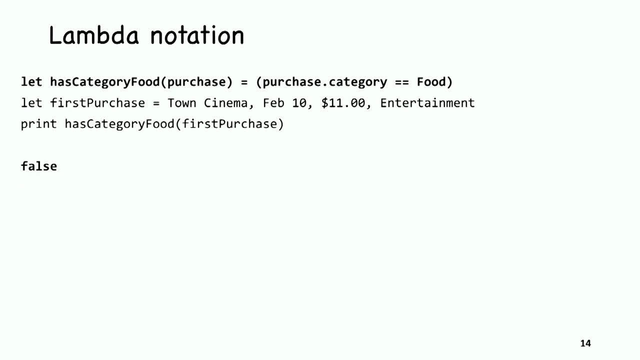 not food. so I get the word false. Okay, fine, No big deal. Let me change my notation a little bit and instead do the same three lines but use lambda notation. The first three lines and the second three lines are exactly the same in meaning. 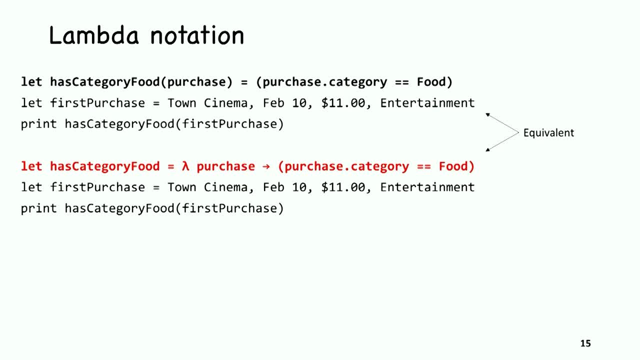 I've used a slightly different notation to define what I mean by has category food, but those two groups of statements do exactly the same thing. I still, when I asked to print has category food, first purchase, get false because that first purchase is for entertainment, not for food. So far, 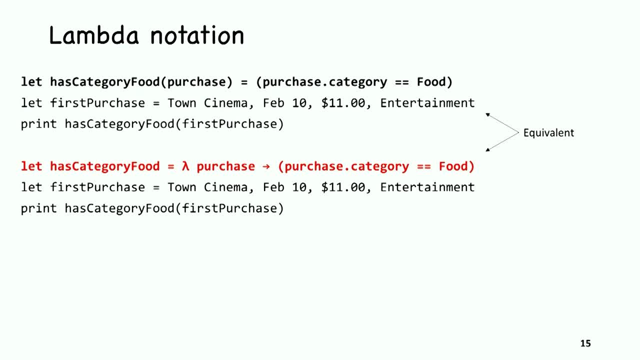 I haven't gained anything by using lambda notation. When can I gain something? Let's take a look at one more version of these statements. In this case it's two statements, not one. And again, we're not trying to save typing here, We're trying to begin with a. 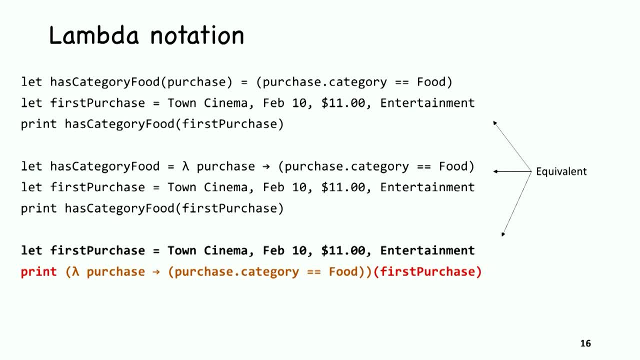 function. We're trying to become more dexterous with functions. In the third version of this mini program, I'm defining what I mean by has category food in exactly the same text as I'm using that definition. And that's the power of lambda notation. 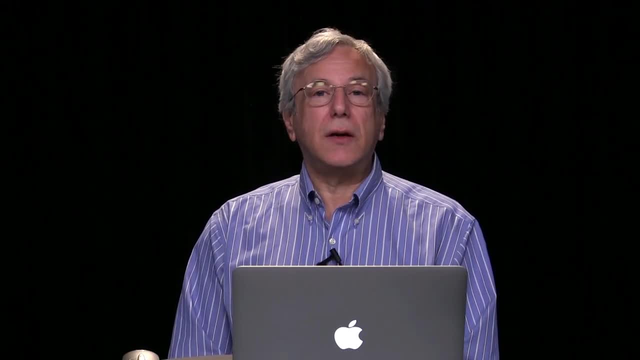 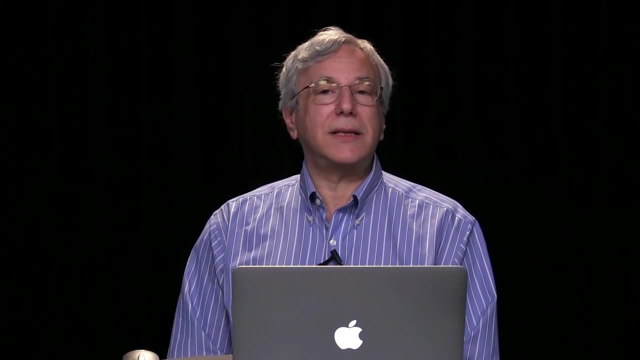 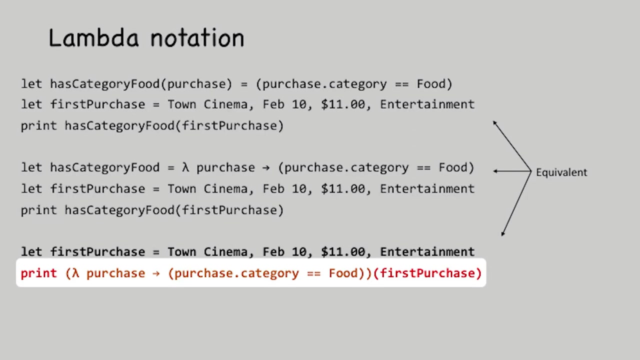 It allows me to define a function and use it all in one fell swoop. So now I've got two lines instead of three. Big deal- Not necessarily saving typing- Yes, saving typing- But the big thing here is that I have more agility with functions. 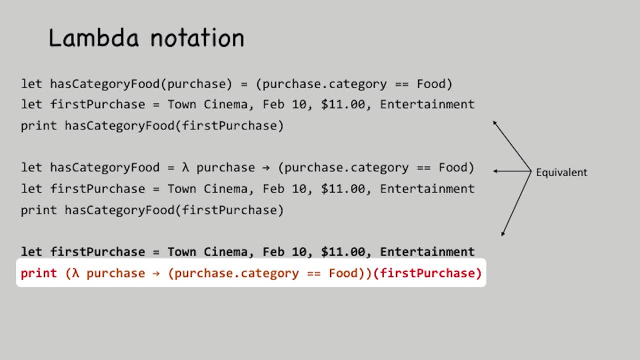 because I can define it and use it in one step and therefore apply it very facilely, very easily, to a print function. So I'm printing now the result of this function, which used to be called has category food. Now it doesn't even have a name. 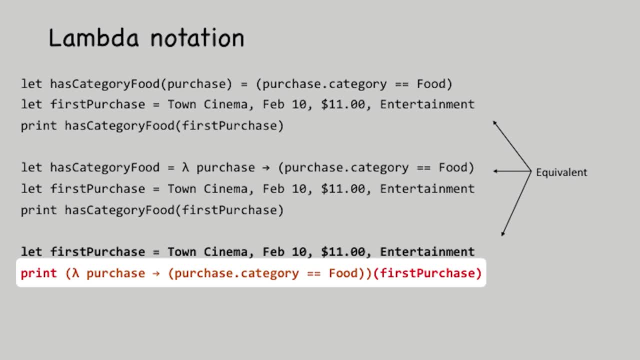 Now it's just a lambda expression And I'm applying that function to first purchase and then printing it all on one line. Cool stuff. Let's take a look at the credit card categorization problem once again and see how to use lambda notation in order to make our problem. 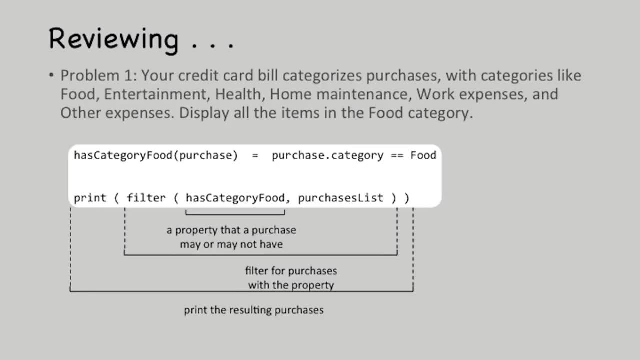 more functional. perhaps Here's the way we were doing it in an earlier slide. We defined a has category food function, We applied it to a purchase, We filtered with the has category food function and a purchases list and got a new list with only those purchases that had the category food. 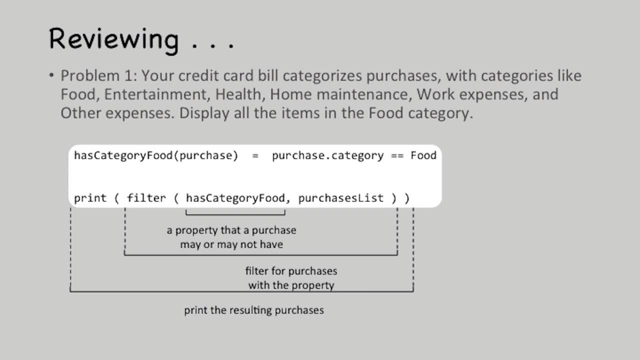 And then we printed that brand new list. Well, using lambda notation, we don't have a separate line to define the has category food function. We create a function with out a name on the fly, in place of the words has category food in the program line. 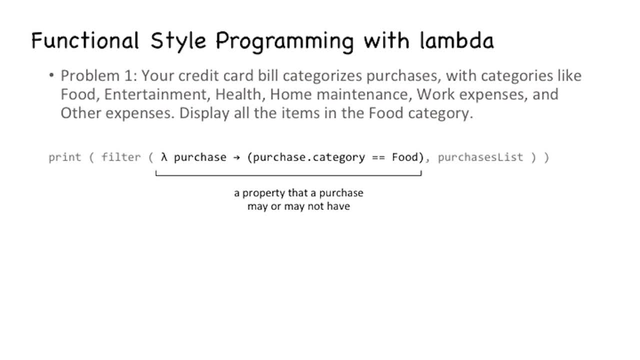 Let's take a look On one line now. we anonymously define a function that does the work of defining, yes, a particular purchase has category food or no. a particular purchase doesn't have the category food. Without naming that function, we apply it to a list of purchases. 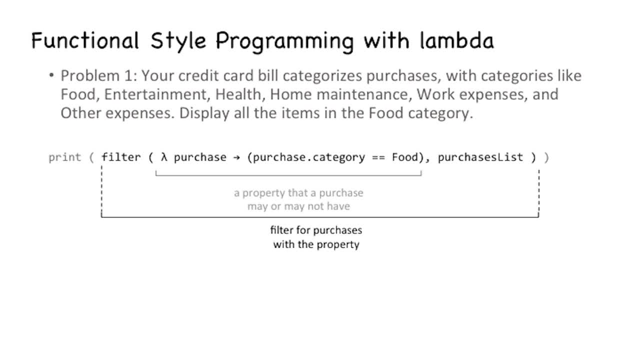 and filter for only the purchases that have category food, and then, once we've got that filtered list, we apply that new filtered list to a print function, which then displays the results. Now we've used lambda notation to be able to create functions quickly on the fly and use them immediately as we define them. 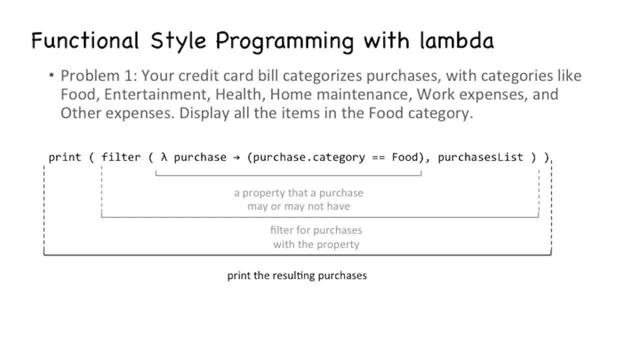 them without having to give them a new name. This is very powerful notation and it's used throughout the functional programming world. Okay, we've categorized purchases and displayed those in the food category. What else can we do? Typically, we don't want to just see: well, what are the purchases in the 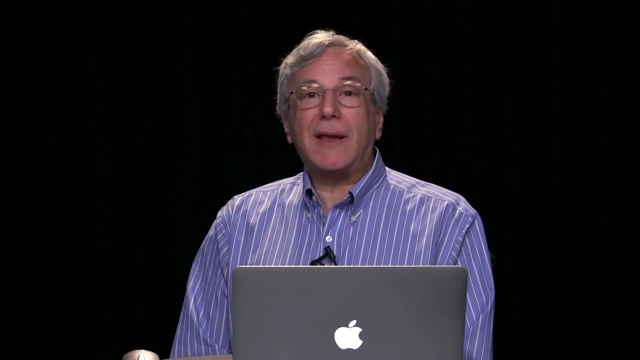 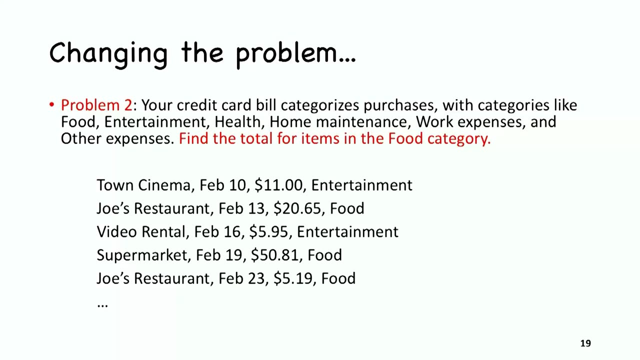 food category. We may want to do something like: add up all the prices, all the amounts for those purchases. That's going to be problem two. So in problem two, your credit card bill categorizes purchases, categories: food, entertainment and so on and so forth. Find the total for the items in the food category. How? 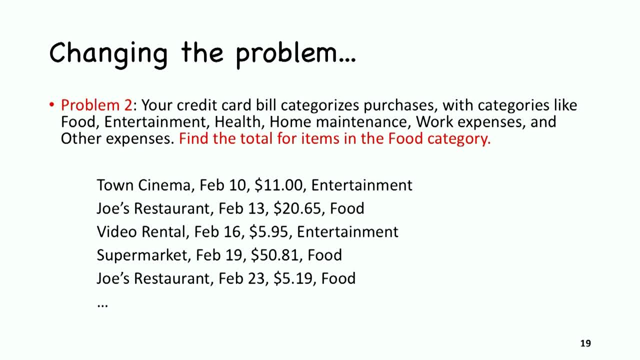 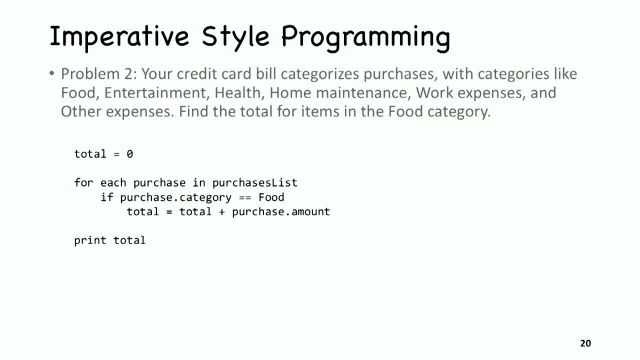 can we solve this problem by thinking functionally? First, let's take a look at the imperative style for that problem. We would have a total. We would start by setting the total equal to some initial value. We would go into a loop, We would go into an if statement- Each. 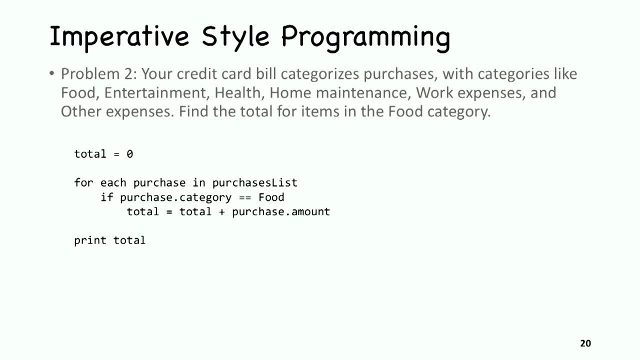 time through the if statement, we would change the value of the total. I emphasized the word change. We would change the value of the total, because I'm going to be talking about that in a later segment. We change the value of the total each time through the loop, Maybe depending on whether the purchases 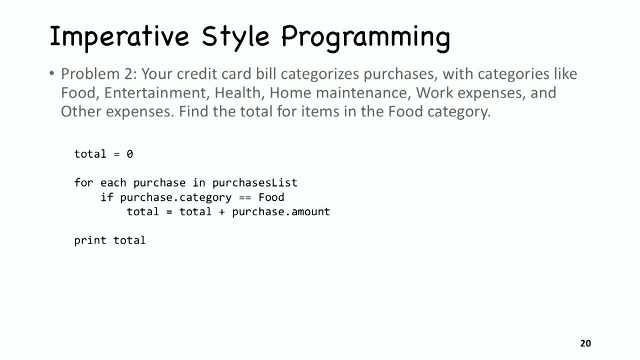 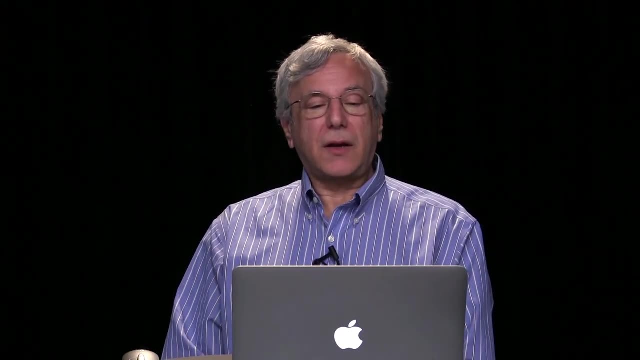 category is food or not. And then, finally, when we loot through our of the purchases, we print the value of the total. That's the imperative style for solving the problem. Let's look at the functional style. In order to appreciate the functional style, we have to look at a brand new kind of function. 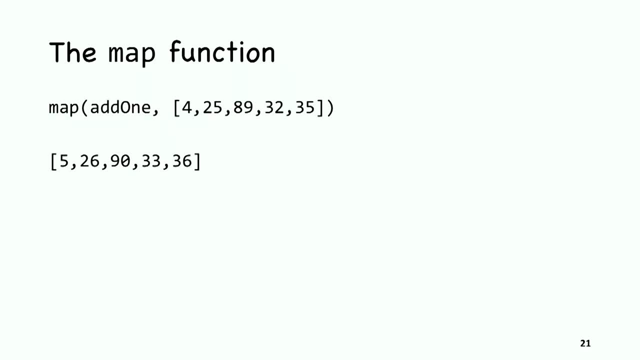 a function that I'm going to call map. Again, some languages call this map. other languages have different names for it. I'm going to introduce the map function by showing you what it does with numbers. So let me take a list: 4,, 25,, 89,, 32, and 35. 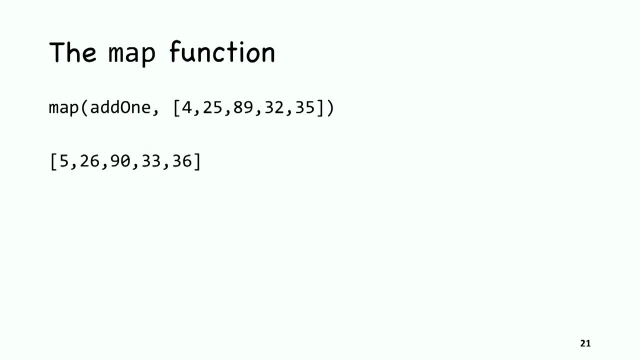 and apply to that list. an add one function, An add function, one function- again- it's a name that I made up- is going to simply add one, increment any number that it sees. So when it sees four, it turns it into five. When it sees 25, it turns it into. 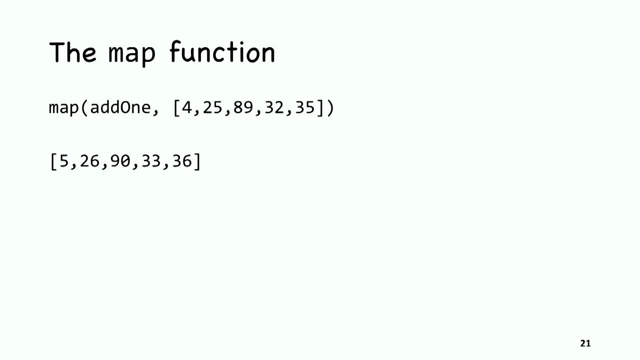 26.. The idea here with the map function is: the map function is a function that takes two arguments. One of them is a function like add one, a function that acts on numbers, and the other is a list. And what map does is it takes the. 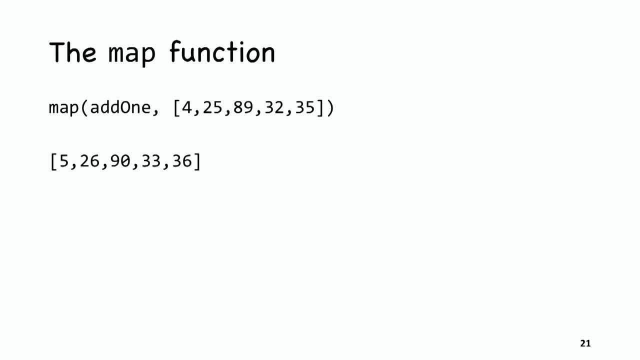 function- that is its first argument- and it applies it to each element in the list. that is its second argument. So map takes a function like add one and a list like 4,, 25,, 89, and so on and gives you back a brand new list And in 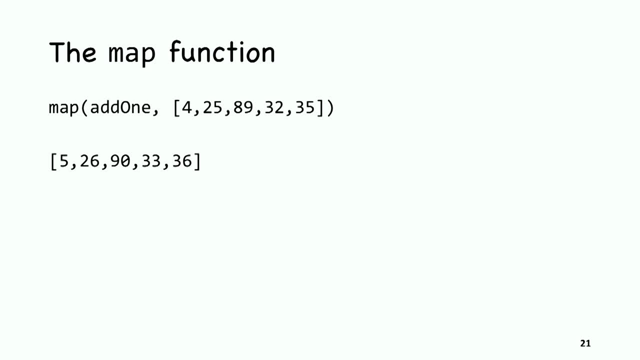 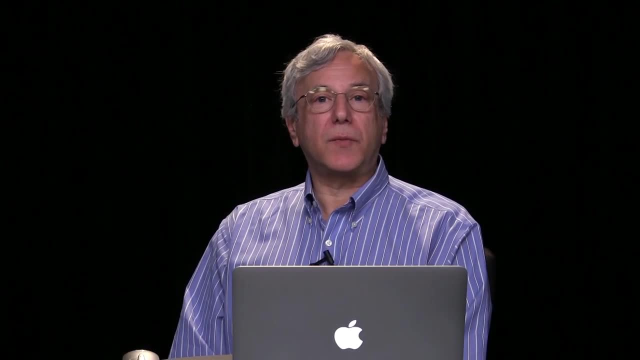 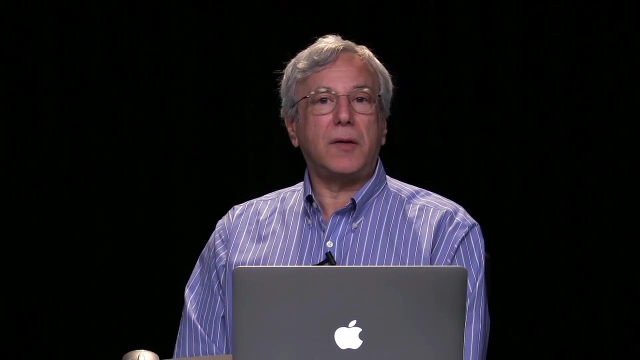 this case, the brand new list is 5,, 26,, 90,, 33, 36.. Now you may have heard of something called map reduce. Map reduce is a particular way of solving problems that's very useful and very commonly used in processing these days. Map reduce the map. 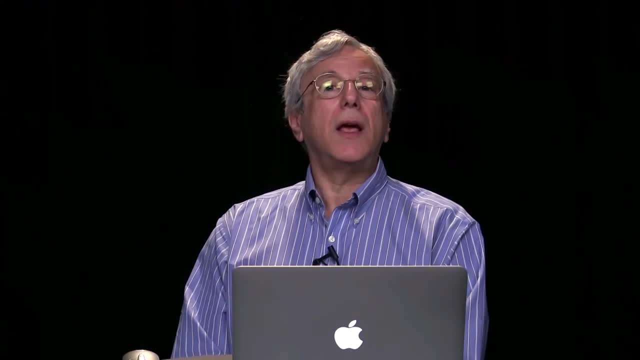 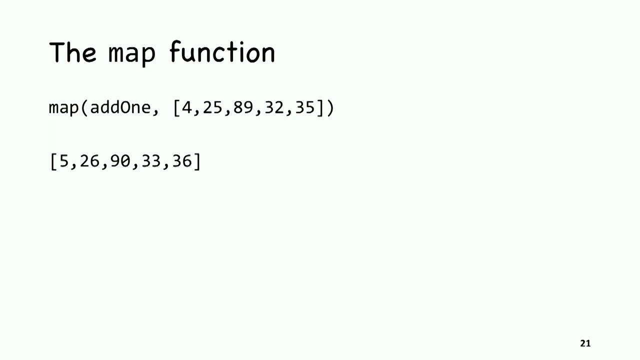 in map reduce is exactly this kind of thing- a map function- And the reduce is something that we'll see later on in this segment. So now that we have the map function down, let's take a look at the way the map function is going to help us. 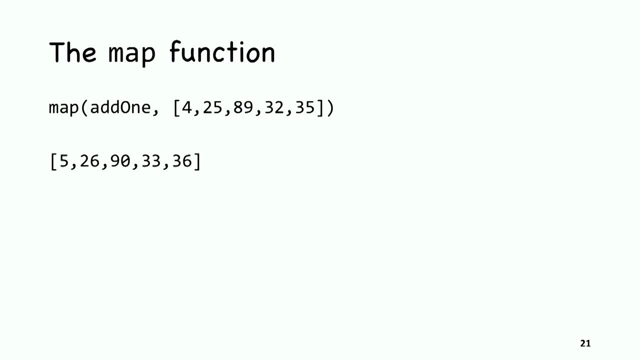 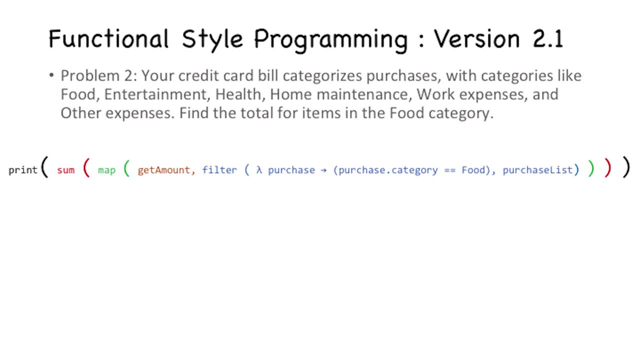 solve the credit card categorization sum problem. Nice colorful slide, Thank you. So once again, I've made sure that I've applied here and I made sure that the parentheses are size so that you can see where everything starts and ends. Once again, I'm going to filter and I'll use the lambda version of the has. 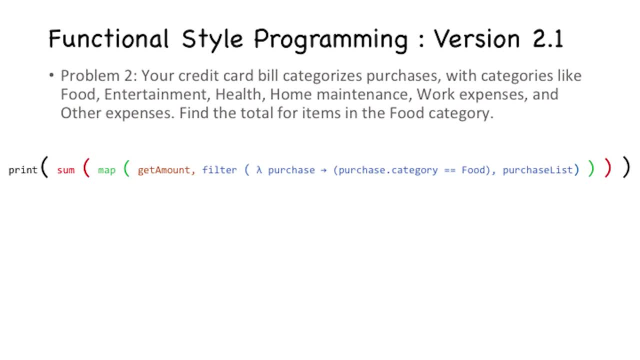 category food function because, hey, that's nice to use. So first thing I do is I filter the purchase list for purchases whose category is food. That gives me a brand new list. Elements is a purchase whose category is food. Then I apply map with a function that I'm sort of. 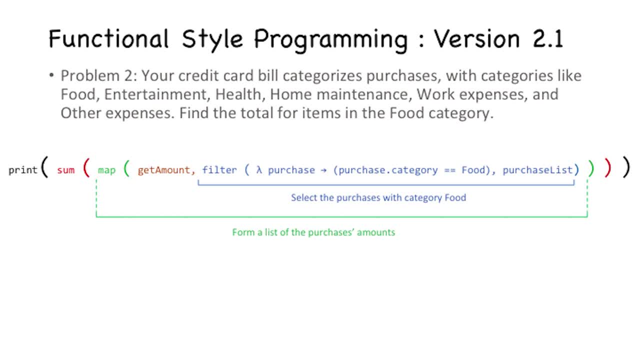 making up here on the fly- I hope you'll be OK with that for just a moment- a get amount function And the get amount function that I'm defining here. admittedly I'm cheating a little bit, but my get amount function is sort of temporarily a function that. 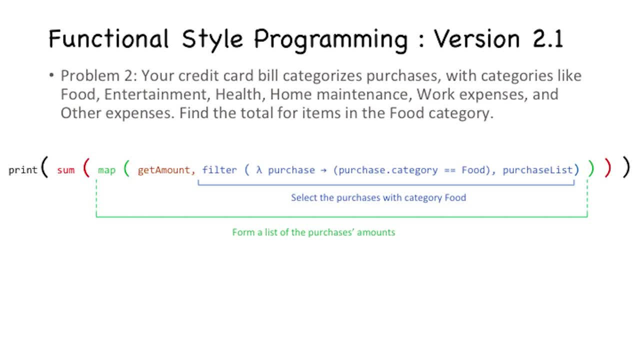 says, take each element in the list and sift out only the amount of that purchase. Well, actually the get amount function applies to one purchase at a time. When I call map with get amount, then the effect is to apply the get amount function to each element in the. 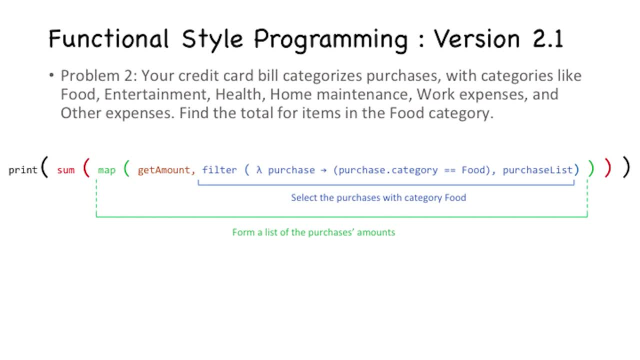 filtered list. So what I end up with in green in this slide is a list of not purchase, But a list of the amounts of purchases. And now I've used the map function with its friend function, the get amount function, in order to go from: 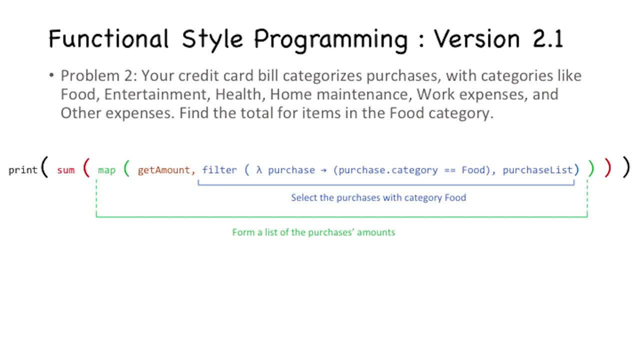 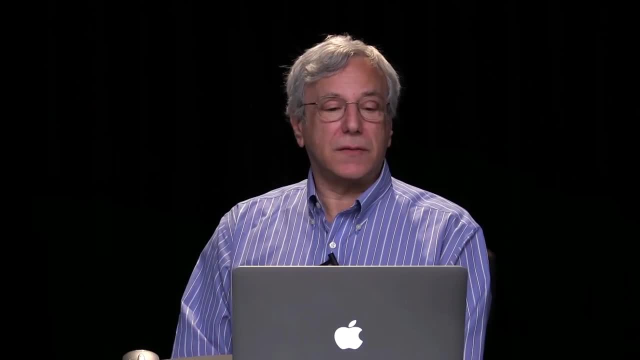 a list of purchases to a list of amounts. Once I have a list of amounts, I can apply what you'd imagine exists in a functional programming language- a sum function. And what the sum function does is: it takes all the amounts, adds them together. 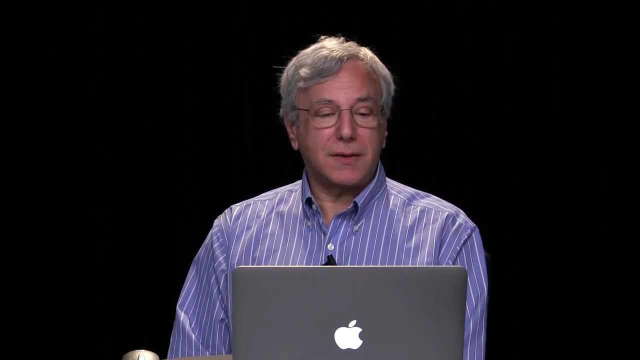 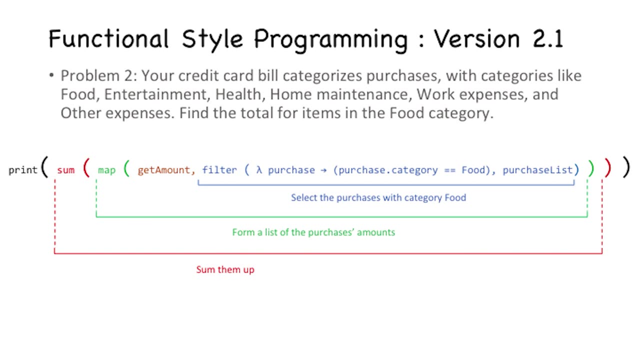 Great, Wonderful. Now I've summed up all the amounts. Before I did that, I made sure to sift the amounts out of the purchases list. Before I did that, I made sure that the purchases list was a list of food purchases and not of entertainment or work. 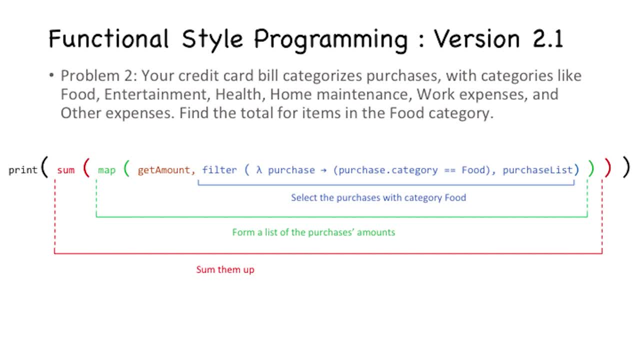 purchases And once I have that sum I can apply that sum to the print function and display the result. I've done a lot of work just by thinking about function application and not by thinking about steps in instructions like: do this, do that? 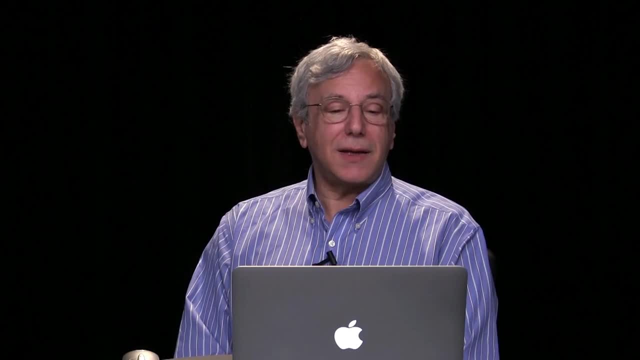 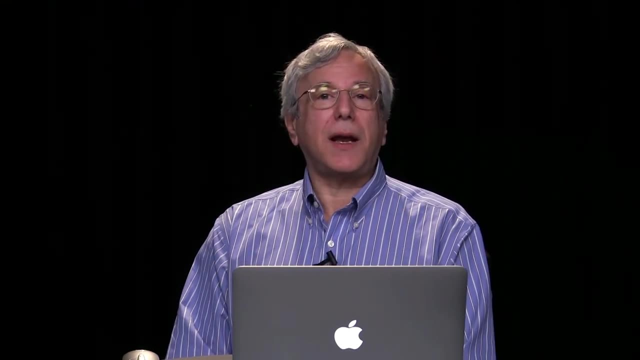 OK, what I have to do is fix that get amount, because that get amount is a function that came out of nowhere And, as you can imagine, a programming language isn't going to have a get amount function, because a programming language isn't going to necessarily be about purchases. 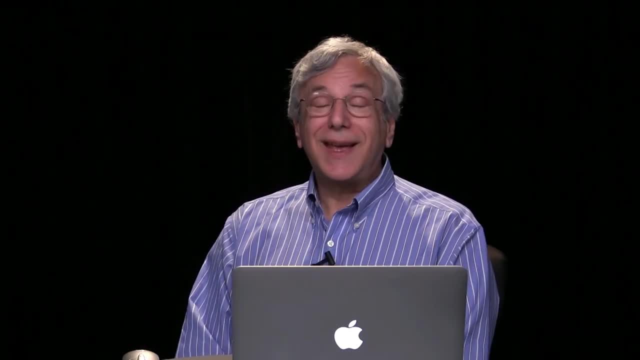 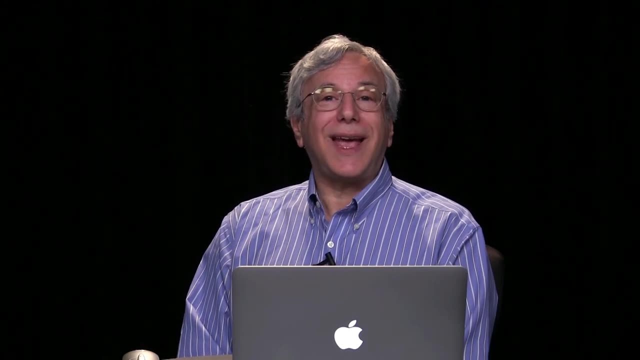 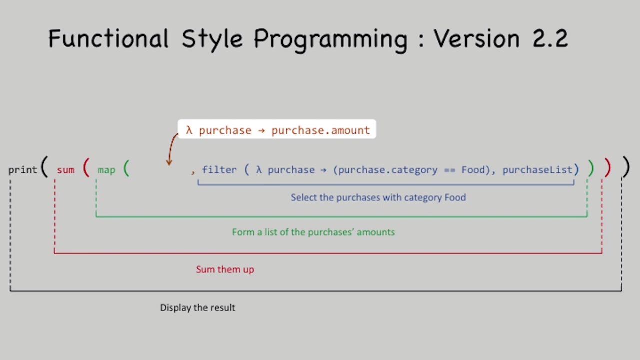 So I have to define the get amount function. Aha, since I've created my lambda notation, I can pretty quickly and easily and dexterously define what is the amount I want to buy. That's a number, my get amount function, and here's the way I do it. I take a purchase and to that purchase. 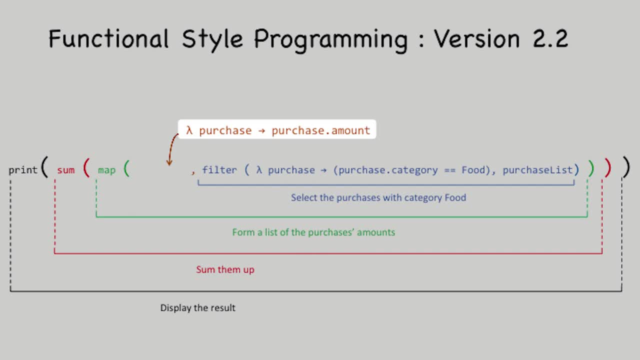 I apply a function that simply grabs the amount of that purchase, and now I don't need to define a new function with a name get amount. I just take that lambda expression and I insert it in place of the get amount words that I had in the previous slide. Now I didn't have enough room to actually 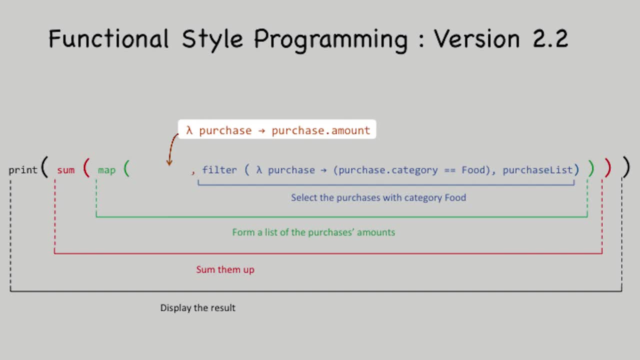 insert it. so I just put an arrow in this slide. but imagine that this is all one line across, or just one application of function to another function's result, to another function's result, to another function's result. Basically, what I've done now is I've applied a collection of functions, a sequence. 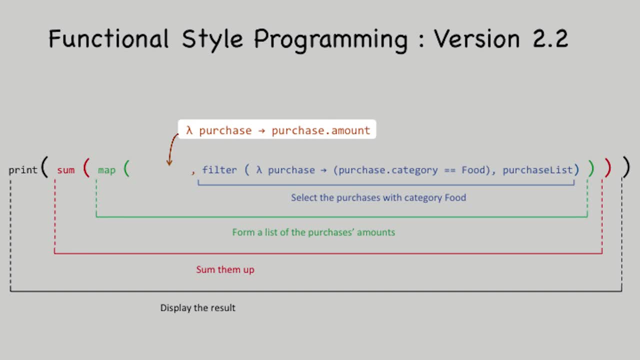 of functions, a bunch of functions to solve a common programming problem. Okay, what else can I do with this? I know Let's take a look at the stuff in red, The word sum. Can I improve on what's there? Well, any. 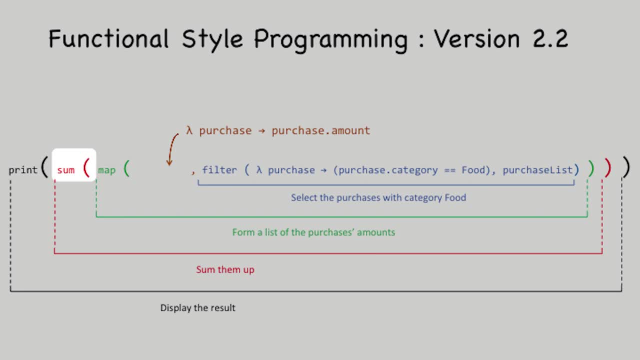 language worth its salt, whether it's a functional language or some other kind of language, is going to have some notion of addition, and so it's not really out of the way for me to think that a functional language will have a sum function, a function that adds each element in a list of. 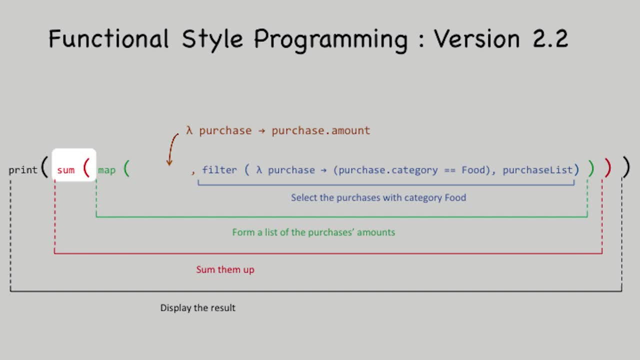 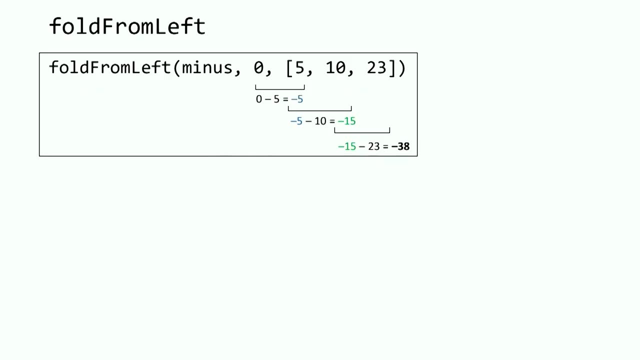 functions together, if those elements can be added together, and comes up with a total. But maybe I can do a little bit better than that. Let me see what I can do. I'm going to define something called fold from left. In this course I'm going to be going to be defining one function after another function. 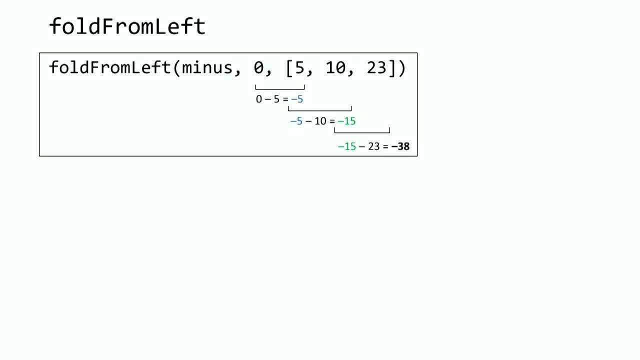 after another function, and in this case I'm defining something that I'm going to call fold from left. Again, the name will be different in a particular functional language that you're using, but I think it's Fridayちゃん. 從東视でもできる口口訳可以說。. 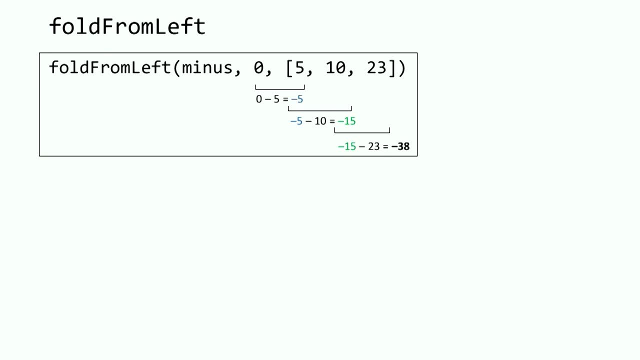 think it's a handy way of naming it. to call it in my pseudo language: fold from left. And what fold from left does is it applies a particular operation to successive elements of a list. So what I'm going to do here is take a function. 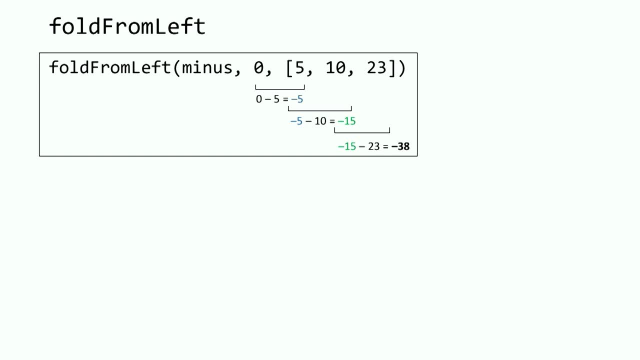 that I'm calling minus a subtraction function and I'm going to apply it between 5 and 10, and apply it between the result from 5 and 10 to the number 23.. Well, wait, a minute. Wait, I have to have a starting place, right. 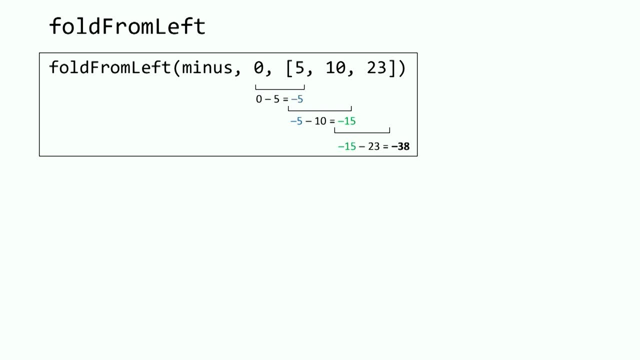 I can't just apply it between 5 and 10.. I have to know what I'm starting with. So that's yet another argument to the fold from left function. The fold from left function, as I define it, has three arguments. 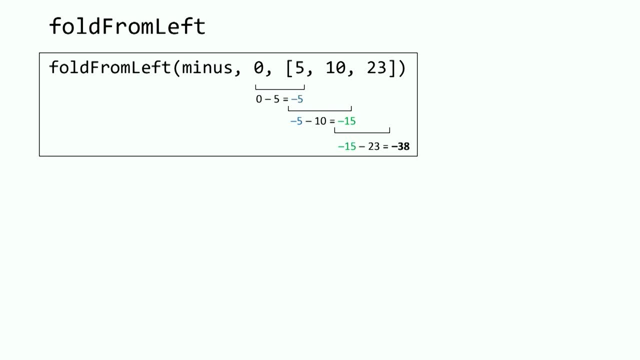 The first is a function like minus, an operation, if you will. The second argument is a starting point like 0.. Start with 0 when you start folding from left. And the third argument to the fold from left function is always going to be a list of numbers. 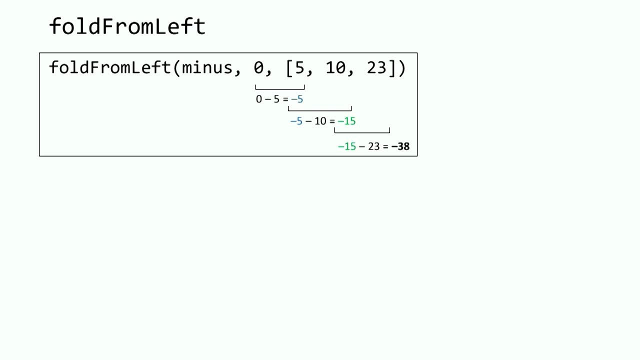 So, as you can see here, when I apply the fold from left function to the three arguments minus 0, 5, 10, 23, what I get is subtracting 5 from that initial value 0, getting minus 5.. 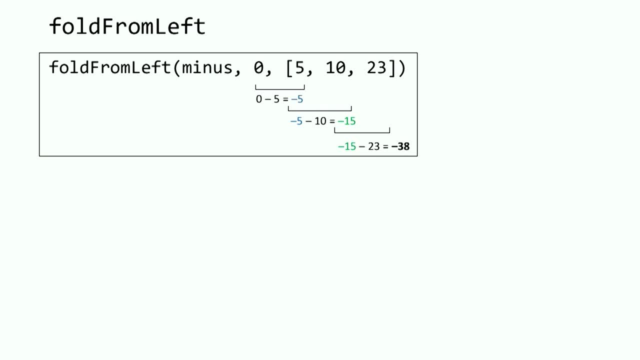 Then subtracting 10 from that minus 5, and getting 15.. And then subtracting 23 from that minus 15 and getting 38.. That's the fold from left function. Well, wherever there's left, there's right. So how about a fold from right function? 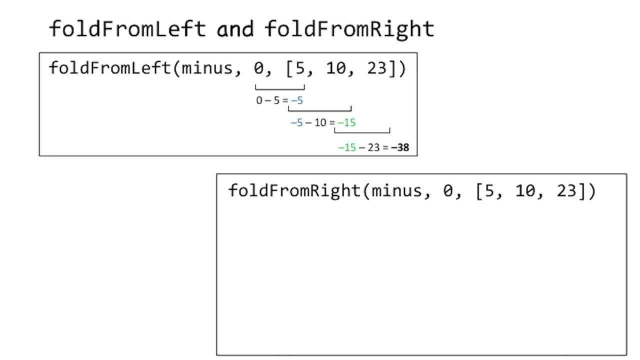 Let's see what that looks like: Subtraction. Subtraction isn't commutative. That means when you subtract two numbers, if you subtract them in the opposite order, you don't get the same result. And what that means is, when I call fold from right, minus 0,, 5,, 10,, 23,. 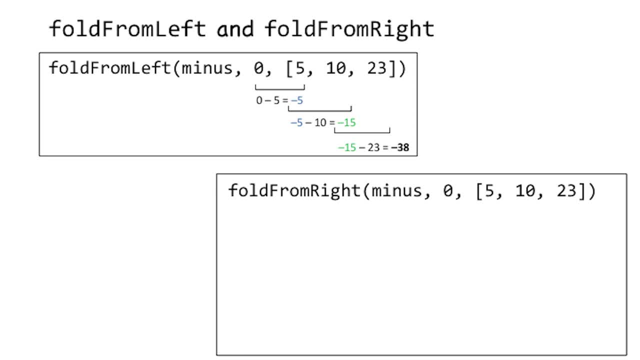 I get a different answer than when I call fold from left. So here's the way I'm defining fold from right. I'm again going to have an operation like minus. I'm going to have a starting point like 0.. And I'm going to have a list like 5,, 10,, 23.. 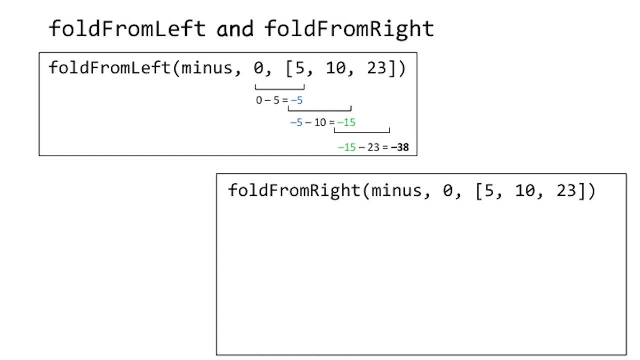 But this time what I'm going to do with that starting point 0 is I'm going to think of it as being on the far right end of the list And I'm going to apply that minus operation between successive numbers starting with 0.. 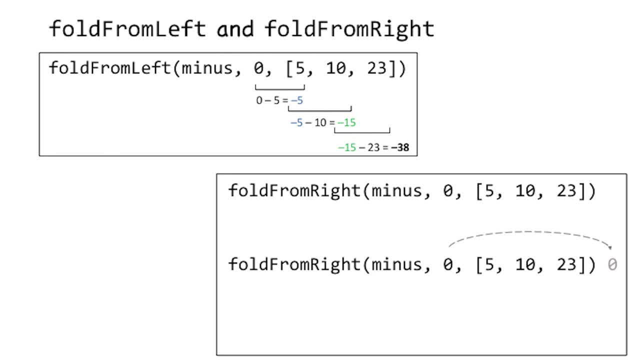 And this time, though, I'm going to start from the right end of the list, subtracting 0 from 23.. And once I've got 0 subtracted from 23,, I'm going to subtract that result: 23, from 10. 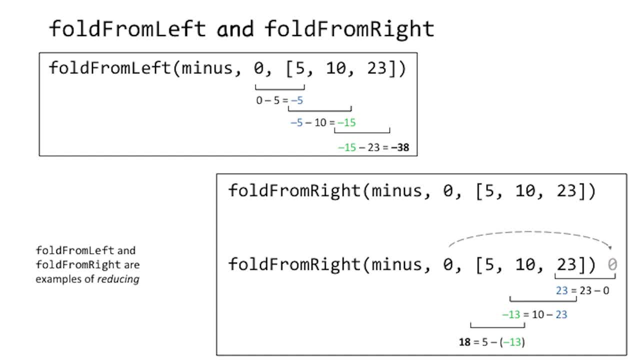 to get negative 13.. And then, when I get negative 13,, I'm going to subtract that from the next value 5, and I'm going to get the value 18.. Applying fold from left to minus 0, and then this list: 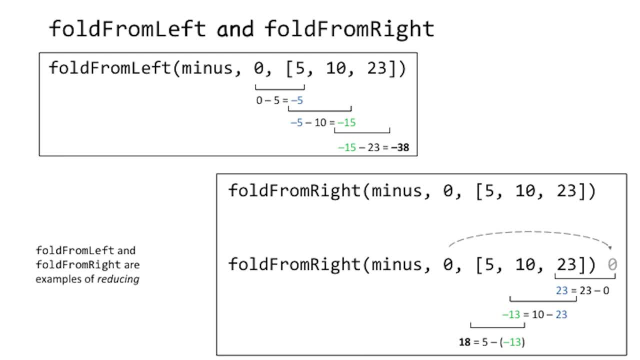 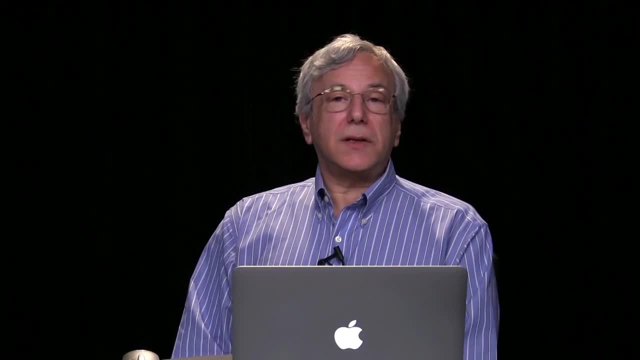 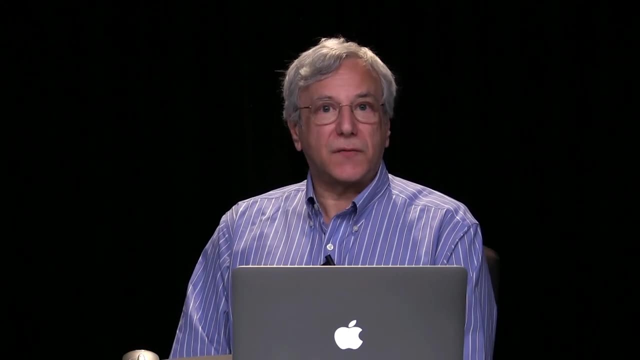 gives me a different answer than when I apply fold from right to minus 0 and this list. When we use the fold function in this course, we'll almost always be folding with a sum function, with a plus function, not with a minus function. 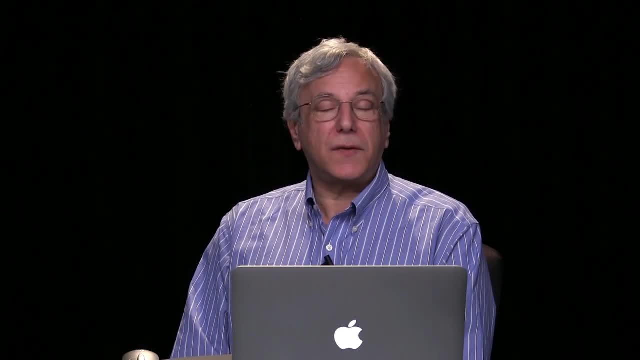 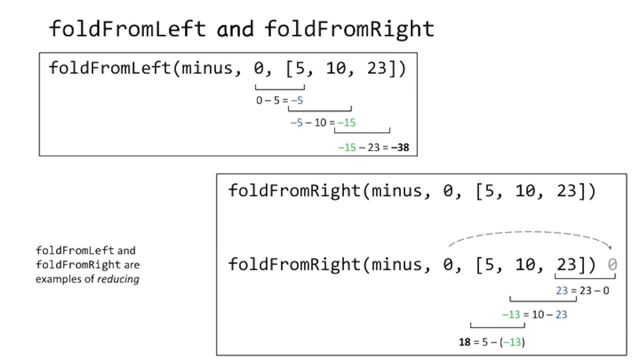 So we won't have to worry about the difference between fold from left and fold from right. So if you're not thinking exactly about fold from left versus fold from right, then you're going to have to think about fold from left versus fold from right in this slide. 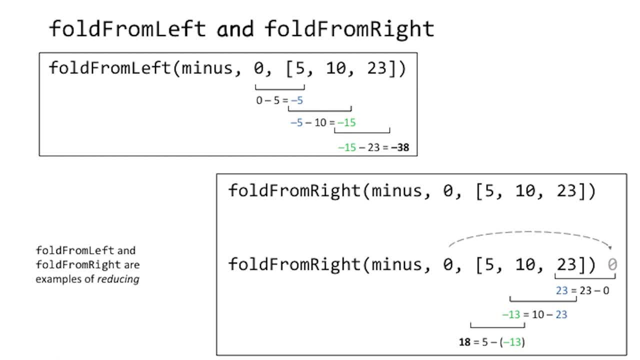 If you're worried about remembering how each of them goes and how each one is different from another, don't worry too much about that. Just make a mental note that folding from one end of the list is potentially different from folding from the other end of the list. 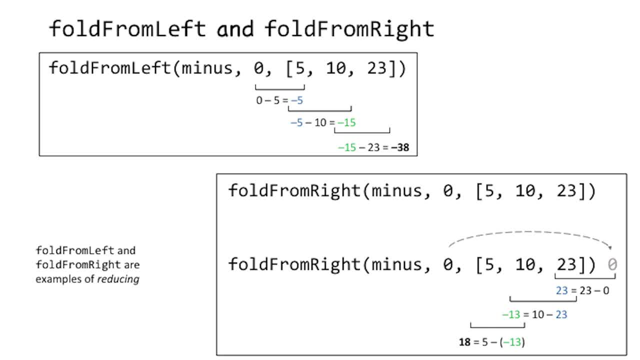 Now, the thing to remember is that the fold from left or from right operation one way or another, accordions the list together and applies a particular operation every two elements of the list. I just want to mention before leaving this slide that fold from left and fold from right. 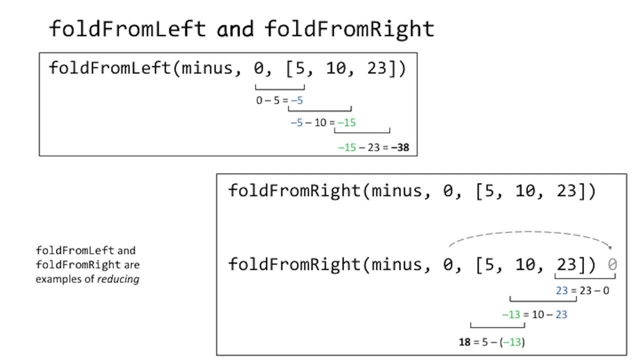 are examples of what's commonly called reducing, which means that now you know when you hear the words map reduce as a way of solving problems. you know basically what map reduce means. All right, I'm going to now apply: fold from right or fold. 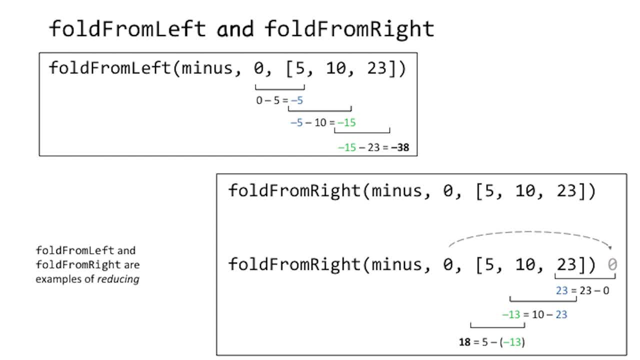 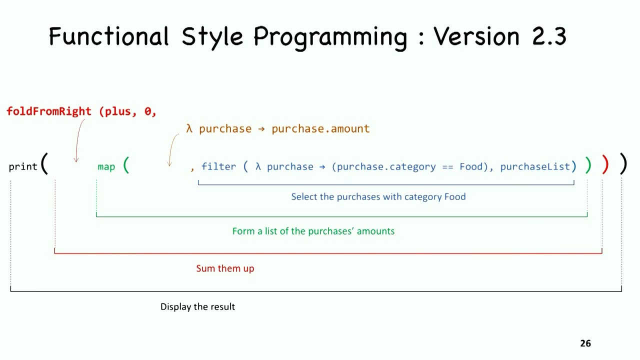 from left To solve the problem where I sum up the values of the food purchases in a credit card bill. If you remember, in the previous version of my solution to this problem I had the word sum there in red, where now I have fold from right plus zero. 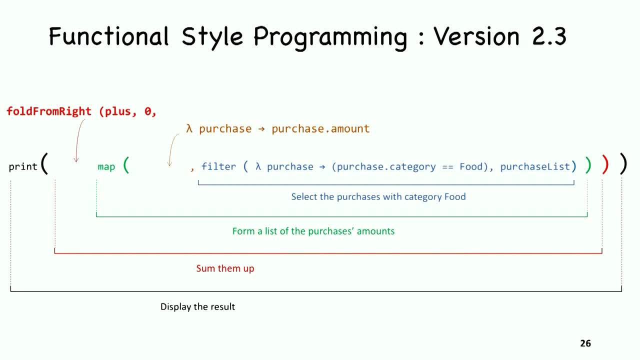 And the idea here is: it doesn't matter whether I fold from left or fold from right, because the plus operation, the operation of addition, is commutative. I'll get the same answer either way. But now I've substituted a fold operation for what I called sum in the earlier version. 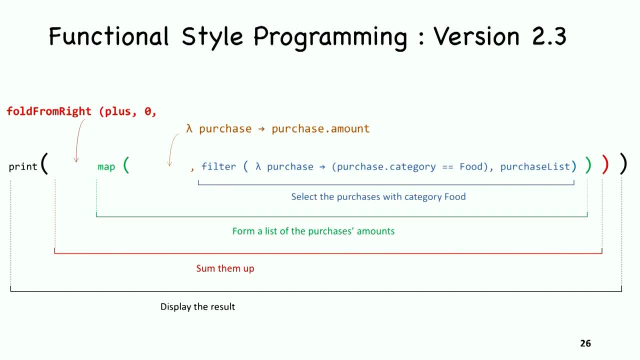 of the solution. I haven't particularly gained anything in the solution of this credit card problem, But what I have gained now is the ability to think about folding as an operation that can apply not only to adding things together but subtracting things from one another. 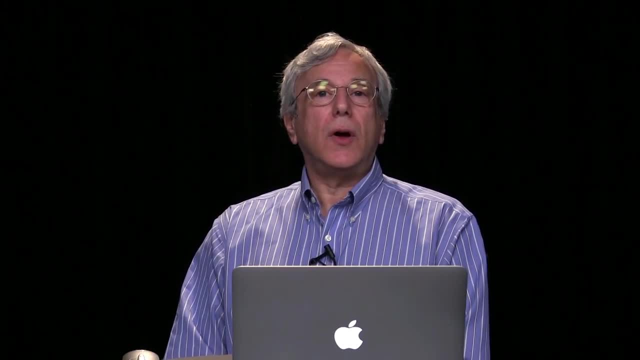 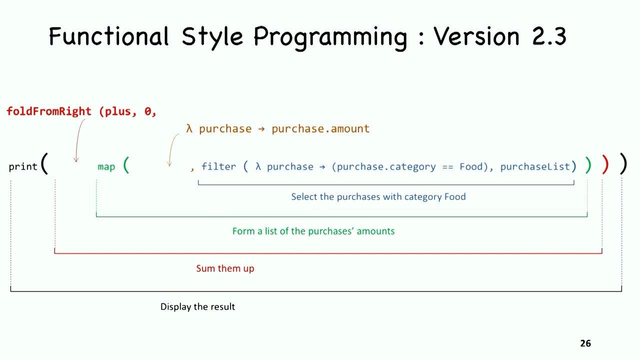 and just about anything that I could possibly do between two items in a list. So, for instance, if I want to multiply together all the items in a list, I can use fold for that, The notion of having a fold operation that I can apply not only to plus but also. 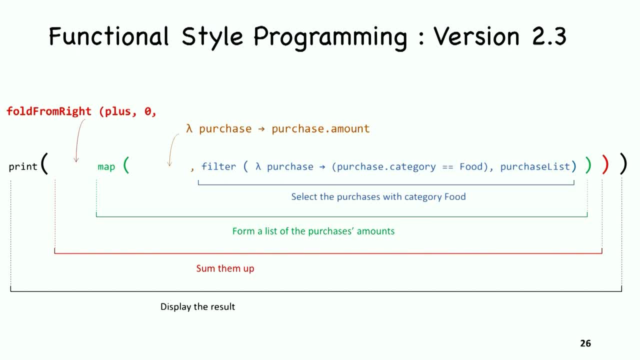 to minus, to multiplication, to minimum, to maximum or to whatever other function I have. I can do that And that's what I have in my vocabulary is a very powerful notion And it will serve you well in the functional programming. 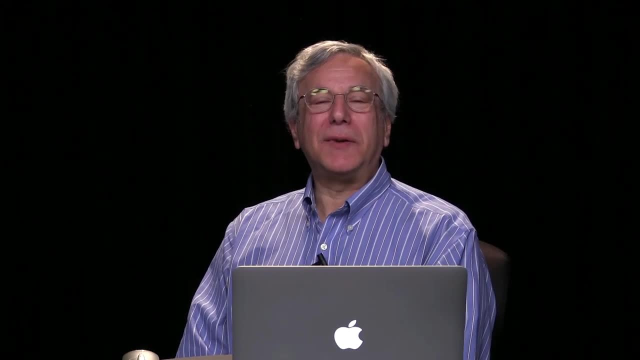 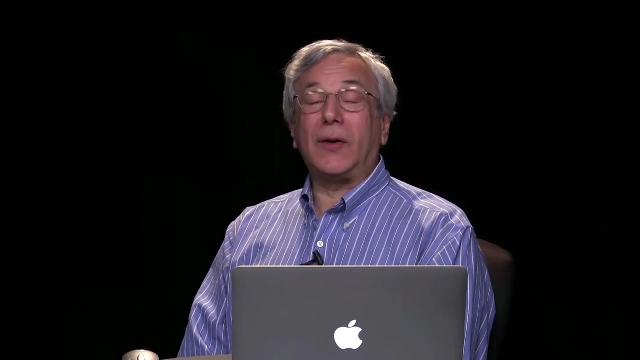 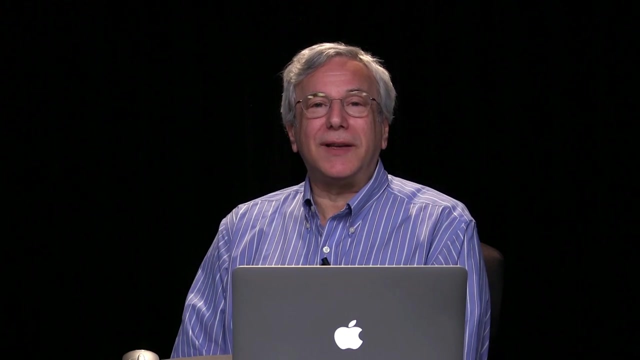 world. We've taken a problem, a small problem, one that you'd see in an elementary programming languages course, or one that you'd see embedded in an industrial strength application, And we've gone from thinking about it imperatively to thinking about it functionally. 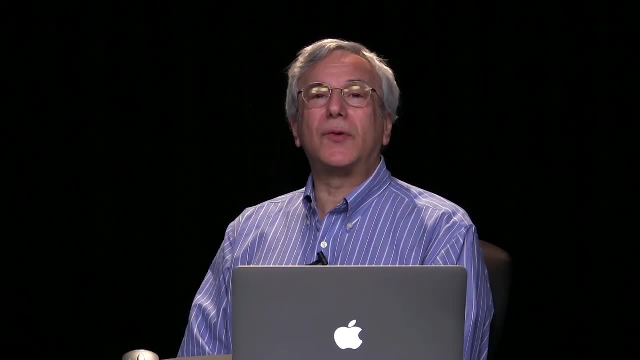 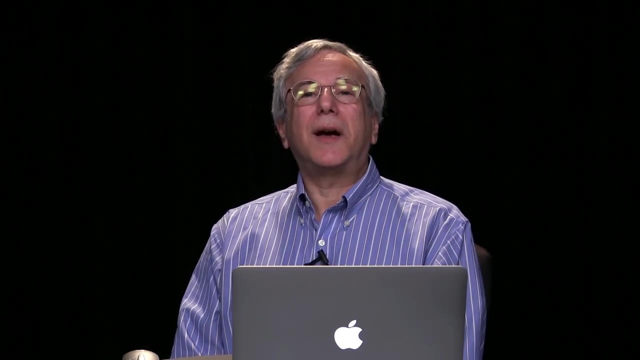 We're going to do much, much more functional thinking as this course progresses. In the meantime, we're going to take a slight break In the next segment. we're not going to look in the microscopic sense about filter functions and map functions. 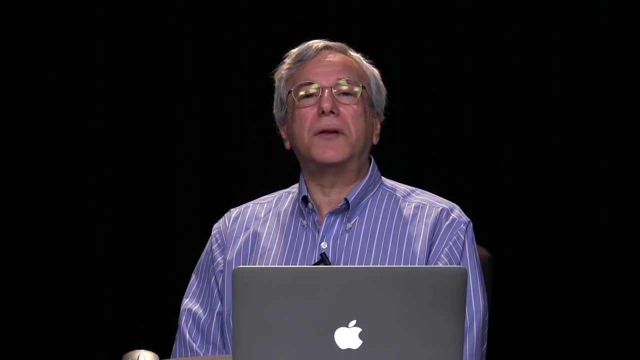 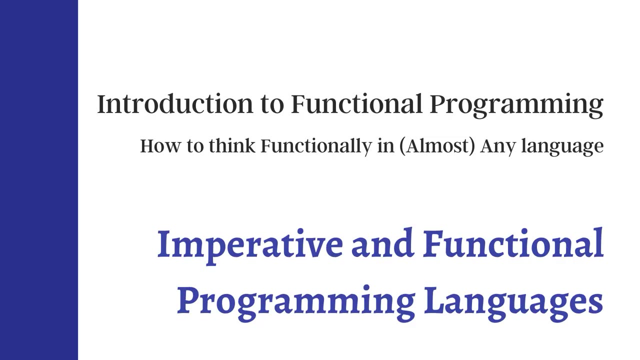 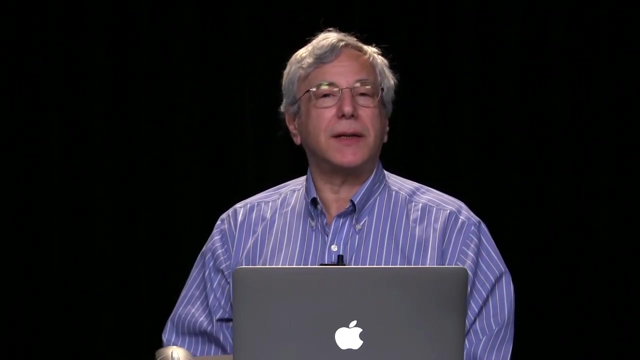 Instead, we're going to kind of take an overview of the notion of functional programming in general. Stay tuned. What have we done so far? We've taken a look at a problem, a small problem, but one that has a lot of very important operations in it. 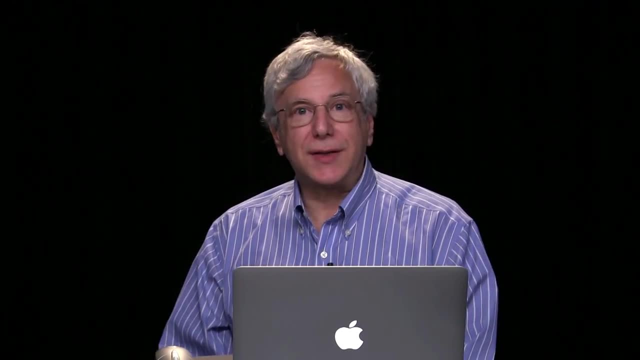 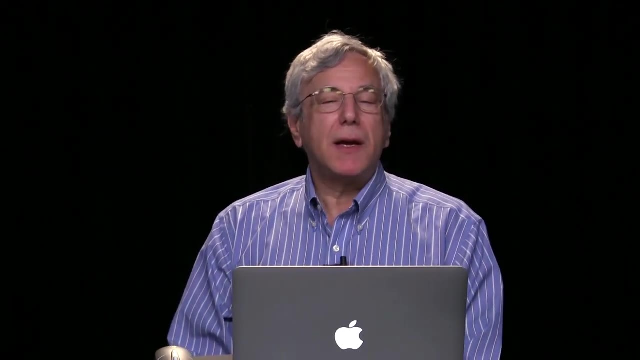 And we've moved it from an imperative style to a functional style. Have we really accomplished a lot? Have we gotten rid of loops and ifs and things like that? I'm not so sure. Let's look over the whole landscape. We've taken the if statement and kind of turned it. 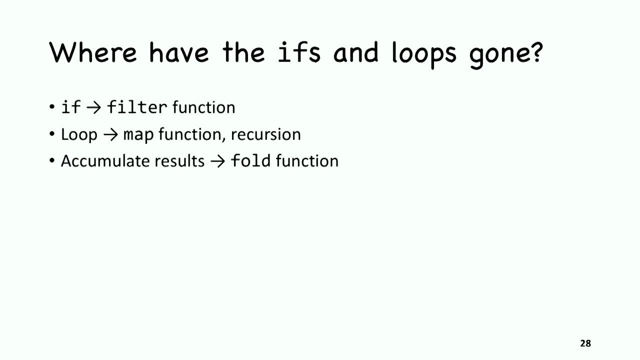 into a filter function. We've taken loops and turned it into a map function And later on in the course we'll be turning it into recursion. So we'll have a couple of things. We'll have a couple of different ways of doing in a functional style what we normally 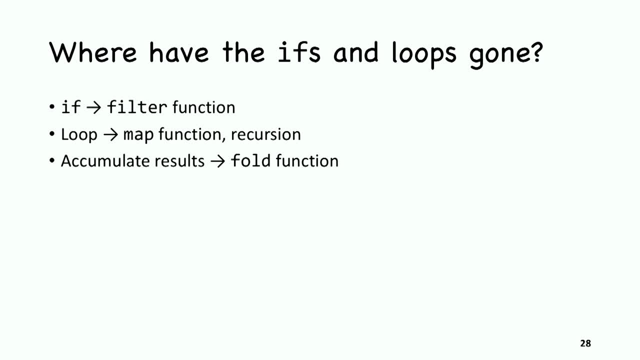 do imperatively with a loop. We've taken accumulating results- total equals total plus new amount- and turned it into a fold function. We've taken the ifs and the loops out of the language itself And instead we've moved it to a place where the programmer 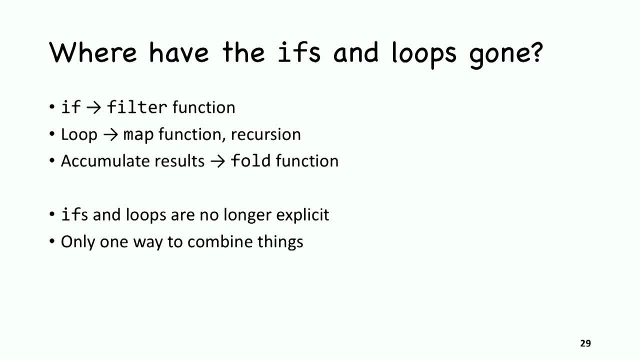 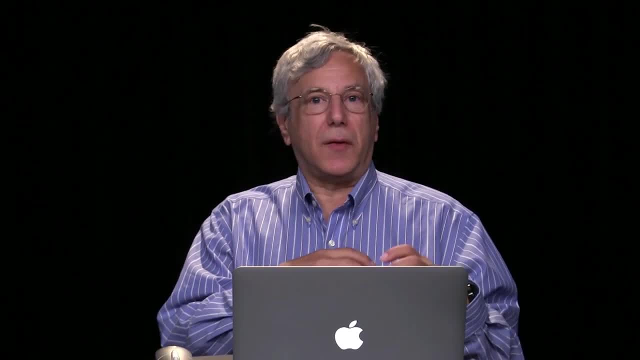 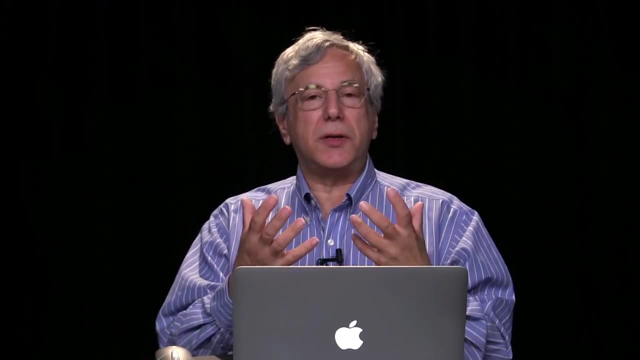 doesn't have to deal with it explicitly. There are still loops And there are still branches in our program. When the program gets translated from its Java source code or its C++ source code or any other kind of code into a machine language or an assembly language. 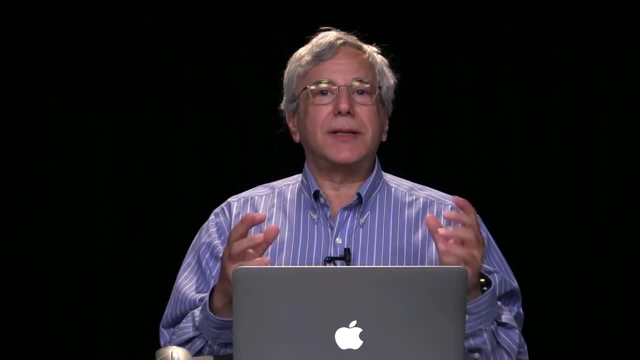 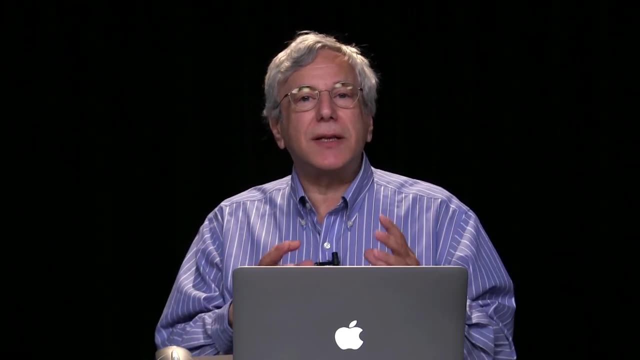 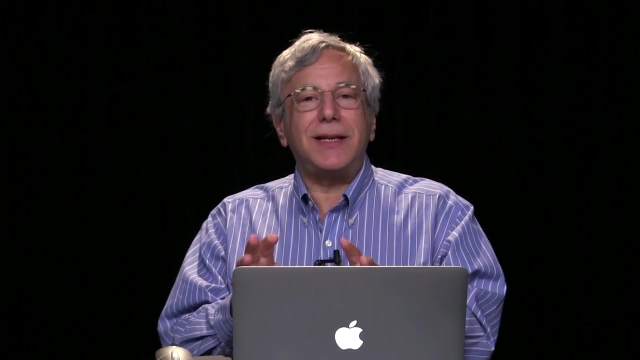 it will still have branches And it will still have loops. Maybe even, who knows, in an assembly language environment it will still have loops. But we're taking them away from the direct view of the programmer. The programmer isn't seeing now. if this, then that. 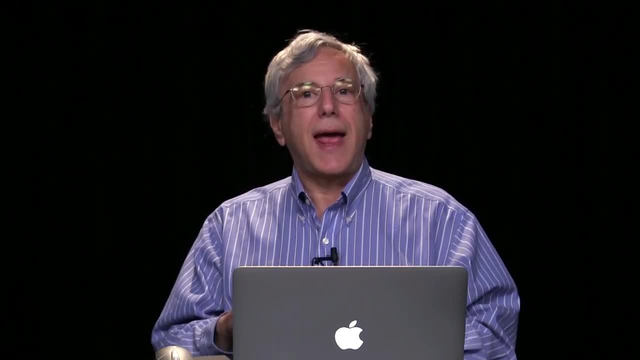 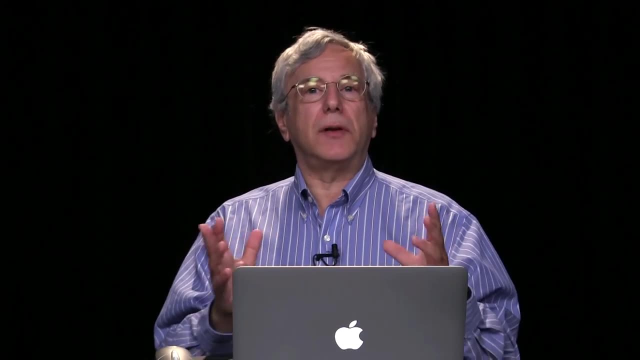 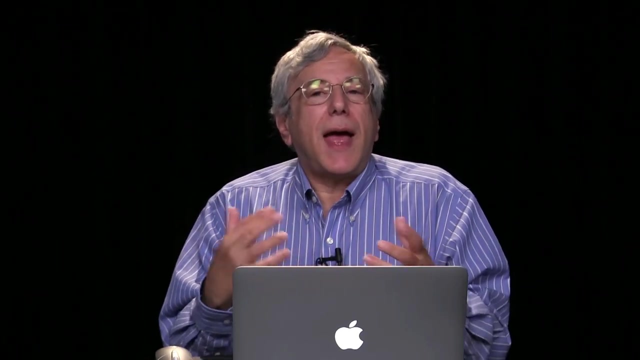 Instead, what the programmer is seeing is application of a filter function. So the idea here is not so much to completely get rid of the notion of choice. if this, then that or repetition somehow have a loop. The idea is to take away. 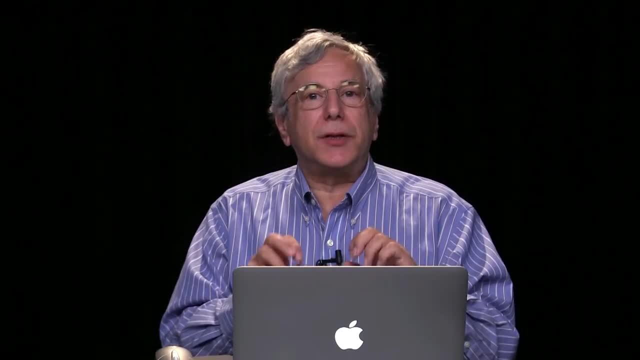 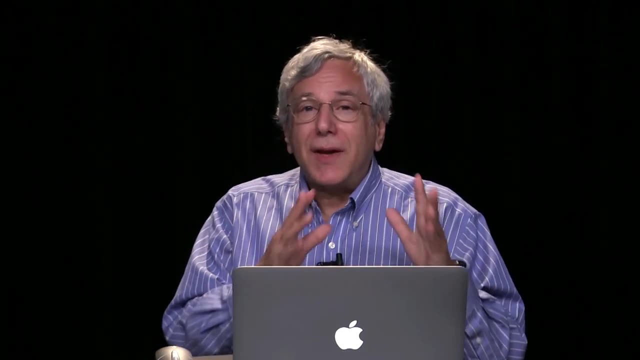 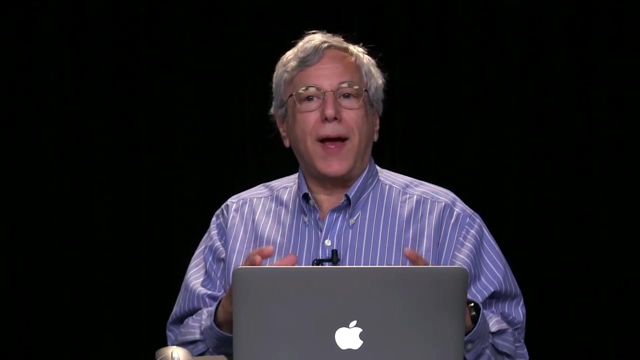 To take it out of the vocabulary of the language and make it part of the nitty gritty that the machine has to deal with. One of the advantages of this- an advantage that I haven't talked about a lot so far now- is that now we have only one way that we have. 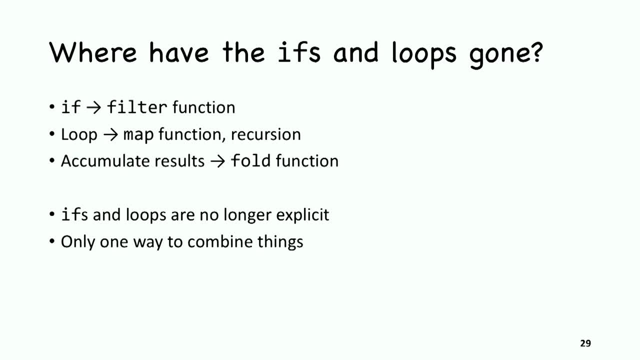 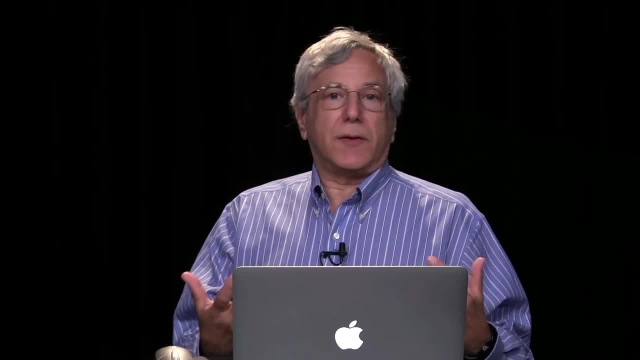 to deal with. to combine things. Let's think about the way you combine things in an ordinary imperative program. There are at least three ways to combine things, maybe more. One of the ways of combining things is saying: do the next statement. Another way of combining things is to say: well, 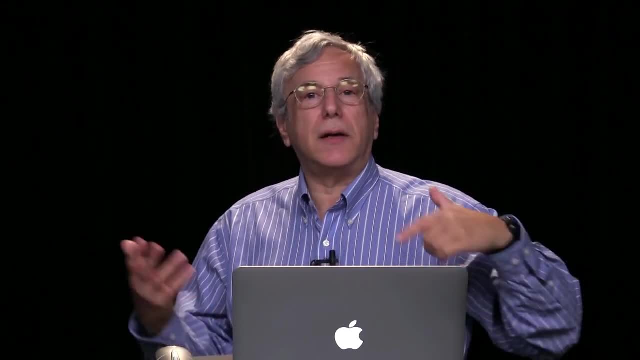 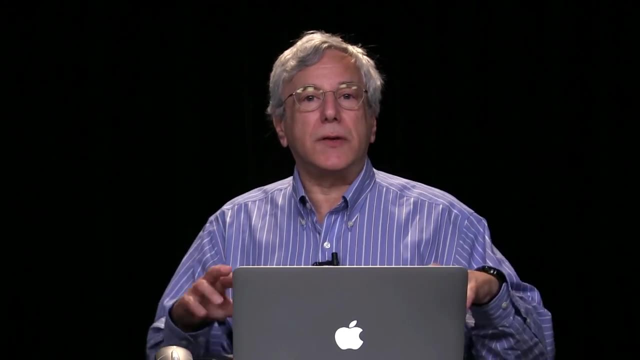 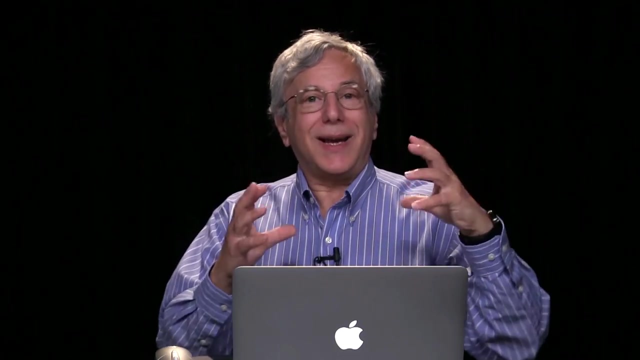 if such a condition is true, then do this, otherwise do that. And a third way is with repetition, Those three ways of combining things means that when the compiler deals with the program, the compiler has to worry about the three possible ways of combining statements. 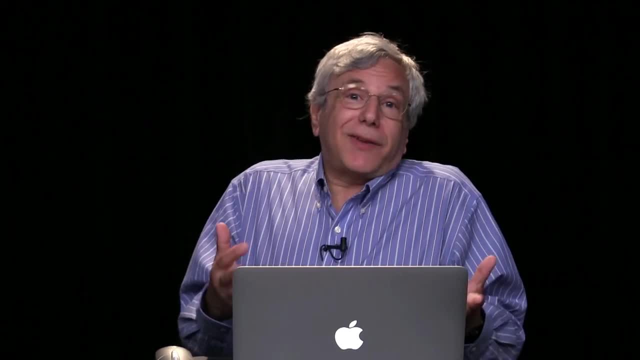 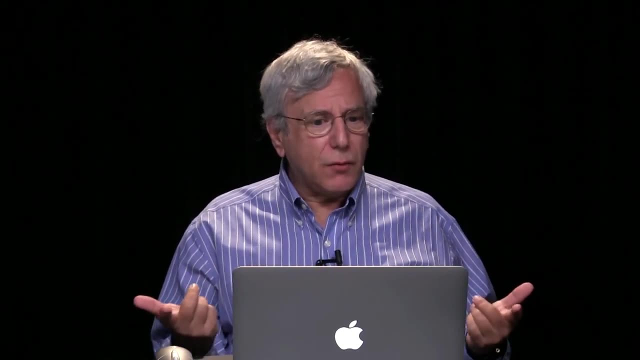 And, in fact, when we analyze the correctness of a program, we have to think about: oh, you know, is this now inside a loop or inside an if statement? With the functional approach, there's actually only one way of combining the parts of our program. 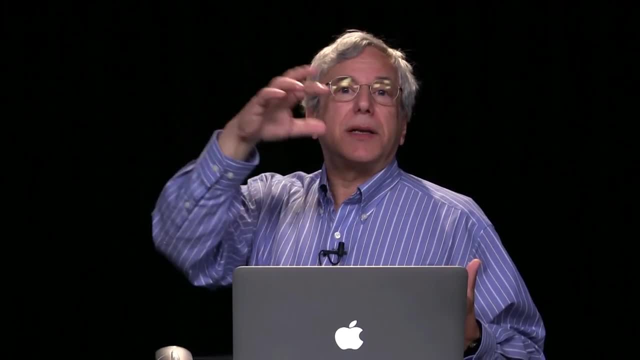 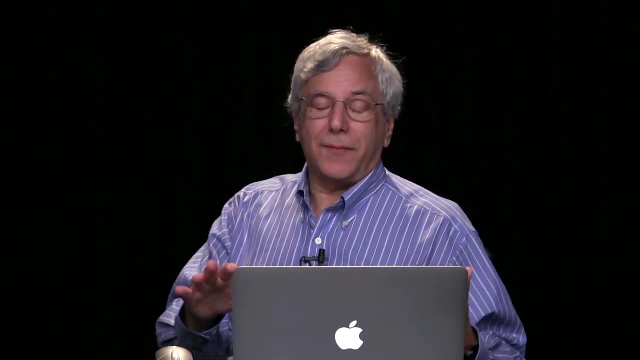 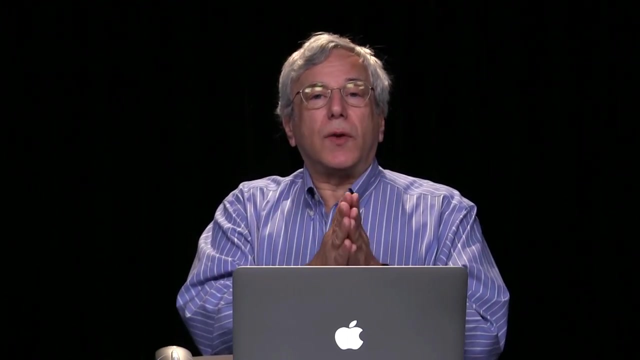 We take the results of one function and we apply it as the argument to the next function, And that makes for a simpler way of dealing with computer programming. Now, if you remember the previous example, you might be arguing with me, or attempting to argue with me, about the way that I'm combining things. 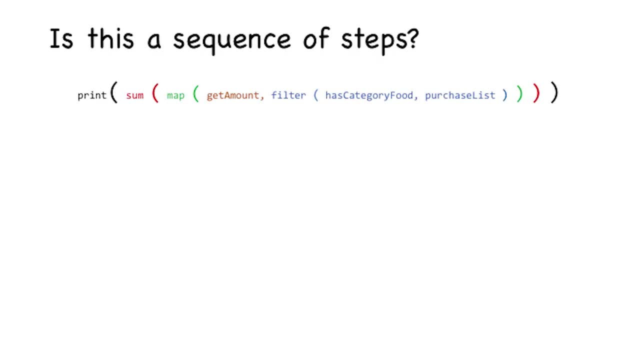 After all, in the previous example- and I'm not using the lambda notation now, I'm just using the ordinary get amount and has category food. In the previous example I combined things, sure, by applying functions to one another, But is this really, after all, a sequence of steps in disguise? 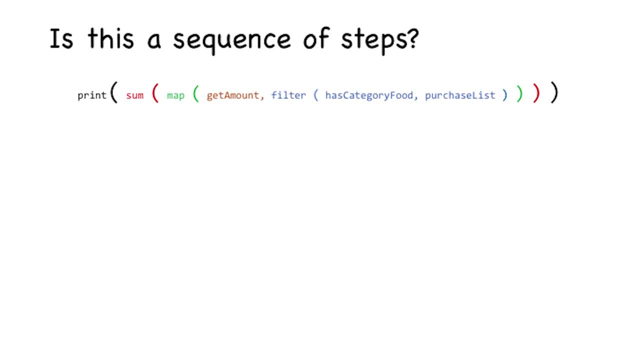 I don't have it on several lines of code. It doesn't look like it's on several lines. It's on several lines of code. But isn't this just a matter of saying take has category food, and then do filter, and then do get amount and then do map? 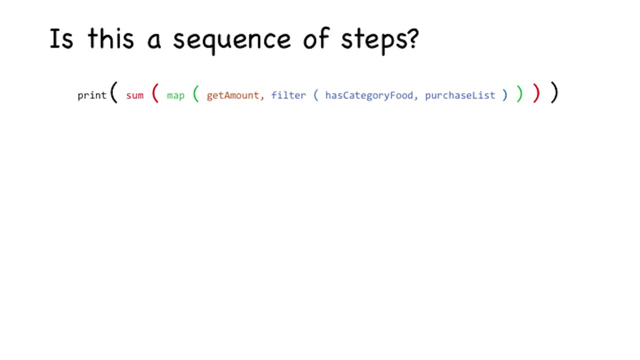 and then do sum and then do print. Is this a sequence of steps? after all? You know, I've taken the if and put it behind the curtain, and I've taken the looping and put it behind the curtain. But is this still sequencing? 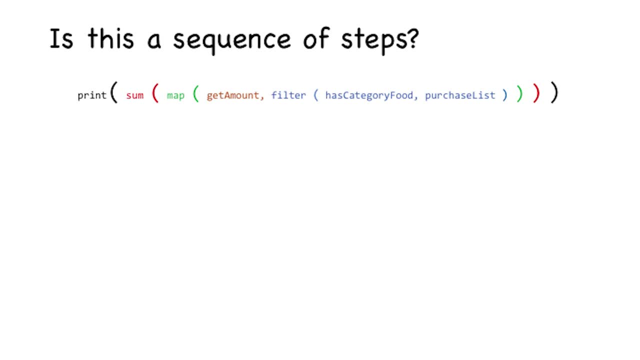 Am I lying to you? after all, Should you turn off the computer and not watch the rest of this course? Definitely that's not the case. You shouldn't do that, and I'll show you why. Let's take the print sum map, get amount filter. 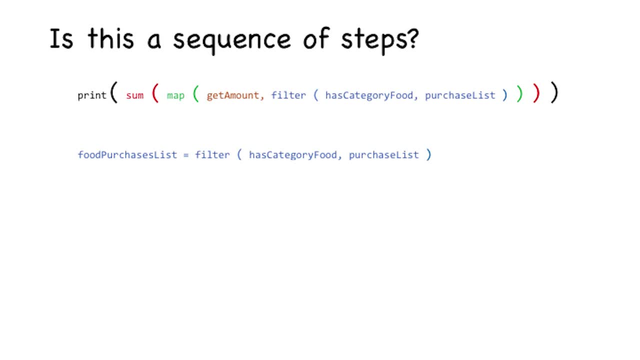 and let's rewrite it just a little bit so that we define a new name, if you will: food purchases list And let's not make that be the result of applying filter to has category food and purchase list. And then let's take what we might consider. 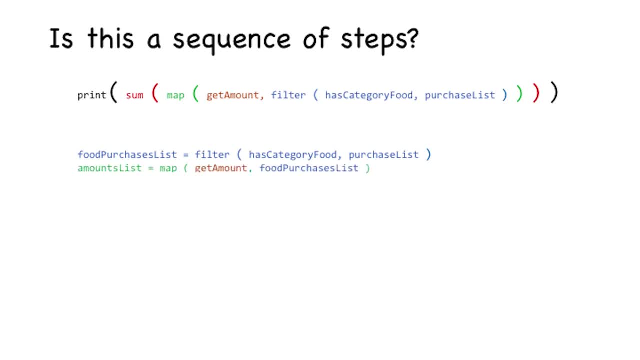 the next step, applying map to food purchases list and get amount and get something called amounts list. And let's continue with this process. Let's take amounts list and feed it to sum and get total and take total and feed it to print. 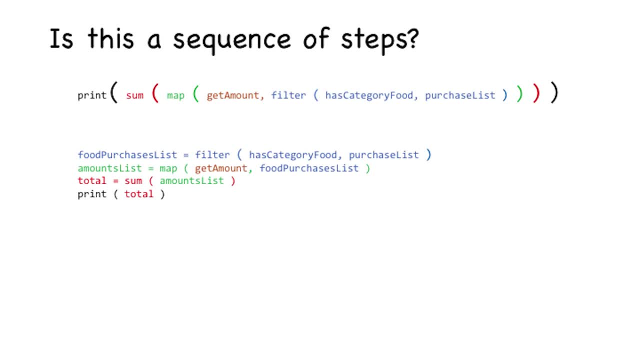 so that it displays on the screen or wherever you want it displayed. Now this looks a little bit more like a sequence of steps. So now you might say I've stepped back a bit from the notion of function and said, OK, first do this. 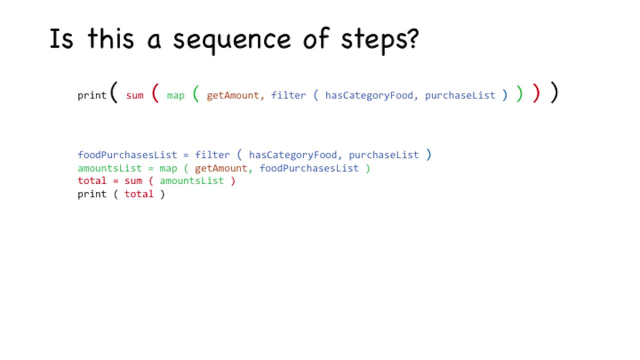 OK, First do this, then do that, then do something else, then do something else. I'm backpedaling, am I not? Not quite, And the reason is because I can rewrite this sequence of four lines by changing the order of the lines. 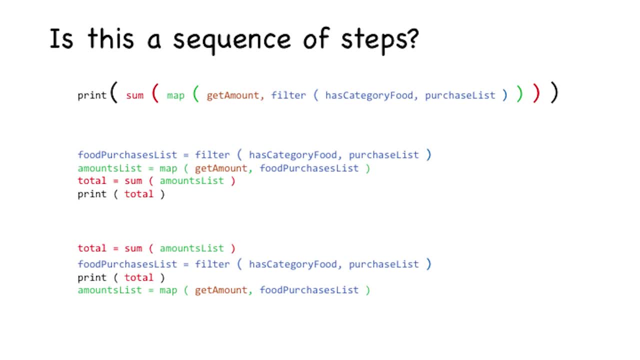 Instead of writing the food purchases list equals filter line first. I can write that second or third or fourth or in any order that I want to put it. What I've done here on this slide is I've changed the order of the lines just in some random fashion. 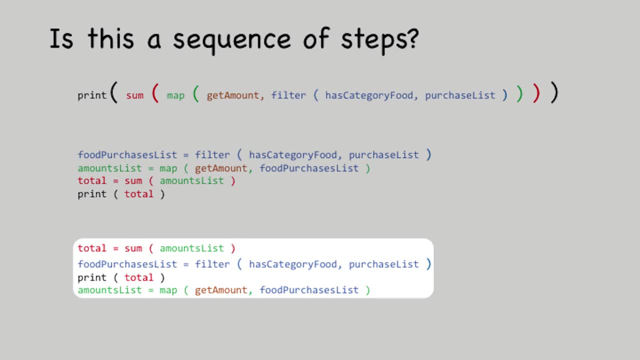 But if you notice, if you look at these four lines, even though they're out of order, you can still determine the order in which they should be applied. So, for instance, if I want to print the total, I have to first find the total. 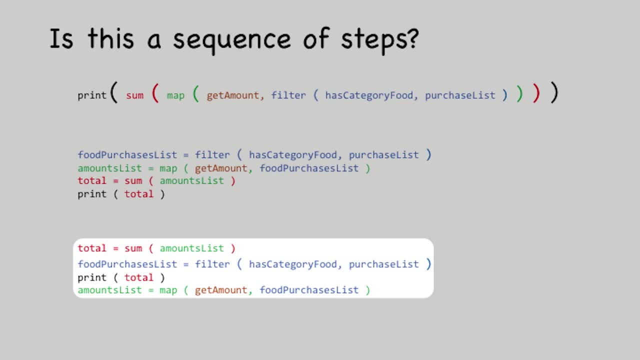 So if I look at the third line and it says print total, I say hmm, OK, That means I have to find out what total is. so I have to jump to somewhere where total is defined. If I look at the top line and I see total equals some amounts list. 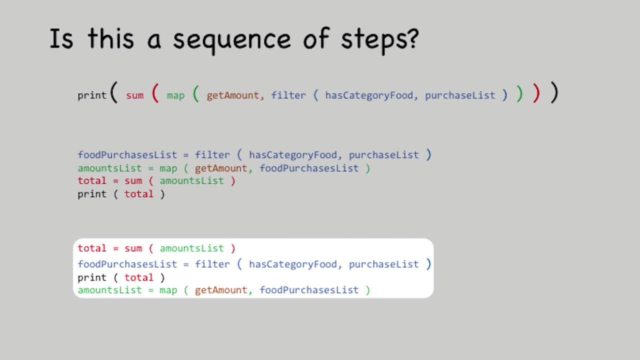 and at that point I say: wait a minute. that means I have to know what amounts list is. So if I want to know what amounts list is, I have to go to some line or other in the code that says where is amounts list defined, and so on and so forth. 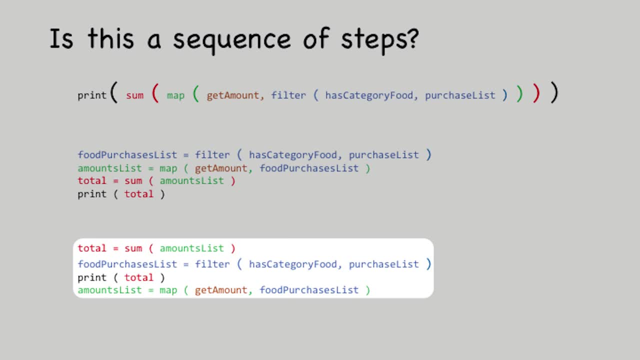 In other words, this collection of declarations doesn't need to be in any particular order. I am not really saying explicitly: do something and then do something else. I'm simply defining a group of functions and then saying: computer or whoever it is, whatever entity is executing this set of function. 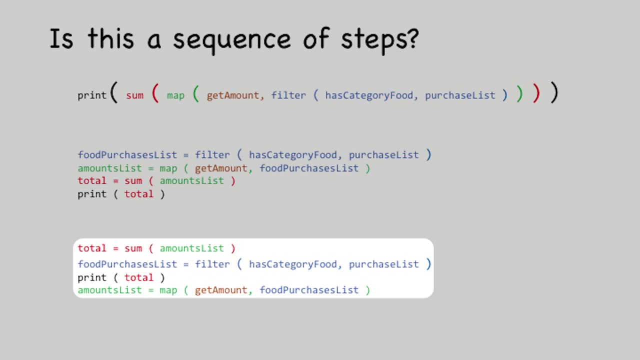 definitions, you go and figure out which functions you have to apply in which order to solve the problem. So, whereas there looks like maybe there are some step-by-step set of instructions here, really what there is is a set of functions that resolve to one solution, to one problem. 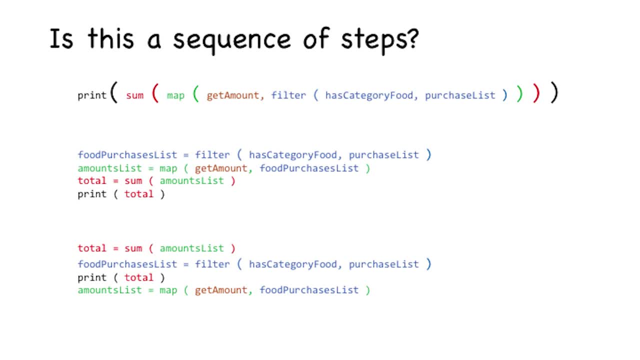 In this case, printing the total of all the purchases And the order in which those instructions are displayed or set out or written down doesn't really matter, And that's an important concept in functional programming. OK, what languages are you used to using? 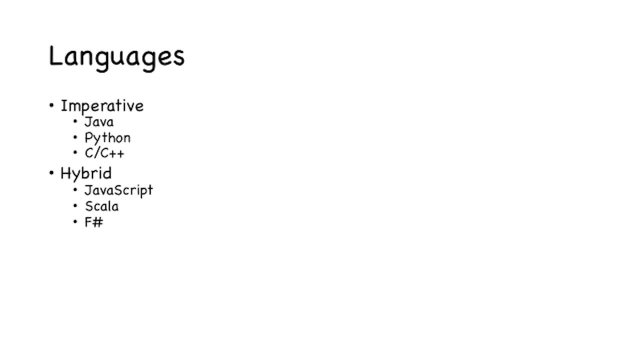 I've written on this slide a modest list of languages. I was tempted on the slide to put down every language that I could think of and categorize them, But that's too hard to do. You take your favorite language and you figure out where it belongs. 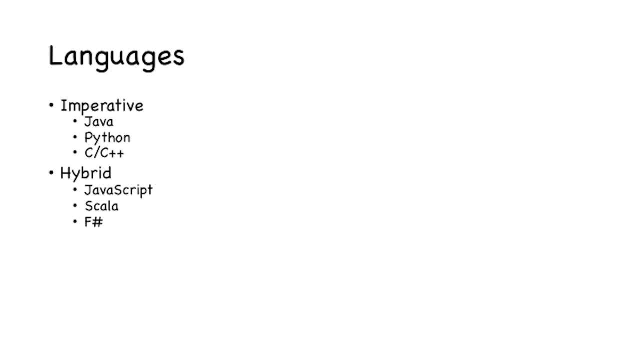 Chances are you're used to a language that's either in the imperative category here or in the hybrid category. So an imperative language is one that's built on the do this, do that paradigm of computer programming. There are hybrid languages, And the hybrid languages are the ones. 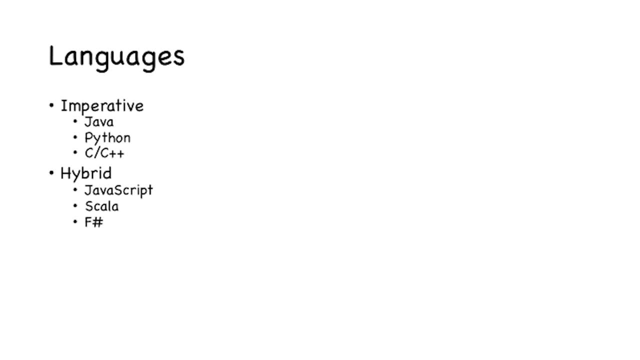 that do both functional and imperative programming from the ground up. So JavaScript is maybe the one that's most commonly used. There's also Scala and F sharp and another of other languages, a number of other languages of that sort. I have to say that languages like Java 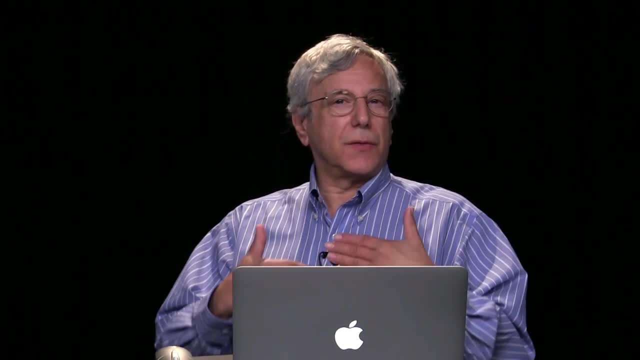 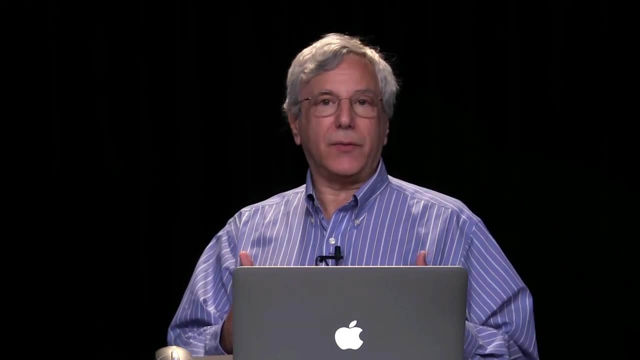 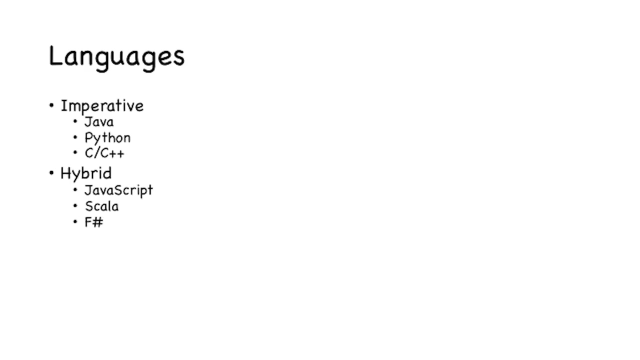 have some functional features, But those functional features are built in after the language was first constructed. So I'm not listing Java as a hybrid language. I'm listing Java as a purely imperative language with some functional features, And that's true also of Python and C, C++. 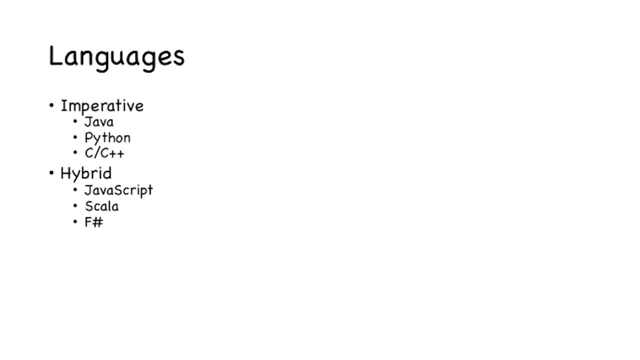 On the other hand, JavaScript was built from the ground up with functional features. Scala and F sharp were built from the ground up with functional features. So I call those hybrid languages, because they allow both functional features and imperative features. There's one language in particular, that's. 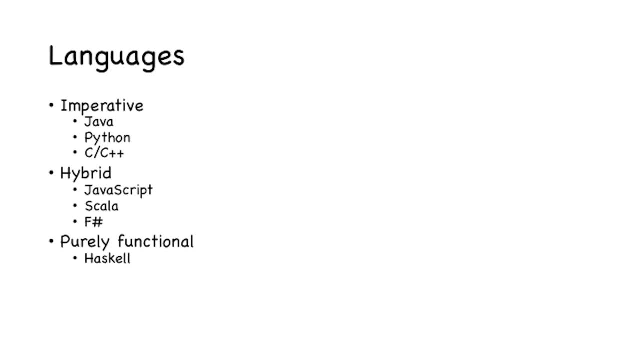 very popular among functional programmers and it's called Haskell. In the Haskell programming language you can program only functionally. You have no imperative features available. in the Haskell language You have some features that look like they're imperative programming, but they're really not. 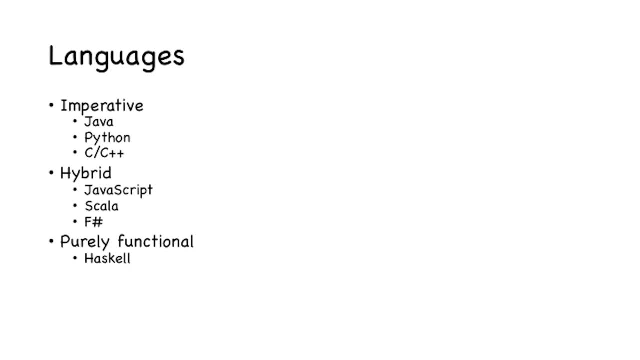 A lot of innovation comes out of the Haskell space, innovation that goes into building features for other languages, such as Java, Scala and F sharp, And I also have to mention at this point that it's not a battle purely between the imperative and the functional languages. 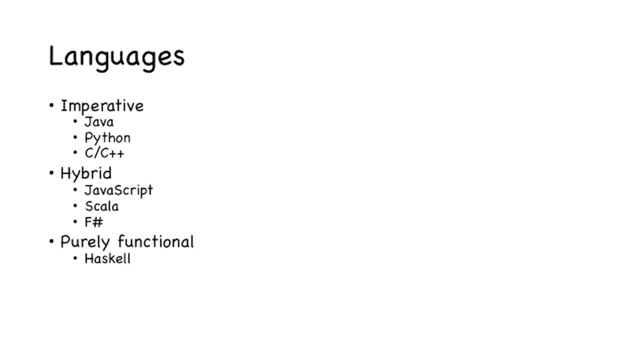 There are other paradigms, too many other paradigms. I'll just mention one to give you an example of another way we can think, and that's with the prologue language. The prologue language is neither imperative nor functional. It's a logic language. 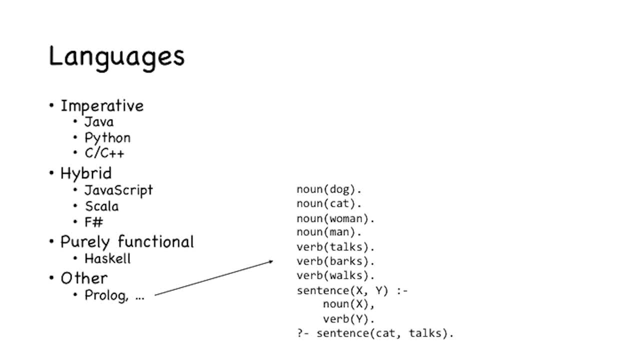 So in a prologue program you would say, for instance, that x and y is a sentence as long as it's a noun followed by a verb. Is cat talks a sentence? Well, computer, you figure it out based on the declarations that I've made so far. 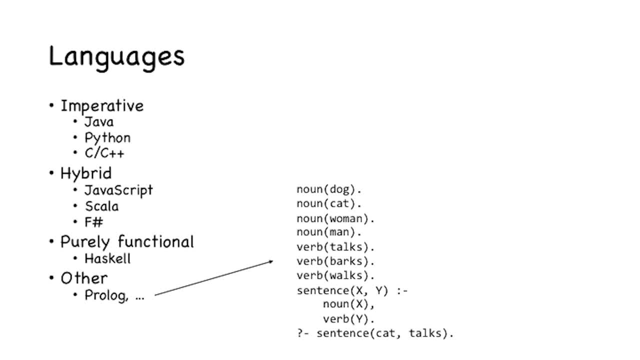 So we've got imperative, we've got functional, we've got hybrid, which are languages that do both imperative and functional, And a lot of languages now are fitting into that category. And then we've got other paradigms, and I don't want to ignore them: logic programming. 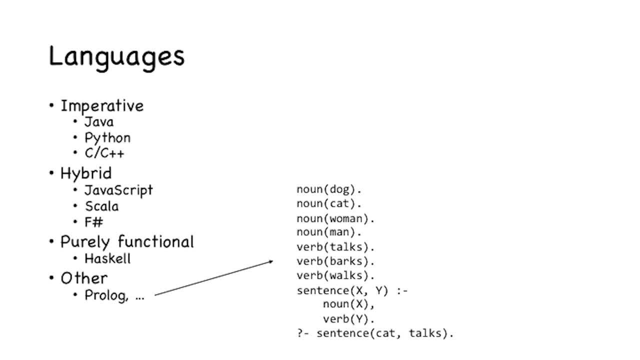 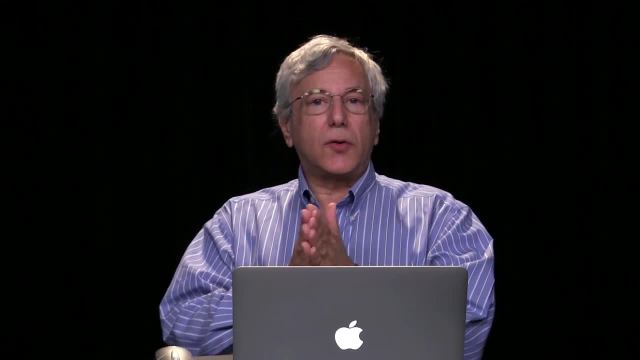 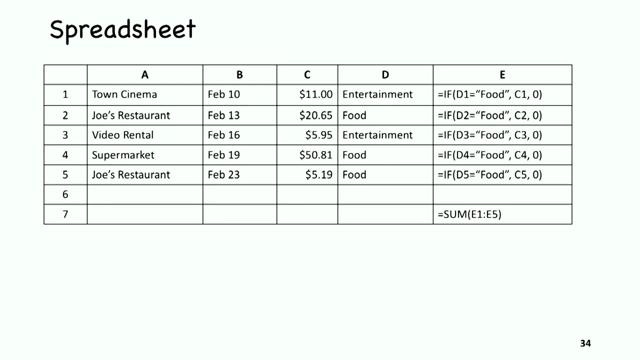 being one of them. Now, if functional programming seems as if it's really something new to you and something you haven't seen a lot of before, you have to consider one special case, which is the case of spreadsheets. Here's a spreadsheet- maybe Excel or some other spreadsheet- 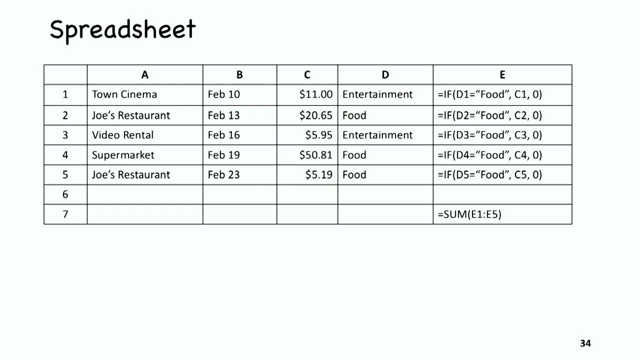 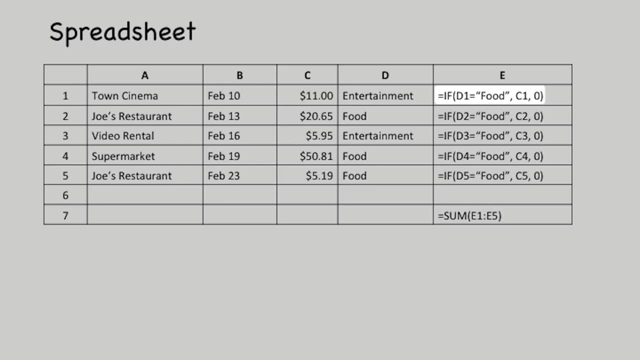 package that you've used, And what I want you to notice about this is it looks a lot like what you'd write in a functional language. I don't have an explicit filter function here, But I do have an if formula or an if function. 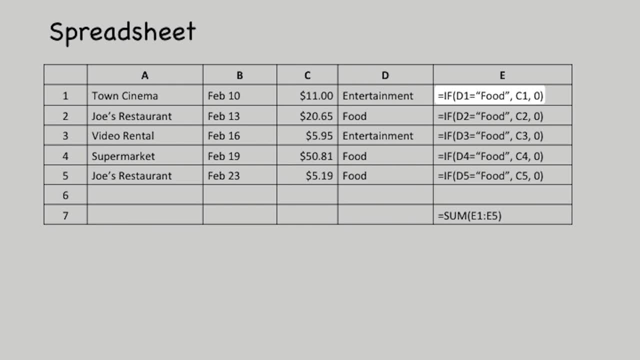 And what the if function does is. it says: well, for instance, if the value in cell D1 is food, then the value in this cell E1 should be whatever is in C1, otherwise make it be 0. And the same with the other cells down the line. 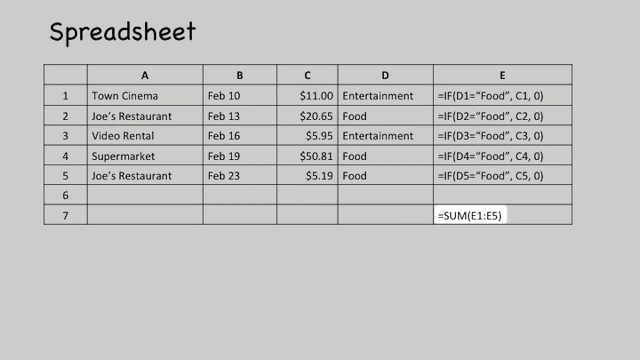 And finally, at the very bottom, it says: well, OK, now sum up for me all the values in cell D1.. All the values in cells E1 through E5.. OK, is this functional or is it imperative? I think it's more on the functional side. 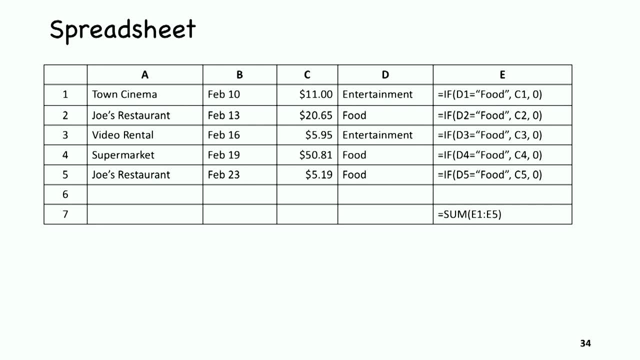 We don't have an explicit filter function. We don't have a lot of the things that we want in what we'd call a functional language, But we do have one important property, That is to say we're using mostly formulas. We're not telling the computer to do something. 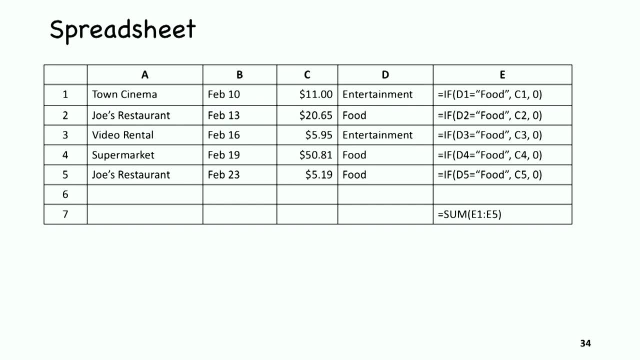 and then do something else Instead. we're laying out a bunch of these formulas and we're saying: OK, spreadsheet program, you figure out which formulas you have to apply when in order to get the answers that you need. So a program that manages this spreadsheet will say OK. 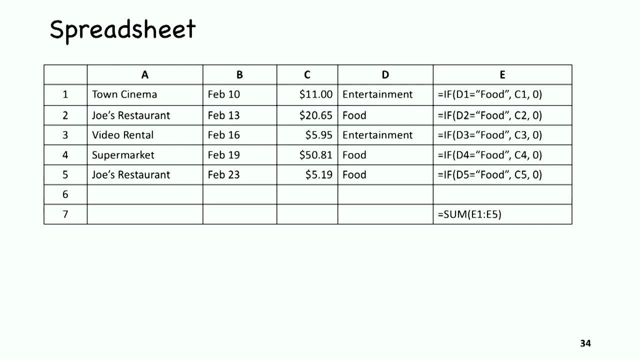 let me see. I know what should be in cell A1.. I know what's in B1.. I know what's in B2.. Let me see- Oh, I have to figure out- what's in cell E7.. That's the sum from E1 to E5.. 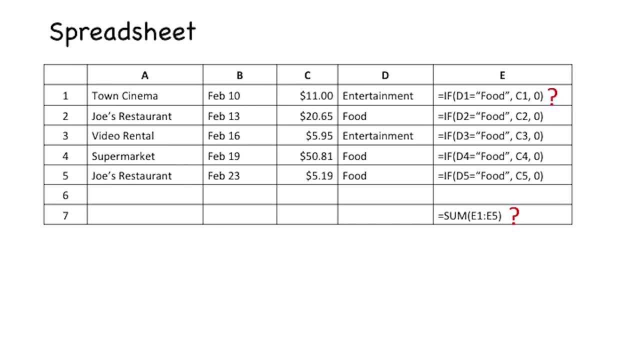 OK, let's see. Do I know what's in cell E1?? Aha, it has to be. well, it depends on what's in D1.. I better check that and so on and so forth. OK, so I could take what's in cell E7 exactly. 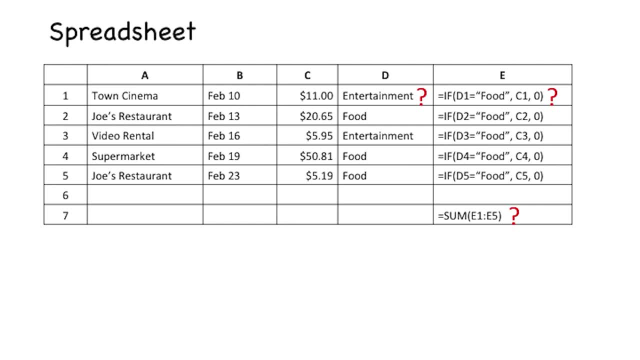 and move it to another place in the spreadsheet. If there were room above the first row, I could move it above the first row, And as long as it's still said sum of E1 through E5, the spreadsheet would work exactly the same way. 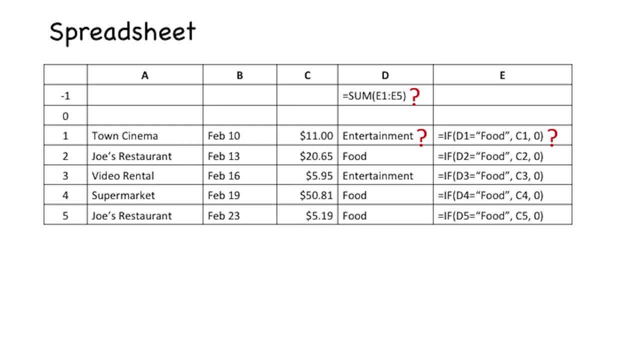 It would give me exactly the same answer. So again, in this spreadsheet, I'm not saying: do this, then do that. Instead, I'm saying: here are the formulas that you have to figure out. Go ahead and figure them out, in whatever order. 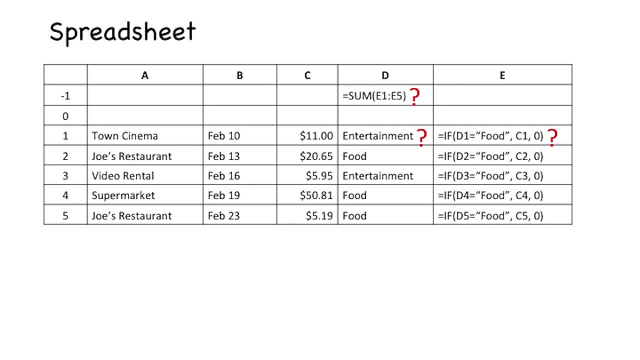 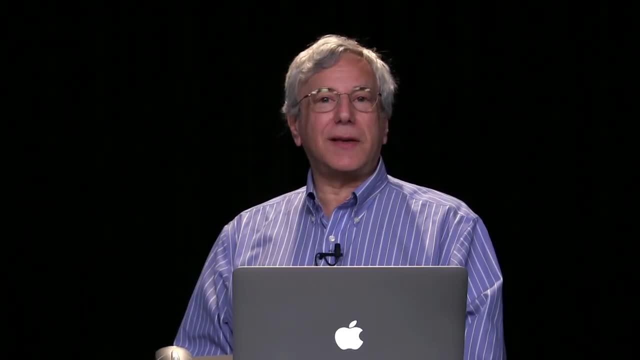 you have to in order to solve the dependencies, And that's the essence of functional programming. So you see, functional programming may look strange, but it's not this strange thing. It's something that you use every day in a spreadsheet, and I'm sure you've used spreadsheets. 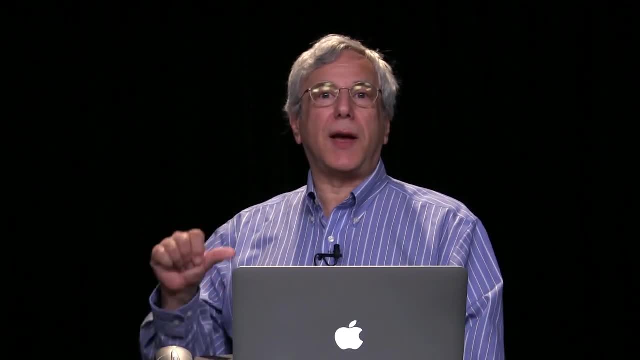 OK, in the rest of the course we're going to delve into much more detail about how to do functional programming, how it works, what it is and what are the nitty gritty details, and I'm sure you'll enjoy it. 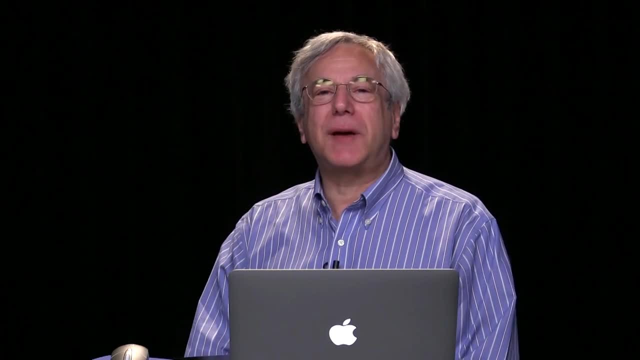 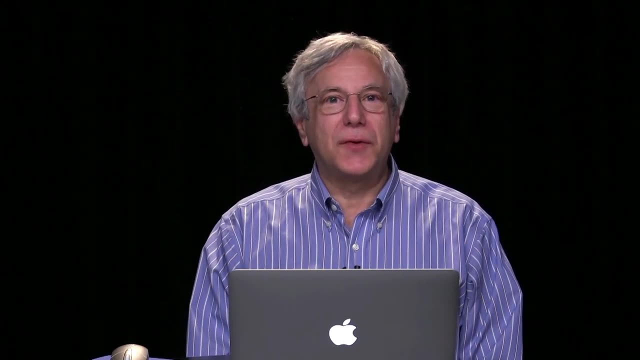 Let's talk about functions. That's, after all, the subject of the course functional programming. I'm going to talk about a special kind of a function called a pure function. A pure function has certain properties that make it really really nice for the kinds of things. 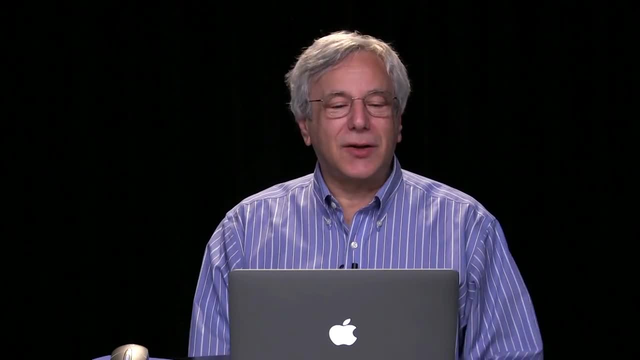 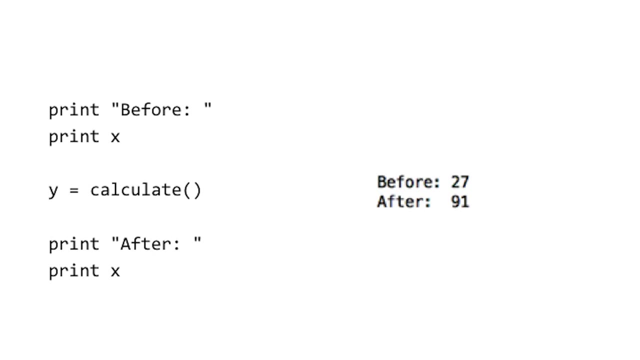 that you want to do when you create a computer program. Let's take a look at this slide. I've got a function called calculate. It does something, does some kind of a calculation, produces a result. The result gets assigned to the value y. 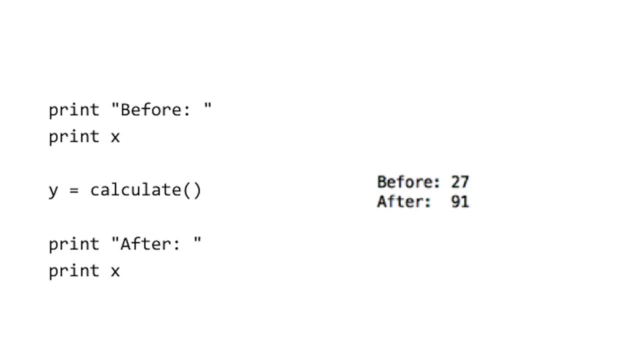 This is an imperative style program, of course. Now, what I've decided to do with calculate is: I am printing the value of x before I call the calculate function and printing the value of x after I call the calculate function. And if I look at the behavior, the behavior. 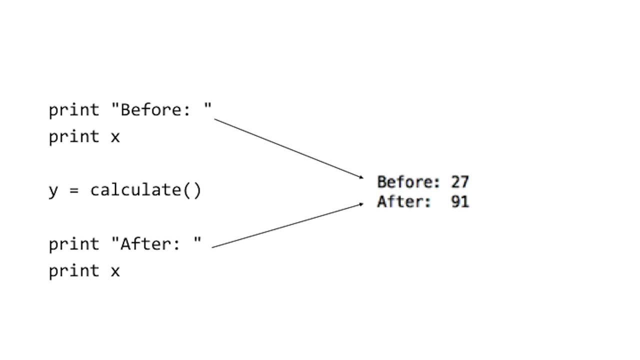 is marked on the slide also. What happens? Well, of course, I haven't really written a function called calculate, but I've mocked up a situation in which the call to calculate seems to change the value of x. Now I'm sure. 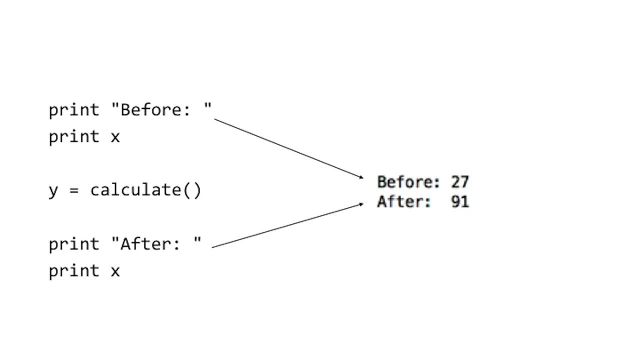 That if you've been working with computer code for a long time, you've observed behaviors like this. In particular, you probably observed behaviors in other people's programs, And the reason I say other people's programs is because that's when it strikes you the most. 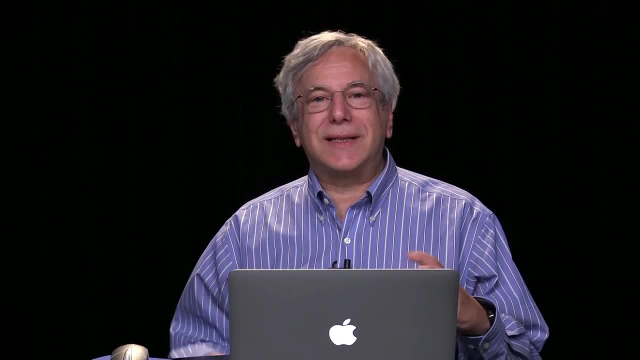 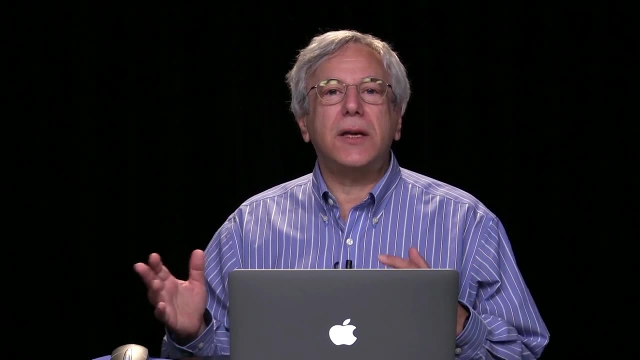 the most severely that this kind of behavior is tough to deal with. It causes angst. It's surprising- Whoops, I've got a value somewhere that I need to manage, but calling a function- calling a function- makes a change to that value. 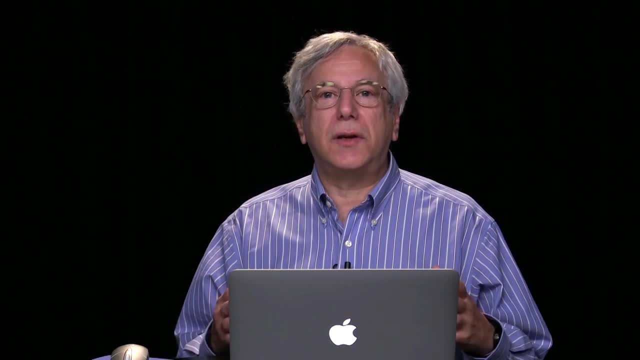 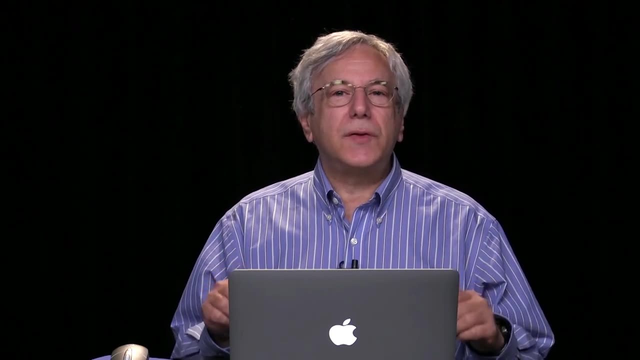 Now, if I want to figure out exactly what's going on in the code, I have to look inside the body of that calculate function. Wait a minute. We're not supposed to be looking inside the bodies of the functions that we simply call. 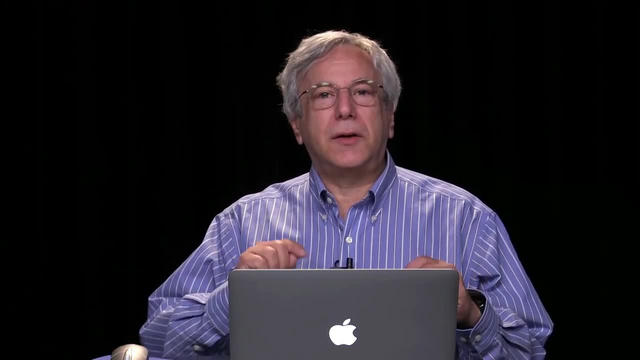 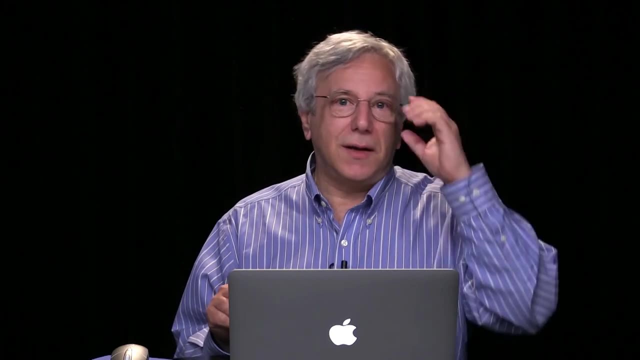 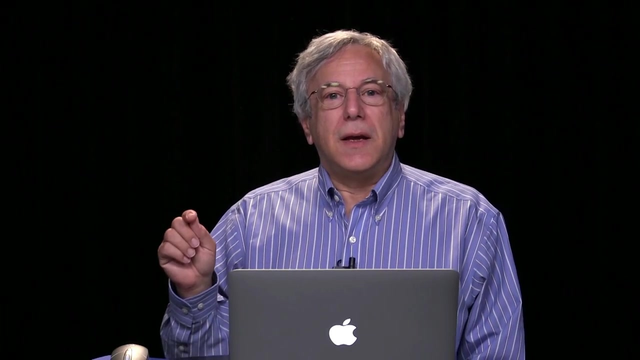 That's not the right way to partition our code so that we can deal with it in a clean fashion. OK, Look, I just started programming and I had to deal with other people's code that did this. I noticed this effect and I said to myself: you know what? 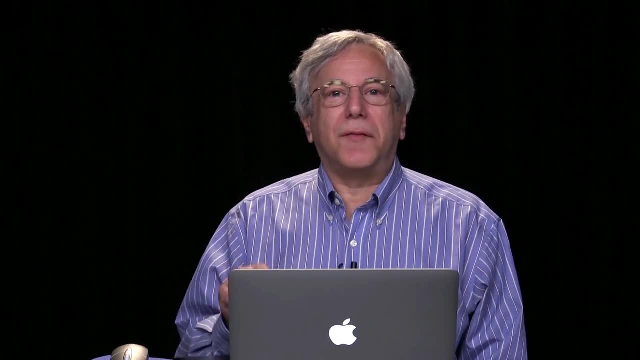 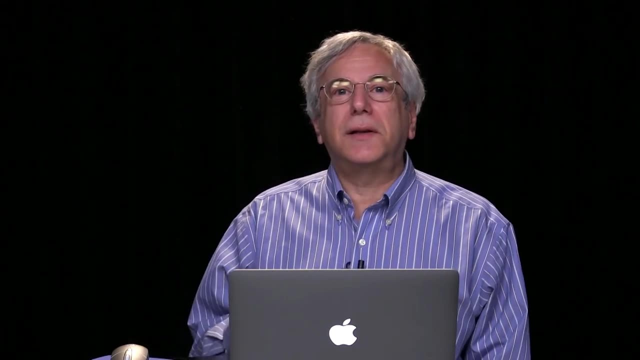 I don't like this happening, but I better get used to it, I better become tough, because this is what happens in the programming world. You call a function It has some- let's call it a side effect, And if I'm a good programmer, I learn to deal with this. 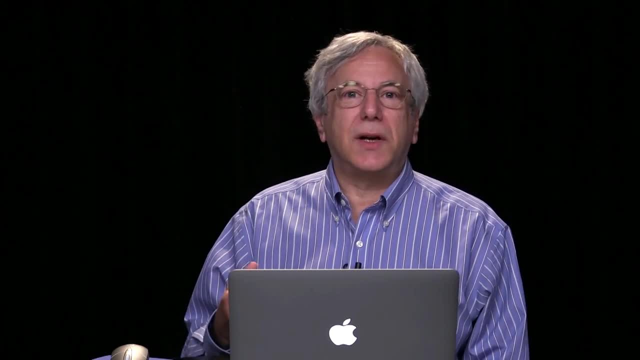 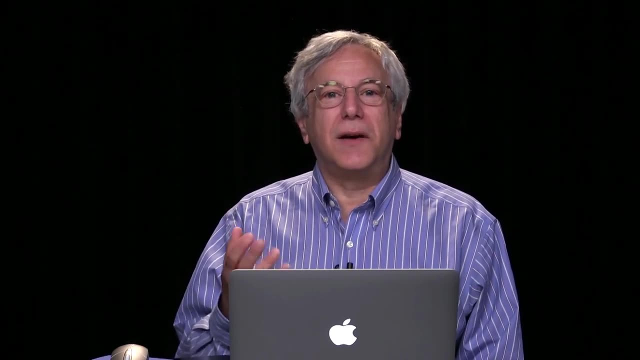 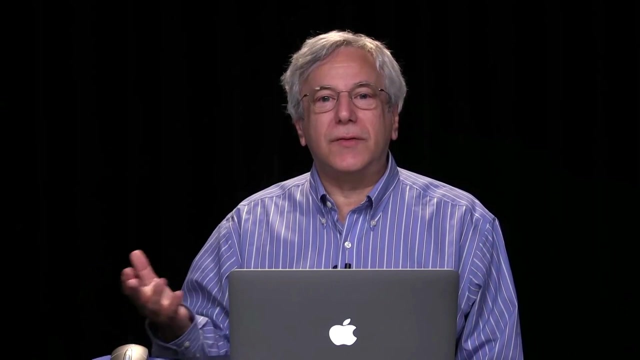 I embrace it, I appreciate it. That's what I said to myself when I first started programming. The problem is that we really should not be embracing this kind of code. We should not accept, tolerate like, become used to side effects. 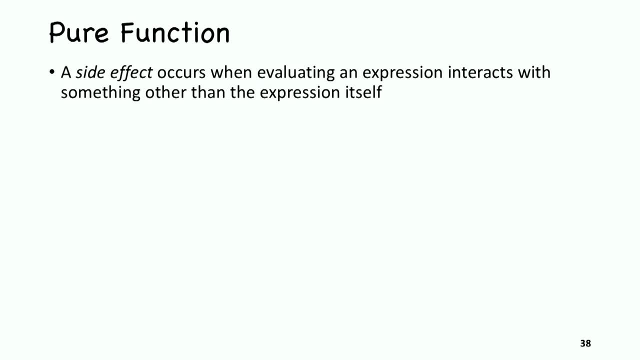 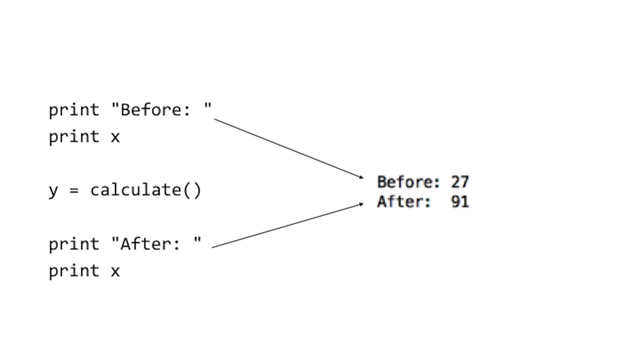 OK, Let's get technical. A side effect occurs when evaluating an expression. for instance, calling a function interacts with something other than the expression itself. So in the previous slide we called calculate. Calculate is an expression. It has a value. 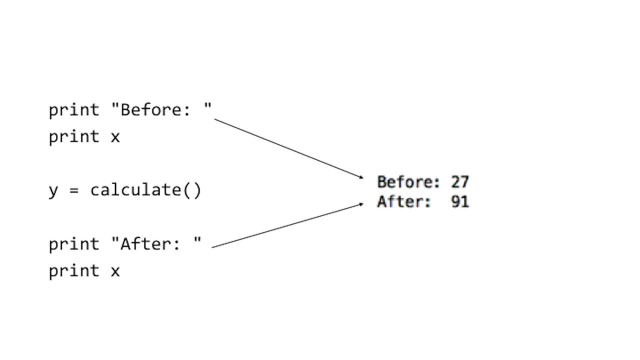 The value gets assigned to y. I evaluate that expression and it interacts with x. No good, No good. That's like something happening behind the curtain while we're not looking. Not a good thing. So we call that a side effect and that's. 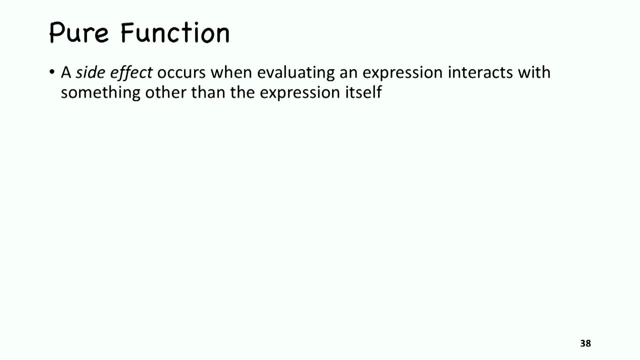 something that we, as functional programmers, are going to say: we don't appreciate it, Sorry, We put up with it for decades. Now we don't like it. A pure function is one that has no side effects. Take a look at the diagram. 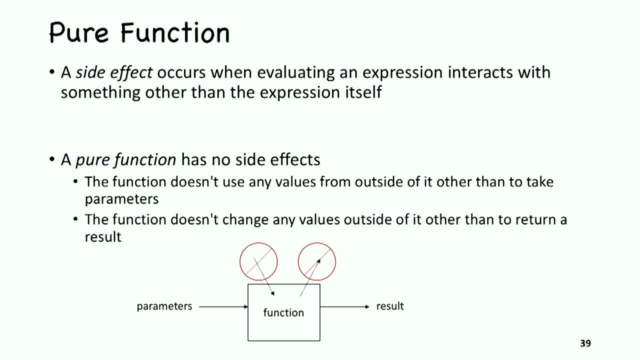 In the diagram you have a function, It takes some parameters, It produces a result And that's all that it should do. It shouldn't take in values, use values from outside of itself while it's executing, while it's doing its work. 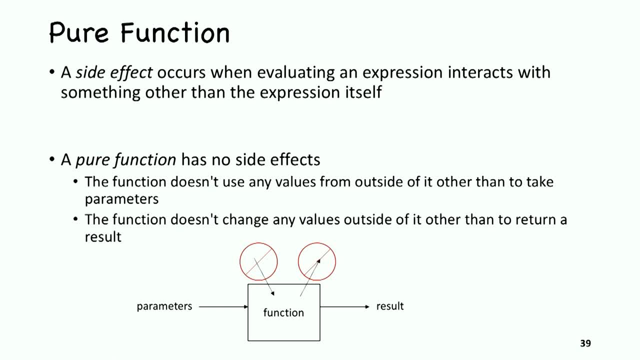 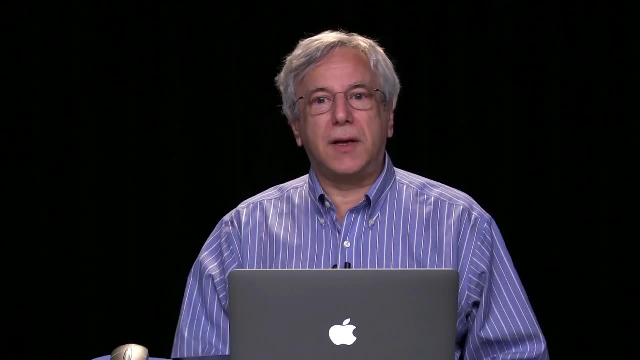 And it certainly should not modify values outside of itself while it's doing its work. A pure function is a function that doesn't use any values outside of itself and doesn't change any values outside of itself. Of course, a pure function can take parameter values. 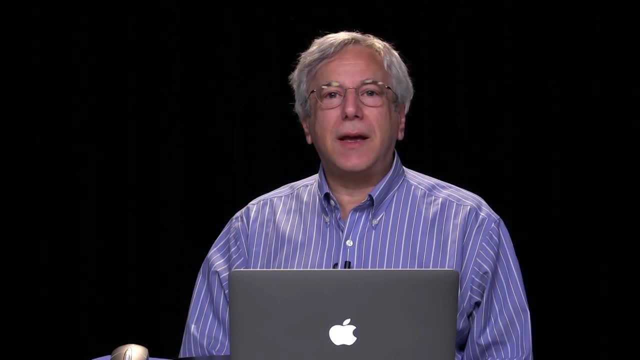 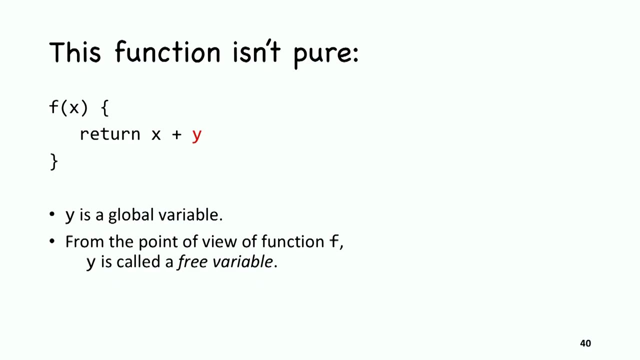 and it can return a result, But that's all it does. And if that's all a function does, then a function is much easier to deal with. Pure, that's what we call it. Good name for it, right, OK? 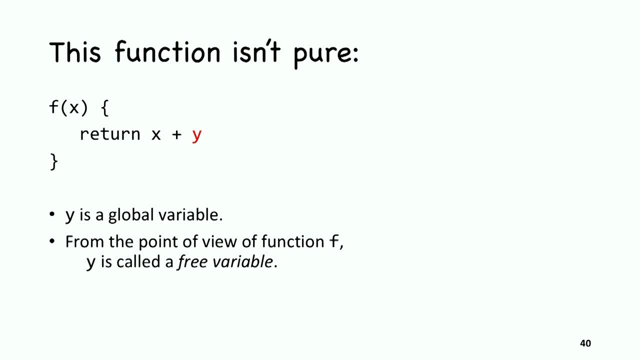 Let's take a look at some functions that aren't pure, just so that we get a feeling for the kind of things that again can go wrong. This first example: I have a function f. It returns x plus y- Whoops. 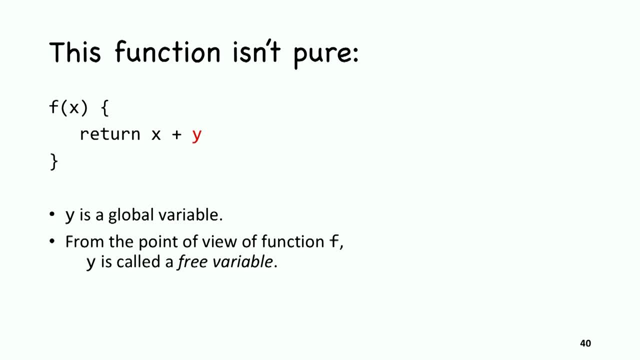 Wait a minute, That y I put it in red. Why did I put it in red? Because I don't like it. It's not that I don't like red things. I just wanted to bring it to your attention pretty graphically. 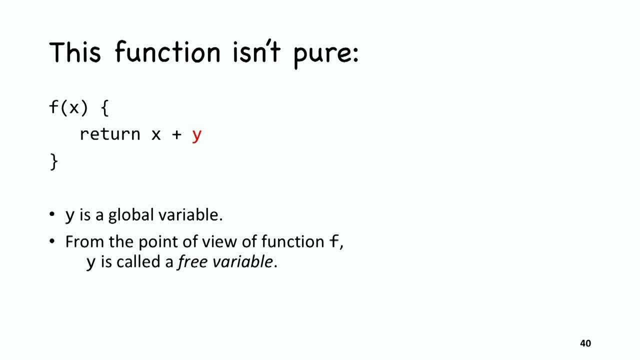 The idea here is that I feed it a value x and I think that what it's going to return is a value that depends on x. No, This particular function reaches out behind my back and finds a value y and says: oops, I'm. 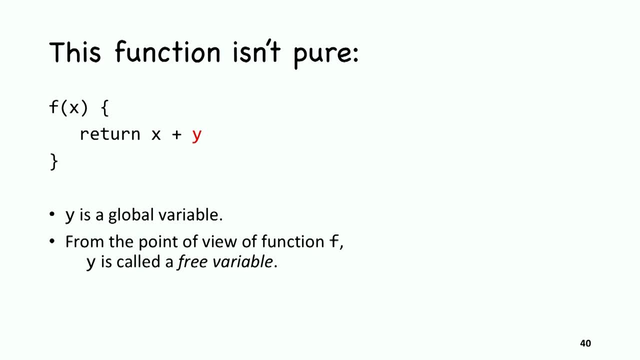 going to use that value y kind of secretly and add it to x and do something with it. You know, every time you call this function with the same value x- like the value x equals 3, you might get different answers. If you say f of 3, one time you may. 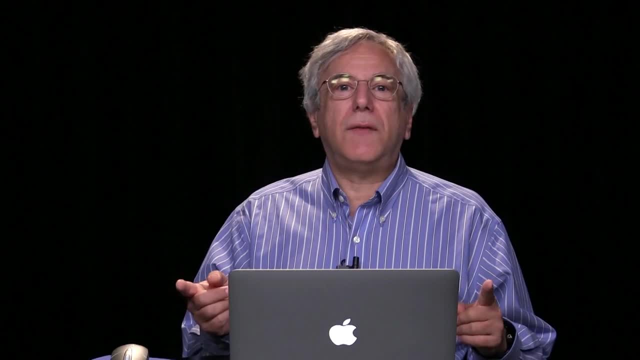 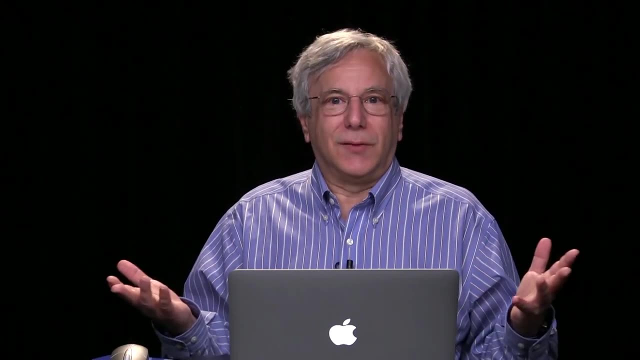 get 7,, because y happens to be 4 at that time. If you say f of 3 another time, a second time you might get 21,, because at that point y is 18.. So you don't always get the same value. 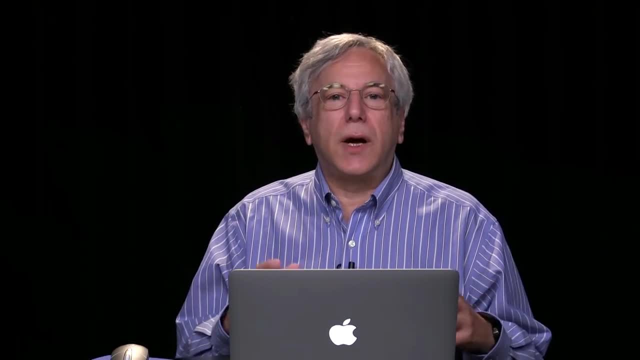 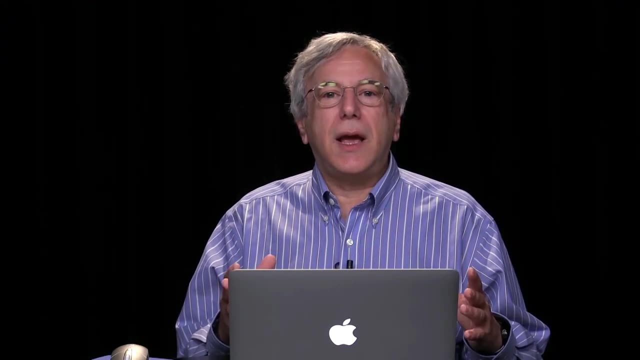 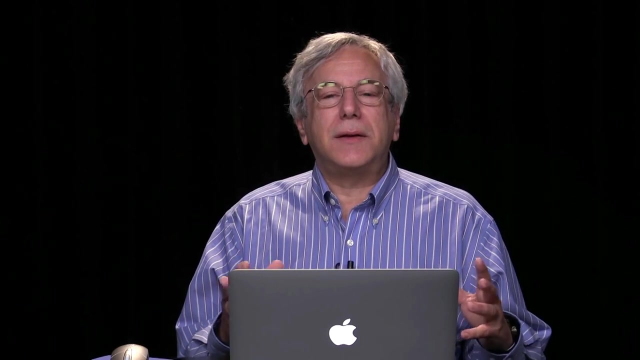 when you call this function In some languages we'd call y a global variable. The terminology I think that's used most often in functional programming is to say y is a free variable of the function f. y isn't bound to any other conditions. 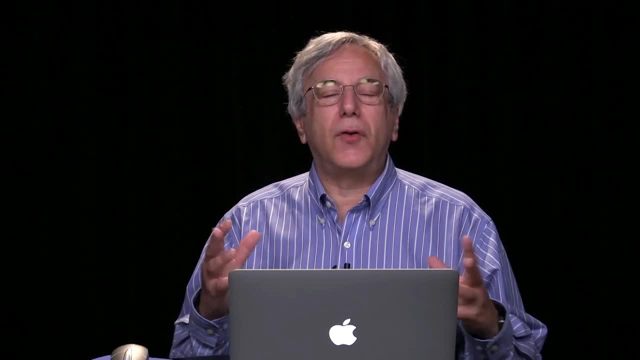 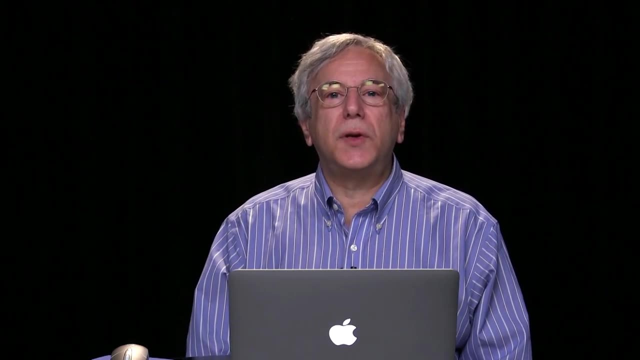 within the function f. It's kind of floating out there. It belongs to the global environment of the program. This is not good stuff. This function isn't pure. We don't like this function. We, as functional programmers, don't particularly. 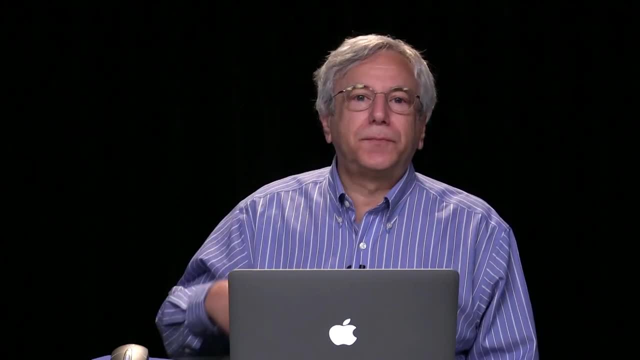 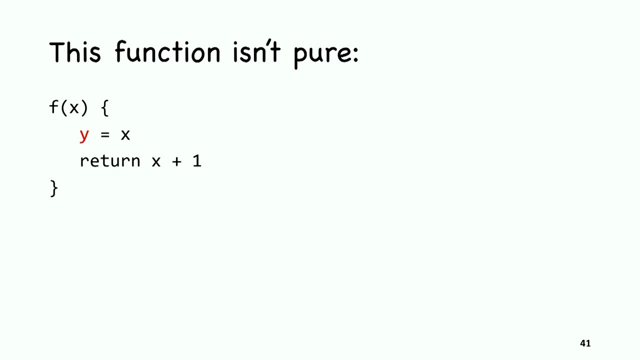 like this function. Let's see another example. OK, In this example I'm not using the value y, But I am changing the value y. It's the same as the example that I had earlier with the calculate function, where I modified the value of x. 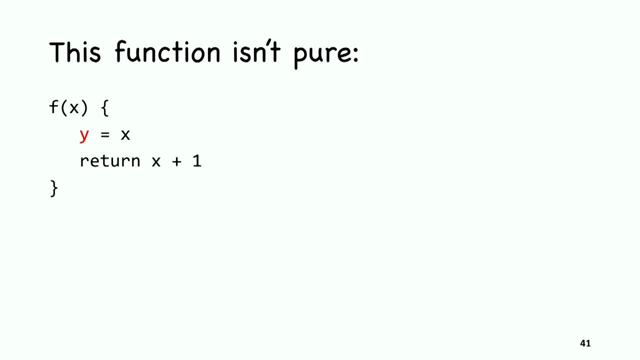 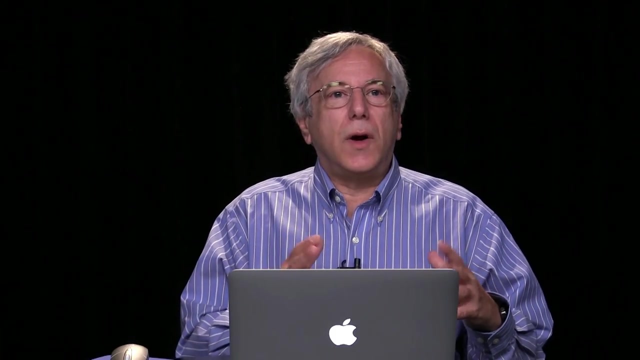 without telling you in the parameter list: Not good stuff. Once again, y is considered a free variable And this is called a side effect. It's an undesirable side effect. This function isn't pure. I just want to pick one particular area, that's. 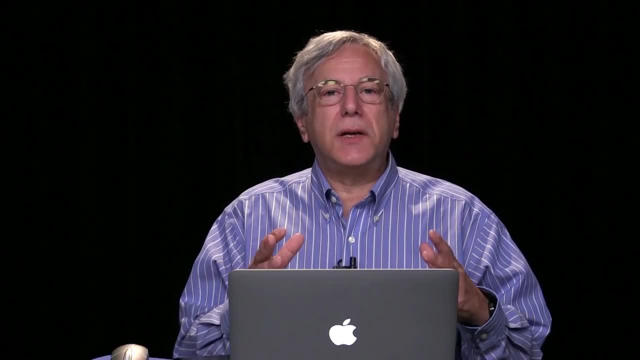 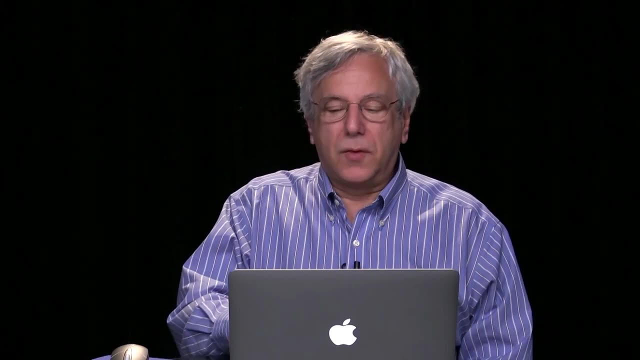 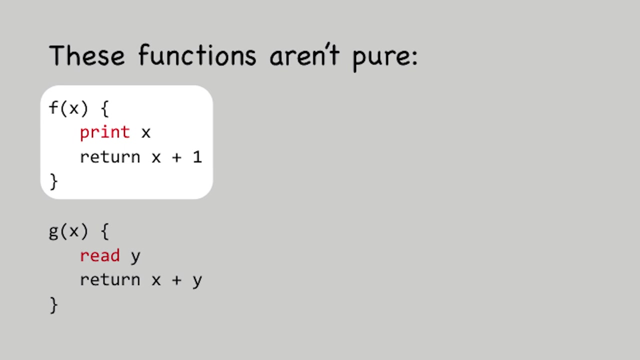 very different. It's very difficult to make pure, And by difficult I don't mean we can't do it, I just mean that it seems to be a problem point for many functional situations. There's the notion of printing and the notion of reading. 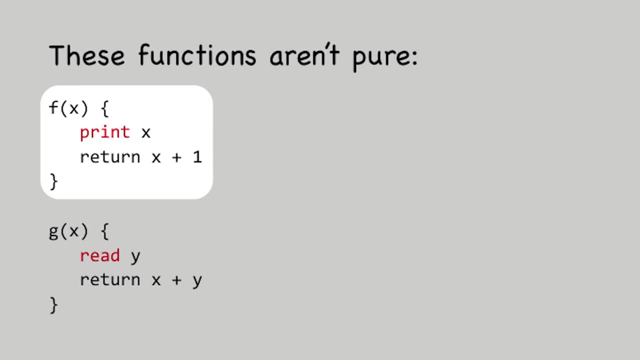 So I want to take a value that I have in my code and send it to the screen. Well, the screen is going to be external to my function. The screen isn't part of it. It's part of the internal workings of my function. 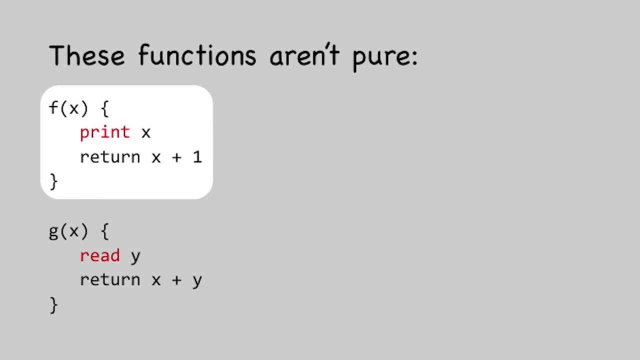 That's a side effect. I take a value like 3.. I print it And that 3 goes and changes something else in the system. that's not part of my function x. That's an impurity, unless I manage it in a way. 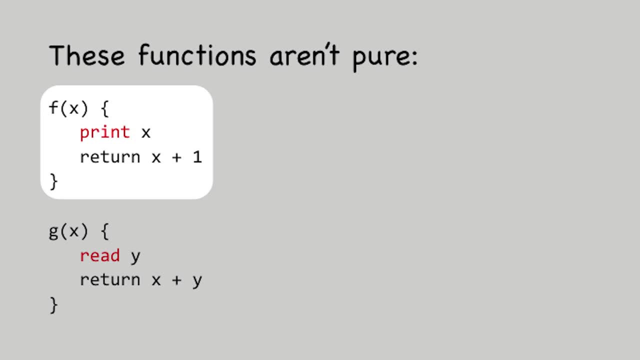 that I'm going to do in the last few segments of this course, But for now let's think of that as an impurity And of course, reading is going to be an impurity. So I am running my code. I encounter a function called g of x. 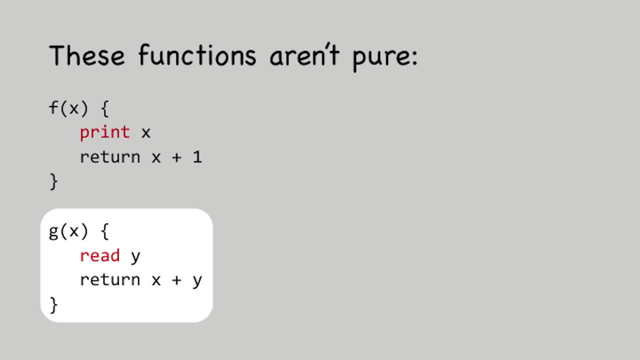 I get a value y, Notice again that y isn't part of the parameter list. So if I call g of x once with the value 3, I may read the number 4 and get back 7.. If I call g of x again with the number 3,, 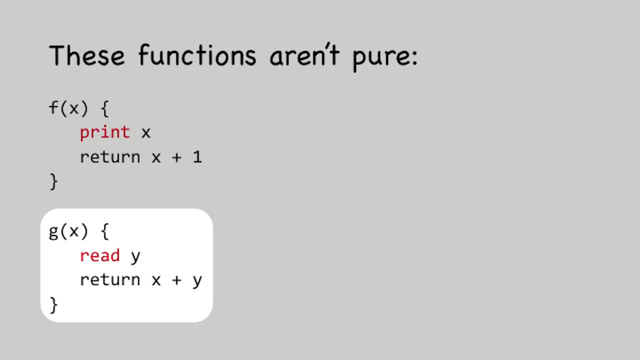 I may read the value 10 and get back the number 13.. OK, Once again I've got this situation where if I call g of x twice with the same number 3, I may not end up both times with the same answer. 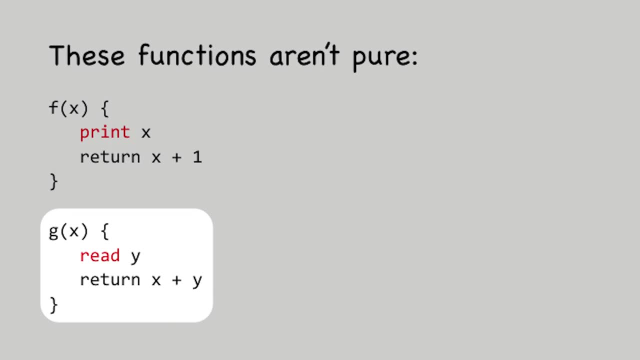 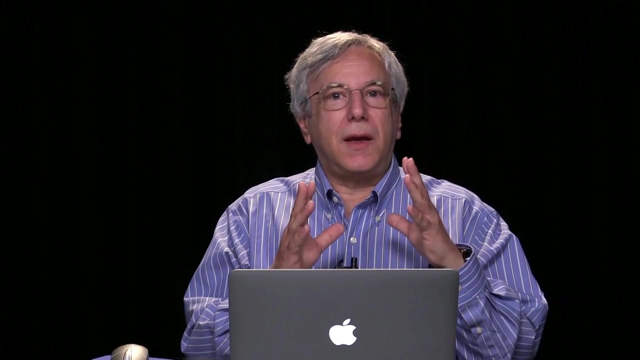 That could be confusing. Whoa Do we like confusing when we're writing computer programs? No, I don't think so. OK, So reading and printing are two points that, if we don't handle them in a very, very, very disciplined, 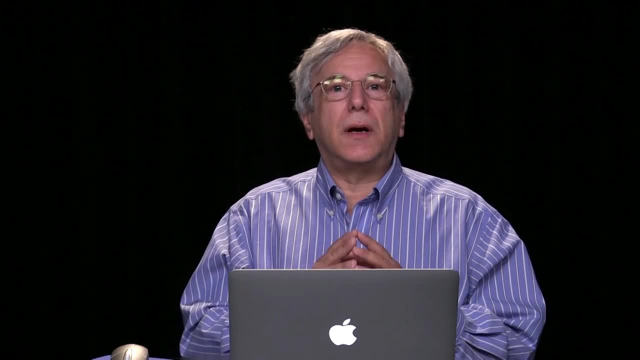 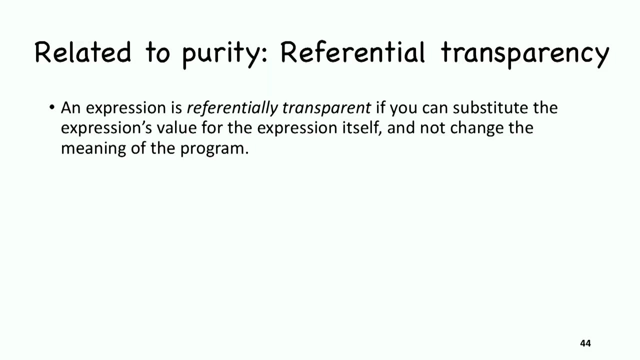 fashion, A fashion that I'll show you toward the end of the course. we're going to have impurities. We're going to have what we call side effects, things that we don't like happening. OK, I want to talk about something that is a bit theoretical. 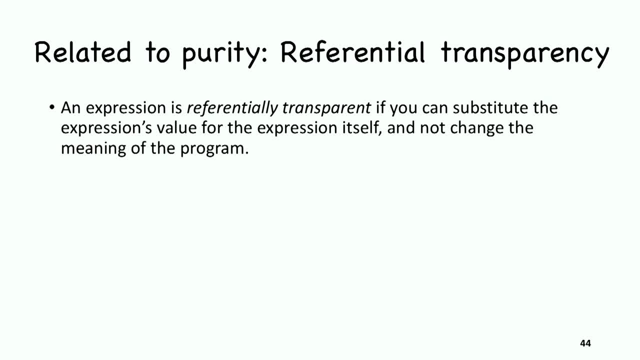 It's related to purity. It's called referential transparency. So let me read what it says on the slide. It's worth reading, It's good reading. An expression is referentially transparent if you can substitute the expression as a value for the expression itself. 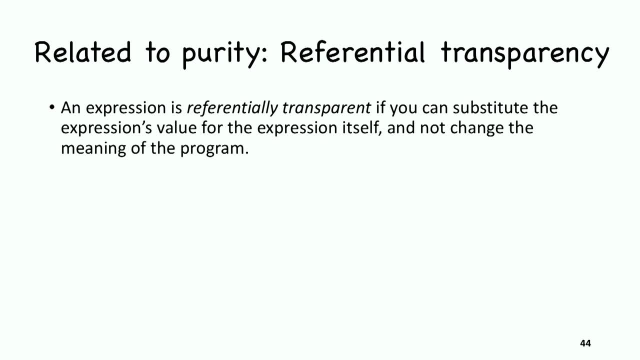 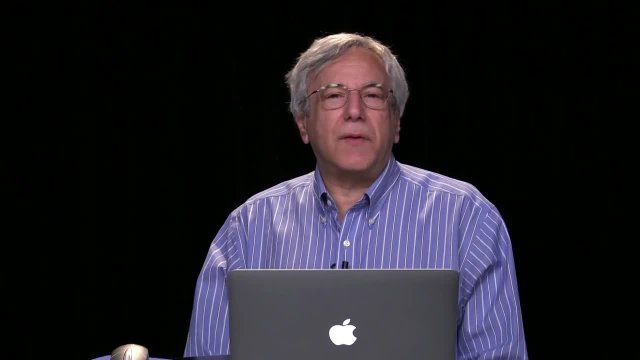 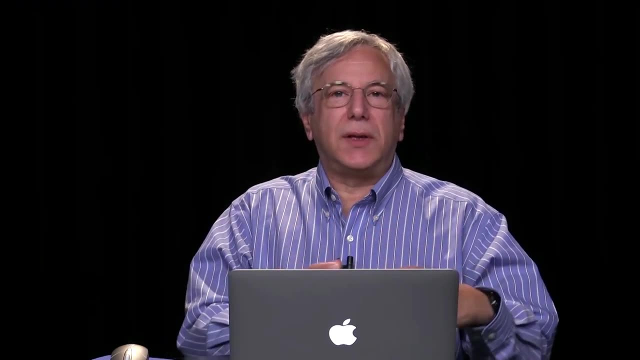 and not change the meaning of the program Seems to make sense that you would be able to do something like that in any program. You may not have ever thought about this. You take the value of an expression and you put it textually where the expression was. 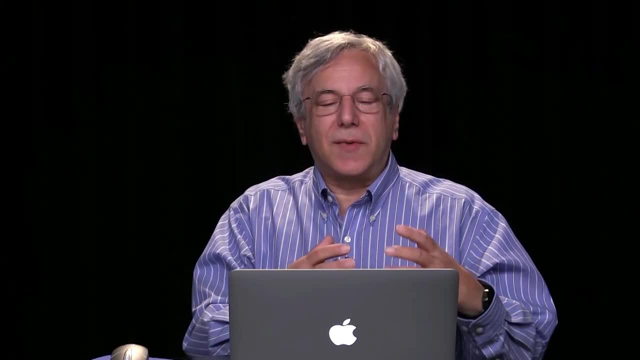 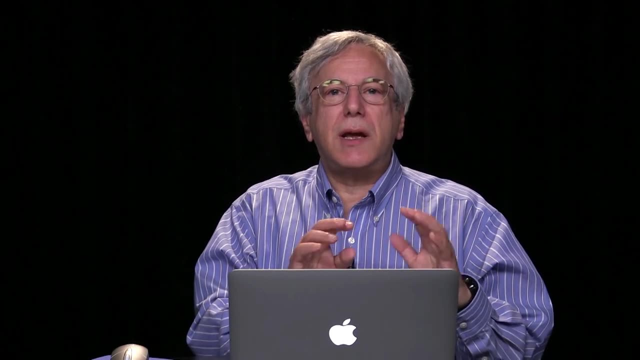 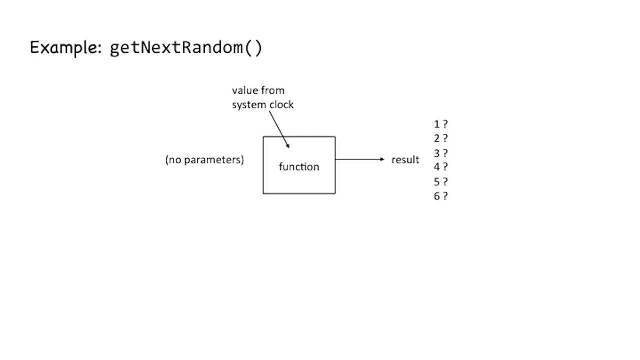 An expression and its value. those should be the same things. Well, Let's take an example and see if we have referential transparency everywhere in an imperative style program. Let's consider a function that we're going to call getNextRandom, And what getNextRandom does is well, it takes no parameters. 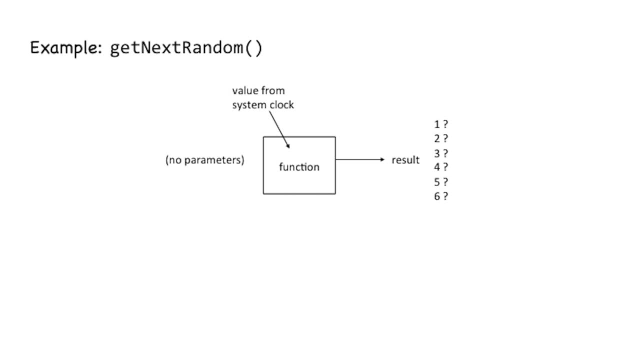 I'm not going to feed it anything. I'm not going to have a seed the way I have in some random generator, pseudo random generators. No, What I'm going to do is take no parameters And sort of get a value from somewhere. 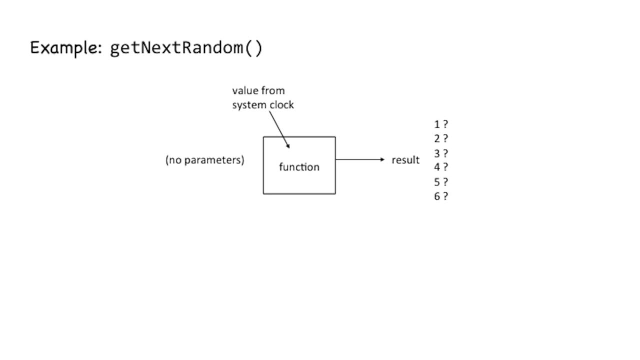 Whoops. Side effect: Getting a value from the system clock, Maybe the milliseconds, digits or something like that. That's what I'm going to use to seed this function and to produce a result, And the result that I'll produce should be different each time. 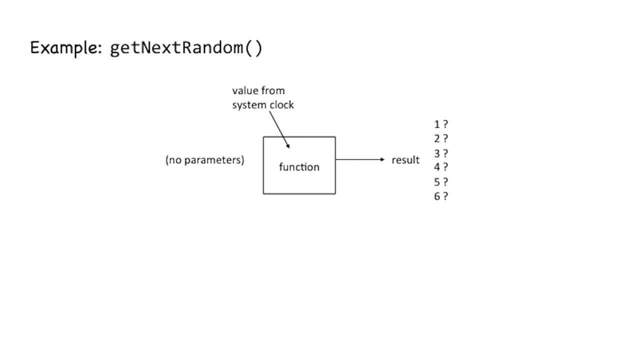 Because that's what pseudo randomness is. Let's say that I'm simulating the role. I'm simulating the role of two dice The first time I might be able to get, I don't know. two and four The next time from two calls to getNextRandom. 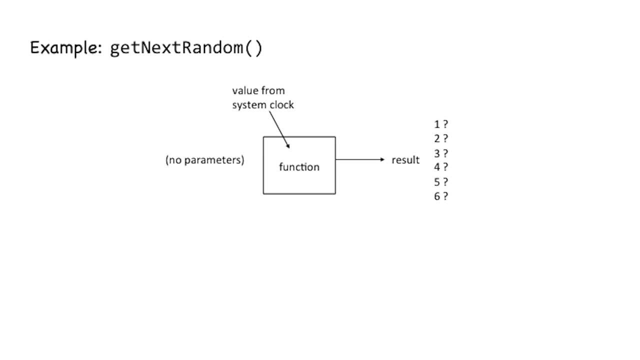 I might get one and six, The next time I might get three and three. So that result, that thing that should come out, should be different within reason, should be different each time, And of course I have a side effect there. 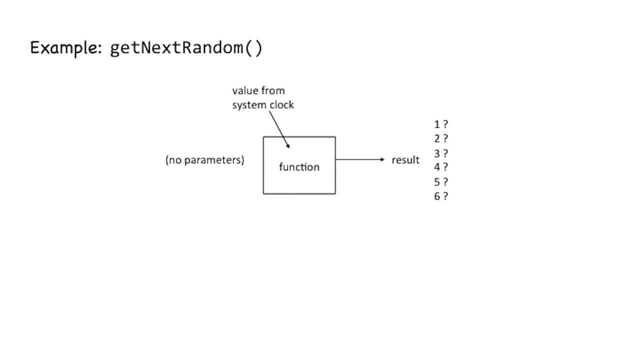 I admit it, And I'm taking no parameters. What I want to do with this function is examine it in terms of referential transparency, So let's see how that works. I'm going to claim that a call to getNextRandom is not referentially transparent. 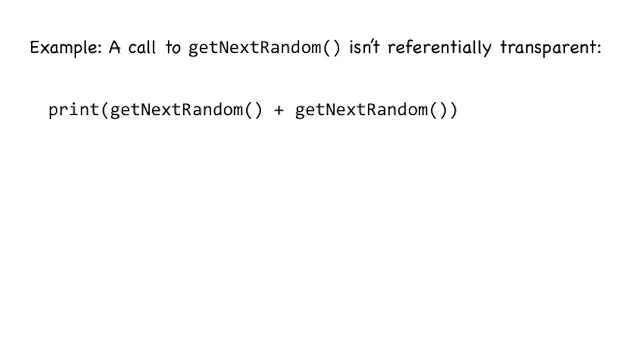 Let's see what happens. Let me print the result of calling getNextRandom and then adding to it getNextRandom again. Now, again, think about rolling a dice. So in this incarnation of my getNextRandom method function, I'm producing, each time I call it a number, 1,, 2,, 3,, 4,, 5, or 6.. 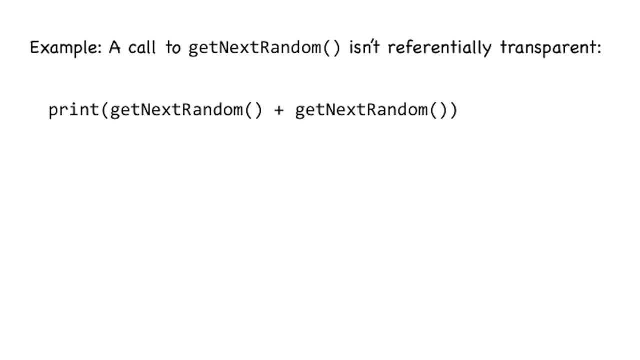 What can happen here? when I call getNextRandom, Well, maybe the first time I call it I get a 1.. And the second time I call it I get a 6.. Fine, that's great. OK, I got a 7 out of it. 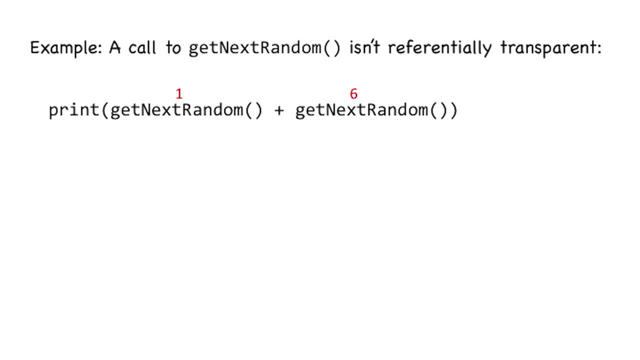 And so OK, OK, OK, I have a value 1 for getNextRandom and a value 6. And what I have in this statement is print and then two calls to getNextRandom. Now what I'm going to try to do in order, 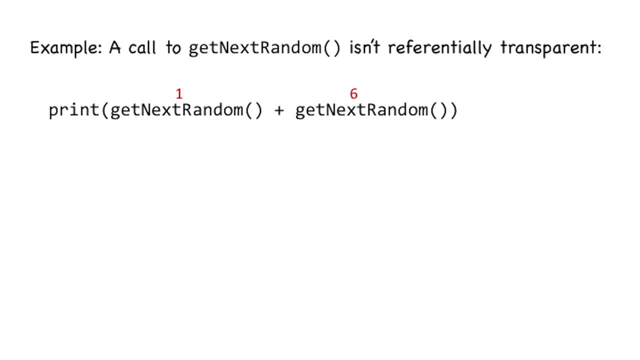 to test referential transparency is that I'm going to substitute for getNextRandom the value of a call to getNextRandom, And I admit it I'm going to be a little bit tricky And the way I do this I'm not just going to plug the number 1 and the number 6. 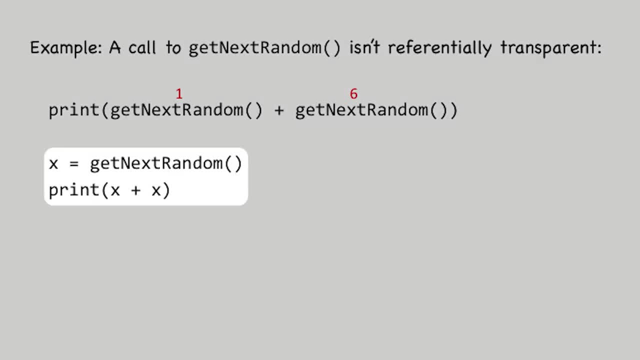 into that expression. Let me show you what I'm going to do. I'm going to call getNextRandom, I'm going to assign whatever I get from it to x, And then I'm going to say: print x plus x. That's the kind of substitution that I should be able to do. 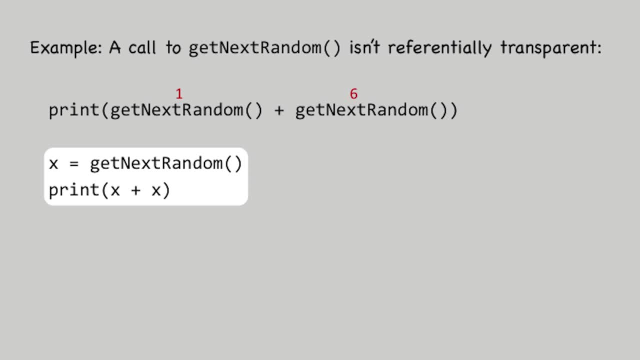 if I have referential transparency And if I do that substitution, I'm going to get a 6. And if I do that substitution, I should be able to get the same result. Well, as you might have already guessed, I don't get the same result, Or I don't always. 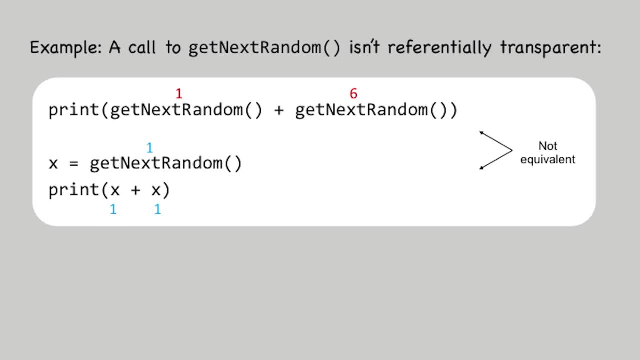 get the same result. And the reason is because in this world, the first call to getNextRandom supplies a value of 1 for me, That gets assigned to x, And then, when I substitute the value of the expression getNextRandom that x. 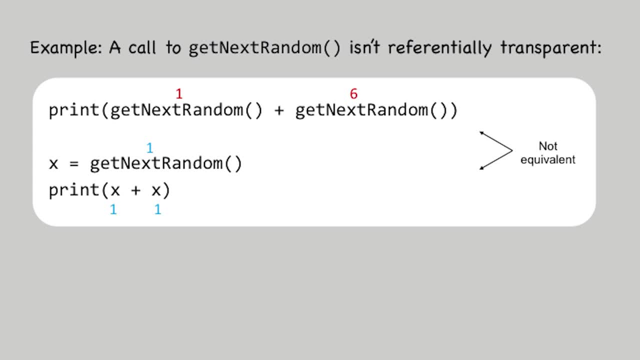 For the getNextRandom call, I get 1 plus 1, which is 2. It's not 7.. So a call to getNextRandom isn't referentially transparent, at least not the way we've set up our getNextRandom function. 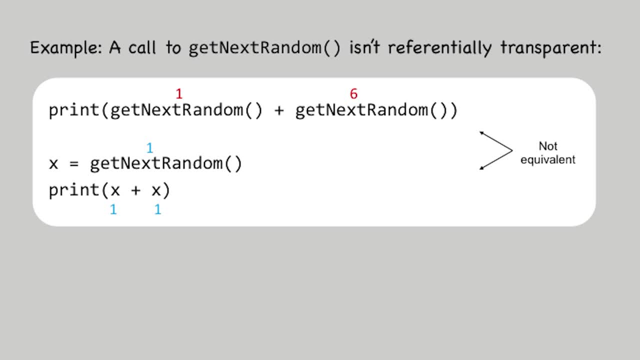 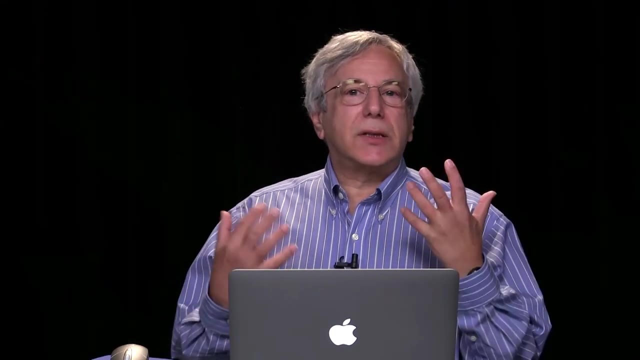 If we want getNextRandom to be referentially transparent and pure, we have to do something called monads. I'm going to discuss monads at the last part of the course. We've already talked about referential transparency in the way it's sort of related to well. 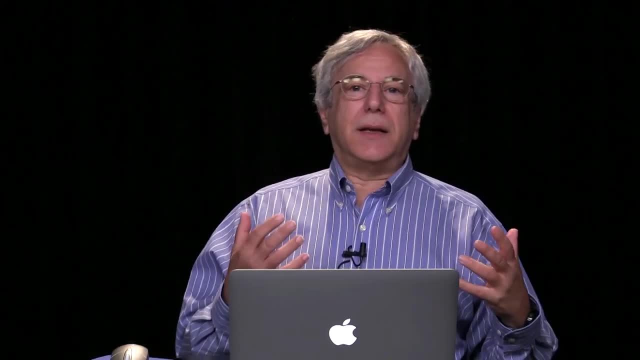 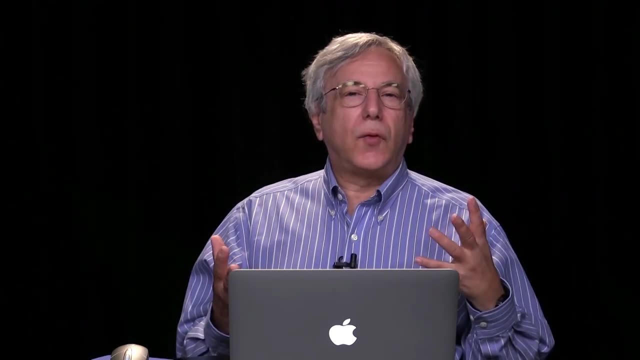 it is related to purity, But I haven't made an exact link. That's fine. I also want to talk about something called immutability. Immutability is something that you've probably already heard of if you've looked at even the imperative languages. 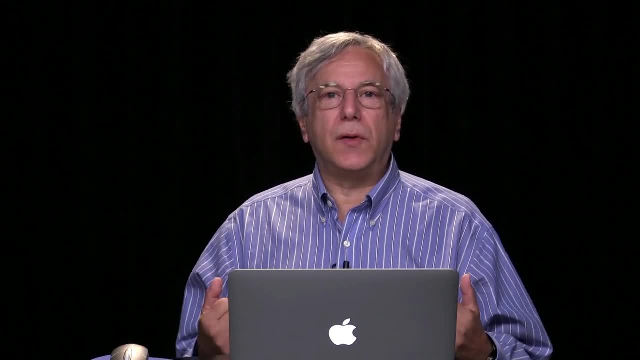 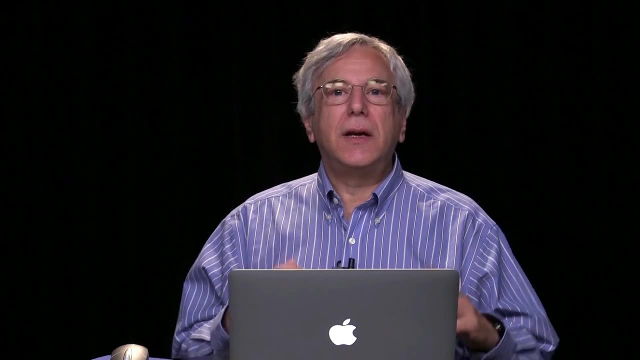 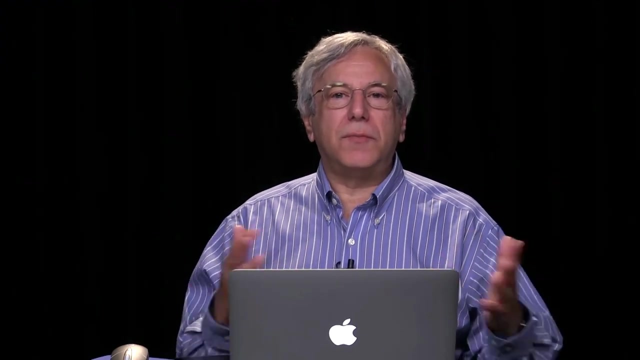 It's nice when quantities are immutable. Mutable quantities, quantities that can change on us, quantities that are time dependent, are difficult to manage, difficult to handle in lots of situations, And I'll talk about mutability and the difficulty of managing such variables in a later segment. 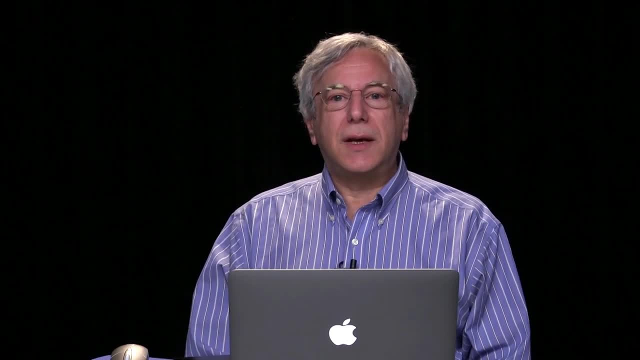 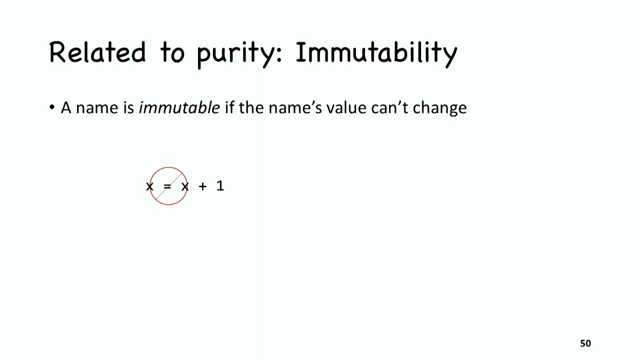 But for now, let's just take a look at what mutable means and see what we can do with mutability as far as functional programming is concerned. Well, here's the textbook. Here's the textbook example of mutability: I've got a variable x. 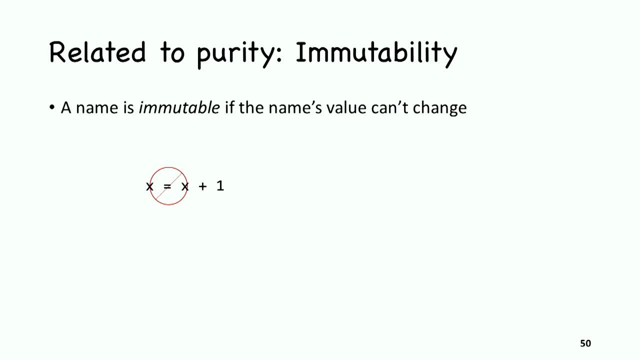 I add 1 to it, I change the value of that change, mutate the value of x so that x becomes what was formerly called x plus 1.. So if x started off being 6, now x is 7.. Well, that means that when I analyze the behavior, 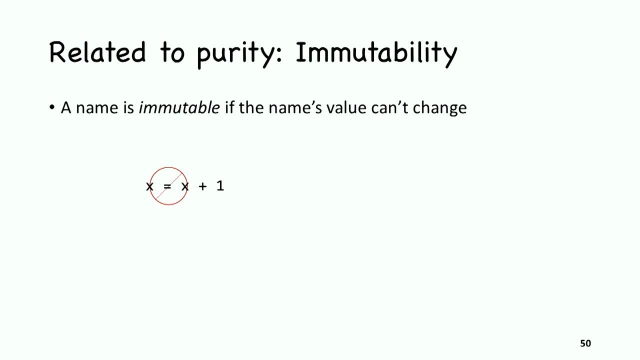 of a program. I've got to consider an extra dimension. I've got to consider the time dimension. I can't say that x has a value throughout the run of the program. I have to think of the program as a mutating blob where x starts. 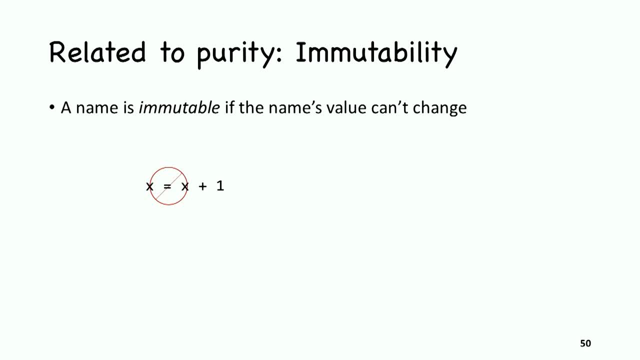 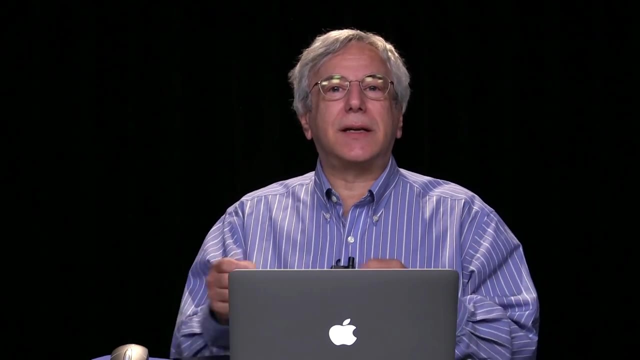 off with one value and could mean something else later. and could mean something else later. You see how mutability creates a problem for referential transparency, Because with referential transparency I should be able to substitute the value of x everywhere I see x itself. 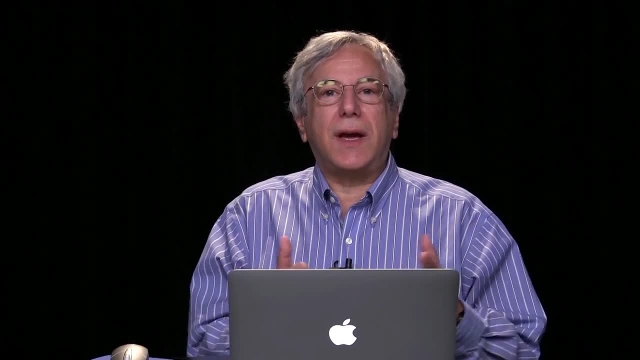 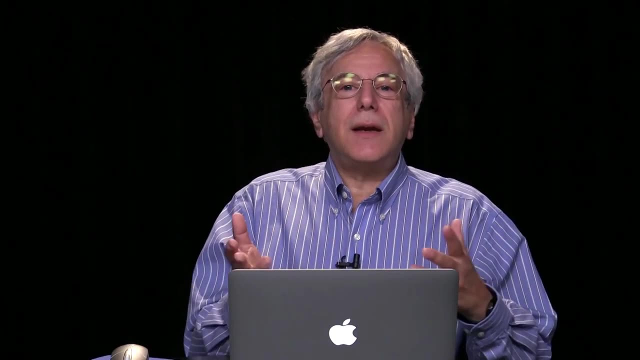 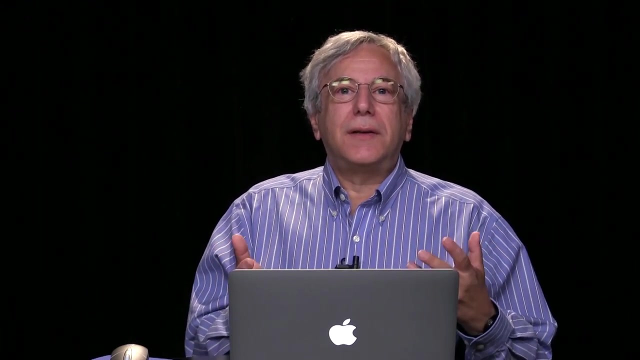 However. However, if x's value changes, if x's value is a moving target, then this notion of referential transparency is hopeless And, in fact, if x is something that exists outside of my function f, then I shouldn't be having f mutate the value of x. 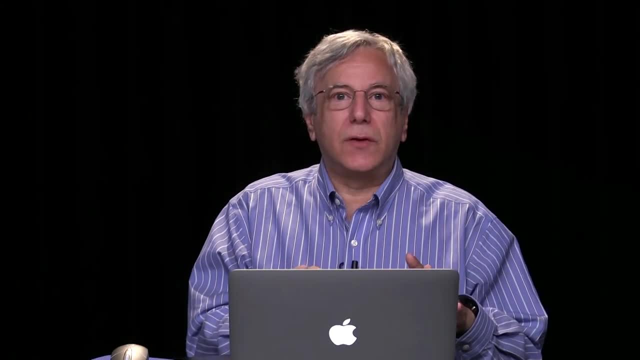 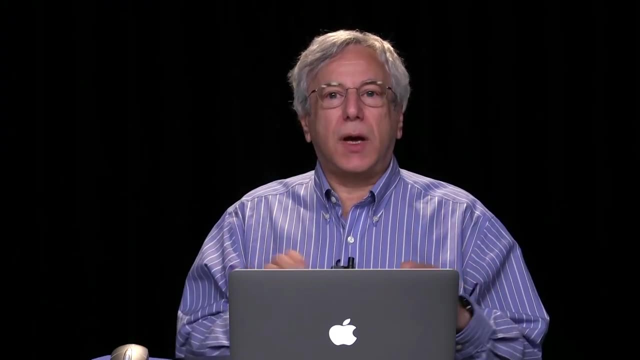 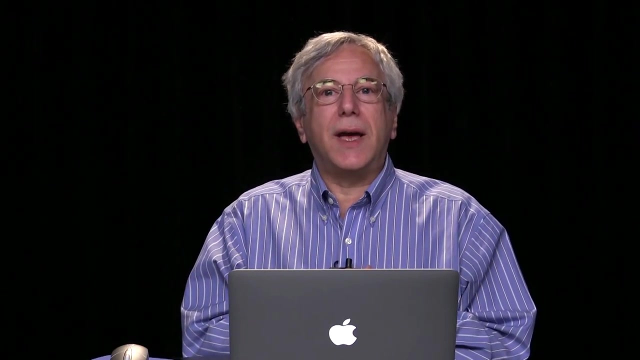 And worst of all, worst of all, absolutely worst of all, I shouldn't have two agents in my program, Right, I shouldn't have two threads in my program, two processors, two different parts of my system trying to modify the value of x. 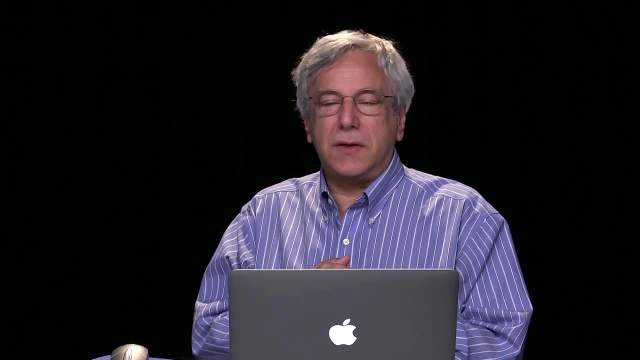 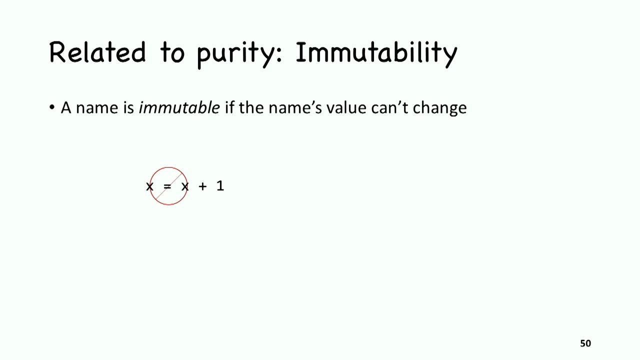 simultaneously. That leads to real confusion and is very difficult to deal with. OK, How does functional programming help with the mutability problem? How does functional programming help me take what would be a situation with mutable values and turn it into one with only f? 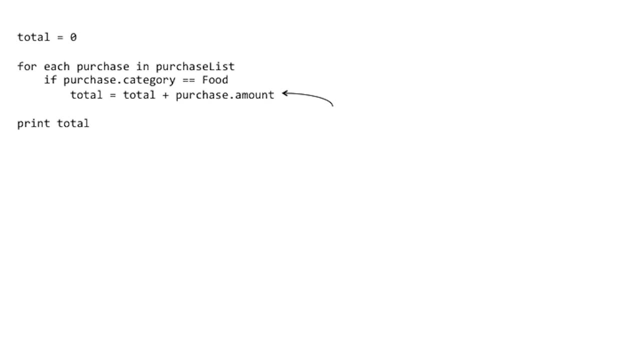 How does functional programming help with only immutable values? Recall in an earlier slide that I talked about a situation where you want to take a bunch of purchases and add together their purchase amounts and get a total. Here's the imperative solution to that problem. the solution. 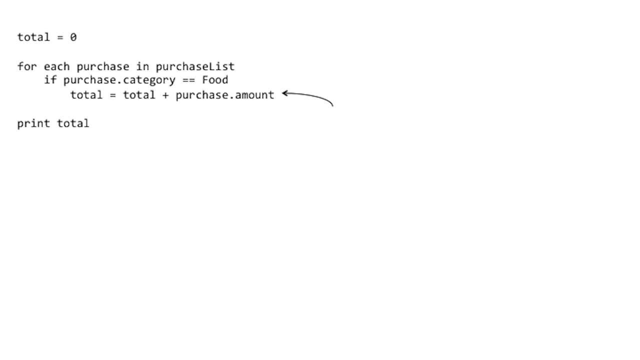 that I gave in the earlier slide. It's an exact copy of one of the solutions. OK, I have the arrow pointing to the words total equals f. OK, I have the arrow pointing to the words total equals f. OK, I have the arrow pointing to the words total equals total plus. 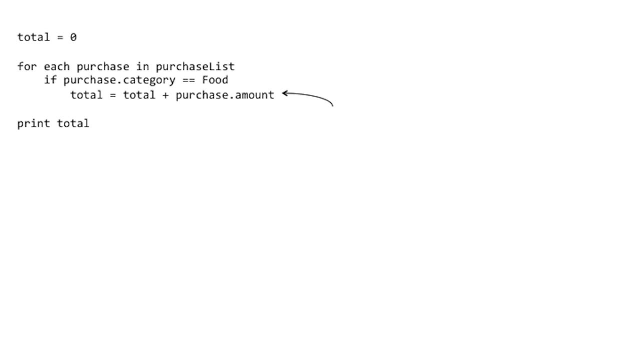 purchase amount. because total is a mutable variable. The value of total is time dependent. It changes from one part of this program to another. In fact, every time you enter that for loop you have the possibility of modifying the value of total, And total is not defined inside of the for loop itself. 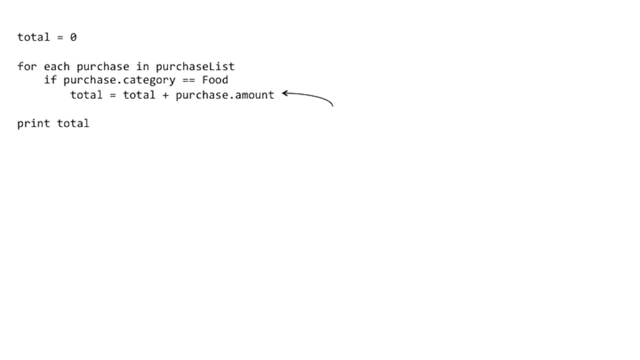 So you could sort of say that this for loop isn't pure. It's modifying something that's defined outside of it, The for loop. you may not consider it a function, because I haven't separated it from the rest of the code. It's really in line. 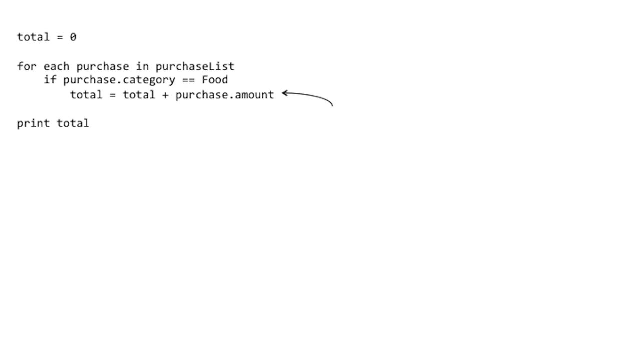 But we've got some impurity here, We've got some problems. Anyway, what I want to focus on is the fact that total gets mutated And there's really no way to change that, the way I've structured the solution to this problem. 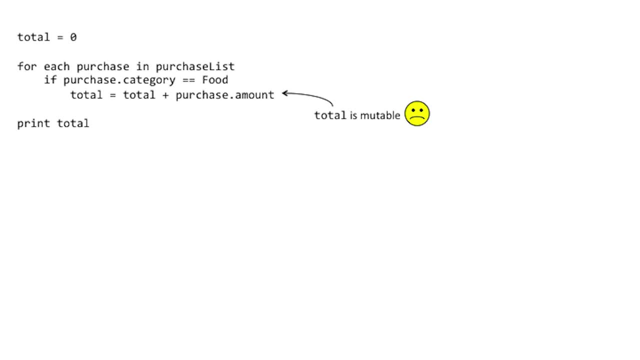 OK, I made very drastic changes to the code. Maybe I could get it so that total wasn't a mutable variable. I don't know. Looking at it the way I'm looking at it, it's hard to imagine how I would do that. 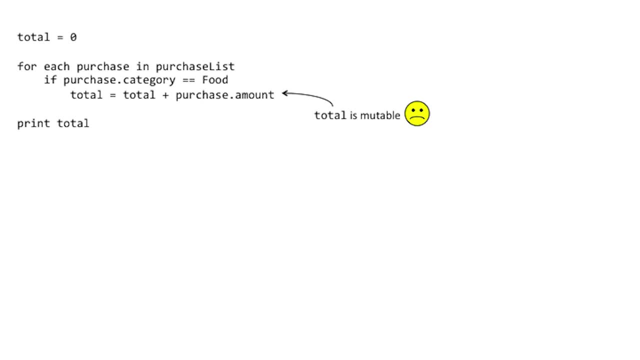 But if I think about this functionally, what you see at the bottom of the screen now is the functional version of this program, the functional solution to the same problem of finding the total of all the purchases that were food type purchases. Now let's look across this nicely colored line. 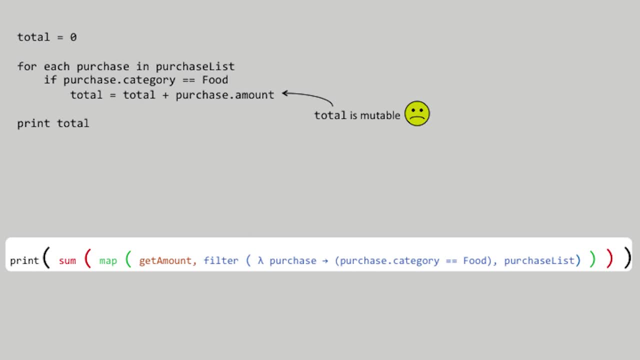 We've got get amount: That's a function. We've got filter: That's a function. We've got map- That's a function. Hey, we've got that lambda expression- That's a function. We've got one thing, that is just one name. 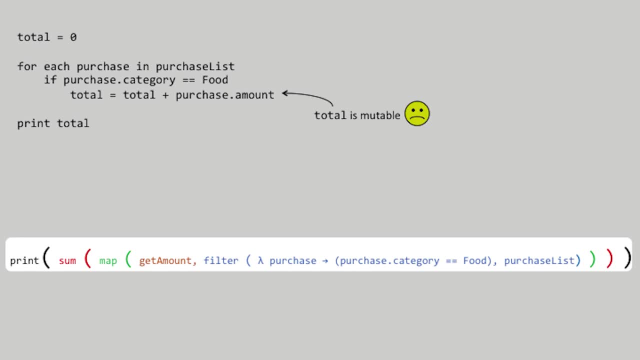 It's purchase list. Purchase list is just one name, So the question is: what do we know about the mutability or unmutability of purchase list? That's something that could potentially change, could it? OK? If I look at this expression, this whole expression, 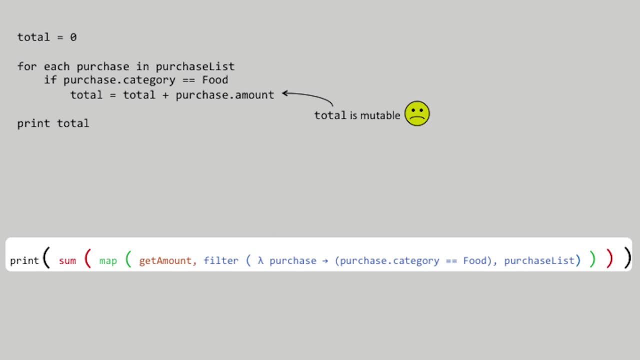 I'll discover that purchase list does not have to change, does not have to mutate, as part of this calculation. As a matter of fact, purchase list doesn't change at all during the evaluation of this expression. I start with the purchase list. I filter for purchases that have category food. 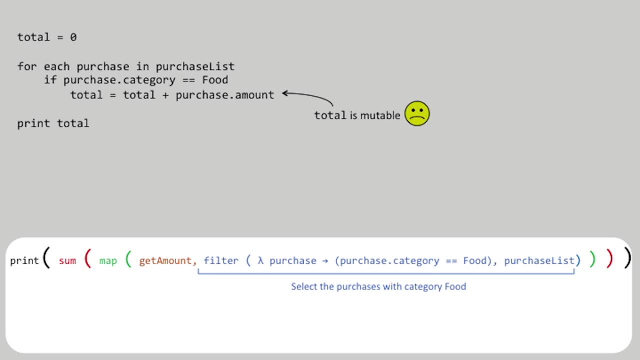 And that gives me a brand new purchase list to which I apply the map get amount, which gives me a new list of amounts. So I'm always getting new lists until, of course, I do a sum, at which point I get a new value: the sum of all the purchases. 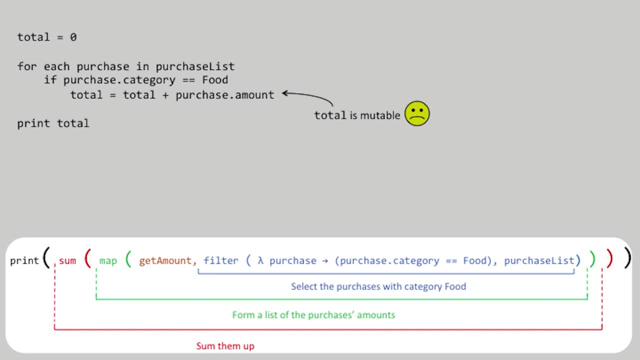 But no way. So where in this entire expression am I saying change any of the purchases? I'm not changing anything here. Now could I change a value in purchases list? Well, I haven't said explicitly anywhere in the code that purchase list isn't going to be changed. 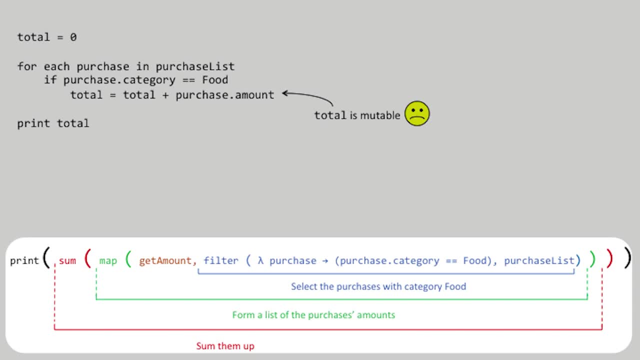 But notice that the way I've got this functional line of code set up, changes simply don't happen. They don't have to happen. Nothing has to be modified here. I have achieved immutability just by thinking of the problem functionally. 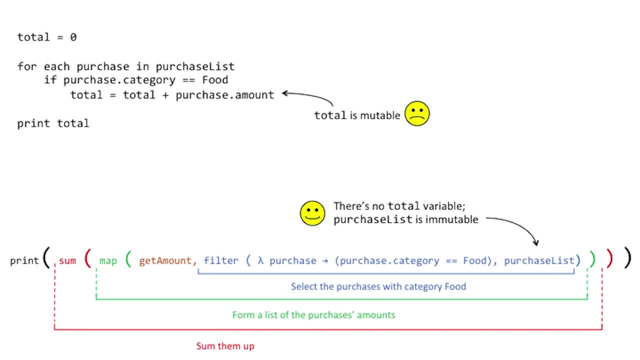 Wow, If you can get rid of mutability and you can make your functions pure, well then you've got code that's much, much easier to manage, And one of the things that functional programming is about is about managing code, making it correct. 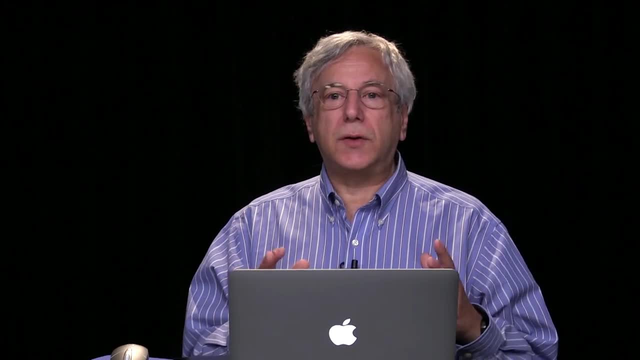 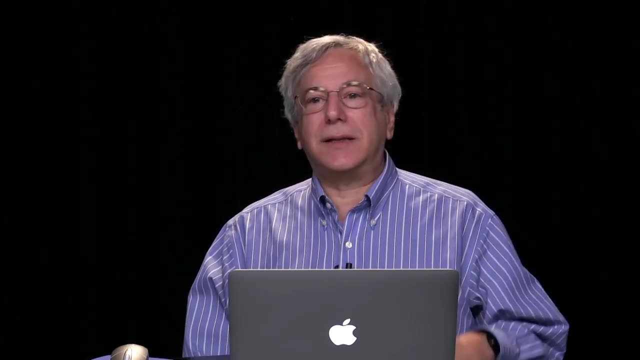 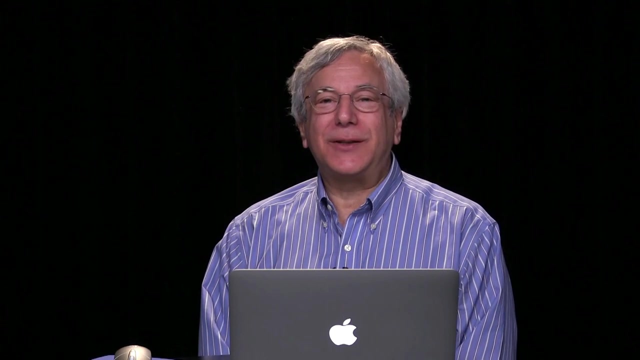 making it easier to maintain. It's all good stuff, and we'll talk more about the benefits of functional programming and pure functions in the next section. In the previous segment, I talked about pure functions. Now, if you're going to call something pure, 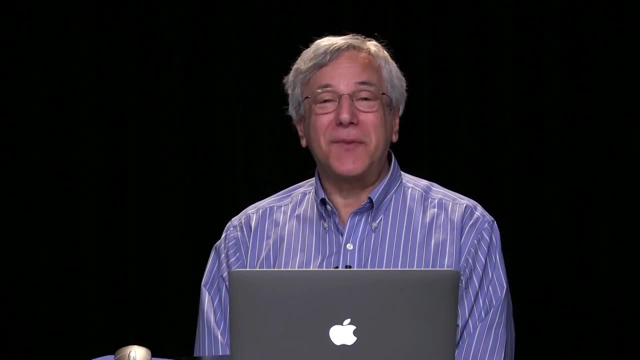 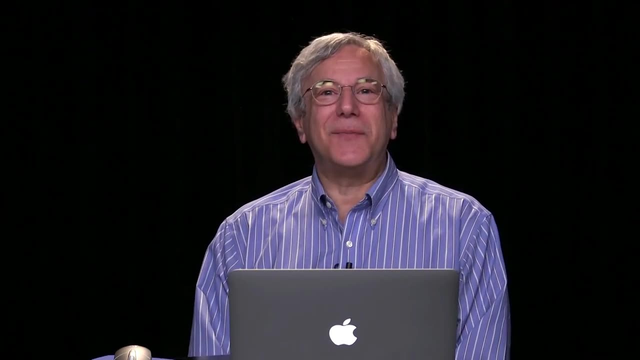 you better have a darn good reason for thinking that it's something that you like. I'm not going to call something a pure function if it's something that I don't like and that doesn't give me any benefits. So In this segment, what I want to do, 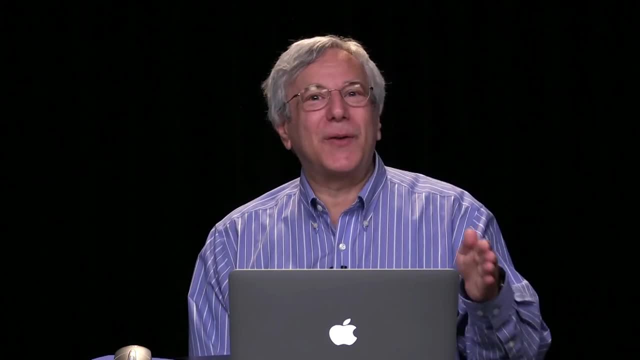 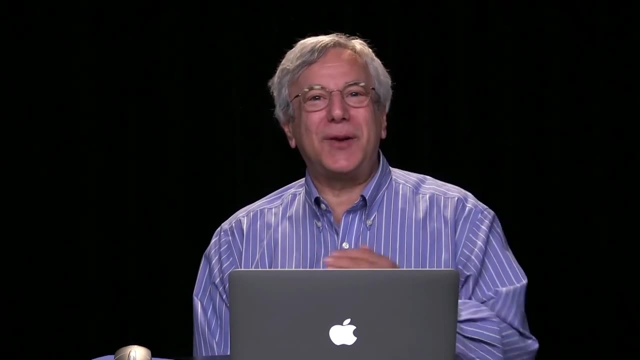 is talk about just the tip of the iceberg for the benefits of pure functions. Some of the benefits of pure functions are going to be a little bit more effort for me to explain, so I'll save them for the next two or three segments, OK. 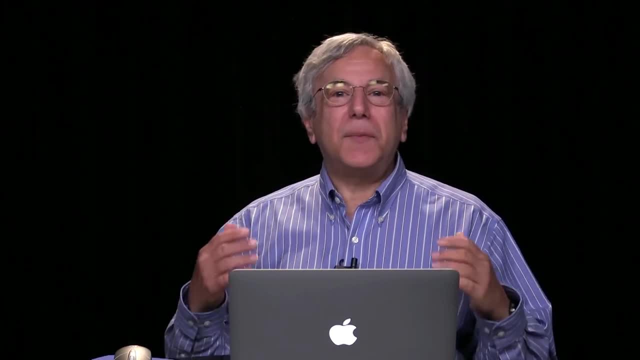 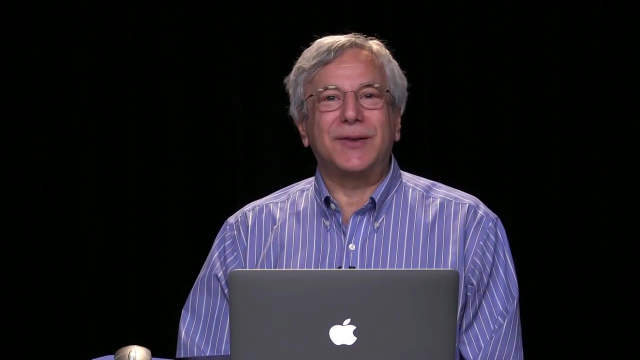 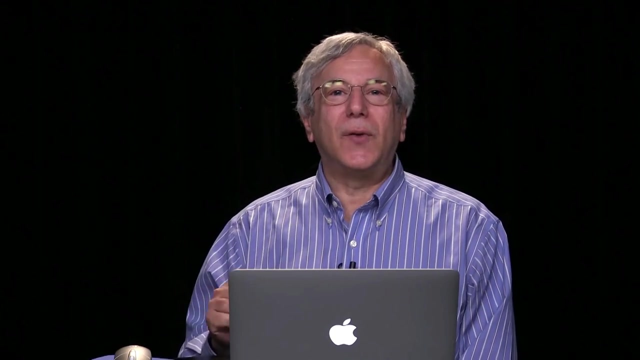 Let's start off with a few benefits. Look, If you've got a pure function, then every time you use it it's going to give you the same answer. It's not going to go. It's going to grab values from the global context. 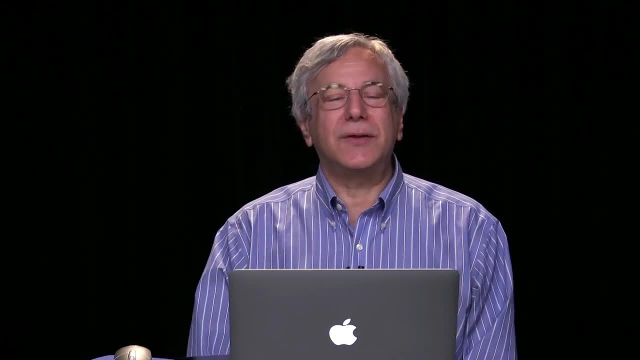 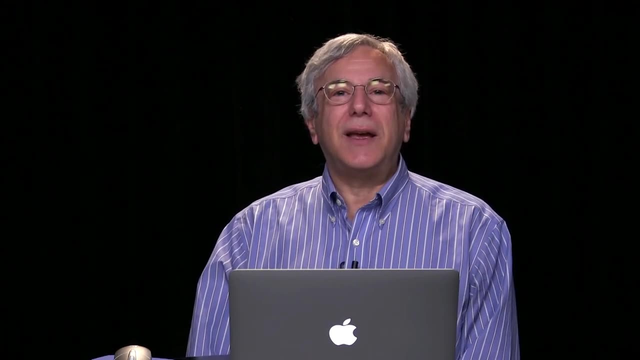 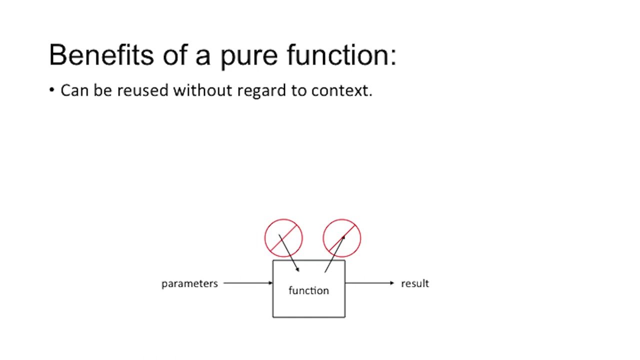 or from the keyboard and use those values to give you a brand new answer. So if I have a function that's pure, then I know that it'll give me the same answer each time. It won't be giving me different answers and I have to worry about how those answers come about. 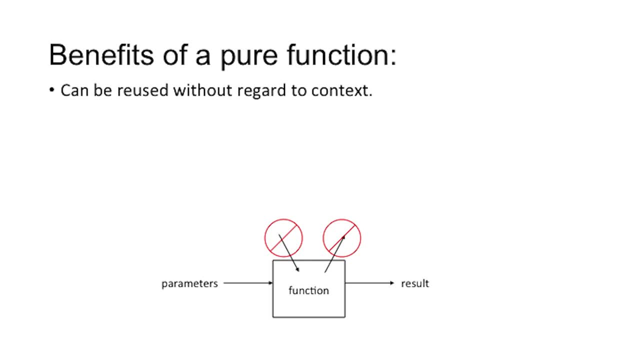 from the enclosing context. I don't have to worry about what the user is typing on the keyboard. I don't have to worry about the values of variables that aren't defined inside the function. So if I have a pure function, I can reuse it. 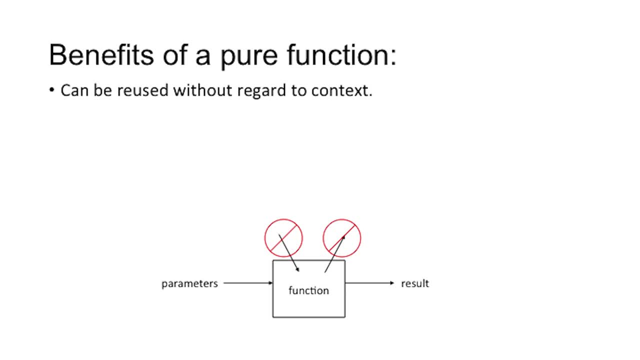 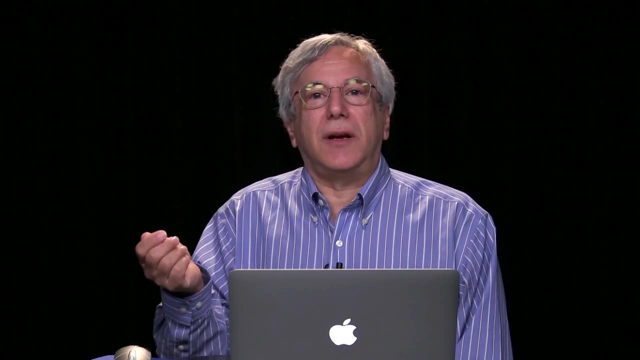 without worrying about that context, without worrying about the values of surrounding variables. Not only do I have to not worry about the values of those variables because they won't affect the outcome, I also won't be changing the values of those variables because I don't want to be using the function over and over. 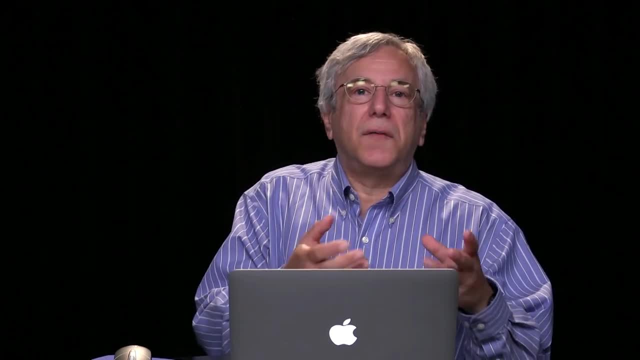 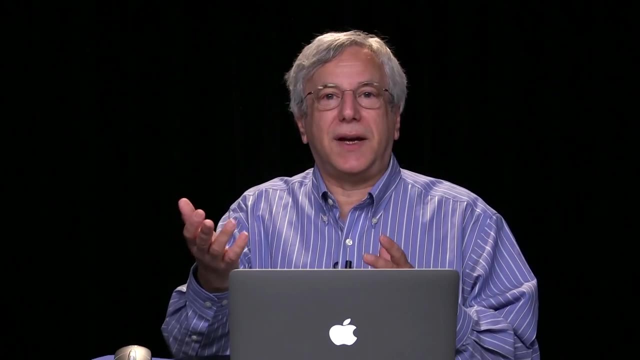 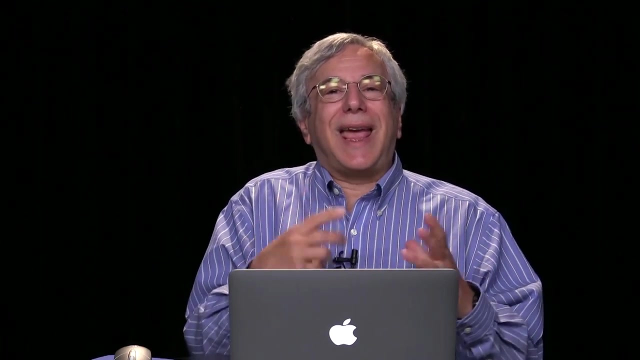 and over again. Imagine for a moment a function that writes something onto the screen. That's OK. In this part of the course, I'm going to call it a side effect. A function writes something onto the screen. What that means is that it makes a change to something. 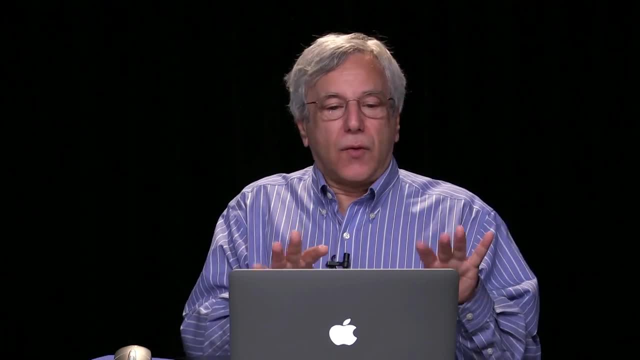 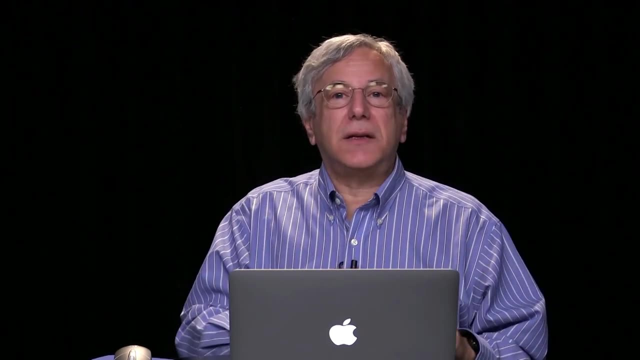 external to itself. Now if I reuse that function, so if I use it once, it writes something to the screen. If I use it A second time, it writes again to the screen. wait a minute, I have to worry about using it a second time. 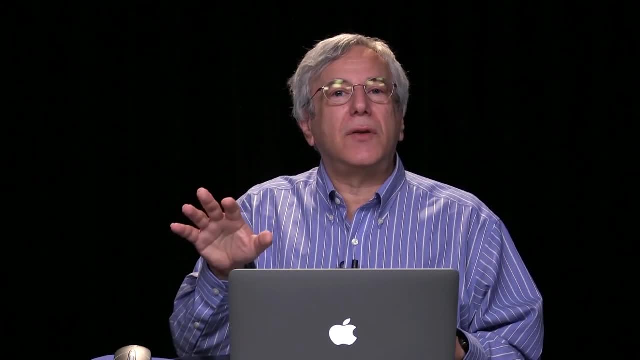 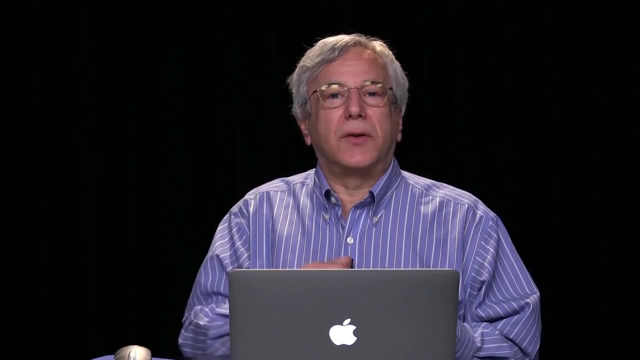 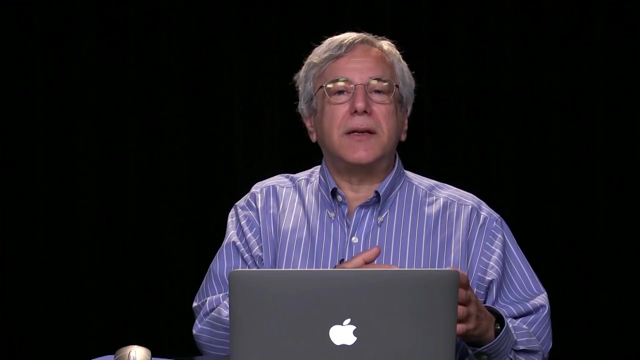 because maybe I didn't want whatever got written on the screen to get written twice. What if I have a function that adds one to some external variable? Calling it once changes that variable from 10 to 11. Calling it a second time changes that variable from 11 to 12.. 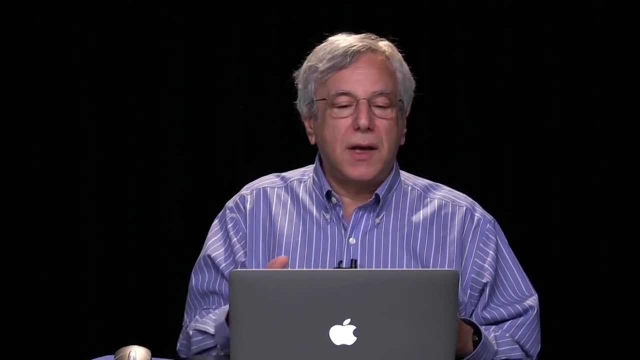 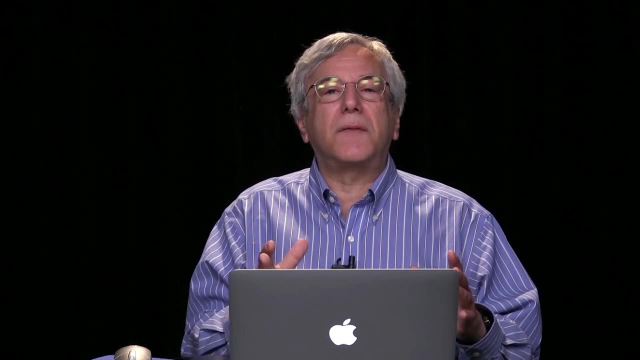 So every time I call it it makes a change to the environment. If I have a function that's pure, I don't have to worry about anything that's going on outside the function, except the fact that the function accepts its parameter values and returns a result. 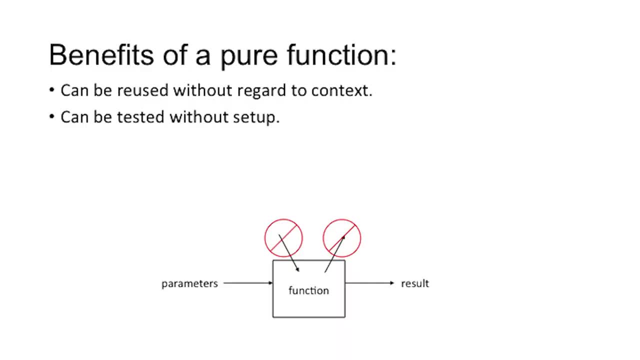 Benefit number one: a pure function can be used, reused, without regard to the context. Benefit number two: it can be tested without setup. In order to test a pure function, all I have to do is feed it whatever parameter values I want to feed it and find out what the result is. 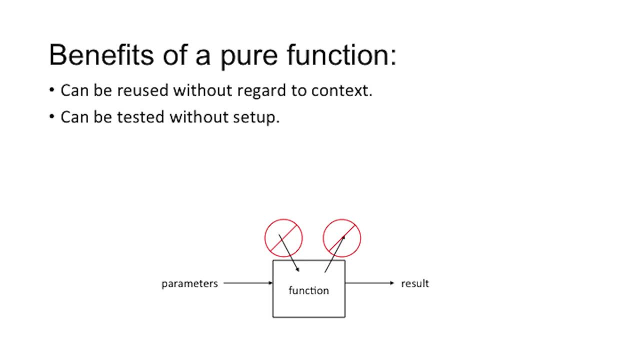 I don't have to say OK, well, the user has to be typing something on the keyboard while this function is being executed. so I don't have to worry about that external setup. I don't have to worry about the environment and the value of a variable that's outside the function. 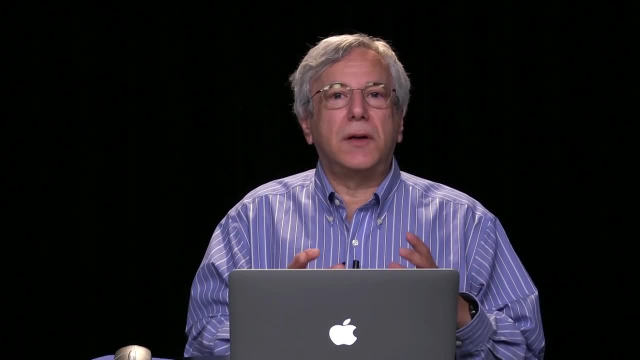 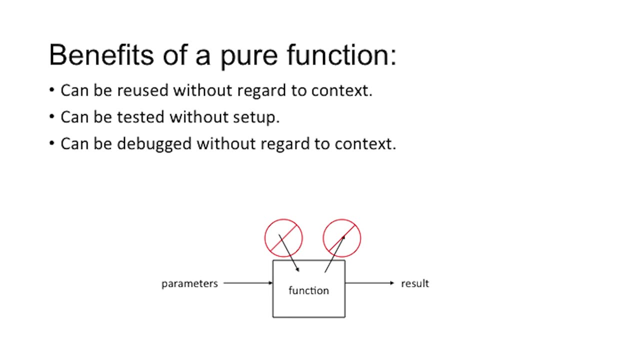 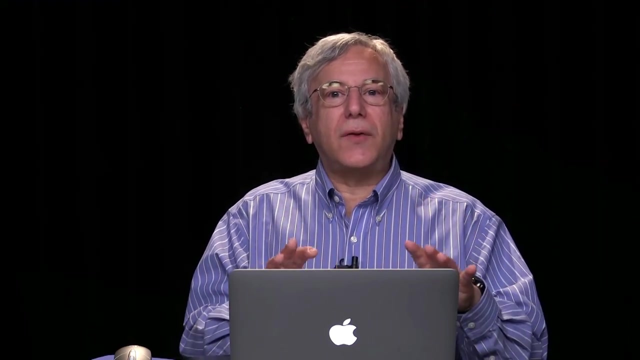 I can test without setting up the environment in which the function is going to be executed, and that's a benefit. And I can also debug without requiring regard to context. How many times have you tried to test debug a function and found that one time the function works just fine? 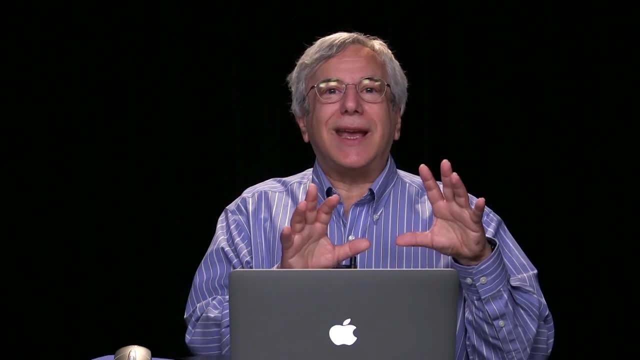 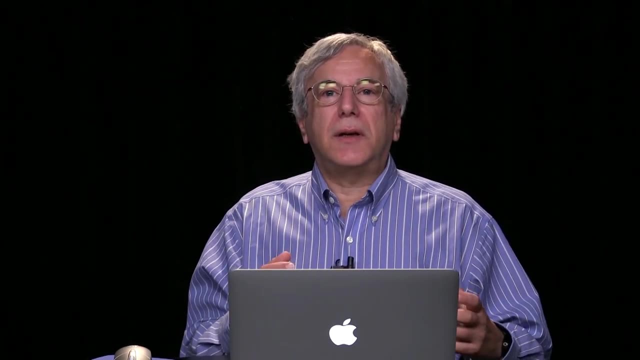 another time. the function works erroneously. You have a function, You run it. Oops, it gave me the wrong answer. Let's see if we can debug this function, find out what's going on. Let's run it again and see what happened. 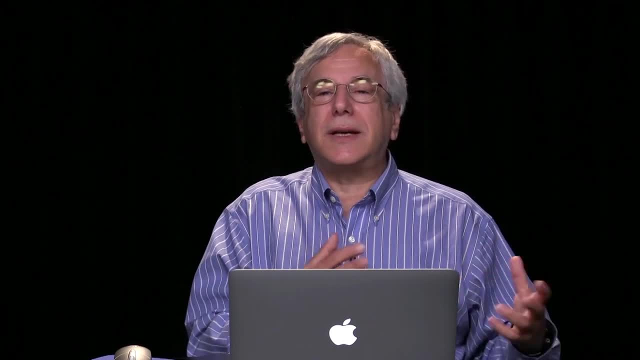 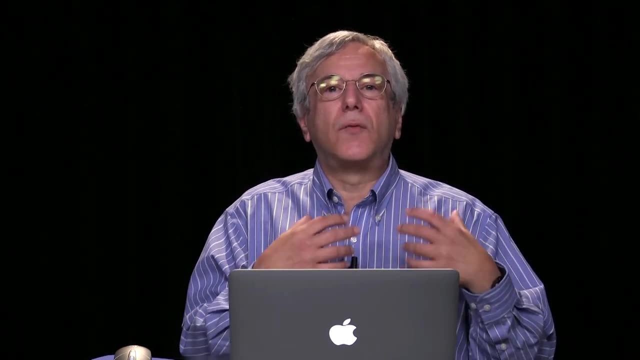 Oops, The second time that I run it it doesn't give me the wrong answer, It gives me the right answer. Oh, and now I have to run it several times until I can get the wrong answer again, so I can replicate the erroneous situation. 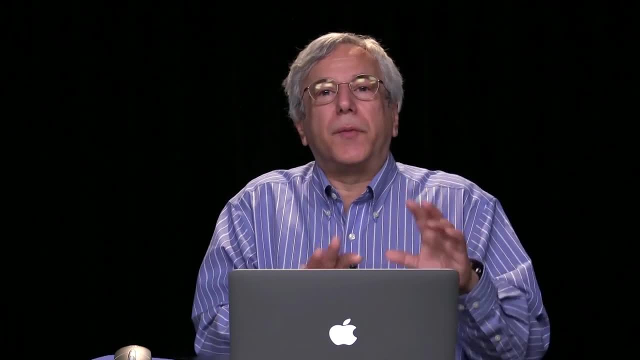 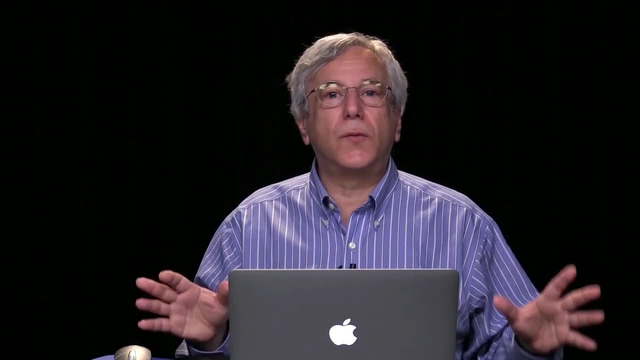 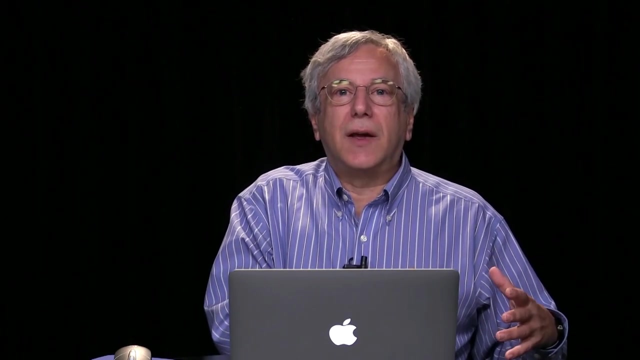 find out exactly what went wrong and fix it. Well, the problem there is that the function is using characteristics of the environment in which it's running to either come up with the right answer one time or come up with the wrong answer another time. 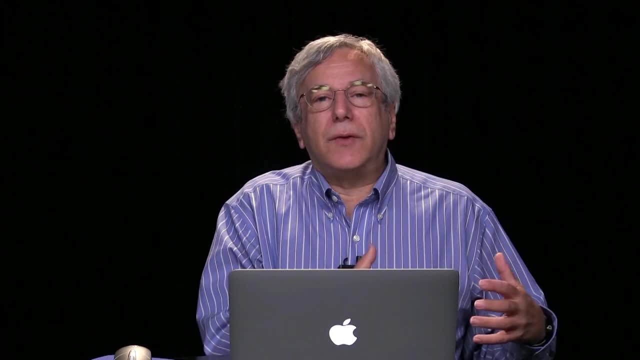 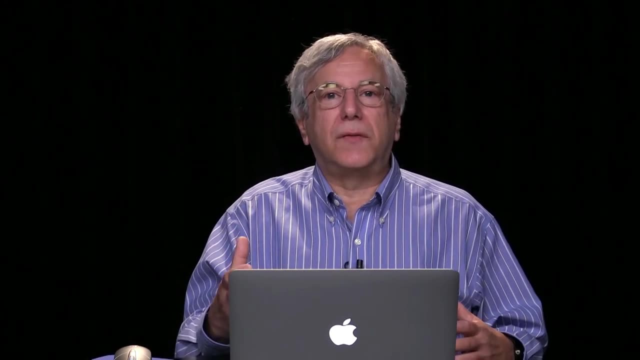 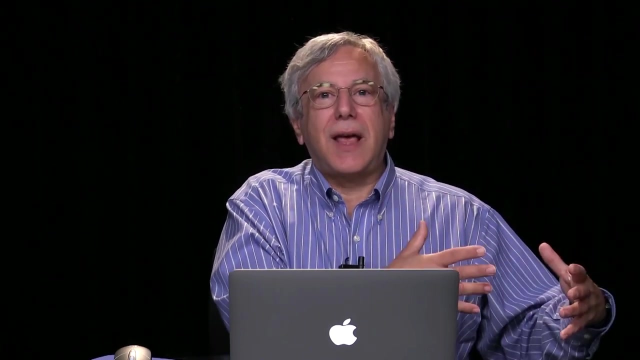 And that means it's difficult to debug because you have to sort of figure out what the environment has to be and try to replicate that external environment in order to make the function fail in front of you so that you can fix that failure problem. So debugging is more difficult when you 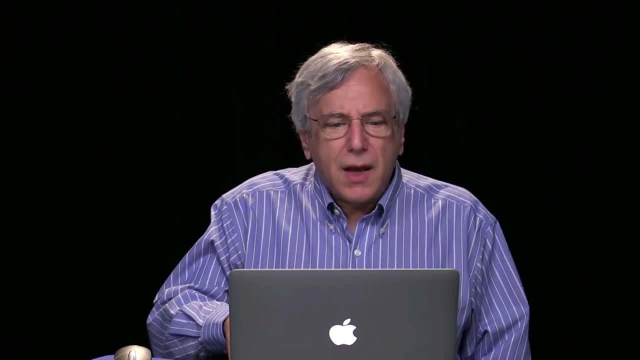 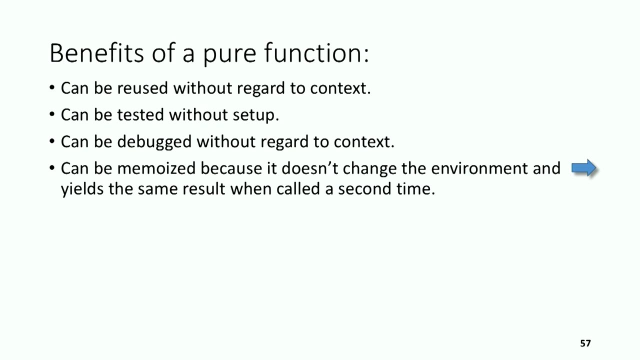 have a function that's not pure. Another important benefit of pure functions is memoization, And memoization that's a funny-looking word. You might look at the slide and think, oh, I should have written memorized there. No, memoization is the correct term. 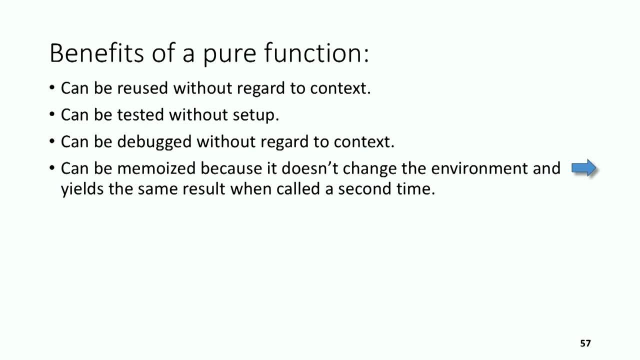 Memoizing just means keeping track of intermediate results while you get a value, so that you can possibly use those intermediate results later on in your code. OK, And only pure functions can be memoized. Let's have a look. The first example that I'm going to show you. 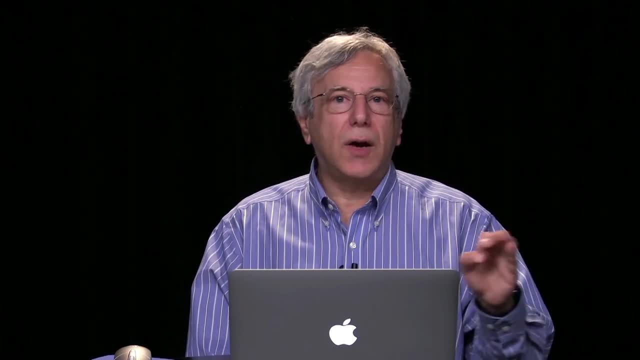 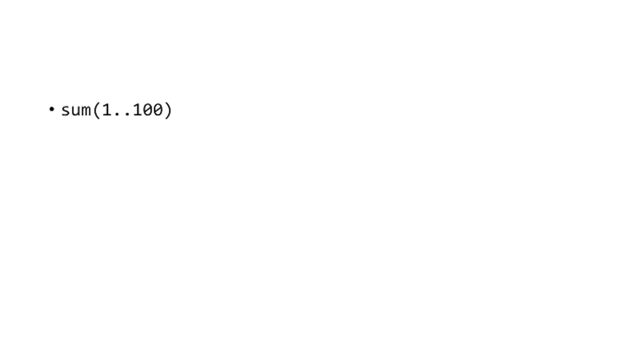 is one that's absolutely trivial And you might say, oh, why would you even bother memoizing with that? But it'll give you an idea of what I mean by memoization. Let's say that I'm trying to add together the numbers 1: 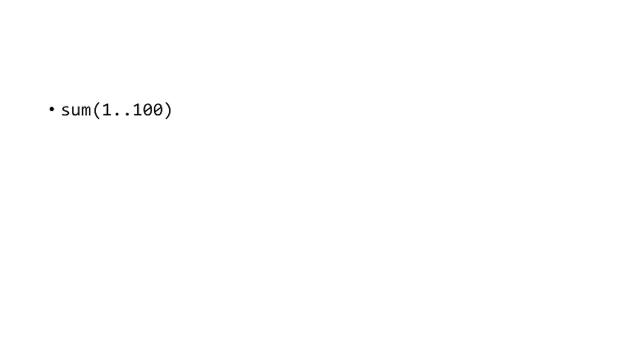 through 100. And you see there on my slide, my little notation. for that Doesn't matter what notation you use. Just imagine that you need to add those numbers together. By the way, I realize that there's a quick formula for this. 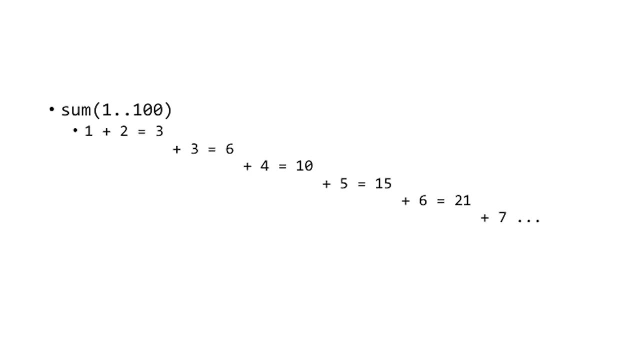 I'm going to ignore that for now and just say that we're doing this problem, solving the problem by saying 1 plus 2 is 3.. And then we're going to add 3 to the value 3 and get 6.. 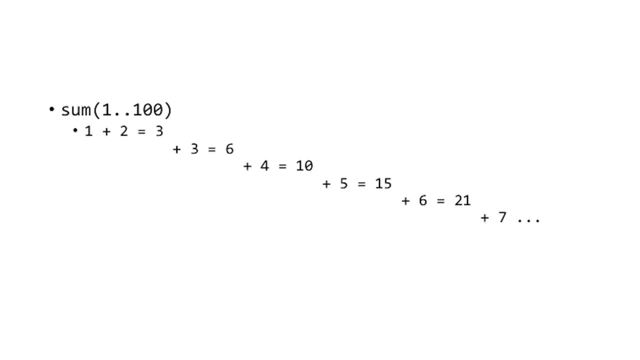 And then we're going to add 4 to the value 6 and get 10.. And then add 5, and so on and so forth, And we end up with the sum of 1 through 100.. Very, very nice. What if? 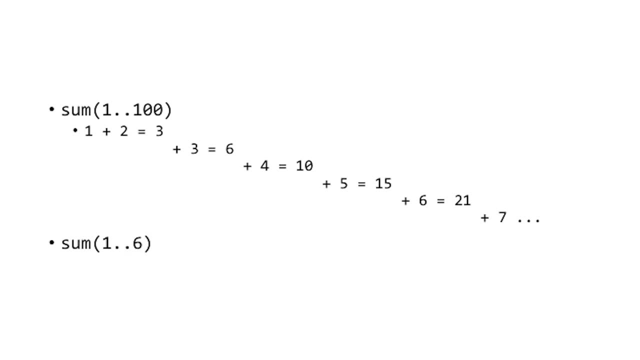 Later on in the code. In the code we need to find the sum of 1 through 6.. Well, I agree, in this trivial example it's very, very easy to find 1 through 6, the sum. But in a more complicated example, 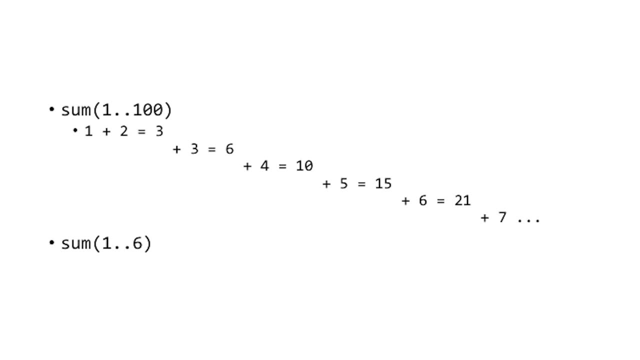 finding the sum of 1 through 6 or finding some other sum of 1 through 60-like things might be more difficult and more troublesome. So what happens now when I want to add together 1 plus 2 plus 3 plus 4?? 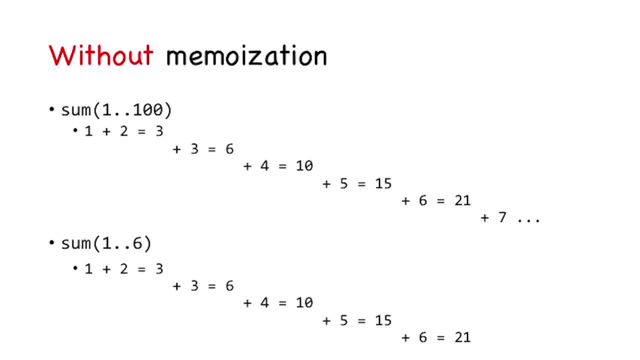 Plus 4 plus 5 plus 6? Do I duplicate the effort and start adding 2 to 1 and get 3?? Add 3 to 3 and get 6? Do I do all that work again? Really, if I use memoization I don't have to redo the work. 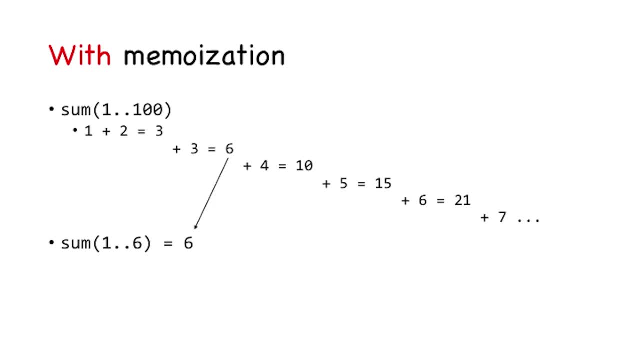 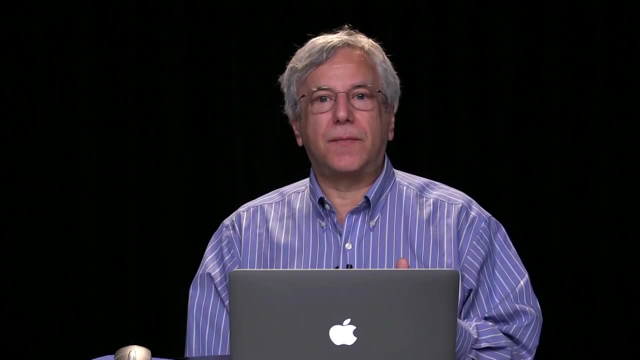 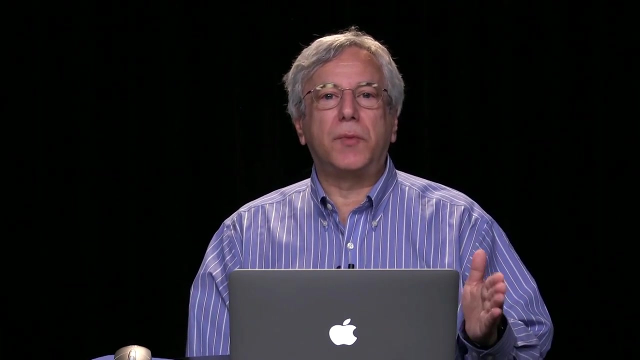 Because the idea with memoization is, as you're computing the value 1 through 100, you save the intermediate results. So Perhaps I have a table, an array, a lookup place where I saved the sum of 1 plus 2.. 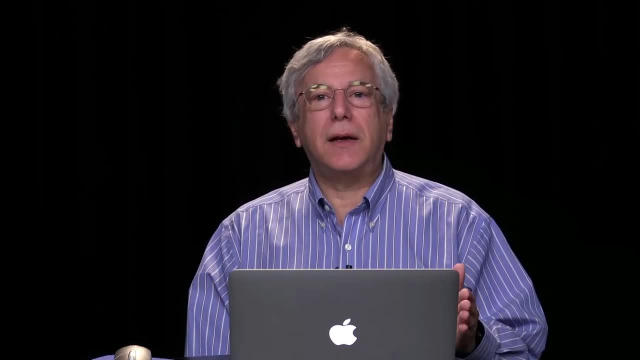 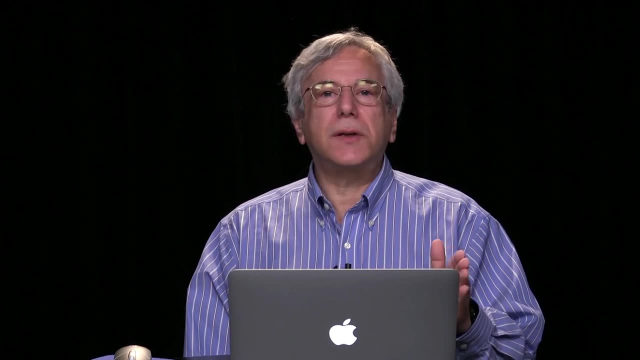 And then where I saved what happens when I add 3 to that, And then where I save what happens when I add 4 to 6. And saved all the intermediate results. So then, when it comes to summing up 1 through 6,, 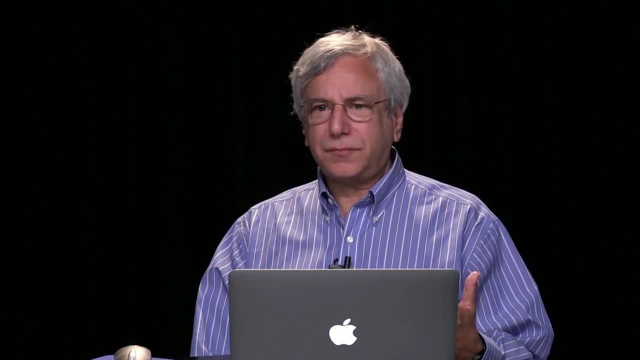 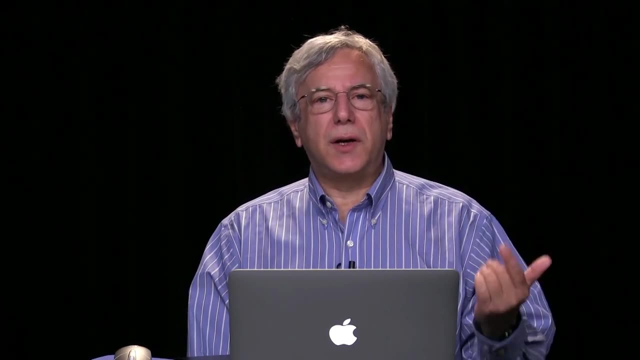 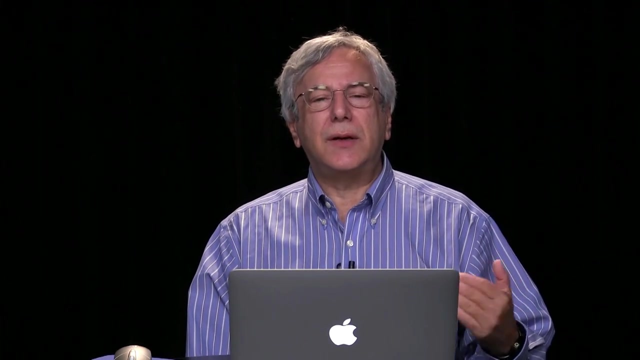 I can just look up that value in one step. OK, You may be saying to yourself, if I'm going to add together the numbers 1 through 100, or do some similar operation? add together the amounts of 100 purchases or the results of 100? 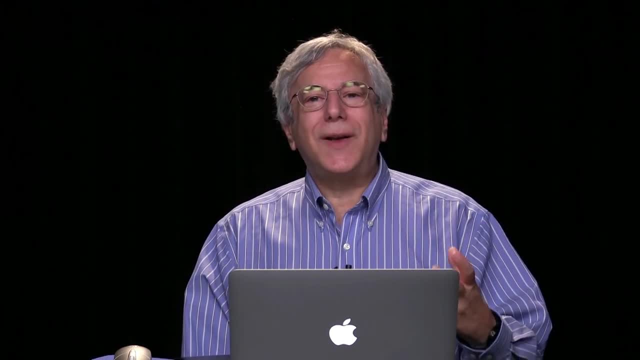 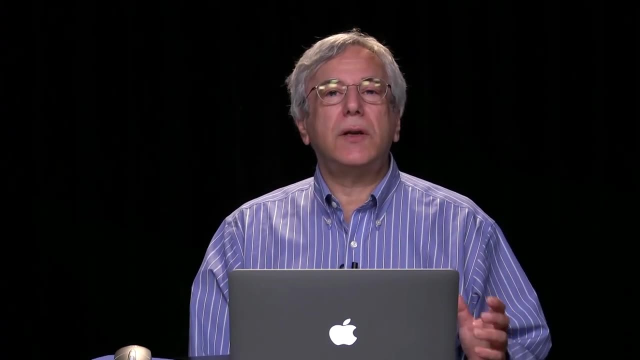 calculations. would I always want to save all the intermediate values? Well, of course, the answer is no. You don't always want to do that. You want to do memoization judiciously. You want to do it judiciously. 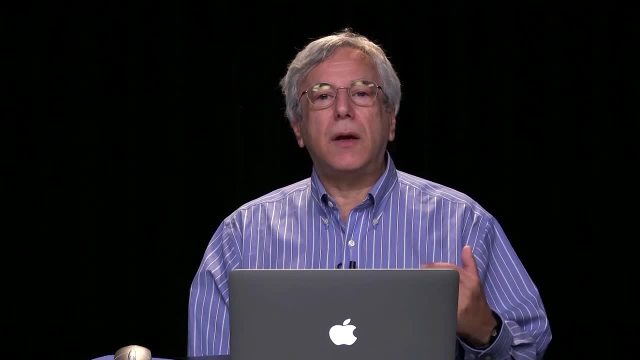 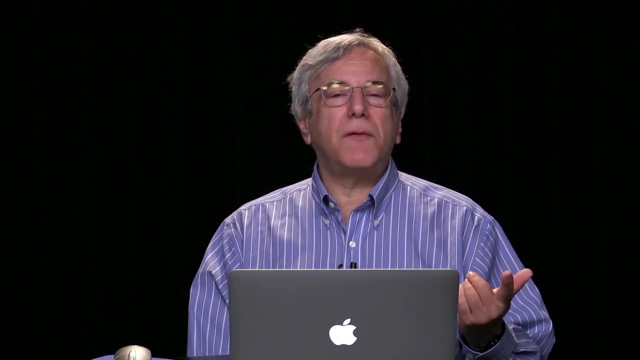 You want to do it memo-wise? OK, You want to do it only when you think that you will be needing those results for a later calculation And, if you can, you want to save only the parts of that calculation that you think you'll need later. 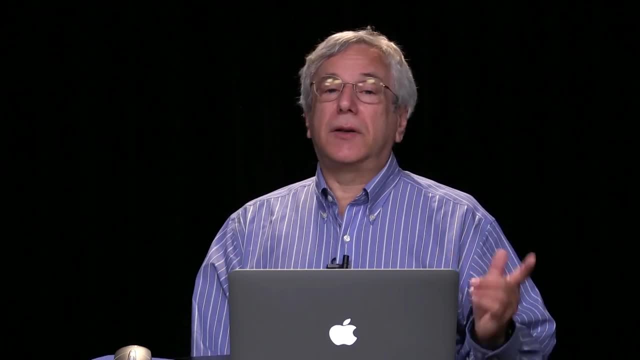 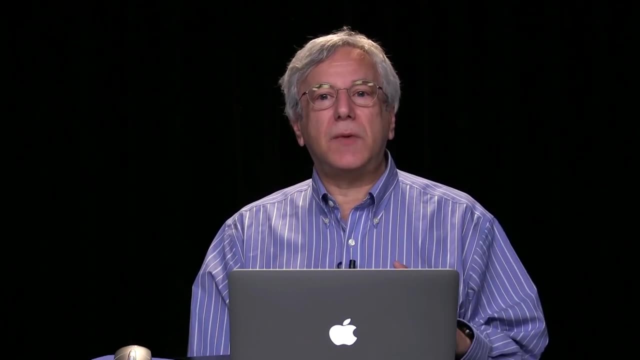 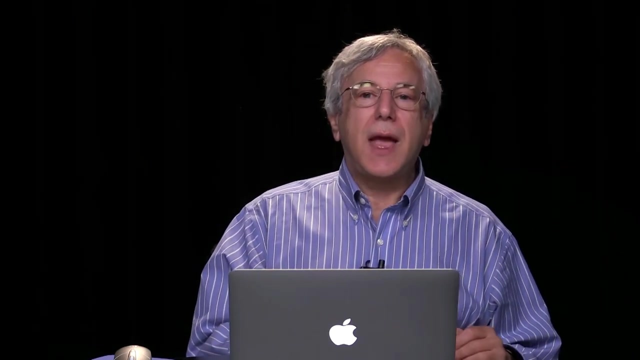 Are there situations where memoization is handy? Absolutely. Are there situations where memoization is not handy? Yes, of course, But memoization is a good technique and it's something that is really useful to be able to do in actually industrial strength situations. 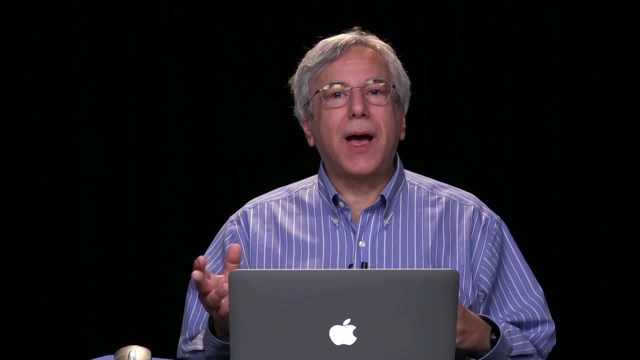 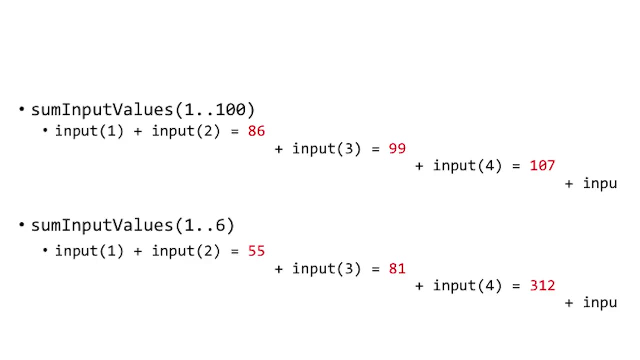 And in fact memoization is only possible when you have a pure function. If it turned out that calculating the sum of 1 through 6, or the sum of the first account, the first six purchase values or the sum of the first six. 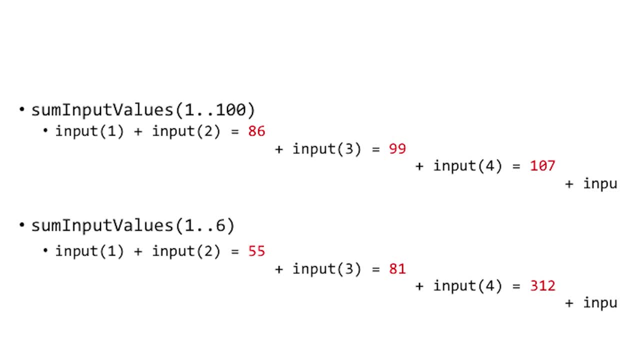 whatevers. if it turned out that calculating the sum of the first six things did not give me the same value each time I calculated it, because that sum involved values that were external to the summing function, then saving the sum of 1 through 6 as an intermediate result. 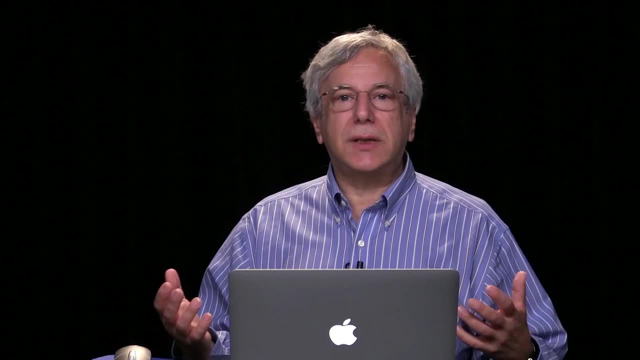 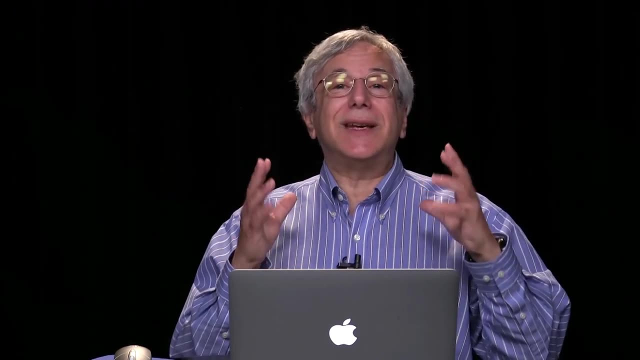 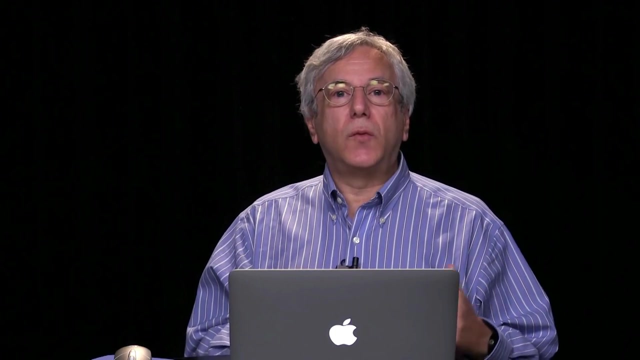 from calculating the sum of 1 to 100 would be useless. So memoization is useful only. memoization is possible only if I have a pure function, And in fact there are some functional languages where there's a keyword or a special feature that just says: 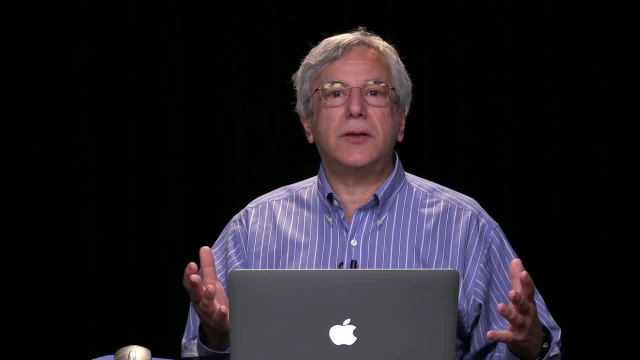 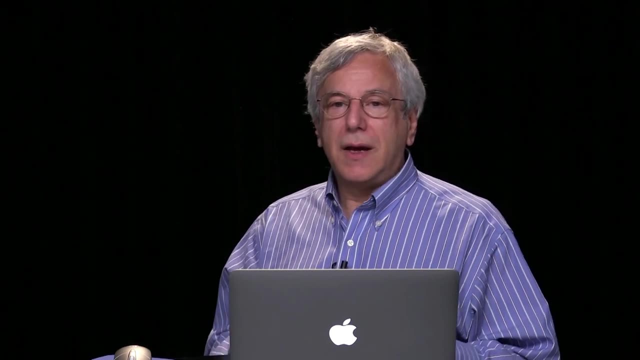 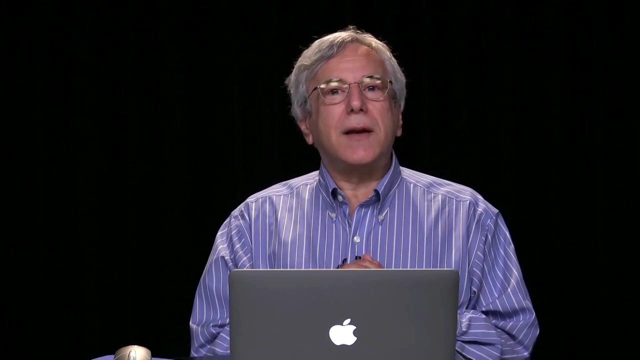 memoize, Do a certain calculation and as you go memoize, save the intermediate results automatically for later use. Since this sum of 1 to 100 problem is, I don't know, something that you might not imagine. wanting to put a lot of effort, 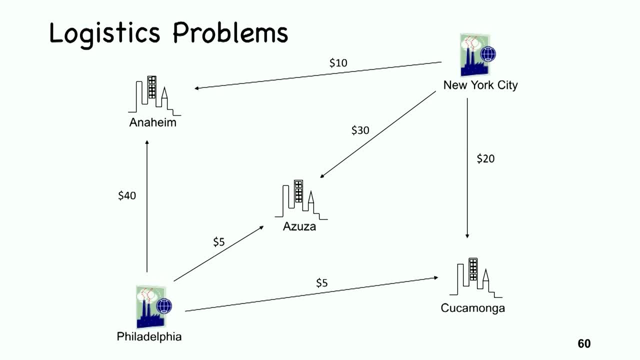 into in a lot of situations. I just want to talk about one situation in which memoization turns out to be really useful. Let's say that I have warehouses and I have places where I have to deliver goods. This is called a logistics problem. 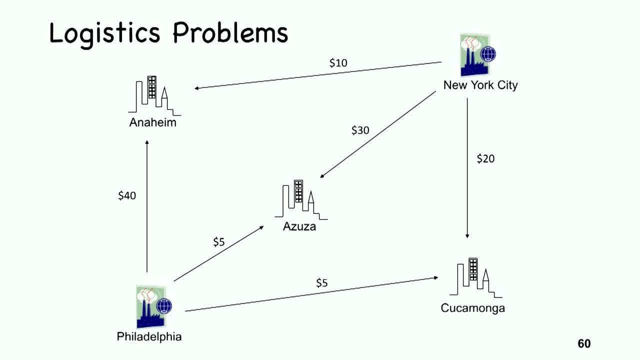 Logistics means you're moving things from one place to another. You're getting them where they should be. Logistics problems are of enormous practicality. This is real world stuff. So in this scenario, in this slide, I have two cities: I have New York City and I have Philadelphia. 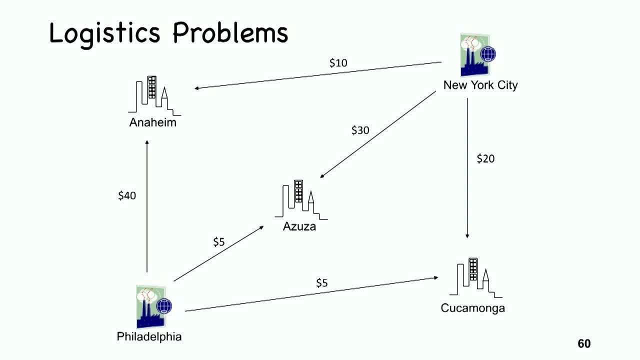 And I need to deliver from my warehouses in New York City and in Philadelphia. I need to deliver to my destination points in three cities in California- Anaheim, Azusa and Cucamonga- And I have various amounts that I know it will cost me to deliver from New York City to Anaheim. 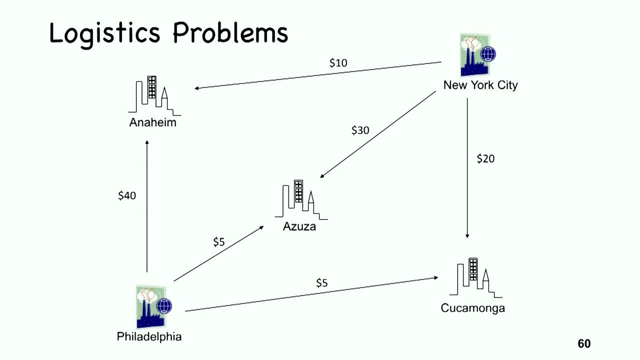 from New York City, From Philadelphia to Azusa, from Philadelphia to Azusa, from Philadelphia to Cucamonga, And so what I want to do is calculate what's the most judicious, the most cost effective way of moving goods from Philadelphia to Anaheim. 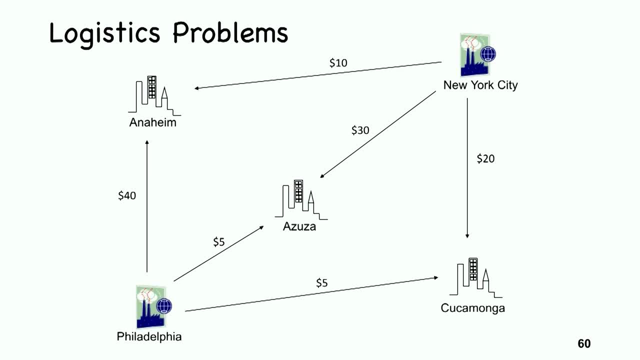 or from New York City to Anaheim. Where should I take these goods and send them from and to? So this is a logistics problem. It's just one way of framing the problem. There could be other constraints, But the idea is you can start playing around with this. 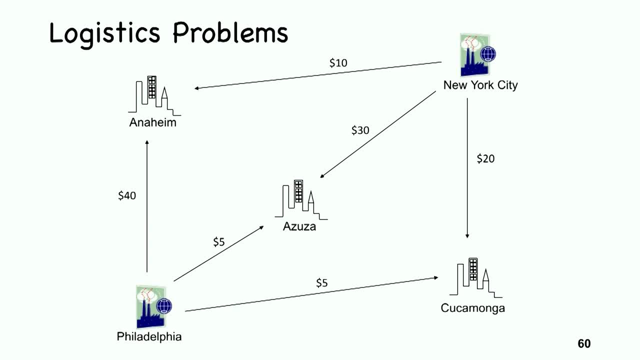 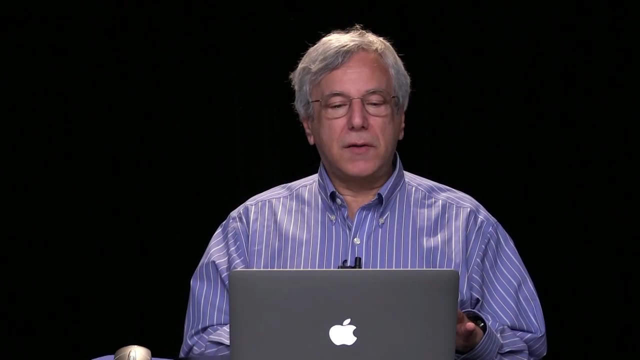 It turns out that if you refine the problem, it's not always the best thing to do to simply send things by the cheapest route possible. Sending things by the cheapest route possible would be what's called a greedy method. Nothing bad about the word greedy here. 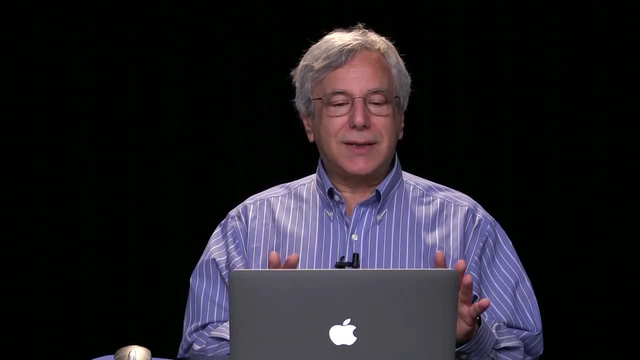 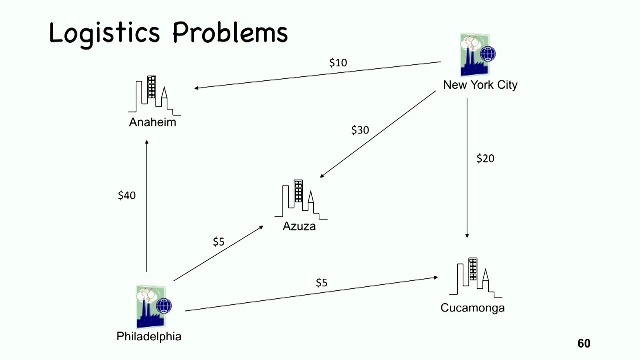 Sometimes greedy methods for solving problems work, But in this case you can kind of go wrong. You can end up taking the The cheapest way of sending things to Azusa and end up then having to use a more expensive way and losing your money by then having to send things. 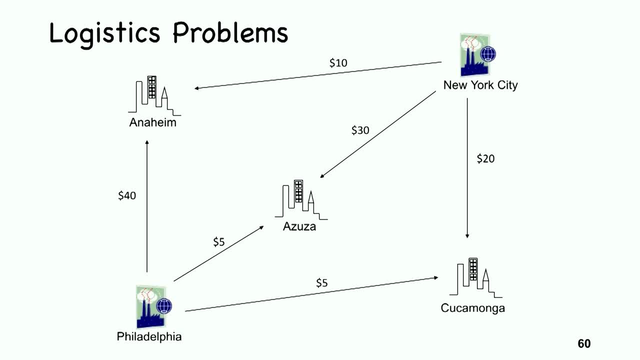 to Anaheim more expensively. Anyway, point is that, in order to solve a logistics problem of this type, what you often end up doing is trying all possible ways of sending goods from Philadelphia to Anaheim, from Philadelphia to Azusa, from Philadelphia to Cucamonga, from New York City. 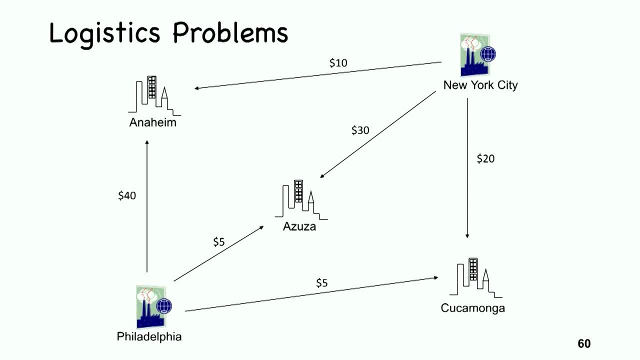 to Anaheim, from New York City to Azusa, and so on and so forth. You try all possible combinations of those deliveries to see which one gives you the best result. Well, as you're in the middle of making a trial, let's say that I haven't delivered anything yet. 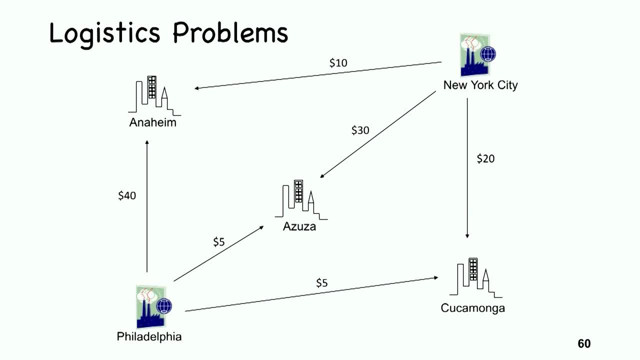 and I decide: hmm, what happens if I send three widgets from Philadelphia to Cucamonga? Just start with that, not send them to Azusa? Azusa has to wait for its deliveries. Anaheim has to wait for its deliveries. Let's just start off by sending three widgets from Philadelphia. 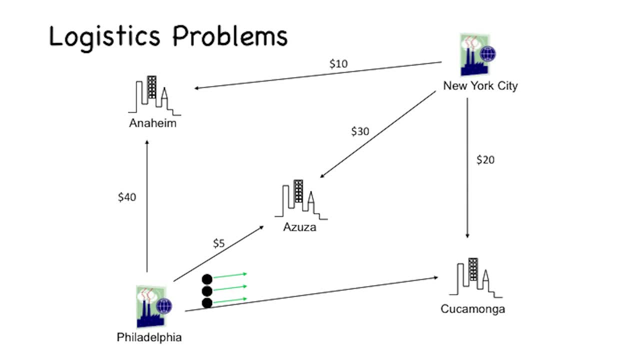 to Cucamonga. What happens? What does that mean? What that means is that I'm going to spend $15, right, Because on this graph you see it costs $5 per widget, So it's a $15 cost to start with those three widgets going. 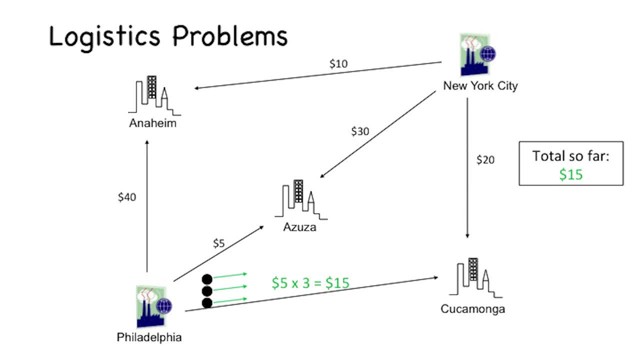 from Philadelphia. Well, maybe I should save that intermediate result so that I can use that later when I start playing with the other possible ways to send widgets from, say, New York City to Azusa, versus sending those widgets from New York City to Anaheim. 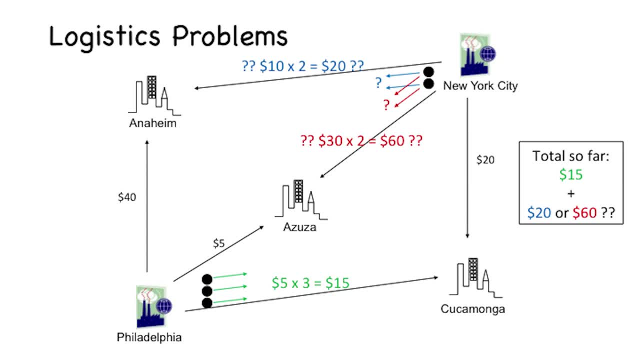 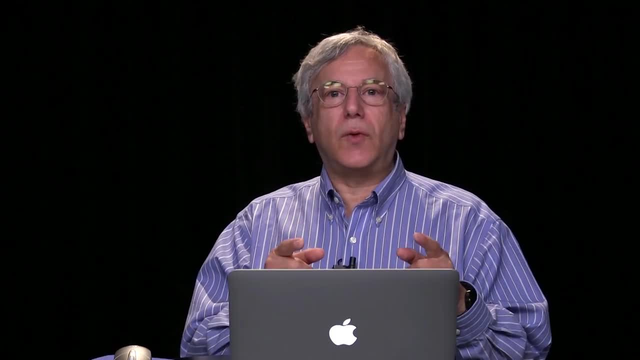 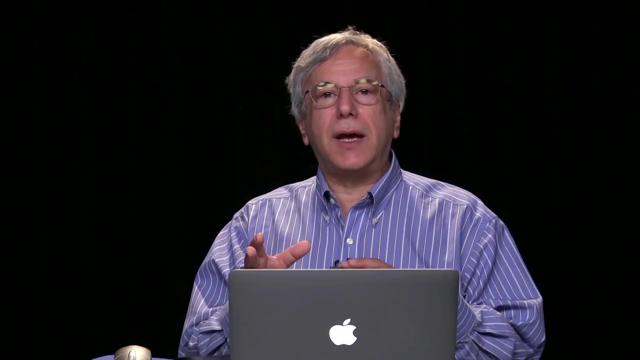 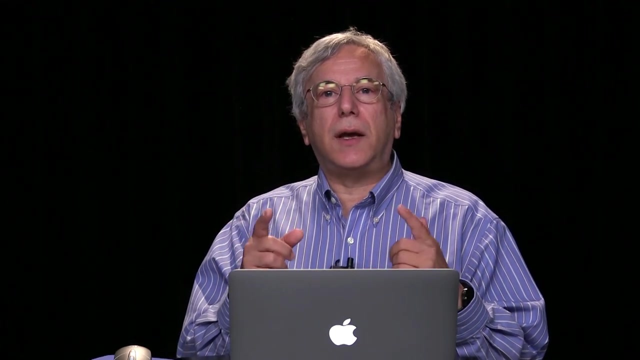 So the deal here is that Logistics problems in particular this kind of logistics problem means trying different scenarios, different ways of sending things from one place to another And, in the process of doing those trials, finding some sort of intermediate results that may help you in doing some trial and error later. 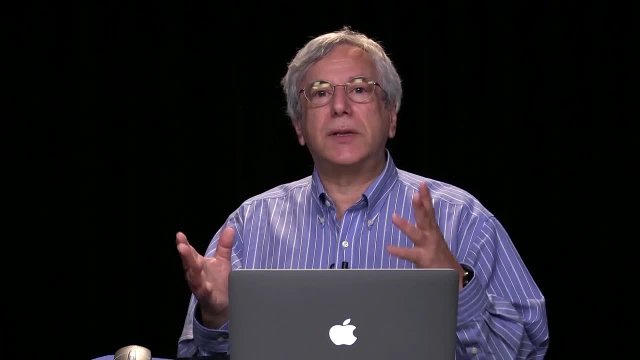 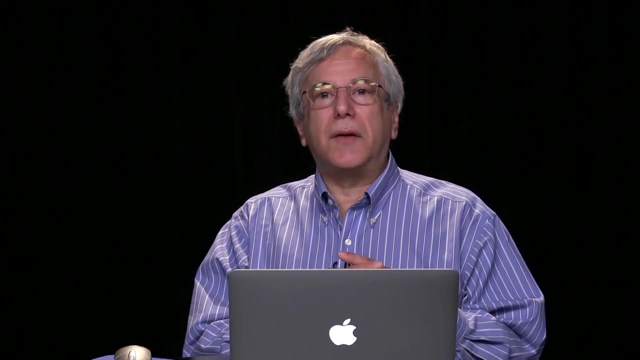 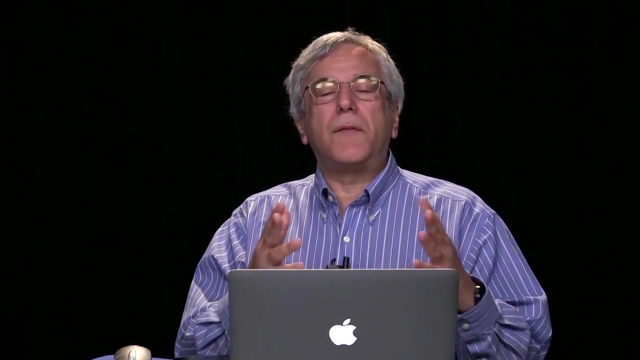 on in the problem: Aha, Saving intermediate results, Memoization. What do we need for memoization? We need pure functions, Really good stuff. OK, Memoization and the benefits of testing and debugging are one of the reasons why we like pure functions. 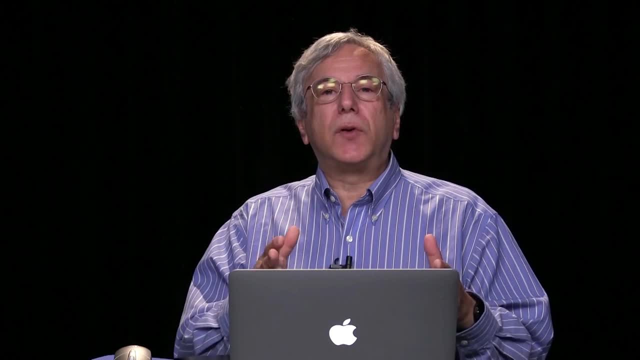 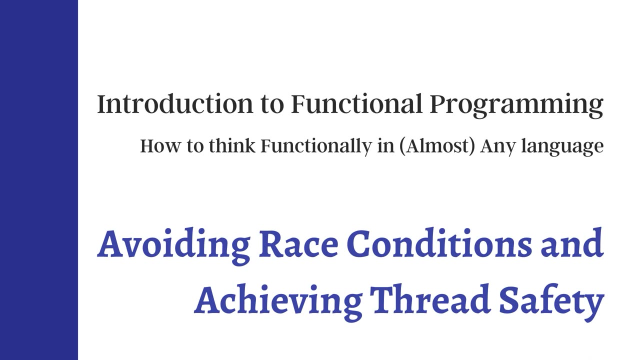 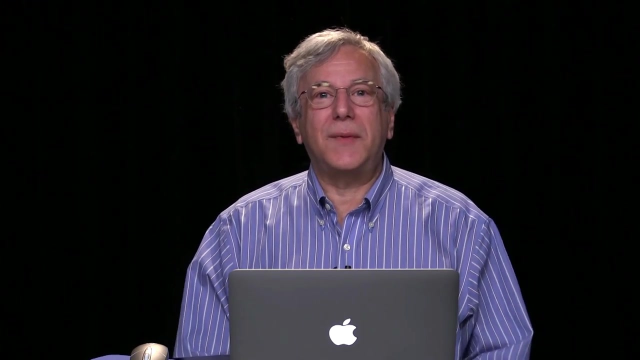 There are other reasons why we like pure functions, And we'll be exploring those in the next several segments. In the previous segments I was talking about pure functions and the benefits of pure functions, And now, because of that, I'm all excited about how. 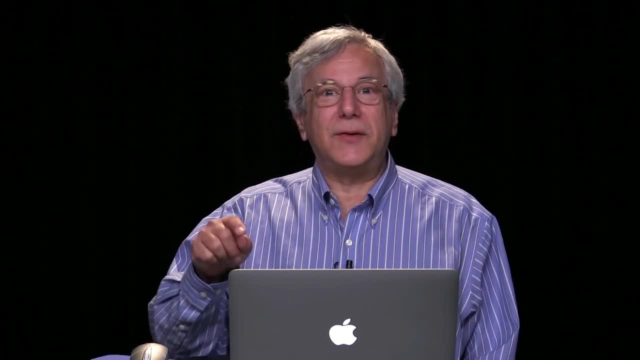 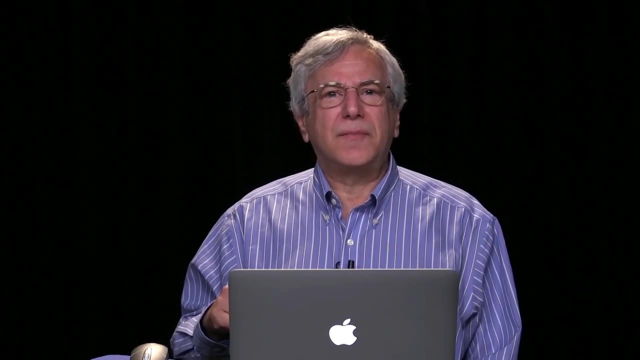 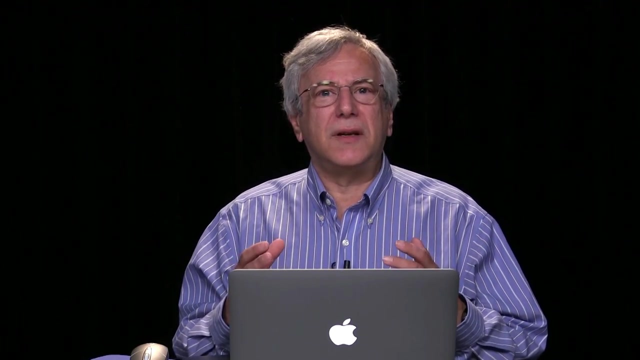 great pure functions are, And for that reason I'm going to tell you about another benefit of pure functions: Thread safety. OK, Thread safety. I'm going to use the word thread in a very general sort of way. A thread of execution is one line of do this, then do that. 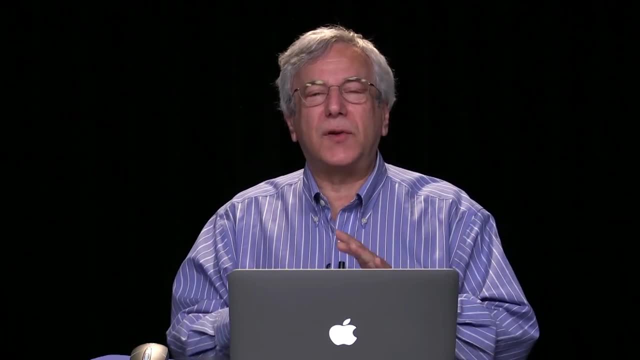 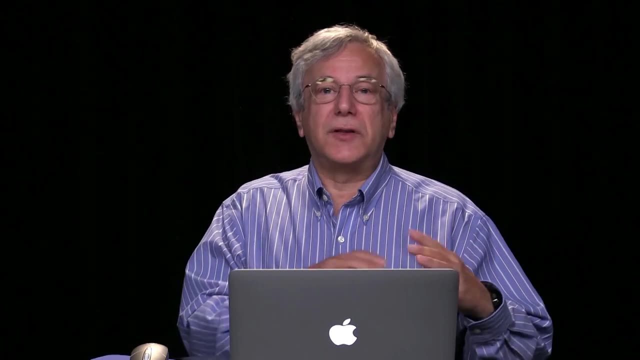 then do something else. Now I know I know we're talking about functional programming, So we don't like it And we say: do this, then do that, then do something else. We like to think of applying functions results to other functions. 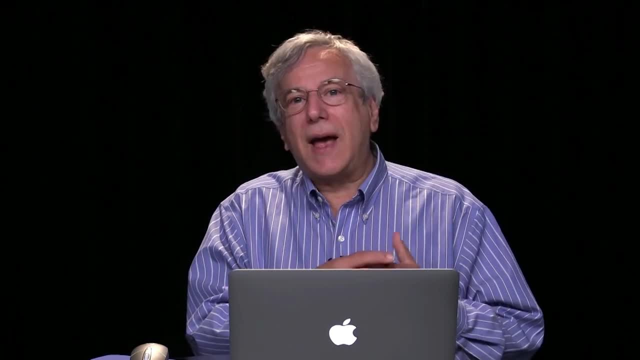 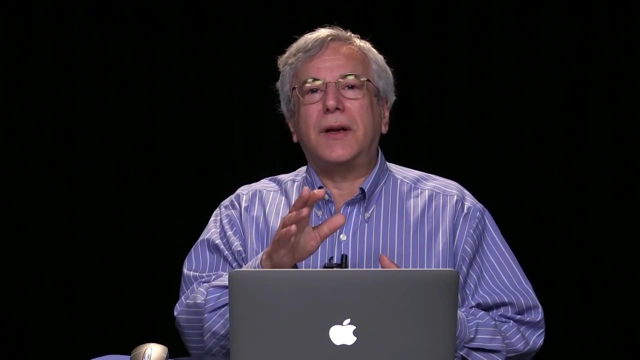 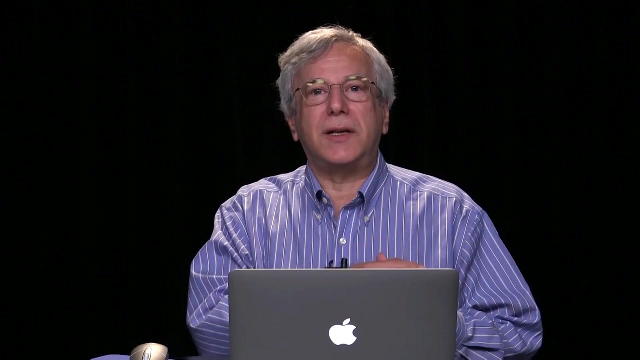 But really, inside of a processor you do have a do this, then do that, then do something else- architecture. Just one note: the reason that you have that going on inside of a processor is because what's called von Neumann architecture. 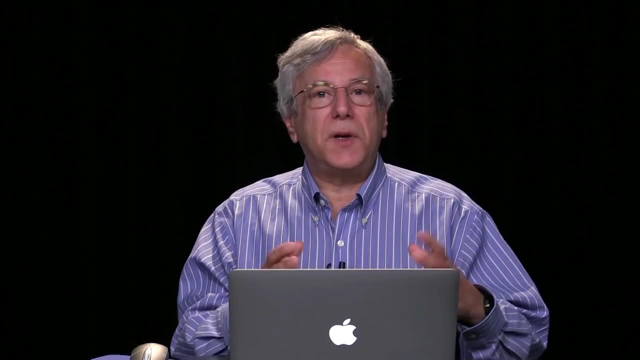 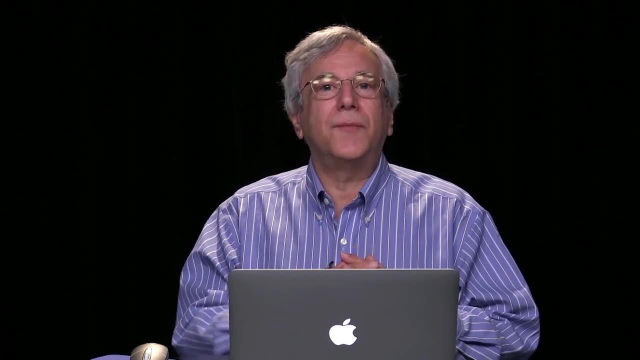 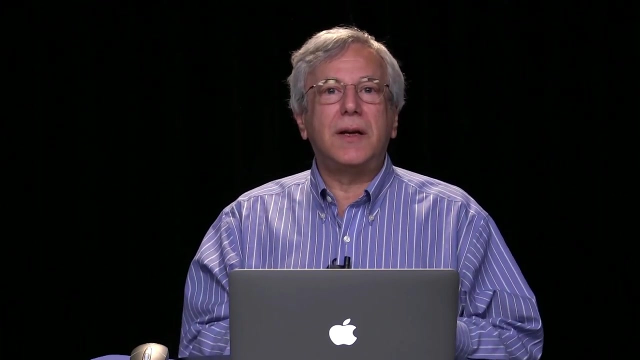 And von Neumann architecture is the way computers are typically built these days, But there are other experimental types of computers that don't use that kind of processing. OK, anyway, let's assume that inside of our computer, our computer is a von Neumann machine. 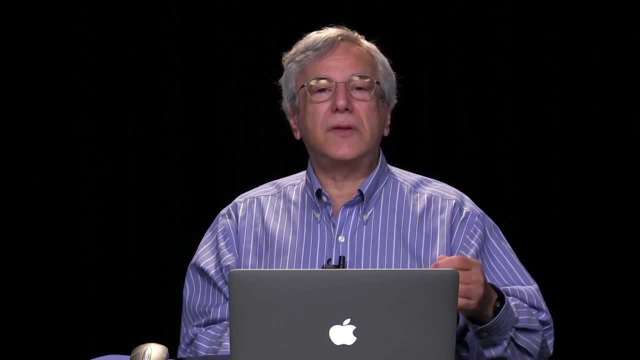 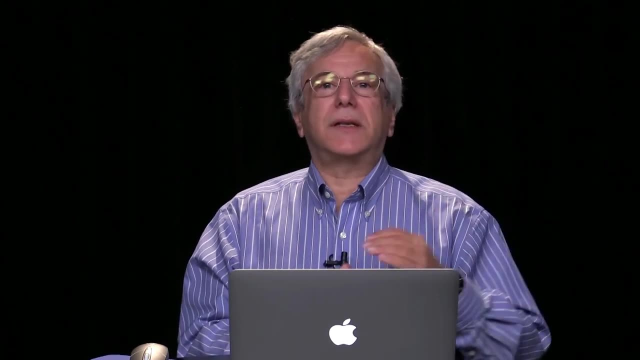 and that it does a do this, then do that, then do something else, Maybe branch. if this, then that, and so on and so forth, That line of execution that's called a thread of execution, And you can have several threads. 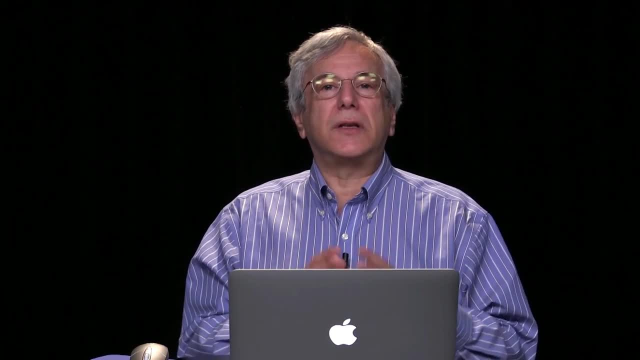 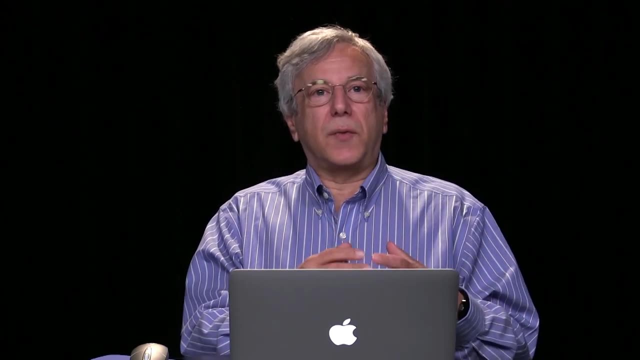 And you can have multiple threads at once in the execution of the solution of a problem. You can take part of the problem and assign it to one core, And you can take another part of the problem and assign it to another core and have those two cores. 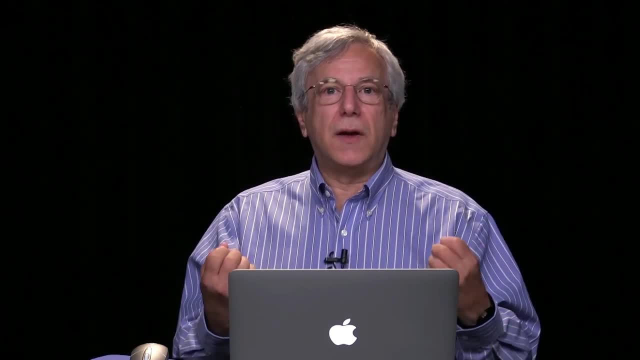 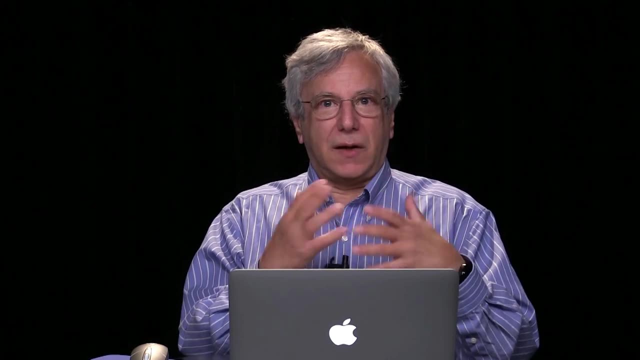 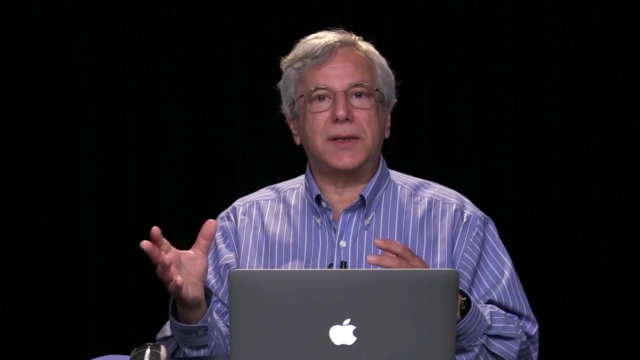 running at once And I'm going to call those two separate threads of execution. Now the word thread has a technical meaning. inside of a program That's a program. It's a little bit more specific than just saying assign it to one core and assign it to another. 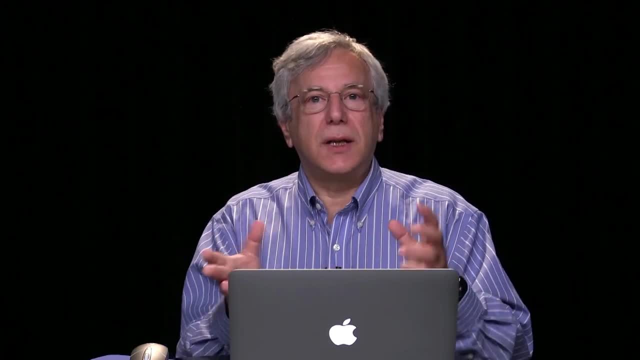 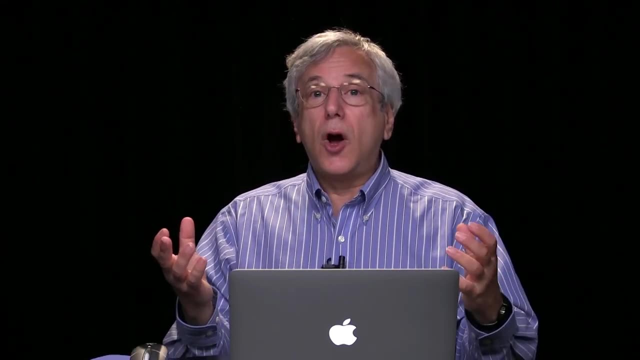 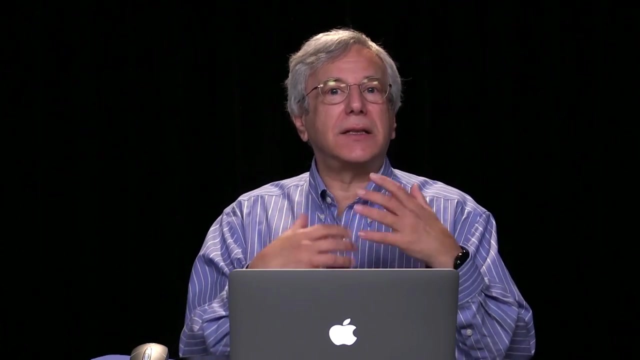 So I'm going to use the word thread most liberally and say you could be assigning it to one core and then assigning another thread to another core, Or you can have one core that is simultaneously interleaving the execution of two threads, Or I'm going to even say that you have two threads. 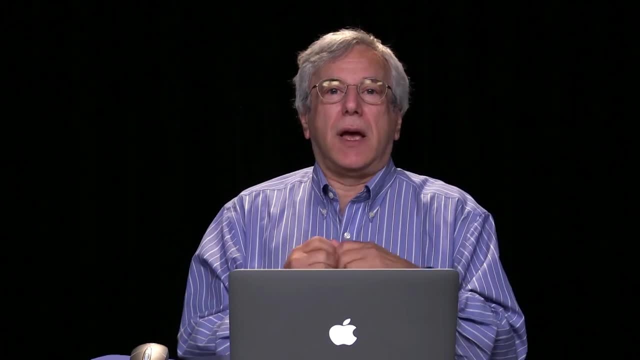 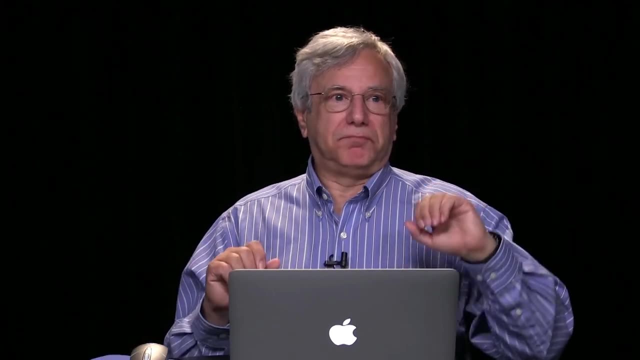 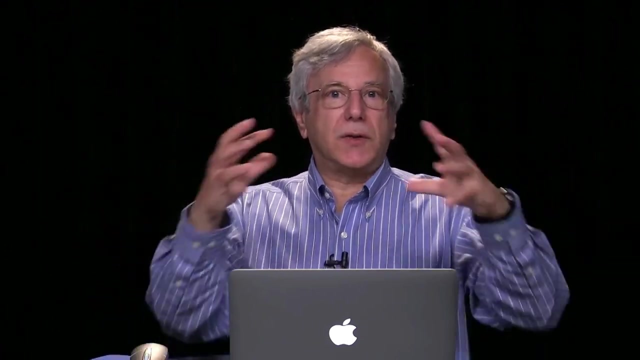 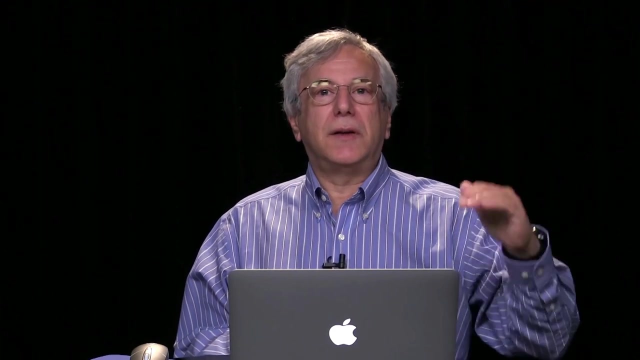 When you have two separate computers to which you've assigned different parts of one problem, and those two separate computers are both running at the same time, both solving parts of a problem, and then those two parts will be put together at the end. So a thread of execution is any step-by-step solving. 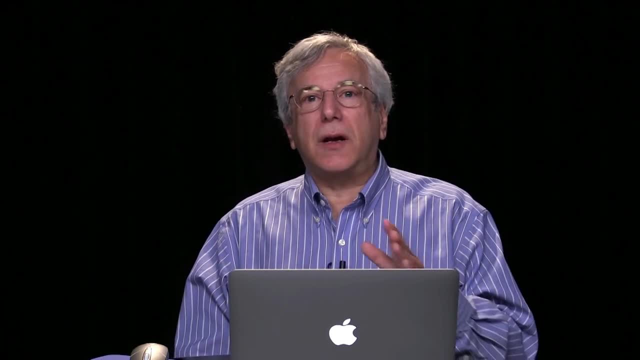 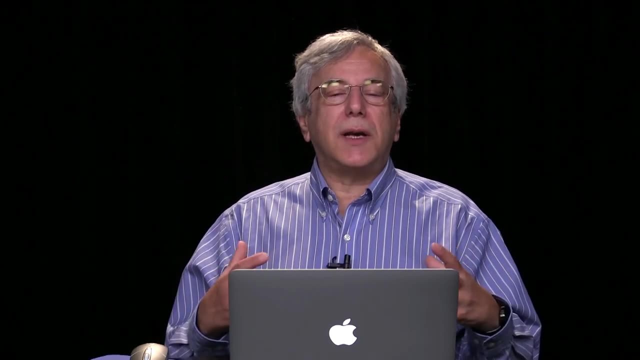 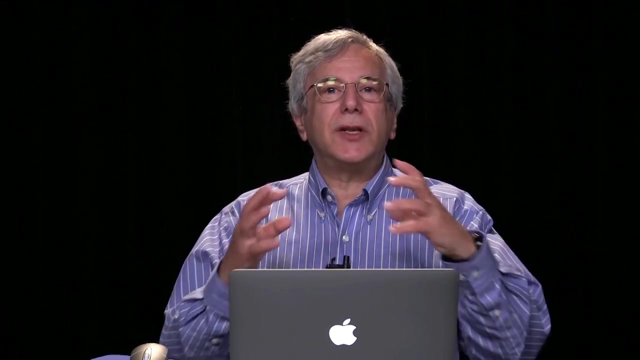 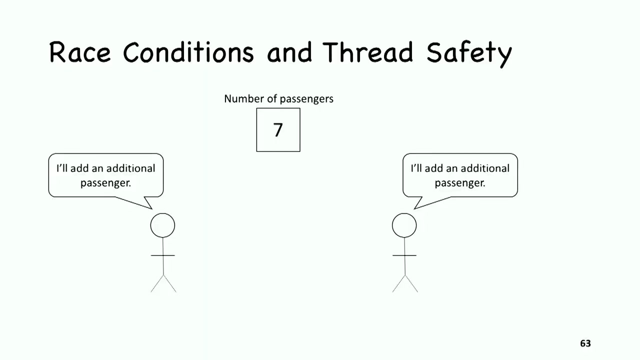 part of a problem. We can even imagine two threads of execution if we have two people on different sides of the world working on some sort of a system that has some line of communication where they're both able to make changes to a particular variable. Let's take a look at a situation like that. I have a count of the number. 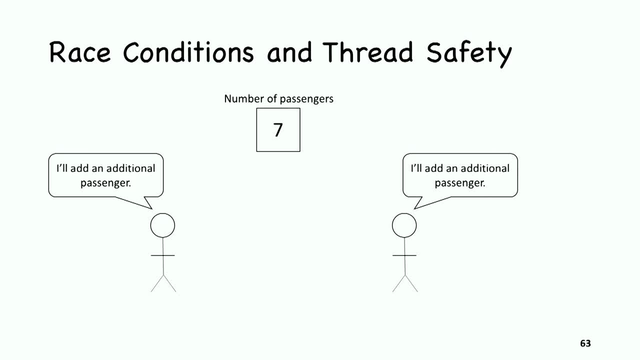 of passengers on an airplane And at this point the airplane is hardly booked. The number of passengers on the plane is seven And I have two separate threads of execution in that I have two separate people on different parts of the sides of the world saying: I will add an additional. 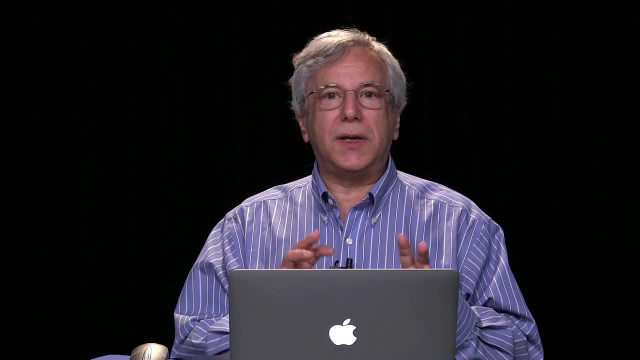 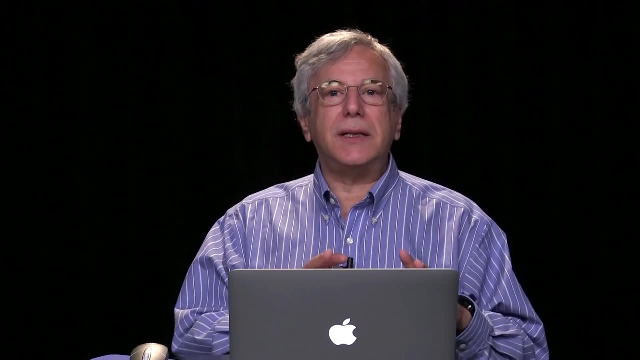 passenger. Now this situation. this is a little bit fake because this isn't going to be the way that real airline reservation systems work, But it'll give you the idea of the kinds of things that can go wrong when you don't have thread safety. 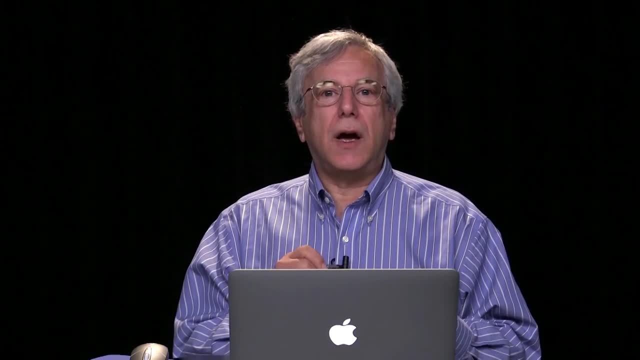 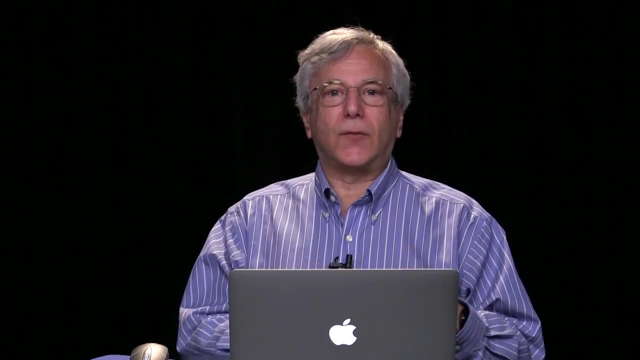 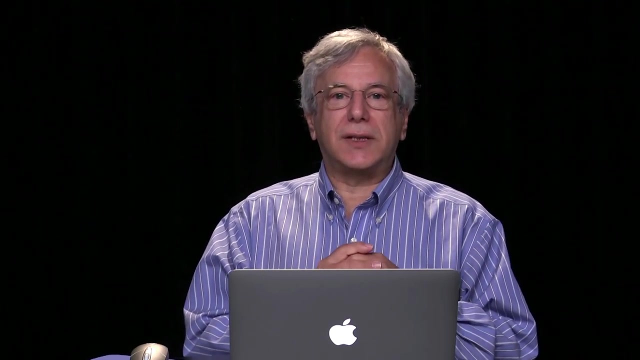 When you don't have thread safety, you're in danger of having a race condition occur. OK, So that means that in this title on the slide, the word race conditions, race conditions, is something bad, Thread safety is something good. It's a heterogeneous title for a slide. 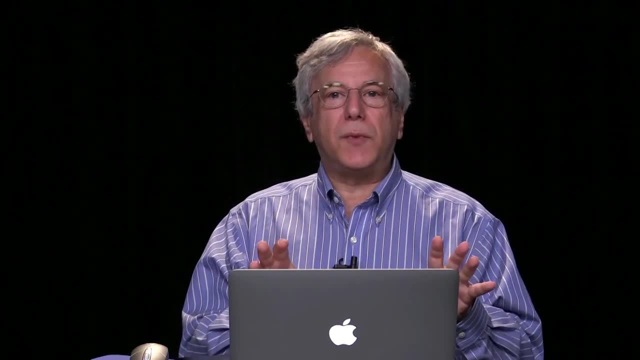 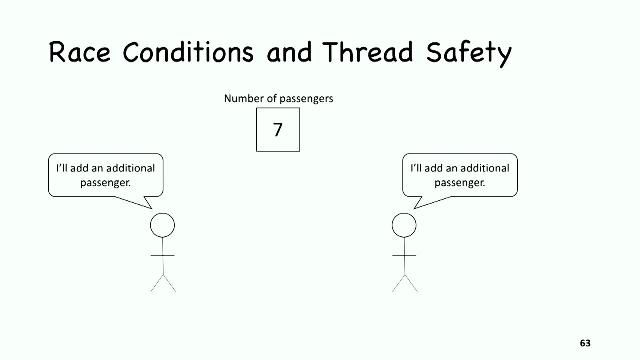 All right: Two separate threads of execution, two separate people in separate parts of the world, modifying one variable, And they're both working independently. They're not talking to one another, another and saying: well, now it's your time to execute a statement, and now it's my turn to. 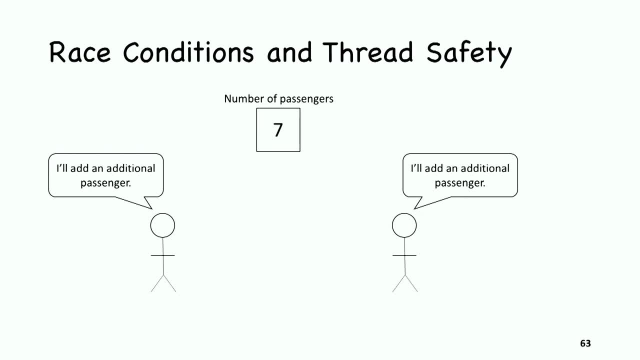 execute a statement. They're both doing their things in different sides of the world. So the person on the left says: I'll add an additional passenger, and the person on the right says: I'll add an additional passenger. Okay, what happens? Well, in order to add an additional. 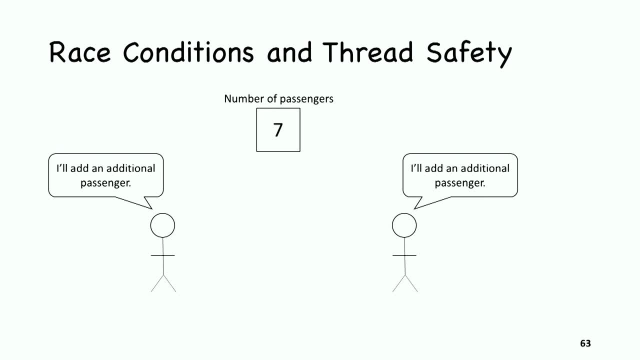 passenger. let's hypothesize that the person on the right grabs the number seven and says: I'm going to add one to it. Well, maybe, as that person on the what did I say? right or left. Let's start with the person on the left. The person on the left grabs that number seven and says: 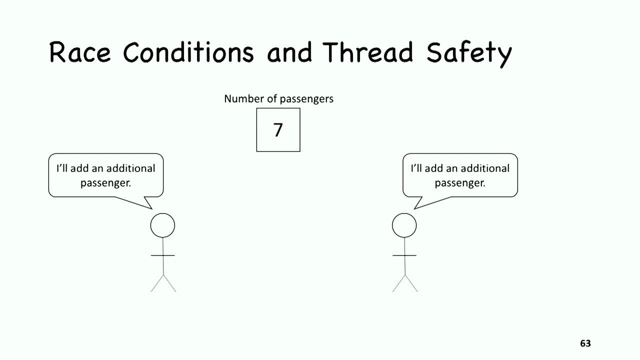 I'm going to add one to it. And at the very same time, on the other side of the world, the other person says: the person on the right says I'm going to grab that number seven and add one to it. So now, simultaneously, 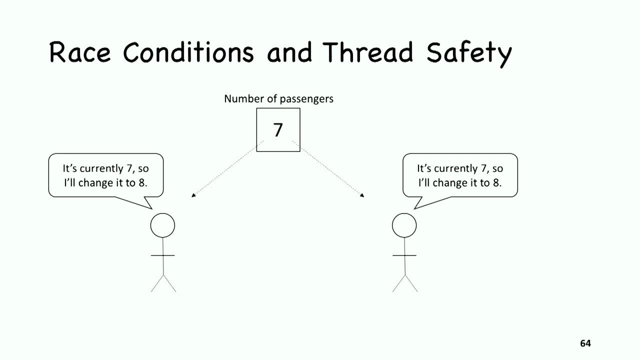 you've got two people, two agents, two different servers, two different processors, two different computers, two different cores within the same machine, saying I'm going to grab the number seven and I'm going to add one to it. Well, of course, since there are two, 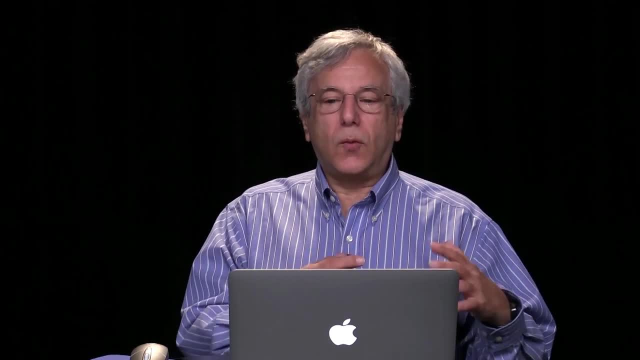 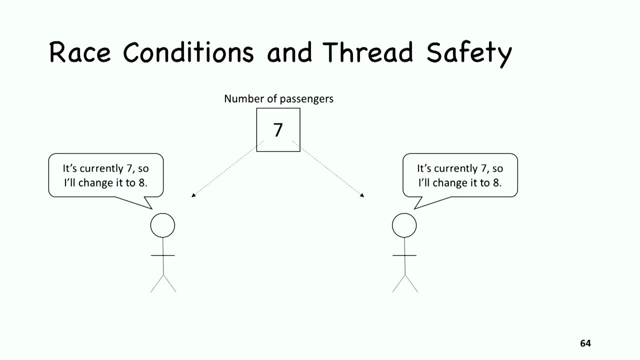 different threads, both trying to add one to the number seven, the result should be nine. However, if the person on the left side says, ah, it's currently seven, I'm going to change it to eight and put it into that memory location. And if the person on the right says exactly the same thing, 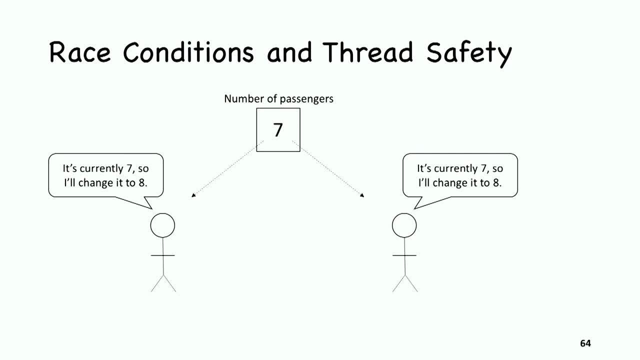 it's currently seven, so I'll change it to eight. Then in the next step, they both take the number eight and deposit it into the number of passengers. slot Whoops: Two new passengers and the count has changed from seven to eight. That's a lack of thread safety. We have two separate. 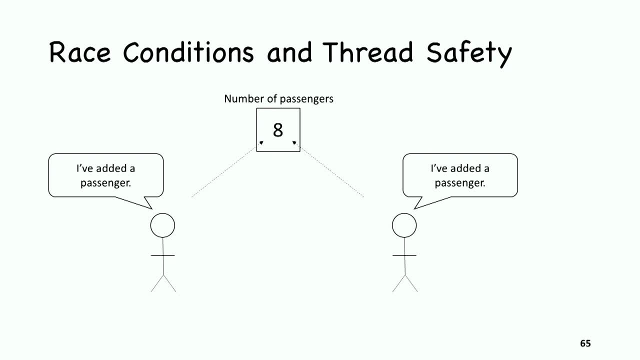 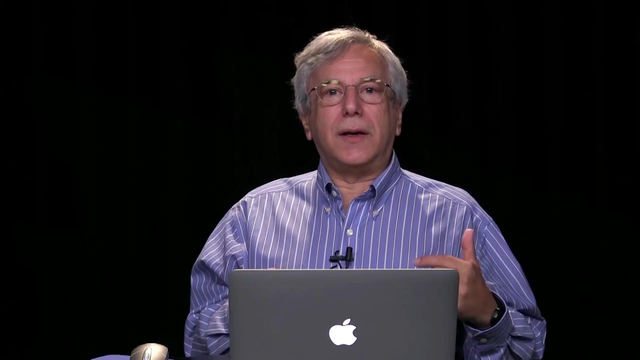 threads and we no longer have the safety of knowing that the value that they get when they update the number of passengers is correct, And when this kind of thing happens, it's called a race condition. Now, what's going wrong here? What's going wrong is that there is a variable number of passengers. 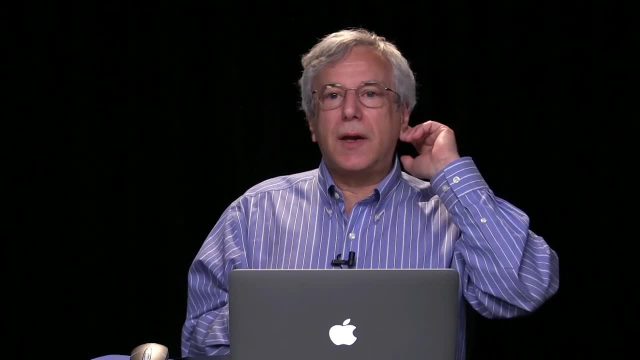 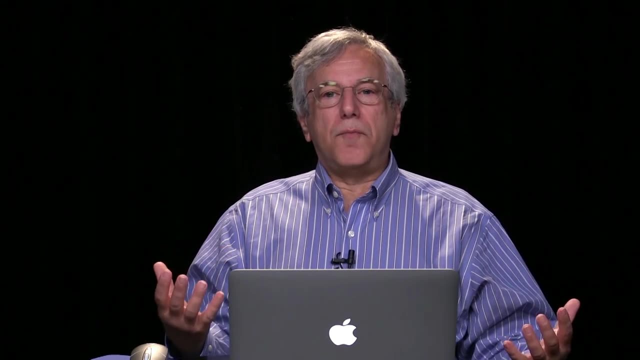 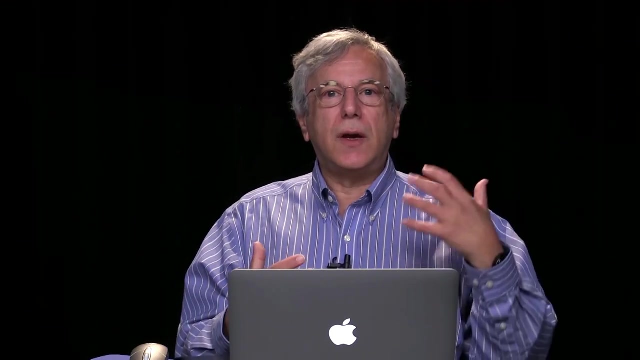 that's immutable- Whoops, we don't like mutability. And also, what's happening is that these two separate threads are making changes to that variable and that variable is external to each of them. It's external to both the agent on the left and the agent on the right. So we've got a situation where 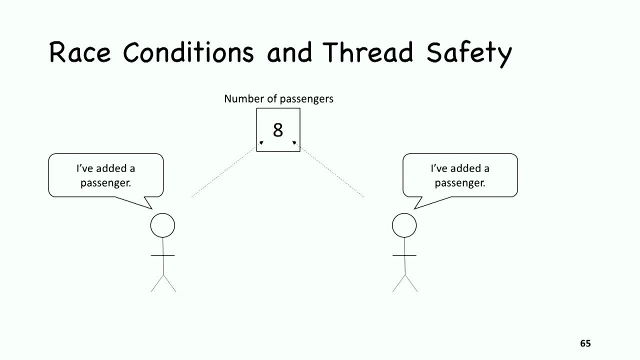 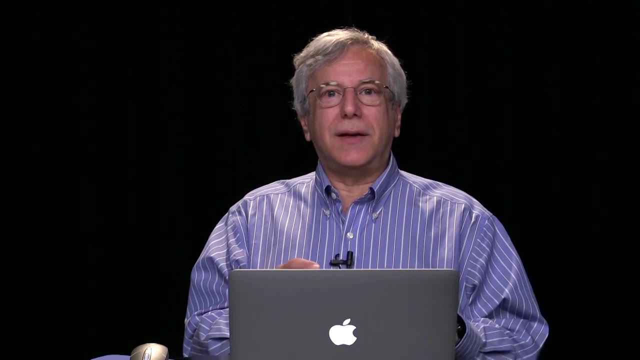 the lack of purity, the lack of immutability, the presence of side effects is a feeding ground for problems, for race conditions. Okay, look, I'm going to admit it In real life, you do have an airplane. You have one of them. You may have several agents. You have 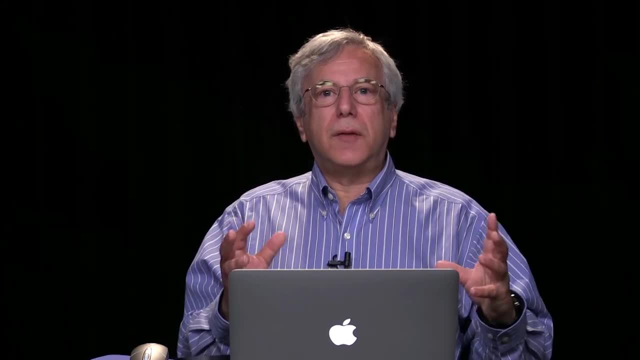 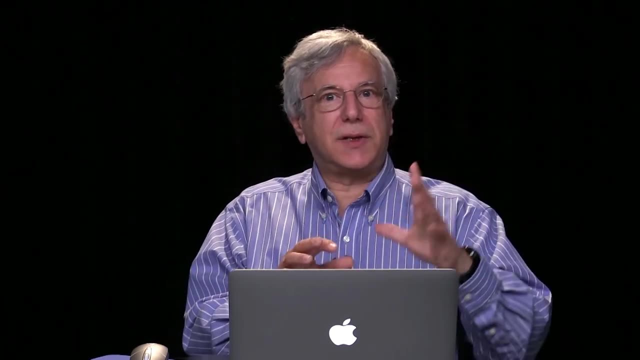 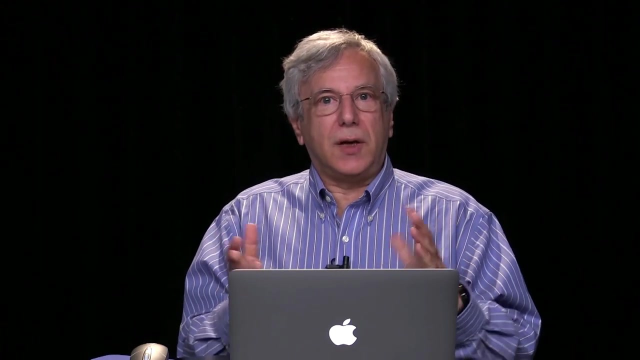 lots of different agents that somehow have to modify the configuration of seats on the airplane. Put somebody in this seat, put somebody in that seat. up the number of passengers. There has to be a mutable variable in this situation, because you have to change the number of passengers, You have to 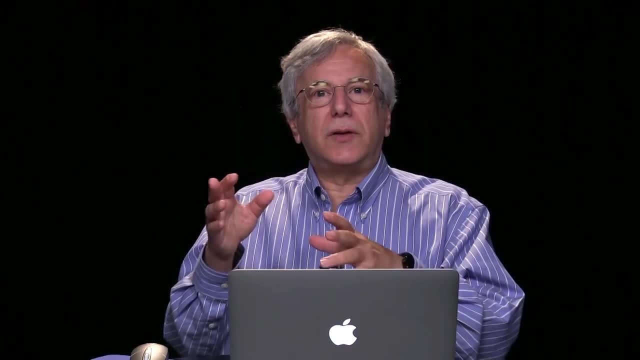 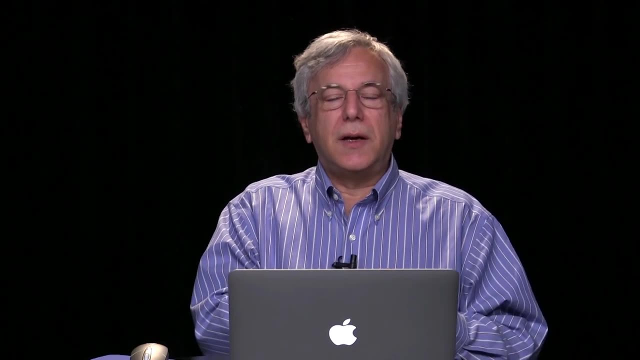 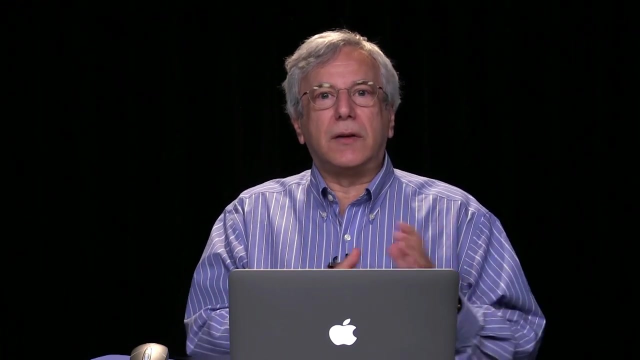 make a seat be from unoccupied to occupied. Or if somebody cancels a reservation, you have to make it be from occupied to unoccupied. The equivalent in this sort of a scenario would be: maybe you'd have a race condition and you'd be accidentally putting two people in the same seat. Well, hopefully one of 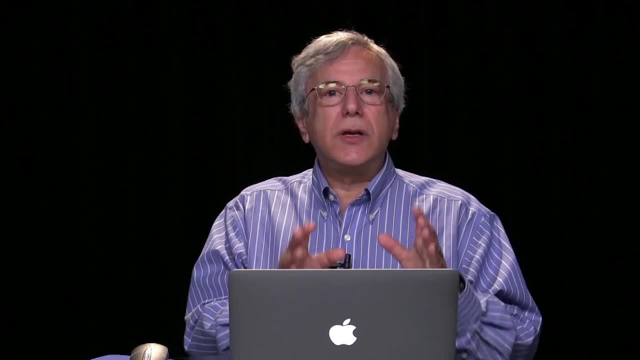 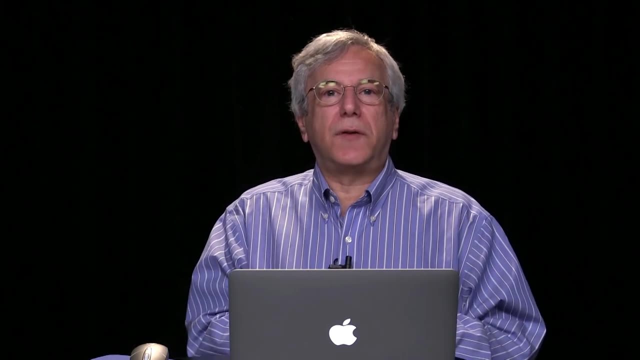 them could sit on the other's lap. In real life we do have things that are mutable. The idea of functional programming is not to wipe this situation off the map and to make it so that we can't make airline reservations. The idea of functional 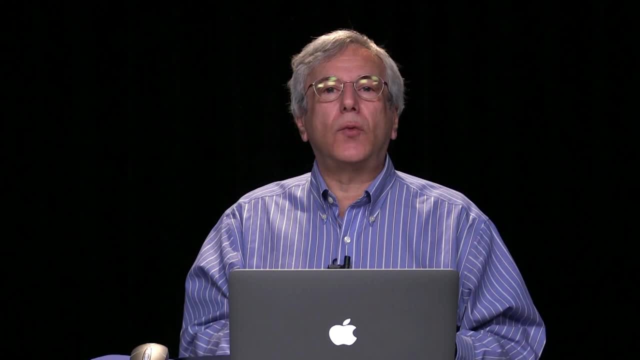 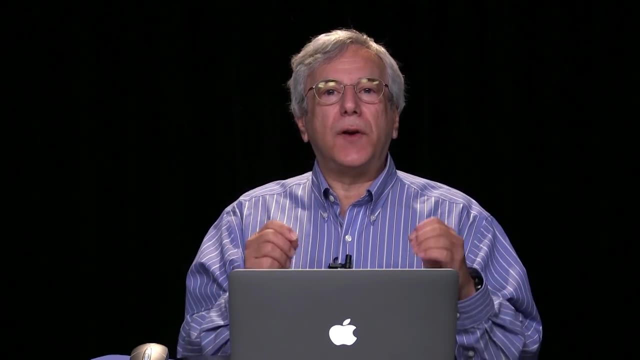 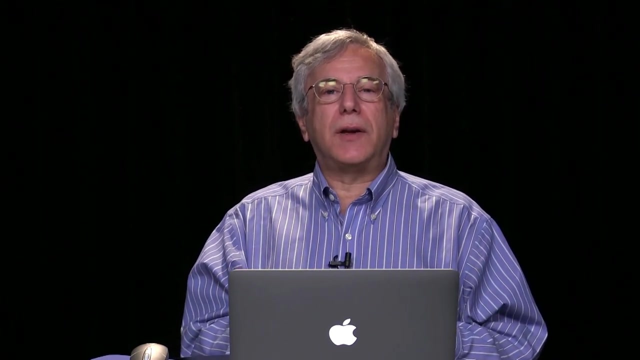 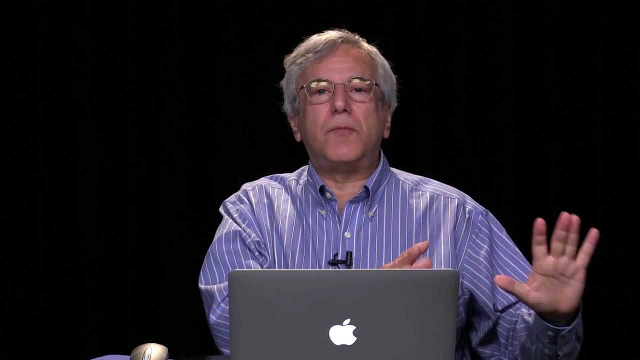 programming is to take all the situations in which we can use pure functions, all the situations where we can have immutable variables only, and make those situations be the focus of our programming effort. And then take the situations where we have to mutate something and either put them to the sideline or, in many 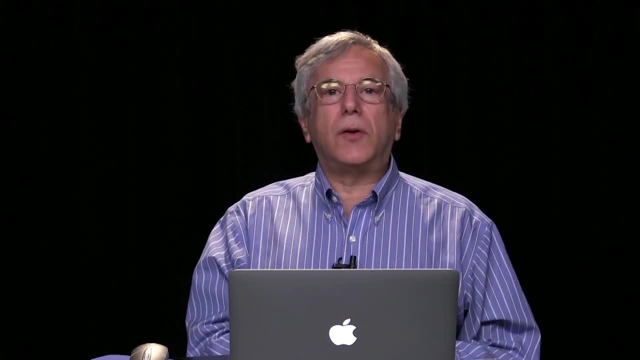 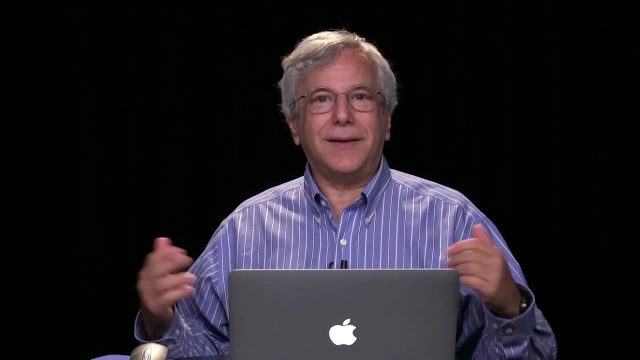 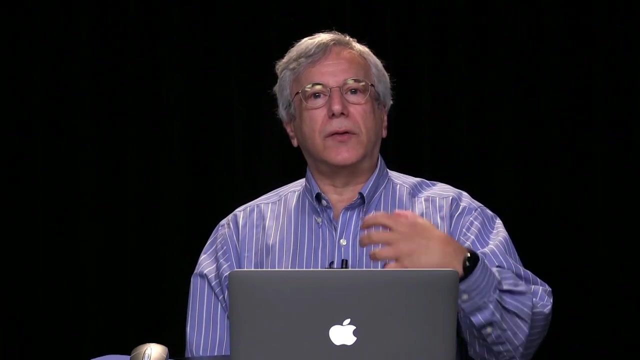 cases deal with them in a very clever way called monads. that helps us make mutable variables and side effects go away, if we can make them go away. So I'm not going to say that I'm not going to modify something external: the number of seats on an. 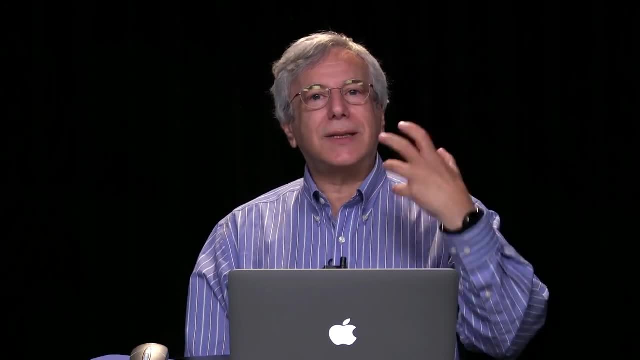 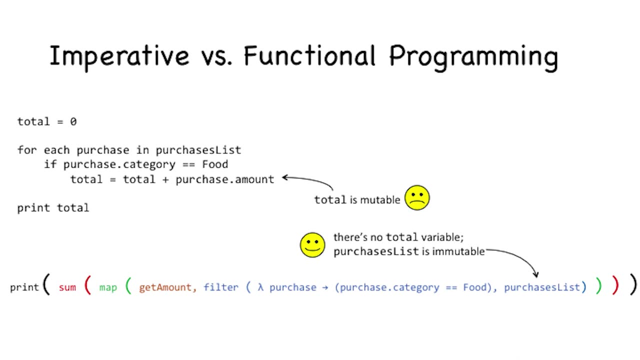 airplane. What I am going to say is that, Just as I did in the initial example, I'm going to take a situation where I take total equals total plus amount and I'm going to substitute that mutable situation, if I can, for a situation where I have purchases list and from that I make a new list of purchases filtered, and from that I make an amounts list and from that I make a sum. 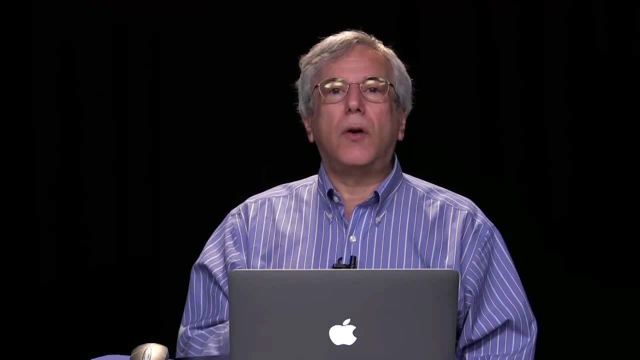 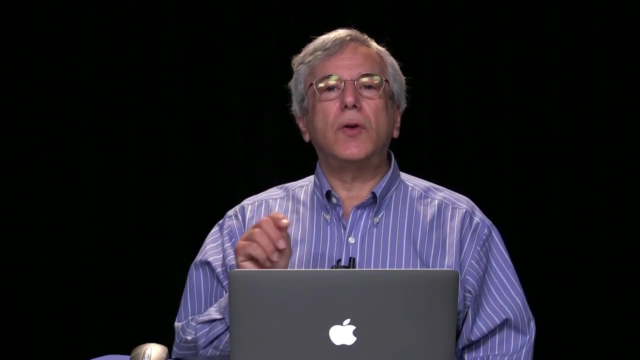 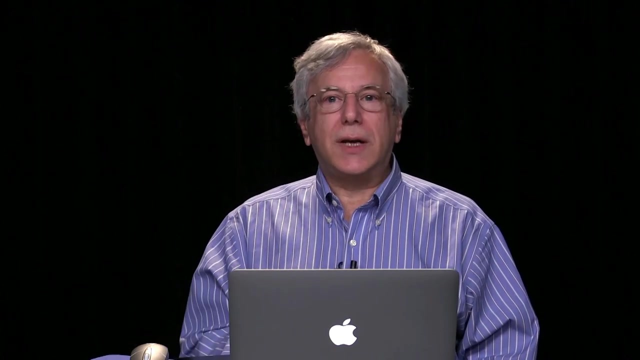 So, to the extent that I can, I'm going to watch out for those situations where there are mutable variables and try to isolate the mutability part to a part of the program where it's easy to manage. Okay, race conditions. avoiding race conditions and achieving thread safety is one of the many benefits of pure functions. 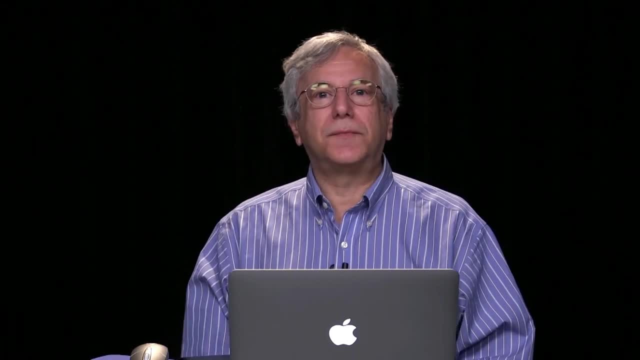 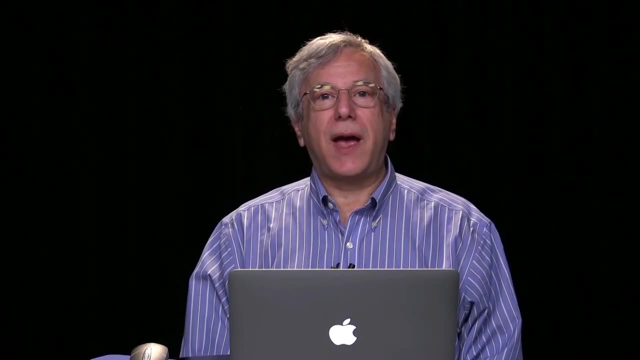 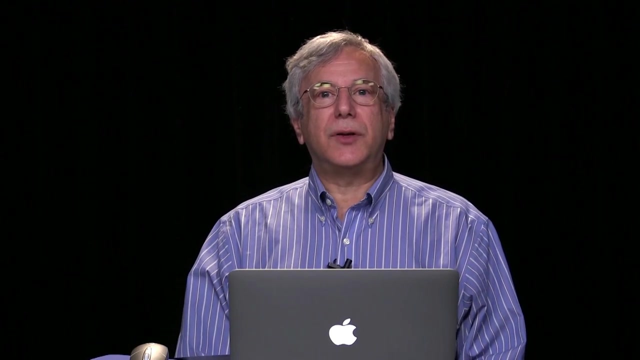 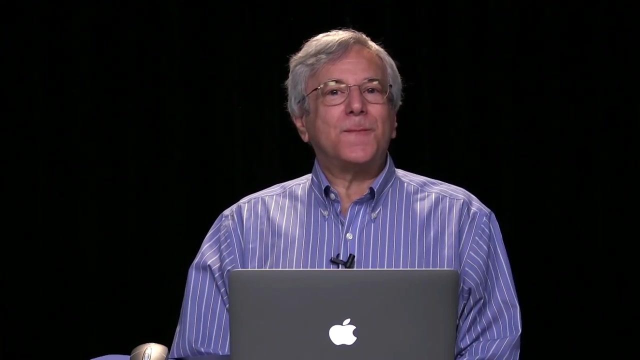 In the next section we'll talk about yet another benefit. We have to pass parameters to functions. We have to take a value that's in one part of the code and supply it as a parameter to a function. And if we've got a lot of data to pass, hmm, sometimes we can be taking a lot of time to pass that data. 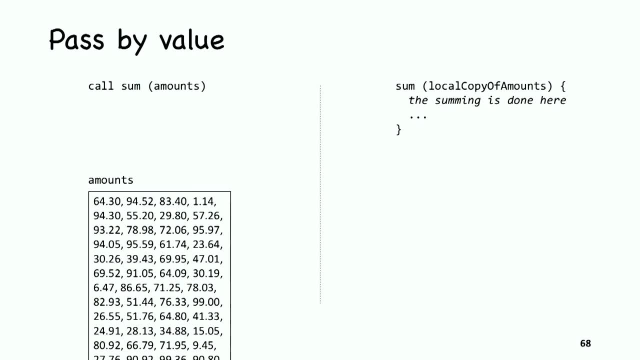 Let's take a look. I want to sum up a bunch of amounts And on this slide I have a bunch of amounts And on this slide I have a bunch of amounts And I've tried to make sure that the amount that it looks like there are many, many, many amounts that I have to sum up. 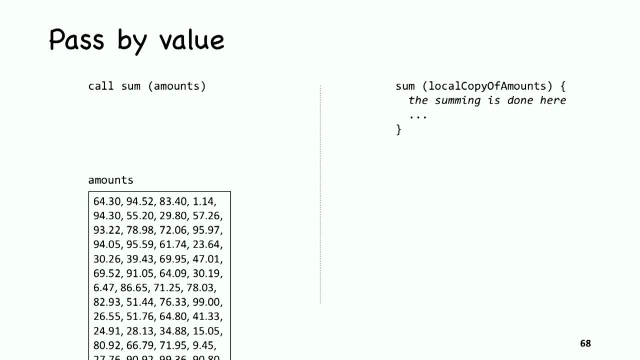 And I've even made it clear that there are even more amounts that you see here. If you can see on the bottom of the slide, I've made sure that you know that there are some amounts that are sort of dripping off the edge of the screen. 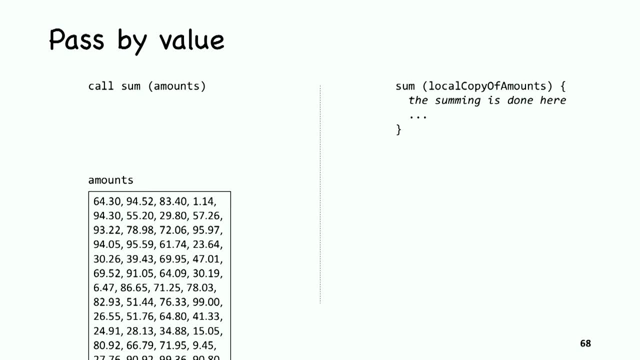 Okay, so I mean to have tons and tons of amounts that I have to sum up, which means there's a lot of data there. Okay, so what happens? I have a sum function And the sum function is on the other side of the slide. 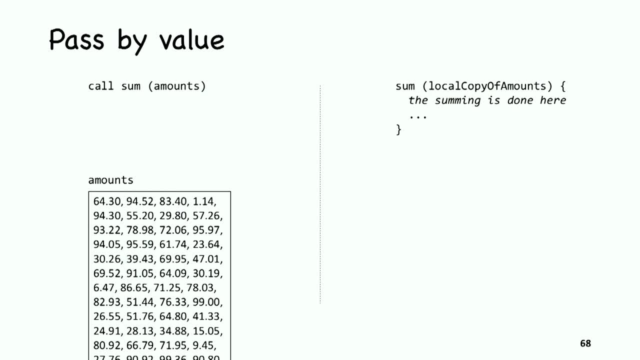 And the sum function has to somehow get access to those amounts. add them all together and, with its return value, return the sum to the left side of the slide. Okay, how are we going to do this? There are a couple of different mechanisms that are popularly used in the implementation of programming languages. 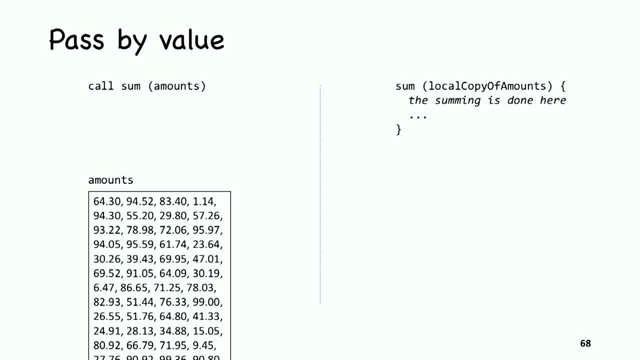 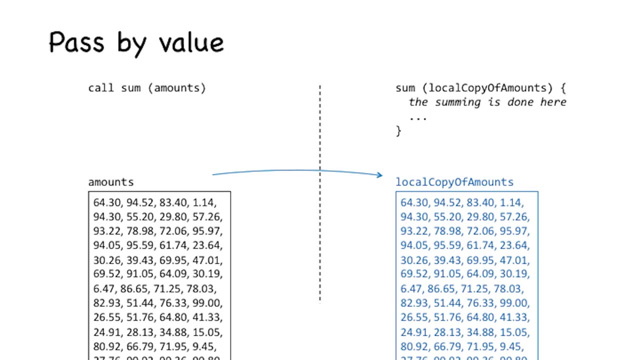 One of them- the title of this slide- is called pass-by value. So, with pass-by value, what I'm going to do is I'm going to take that huge collection of amounts and I'm going to make a copy of it, a local copy that the sum function can see. 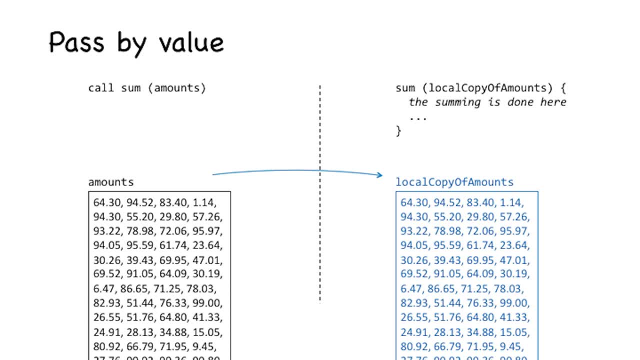 Now, there are good reasons for doing this and there are reasons not to do this. Let's start with the reasons, not The main reason not to do this, as far as I'm concerned, is because you now have the overhead of taking all the amounts, all the numerous amounts on the left side of the screen. 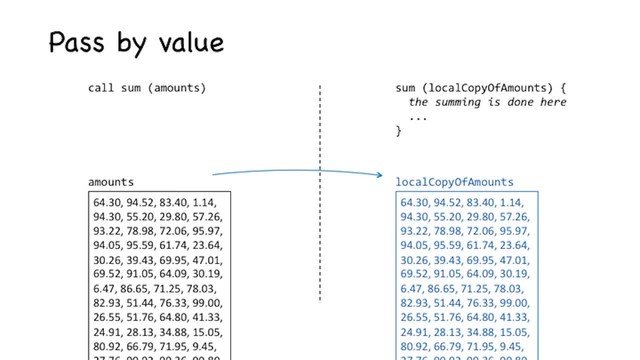 and taking the time to copy them one after another to somewhere where the sum function can access them. That's why I call it a local copy of amounts. All right, And if that's a lot of data, then that's a lot of time and a lot of space used just to make a copy. 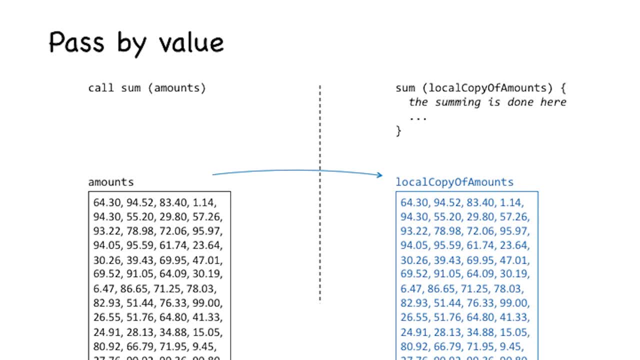 That's a lot of time and a lot of space used just to make a copy of something. That's not a good thing. That's a bad aspect of pass-by value- a potentially bad aspect. What's good about taking all those amounts and copying them to the other side of the slide? 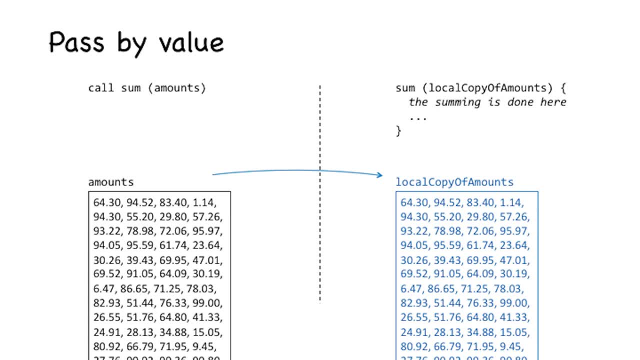 What's potentially good about it is that if some programmer inside the sum function decides to do the summing by temporarily modifying any of the amounts, then what that sum function will be doing will be modifying its own local copy. The amounts on the left side of the slide, the amounts that are accessible by the calling routine, are safe. 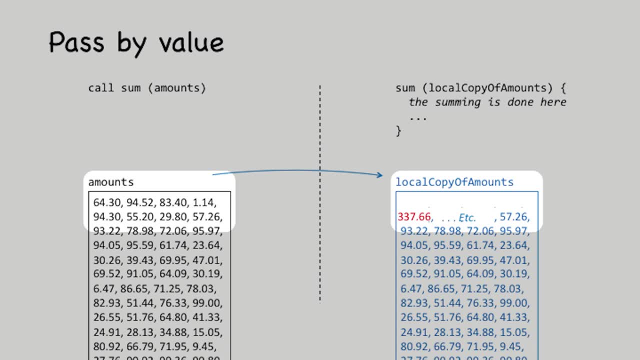 They're not going to be modified, no matter what the programmer on the right side of the slide does, And that's good If you've got something important, like the amounts of your purchases or the amounts of your profits or the amounts of your whatever. 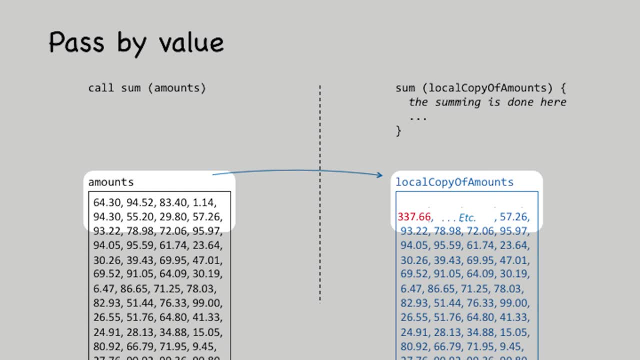 you probably don't want those to be modified accidentally by a call to a sum function. After all, if it's called a sum function even in its name, it doesn't imply that it's going to make any changes. But there are different clever ways of summing where you might temporarily modify the values of those amounts. 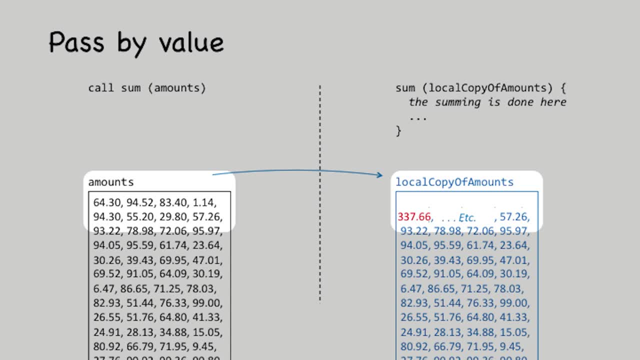 You don't intend for the values of the amounts to be permanently modified, But you might do it by accident. But if you've got your local copy over there in blue, then everything is safe And that's a good reason for using pass-by-value. 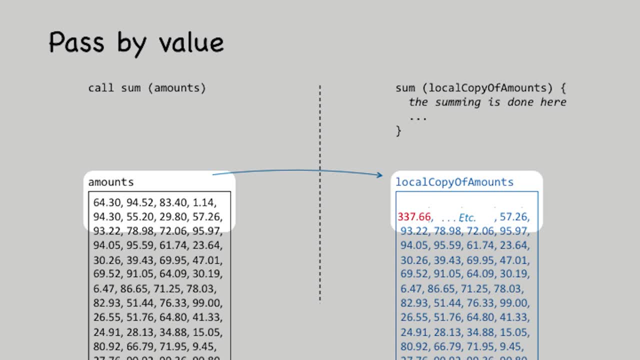 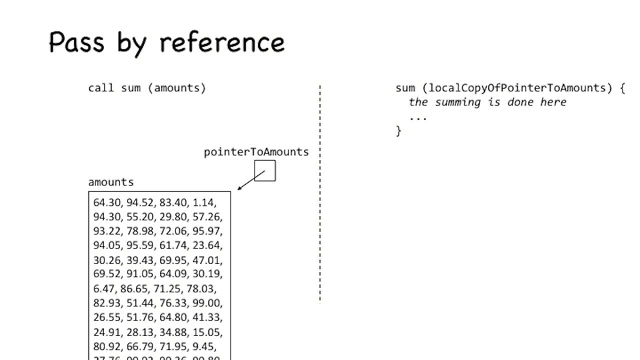 Well, what's an alternative to pass-by-value? The alternative to pass-by-value is going to be pass-by-reference, And pass-by-reference is going to be not as safe as pass-by-value, but it's going to be a heck of a lot more efficient. 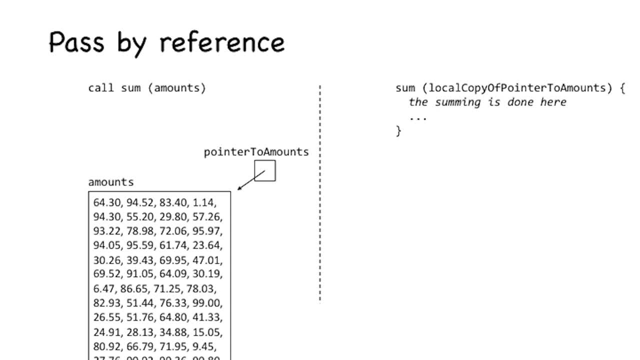 Let's take a look at the way pass-by-reference works. You start off with some sort of a pointer to this huge collection of amounts. Now the word pointer is scary to some people who are learning programming. I don't intend it to be scary. 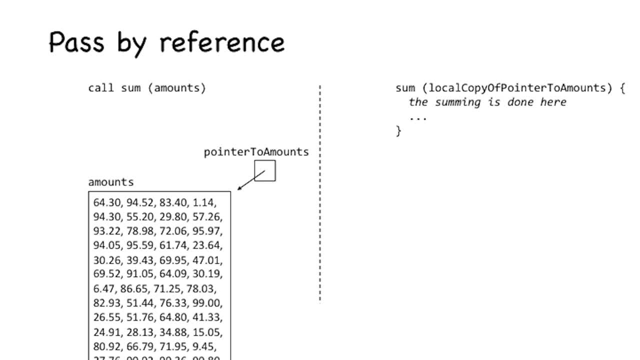 That arrow simply indicates that you've got a variable called pointerToAmounts and it somehow indicates where in memory to find this list of amounts. If you like, you can think of the amount collection as starting in memory, location 2,000,. 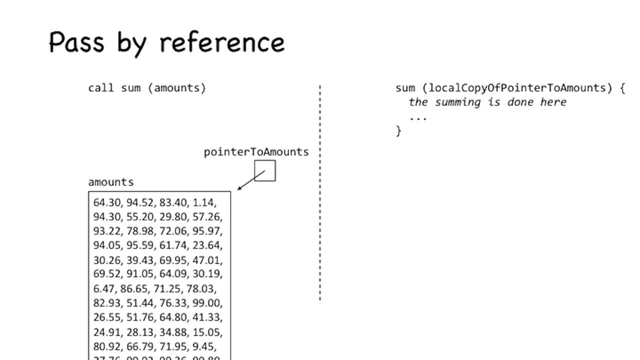 and maybe what's stored in the pointerToAmounts variable is just the number 2,000.. Okay, All right. Anyway, I've got some pointerToAmounts thing that indicates where on the system to find the amounts. Well, with pass-by-reference, what I do is when I call the sum function. 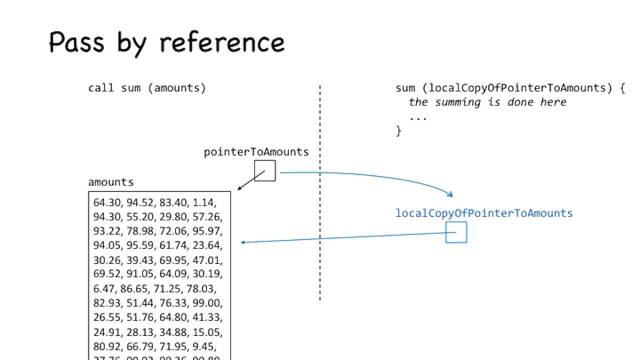 I'm going to just send it that pointer. I'm just going to pass not the entire number, not the entire collection of amounts, but instead I'm just going to pass what's called a reference to amounts. Maybe it's the address where amount starts. 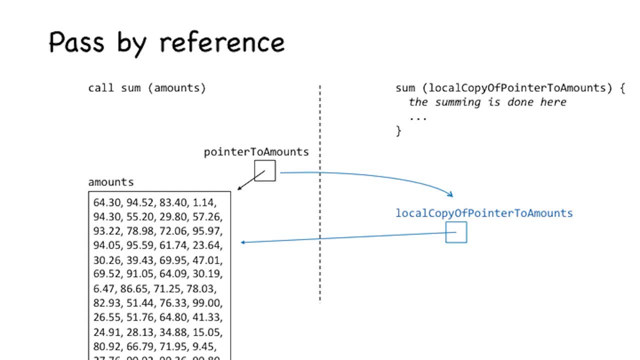 or maybe it's some other indicator of where to find amounts in the system. Now that means that what the sum function is doing is it's looking at that pointer and it's saying, aha, the first amount is 64.30.. 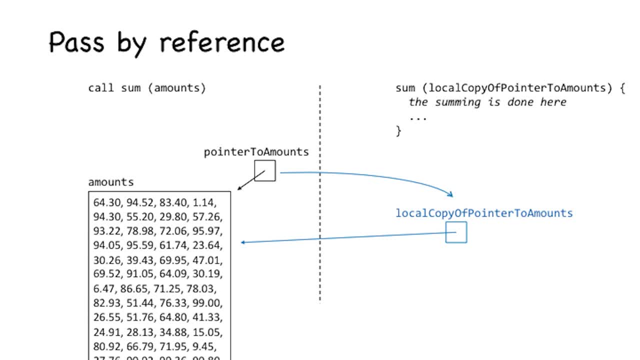 The second amount is 94.52.. I'm going to add those things together and come up with a sum. Ah yes, I've managed to pass one tiny piece of data to the sum function. I didn't copy all the amounts. 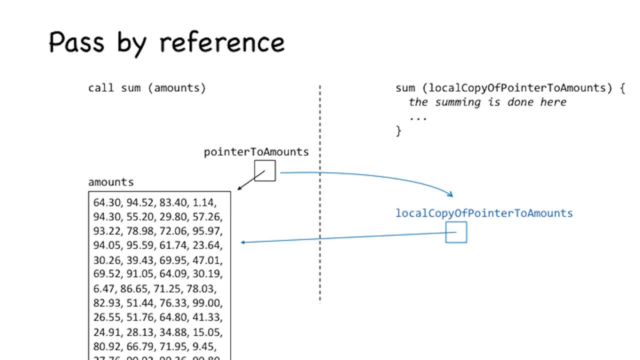 I didn't incur any of the overhead, I didn't waste any more space by duplicating that big set of amounts And I didn't take time in copying them. But what did I do? I lost a little bit of safety, And the safety that I lost was that now the sum function refers to the original bunch of amounts. 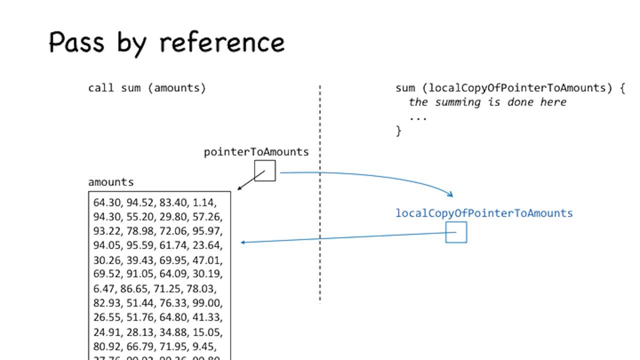 So if the sum function, accidentally, or maybe even in an attempt to be clever, starts modifying the amounts, thinking that it's doing it temporarily, the problem is that those amounts can change. Now if you're looking at it just from this slide and saying 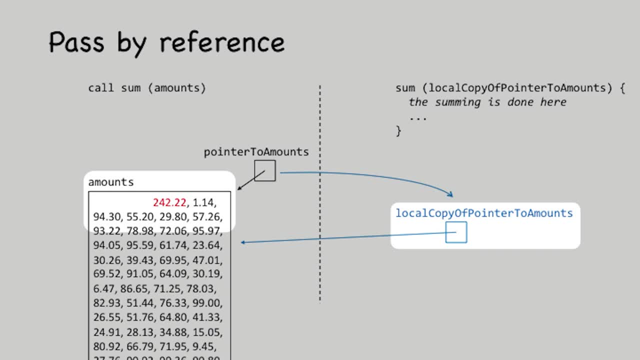 well, this is a simple situation. I'm sure that a person who's writing the sum function can avoid making that change. Well, in a simple scenario like this, you're probably right. But in a more complicated scenario where you've got millions of lines of code, 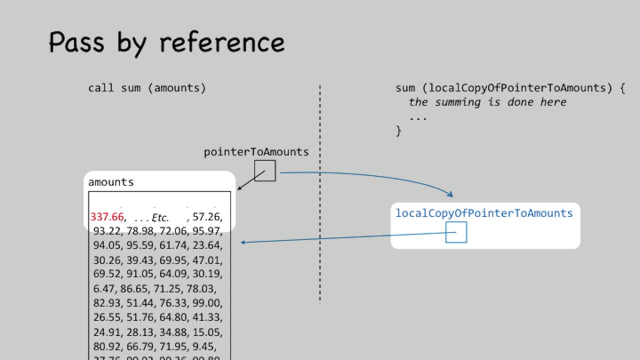 it's really easy for a programmer to accidentally do something that modifies something like that list of amounts. So with pass-by reference you're trading. You're kind of making a trade, You're getting much more efficient code, but you're also risking a little bit of. 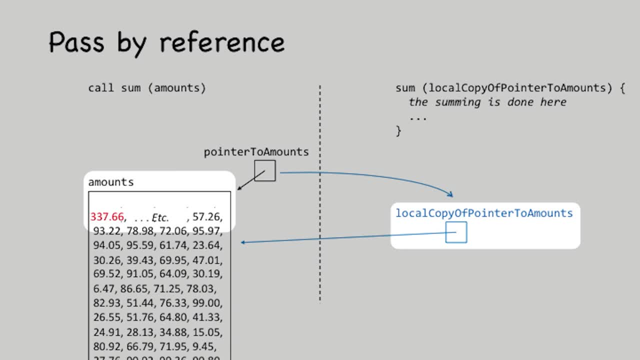 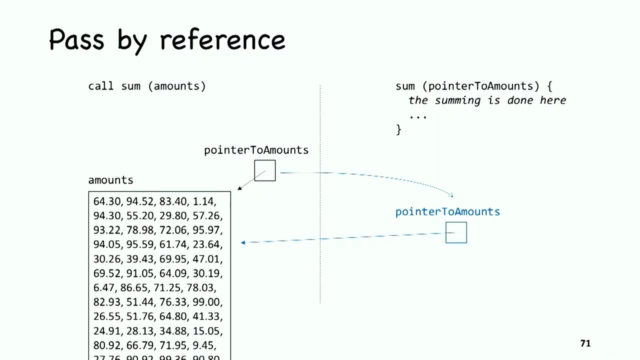 safety in being able to change the amounts. Well, what does this have to do with pure functions If you're in a programming environment where you use only pure functions, where perhaps the language enforces the use of pure functions, or where you have somehow agreed to check for the purity of functions? 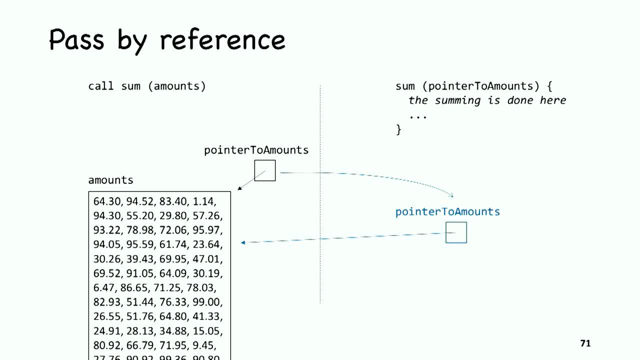 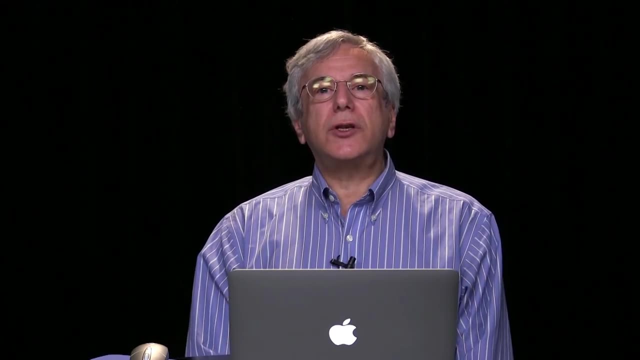 or where somehow the language structures are set up so that the functions in a certain situation, in a certain context are guaranteed to be pure, then if you know that the sum function is pure, that is an assurance that the sum function will not change anything external to it. 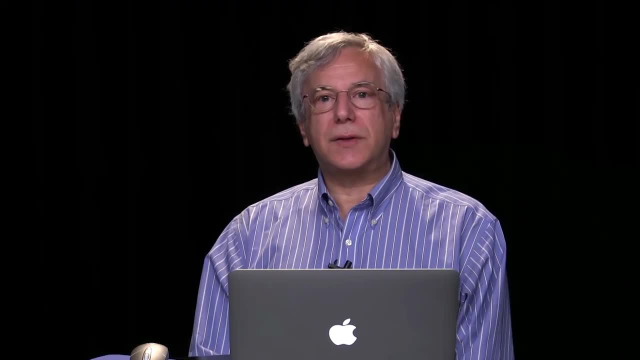 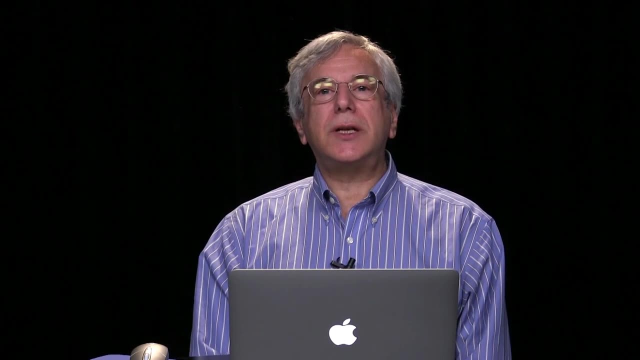 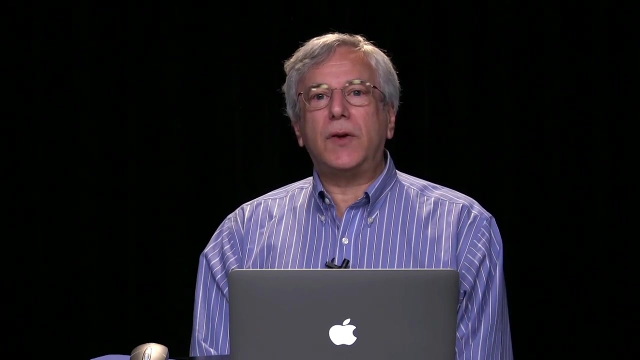 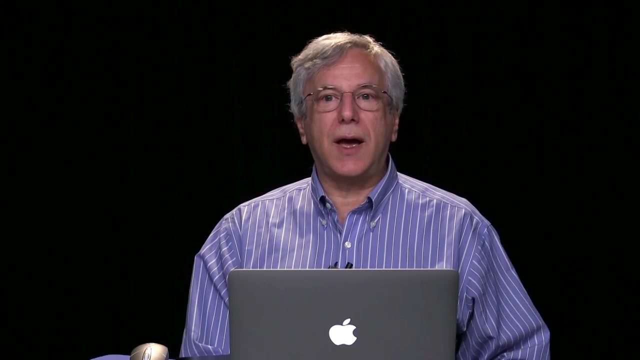 It will not change the values of amounts. So in this case, purity- the notion of a pure function- helps us achieve a good, good mix between two benefits. We can do pass-by reference and only pass a tiny bit of information instead of an entire collection of amounts. 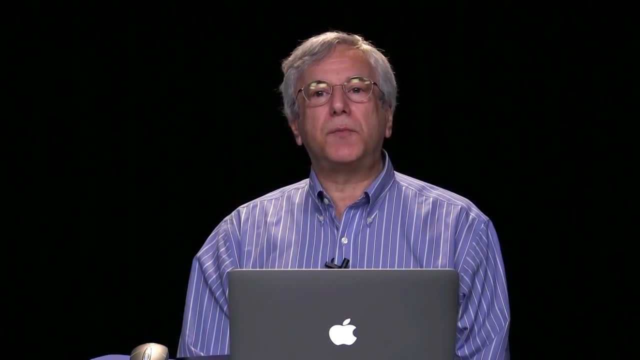 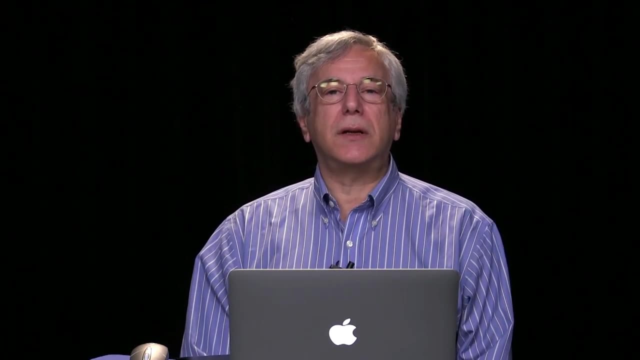 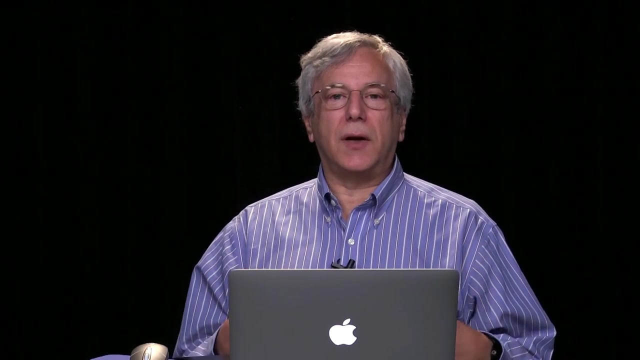 But also if we're sure that the sum function is pure, we know that we have the safety of having the sum function not modify the amounts that it started with, so that the situation, the program, the processing environment will maintain its correctness. 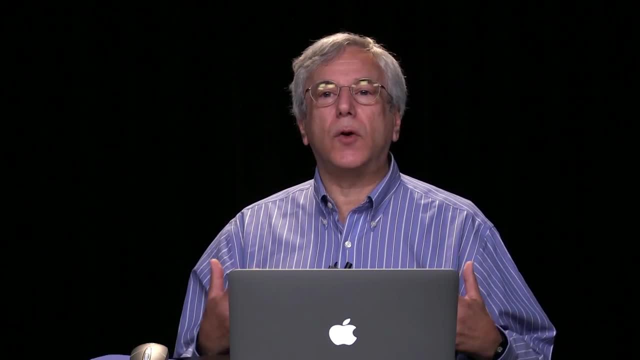 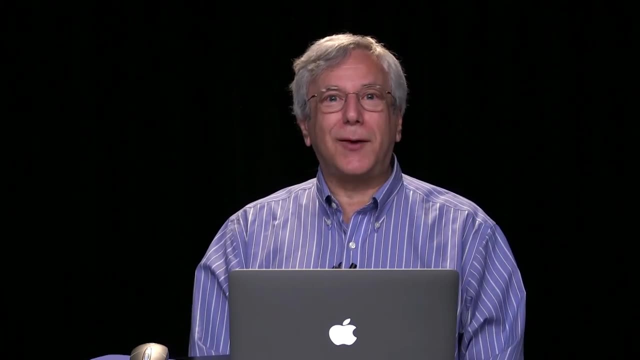 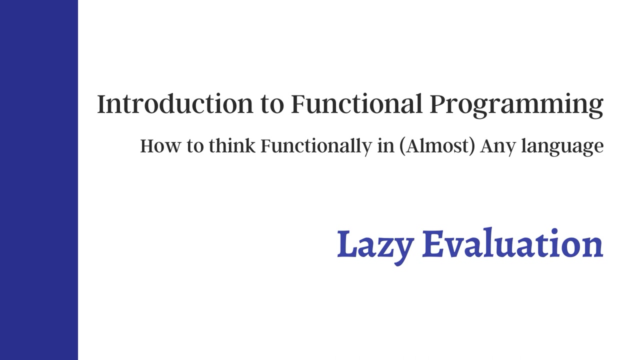 will maintain its integrity. The values and amounts won't be changed. Aha, There we have it: Another benefit of pure functions. You want to see another one? I've got one more. Check out the next segment. I don't know about you, but I enjoy being lazy. 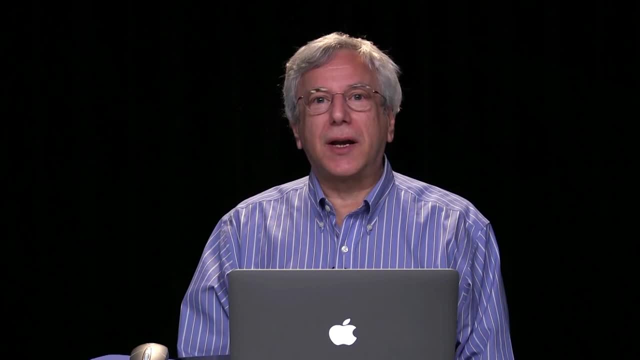 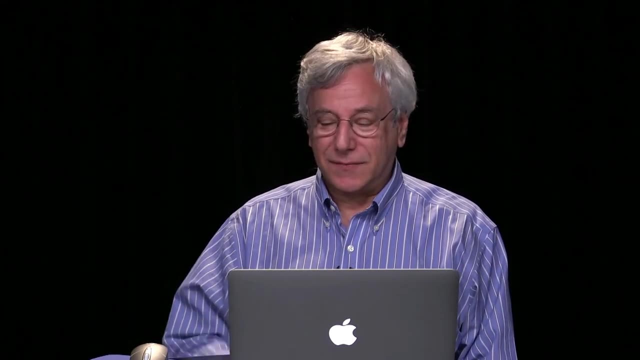 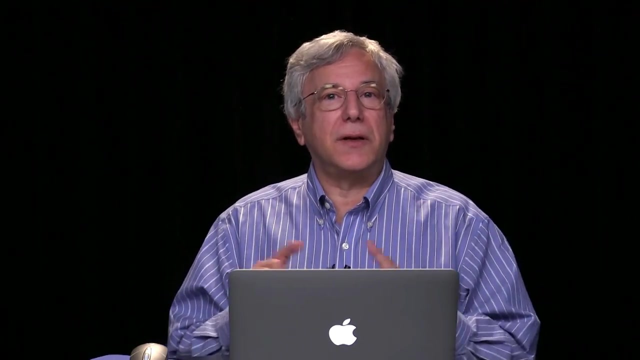 I really do. Instead of starting this course at 9 am on video, I started it at 10 am today. I like laziness. I like sleeping a lot. I really appreciate being lazy, but the word lazy has a bad connotation in most circles. 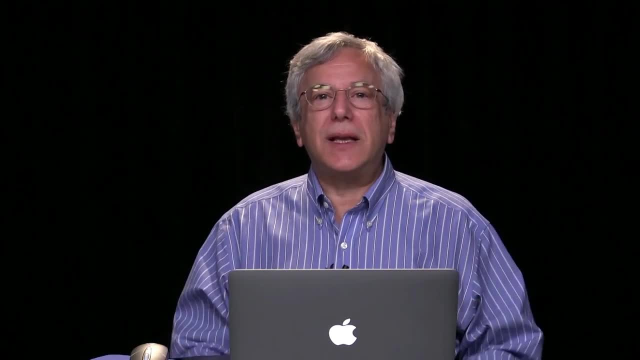 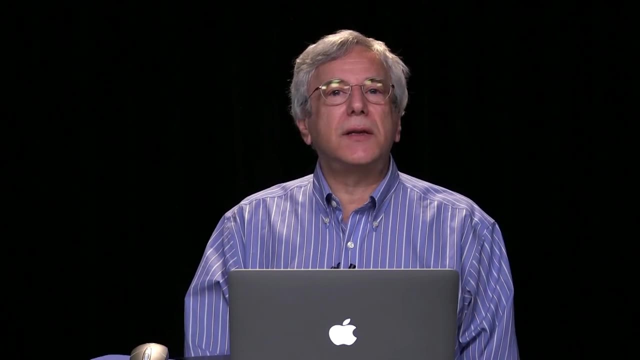 It's: oh no, you shouldn't be lazy. Well, should your computer be lazy? I think sometimes it should. You know, a lazy computer is one that doesn't do any more work than it has to do. It achieves the result that it has to achieve. 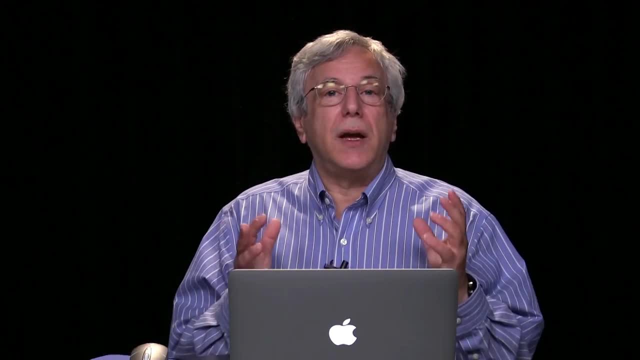 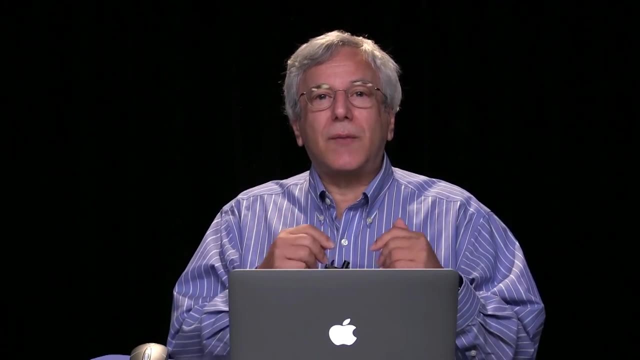 but doesn't take any more time to achieve it by doing computations that it doesn't have to do. Laziness can be good, And let's see some examples of laziness. Let's see some examples of non-laziness and see the difference. 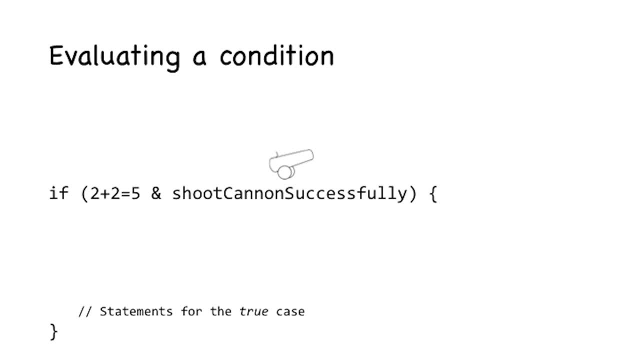 Here's my first example. My first example is a- yeah, kind of a very stilted, manufactured example. I'm going to have an if statement and the if statement is going to evaluate two conditions and then combine them with an and. 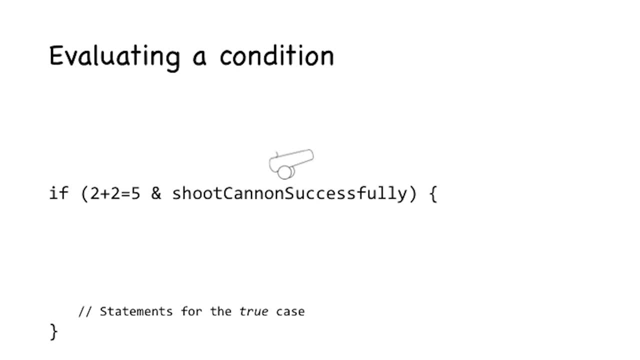 And the two conditions are: 2 plus 2 equals 5 and shoot cannon successfully. Now, yep, I agree, 2 plus 2 equals 5 is going to evaluate to false. What about shoot cannon successfully? What I mean by shoot cannon successfully is: 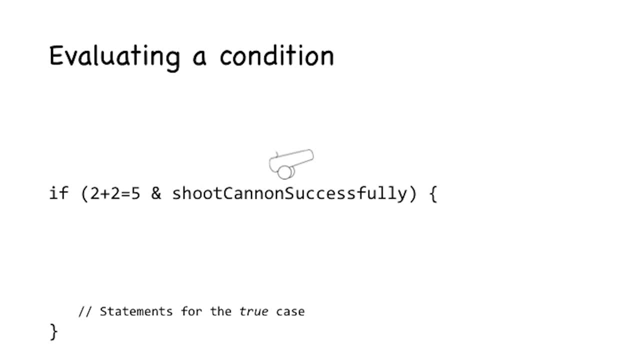 I'm going to when I evaluate that expression. try to shoot off a cannon and if the cannon actually gets shot, then shoot cannon successfully is going to return. true, If the cannon isn't successfully shot. hey, sometimes cannons don't go off when they should. 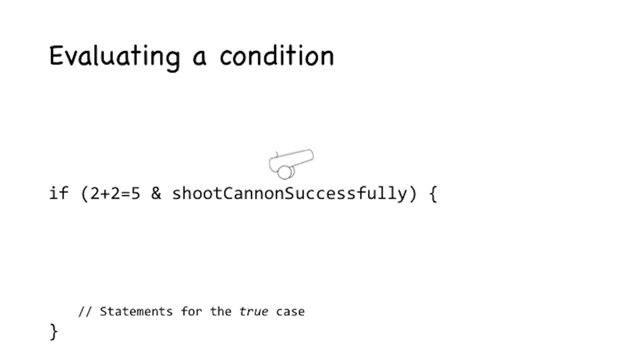 then shoot cannon successfully, is going to return false. Now, what do we know about the stuff inside the parentheses? We know the following: It's going to end up being false, whether the cannon shoots or not. And the reason it's going to be false. 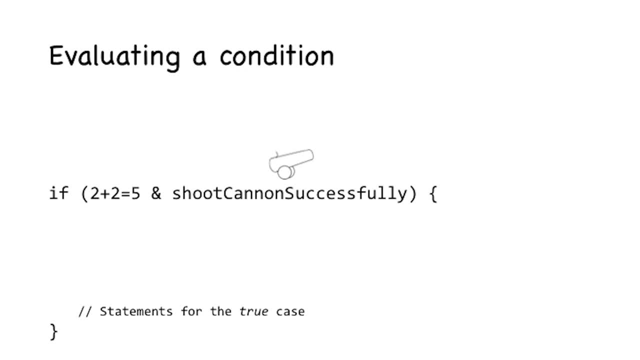 is because 2 plus 2 equals 5 is false. So the part of the expression that's to the left of the ampersand symbol is going to make the whole condition false. So the question is, do I really need to bother evaluating shoot cannon successfully? 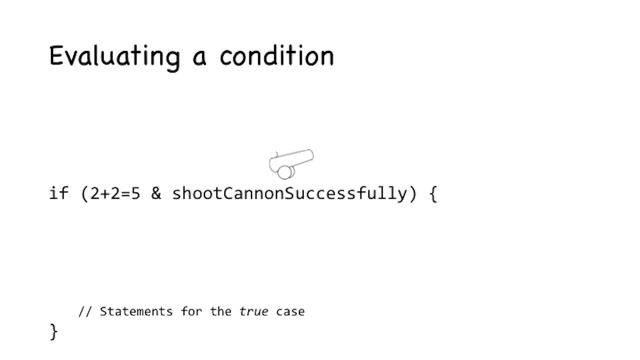 in order to know how this if statement is going to turn out. The answer is no, So I have two alternatives here. I can evaluate this expression lazily by saying: all I need to do is find out if 2 plus 2 equals 5. 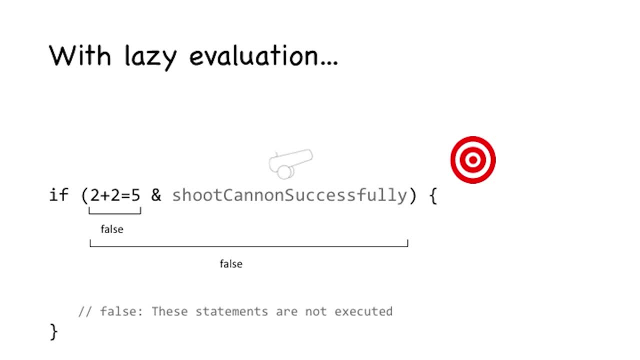 and then stop evaluating, Or I can evaluate this expression in a non-lazy fashion, And the word for non-lazy is eager. I can evaluate this expression in an eager fashion, And evaluating this expression in an eager fashion means well, doing the extra work of evaluating everything. 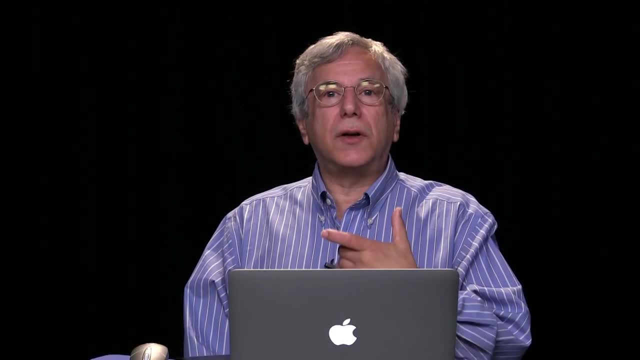 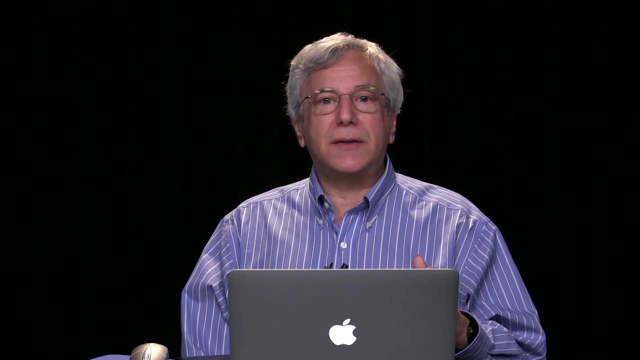 even though I don't have to, in order to find the ultimate result. So, with eager evaluation, what I will do here is: first I'll find out if 2 plus 2 equals 5. No, it isn't, But I'm eager. 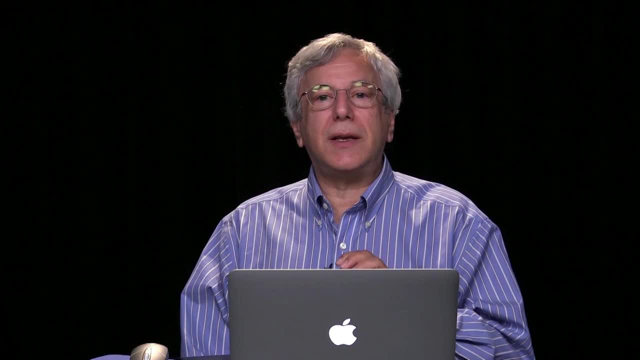 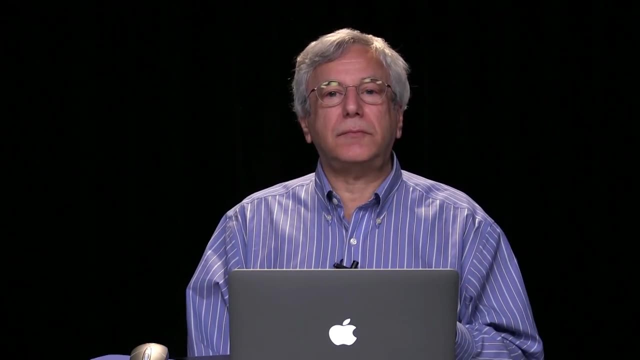 And before I combine 2 plus 2 equals 5, with anything I'm going to do, shoot cannon successfully. I'm going to try to shoot the cannon. Well, let's assume, for the sake of argument, that the cannon does shoot. Cannonball goes out. 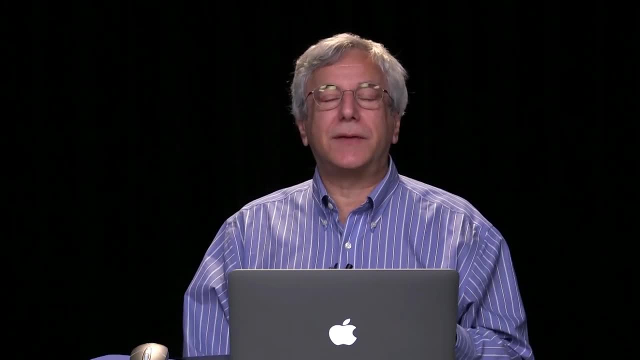 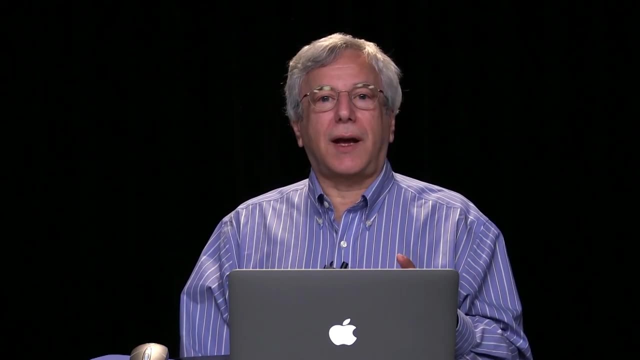 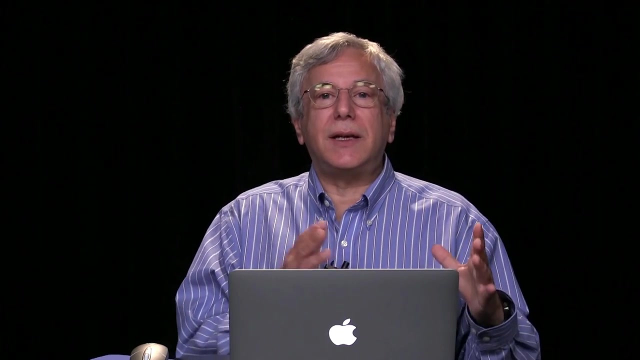 It flies in the air, It goes and hits something- All kinds of damage. Well then, what's happened? As a result of doing eager evaluation, I actually shot the cannon. That's a different outcome overall than I had with lazy evaluation, where I didn't even bother evaluating. 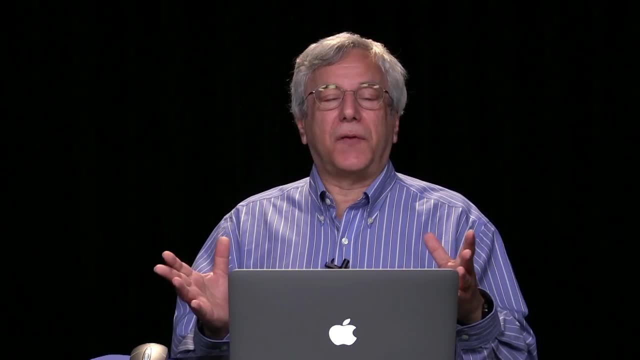 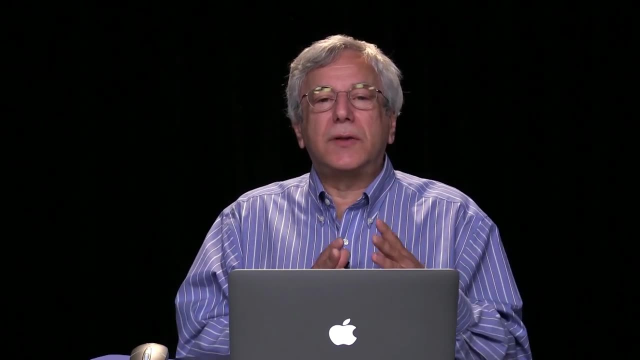 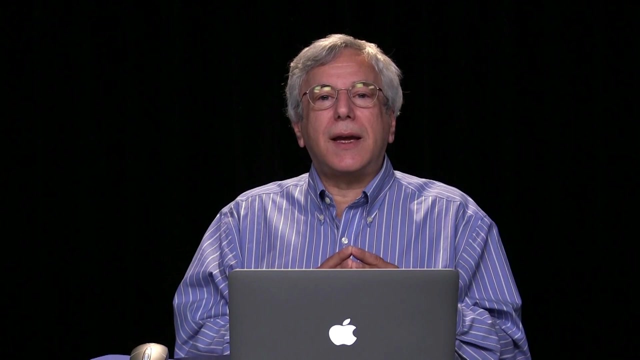 shoot cannon successfully. And what did I get for that? I got nothing. I still got the same conclusion with the if statement that 2 plus 2 doesn't equal 5, so the whole business inside the parentheses is false. Okay, I guess you might indeed want to shoot cannon successfully. 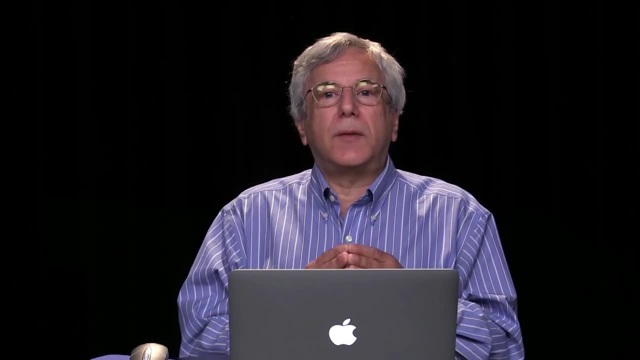 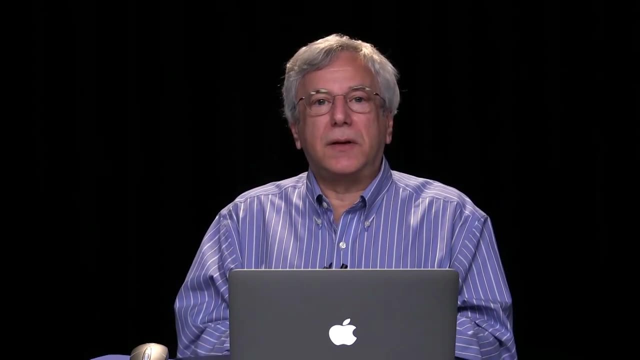 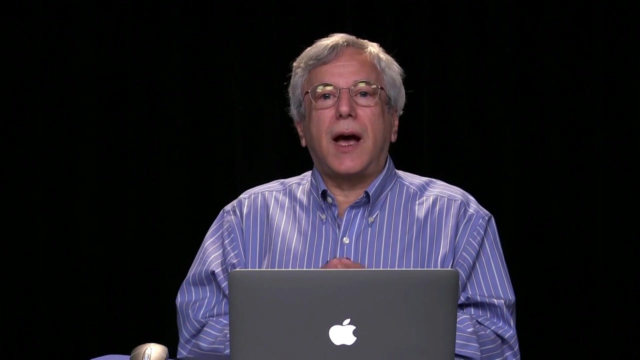 You might want, in a case like this, some kind of eager evaluation, But let's note the difference in the two ways of evaluating this expression. With lazy evaluation, I will not even try to shoot the cannon. With eager evaluation, I will try to shoot the cannon. 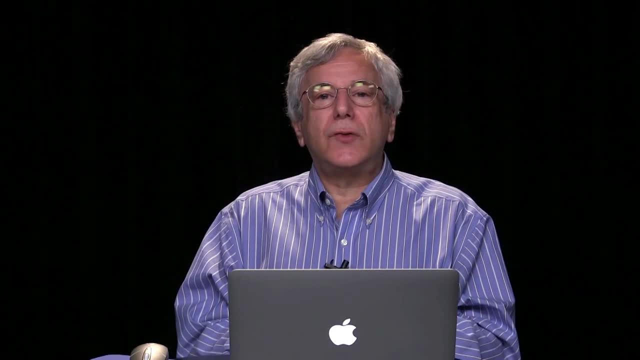 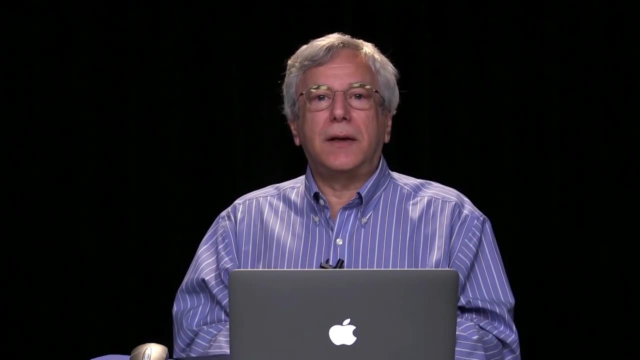 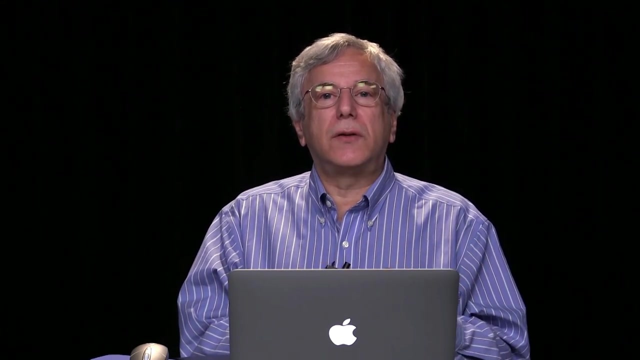 So 2 plus 2 equals 5, and shoot cannon successfully has computationally a different overall effect if I'm doing lazy evaluation than if I'm doing eager evaluation. So lazy evaluation and eager evaluation make a difference. And why does it make a difference? 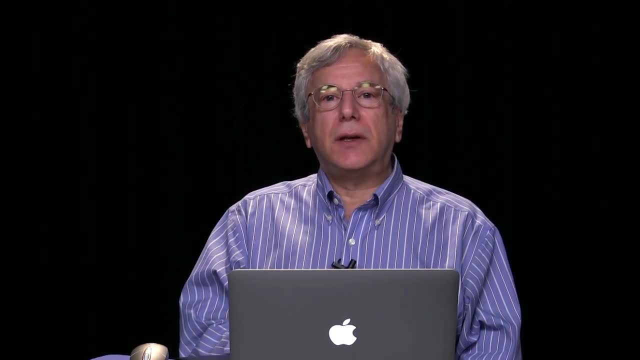 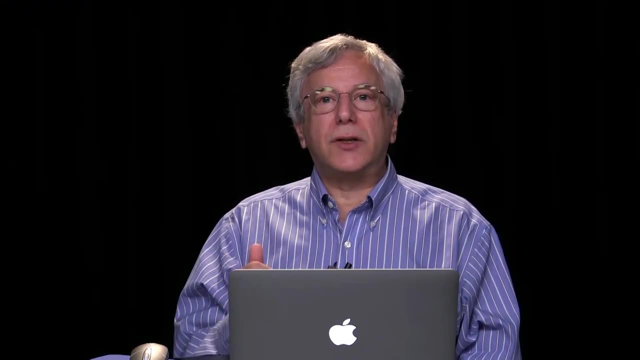 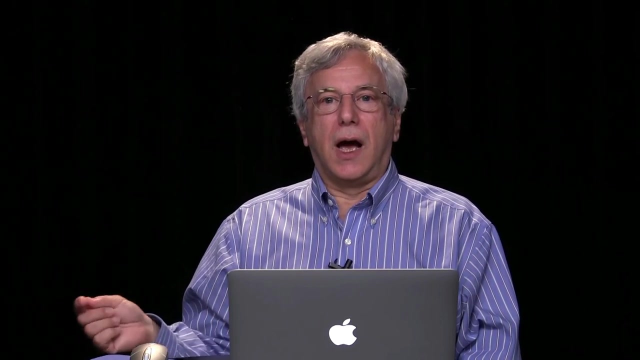 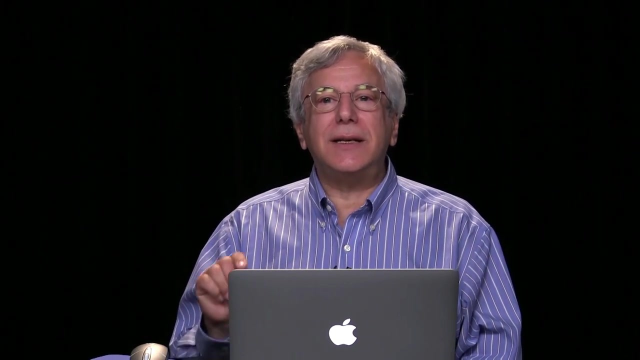 Why does lazy evaluation give you a different overall result than eager evaluation in a scenario like this? It's because shoot cannon successfully is an expression with a side effect. If shoot cannon successfully didn't have a side effect, if shoot cannon successfully was pure. 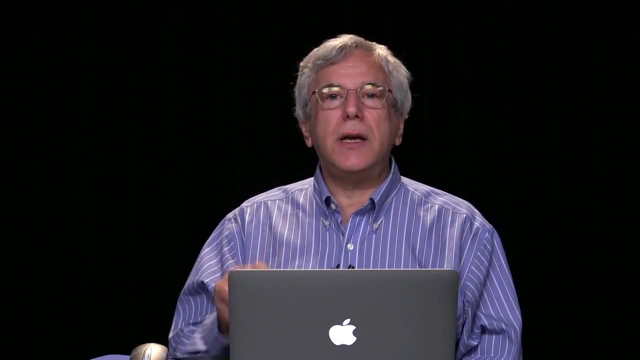 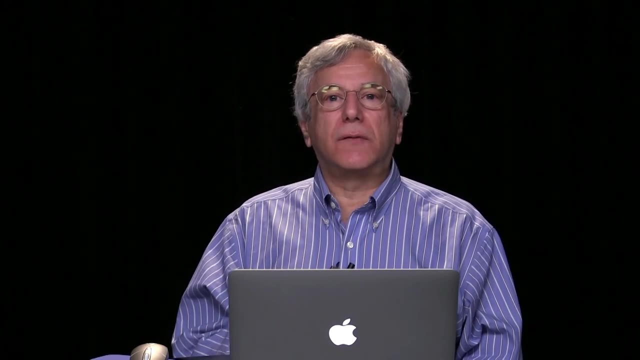 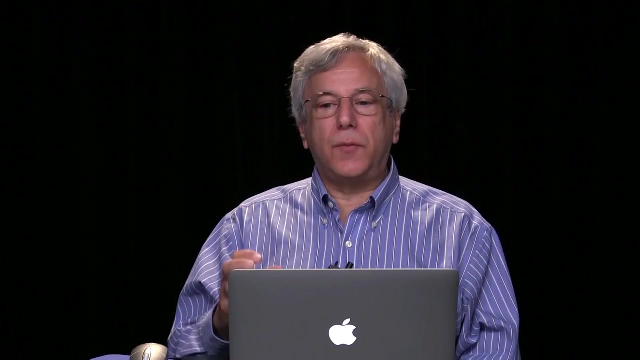 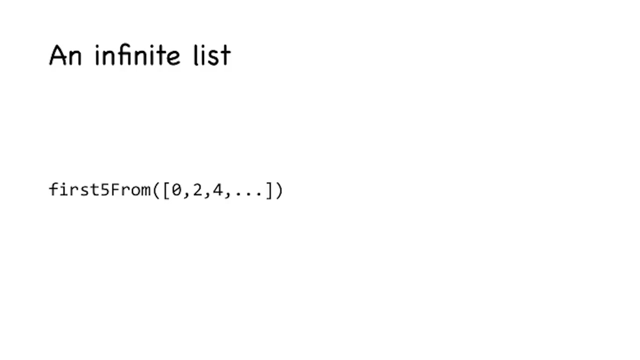 then the lazy evaluation and the eager evaluation would be exactly the same. So purity matters when it comes to the use of lazy evaluation, And lazy evaluation can be good for avoiding extra computational effort. Let's take a look at another example. In this example I have a list of numbers. 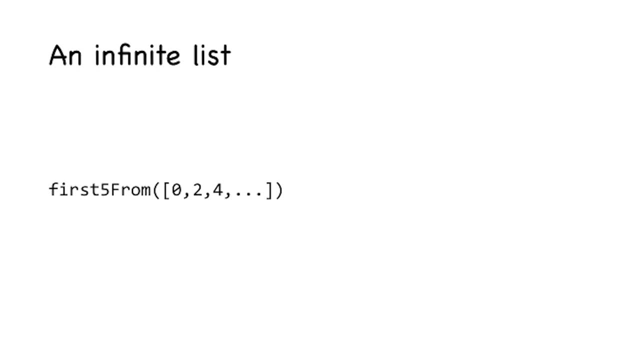 0,, 2,, 4,, 6,, 8,, 10, 12.. The list that's a parameter to the function. the list with dot dot dot in it, ellipsis in it, that's meant to be an infinite list. 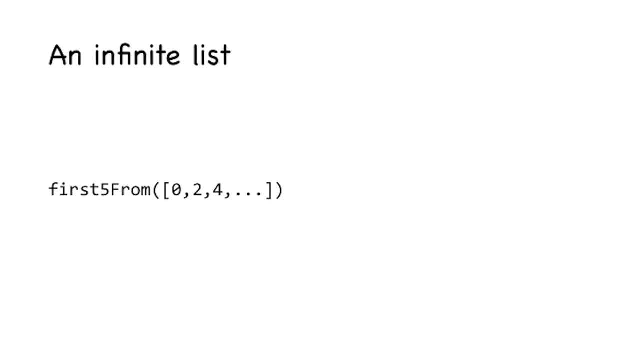 So if I were to evaluate what does 0,, 2,, 4,, dot, dot mean, I would get that it's a list of numbers that goes on forever. And if I want the first five values from that list, well, I have two ways of doing it. 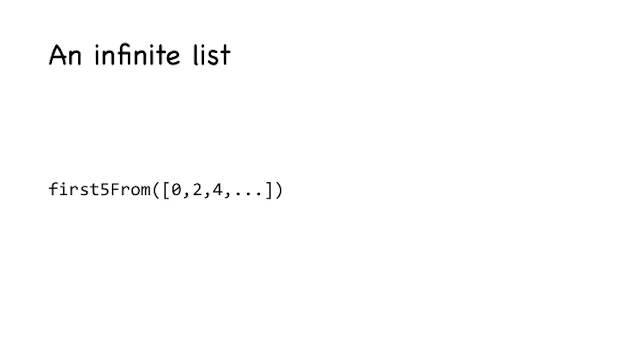 I can do either eager evaluation or lazy evaluation. How do eager and lazy evaluation differ in this scenario? With eager evaluation, I would say I'm going to first evaluate completely what's in the list: 0,, 2,, 4,, dot, dot, dot. 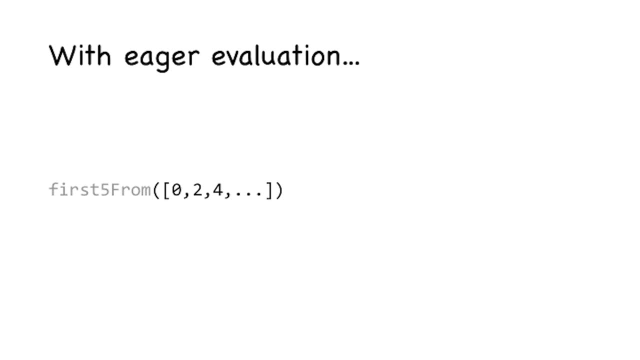 So, with eager evaluation, I have to find out what that dot dot dot means before I can do anything else, before I can take first five from Now, look to find out what 0,, 2,, 4, dot dot dot means. 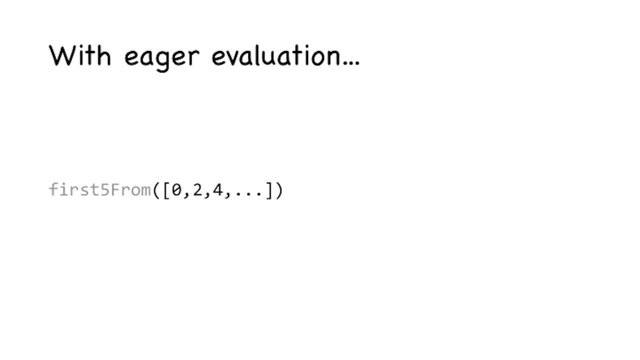 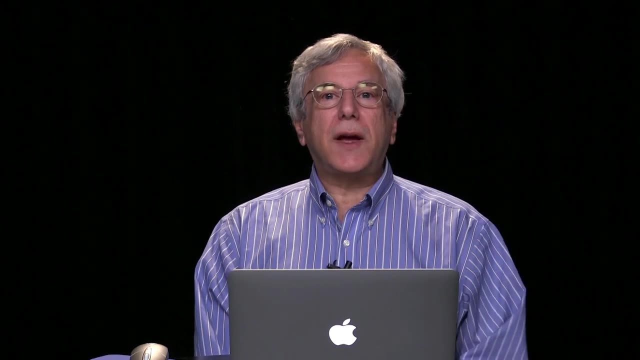 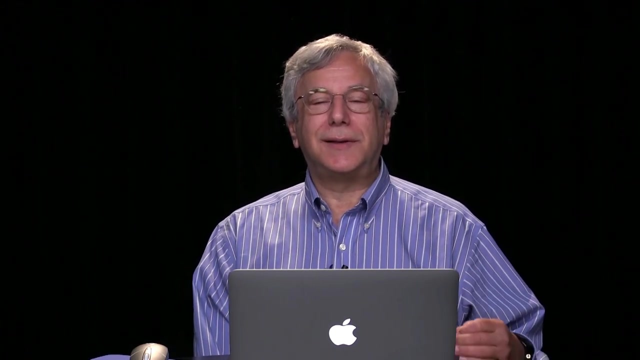 is going to take, well, potentially an infinite amount of time. It's going to send me into an infinite loop. I'm never going to finish doing it. So if I use eager evaluation in this scenario, I will never stop computing. I can't use eager evaluation. 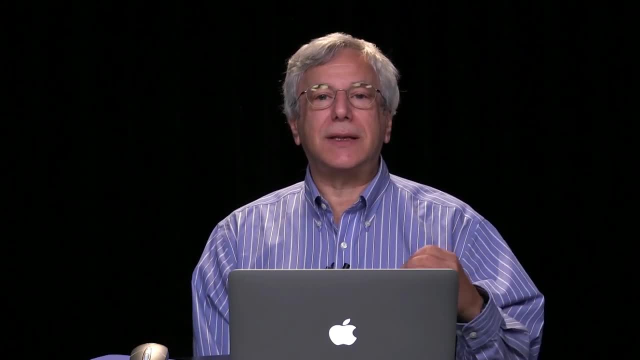 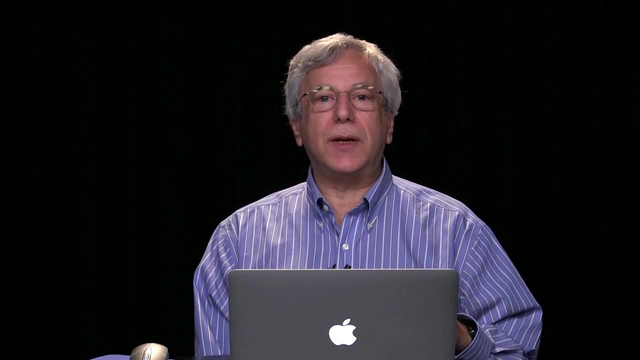 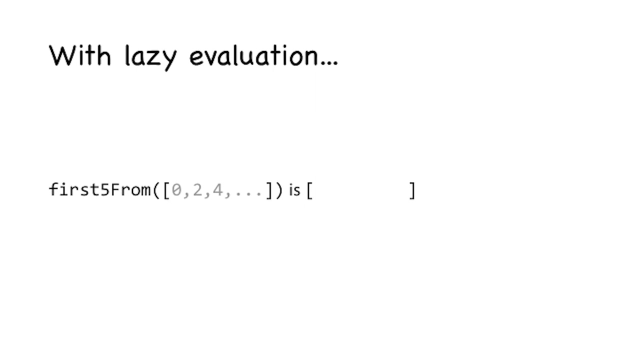 to find the first five elements in this infinite list. Instead, what I have to do is use lazy evaluation. What does lazy evaluation do for me? It says that to compute the first five elements of that list, I have to do as little work as possible. 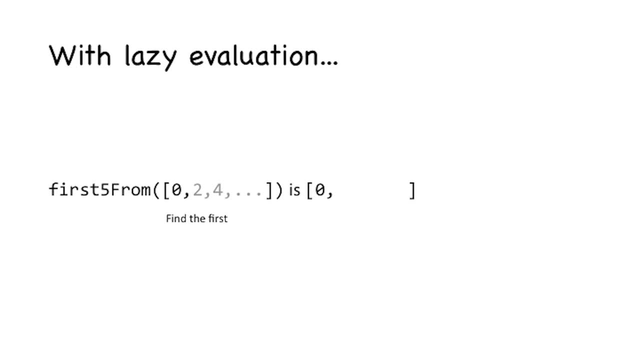 I just have to find the first element, which is 0,, the second element, which is 2,, the third element, which is 4,, the fourth element, which is 6, and the fifth element, which is 8,. 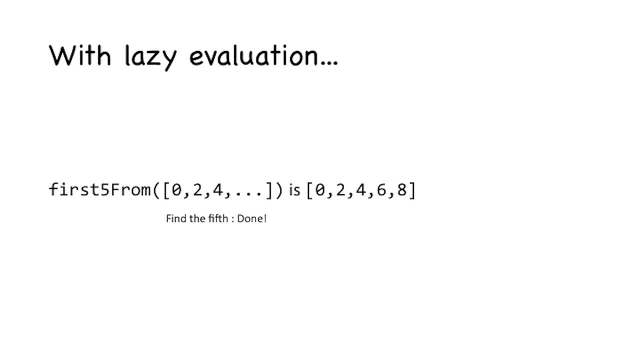 and then I stop. Here's a situation in which lazy evaluation isn't just more efficient, It's the only way to go. It's the only thing that's possible. If I try to do this expression, if I try to figure out first five from: 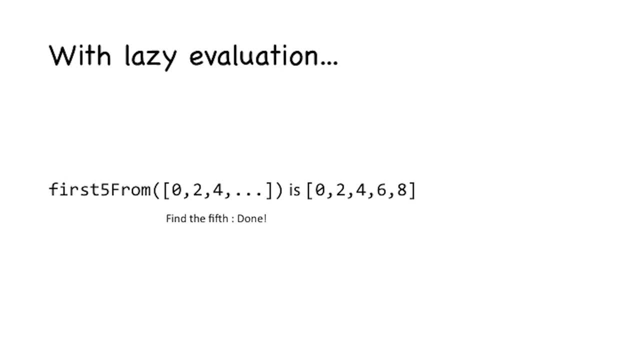 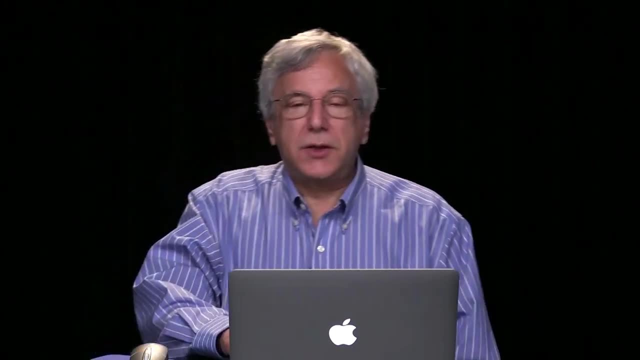 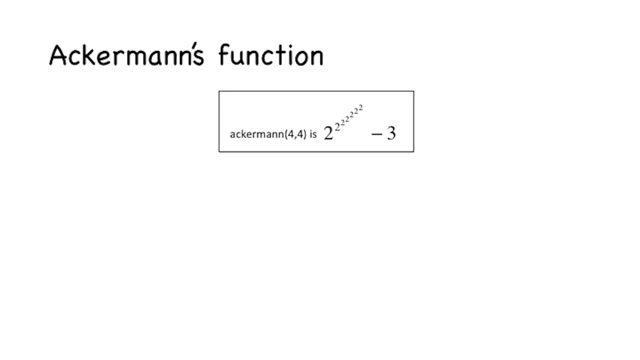 an infinite list in an eager fashion, I will fail. Fail meaning I'll never finish computing. Alright, speaking of never finishing computing, let's take a look at a really interesting function called the Ackermann function. Now, as soon as the words 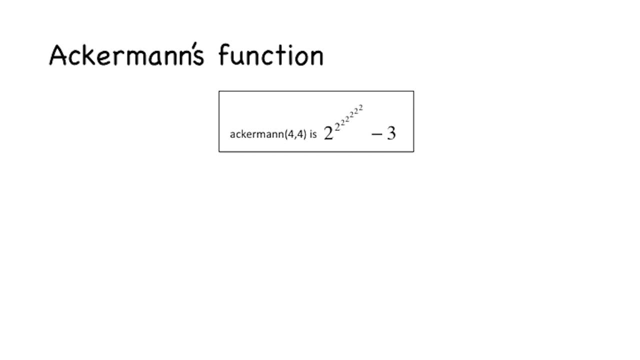 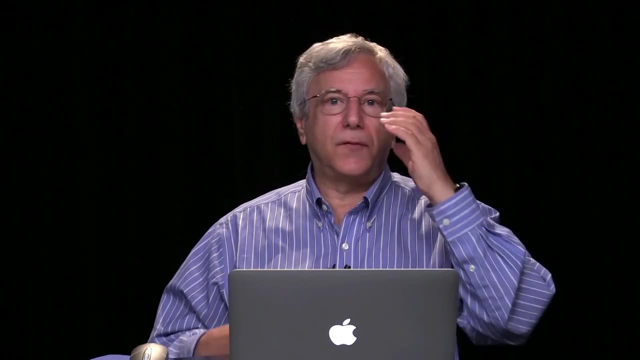 really interesting come out of my mouth. I realize I'm not even going to show you the definition of the Ackermann function. It's a mix of three formulas And they're recursive formulas And it's very clever stuff. The point is that 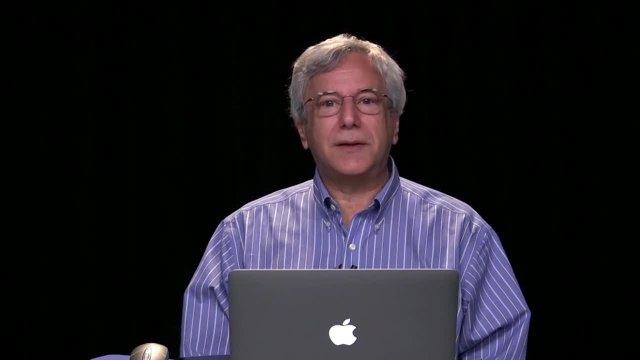 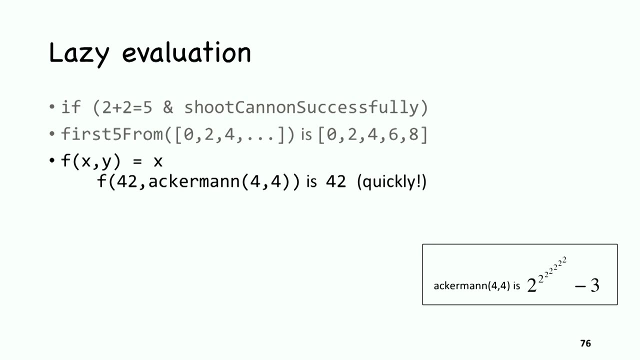 Ackermann function takes two arguments. a first argument, a second argument: On the slide it says 4, 4,, but I could just have easily substituted in 0, 1 or 1, 2 or 20, 50,, something like that. 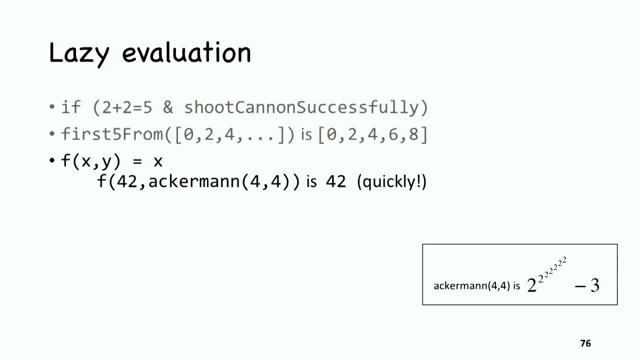 Interesting thing about the Ackermann function is that its height, its value grows very, very, very, very quickly. So the value of the Ackermann function when I plug in 0, 1 is some small number, No big deal. 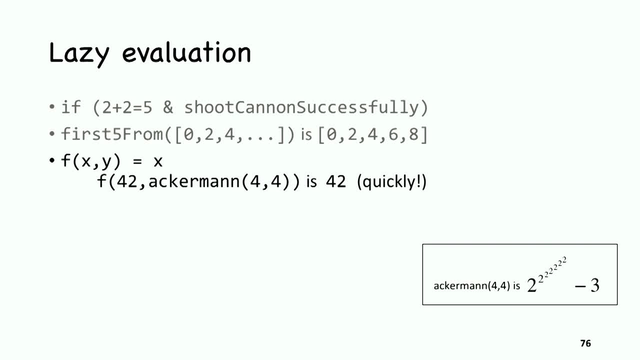 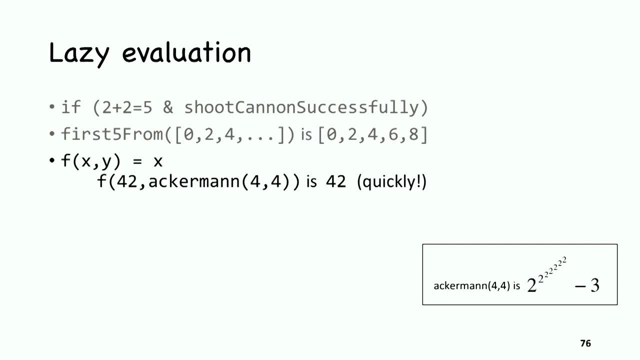 I think I got the number of 2's right. OK yeah, you have to subtract 3 after doing all those two exponents, But what you get there- the number in the box- is a number that's larger than the number. 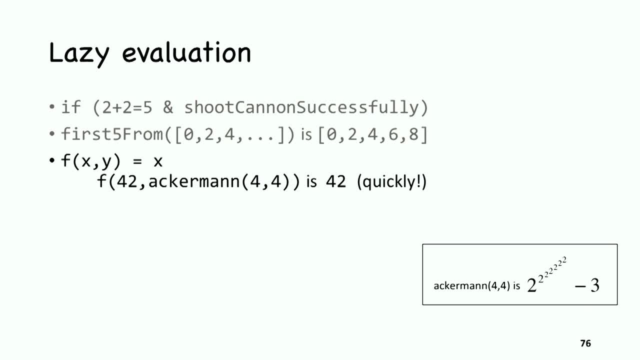 of atoms in the universe. So yeah, Ackermann 4, 4 is an extremely large number which takes an extremely long time to compute. What if I created a program where I said I'm going to compute Ackermann 4, 4?? 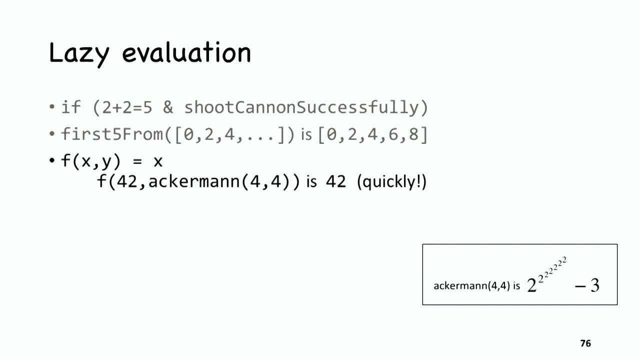 It would look as if the program were in an infinite loop, because it wouldn't stop running. Maybe if I left it going overnight? Nope, sorry, it takes longer than that. What if I left it going until I was 80 years old? 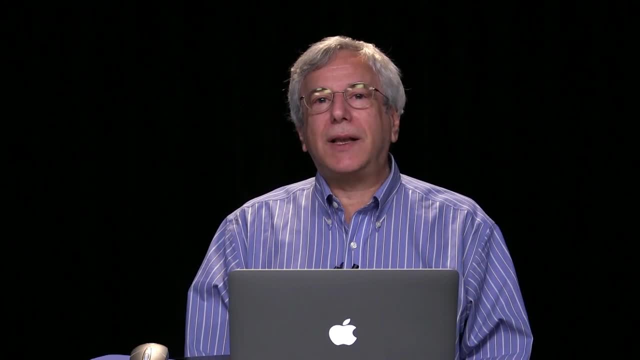 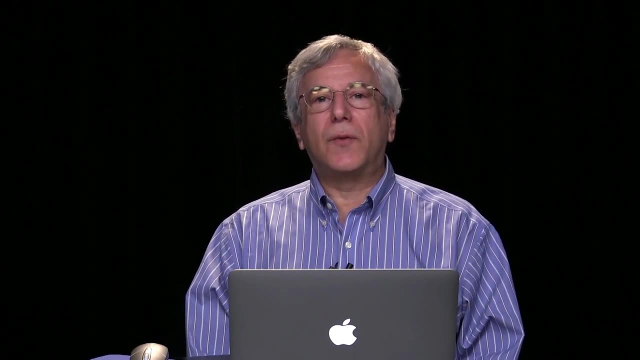 Nope, sorry, it would take longer than that. What if I left it going for a few generations? put it in a time capsule? Nope, sorry, the Ackermann function would still be running. So computing Ackermann 4, 4. 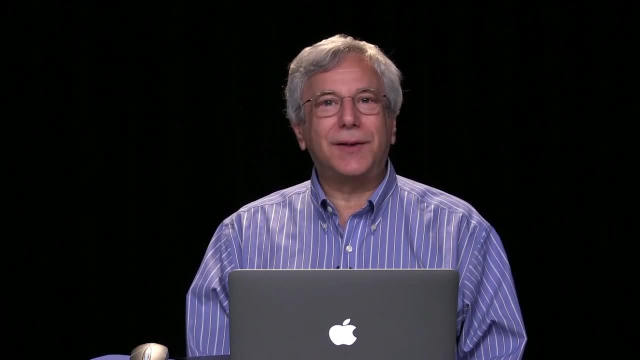 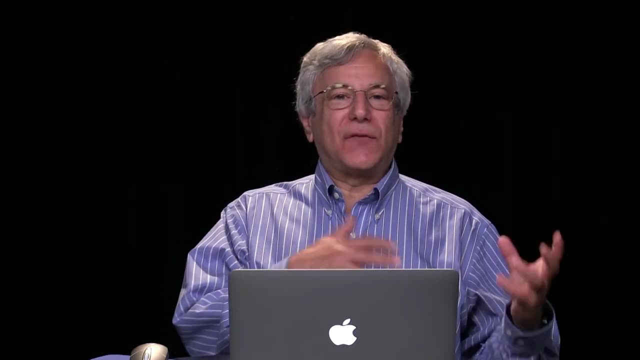 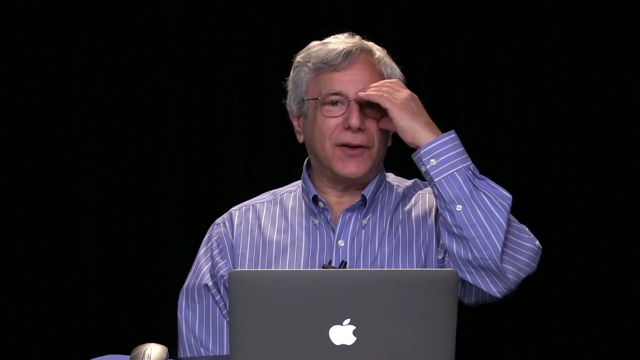 takes longer than you have to compute. But what if I have a function f of x- y that simply takes its first argument, x, and returns it? This is called a projection function. OK, and yes, we do use projection functions in many situations in computing. 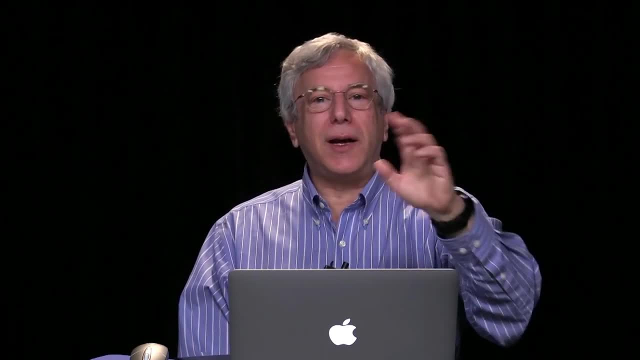 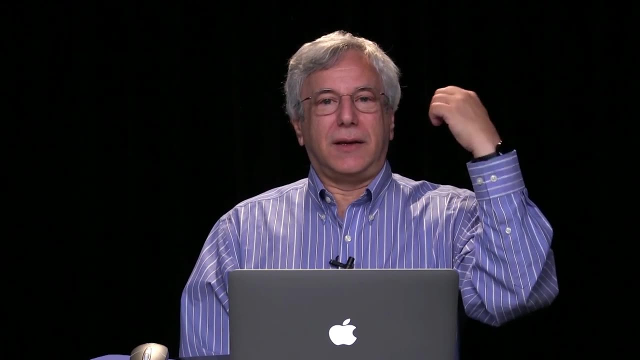 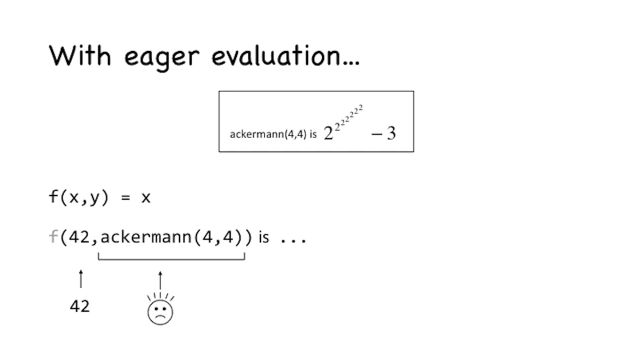 Anyway, I have a function f and it returns the value x. So let's say I try to compute f where the leftmost argument is 42 and the rightmost argument is Ackermann 4, 4.. What will happen If I try to do eager evaluation? 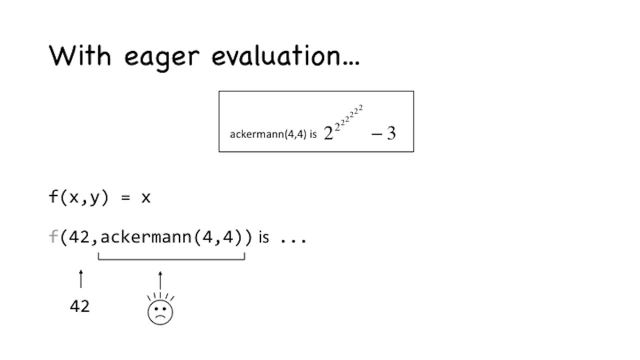 forget about it, It'll never happen. If I try to do eager evaluation, it'll try to find: well, 44 is 44, that's great, And Ackermann 4, 4, let's see. well, I'm being eager. 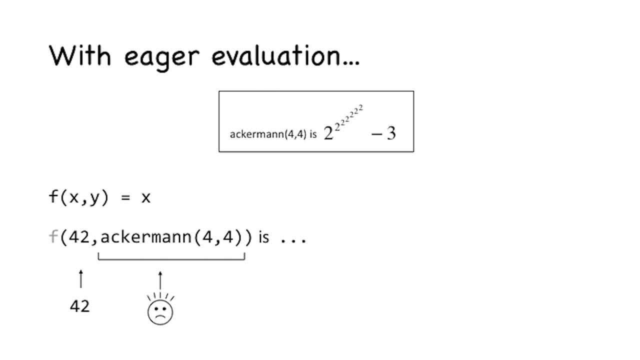 so I've got to figure out what that is. Well, months later, years later, decades later, hasn't finished computing. If I do lazy evaluation, which pure functions are good for? if I do lazy evaluation, then Ackermann 4, 4. 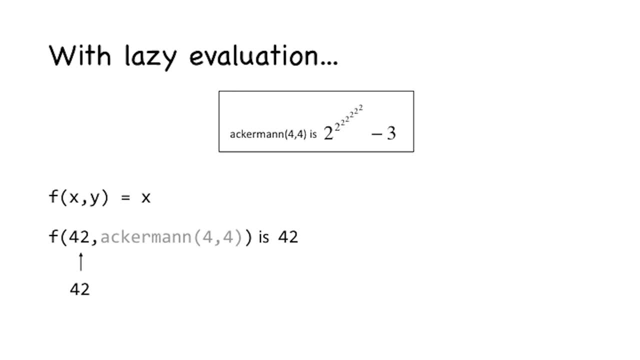 never gets computed, because it never needs to be computed. So it pops up with the number 42 and it does so very, very quickly. Oh, that's cool. One more benefit of lazy evaluation. I said that I don't particularly like ifs. 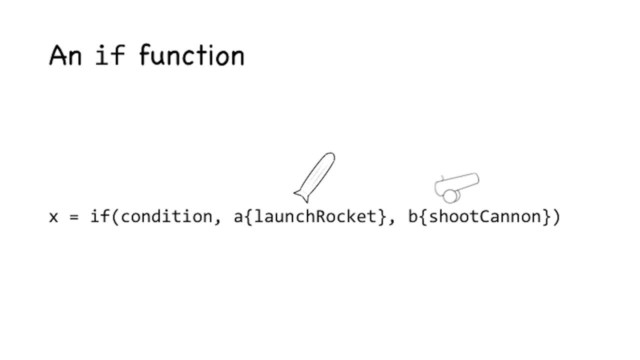 in the beginning of this course. Okay, maybe I want a function that takes three arguments. I'm going to call it an if function. You see these on spreadsheets. You see these in a lot of places. I'm going to start with a word: if. 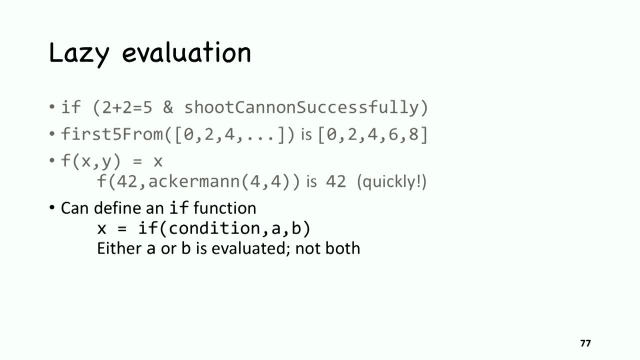 and then I'm going to have a condition and then I'm going to have an expression A and another expression B, And the idea here is that I'm going to evaluate the condition, see if it's true or false. If it's true, then I'm going to evaluate A. 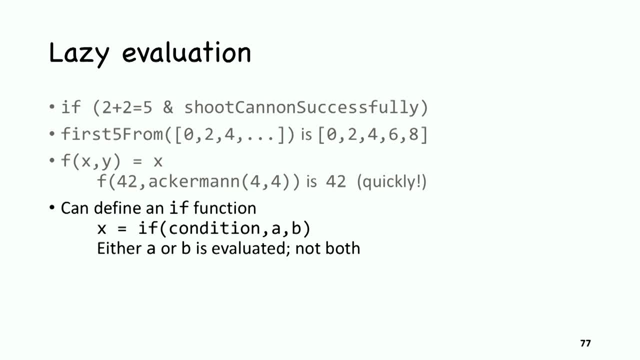 and return the result of having evaluated A. If the condition is false, then I'm going to evaluate B and return the result of having evaluated B. So I now have an if function, which I think is better than an if statement. I'm not jumping from one place to another, you see. 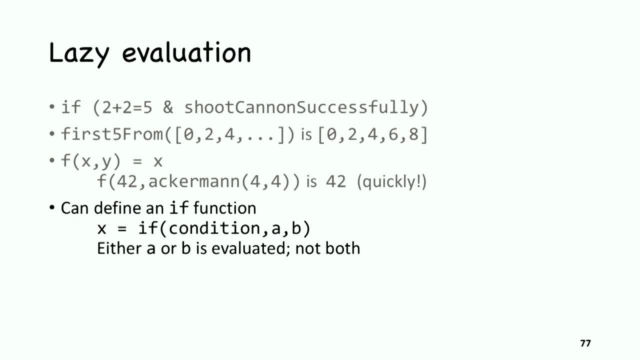 I'm just evaluating a function, And when I evaluate the function, I have the condition and I either get A or B. Now, where does lazy evaluation fit into this? Well, if I don't do lazy evaluation, that means I have to evaluate. 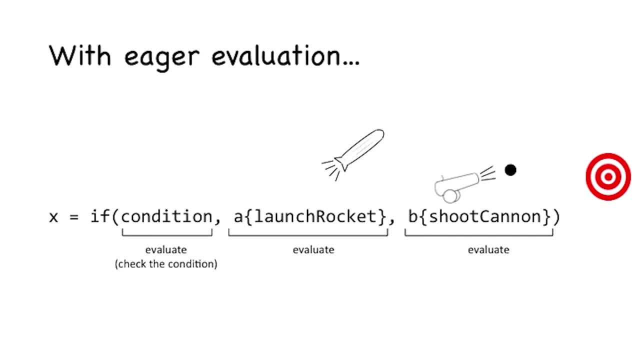 all three of the expressions inside the parameter list. That means I have to evaluate the condition, I have to evaluate A and I have to evaluate B. But wait, wait a minute. According to the rules of the if statement, I don't want to evaluate both A and B. 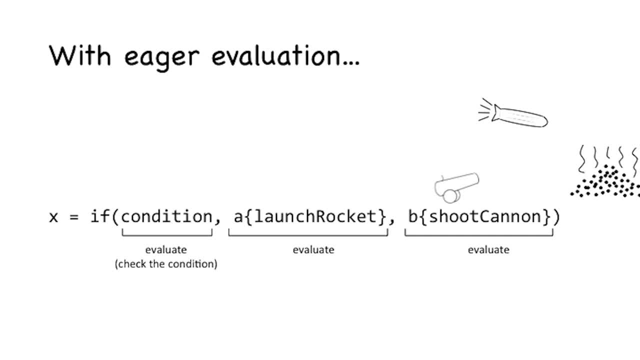 I want to evaluate A only in case the condition is true and B only in case the condition is false. So here lazy evaluation is essential. If the condition is true, I lazily evaluate A and then I ignore B. 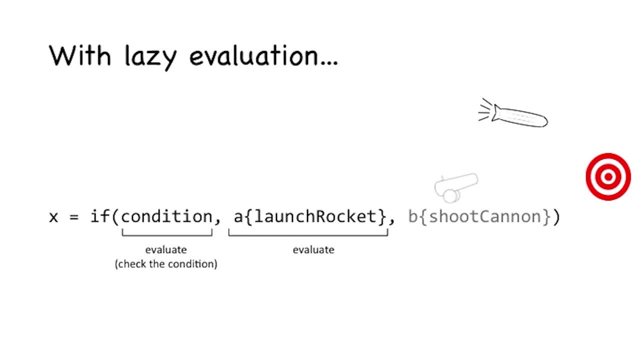 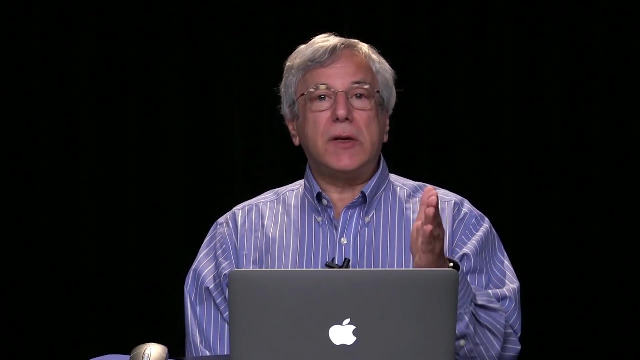 lazily ignore B. If the condition is false, then I evaluate B and I lazily ignore A. So this is a situation where I can have an if function, and the reason that I can have it is because I'm using lazy evaluation and not bothering to evaluate. 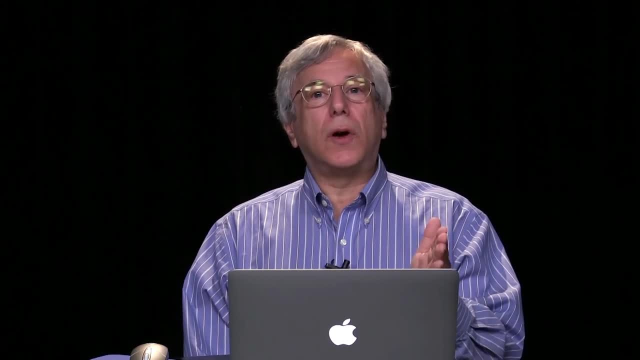 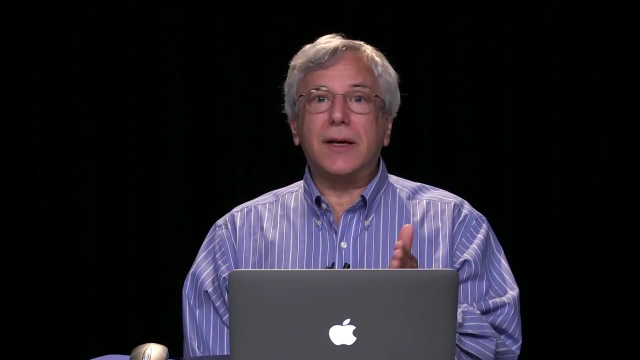 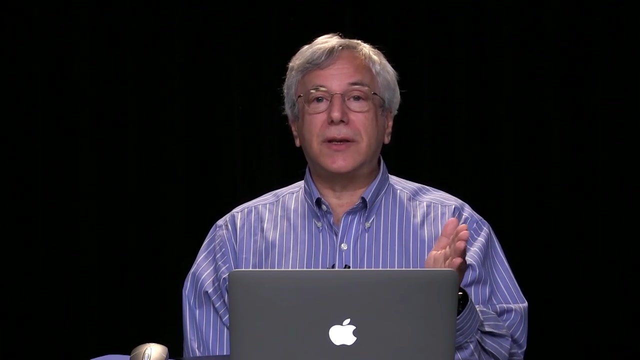 the expression A when I don't have to, or not bothering to evaluate the expression B when I don't have to. Hey, the sum story is: pure functions are nice, Pure functions. let us have lazy evaluation. Lazy evaluation is a good thing. 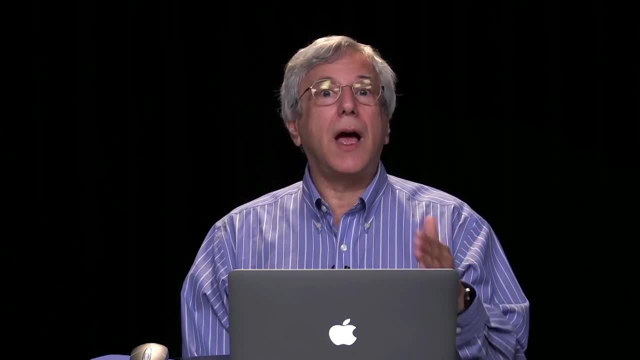 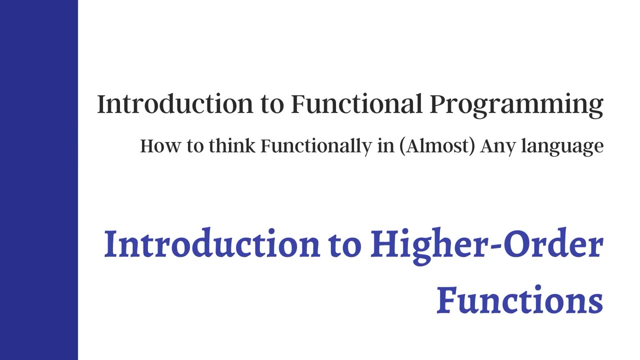 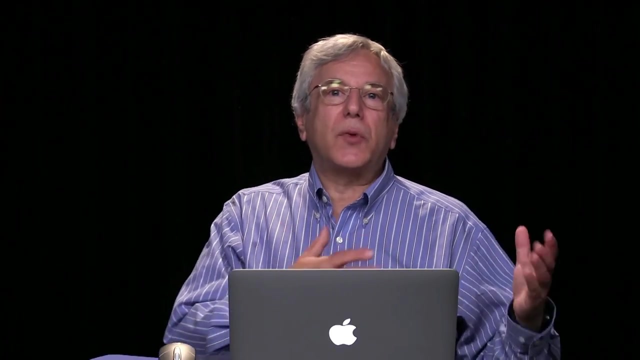 I said it in the beginning of this segment and I'm going to say it again: I like laziness. More course to come. This course is filled with terms to describe functions. In the previous segments I talked about pure functions. What could be better than something called? 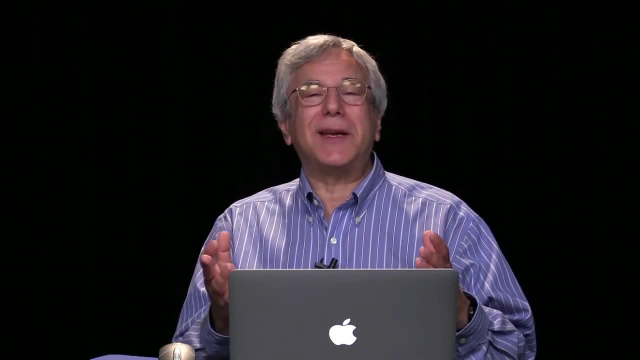 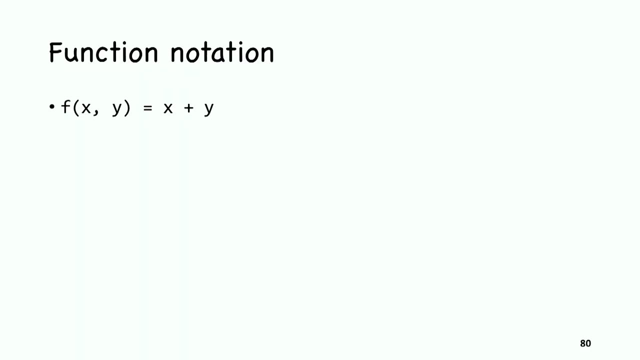 a pure function? Well, maybe something as lofty as a higher order function. So in this part of the course I want to tell you about higher order functions. Now let's just start with some notation Function. notation f of x- y equals something or other. 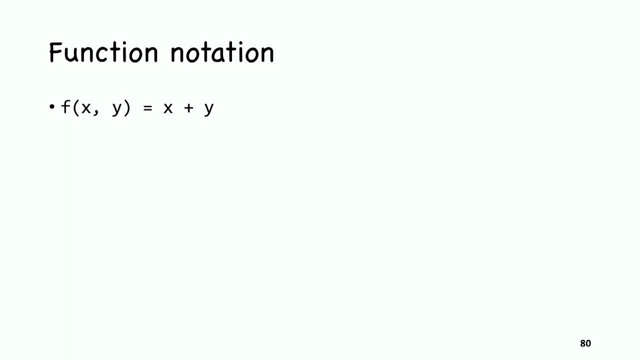 some expression. So I have f, I have parentheses, I have some parameters. The parameters are separated by commas. That's one bit of notation. I also have my lambda notation, but I'm not going to use that much in this part of the course. 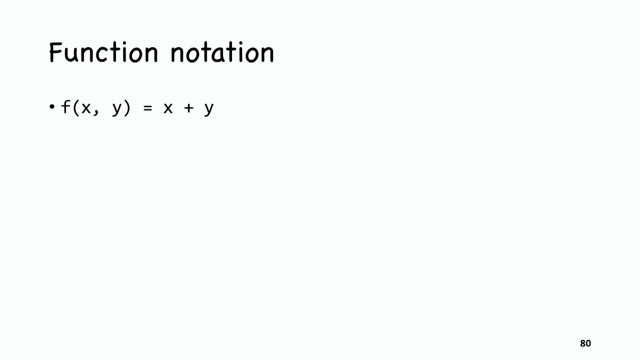 Okay, what about describing the kinds of parameters that this function takes and the kinds of result that it returns? For that, I'm going to have a slightly different notation, And the notation that I'm going to use is the name of the function. 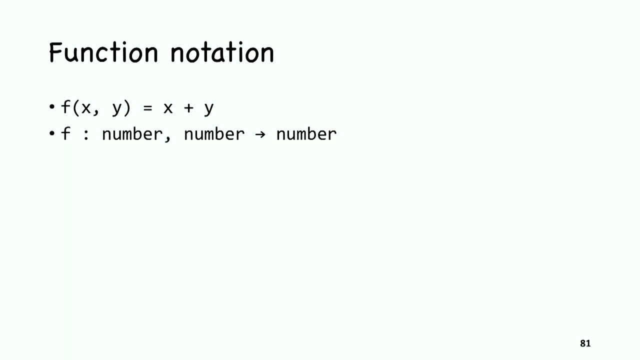 in this case f, a colon, and then the types of the parameters, separated by as many commas as I need. So in this case, number, comma number means that the x parameter is going to be a number and that the y parameter is going to be a number. 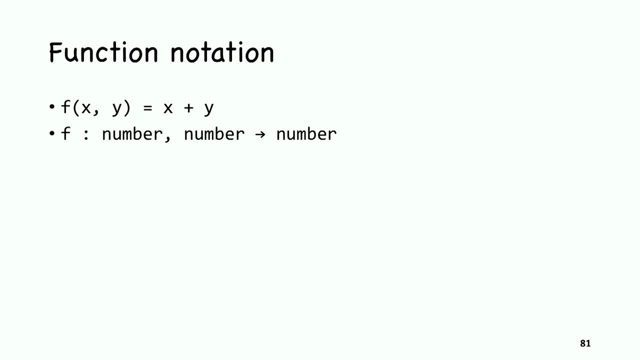 I could be more specific and say x has to be an int value, an integer value, or that x has to be a floating point value, but I'm not going to need that kind of heavy artillery in this part of the course. I'm then going to have an arrow. 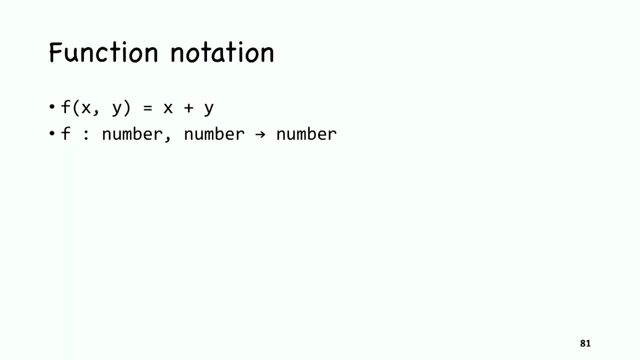 and after the arrow I'm going to say what's the result type of the function. So in this case, if I take x and y and they're both numbers and I add them together, then I get another number. So this notation is a way of my. 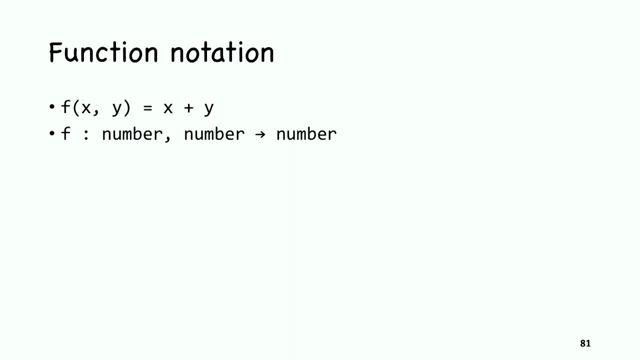 making sure that we all understand what types of things f takes as its parameter and what type of thing f returns as its result. And I want to do one more bit of I don't know- call it notation, maybe call it terminology. I want to make sure that we have a word. 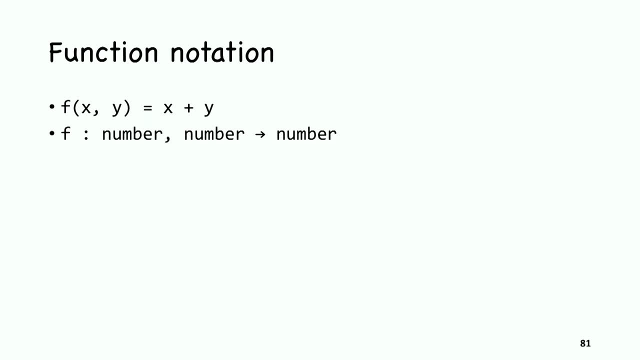 for what we're doing when we take the result of one function and apply it as parameter to another function. I haven't given that a name up until this point in the course, but it's called function composition. Let's take a look at two functions. 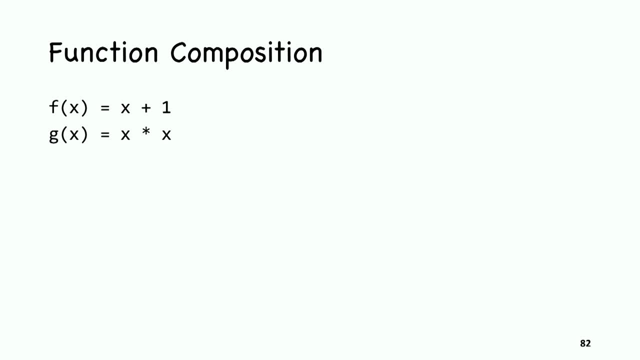 Again, I like to use these simple arithmetic functions because they're easier to understand than more complicated examples. So f is going to be a function that just adds one, and g is going to be a function that takes x and multiplies itself. f is increment, maybe, and g is square. 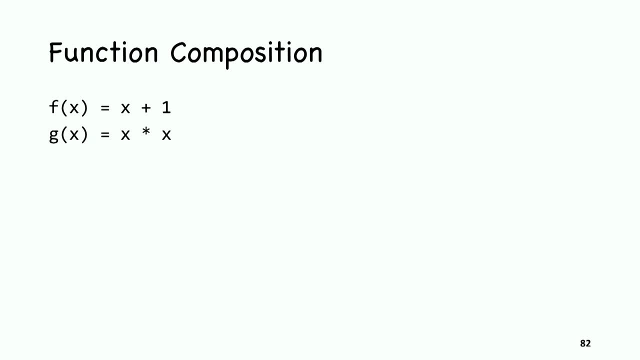 Well, what do I mean by function composition? When I compose two functions, I take the result of one and I apply it as a parameter to the next. I've been doing it all along in the course. I'm just giving it a name now. 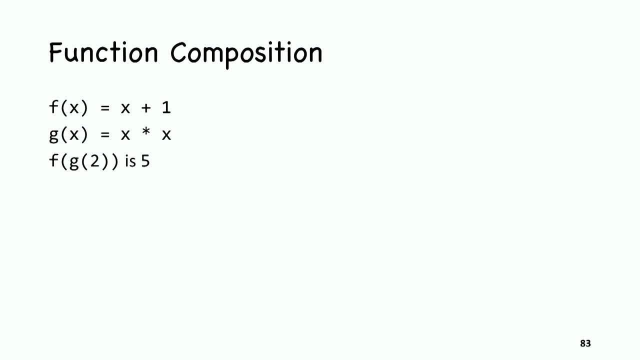 It's called function composition. So if I first apply g to the value 2, and I apply f to that result, I've composed the functions and I've gotten the number 5.. If you're not sure that you're supposed to get the number 5,, 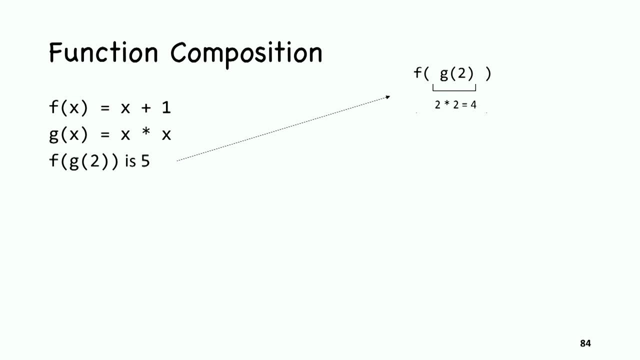 let's make sure that we do So. I apply g to 2.. When I apply g to 2,, I take 2 times 2, and I get 4.. And what happens when I apply f to the number 4?? 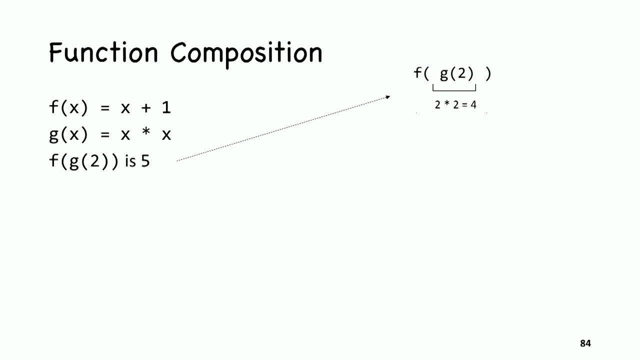 Well, the function f adds 1 to whatever you feed it, so that gives me 4 plus 1 is 5.. So that's function composition, And although I don't in this course need a special symbol for function composition, 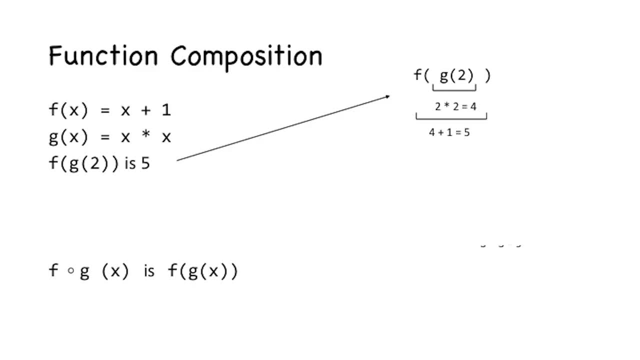 I'm going to have it in my back pocket, something that you should have in your back pocket. Mathematicians use the little circles. that's, I don't know, looks a little bit like an O. So if I write down f og f, circle g, 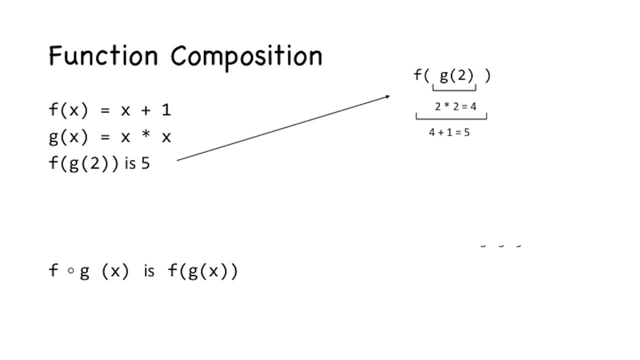 you can pronounce it fog, if you like- of x, then what I mean by that is f composed with g, which means apply g first and then take the result of applying g and apply it to f, And I can actually write down a formula. 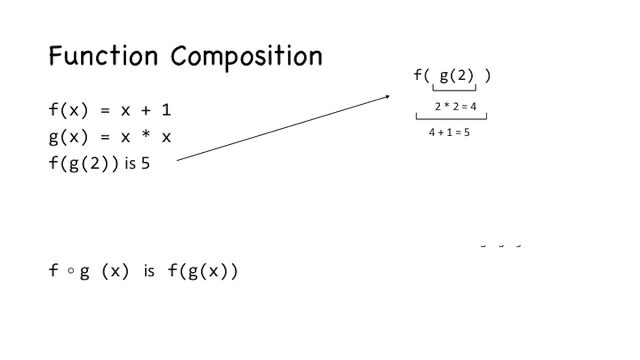 for the composition f? og. It's going to be well, what happens when I apply g, which is x times x, and then after that I add 1 to it. So the formula for f? og is x times x plus 1.. 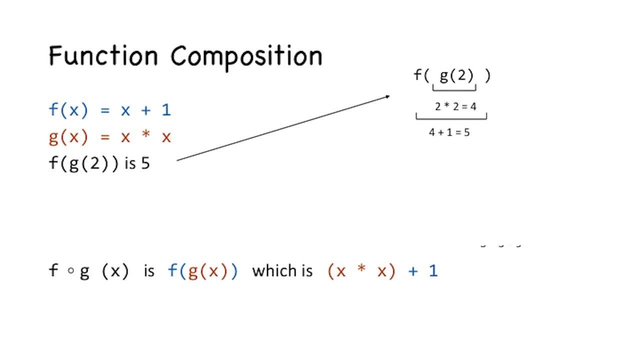 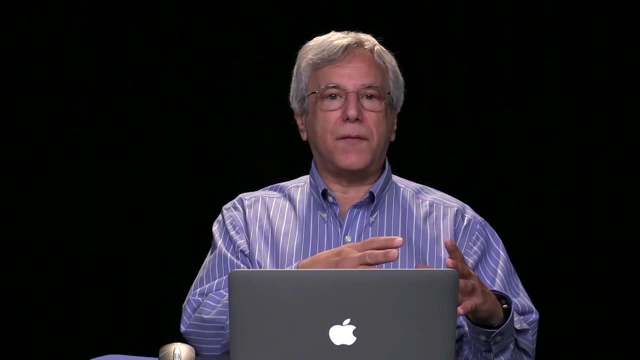 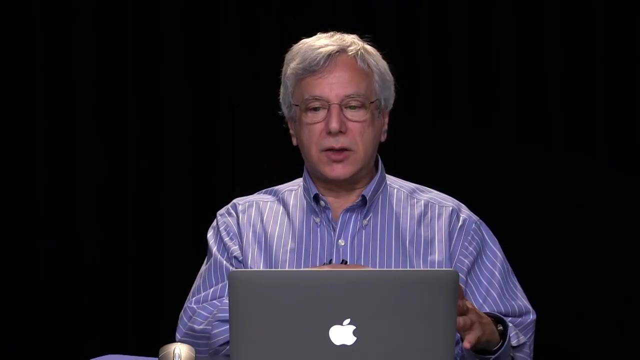 Okay Now function composition isn't commutative. That is to say, if I apply g first and then apply f, that's not necessarily the same as applying f first and then applying g. So on the next slide, what I've done is shown you what happens. 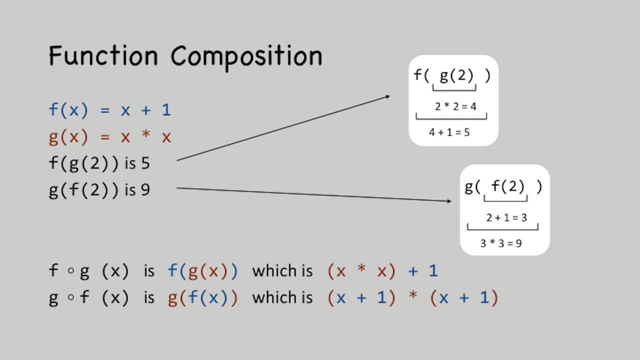 when, instead of applying g first, I apply f first. Let's take a look: If I apply g to 2 and then apply f to it, I get 5.. That's what happened on the previous slide. On this slide, if I apply f first to 2,. 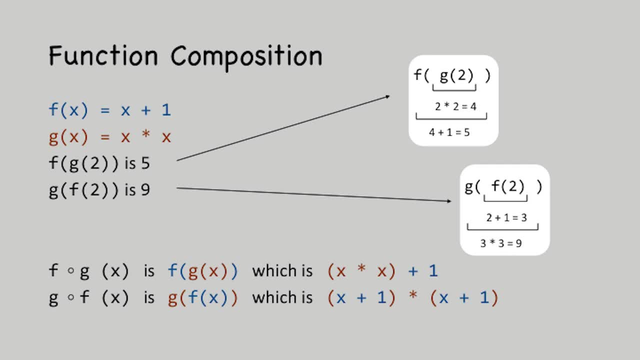 well, that's like adding 1 to 2, so I get 3.. And then if after that I apply g to the result, well, I get 3 times 3 is 9.. So composing with g first and then f gives me 5. 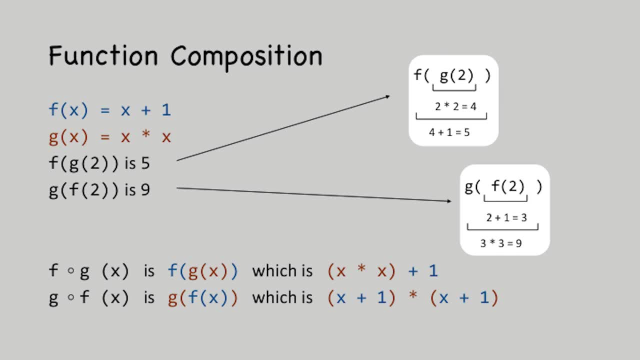 when I apply it to 2.. Composing with f first and then g when I apply it to 2, gives me a different result: 9.. It's just one of those features about function composition that you might need to be careful of down the line. 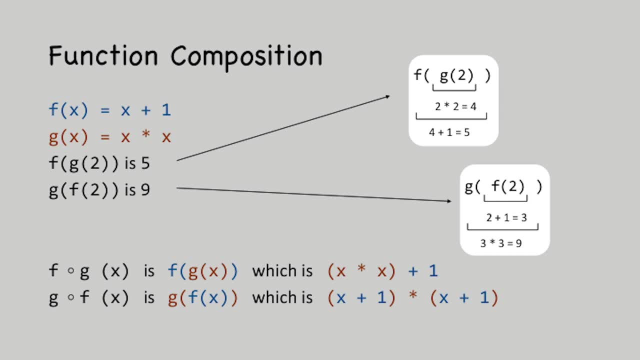 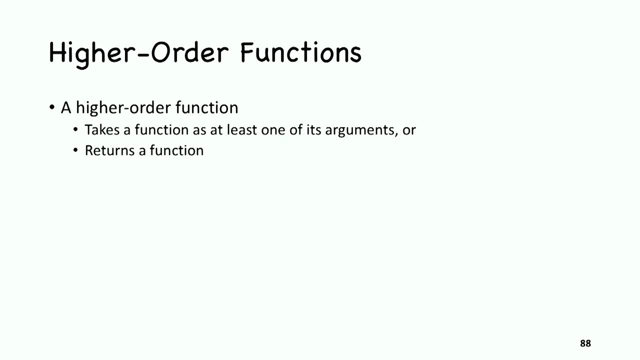 Okay, We've got some notation and some terminology behind us. Let's take a look at higher-order functions. A higher-order function takes a function as at least one of its arguments or returns a function as a result, or possibly both, So a function that's a higher-order function. 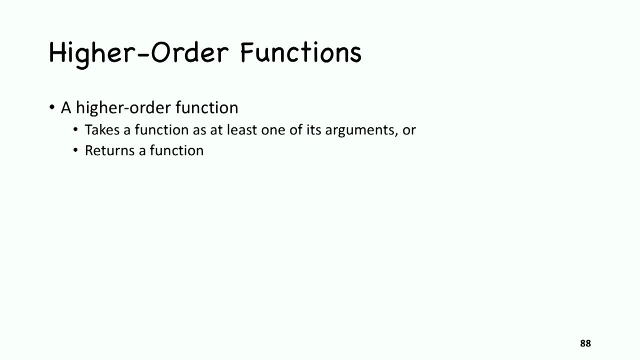 deals with other functions, perhaps other functions, maybe even deals with itself as a function, But somehow a higher-order function involves the use of a function as either its parameters or its return type. And the mantra that you use, that you'll hear over and over again. 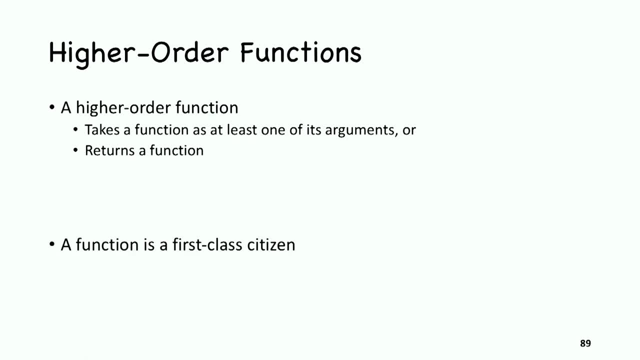 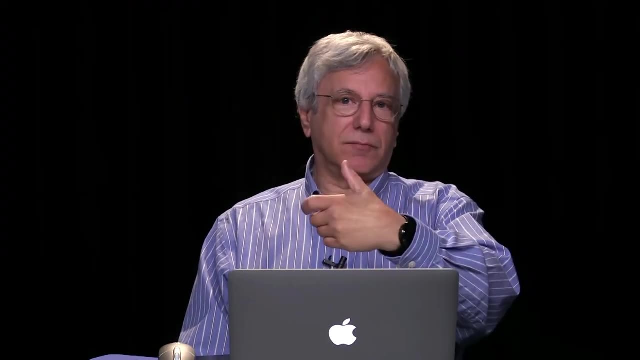 when people are talking about functional programming, is a function should be a first-class citizen. Hey, I can take a number like 2 and use it as an argument to a function. Well, that means 2 is first-class. I can take it and I can use it as a parameter. 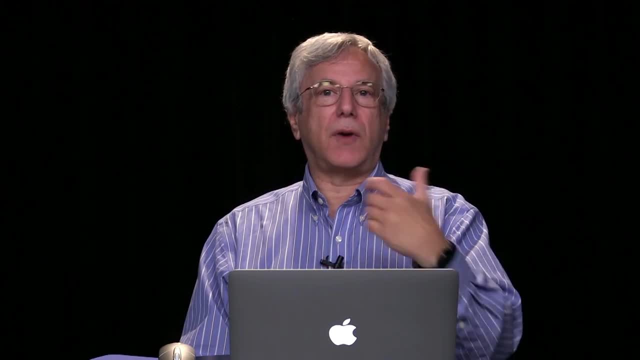 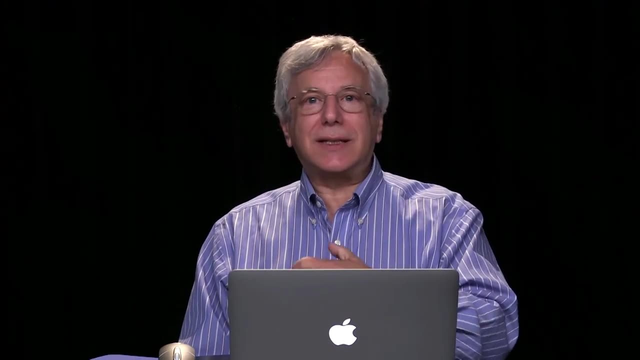 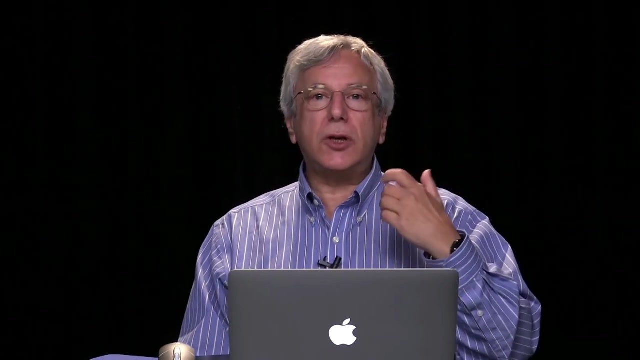 Well, what about a function? Can I use that as a parameter to another function? If I consider a function to have first-class citizen status, to have all the rights that any other entity in my language has, then if I can take 2, 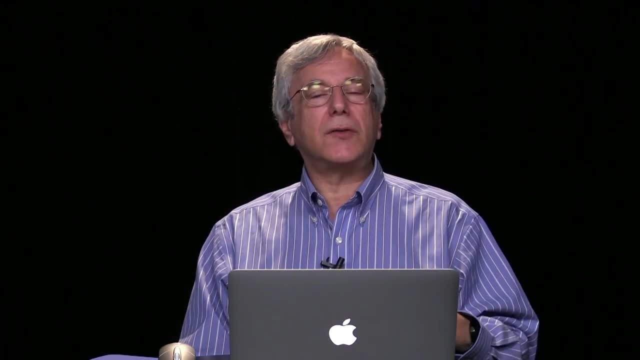 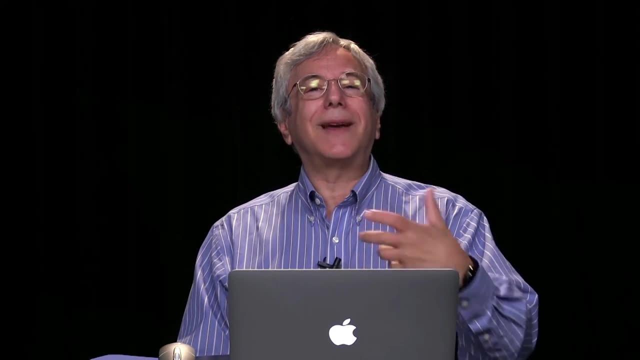 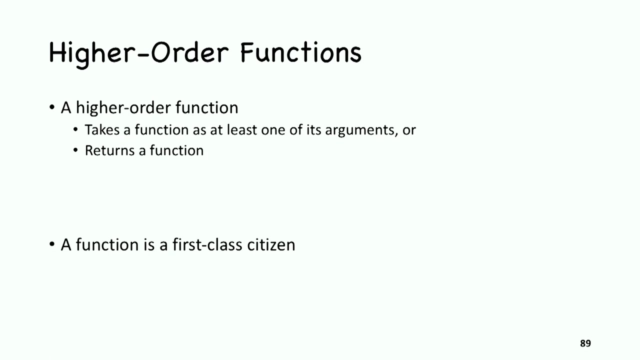 and plug it in as a parameter to a function. then I can also take some other function, a first-class citizen with all the rights and responsibilities thereof- and plug that into a function. So now I'm going to consider as my arguments not only numbers like 2. 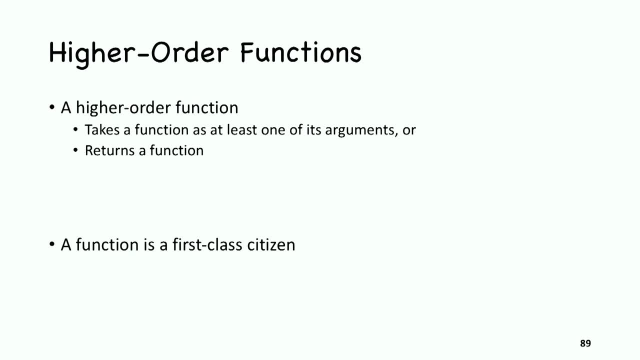 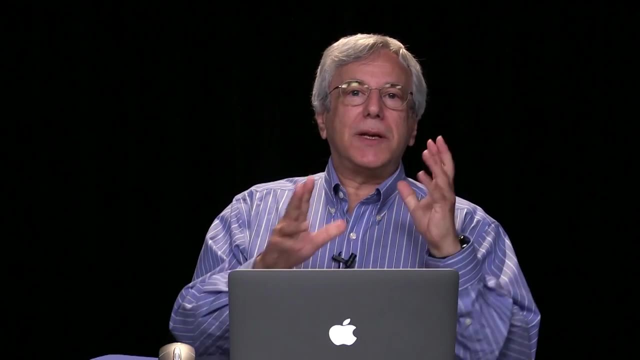 and values like amount or values like person, but I'm also going to be able to plug functions in as arguments and return functions as results. Is this a new concept for us? Not really. We've been dealing with it, we just haven't made a big deal out of it. 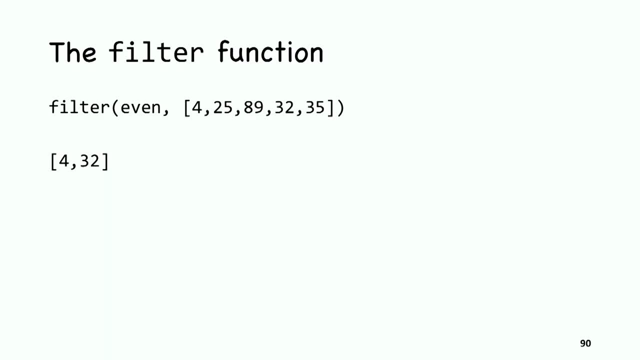 Let's take a look. In an earlier part of the course I talked about a filter function. In my first example I said filter takes two parameters. One of them is what I guess I called a condition or a criterion, that of being even. 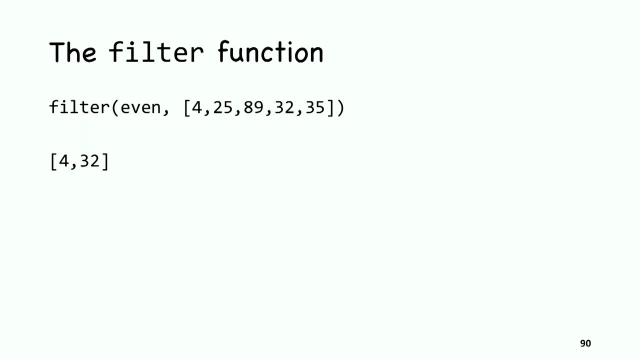 And the second parameter to the filter function is a list In the slide. that list is 4,, 25,, 89,, 32,, 35. And when I apply the filter function to those two arguments, I get back a new list. 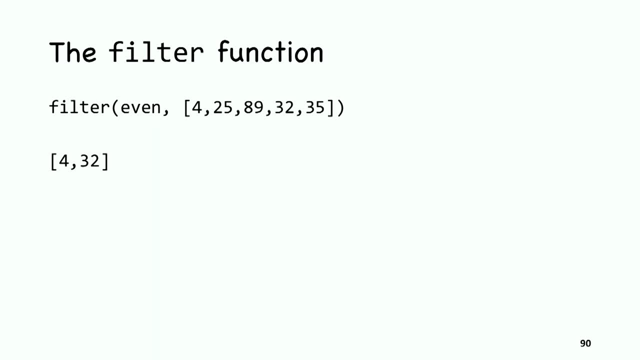 In this case, 4, 32.. Well, I called even a condition, but let's be careful here. What really is even. Even is a function that takes a number and returns true or false. Even takes the number 4 and returns true. 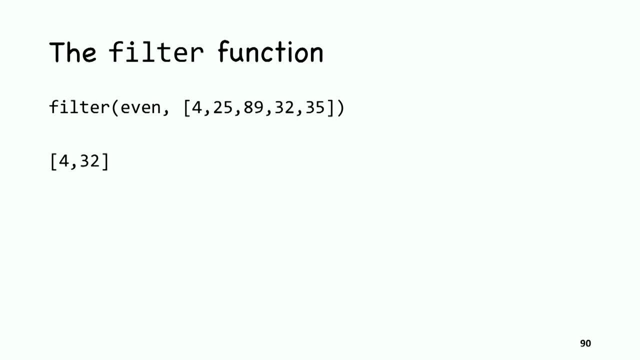 because 4 is even Even, takes the number 25 as its argument and returns false because 25 isn't even. So even is really a function, and that means that the filter function takes two arguments, the first of which is a function. 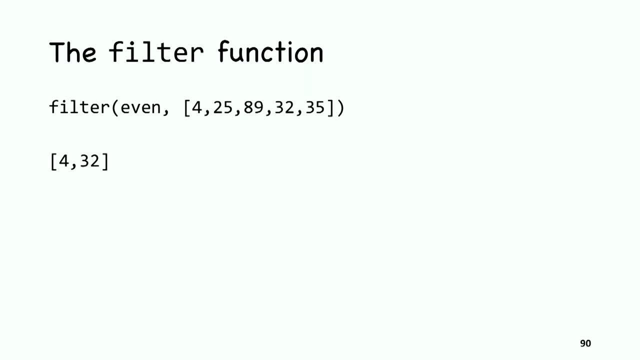 and the second of which is a list. I'm going to notate that this way, Filter is a function which takes as its first argument a function and as its second argument a list, and returns a list. Filter is a higher order function. 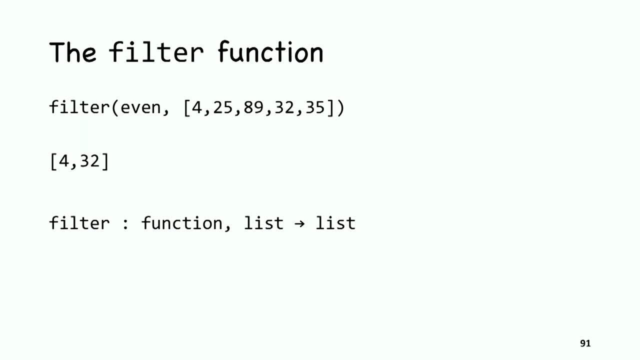 It takes a function as one of its parameters. Let's look at another example, Again an example that you saw earlier on in the course: The map function. If the map function takes add one as its first argument and the list 4,, 25,, 89,, 32,, 35 as its second argument, 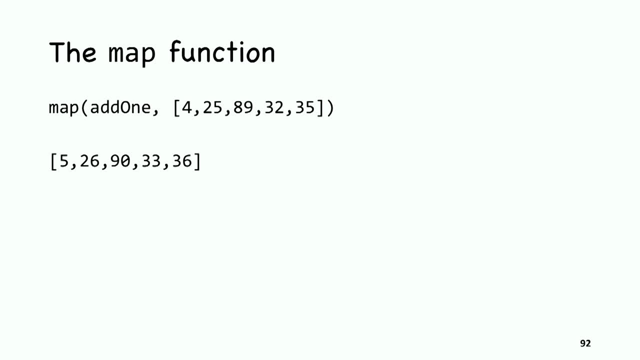 then it returns, as its result, the list 5,, 26,, 90,, 33, 36.. You take all the numbers in the list and you add one to each number. You apply the add one function to each of the elements in the list. 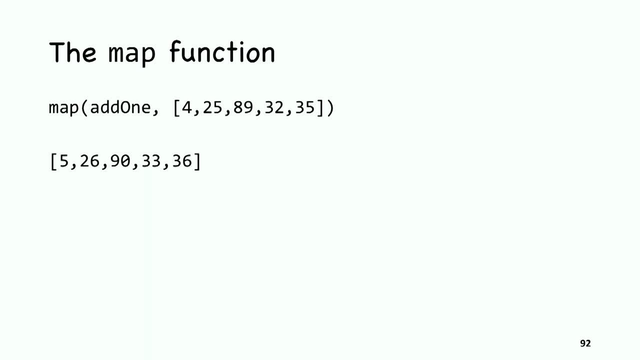 So add one is the first argument, That's a function. The list 4,, 25, and so on is the second argument. Well, that's a list. So again we have a higher order function. The map function takes two arguments. 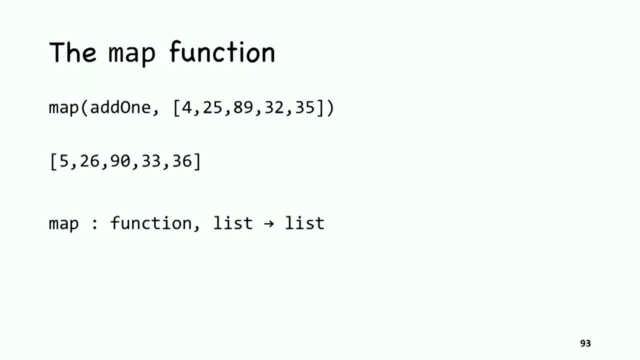 the first of which is a function, the second of which is a list, And it returns a list as its result. Now we're not going to stop with filter and map. We also saw some fold functions. We saw fold from left and fold from right. 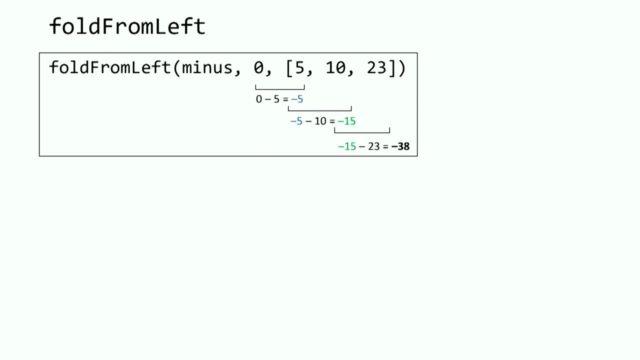 And if we're not worried about minus, if we're doing plus, it doesn't matter which we use. Okay, One way or another. what fold does is it takes an initial value such as zero, and applies the minus function to zero and to an element in the list. 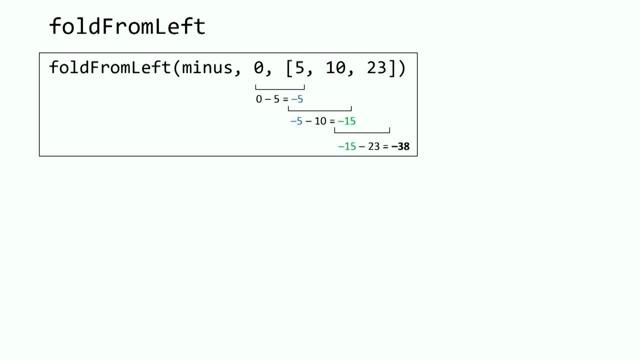 So in this case, you're reminded that it subtracted 5 from zero, then it subtracted 10 from the result, and so on and so forth. But look, The first of the three arguments to the fold from left, function is minus. 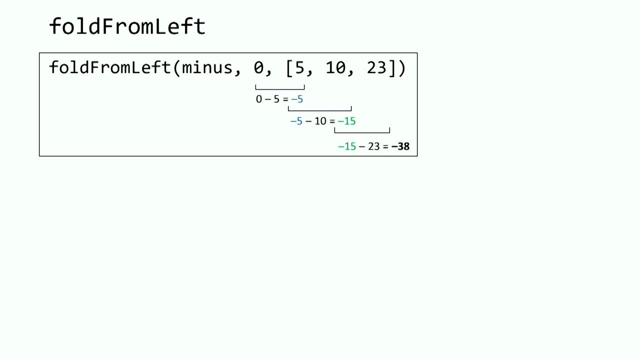 That's a function. It takes two numbers and returns another number. So the signature for the fold from left function is: it takes three arguments: The first is a function, The second is a value And the third is a list And it returns a value as its result. 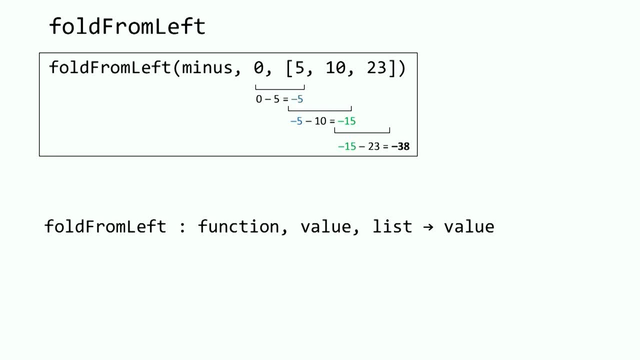 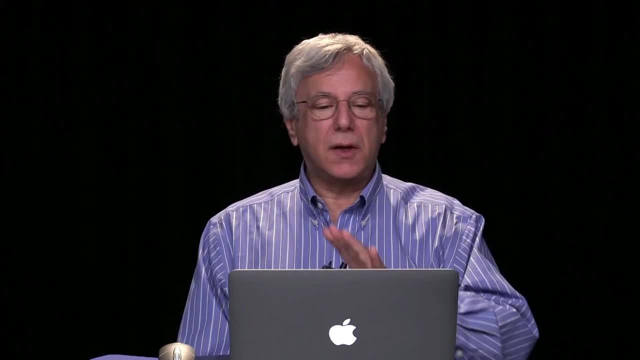 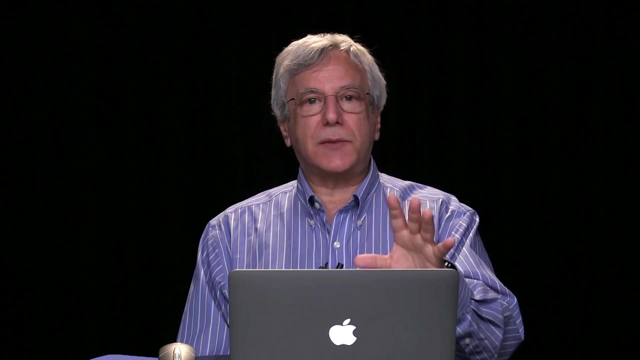 Okay, So in this segment we've seen three higher-order functions, three functions that came from earlier in the course, but now we called them higher-order functions and brought to your attention the fact that they take functions as parameters. What we want to do now. 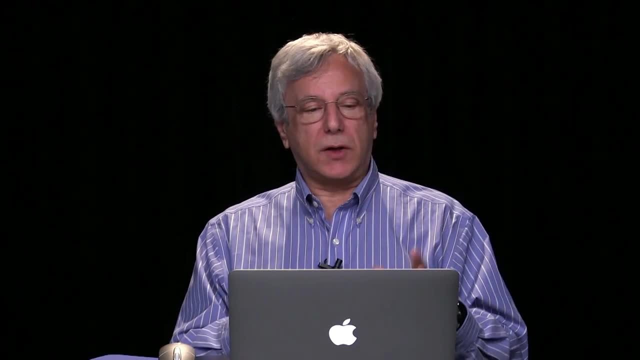 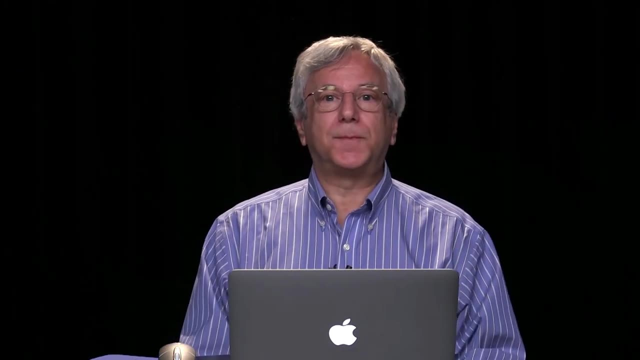 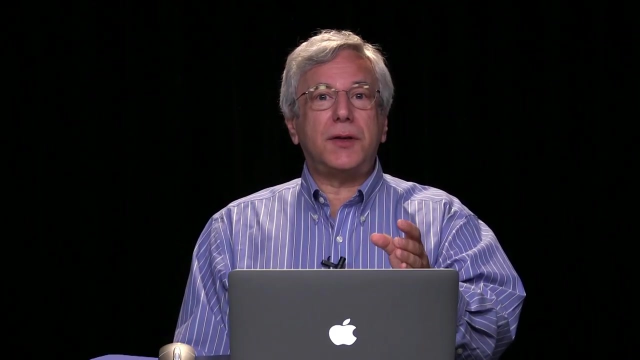 is find out what we can do with higher-order functions. I want to show you some functions that return functions as results. That's all coming up in the next few segments. Sometimes you have a function and you want to apply it several times with a default argument. 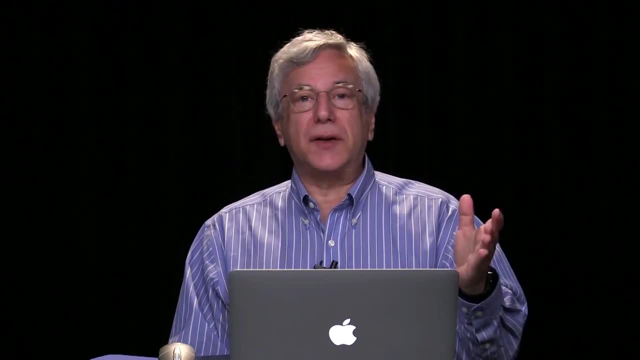 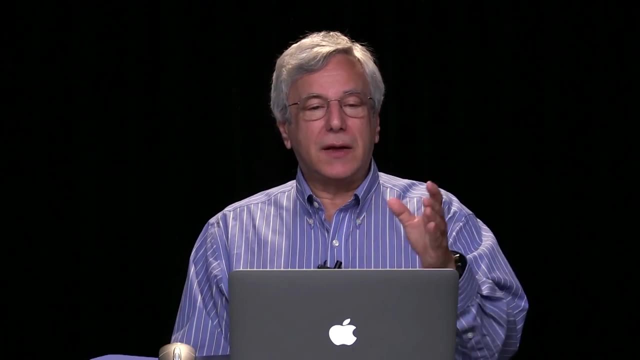 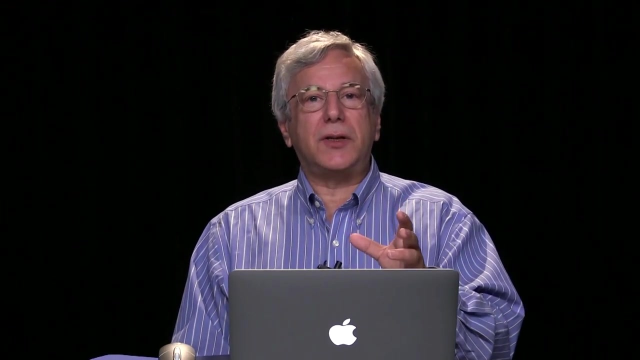 Sometimes a language library supplies another function that already has a default argument for you, but sometimes you want to make your own function with a default argument. Well, in this segment you'll see a couple different ways to do that. One of them is called partial application. 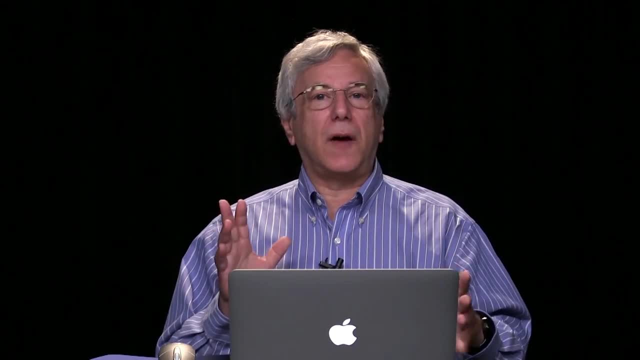 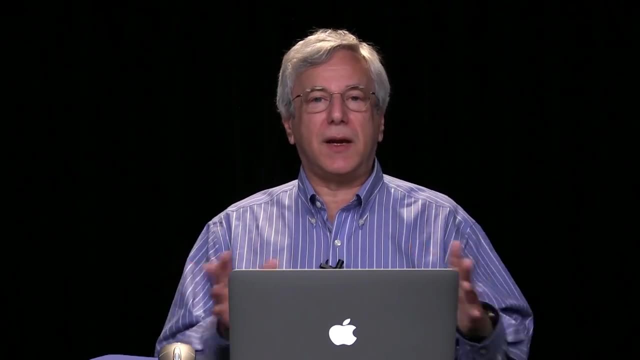 The other is called currying. Partial application and currying are very close cousins of one another. In fact, some authors use both names to mean the same thing. They are in fact slightly different, but I'm going to show you the two. 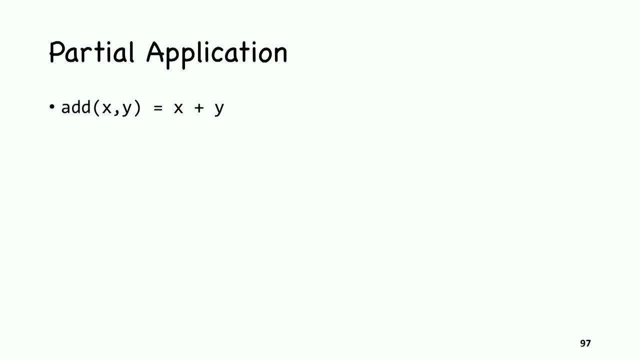 and whether you see the difference or not is not terribly important. yet Let's just take a look at the slide. I have a function called add and the function- Oh, I guess it's my favorite function- for examples- It adds two numbers, x and y. 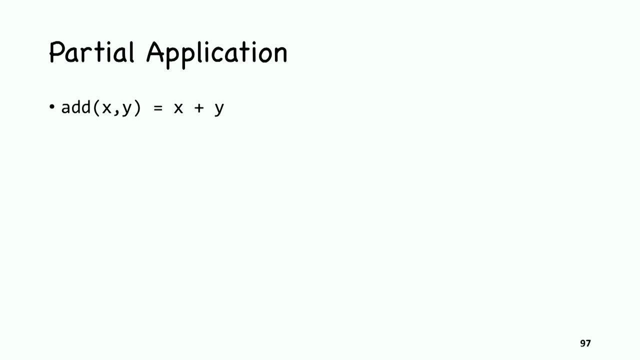 Now let's say that I want to always have 2 as the first argument. What am I going to do? I'm going to create another function called add2.. And what add2 is? well, it's kind of like the add function. 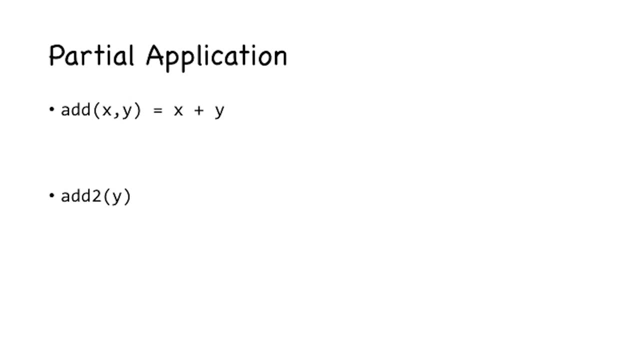 but it always takes a 2 and adds it to whatever one argument you feed to the add2 function. Well, thinking about this in terms of partial application, you can think of the add2 function as being the same as the add function when you've partially applied the value 2.. 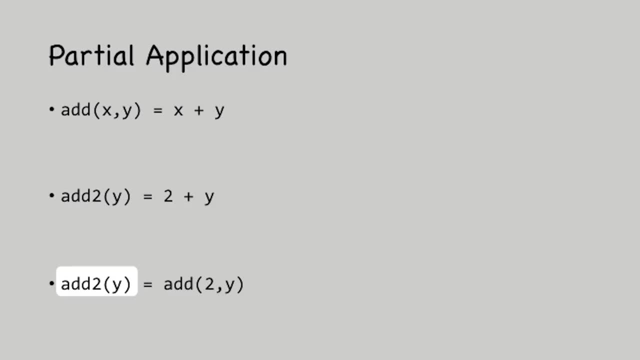 So add2 is the same as add, where the x is given sort of semi-permanently the value 2.. Partial application means you partially apply the function by supplying one of the arguments, but not necessarily the remaining arguments. It's not terribly deep. 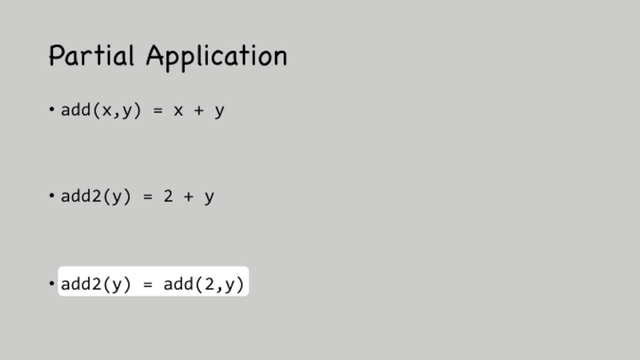 It's an okay concept. Let's see another example of partial application. I start with a function that I'm going to call anyline, And the anyline function takes three parameters: an, m, an x and a b parameter, And I'm not calling them x, y, z. 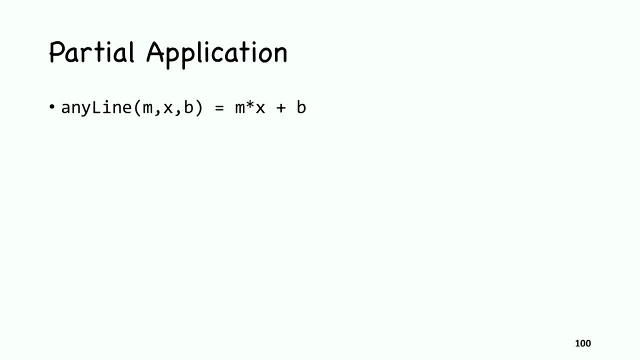 because lines are sort of familiar things. The formula for a straight line in algebra is m, x plus b, So I'm respecting that tradition and using the letters m, x and b in this example. Now, what does a real honest-to-God line look like? 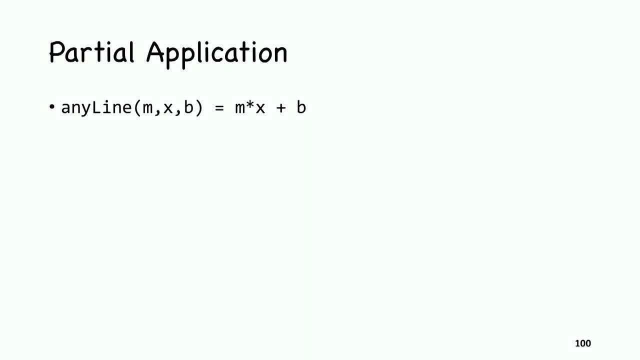 Well, a real, honest-to-God straight line has a value that's fixed for m and a value that's fixed for b. So anyline is just well: m, x and b, multiply them and then add the b. But myline has a fixed value for m. 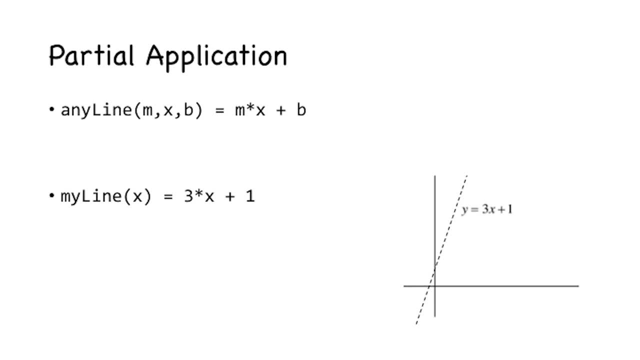 and a fixed value for b. Myline is one where m is sort of permanently set to 3 and b is permanently set to 1.. I want to partially apply the anyline function by supplying a value for m and a value for b. 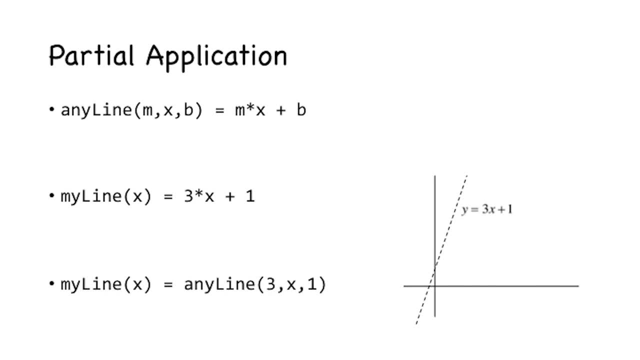 And I could do that by thinking of myline as being what I get when I call anyline, by partially applying it and saying: oh, m is definitely going to be 3 and y or b is definitely going to be 1.. 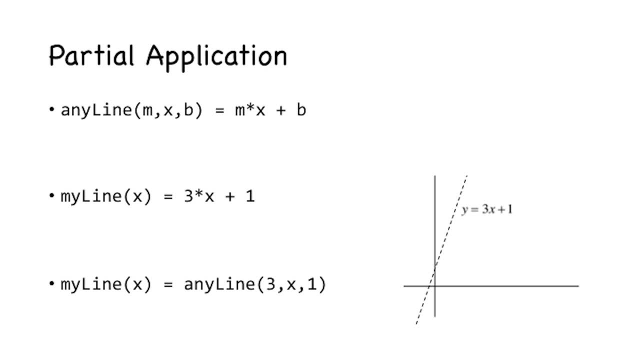 So that's partial application, The notion that you're supplying default values which you're going to kind of carry along every time you call the myline function OK. Now, functional programmers have another way of looking at this, And the other way of looking at it is almost the same. 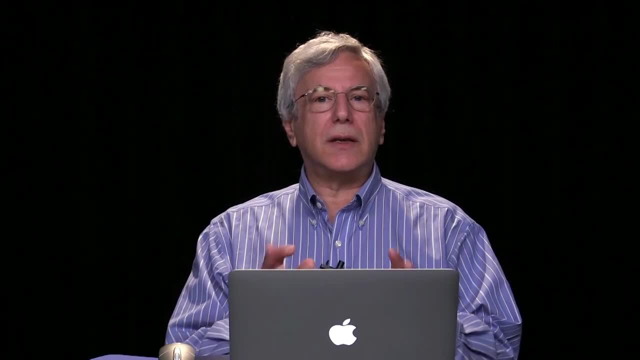 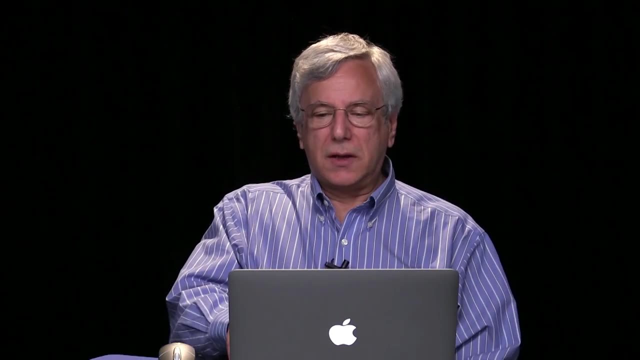 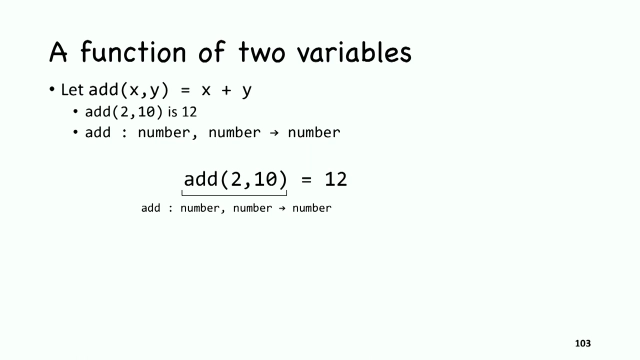 It's just a slightly different take on it so that we can think of it in terms of functions that act on other functions that act on other functions. Let's have a look. I'm going to start again with my function of two variables called add. 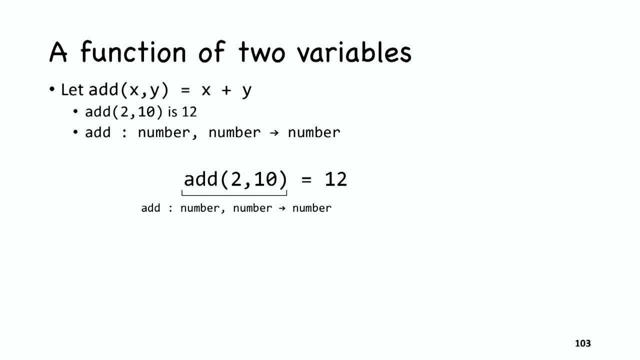 And add is going to take 2 and 10 and give me 12.. So add is a function, not a higher order function. It takes a number and another number and gives you a number back, And I see that I have that written twice on this slide. 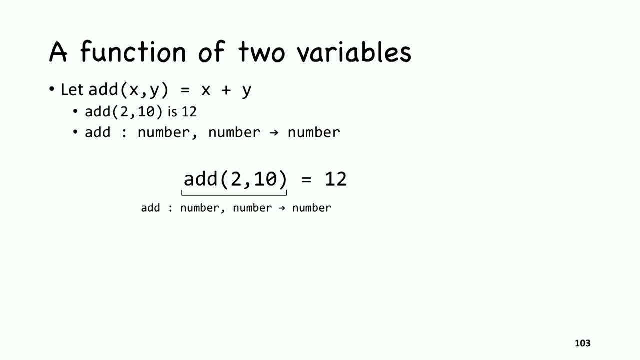 That's good. OK, I want to bring to your attention something that's called currying. The word curry doesn't come from the food substance. It comes from a person's name, the person who developed this technique. That person's name was Haskell Curry. 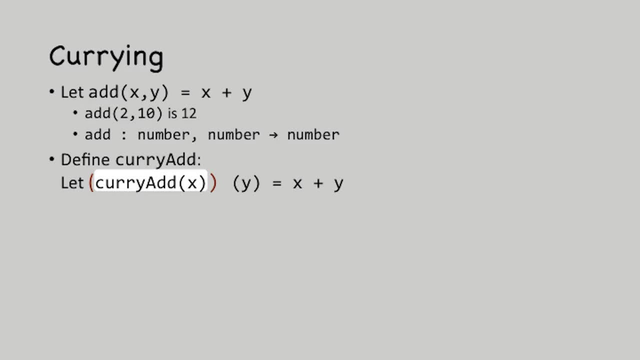 So let's curry the function add. And when we curry the function add, what we're going to do is I'm going to create a brand new function And I'm going to call it curry add And curry add instead of being a function. 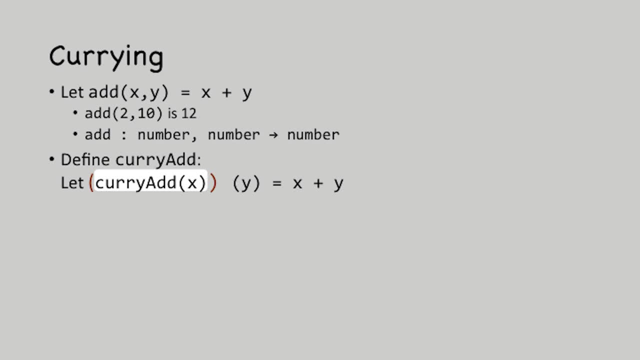 of two variables is going to be like that add function, But it's only going to take one variable x, namely the leftmost variable x, the first parameter. OK, So curry add is a brand new function. It's like the add function. 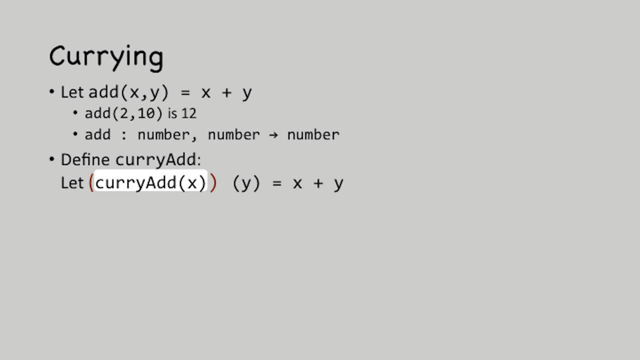 except instead of taking both variables x and y, it takes only the variable x. And now curry add: the thing in red parentheses is a new thing to which I can apply the second parameter, And when I apply that second parameter, I get x plus y. 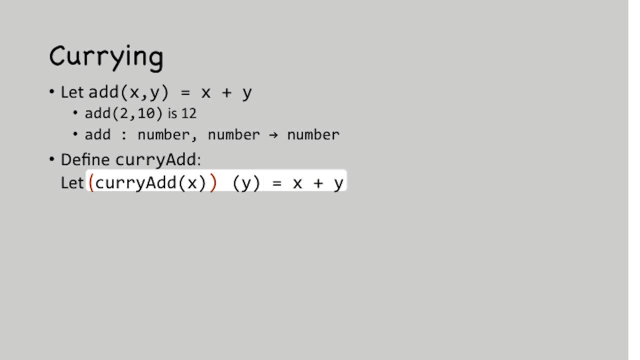 OK, So it's kind of like partial application. only, I'm going to be very, very careful now with the types of things that I get. Let me make sure that you understand what we're doing here If I call add on 2 and 10,. 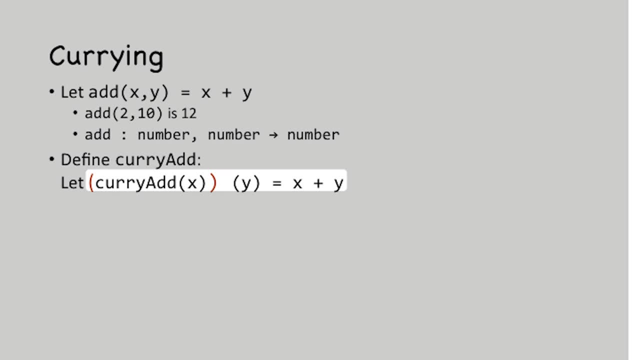 I get 2 and 10.. I get 12.. Well, if I first create curry add of 2, and then I apply that to 10,, yeah, I get 12.. The answers that I'm going to get aren't going to change. 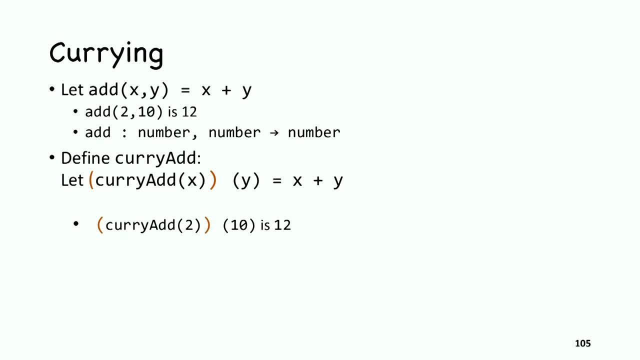 It's just the way that I think about my functions is going to change a bit. So, taking curry, add 2, that's a brand new thing. I can apply it to 10, and I can get 12.. I can apply it to 55,. 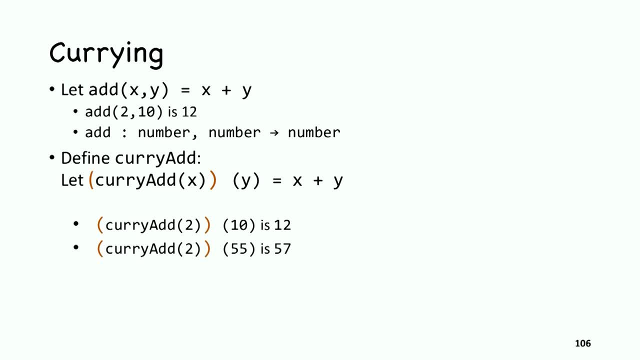 and get 57.. It's just going to add 2. And I can apply it to minus 3, and get minus 1.. OK, The thing to notice here is that that thing in red parentheses, curry add 2, is now a thing. 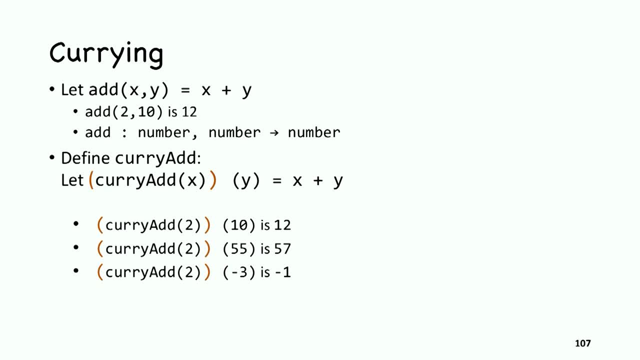 It's something to which I can apply a number like minus 3, or 55, or 10.. I can even give it a name. I can say that add 2 of y is like taking curry add of 2, and applying it to y. 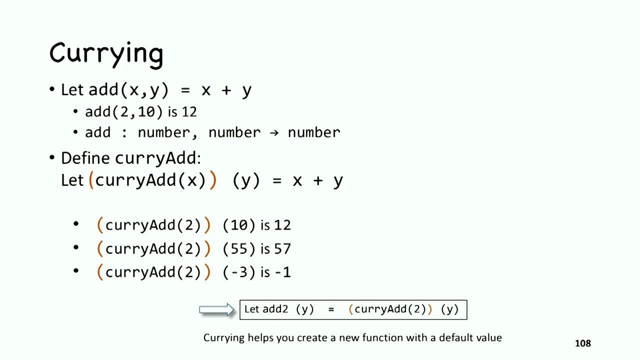 Currying then helps me create a new function with a default value from an older function. OK, Here's the punchline. What kind of a thing is this? curry add 2?? That's the question. What kind of a thing is curry add 2?? 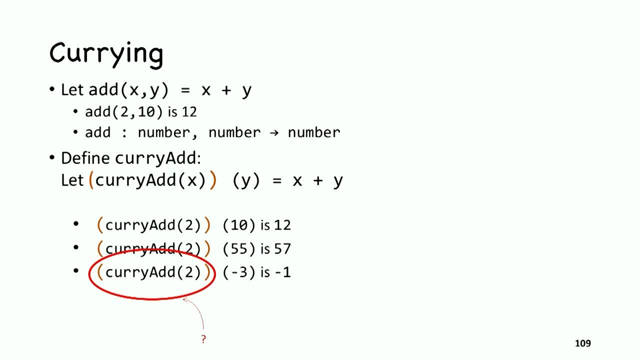 Well, let's take a look. Curry add 2 is a function and I can apply a number to it- a number like minus 3, and I get back a number, a number like minus 1.. OK, That's what curry add 2 is. 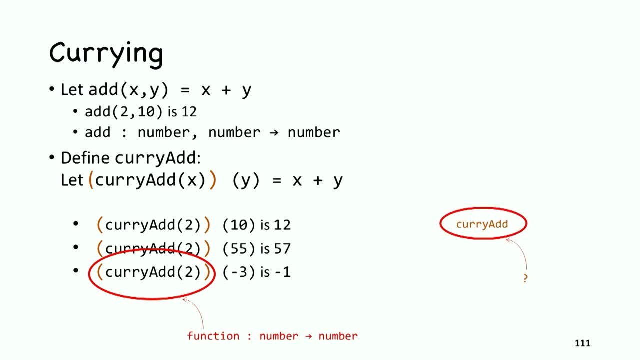 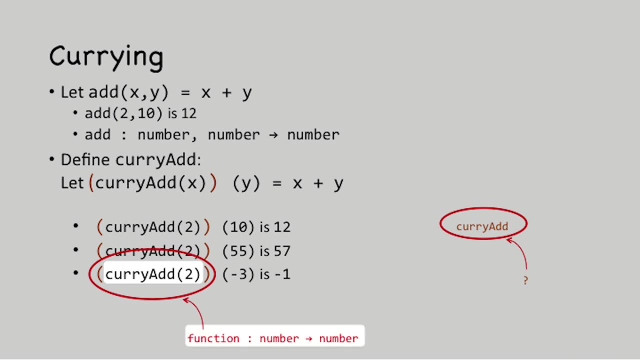 But what does that mean? What kind of a thing is curry add alone? Curry add is something that I can apply 2 to and get this brand new function. OK, Curry add is something that I can apply 2 to and get the function. 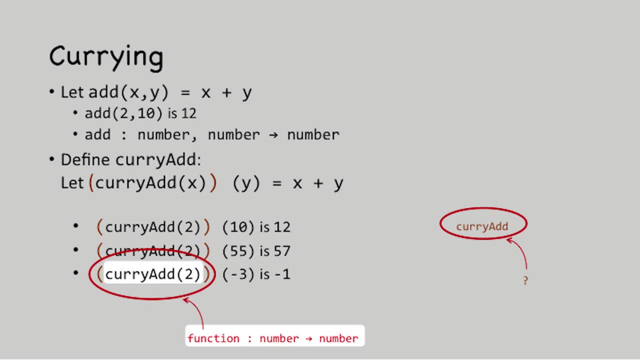 that's notated on the very bottom of the slide. So curry add is something that takes a number and gives me back a function- Curry add when I take the number 2 and apply it to it. when I take the number 2. 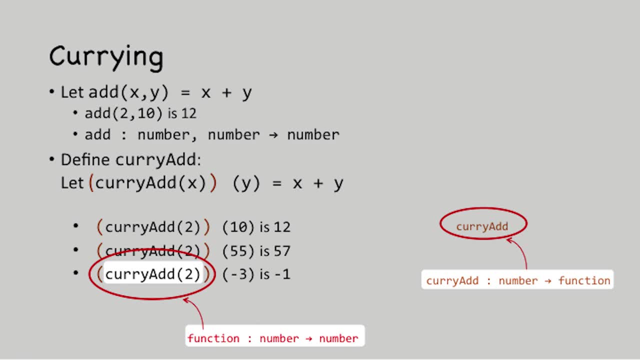 and feed it to curry add as a parameter gives me a function, and that function is the add 2 function. So curry add is a higher order function. It's a function that takes a number and returns a function as its result. OK, 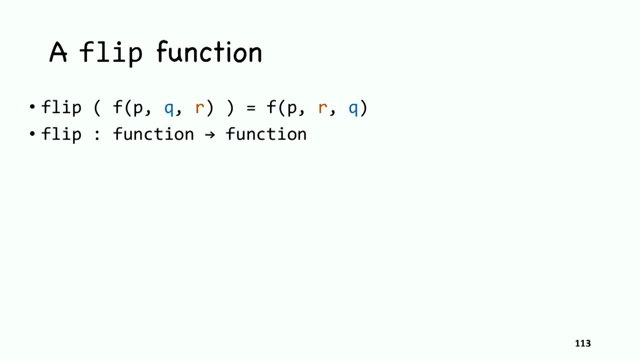 Let's take a look at another example. I'm going to define a flip function, and many different languages have their own words for this, and many languages have flip functions that don't do exactly what I'm describing here, but that's OK. 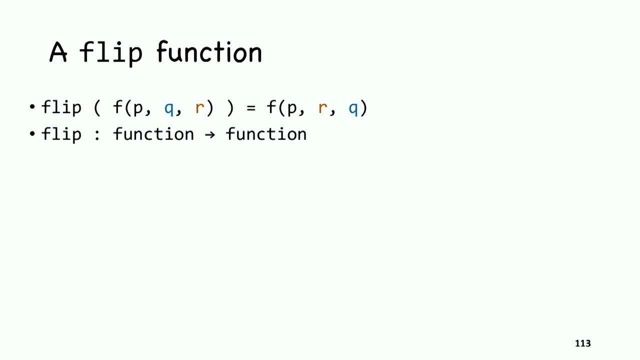 It's my course, It's my notation. I get to call this thing a flip function. When I apply flip to a function of 3 arguments, I'm going to get a brand new function that takes the same arguments but takes them out of order. 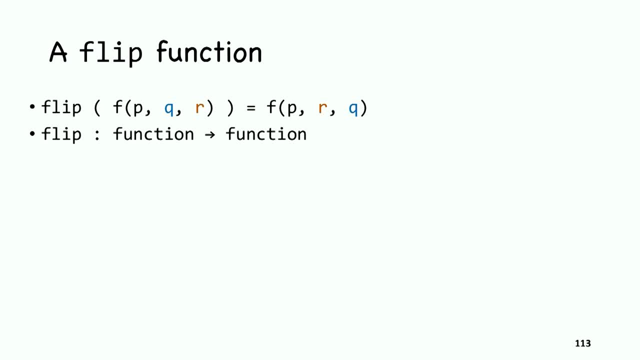 Instead of requiring a p, q and an r, the new function, after having flipped, is going to require p, r and q, And this may be a little bit confusing. I'll show you some examples in just a minute. 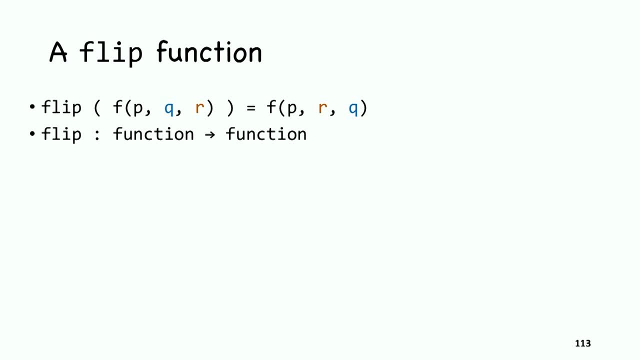 In the meantime, let's agree that flip is super-duper higher order in that it accepts one function f of p q r and it gets back, as its result, type another function f of p r q, And you have to mind. 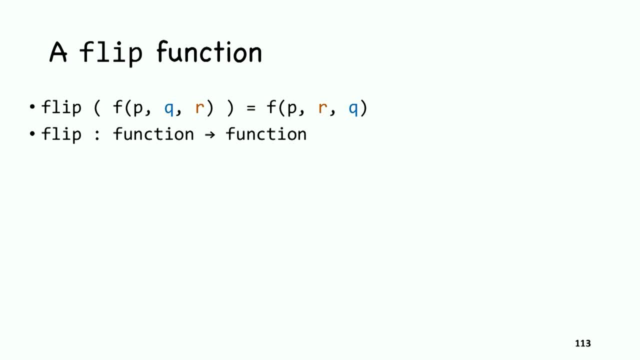 your p's and q's while you watch these slides. Ha ha. OK, Let's take a look at some examples. So let's take my- and I called this earlier. I called this anyline, but you can't fit the words. 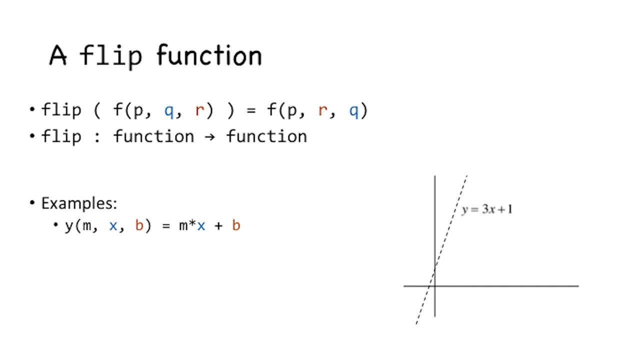 anyline on the slides the way I wanted to. So let's call this the y function, And that's OK, because that's the notation that's used when you describe a straight line: y of m x r and y of m x b. 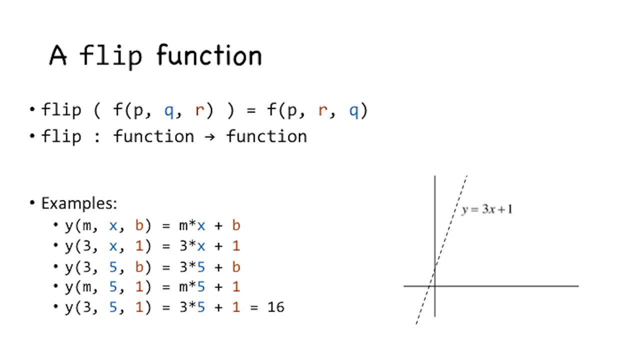 is going to be m x plus b And below the m x plus b line, what you'll see on the slides is several different ways of plugging in values, none of which are terribly surprising. So if I plug in 3 for m, 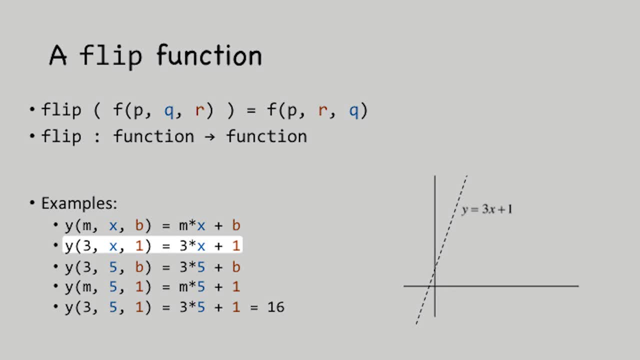 and 1 for b, I get my favorite line, 3x plus 1.. On the other hand, I can do something like just plug in a value for 3, for m and for x, Or at the very bottom of the slide. 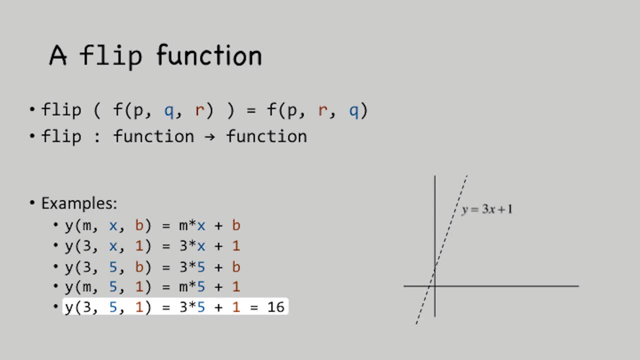 I can plug in values for m and for x and for b and get 3 times 5 plus 1, which is 16.. So I've got three parameters, three arguments to this y function And I can use partial application to do all kinds of things. 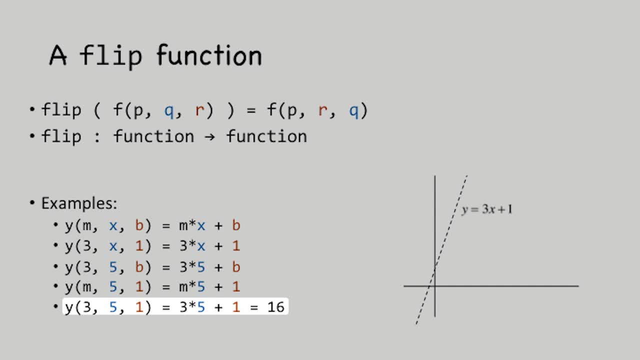 and plug in values as I please. What I want to do is look at this from a point of view of flipping and currying. First, let me talk about what happens when I apply my flip function to the y function. My notation now is that: 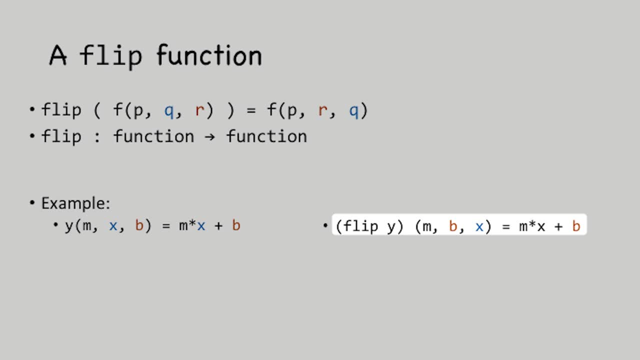 flip y takes three arguments and I'm going to call those arguments m, b and x. I could call them anything I want, but it just will keep our heads screwed on straight if I call them m, b and x. And now you see what flip does. 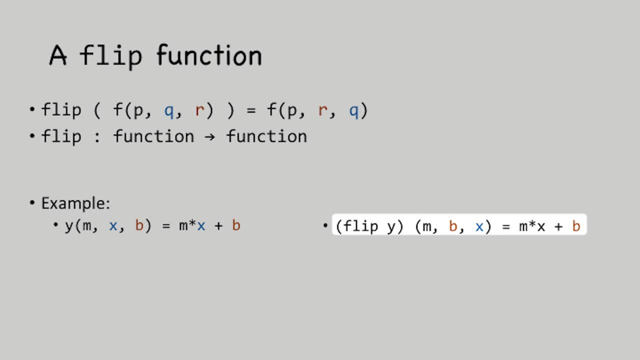 When I start with y, just plain old y- I take three arguments and I multiply the first two together and then I add the third argument. So if you look at y, m x b, right below the word example, you see y of m x b. 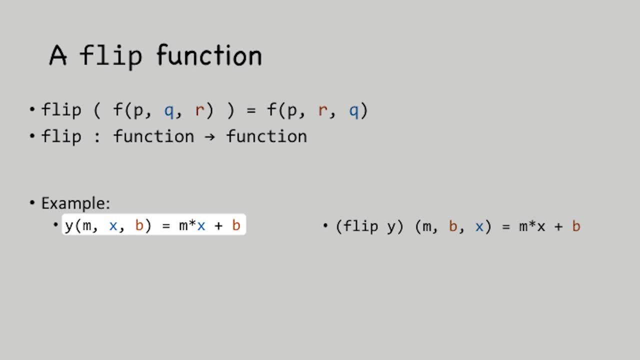 equals m times x plus b. That means take the first two arguments, the m and the x, multiply them and then add the third argument. That's what happens when I just do y, When I do flip y, then I don't take the first two arguments. 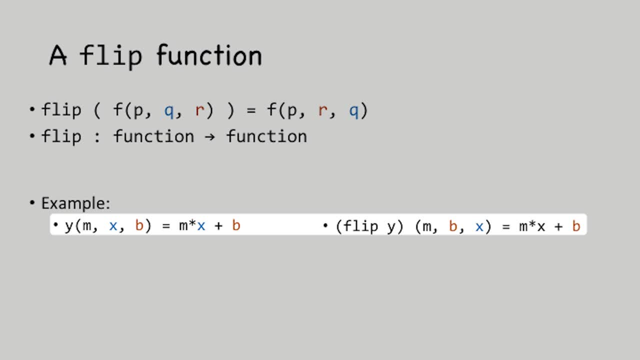 and multiply them. Instead, I take the first and the third argument, the m and the x, and I multiply those getting m times x, and then I add the middle argument b. So that's the effect of applying the flip function. 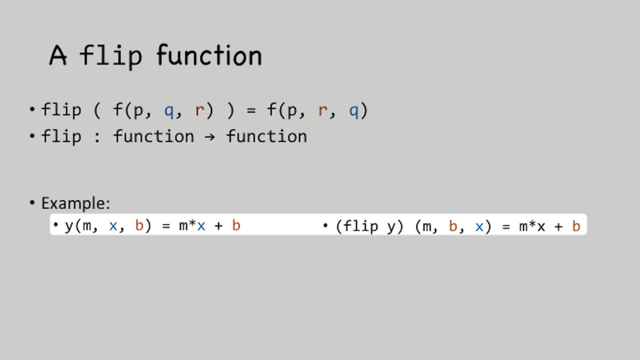 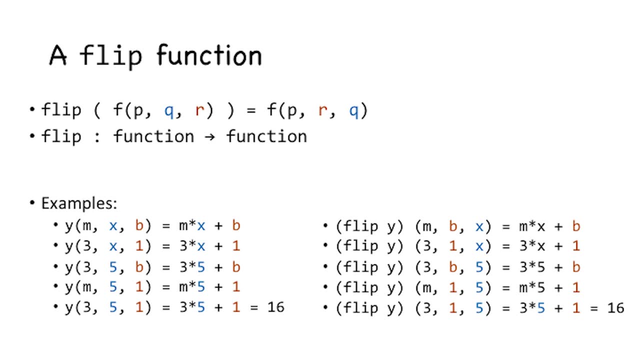 to this y function. It just juggles two of the arguments to the function. So, below the first use of flip y, I've shown you what happens when I plug various values in: for the m, for the x, for the b, and so on and so forth. 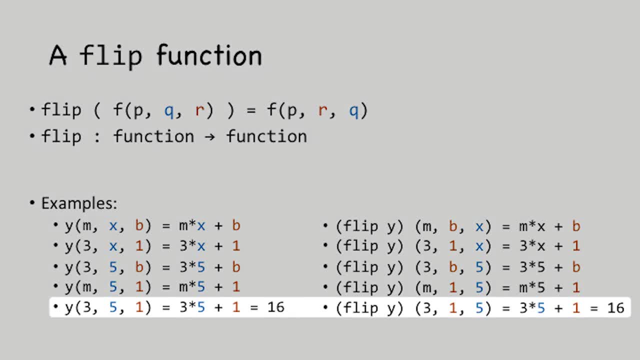 Ultimately, if I put three, five and one into the flip y function, if I put them in in the correct order, I still get 16.. So I haven't really changed what I'm computing. I've just sort of changed the order. 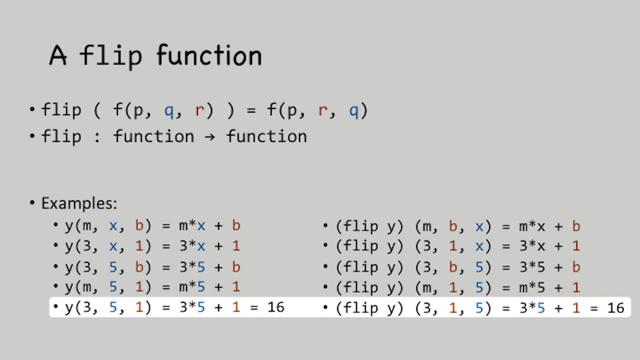 in which I'm supposed to feed it my arguments. Now, what does this do for me? Okay, What this does for me is it means that the arguments that I will normally want to make set in stone the m and the b. those are the ways. 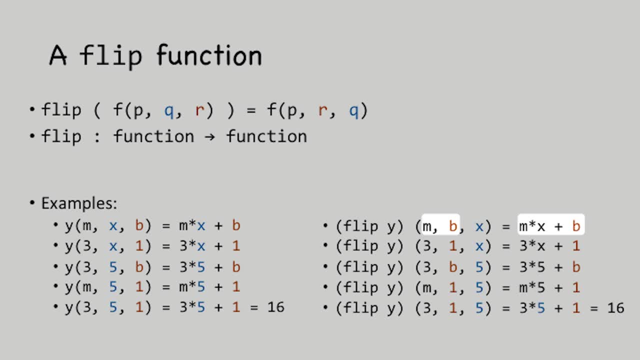 those are the two arguments that I want to create defaults for in order to create a straight line. Those two arguments are the ones that are the leftmost arguments in the calling of the function. Now, with my flip y function, I can set a default value. 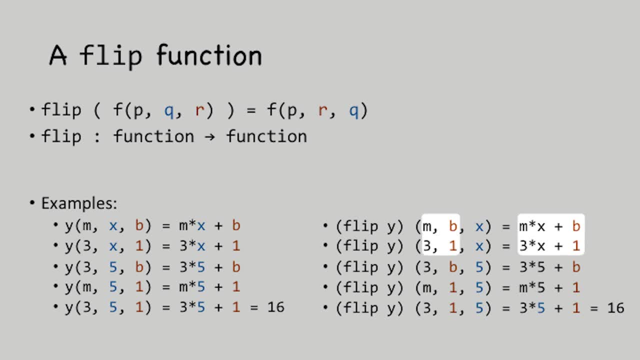 for the m argument, the leftmost argument, and then I can set a default value for the middle argument, the next two leftmost arguments, and I have my line three x plus one. Let's have a look. I'm going to start with. 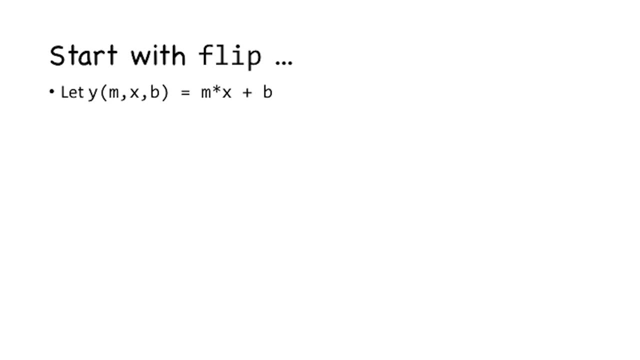 y, m x, b equals m x plus b. That's my regular y function. Then I'm going to flip it. When I flip it, I get m as the first argument and then b as the second argument, and then x, that thing. that's going to vary. 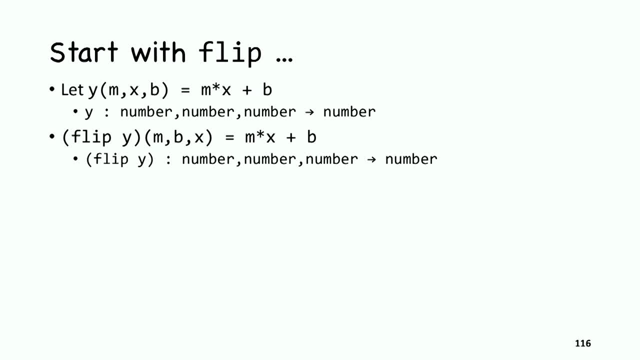 all the time. as my third argument Now, both y and flip y are lower order functions. They take three numbers and they give you back a number. But remember, flip is a higher order function. Flip takes the y function and returns the flip y function. 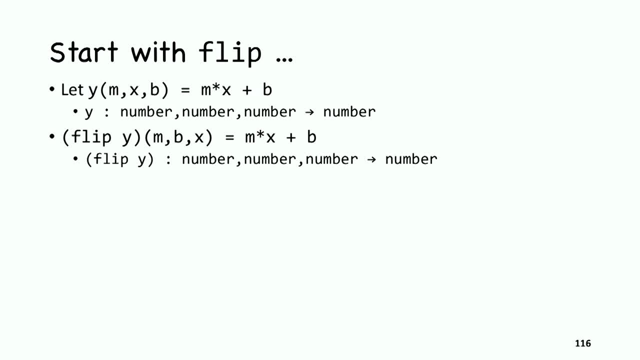 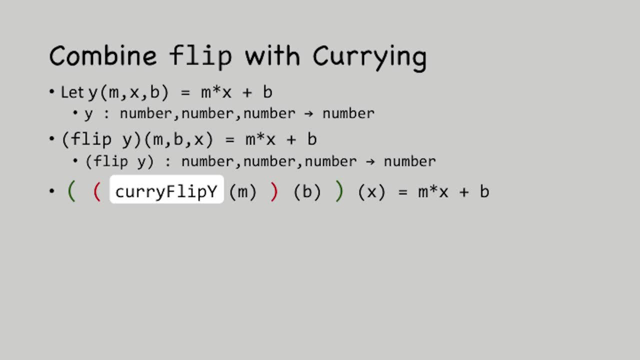 All right, let me take the bold step now of doing currying. I'm going to create something new called curry flip y. I'm going to take flip y, which takes three arguments, and when I curry it, it's going to take only one argument. 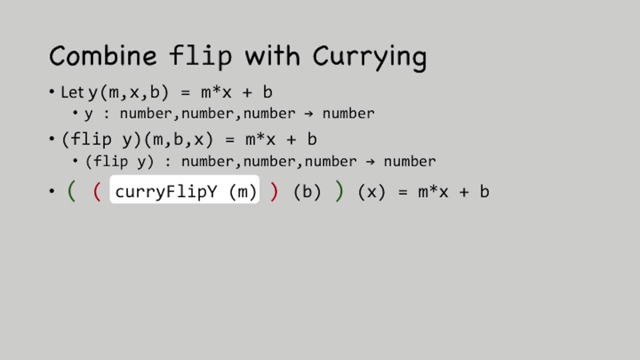 the leftmost argument, the m, So that thing, curry flip y m that thing in red parentheses. that's a thing now, and it's a thing to which I can apply another argument b and that gives me a thing in green parentheses: 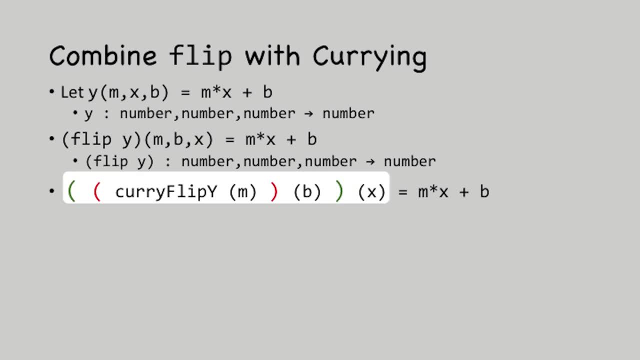 to which I can apply another argument. a third argument: x. All right, again, no big mystery, I'm not computing anything that I didn't compute before. On the second line that you see here, when I take curry flip: y of three: 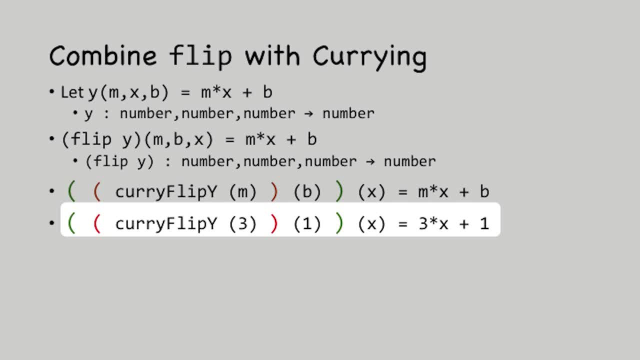 and I apply it to one, and then I apply it to x. I get my familiar old equation for a line three x plus one. But now that thing in green parentheses, that's well, that's a function, and I can apply x to it. 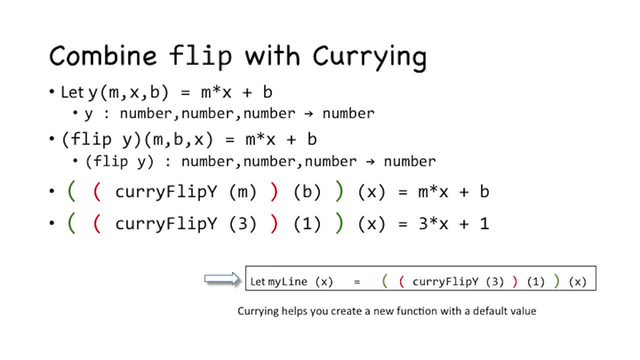 and I can give it a name. I can call it my line, So that thing in green parentheses. I can call that my line and I can apply x to it, And then what I'm saying is that my line of x is. 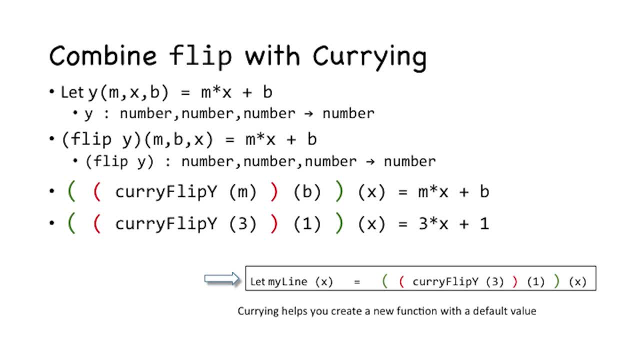 well, three x plus one. So once again now, currying is helping me create a new function- my line- from an original function y that didn't have any particular default values. Okay, again, what we want to do is examine. 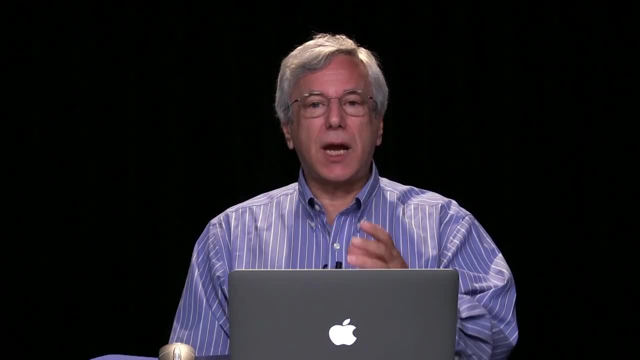 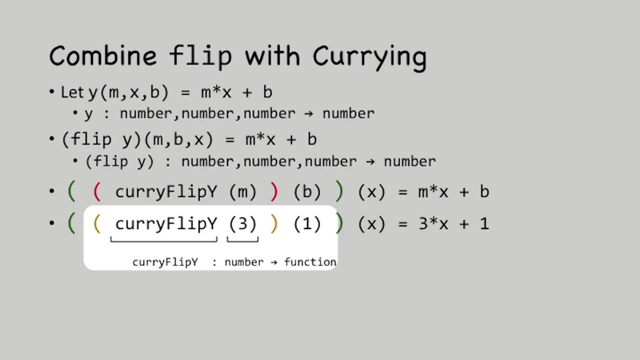 what kinds of functions we've got here. What types of values do our functions accept? What types of values do our functions return? What's curry flip y? It takes a number and it gives me a function. Curry flip y takes a number like three. 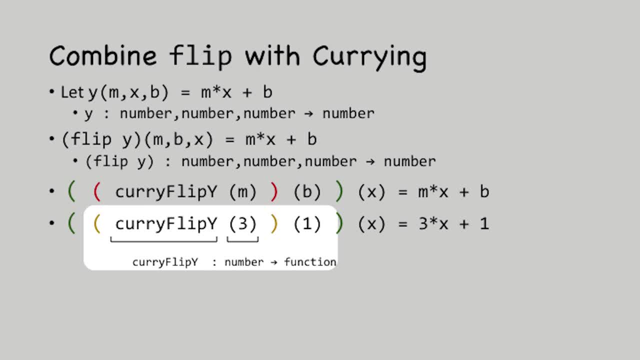 and gives me back a function, the stuff in I don't know red or brown to which I can apply the number one. So that stuff in the brown parentheses curry flip y parentheses three, that stuff is a function to which I can apply. 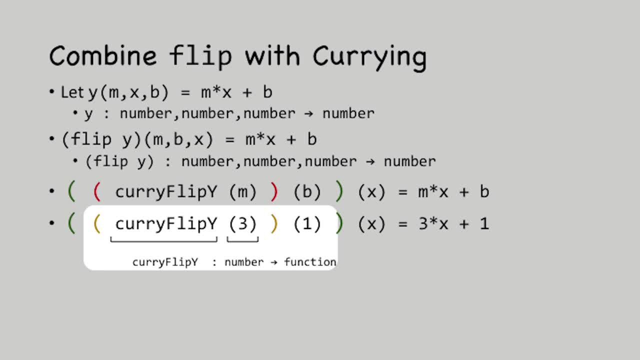 the number one or any other value. b: Curry flip y. then took the number three and gave me back a function. Curry flip y is a higher order function. Let's continue. What's curry flip y three? Well, it takes a number like one. 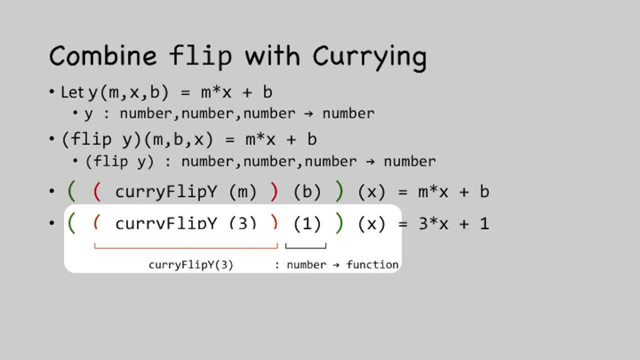 and gives me back another function. When it takes the number one, it gives me back a function- the function in green- and that thing is a function and the reason that I know that it's a function is because it can take an argument. 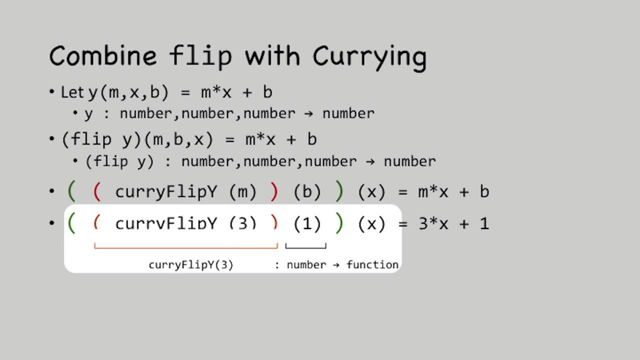 the argument x. So far, so good. What kind of a thing is the thing in green? It's a function and it just takes one argument. It takes the argument x. the argument x is a number and it returns another number. 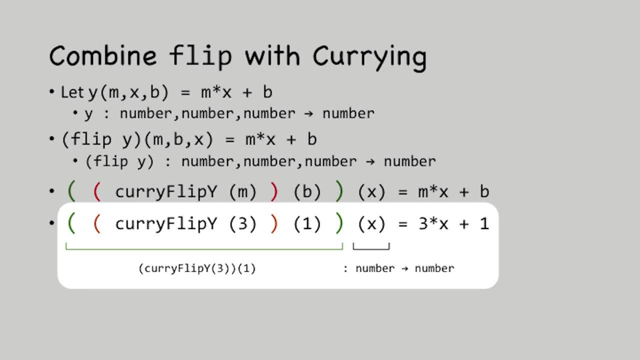 If x is seven, then the value returned by the application of seven is three times seven plus one 22.. Okay, So what I've done is with currying. I've started with a function of. well before curry, I started with a function. 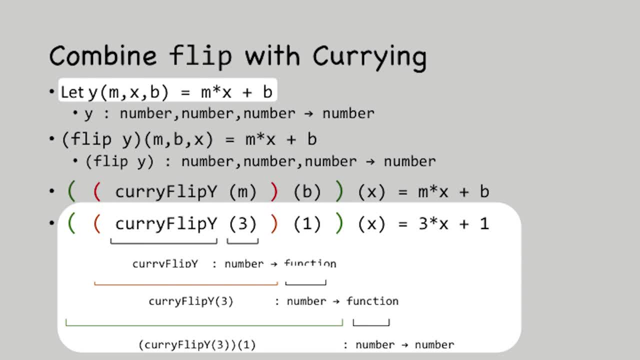 of three arguments and I ended up, after currying, with a function of one argument that gave me another function and that other function took a function of one argument and then I could apply that function to x. So I have functions that return functions. 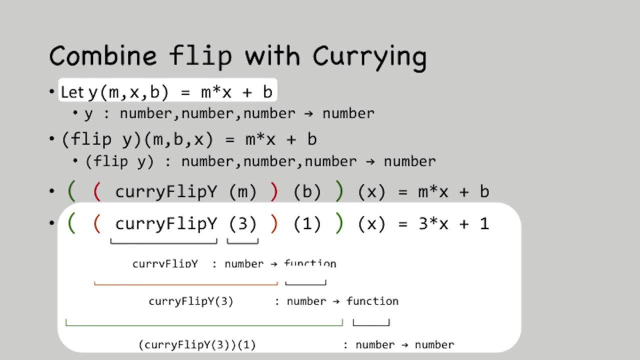 that return other functions. Eventually, I get a function that takes a number and gives me back another number. It's the function of a straight line. Currying, then, is a way of using higher-order functions to fill in default values for existing functions. 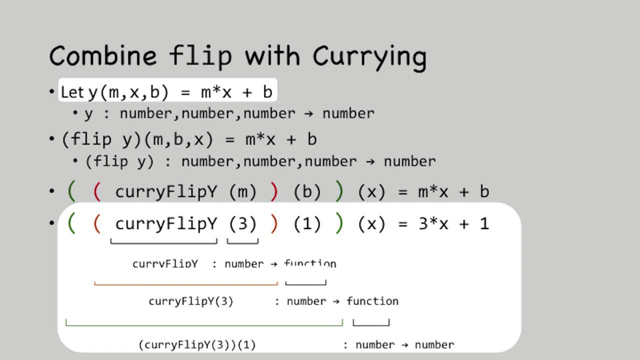 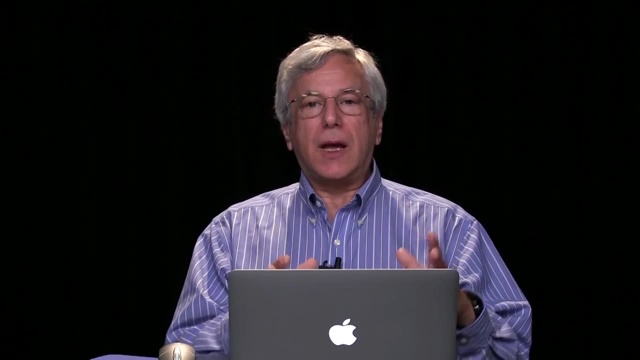 to make new functions from old. Why is making new functions from old functions important? Because this is all about functional programming, and when you've got functional programming, you want to have as much dexterity with your use of functions as possible. In the next segment, 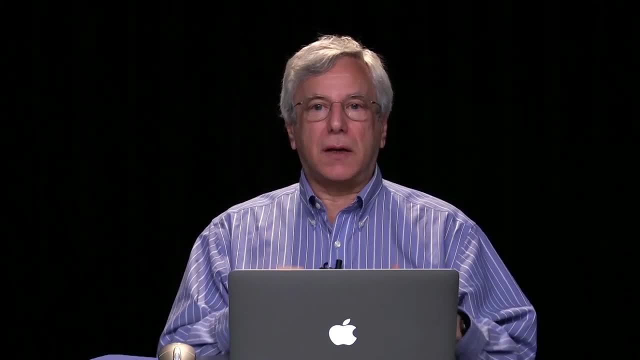 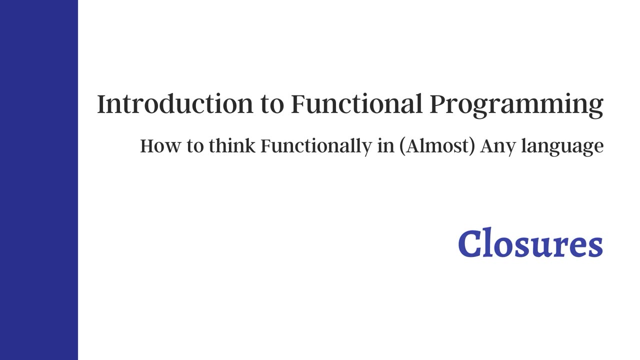 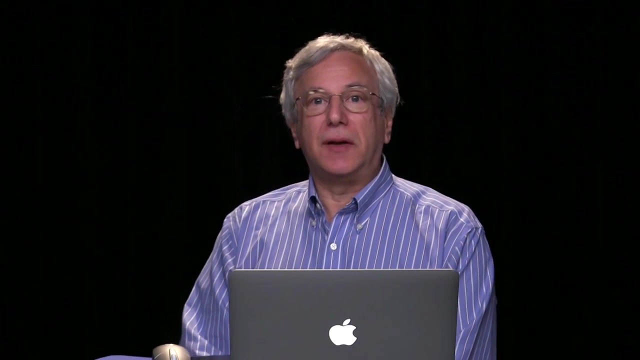 I'll talk more about different kinds of higher-order functions. A higher-order function is a function that takes functions as one or more of its arguments and or returns a function. as a result, Higher-order functions come in many shapes and sizes, many different forms. 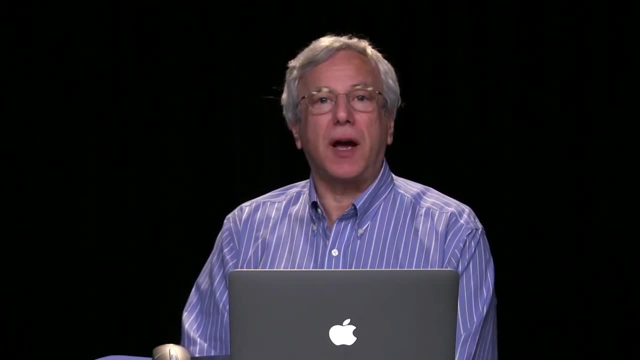 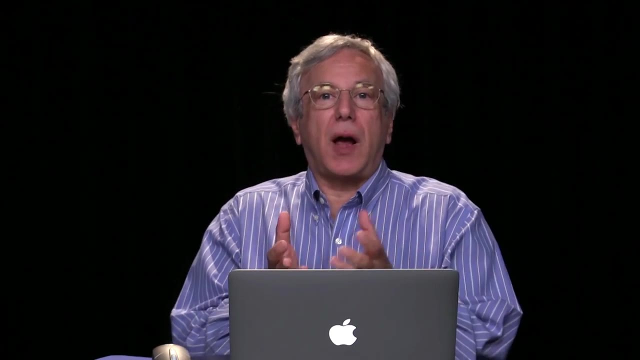 and, in this section, what I want to do is talk about one form that a higher-order function can take, that being the form of a closure. So let's think about a problem that you might want to solve. You might want to create a counter of some sort. 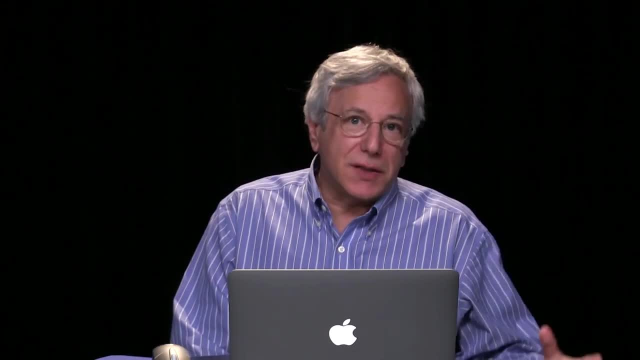 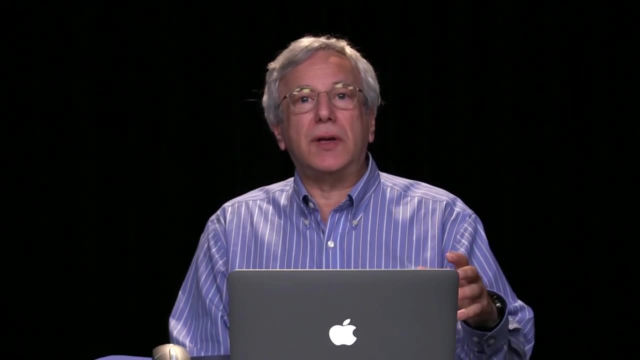 A counter is something that might start off at zero. When you do something, or something happens in the execution of your program, it'll increment to one. When you do something else, it'll increment to two, then to three, then to four. 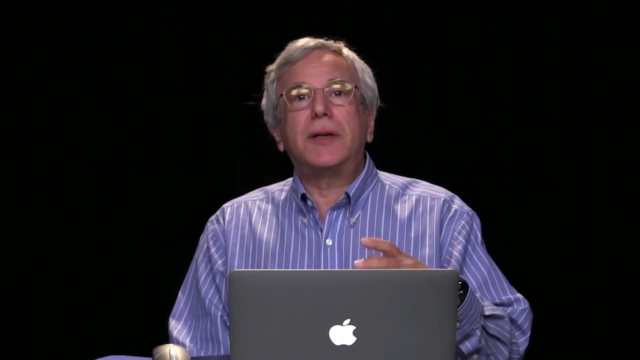 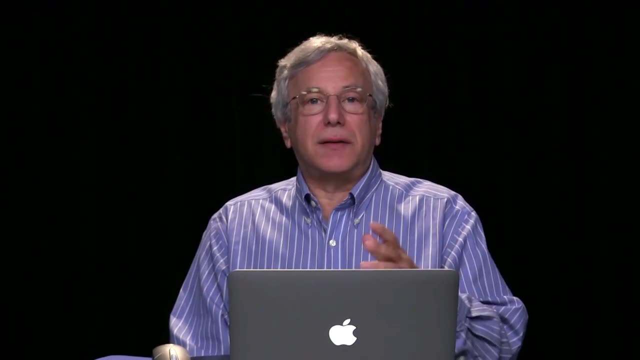 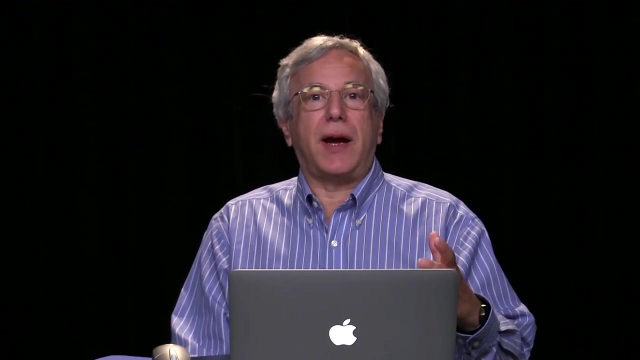 You may want to have several different counters in your program to count several different kinds of things going on. Well, in a straight, imperative program you'd have a variable named count and then if you wanted to keep track of the counting of two things, 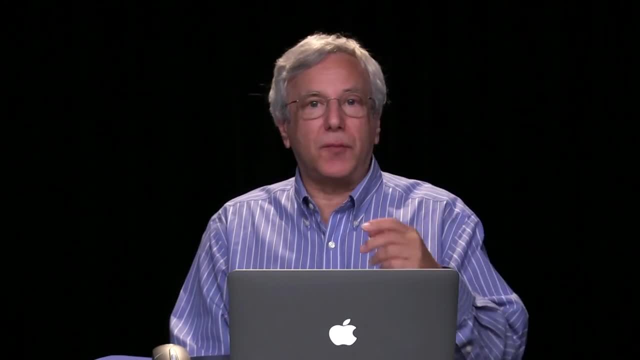 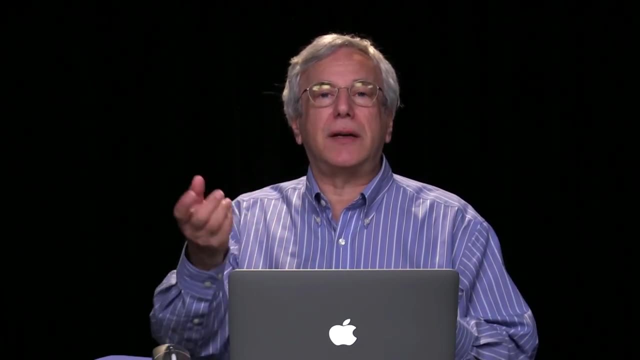 you'd have a variable named count A and another variable named count B. Okay well, that's kind of an undisciplined way of doing it. Let's think object-oriented. now You'll have an object that contains a counter field. 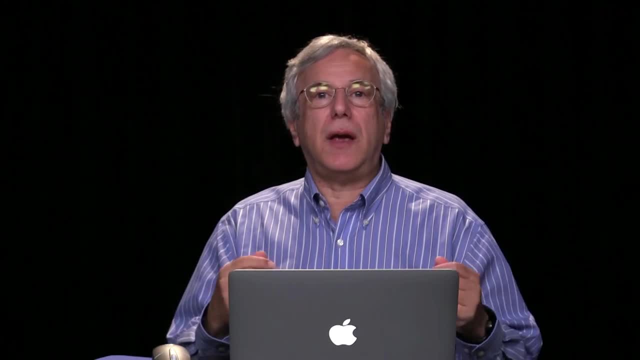 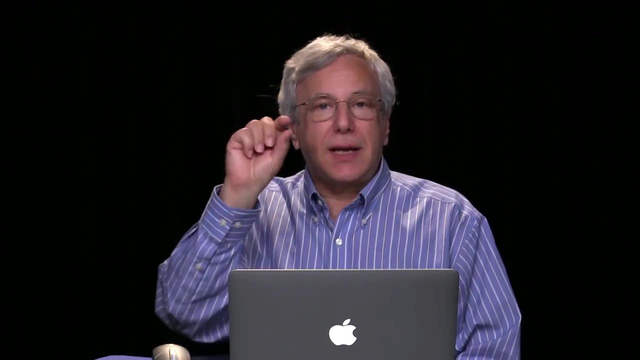 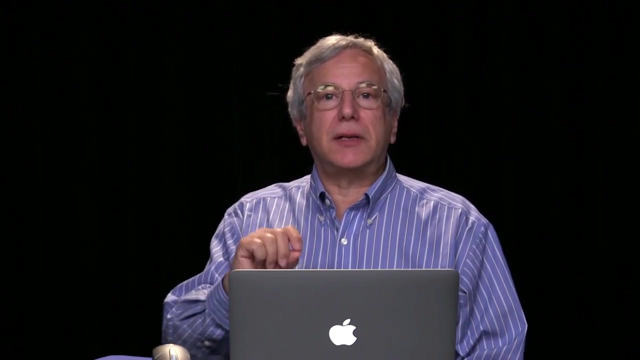 a counter property and you'll create one instance of that object and it has a count within it and that object will also have a function inside of it, a method, and so when you call that method, it increments the counter And then, if you want, 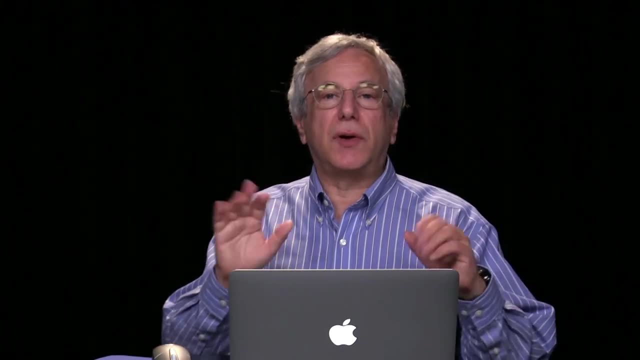 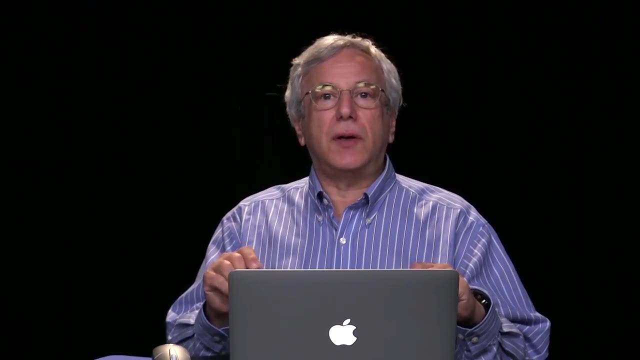 to count two things. you have to create two different objects, So each of those objects has its own counter and each of those objects has its own function. and you want to increment the count of some kind of thing, A, so you call object A's function. 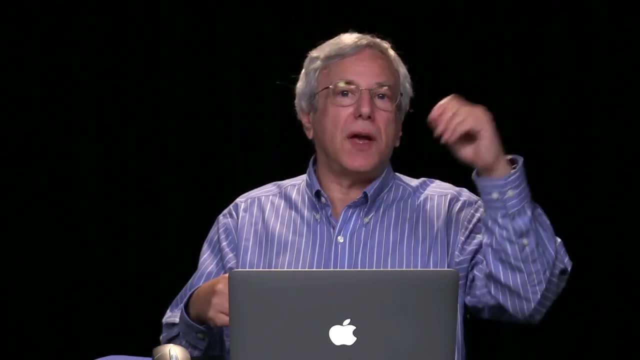 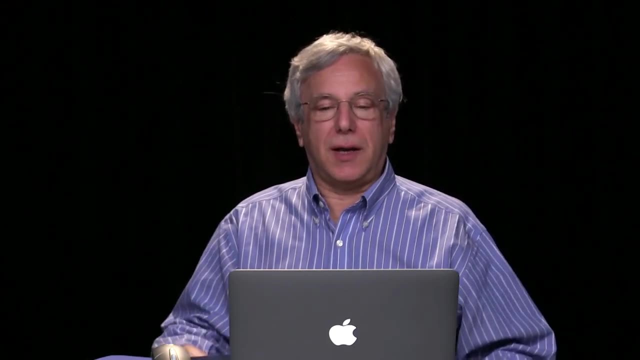 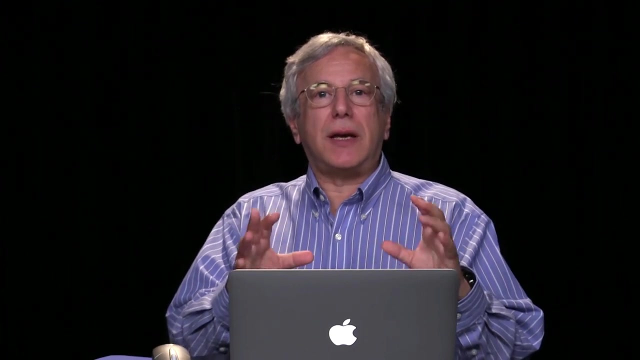 to increment, and then you want to have event B occur. When event B occurs, you call object B's function to increment the count B. Well, the object-oriented way of doing it is a bit more disciplined, because the counter then is localized to these particular 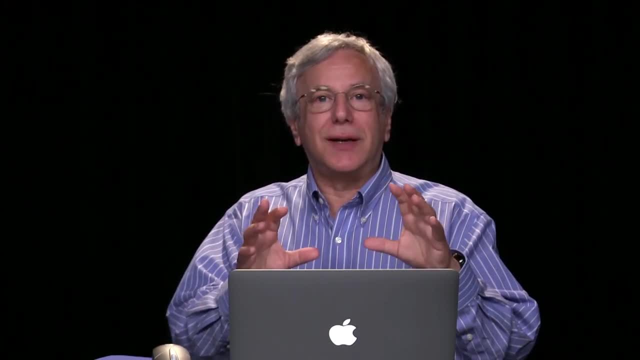 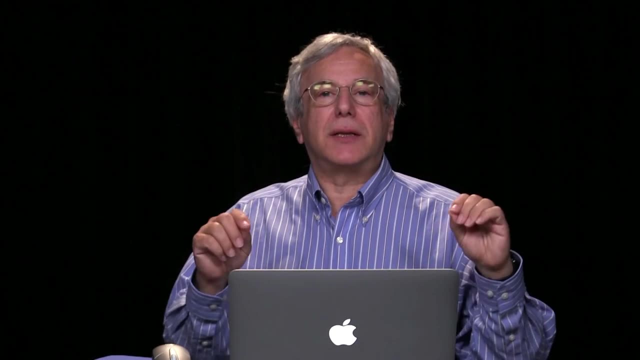 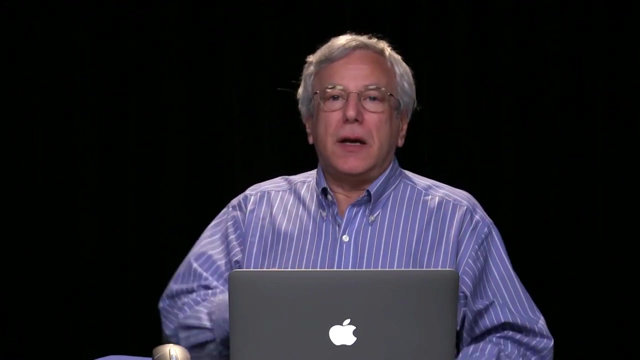 objects that you create. The counter is safely tucked away inside these objects so that only the functions, the methods that belong to the individual objects can get at these counters. That's safe, but you also have the overhead of creating two or three or more brand new objects. 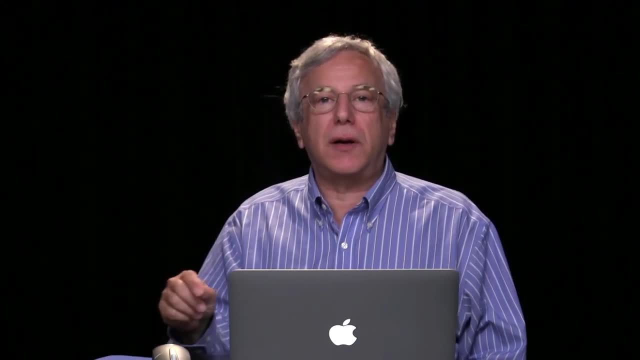 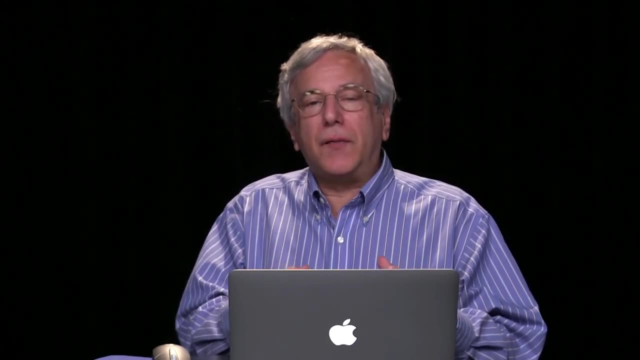 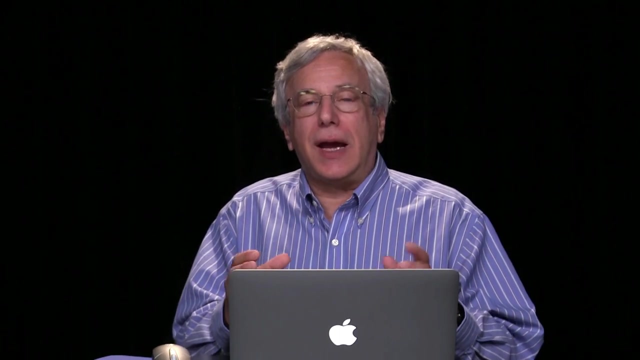 and creating objects in an object-oriented context takes time. Is there a way that we can get the best of both worlds and have a kind of a counter that's safe and can only be incremented in a disciplined way and yet doesn't incur the overhead of creating? 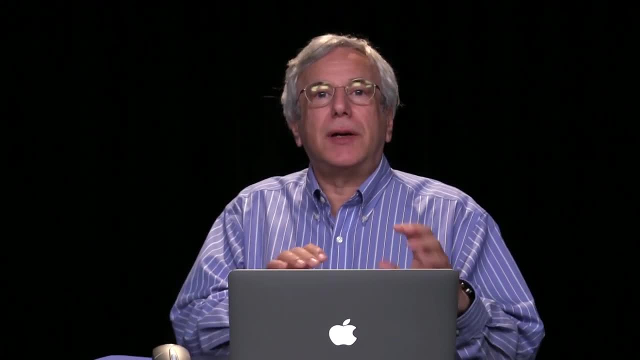 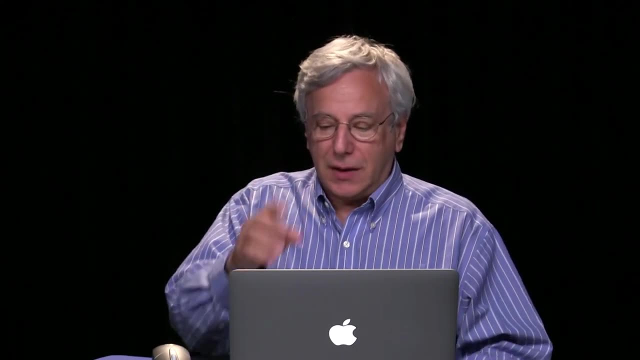 a brand new object every time you want to count something different, We can do that with a mechanism involving higher-order functions called a closure. Let's have a look. I'm going to have a count variable. I'm going to start it off to zero in this instance. 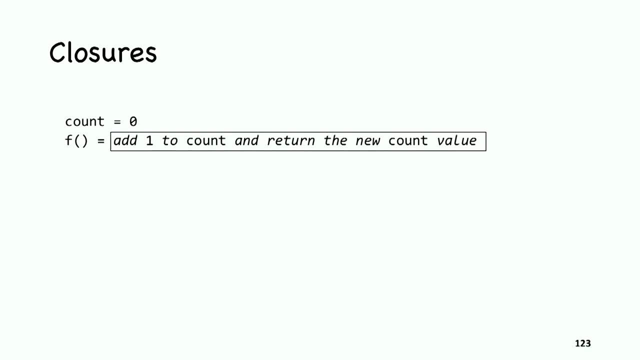 and then I'm going to have a function and that function takes no arguments. The only thing that function does is it adds one to the count and returns the new value of count. So if I call the function once, then that first call to f. 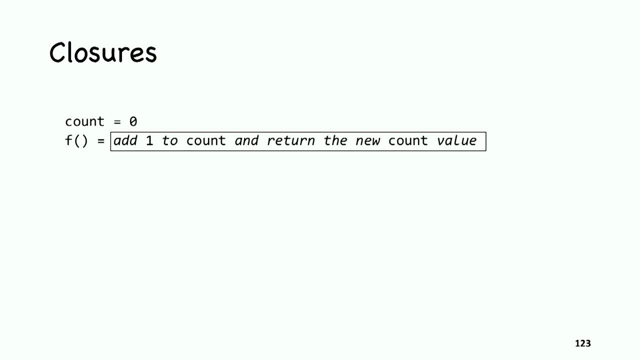 with parentheses around. it changes the count to one and returns the value one. If I call it a second time, it changes the value to two and returns the value two, and so on and so forth. So far, this is not a higher-order function. 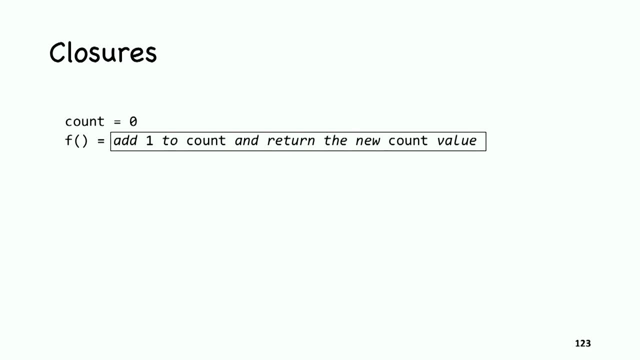 And this function f is sort of out in the wild. I want to bottle up this function and I'm going to bottle it up by creating a kind of a closure. I'm going to close around this function In particular. I'm going to enclose. 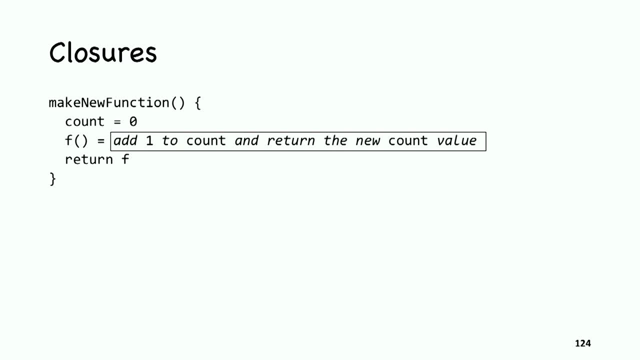 that count variable around the function f and you'll see what I'll get. I'll get something that's kind of like an object in an object-oriented setting, but a little bit more lightweight. So let's have a look, I'm going to create something called 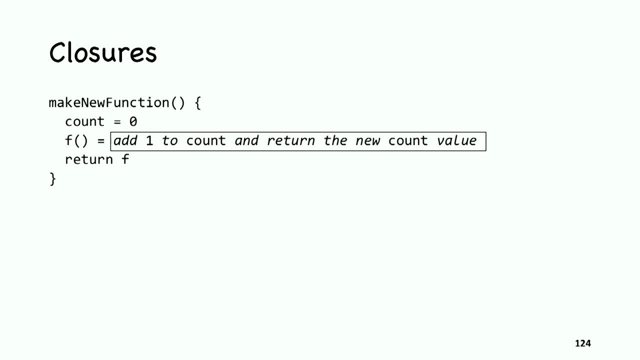 makeNewFunction. makeNewFunction has a local variable named count, so you can't get at that count value willy-nilly from the outside of this code. What makeNewFunction does is it has its variable count and it also has its function. 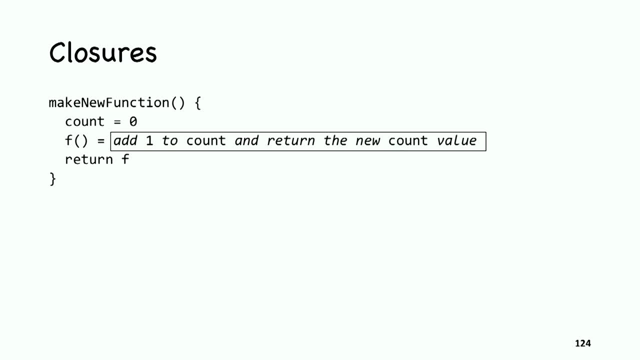 that we had in the previous slide. that function adds one to the count and returns the new count value, But now in a higher-order function way, the makeNewFunction thing returns the function f as its result. Okay, It's higher order. 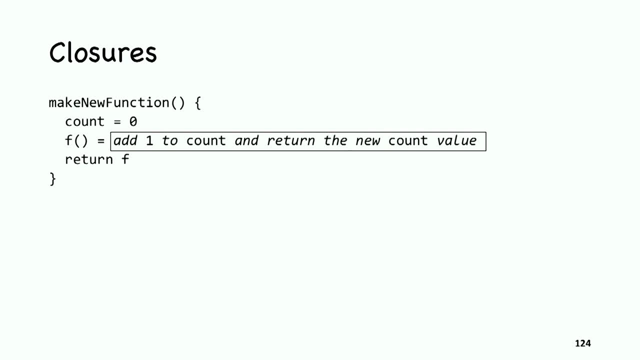 I'm not returning a number. I'm not returning an array. I'm not returning a list, I'm returning a function. So this is higher-order stuff. Now, when I call this function, so makeNewFunction, what I get back is a function. 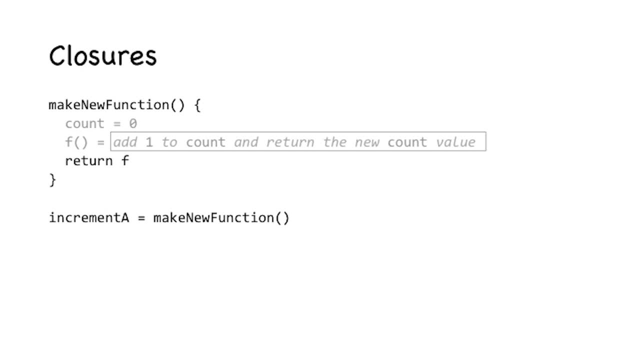 So in this slide, increment a, its value, is a function. It's the function that I defined as f inside of the makeNewFunction's body. Okay, What does increment a do when I call it Increment a does what the newly defined function f does. 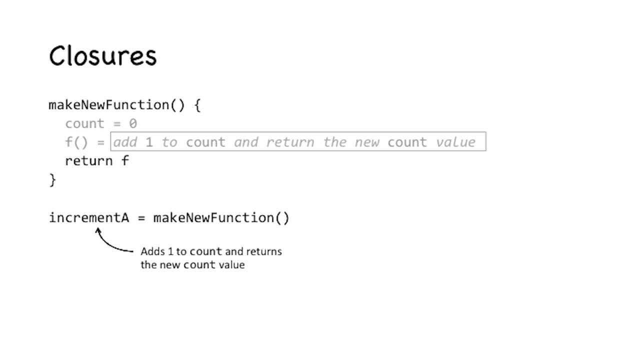 It adds one to the value of count and it returns that new value of count. If I define increment a as the result of call to makeNewFunction, then I can call increment a and print its results and the first time I call it. 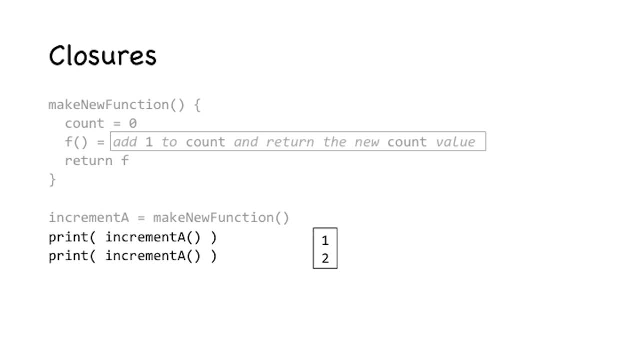 I get back the number one, and the second time I call it I get back the number two, and so on and so forth. I have enclosed the count value around the function f. Notice, by the way, that makeNewFunction has exited. 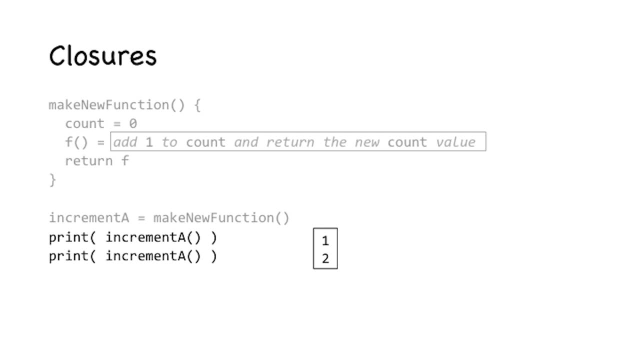 by the time I call print increment a, makeNewFunction is no longer alive. when I call print increment a, and yet, by the rules that I have assigned to the notion of closures, that count variable still exists. And when I call increment a. 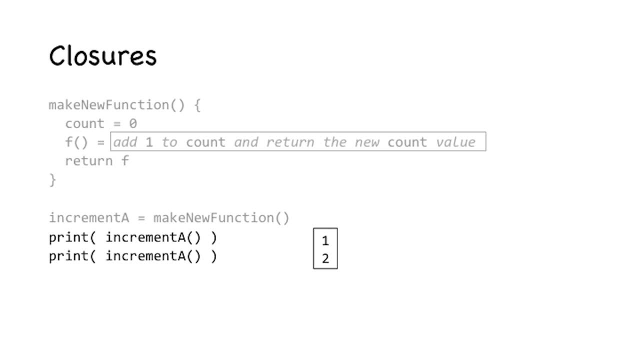 that count variable gets one added to it and becomes one The first time. the second time it becomes two. Okay, That's a function that returns a function, That's the makeNewFunction. Now, what kinds of things can I do with this? 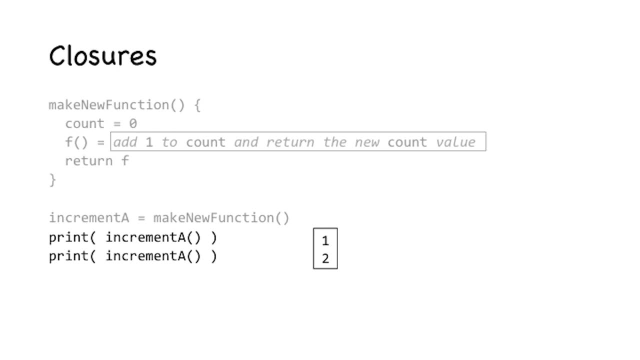 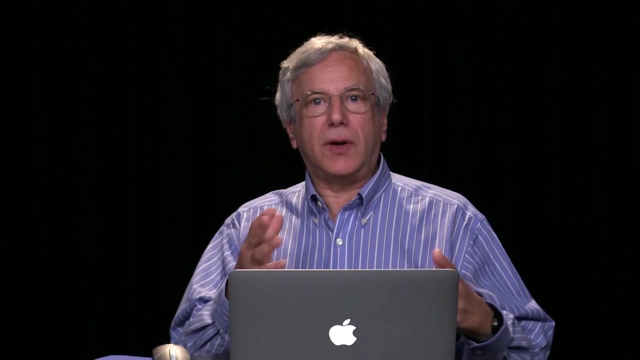 I said earlier in the discussion that I might want to have two different things that I'm counting and in an object-oriented setting, I might create two different objects from an existing counter count. Well, okay, Is there a parallel in this closures world? 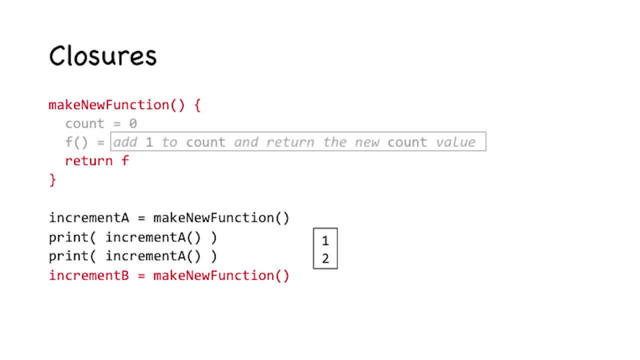 Yes, there is What if I call makeNewFunction again? And this time when I call makeNewFunction, I take the result of having called makeNewFunction and I assign it to increment b. All right, Increment b is different from increment a. 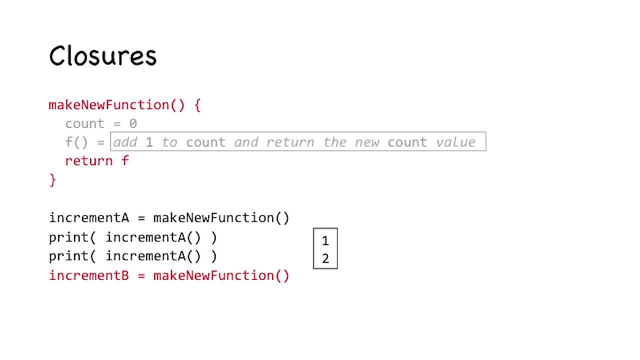 Yes, the value of increment a is a version of the function f and the value of increment b is also a version of the function f. But the way we like to think of closures, we're going to make increment b be a different value. 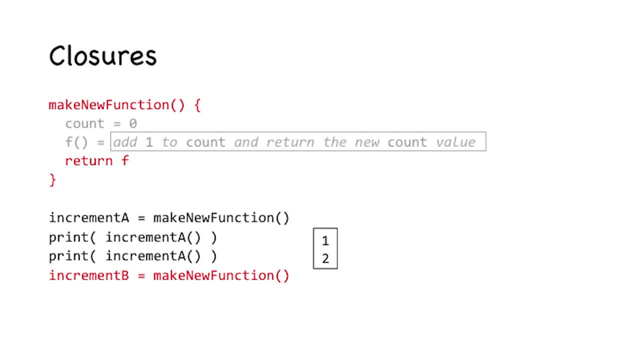 a different version of the function f, a sort of a different copy of the function f with its own copy of the variable count. After calling increment b and making increment b be a function, I can call increment b and when I do. 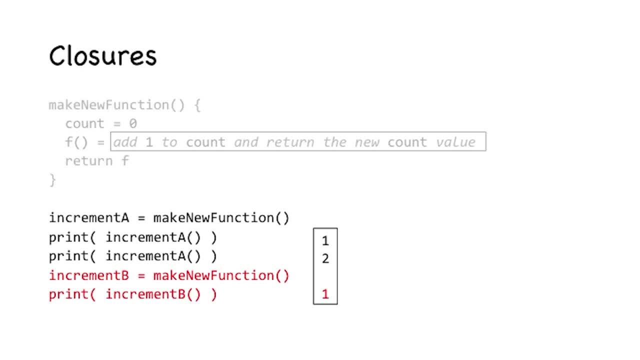 if I print the result, I get one. I don't get three right away. If I call increment b count, it's a brand new count. It started off again at zero and when I call increment b it becomes one. 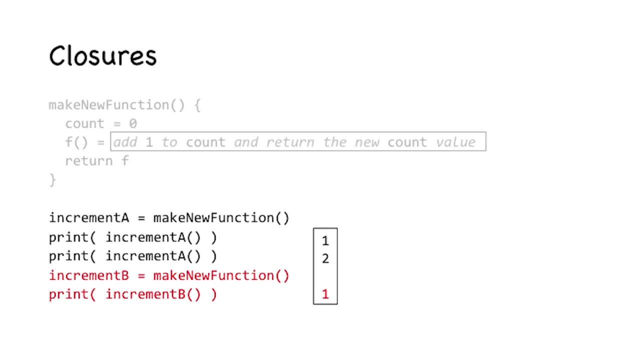 And then maybe something would provoke me to call increment a, And if I do, when I call increment a, increment a takes its counter, which already was two, and turns it into three, and if I print that I get three. 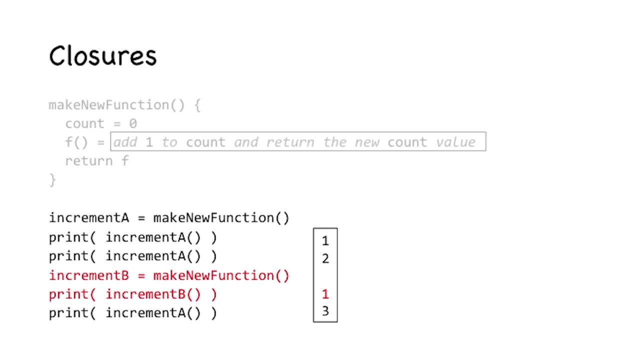 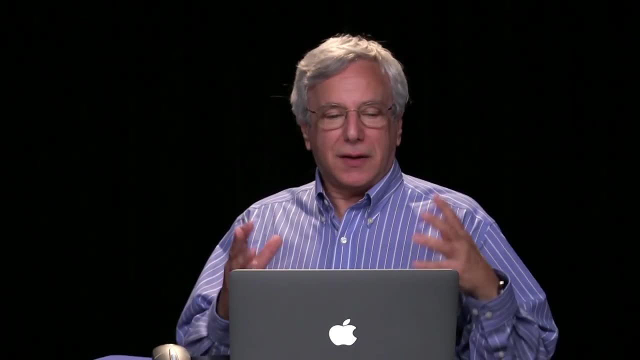 I can create new counters, many new counters, and each time, all I do is create a brand new function. I don't create a brand new object, And this is a powerful idea. So what is a closure? A closure, something like increment, a 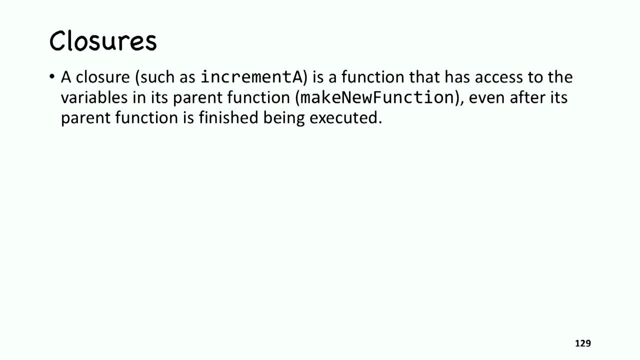 it's a function that has access to whatever variables its parent function had. The parent function in this case is make new function and, even though the parent function is finished being executed, increment a still has access to that count variable that I initially set off. 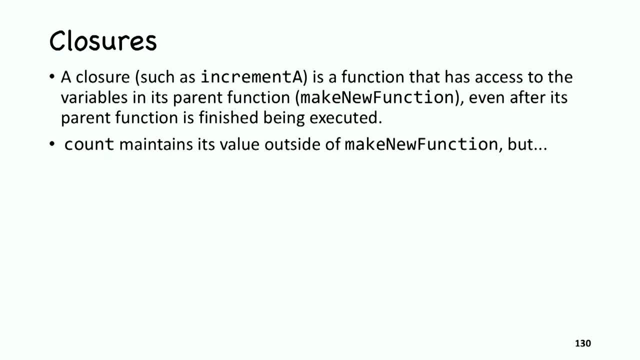 started off as zero, So the count variable maintains its value outside of the execution of make function. However- and this is a very important point- that count variable is still local to the make new function and it's available to the increment a function. 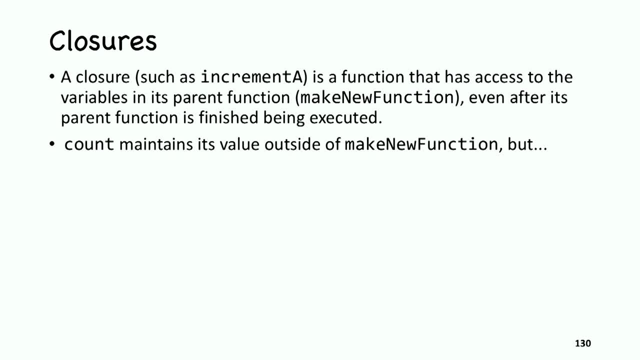 Count variable is still safe. it's still disciplined. The only way that I can change the count variable is if I call increment a or increment b or, as the slide says, increment x. you name your letter Okay, So each increment x function. 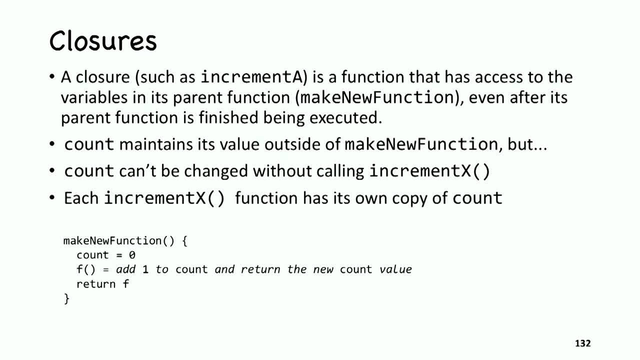 has its own value, its own count variable. Right, If I call increment a, then I can start incrementing that count variable, and then, if I call increment b, the count variable starts again at zero. Now, that's the basic idea of closures. 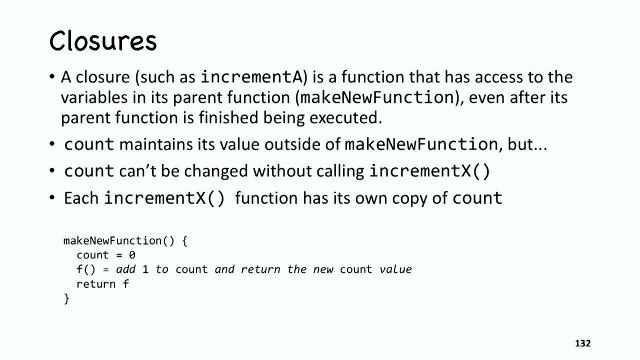 Now, if I want to enhance this idea a little bit, let me do that. Let me create another function. I'm going to call it make new function again, but it's going to be a little bit different from the make new function in the previous slide. 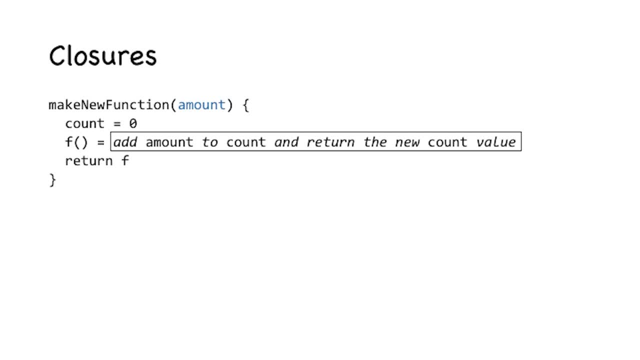 Let's take a look here. This version of make new function takes a parameter and the parameter is amount. And okay, I've decided to keep the count starting off at zero. but now my function f is going to use the parameter that I passed. 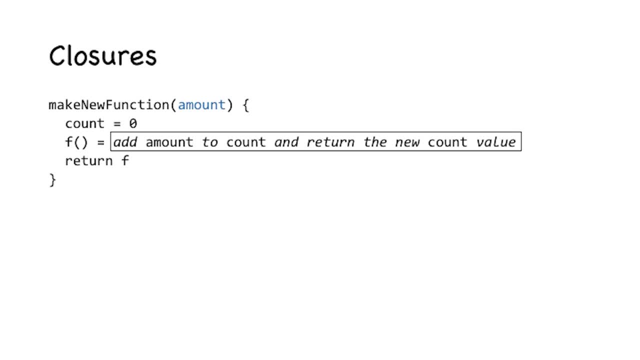 to make new function. So, instead of adding one every time I call count, it's going to add amount every time I call count And, of course, it's going to return the new count value. So take a look at the things that I can do. 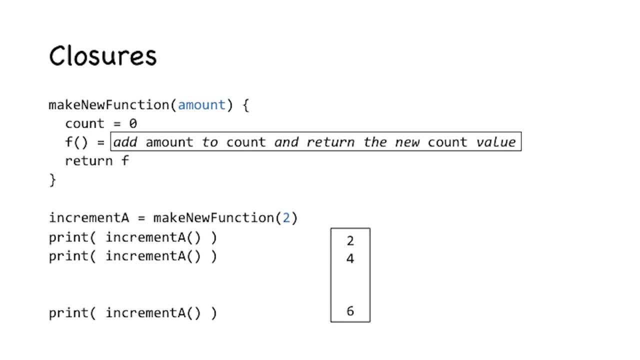 at the bottom of this slide. now, If I call increment a with make new function with the parameter two, then I get an incrementer that the first time adds two to zero and gets two. The second time adds two to the existing two value and gets four. 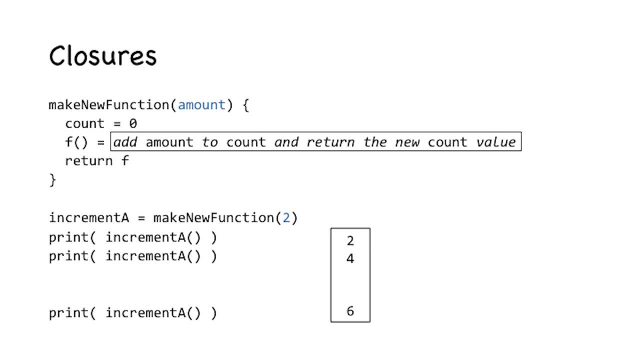 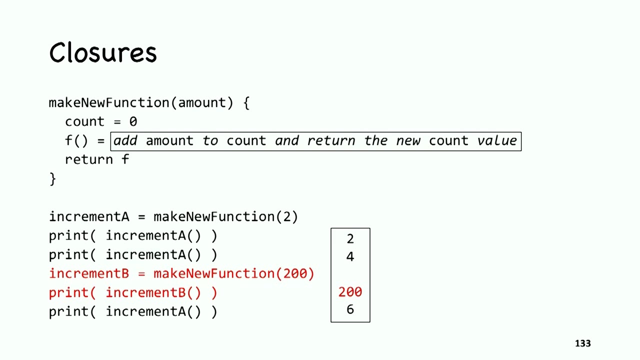 And the third time eventually adds two to the four value and gets six. At the same time, I can create another function called increment b, with a different call to make new function, And the different call to make new function in this case takes the amount value of 200.. 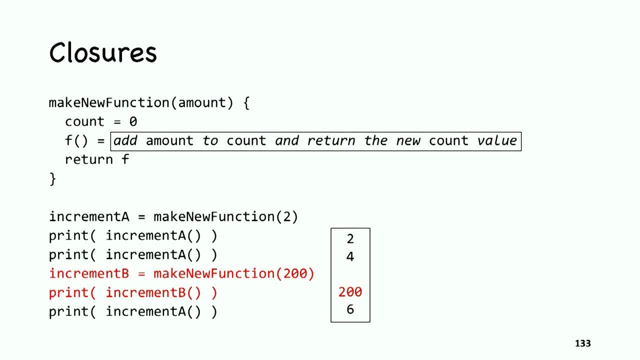 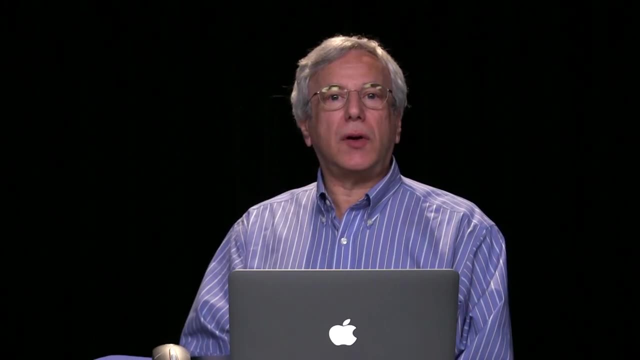 Every time I call increment b, it increments its own counter by 200.. So what I've got now is the ability, not a count variable that's willy-nilly just available anywhere in the code. No, I've got a count variable. 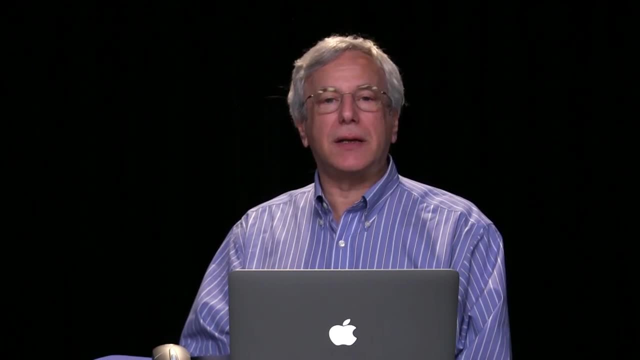 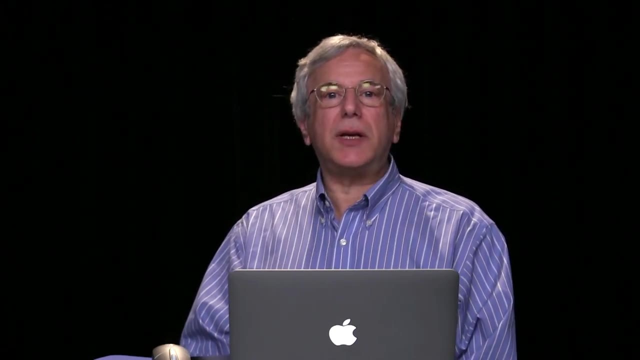 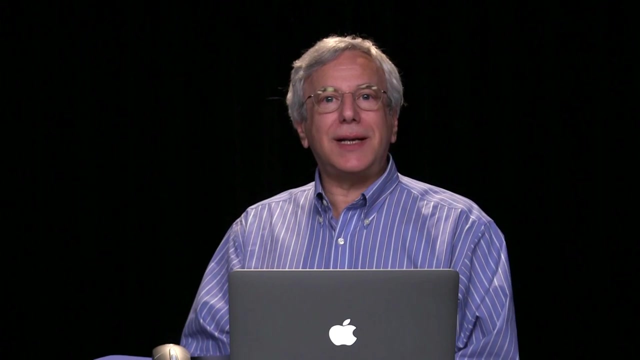 that's safely tucked inside of a context. It's safely tucked inside of the make new function function And it's available to increment a. And another version of the count is available to increment b, But in a safe way. no other code. 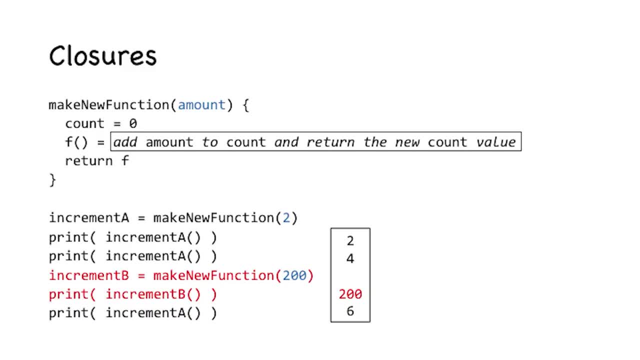 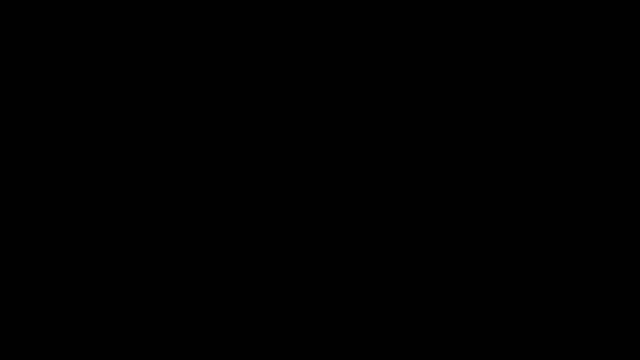 no code except increment a and increment b and maybe increment x. if I create it can modify a value of count. That's really really good stuff, And we get it all because we think in terms of higher order functions. What is a data structure? 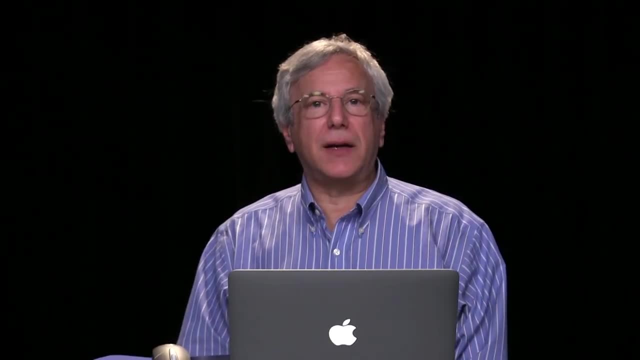 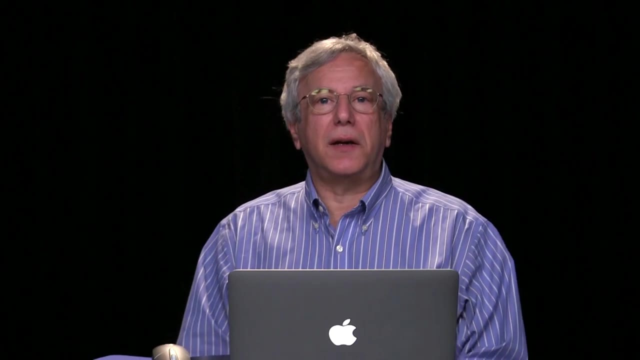 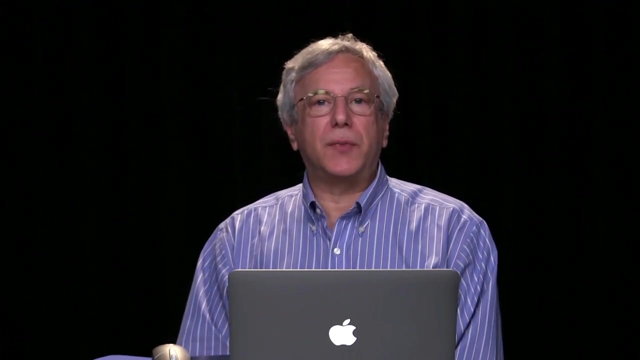 Well, a data structure is a bunch of data combined and given a new name, A sort of a way of managing clumps of data effectively. Well, how do we do data structures in object-oriented? object-oriented programming? We take a bunch of values. 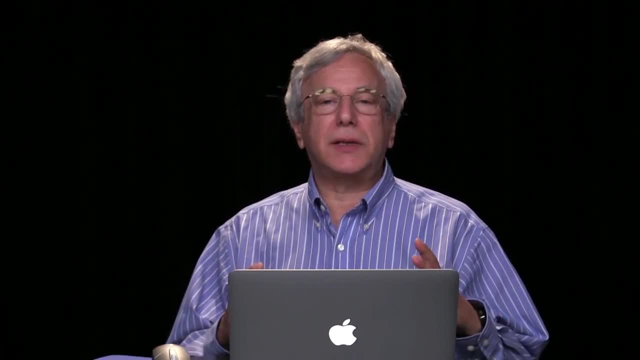 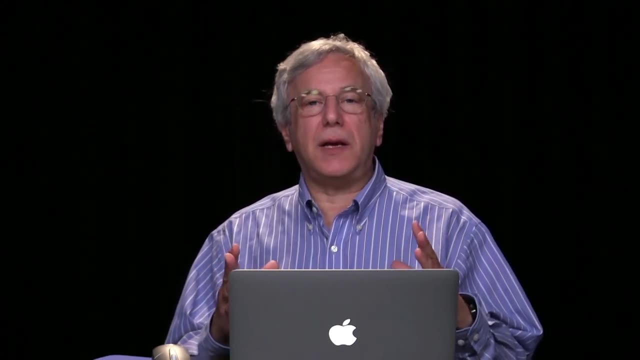 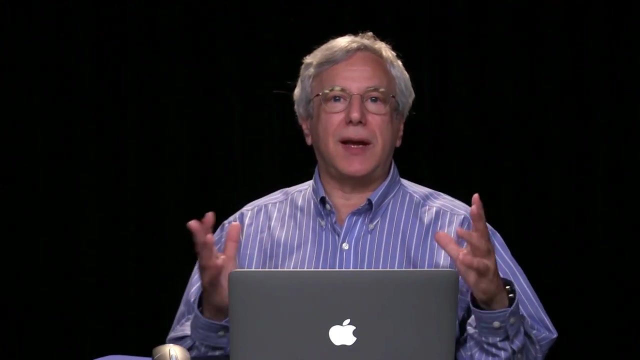 and we pack them together into something called a class or an object. And these data structures can be rather complicated. The account data structure may have 50 or 60 different fields. The window data structure may have a dozen fields. Who knows In functional programming? 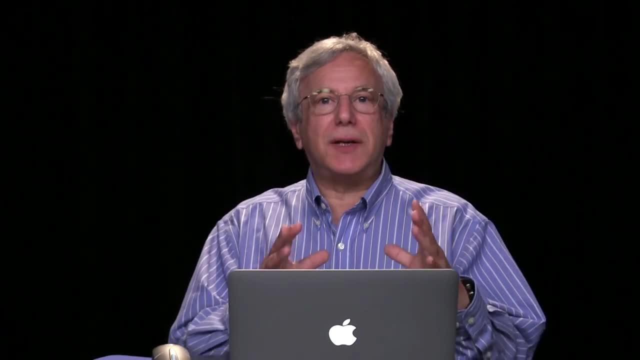 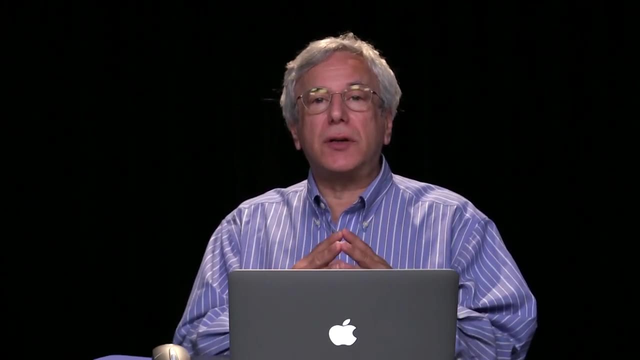 I like to focus on a specific data structure called a list. Turns out, a list is very, very versatile, So what I want to do is talk to you for a while about lists, And this whole chapter of the course is going to be about lists. 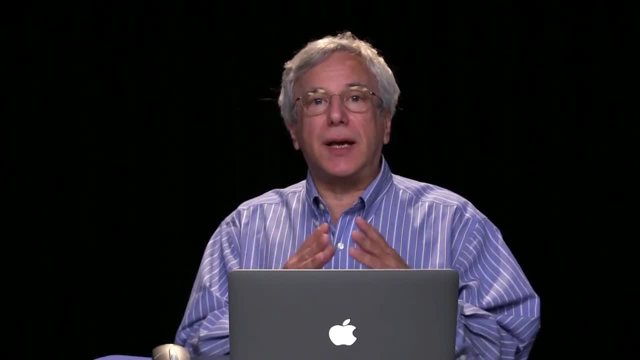 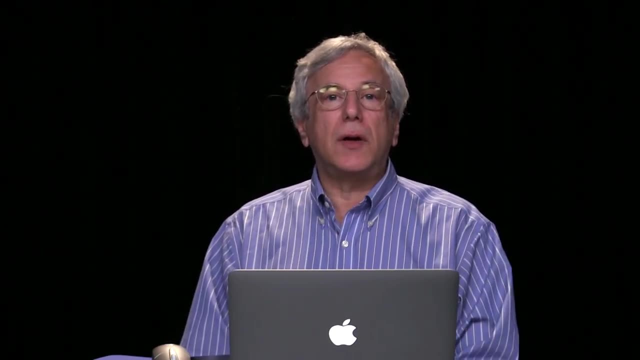 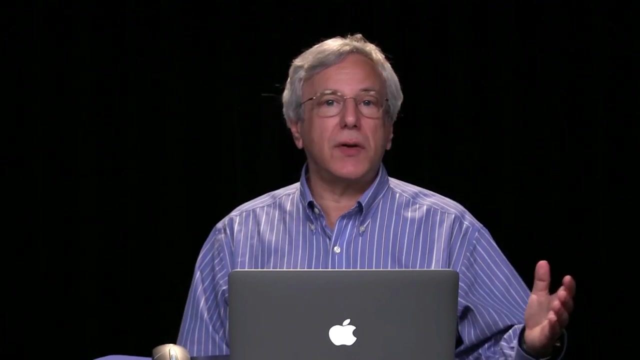 and what we can do with them. Interesting thing about lists: one of the really, really effective ways of dealing with a list is with recursion. Now, you may have seen recursion in other contexts, in other courses, in other reading. Sometimes recursion is scary. 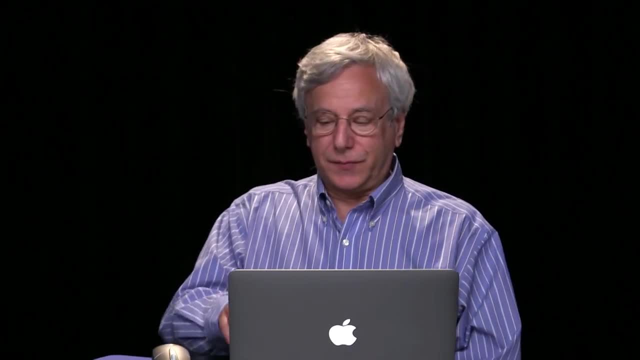 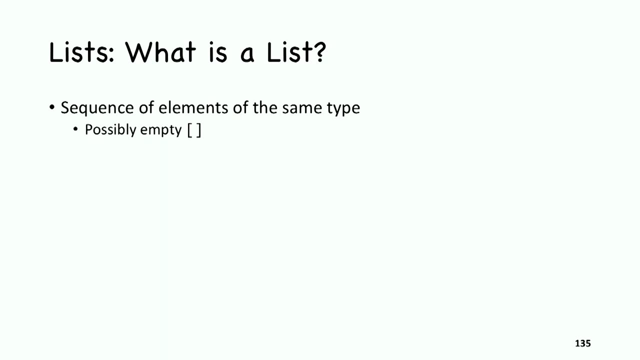 I'm going to try to make it unscary. Let's see how it works. A list is a sequence of elements of the same type. My first list. I'm going to start out with a list that has no elements. OK, sequence of elements of the same type. 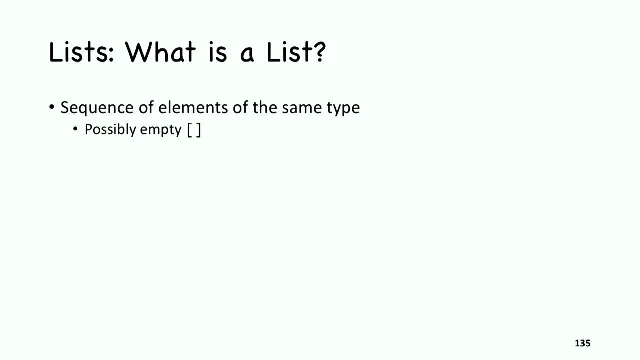 Yeah, maybe To denote an empty list, I'm just going to have square brackets- Open square bracket, close square bracket, nothing between them. That's a list with nothing in it. Well, that's a finite list. But on the next line, on the next slide, 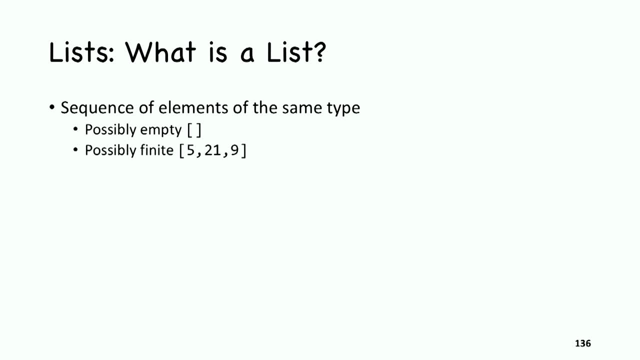 I have a finite list that doesn't have no elements in it, A finite list that has three elements in it: Five and 21 and nine. That's a finite list, All right, But not every one of my lists is going to be finite. 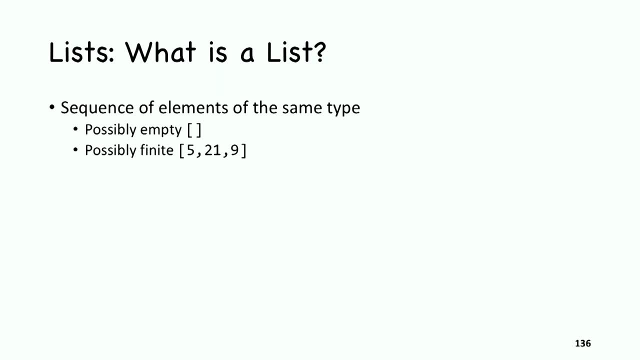 I showed you an infinite list earlier in the course. I want to remind you that such things exist. I can have an infinite list and in this infinite list I go out of my way to emphasize that it contains all of the even non-negative integers. 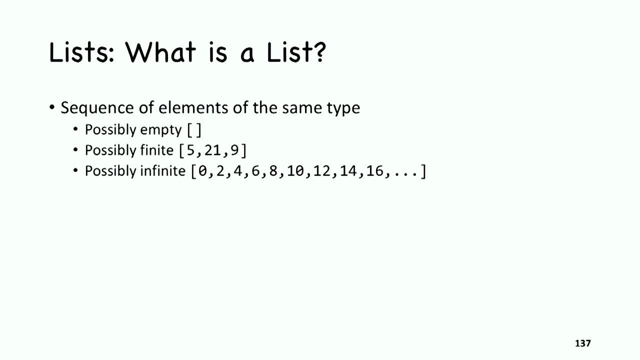 So it starts out with zero, then two, then four, and so on and so forth. Yeah, I admit it, I didn't have to name all of those things up to and including 16 to give you the idea. Maybe I became very exuberant when I created this slide. 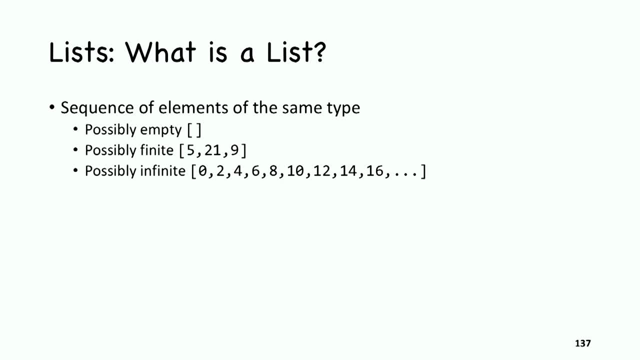 OK, Anyway, this is an infinite list. It has all of the even non-negative integers. You get the idea. Start with zero, two, four. But it's an infinite list. It's got an infinite number of elements in it. 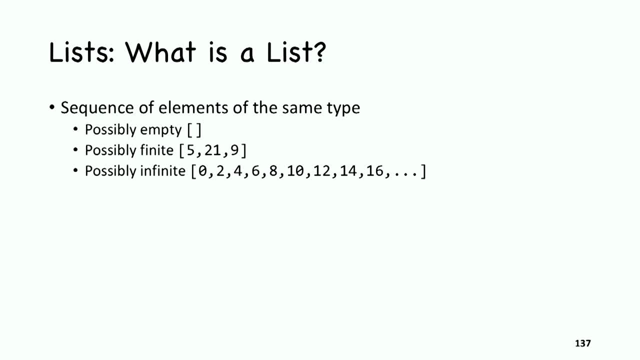 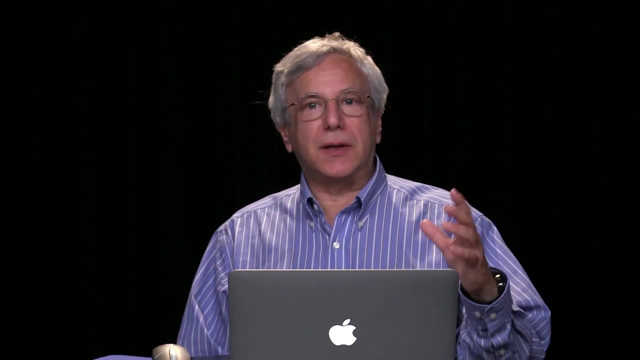 Now, if I'm going to deal seriously with lists, I need some functions that work on lists, And functional programming has some functions that date way back to the 1960s for operating on lists. They're absolutely the ones that are used very, very commonly all the time. 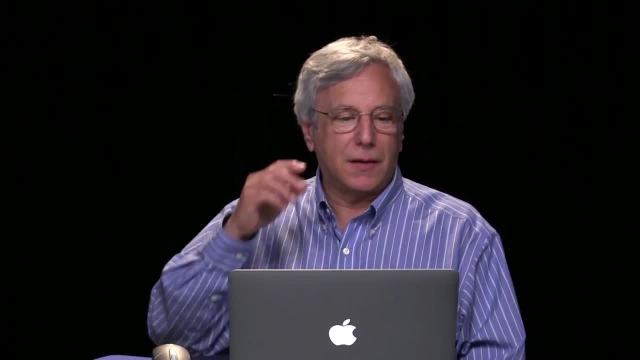 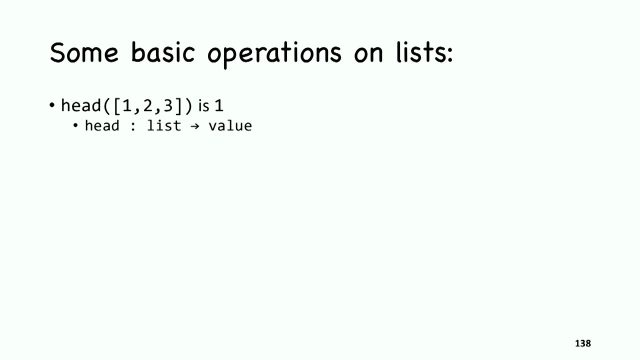 You'll find them in many, many different languages. So the first function that I want to define is the function called head, And the head of a list is simply the first element in a list. What kind of a function is the head function? 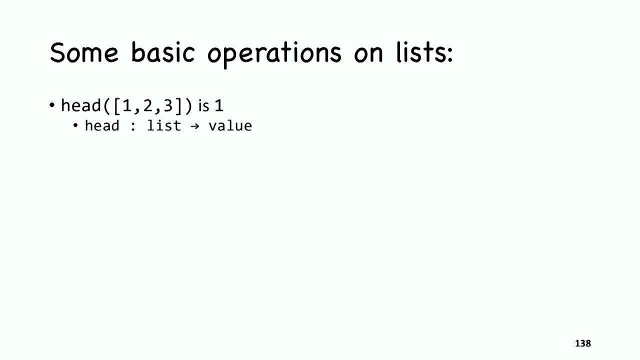 You might want to focus at the. Well, I know I want to focus. Here we go. The head is a function that takes a list and gives me back a value. In this instance, the head function takes the list: one comma, two comma three. 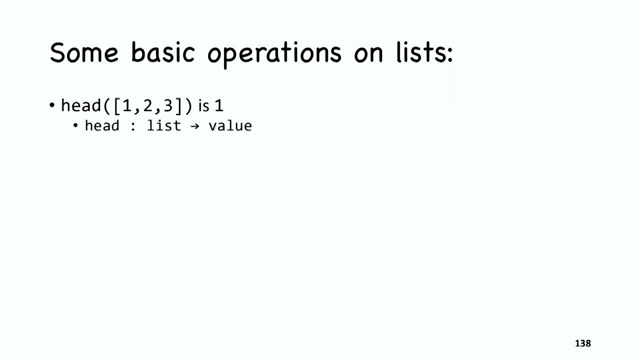 and returns the value that's at the very start of the list, the head of the list, the value one. Whenever I apply the head function to a list, I get back a value, one of the values that's in the list. I'm emphasizing the getting back a value. 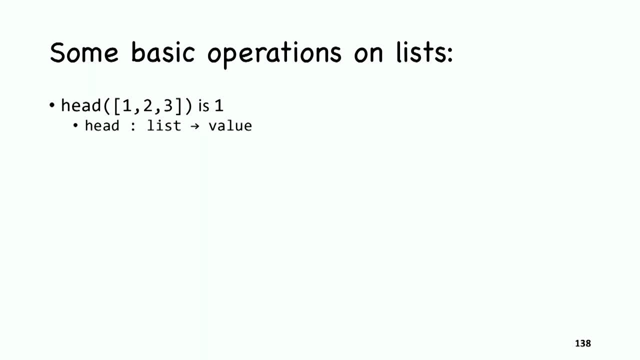 because the next function that I look at isn't going to give me back a single value. It's going to give me back another list. Here we go, It's the tail function. The tail function takes a list and it returns a brand new list. 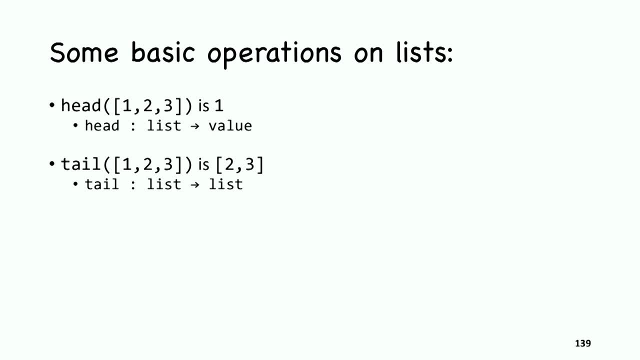 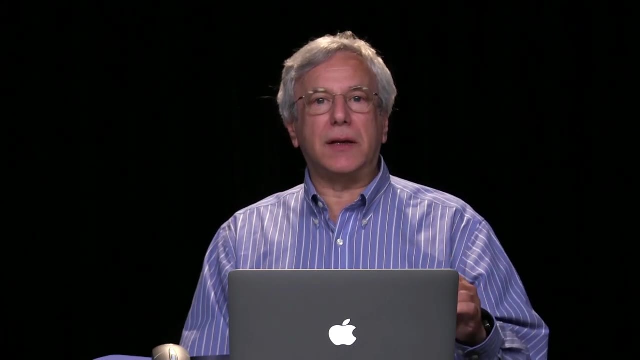 So the tail function starts with one, two and three and then ends up giving me the list that includes just two and three. Now I have to emphasize whenever I call the head, the head function, if the list has any elements in it. 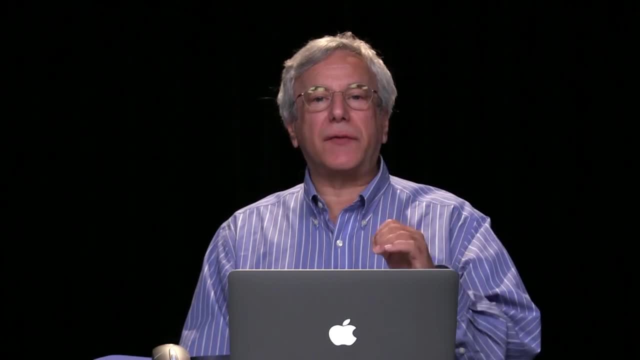 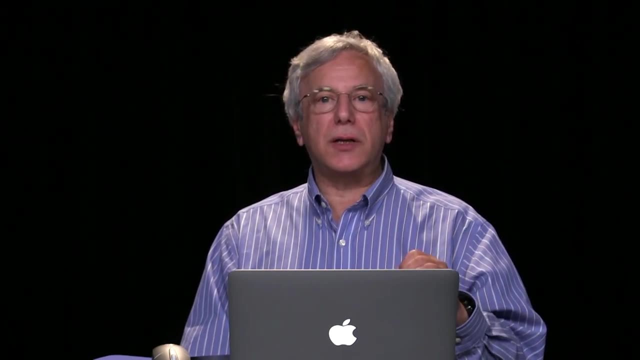 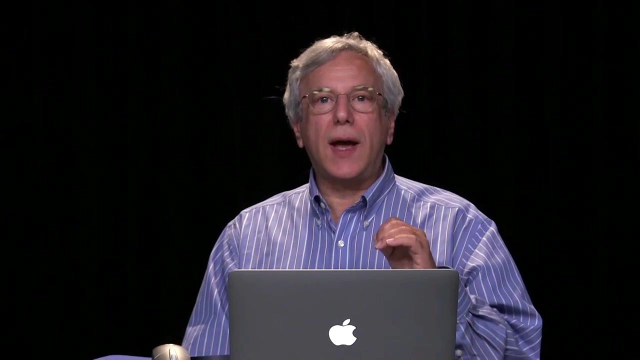 the head function gives me back the very leftmost element, the initial element in the list. It gives me back just one element. The tail function, in contrast, always gives me back a list. So if I start with a list with two elements, 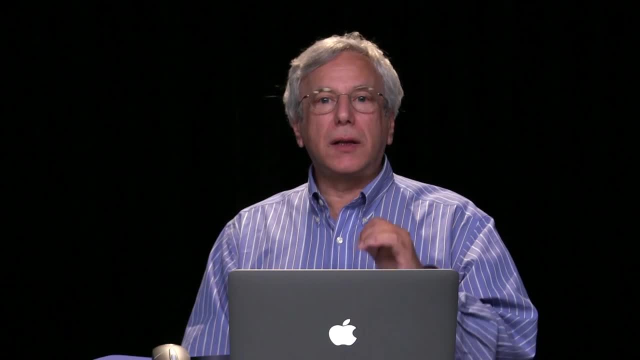 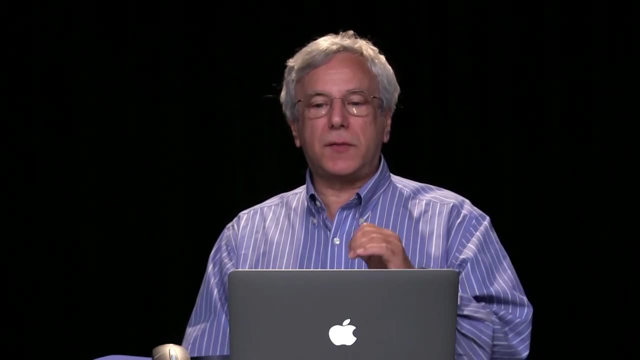 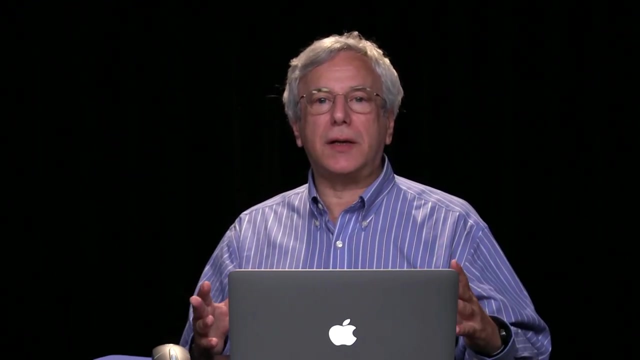 then I get back from the tail function, a list containing only one element. The head gives me a value, The tail gives me a list, And if I take the head and the tail together, I can reconstruct the entire list. Hey, let's do that. 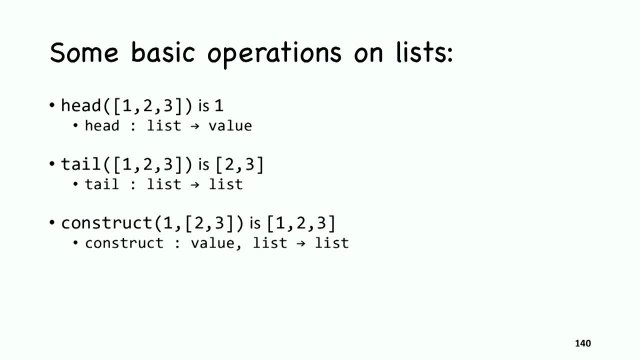 Let's create a function called construct. Construct is the opposite of head and tail. The traditional language for construct is to call it cons, But I kind of like the word construct. The word construct reminds me that I'm constructing a list from its two parts. 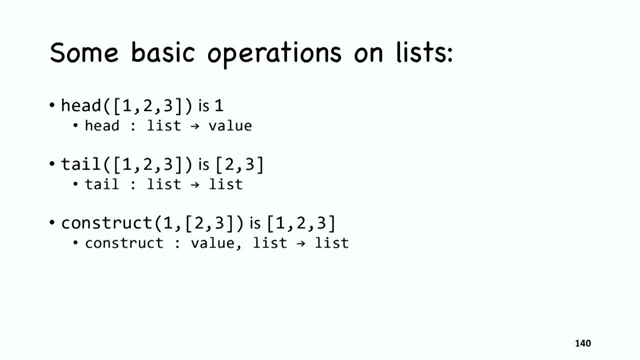 from the head and from the tail. So if I start with a value one, a single value one, and a list two, three, then if I call construct on those two arguments, I get back a brand new list with the values in it: one, two and three. 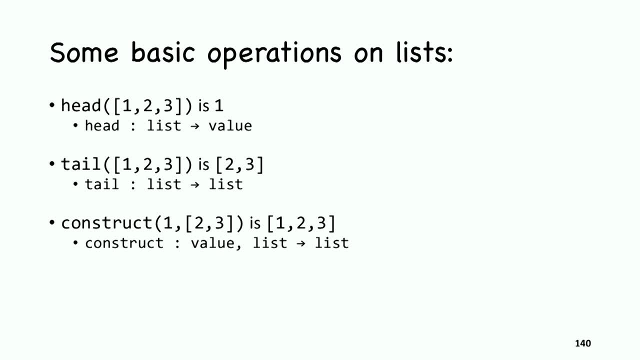 That's what construct does? It reverses what I did when I chopped a list into a head and a tail. So now I've got these three functions that I can use to pick out the first element in the list and, if I want, 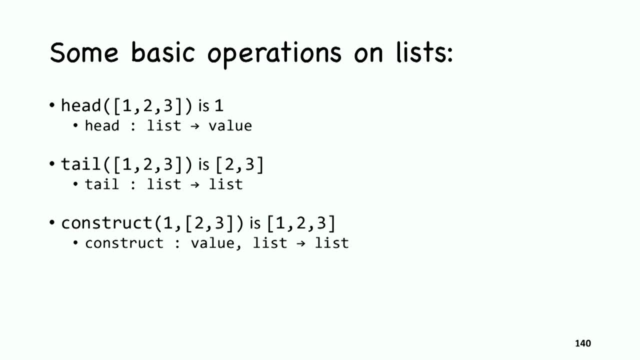 to put that first element back into a list. It's a very powerful idea. I'm going to give you one more function and it's not part of this traditional triumvirate, but it's kind of useful. I'm going to call it concatenate. 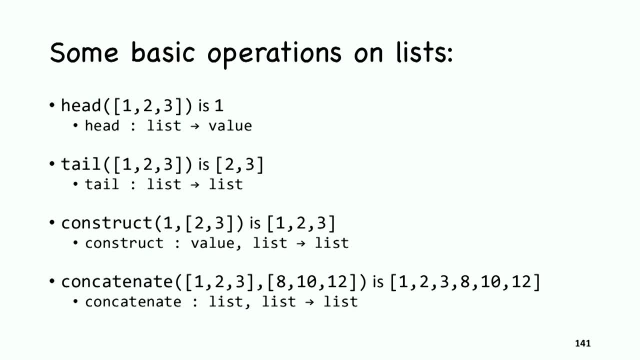 and it's closely related to another function that I'm going to call flatten. But let's just take a look at what I call concatenate here. I'm going to make my concatenate function in this case. take two lists. In this case it takes the list one, two, three. 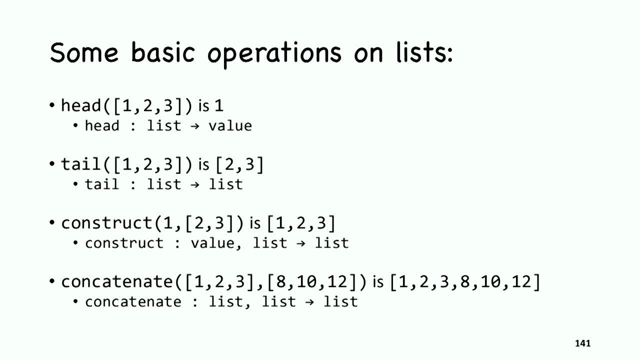 and the list eight, ten, twelve. When I concatenate those two lists together, I get a brand new list, and the new list simply includes the elements from both the first argument list and the second argument list. Okay, so the concatenate function takes two lists. 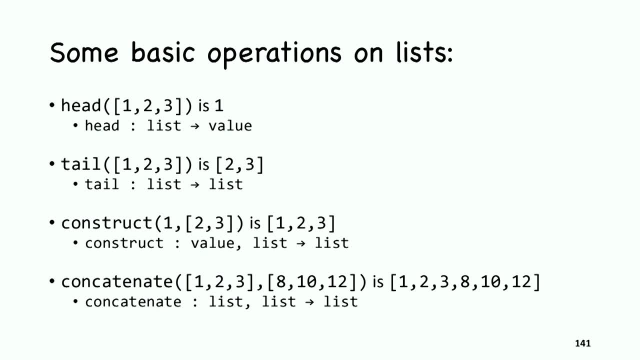 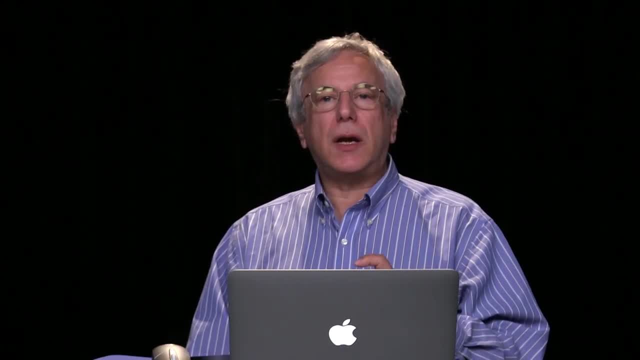 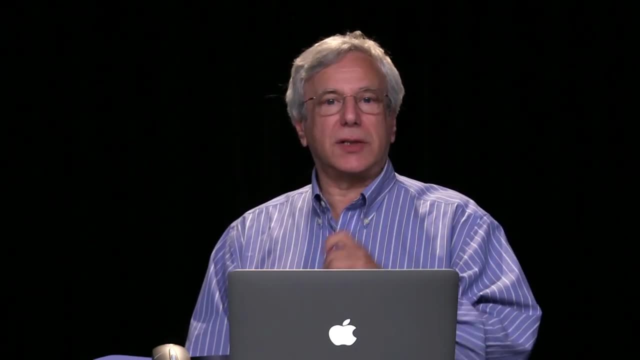 and gives me a brand new list. Okay, four functions, good stuff. What I want to do in the next section is take these four functions and use them in order to do some very, very, very tricky but very, very nice recursive operations on lists. 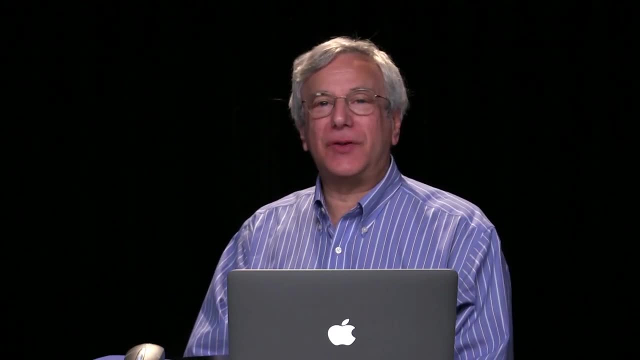 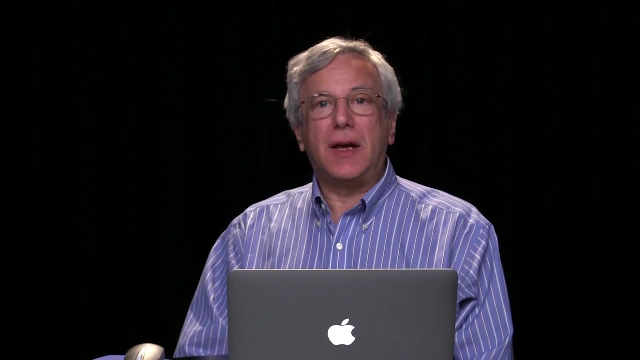 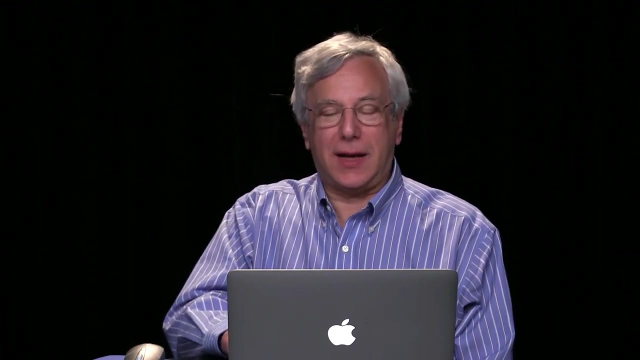 In the previous section we introduced the notion of a list, talked about some important functions that are good for working with lists. Now I want to use those functions to do recursion on lists. Are you ready? Yes, you are. Let's do a really quick review. 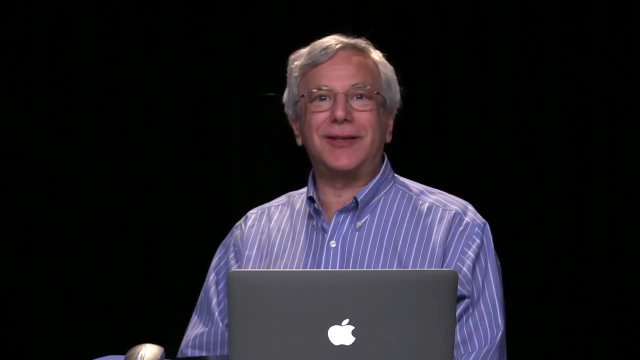 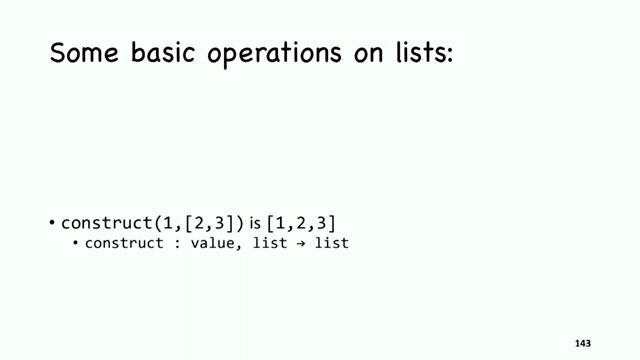 of one of those functions. One of those functions is called construct, and when you call construct on a value and a list, you get a brand new list. All right, I want to create just a nice shorthand notation for that construct function. I want to turn it into something. 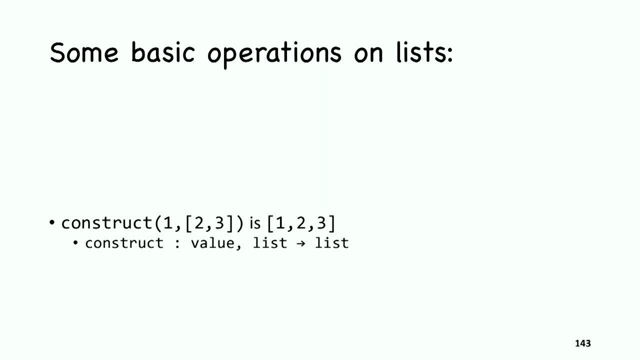 that looks like an operator. So instead of using the word construct and having some parentheses, I'm going to kind of make it look like a binary operator, the same way you'd use a plus sign or a minus sign or something like that. So I'm going to use two colons to say: 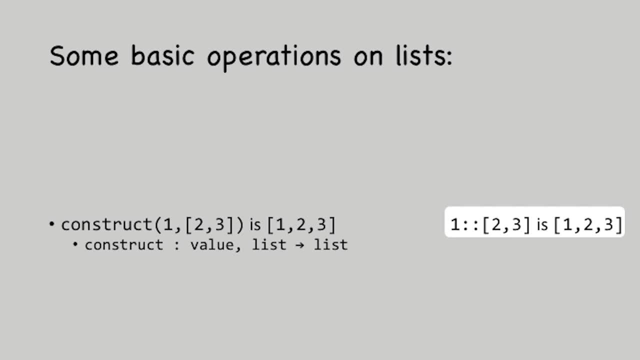 for example, that I want to construct the two arguments 1 and the list 2, 3.. And when I do that construct, those two colons mean construct, when I do that construct on 1 and on 2,, 3,. 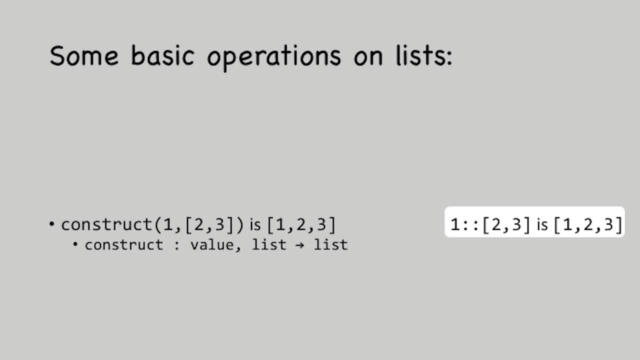 I get back the constructed list 1,, 2, 3.. Okay, Just a different way of notating the construct function. What do I get for this? What I get for it is that I can use those two colons as a sort of a pattern matching scheme. 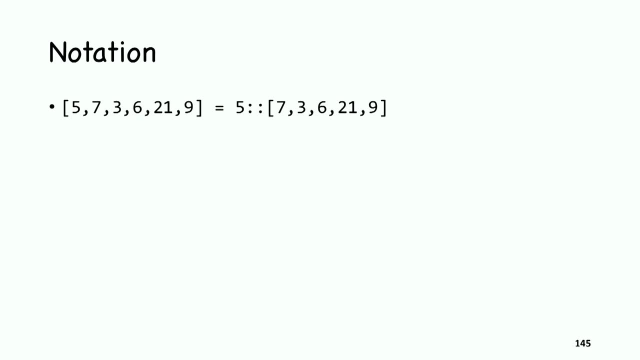 Let's have a look: 5,, 7,, 3,, 6,, 21,, 9 is the same as 5 constructed with 7,, 3,, 6,, 21, 9.. Okay, That's one way of looking at it. 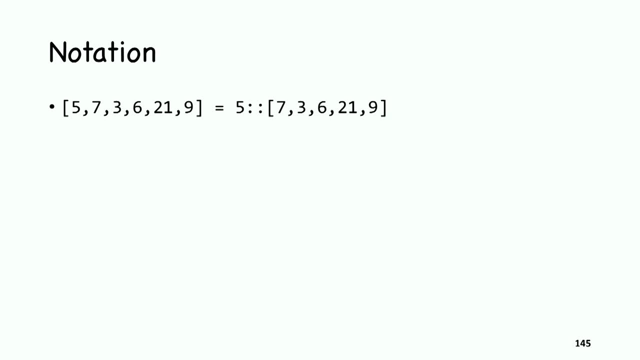 Something that you might not have thought of is that if I construct a number such as 8, with the empty list, then what I get back is a list containing only the number 8. And that's going to be very important, Okay. 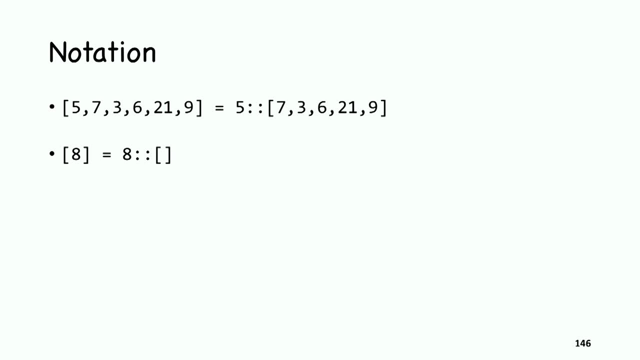 The list containing the number 8 is the same as applying the construct function or the construct operator to the head of the list, which is just the number 8, and the tail of the list, which is the empty list. All right, Now I want to do something called pattern matching. 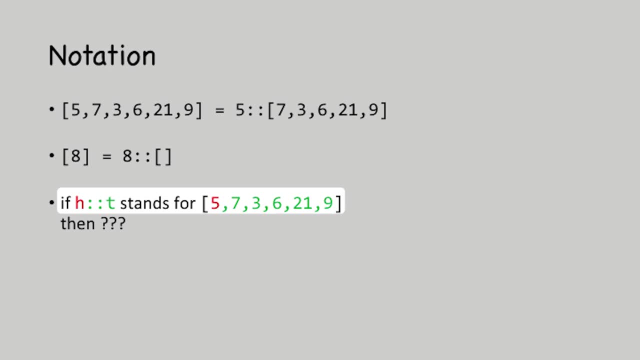 So if I write down H, colon, colon T, if I want to try to match that with the list 5,, 7,, 3,, 6,, 21,, 9, then I can make a match. And what does it mean to make a match? 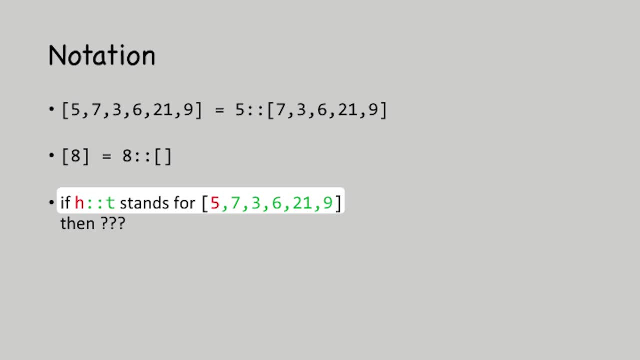 It means that when I identify that list with the notation H, colon, colon T, then H stands for the number, the plain old number 5, and T stands for the rest of the list: 7,, 3,, 6,, 21,, 9.. 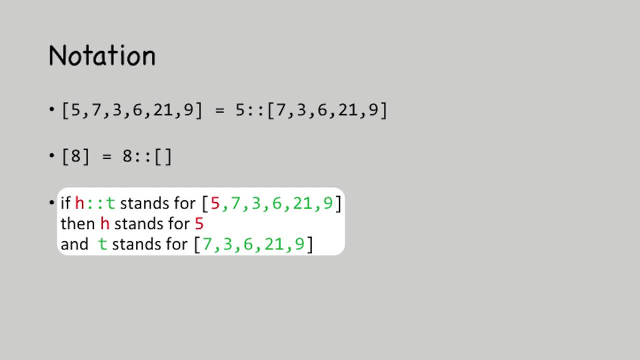 Of course I'm using H because I'm trying to suggest the word head And I'm using T because I'm trying to suggest the word tail. But I don't mean to say that I'm applying functions here, I'm just making a match. 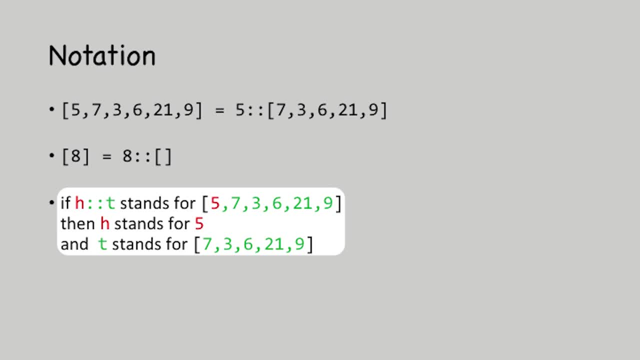 I'm just saying, if the list 5,, 7,, 3,, 6,, 21,, 9 can be notated as H, colon, colon T, then here's what the H part stands for. It stands for the 5.. 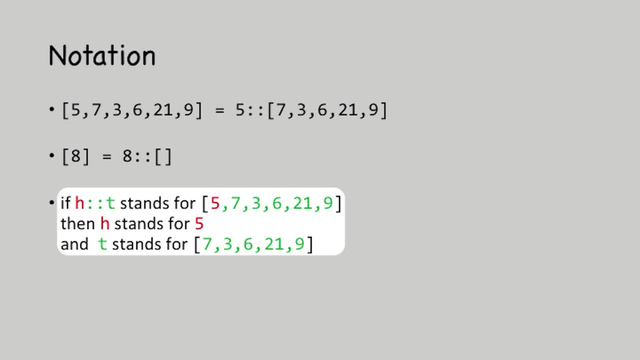 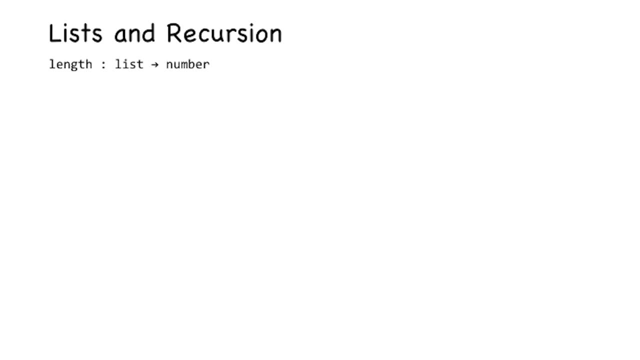 And here's what the T part stands for. It stands for 7,, 3,, 6,, 21, 9.. Nice colors, eh, Looks like Christmas time. Okay, here we go. Now I'm going to do some recursion. 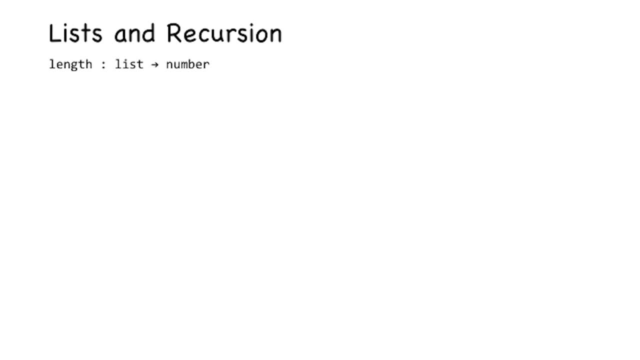 So I'm going to create a length function, And the length function takes a list and returns a value. The value, of course, is going to be the number of elements in the list, And you can say, yes, the language that I use. 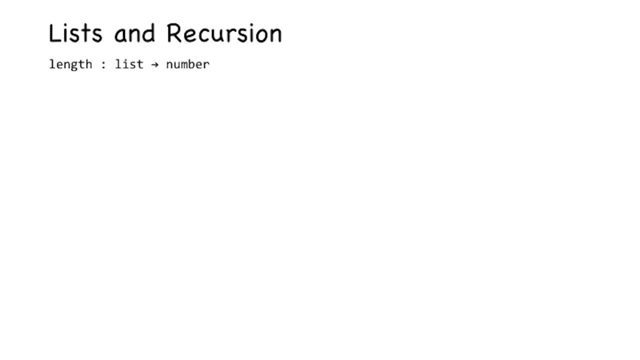 has its own built-in length function And then I can do the length function with some sort of a loop, or I can even keep a counter and add one to that count value whenever I add one more element to a list. But I want to do this with recursion. 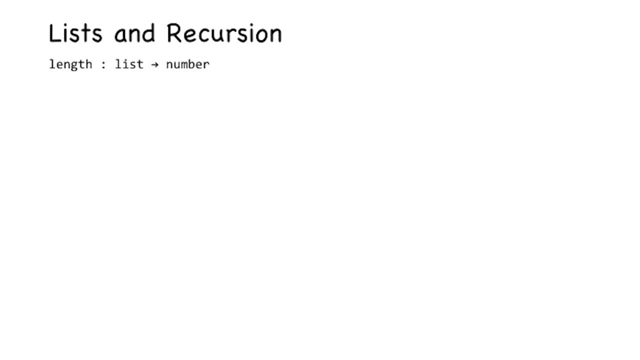 Let's see how I would do it. In order to do it recursively, I'm going to have two formulas for defining what I mean by length. The first formula says: if I ask for the length of an empty list, I get zero. And that formula, the formula in blue, 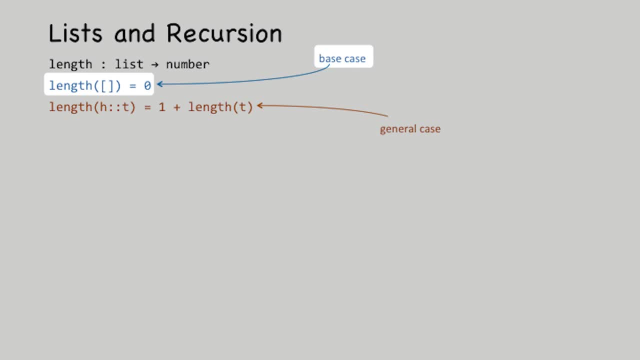 is called the base case. So the base case says: if I start with a zero length list, its length is zero. Okay, Base case. I'll tell you in a minute why I call it the base case. The second formula, the formula in brown. 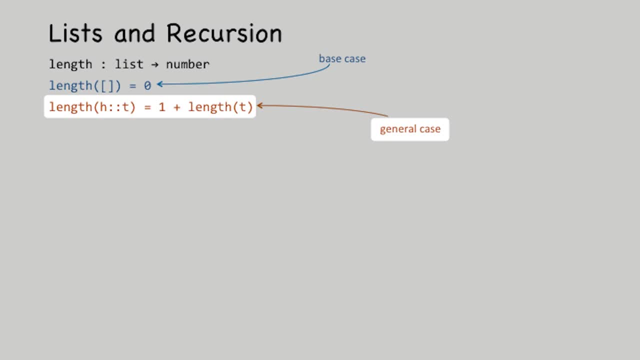 says that if I have a list that I can match with the H, colon, colon, T pattern, then how do I calculate that length's list? Well, I find the length of the T part and I add one to that. All right, That's called the general case. 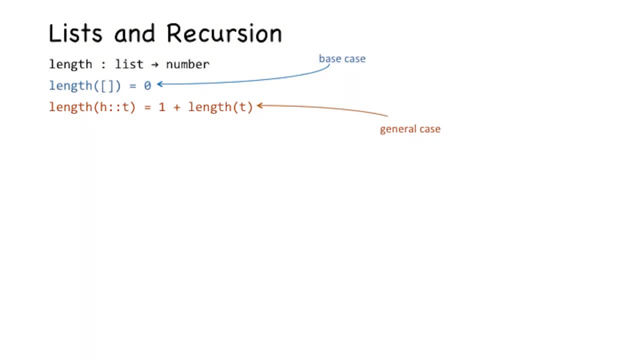 So I've got two formulas to define what I mean by length. I've got a base case formula and I've got a general case formula And whenever I use recursion I'm going to have at least two formulas, maybe more, But I've got to have a base case. 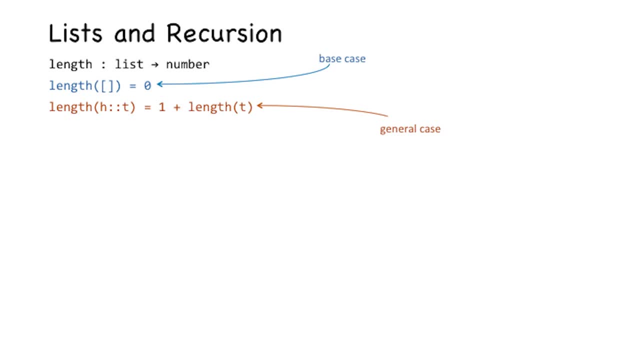 Why do I have to have a base case? Well, let's take a look at the general case. The general case says that I'm defining the length of a particular list in terms of the length of a smaller list: The length of H colon, colon T. 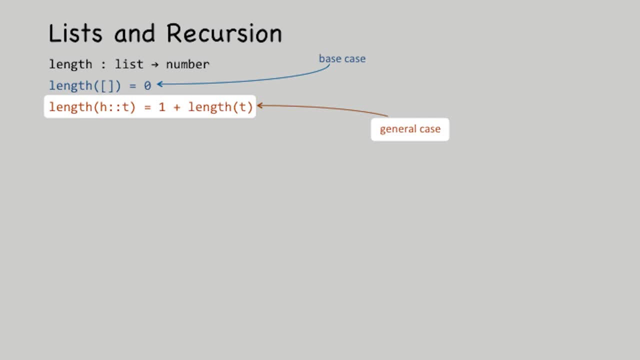 is defined by examining what's the length of T. Now, if I just wrote down the general case and never wrote down the base case, then I would be defining the length of a list in terms of the length of another list which would have to be defined. 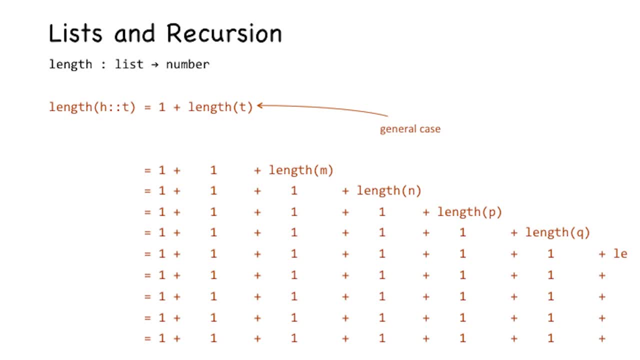 in terms of the length of another list, which would have to be defined in terms of the length of yet another list, And without a base case, this call to the length of another list would be an endless sequence of calls. If I write down the formula in brown: 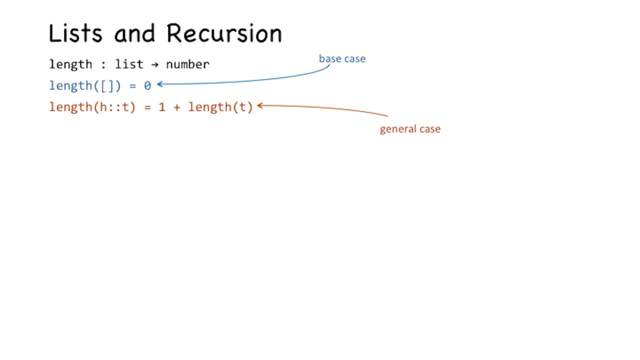 the general case. and then I say, okay, when you get to the situation where you have the empty list, you can stop making further calls to length. You can just say 0.. If I have this general case and the base case, 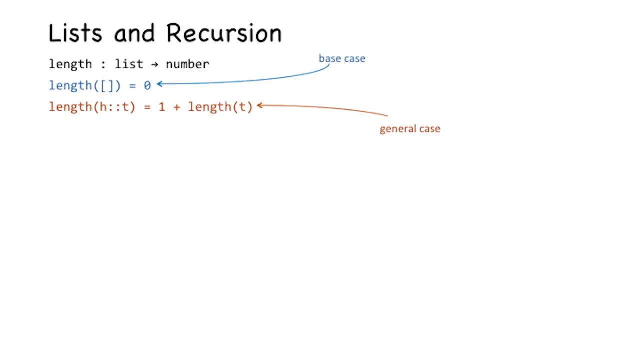 then I have enough in order to determine the length of a list. Let's see it in action. Let's start by trying to find the length of the list that contains 5 and 7 and 4.. I don't know if you can see it. 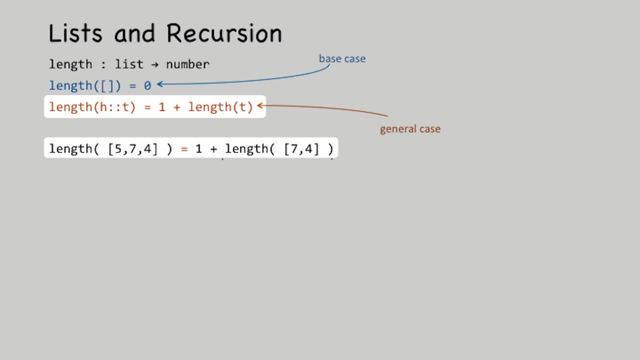 but I made that little equal sign between the two halves of that formula. I made it brown-colored to suggest that I'm applying the general case. I'm saying the length of 5,, 7,, 4 is by virtue of the general case. 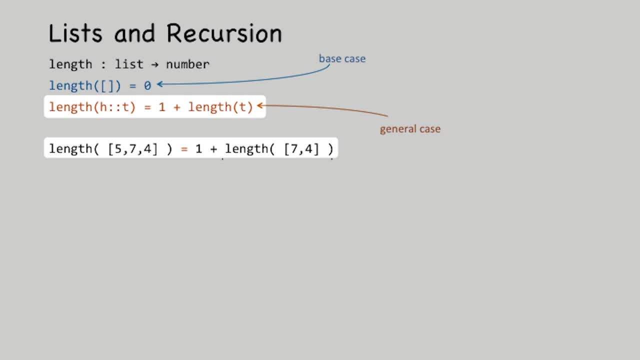 1 plus the length of the T part of the list, the 7, 4 part of the list, And of course it looks a little bit like a circular definition. I'm defining the length in terms of another length, But remember that I've got an advantage here. 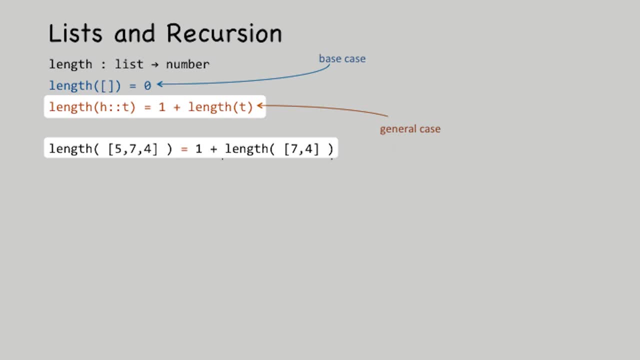 The length of the list of the 7, 4 part is trying to determine the length of a list that's a little bit smaller than the list that we started out with. Okay, but I've still got some work to do. I've got this thing where. 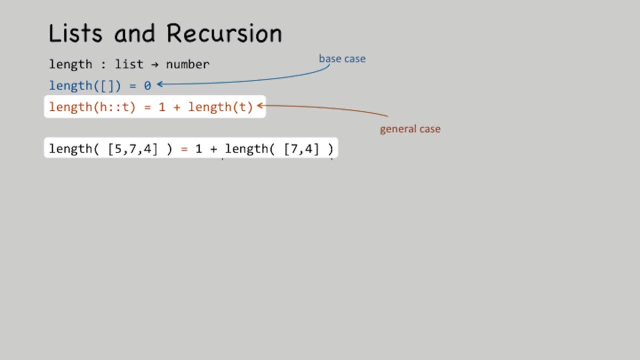 I'm trying to find the length of the 7, 4 list. I've got to apply a formula. Oh, I wonder what formula I know. Since 7, 4 is not an empty list, I'm going to use the general case. 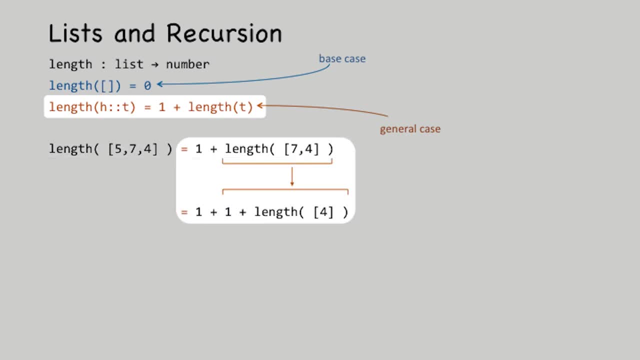 The length of 7,. 4 is, according to the general case, 1 plus the length of the T part, And in this case the T part is just plain old 4.. Okay, I've made progress because now I've got the length. 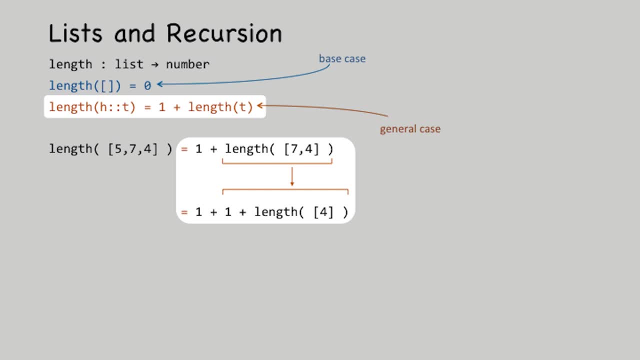 of an even smaller list, the 4 list, the list with only 4 in it that I have to deal with. Okay, So I've gone and substituted length 7, 4 for what the general case says to substitute for it. 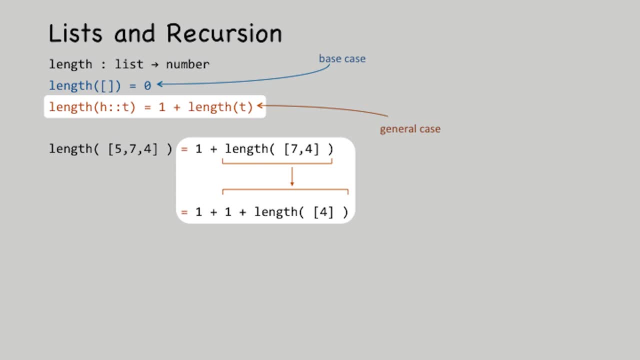 1 plus length of 4.. And in the meantime, I'm taking that leftmost 1, that initial 1, and, just remembering it, dropping it down to the next equality part of this whole computation. All right, now I've still got a problem. 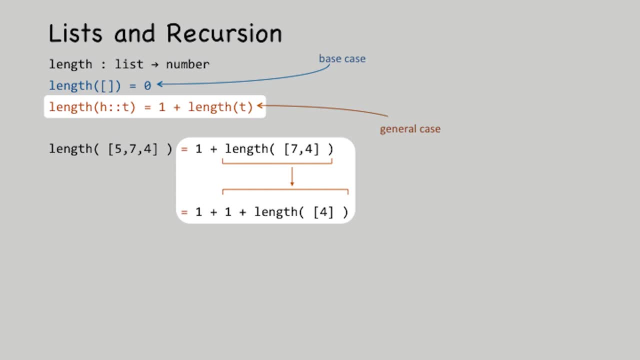 I've still got to compute length of brackets 4.. Well, what do I do then? Well, hmm, let's see, Is 4 brackets 4, is that the empty list? No, it's not Okay. So when I don't have the empty list, 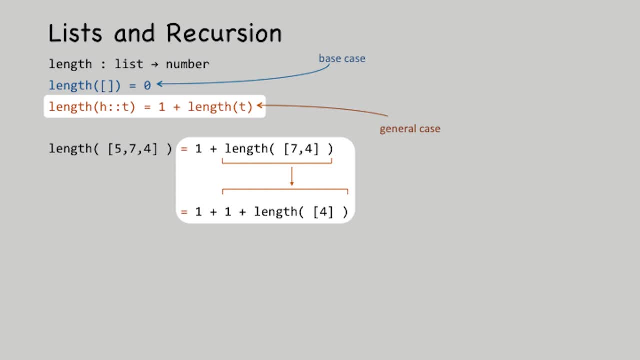 I've got to apply the general case. I'm starting off with 1 plus 1.. I'm going to keep that. I'm just going to recopy it. But in place of length, brackets 4,, I'm going to substitute what I'm told to substitute. 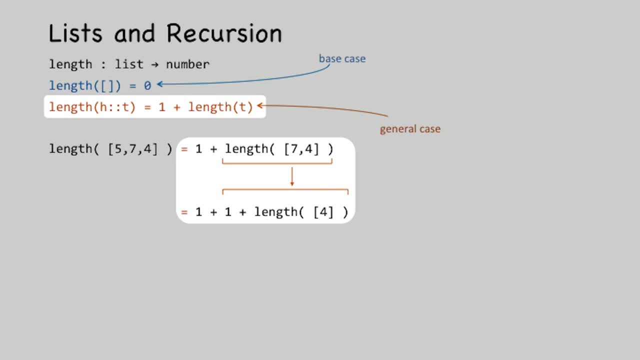 by virtue of the general case formula. Here it is Now I've got my original two 1s, but because of the general case formula I have an additional 1 plus the length of something, And in this case that something right. 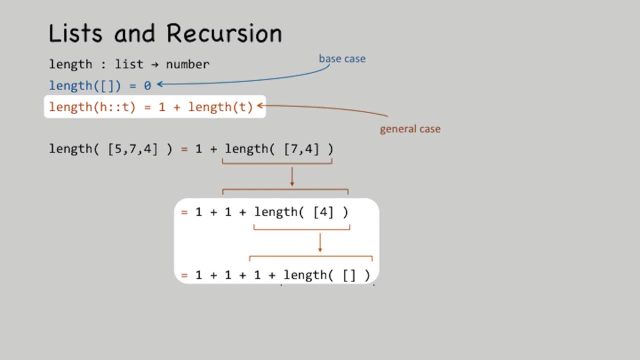 is the T part of the list that includes only 4.. Now, when you're taking the tail of a list that has only one element, that tail is just the empty list. So there we go. Now I'm trying to compute the length of the empty list. 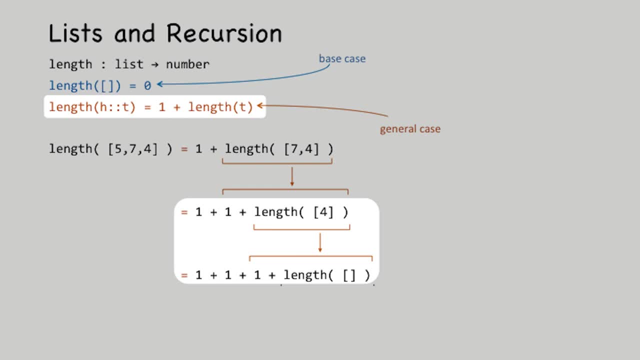 Hmm, I've still got a length that I have to figure out. However, now the length that I'm trying to figure out is the length of the empty list. I don't have to figure out the length of the empty list by finding the length of something else. 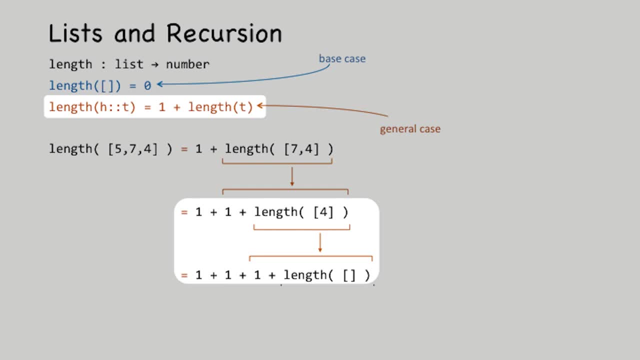 By virtue of the base case formula, I can just substitute 0 for the length of the empty list. So I recopy my 1s and I use the base case to substitute 0 for the length of the empty list, And what I end up with is: 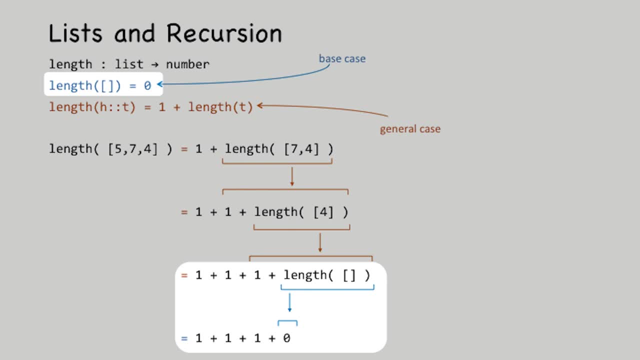 1 plus 1 plus 1 plus 0.. Well, I don't have to do any more length calculations. 1 plus 1 plus 1 plus 0, I know what that is. That's 3.. I'm done. 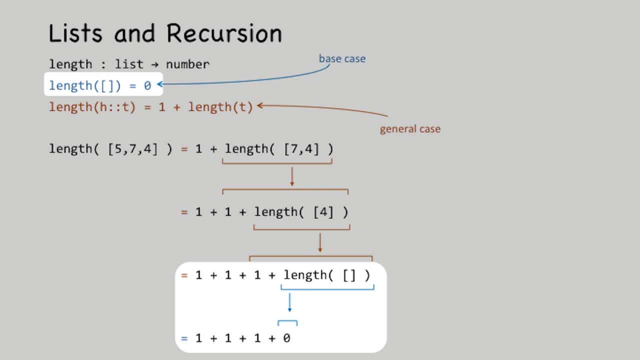 Okay, So I've used recursion in order to find out how many elements there are in a list. It's yeah a lot of work to do in order to do something that you can just eyeball on the slide, But it's also a good introduction. 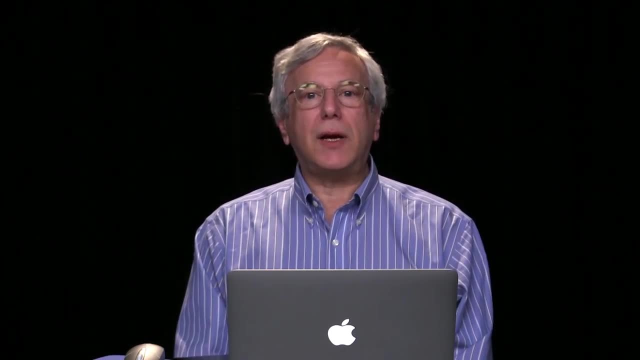 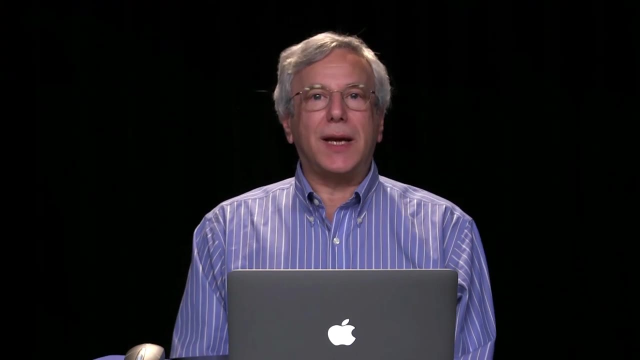 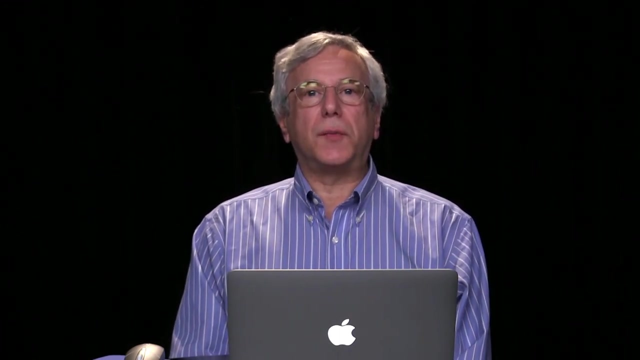 to this notion of having a general case and having a base case, repeatedly applying the general case until you get down to the base and eventually getting yourself an answer. Okay, recursion is used all over the place with lists and, in fact, recursion is used. 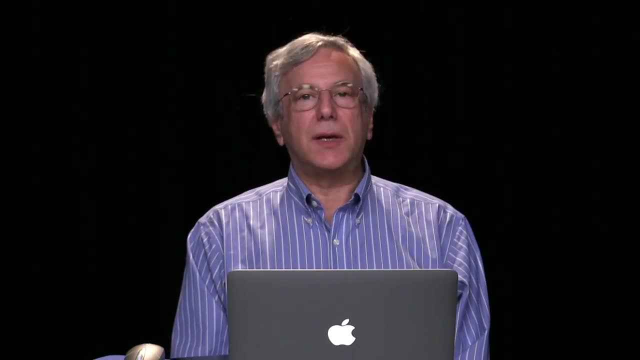 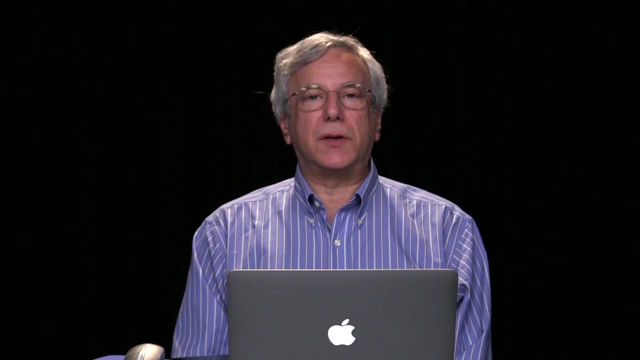 all over the place in many other kinds of problems. It's a really good thing to understand recursion. So I don't want to stop here. I want to do a few more examples of recursion, and I'll do them in the next segment. 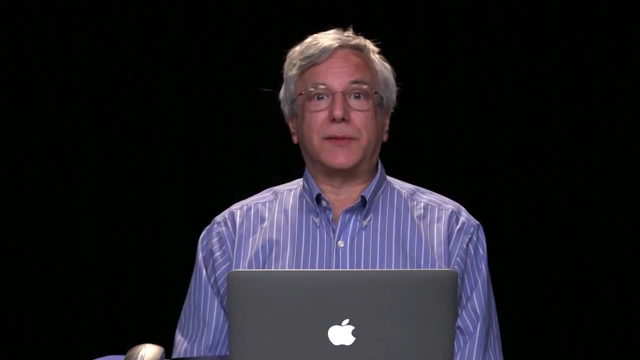 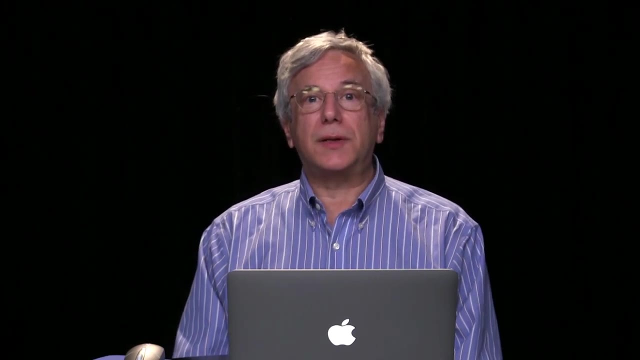 You've heard the old joke: how do you get to Carnegie Hall? Practice, practice, practice. The more practice you get with recursion, the better you're able to deal with it. So let's see a couple more examples. Of course, these examples of recursion. 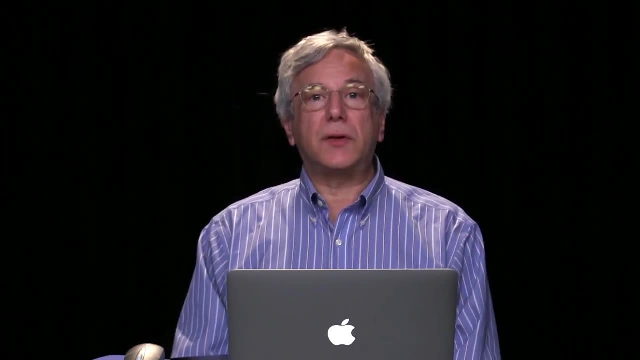 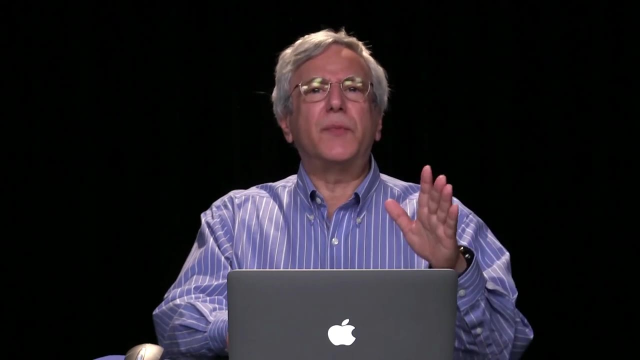 will use lists. Other examples of recursion may use other kinds of structures, But in this course I'm focused particularly on lists And I'm going to do pretty simple operations on lists. nothing fancy I'm going to do. well, let's say, 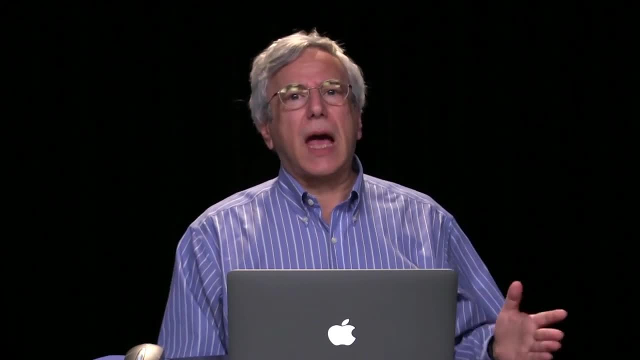 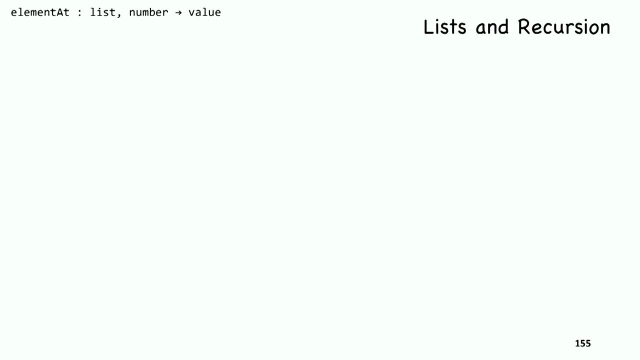 element at. So the element at function, as I define it, is going to take a list and a number and give you one of those values from the list. For instance, if I have a list that includes 21,, 84,, 5, and 99,, 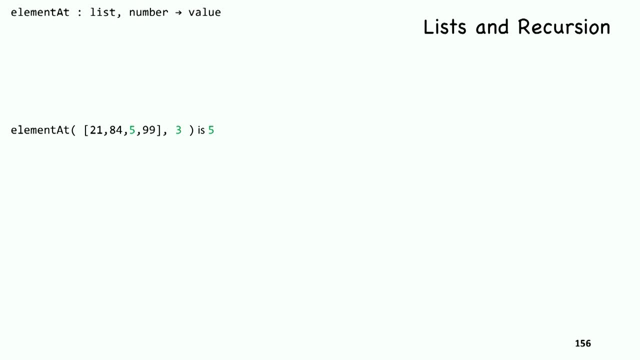 and I ask for the element at 3,, that's position 3, then it's going to return the value 5 for you. Now, sometimes with element at, you want to start by indexing with 0. I'm just choosing not to do that. 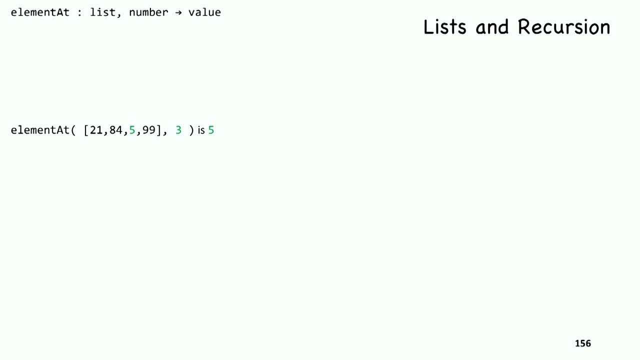 No particular reason, just decided to set up element at this way. If you like setting up your element at, with the 21 being called the 0 element and the 84 being called the 1 element, that's up to you. It just takes a little bit of tinkering. 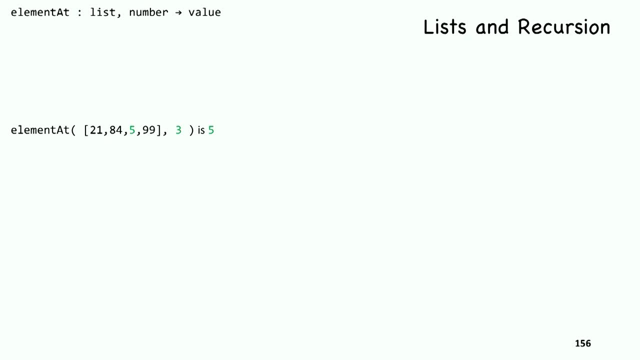 to modify my formulas. All right, I want to define element at recursively And to define it recursively once again. I'm going to have a base case and a general case. Let's take a look at them. If in the base case, 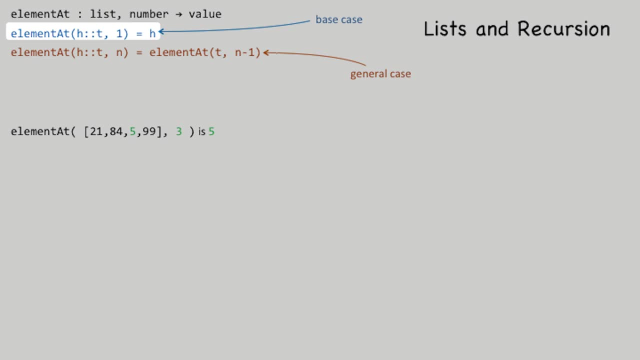 I'm looking at element at 1, the first element in the list, then I'm just going to take the head of the list And no further work has to be done. But if I want to take the element at the nth position in the list, 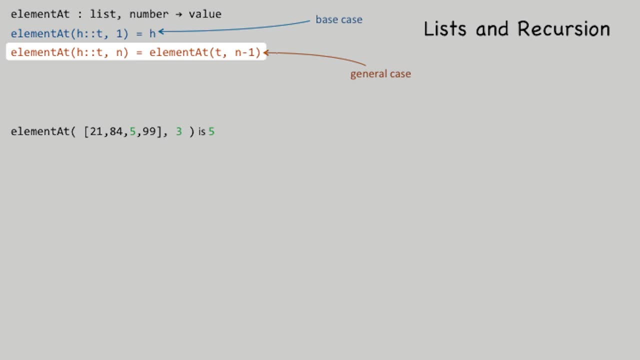 the third position, for example, then what I'm going to do is I'm going to chop off the head of the list. That sounds drastic. I'm going to take away the head of the list and just get the tail of the list. 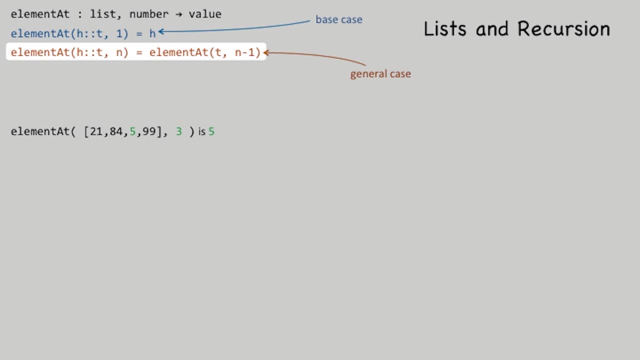 And in the tail of the list I'm going to look at the element at the n minus 1th position. So that's the general case And once again the base case says: in order to compute element at, I just do it and I get an answer. 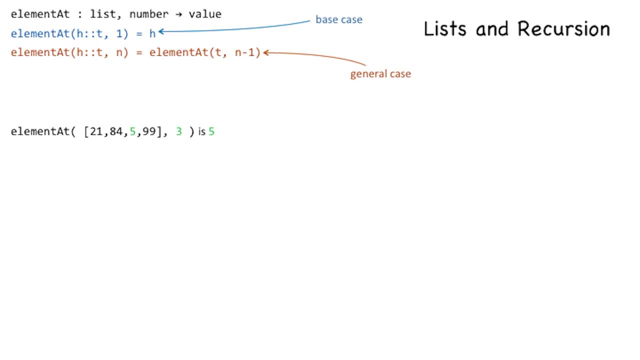 I get the head. The general case says, in order to compute element at, I have to compute element at for something else, For a slightly smaller list, for a list that includes only the tail. Again, what I want to do is trace through this to show you. 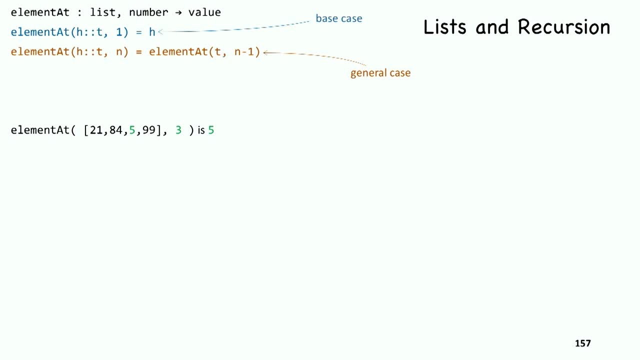 hey, it really does work. I've seen students be amazed when they saw how this worked. It's very satisfying to see people be amazed at recursion. Okay, I'm going to start off by trying to find the element at the third position in a list: 21,, 84,, 5,, 95.. 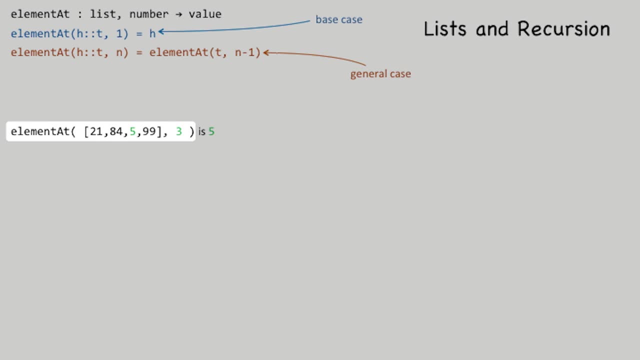 Well, I'm going to use my general case And for the general case I'm going to go from the original list with four elements to the tail of that list with only three elements, And I'm going to take my number 3 and subtract 1 from it and get 2.. 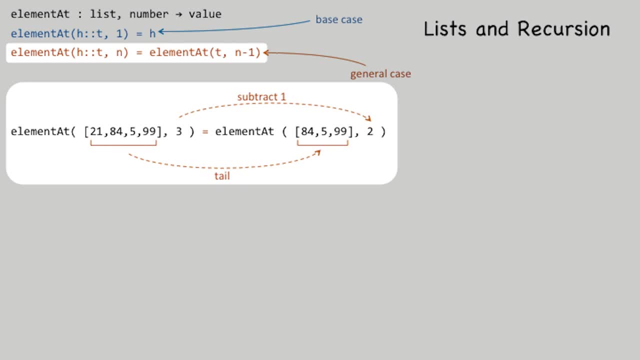 So, using my general case, I started off with having to find the element at in a list of four things, And I'm going now to find the element at in a list of three And, nicely enough, that number 3 got reduced to the number 2.. 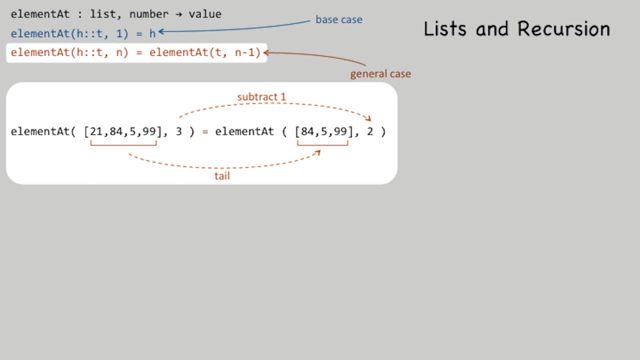 Eventually it's going to get down to 1, and then I can apply the base case. All right, let me try that. I'm now looking at the formula on the right-hand side of the expression, on the right-hand side of the equal sign. 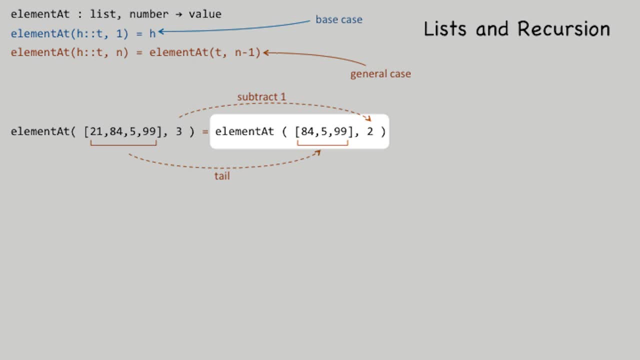 element at 84,, 5,, 99, and I'm looking for element number 2.. Okay, let's continue. I apply the general case, And the reason that I apply the general case is because if I'm looking for element at 2,, 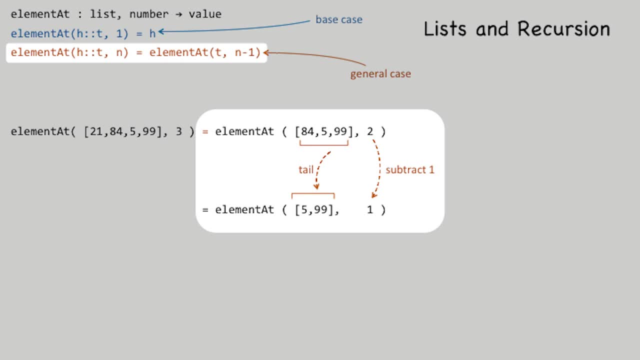 the general case applies and the base case does not. The base case doesn't apply because I'm looking for element at 2.. I'm not looking for element at 1. So I apply the general case. I subtract 1 from 2.. 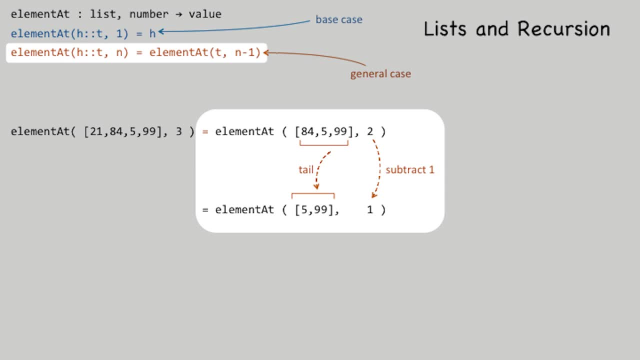 And I take the tail of 84,, 5, 99.. When I take the tail of 84,, 5, 99,, I get just 5, 99.. I've applied the general case. Okay, what have I done? 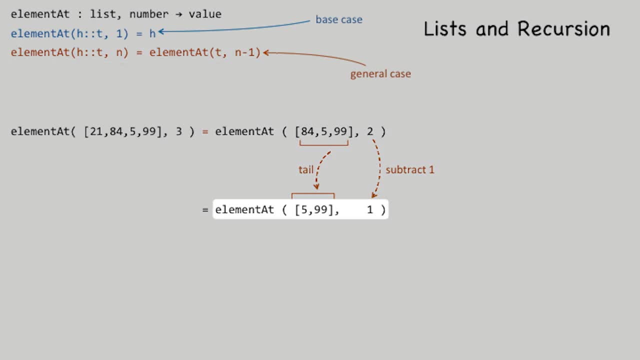 I've said that to find the element at 2, I have to find the element at 1 of some other list. But the nice thing now is finding the element at 1 is easy. And the reason that it's easy is because 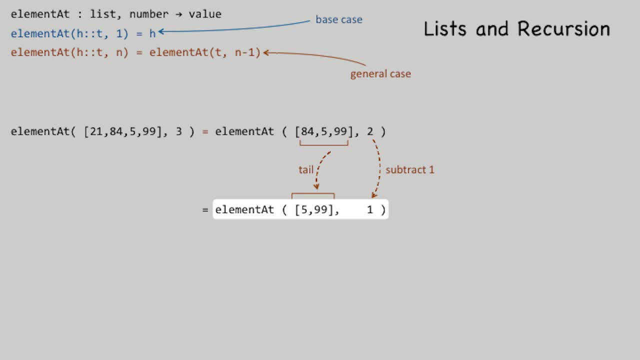 finding the element at 1 matches with the base case. To find the element at 1 using the base case, all I do is grab the head of the list that's in my element at function, And the head of that list is 5.. 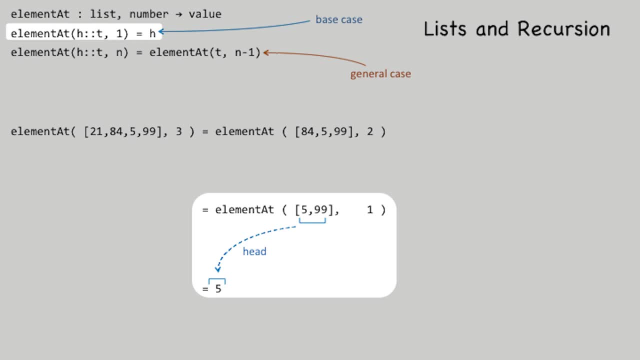 Fair enough To take the element at 1,. I apply the base case, I take the head of the list 5,, 99, and I just get the number 5.. Wow, what that's given me is eventually, after a few recursive calls, 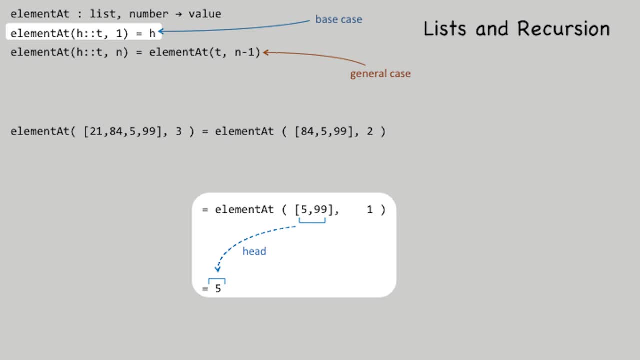 it's given me the element at 3 in the original list. I've done it. I've solved the problem by successively applying the general case until I could get down to the base case and then applying the base case in this situation once and for all. 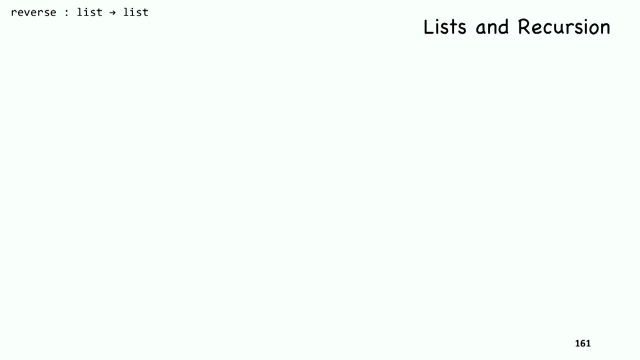 All right, let's take one more example. I want to find the reverse of a list, So I want to start with x y z and end up with z y x. I want to start with 1,, 2,, 3,, 4,. 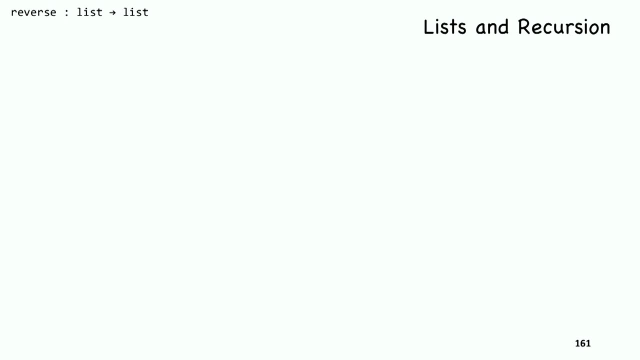 and end up with 4, 3, 2, 1.. How am I going to do that? I'm going to have a base case and a general case. Boom. The base case says that if I want to reverse the empty list, 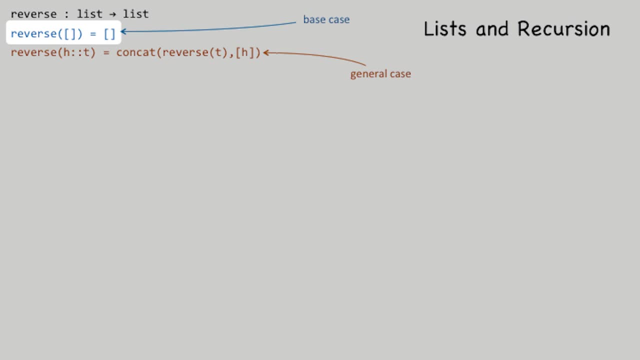 I don't do anything with it, I just get the empty list. No sense in trying to reverse nothing, You just get nothing. Oh, that's cool. How do I reverse a list with a head and a tail, With h, colon, colon, t? 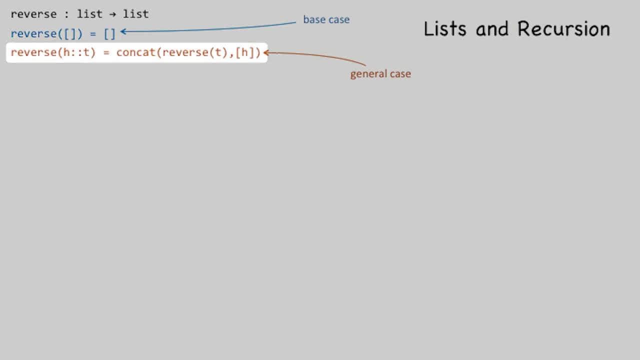 Well, what I'm going to do is take that h part and I'm going to move it to the very rightmost end, And then I'm going to paste that together with the reverse of the t part. Okay, So concatenate the reverse of the t part. 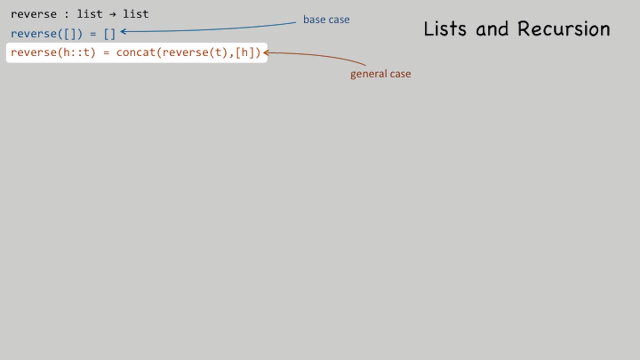 with the h part. That's the general case And of course the reverse of the t part is a recursive call. I'm asking to get the reverse of h colon, colon t By computing the reverse of something else, But that something else. 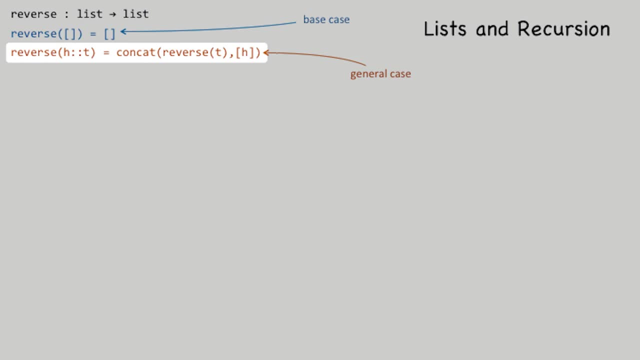 that t part is a little bit smaller than the whole h colon colon t part, And that's going to work to my advantage. When I'm done, I'm going to concatenate the whole thing together Now, by the way. 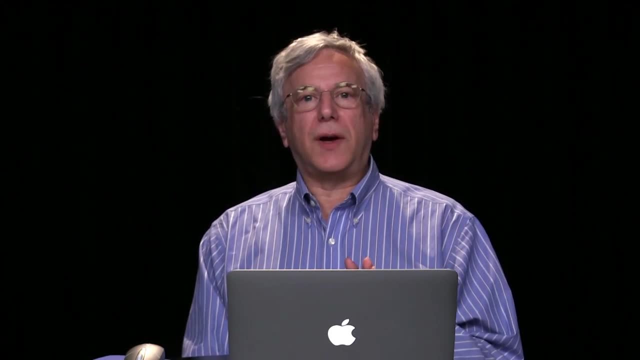 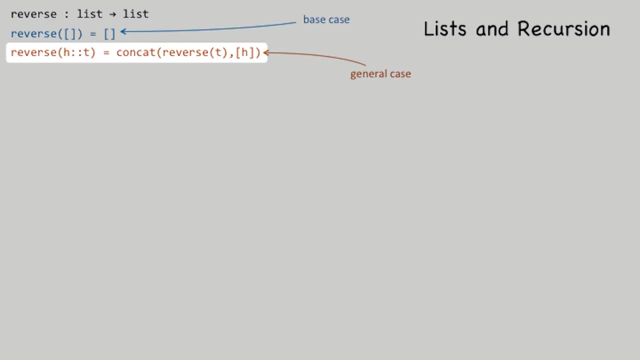 just notice here- it's a feature of the way I've defined concatenate that I have to put h in square brackets at the very rightmost part of this expression. So I'm taking what is just a single element h and I'm making it a list. 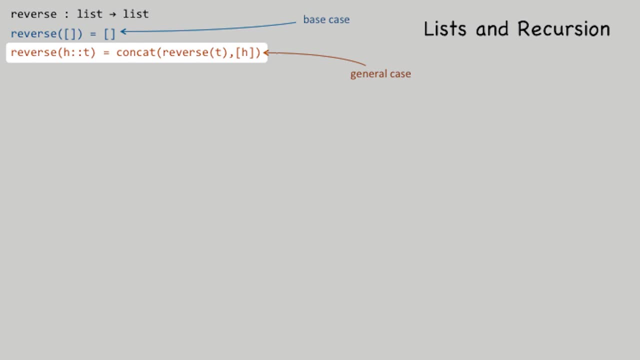 including the element h, And I'm doing that so that I can apply my concatenate function. You don't really have to do this. I could have defined something else besides concatenate. that would have just pasted a single element to the end of a list. 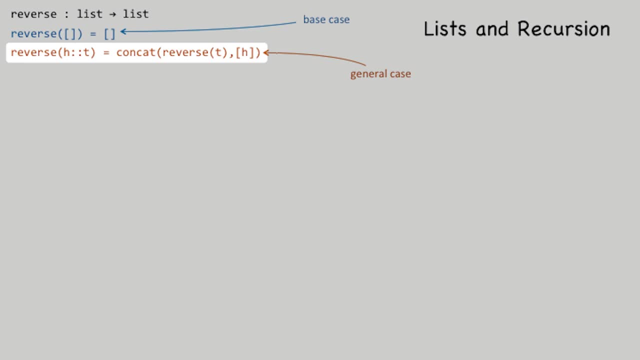 But I don't know. I created concatenate. let's use it. So I take h, I put it in square brackets, I put it at the very rightmost part and then I reverse the t. How's it going to work? 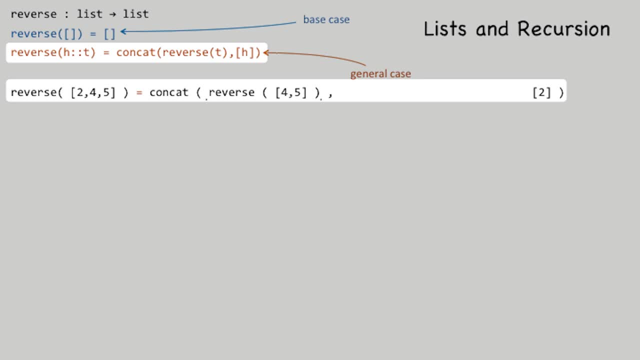 I'm going to start with 2,, 4,, 5, and I want to reverse that list. The way I've reversed the list is I've applied the general case. The general case says concat, and then it has a reverse part. 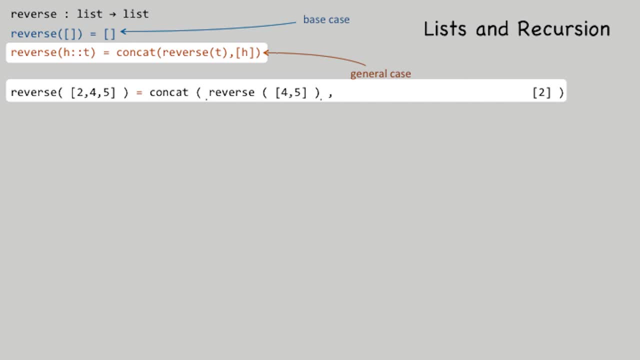 and then it has that brackets h part. I wrote the brackets h part in this case all the way at the very right end of the slide. So with your eye, follow along from the left end to the right end of that new black line. 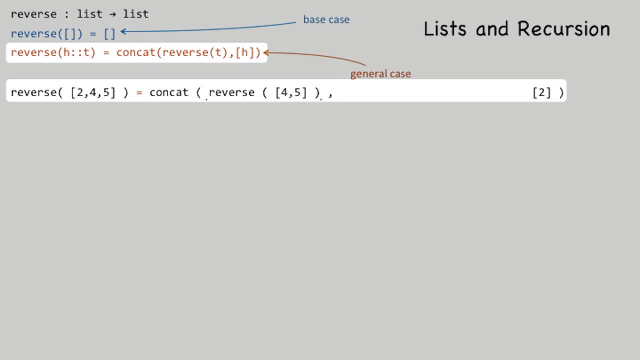 You see that reverse 2,, 4,, 5 is the same as concatenating the reverse of the tail, 4, 5, and then, after a bunch of blank spaces, pasting on to the end of that, the list containing only 2.. 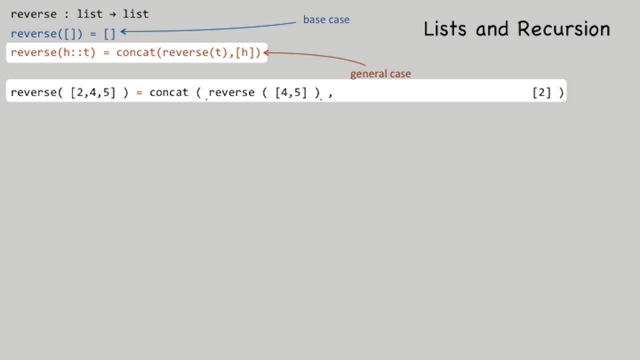 Okay, I left all that space because I'm going to need it for the next several lines that I'm going to show you. So this is the application of the general case And, of course, I'm going to do the same thing here that I did in earlier examples. 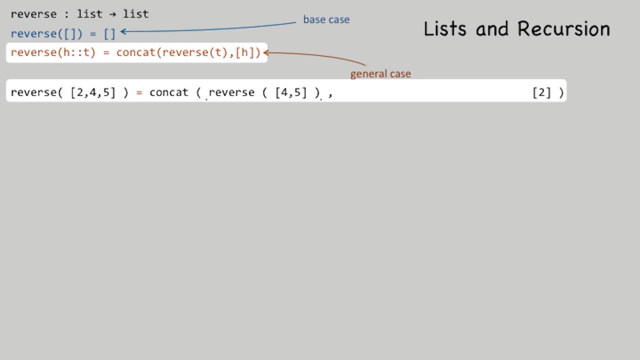 I've got now the reverse of 4, 5 that I have to deal with. I'm going to deal with it using the general case. Here you go To take the reverse of 4 and 5, what I've got to do is: 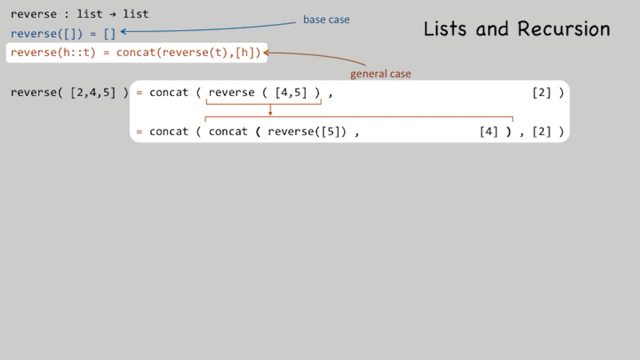 I apply the general case and I concatenate the reverse of 5 to the head element and I list 4.. All right, So I've substituted concat reverse 5, comma brackets 4 for the reverse formula 4, 5.. And of course, 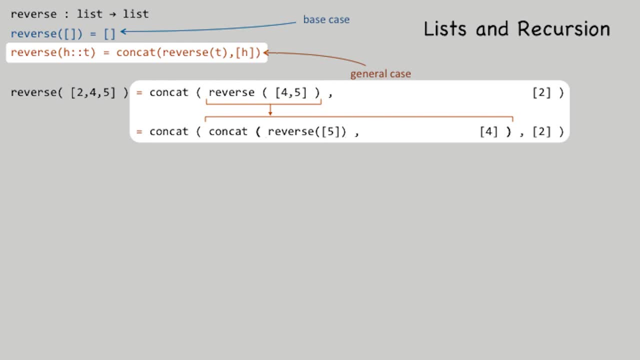 I'm just applying the general case. I just keep applying the general case as long as I have to, And I need to apply the general case again because in this latest formula I have reverse brackets 5, and that still doesn't match the base case. 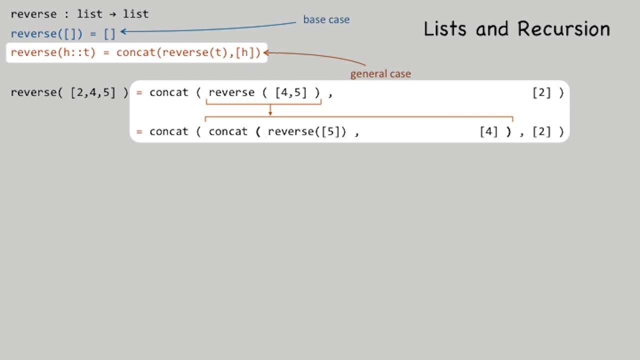 The base case. in order to match the base case, I've got to have an empty list And brackets 5 is not an empty list, So I have to apply the general case again. And when I apply the general case to reverse brackets 5,. 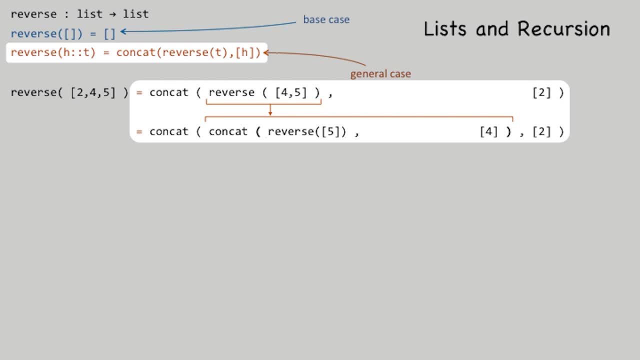 once again, I'm going to do a concat type thing. Here we go. In order to apply the general case to reverse brackets 5, I'm going to concatenate together the reverse of the tail with the head enclosed in brackets. So I'm going to concatenate together. 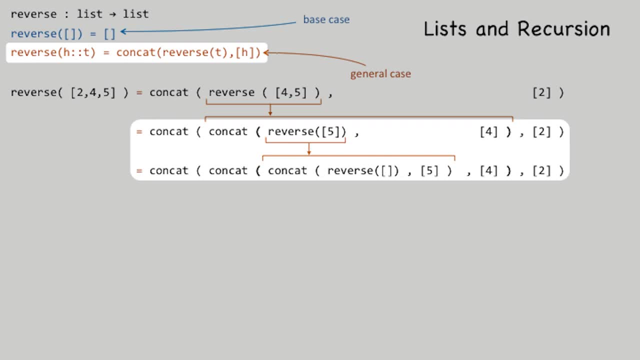 the tail of that one element list with brackets 5.. And the tail of the one element list is once again the empty list. Okay, I end up with concat: concatenate the reverse of the empty list, comma 5.. Hooray, hooray. 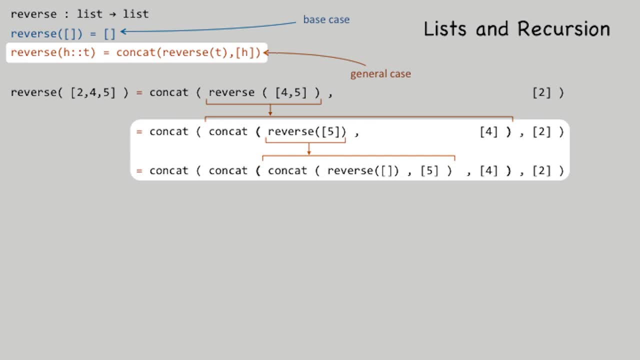 Look what I've got now. I've got the reverse of an empty list, And when I have the reverse of an empty list, that means that I can finally, whew, apply my base case Whenever you can apply the base case. 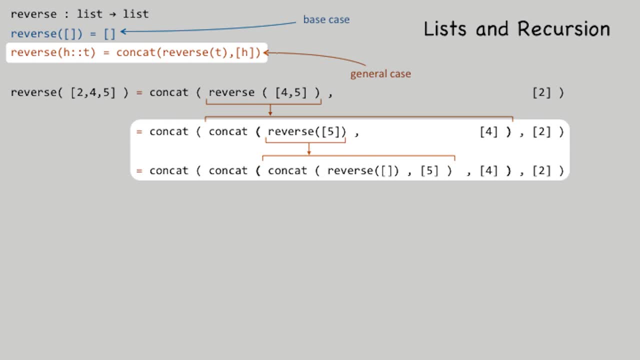 that's really good, because that means the light is at the end of the tunnel. When I apply the base case to that reverse empty list expression, I get simply the empty list. Oh, things are getting nice. I'm not continuously getting. reverse this, reverse that. 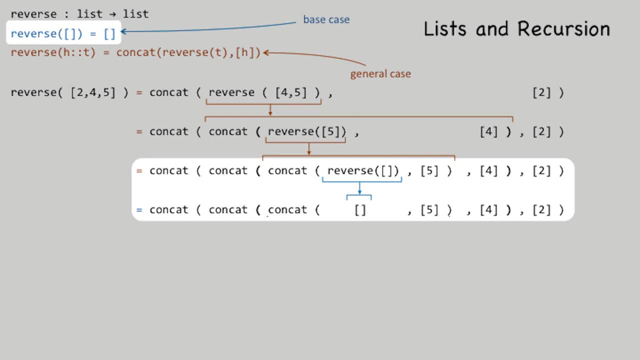 reverse, reverse, reverse. I've just got the empty list, So now what do I have to do? I have to concatenate together the empty list with the brackets 5 list. Well, when I concatenate what is essentially no stuff with a list containing 5,. 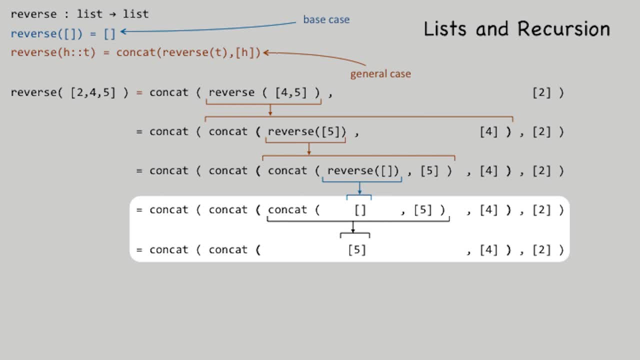 I get simply the list containing 5.. And now again I have an expression without the word reverse in it. I don't even have to apply the base case or the general case at this point. I just have to do concatenation. 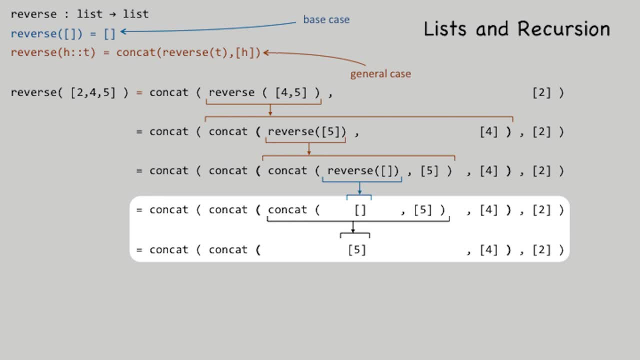 Well, when I concatenate together the list containing 5 with the list containing 4, I get the list containing 5 and 4.. And now I've got one more concatenation to do. I've got to concatenate the list containing 5 and 4. 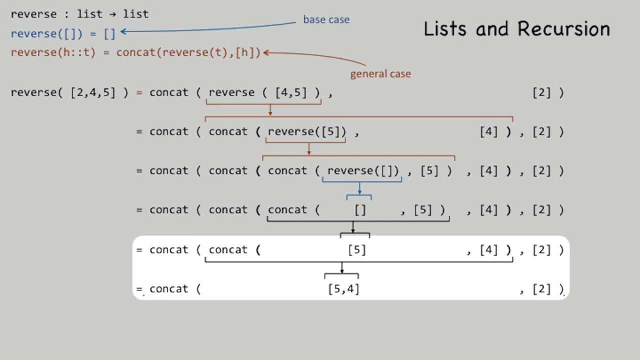 with the list containing 2.. And when I paste those two lists together, I get 5 and 4 and 2.. Very, very cool. Recursion is such nice stuff. I really like it And it's useful And it's extremely useful. 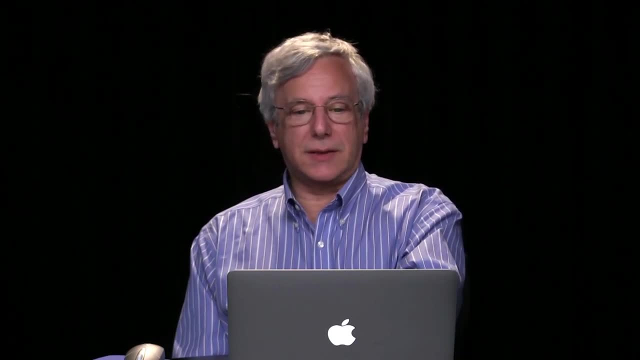 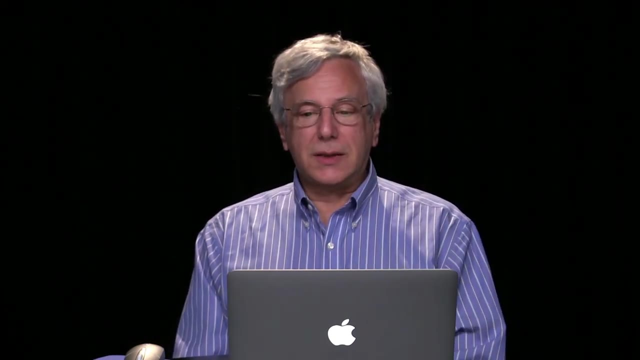 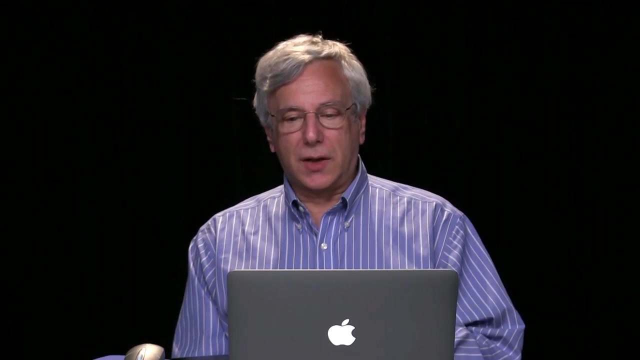 when you're talking about lists. Okay, I want to end this section with one more application of recursion. It's not for everybody. It's for people who have dealt with something called sorting. So if you haven't dealt with sorting, you may want to take a look at what comes next. 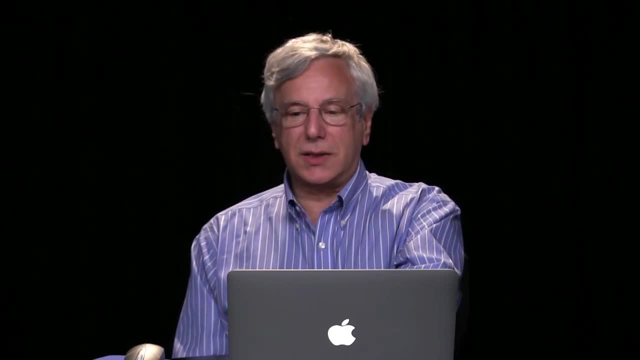 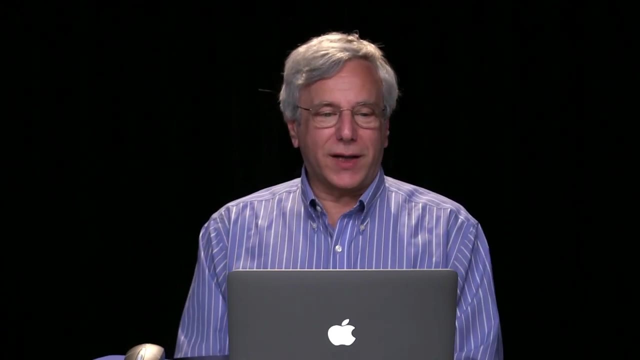 Otherwise, you may want to skip the next two minutes, the last two minutes of these slides. Oh, come on, Watch it anyway, It'll be good for the soul. Let's see what happens. Here's the quicksort. What the heck is the quicksort? 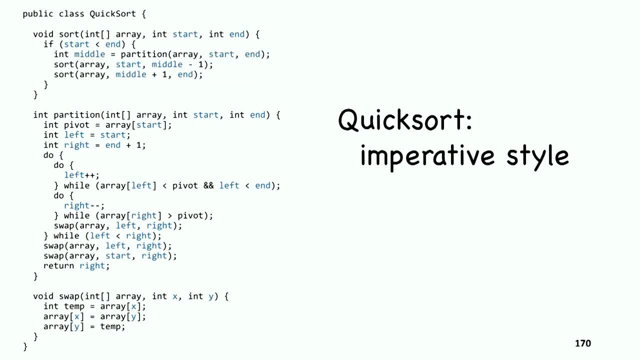 Well, in all kinds of applications we need to sort values, We need to take a bunch of values and get them in, say increasing order, And over and over again. I'm going to say increasing order because that's just one way of thinking about it. 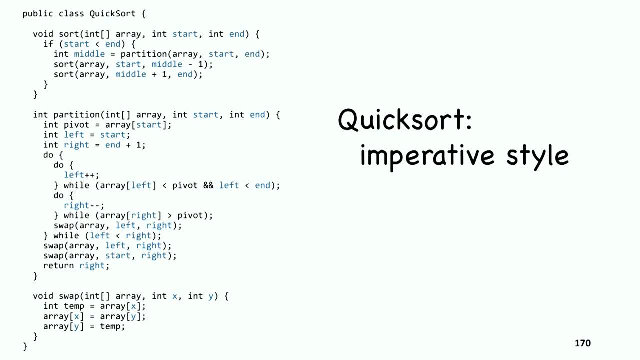 You might want to get things in decreasing order. I don't know. Let's just say increasing order. A quicksort is a super clever way of putting things into increasing order And, by the way, in most cases it's quite an efficient way. 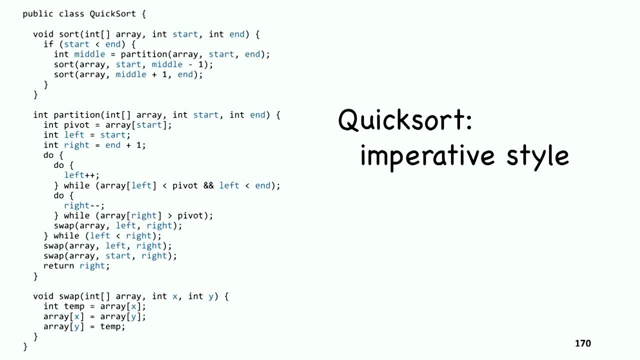 of putting things in increasing order. It was created a number of years ago and it's used in all kinds of applications, And what the quicksort does is it says: well, take an element kind of put it in the middle, put everything to the left of it. 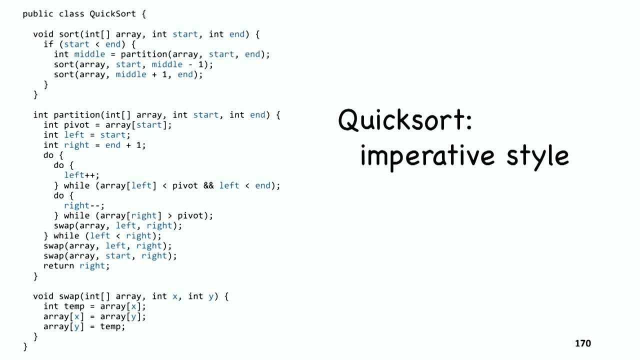 make everything to the left of it be smaller than that element, make everything to the right of it be larger than that element, and then recursively keep going. I don't intend to instruct on the details of the quicksort here. All I want to do is show you. 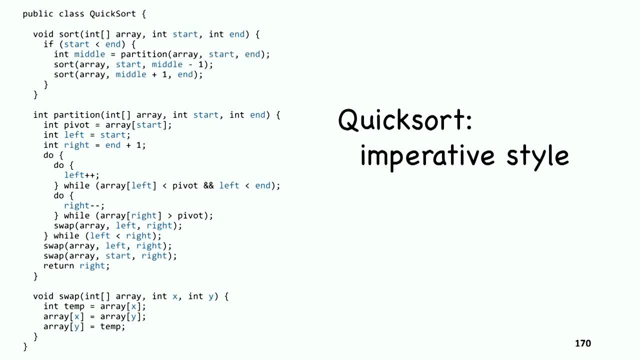 a version of the quicksort in imperative code. So I don't know. 20 lines, is it? Yeah, I mean it's a lot of lines. I guess I'm not so concerned about the number of lines here as I am about the things that are in blue. 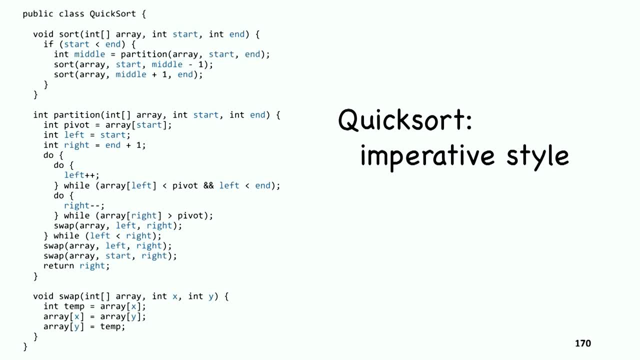 The things that are in blue are indices: The fifth element, the sixth element, the seventh element. They're little numbers that I kind of have to worry about when I'm creating this code And, believe me, when I create this code the first time. 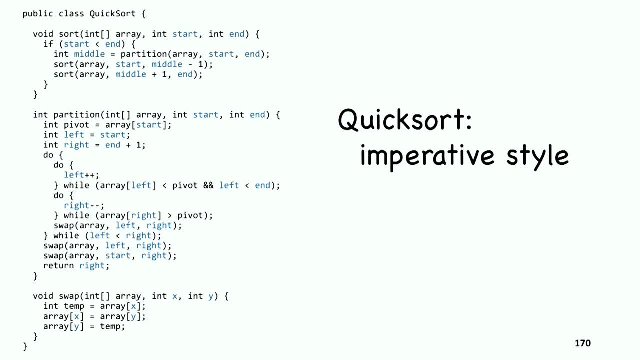 I always get these numbers wrong the first time. For instance, slightly down from the top of the code, you'll see the words middle plus one, right, And all the time instead of middle plus one, I'll write middle, or you know. 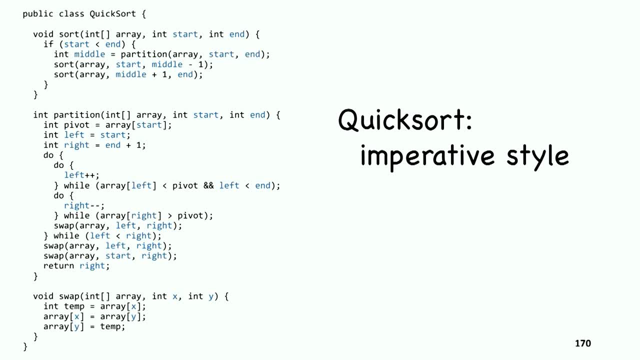 middle minus one or whatever. And whenever I write the code the first time I get those things wrong and have to fix it. All the things in blue, all the words in blue here, are places in the code where you have to worry. 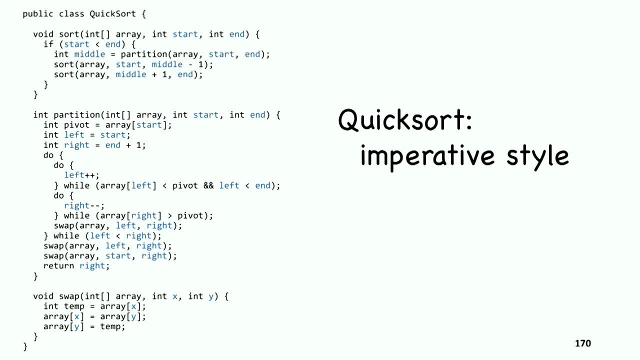 micromanage the positions of things that you're looking at in the list. That's an imperative thing, An imperative solution to the quicksort algorithm, An imperative way of solving the quicksort algorithm. All right, on the next slide, what I'm going to show you is a purely functional way. 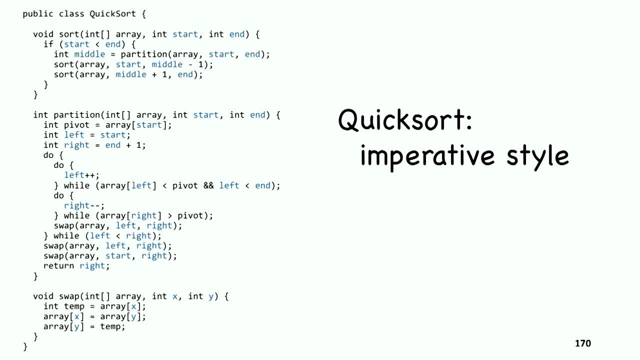 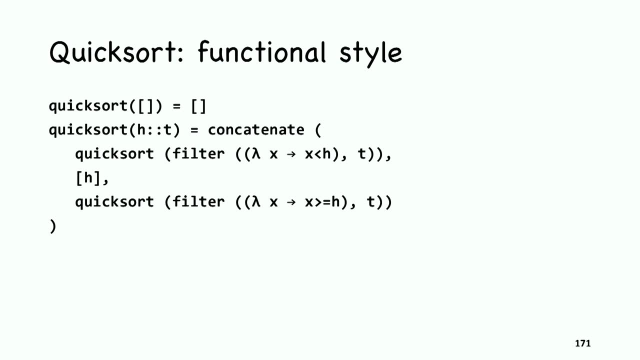 of looking at the quicksort algorithm. The code I won't keep you in suspense is much, much shorter, Much shorter. Great, I love saving typing, but saving typing isn't the issue here. What I like about this code is that 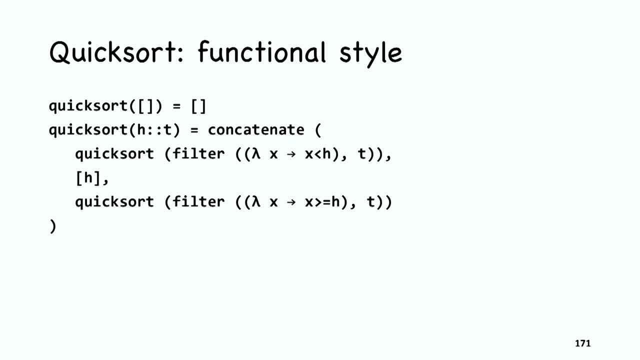 number one: it looks more like what I consider to be the definition of quicksort. But number two: it also doesn't make me micromanage the positions of elements. There's no place here where I have to write plus one or minus one or this and that. 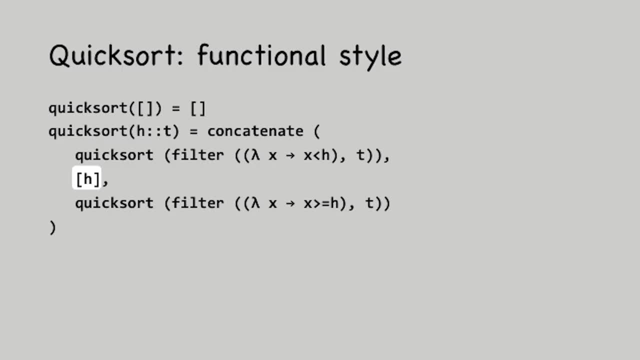 Nothing's in blue. All I'm saying here is: take the head of the list, put it sort of in the middle and then make sure that the stuff to the left of it in the list is filtered for being less than that middle of the list. 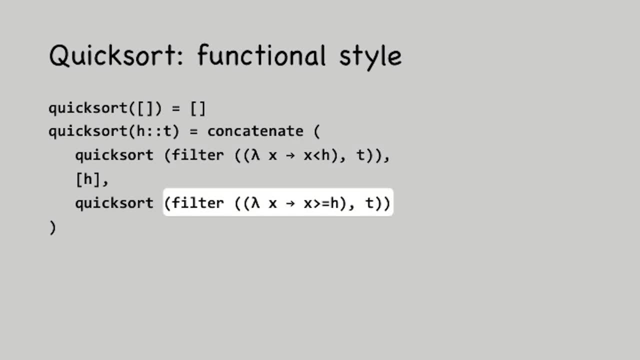 And make sure that the stuff to the right of it is filtered for being greater than that middle of the list And then recursively call the quicksort on the left half of the list and on the right half of the list. It's extremely elegant, this solution. 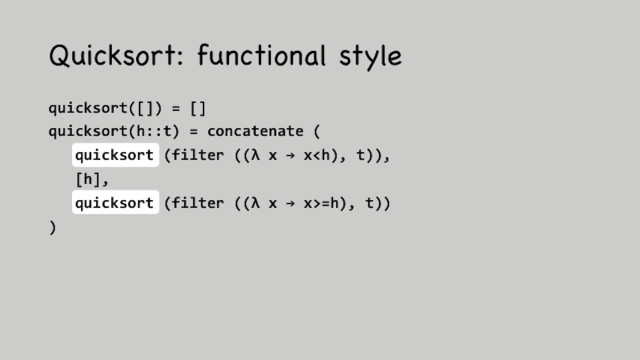 and it works. If you code this in a number of different languages that have this vocabulary, you can get an answer, and it's very nice and very cute. I have something even cuter for you. This is the quicksort. Can I use the quicksort? 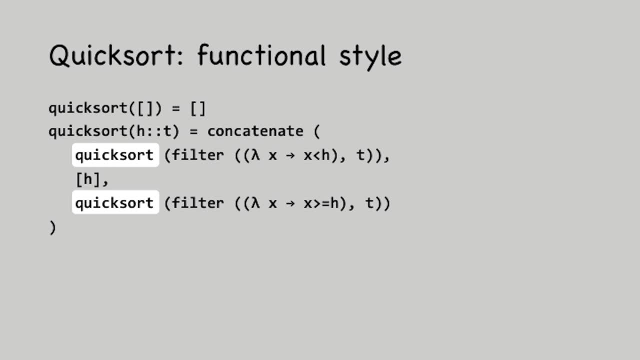 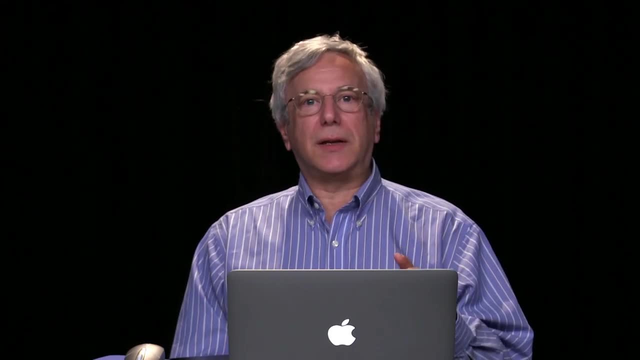 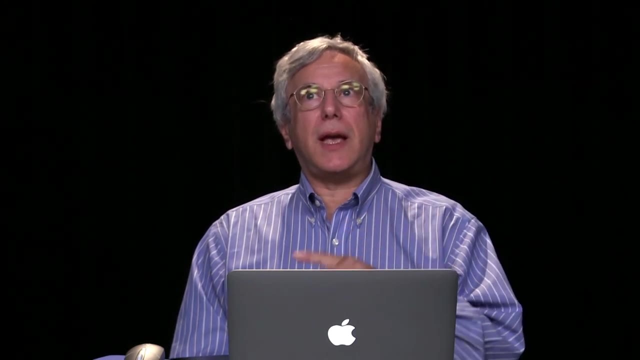 to efficiently find the smallest element in a list? Let's think about that. How would you normally find the smallest element in a list? Well, let's see One way of doing. it would be to march from the beginning of the list to the end of the list. 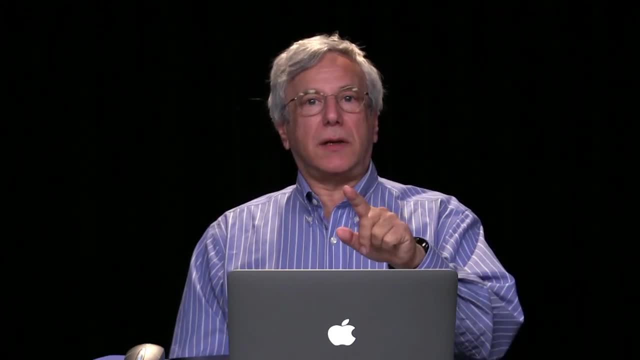 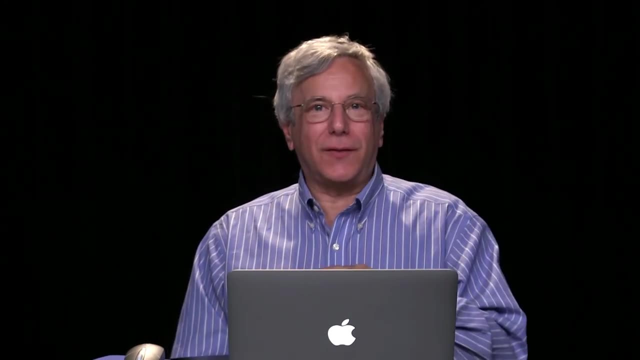 and each time keep track of the smallest element that you've seen so far. That's actually a very good way of doing it. I'm not going to pretend that that's not a good way of doing it, But another way of doing it. 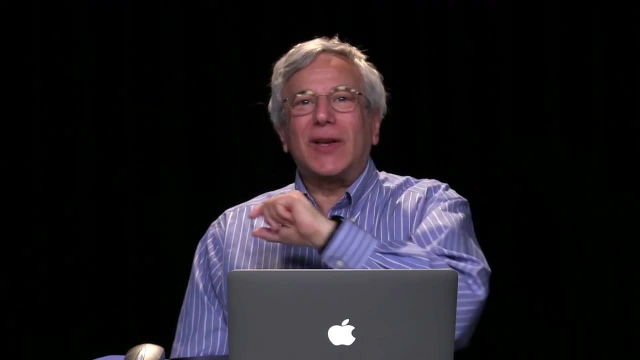 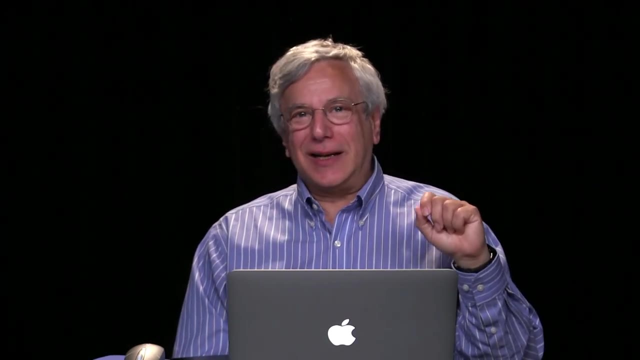 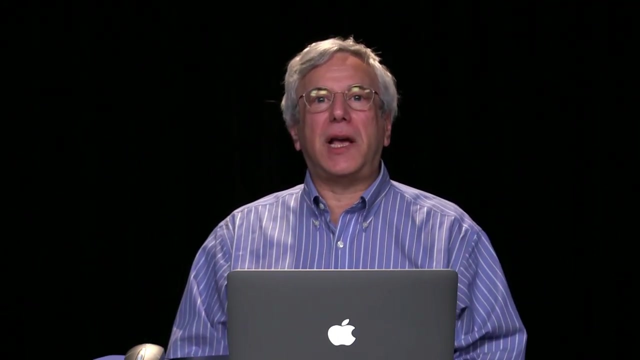 maybe a little bit cuter is to sort the list first and then pick off the first element. I call it cuter, but you know I'm really cheating. Why in the world would you bother sorting the entire list just to pick off the leftmost element? 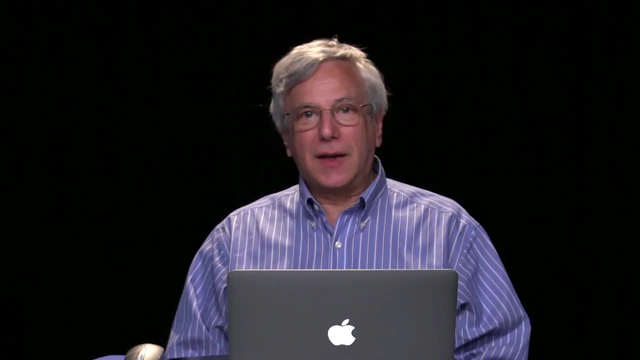 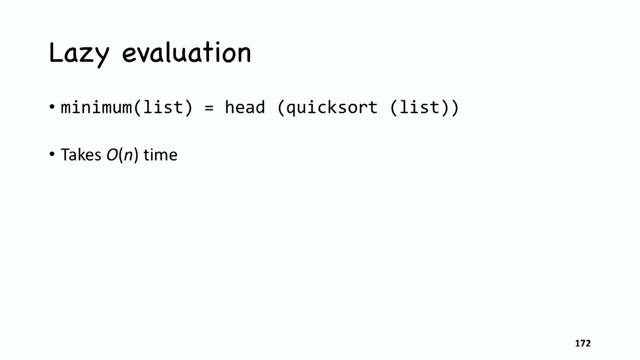 Seems a little crazy, right? Well, that brings us back to a topic that I was talking about several segments ago: Lazy evaluation. One way of finding the minimum of a list is to call on quicksort to do its thing and then say: 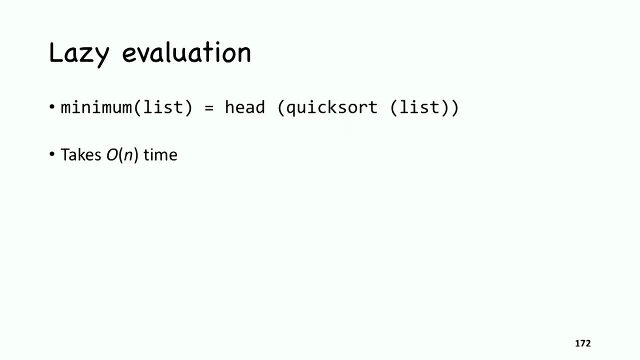 well, as part of the quicksort, I'm going to be looking for the head of the list, the leftmost element in the list. Wait a minute, Aren't I sorting the entire list just to find the minimum element, the leftmost element? 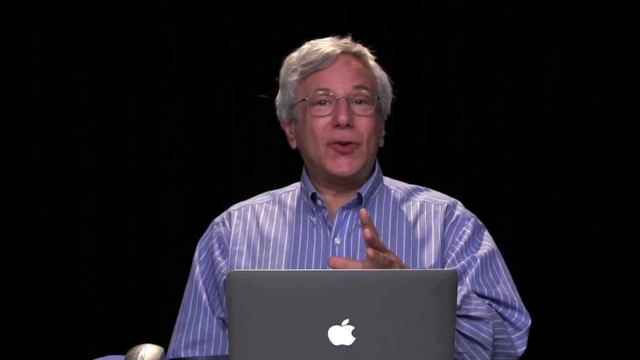 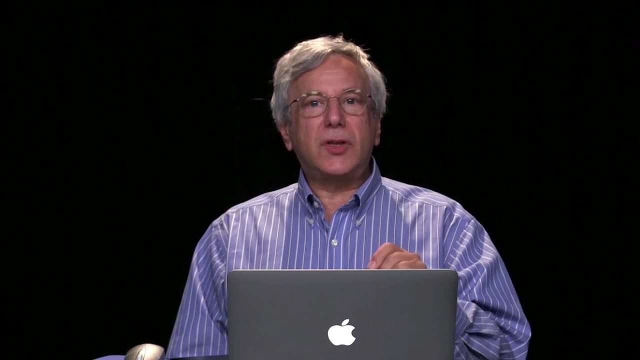 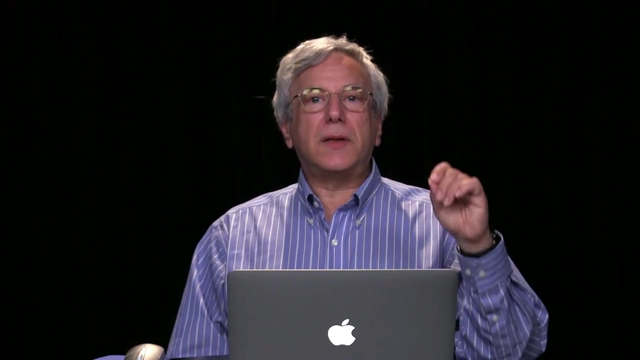 No, If lazy evaluation is doing what it's supposed to do, then this call head of quicksort of list is doing only enough work of the quicksort to get the smallest element to the very leftmost position in the list. So yes, I'm trying to evaluate. 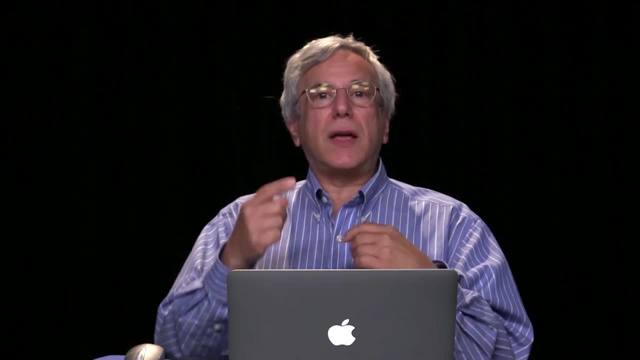 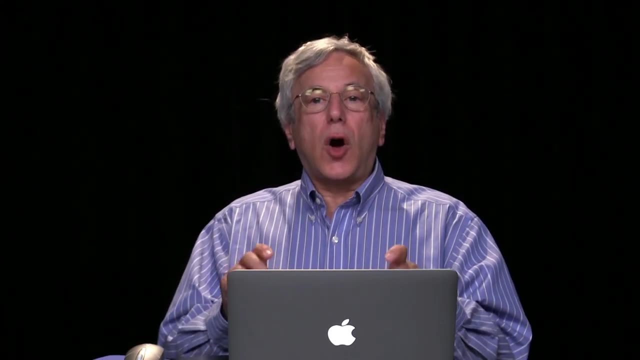 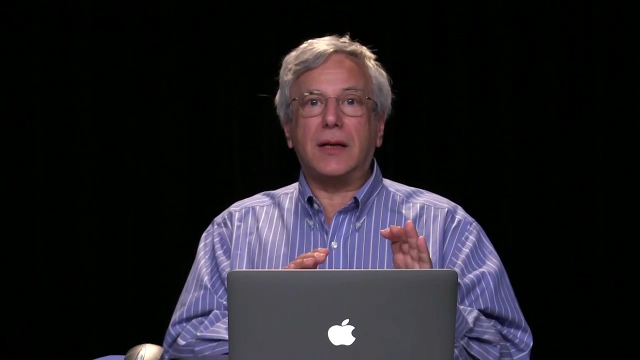 or proposing here that I might evaluate the expression quicksort list. but with lazy evaluation I do only enough quicksorting, only a lazy amount of quicksorting. that's necessary to find the head Turns out if you play your cards right, this algorithm. 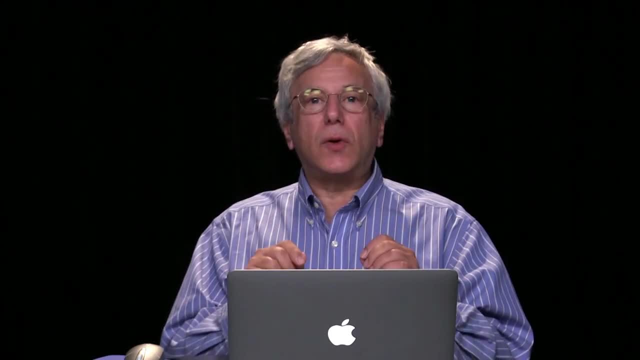 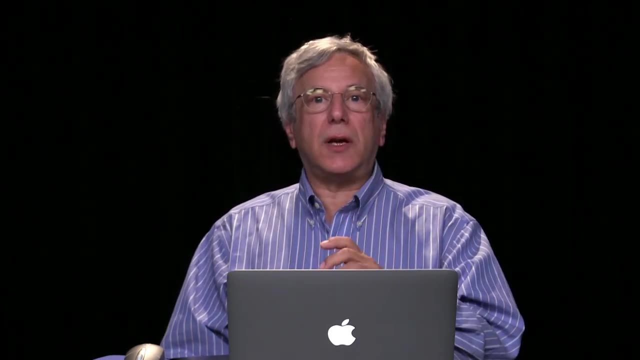 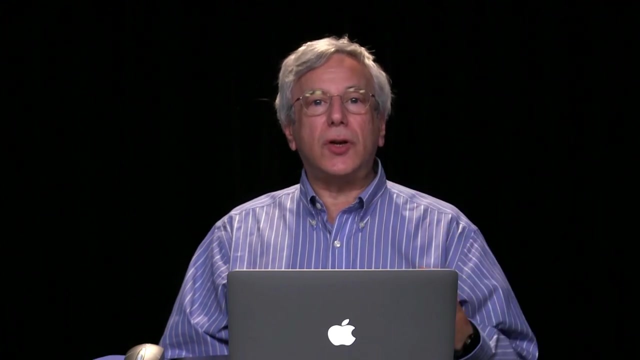 this way of finding the head of the list is equally as efficient as marching from one element to the next. A proposed solution in which we try sorting the list and then picking off the first element is just as good as the situation in which you just go one by one through the list. 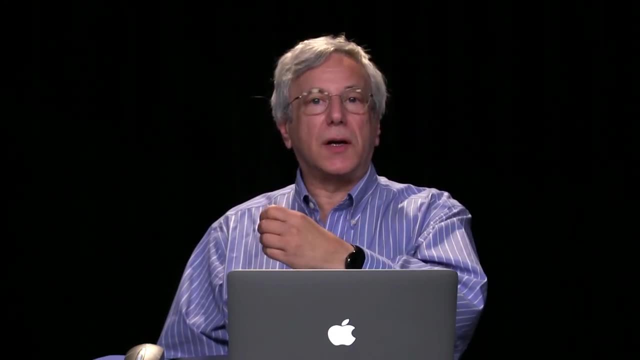 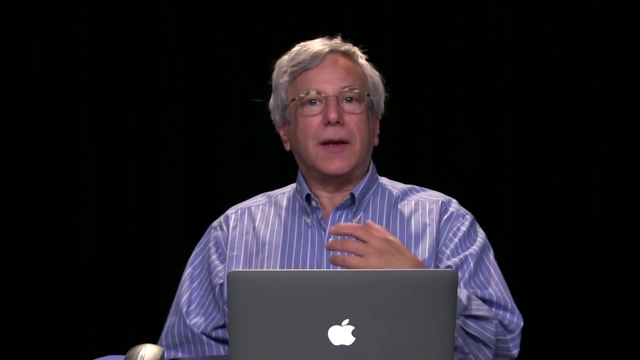 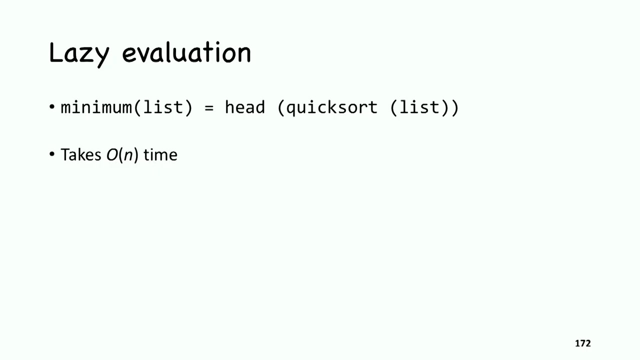 keeping track of the smallest so far In the terminology of computing. both solutions take order and time. It's not the most useful thing in the world to know that you can take head of quicksort and efficiently find the minimum, but it's magic. 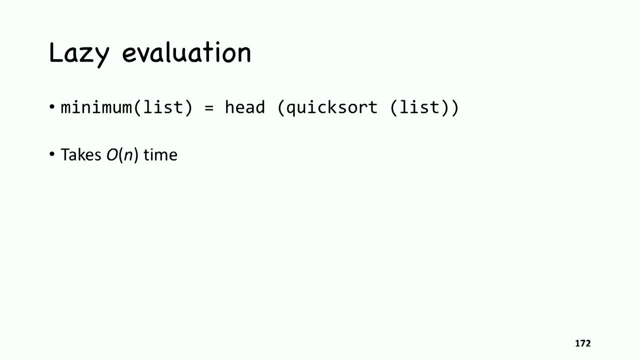 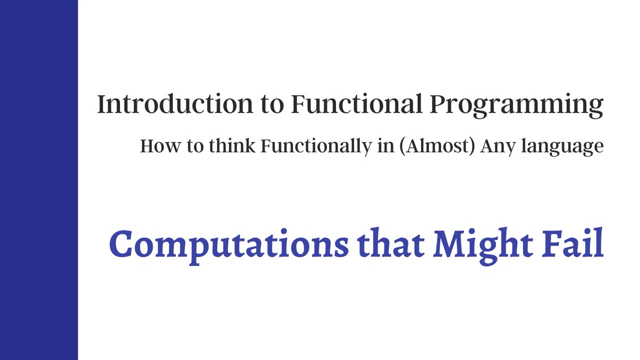 It's really, really cute, So I just had to show it to you. Okay, we're going to march on The next thing that we do: monads. This section of the course is about monads. What is a monad? 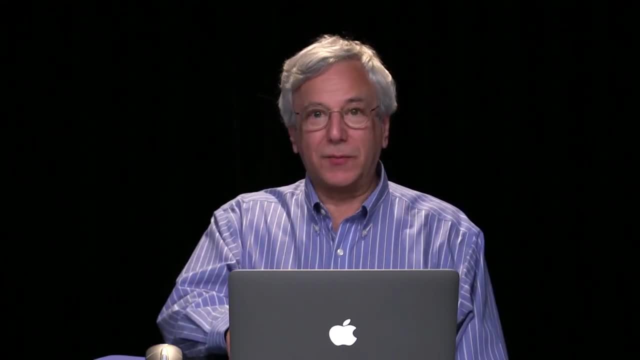 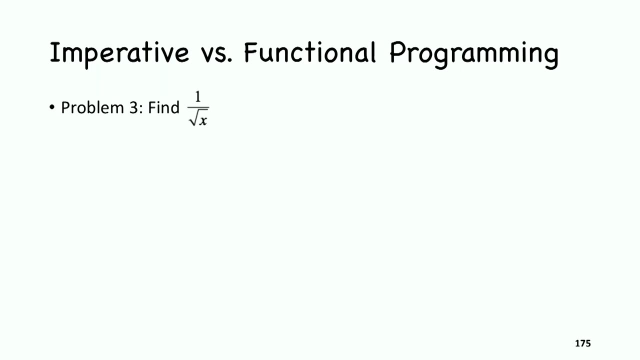 I'm going to tell you: Let's start with a problem to solve. What's the problem? I want to find 1 over the square root of x. What could be so complicated about that? Well, if you're doing it right. 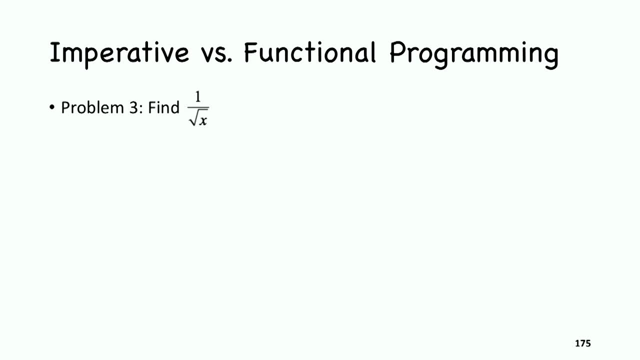 then you want to check for things that can go wrong. What can go wrong? Oh, I know, Maybe x is negative and I can't take the square root of it. Yeah, yeah, If I have complex numbers, I can take the square root of it. 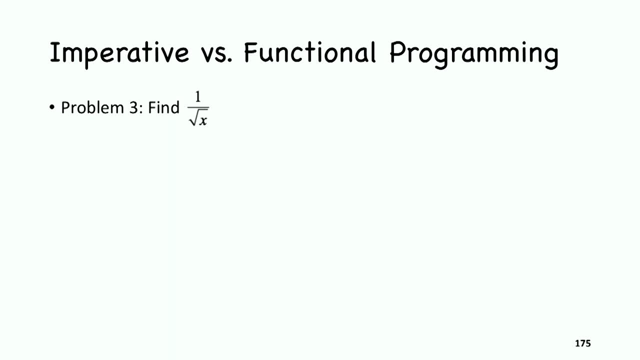 but let's not do complex numbers, Let's just do real numbers, floats. So there's not going to be any such thing as the square root of negative 1 here. If I try to take the square root of a negative number, failure. 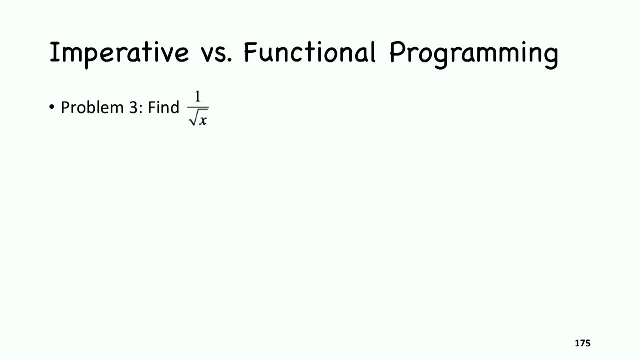 I've got to deal with it somehow. If I have to deal with it in an imperative style, there's going to be some if-thens, There are going to be some exceptions. I don't know. Hey, something else can go wrong here. 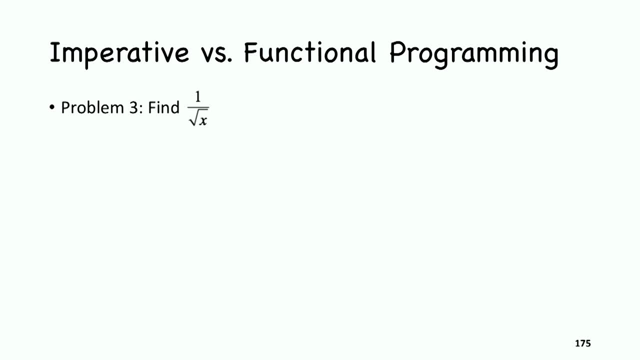 If I try to divide by zero, trouble. Can't divide by zero, No answer. You just don't get an answer from that. So there are two places during this computation that things can go wrong, and one way or another I've got to deal with them. 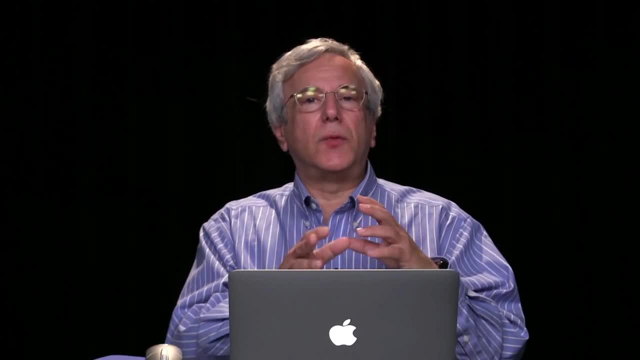 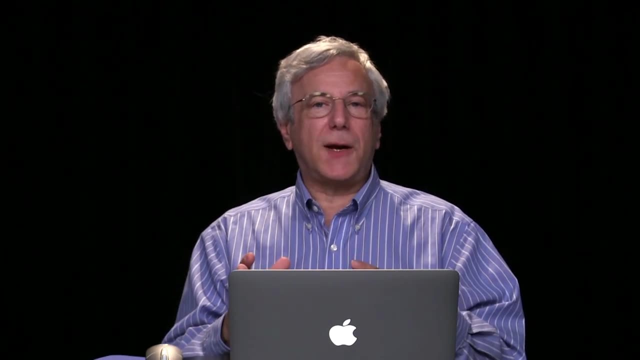 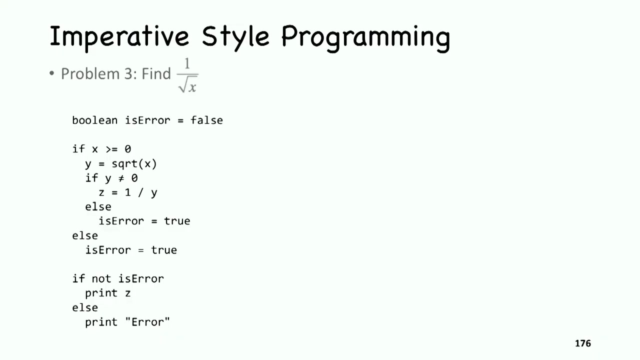 Now in an imperative setting. I'm going to deal with them by maybe jumping around branching, going from place to place in my program. Well, we'll see. Here's a proposed imperative solution to the problem. Again, this may not be your favorite way. 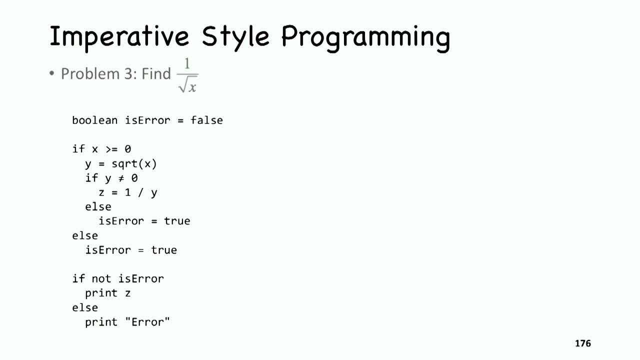 of handling the potential problems with an imperative style, but it's a way, and most ways will look something like this. I decided to start off with a Boolean value called isError. Set it equal to false, because there are no errors to start with. 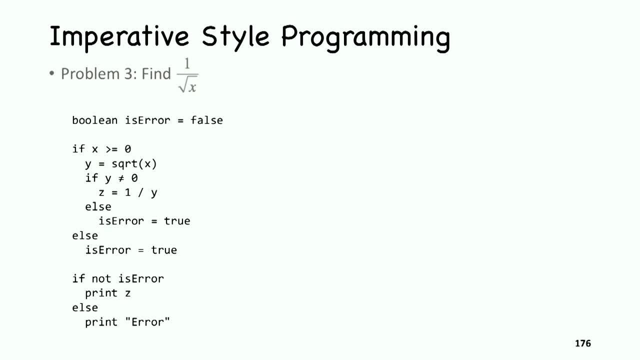 Try to take the square root of x, if I can, Then go ahead and try to divide the result into one. If I run into a problem along the way, then in this version of the code, what I'm doing is I'm setting my isError flag to true. 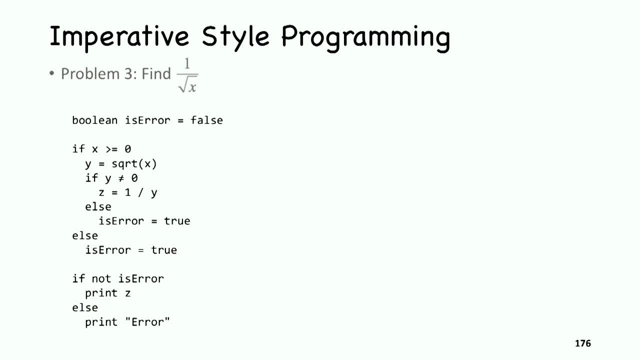 and kind of dealing with that later on in the code. You might not do this with ifs and thens. You might do it with some kind of exception handling mechanism. but one way or another you're going to have a collection of statements that describe things in a sequence. 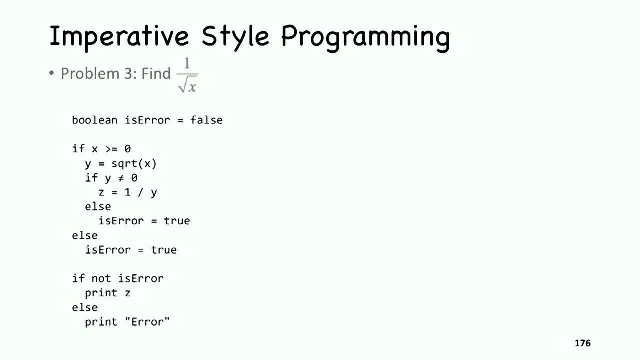 and possibly within that sequence, you're going to be jumping from one part of the code to another. In this case, you're jumping either to the if part of an if, then else, or to the else part. But anyway, jumping around. I don't like jumping around. 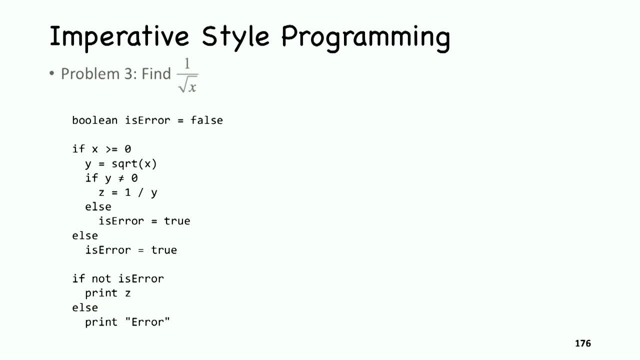 as you know from looking at the earlier parts of this course, And you know if you look at that it's not the easiest thing to understand, if you just stare at it, if you just glance at it at first. Yeah, if you're careful about looking at the ifs and the else's. 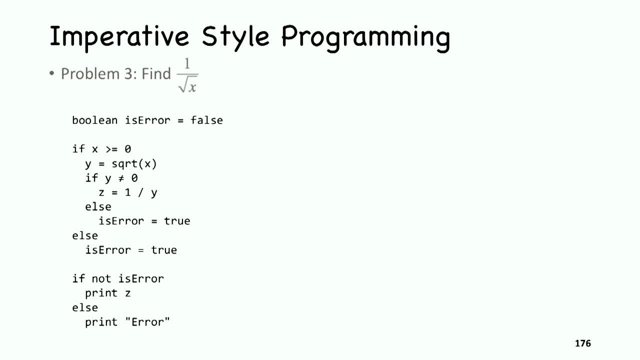 you decide that it works. But it's what? maybe ten lines of code, Not something that you'd want to look at at a glance and certify it as being correct. So what we want to do is change the solution to this problem from the imperative style. 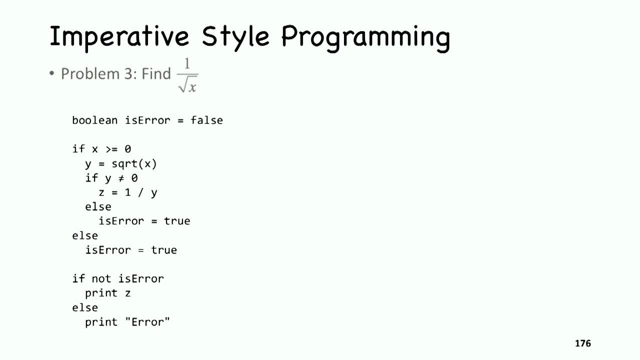 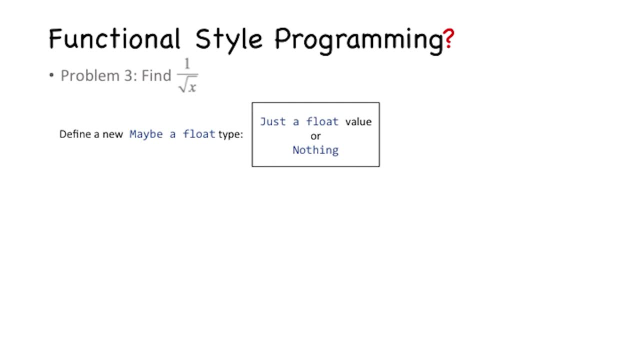 into the functional style. Let's see what we can do. I'm starting with the problem: find 1 over the square root of x. Now I'm going to define a new type of thing, And that new type of thing is going to be called. 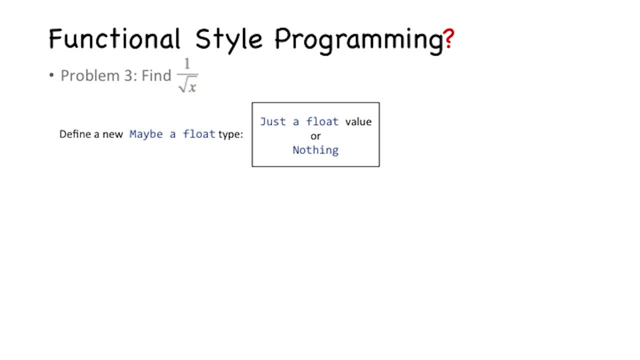 maybe a float, And that new type of thing is going to contain one of two different kinds of values. It may contain what I call just a float value, or it may contain what looks like a keyword here: nothing, 1, that's just plain old 1.. 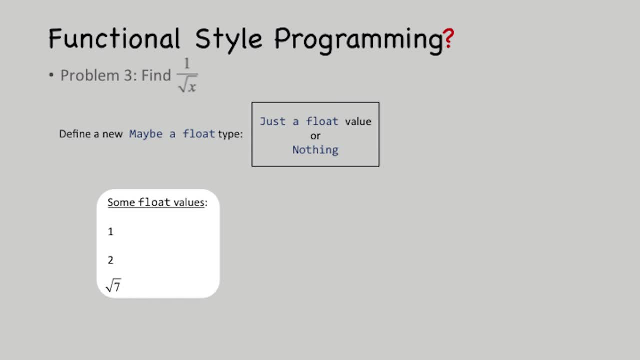 2, that's plain old 2.. But I can also have a number like 2 sort of embedded inside of one of these, maybe a float things. If I have the number 2 embedded inside one of these, maybe a float things, then I won't call it 2,. 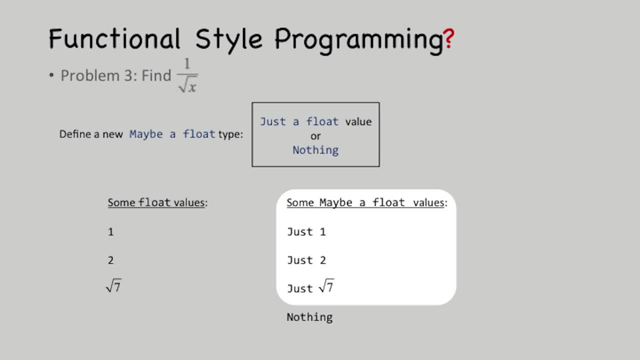 I'll call it just 2.. And if I end up with an erroneous condition, like trying to take the square root of minus 1, or trying to divide by 0,, then my maybe a float type is going to contain nothing. So my maybe a float type. 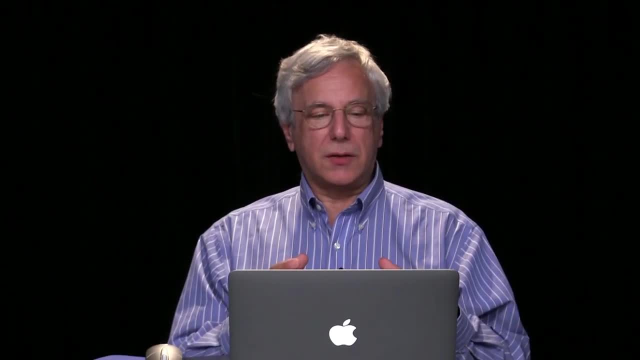 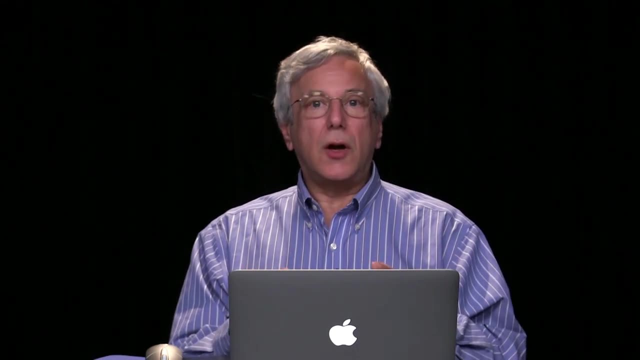 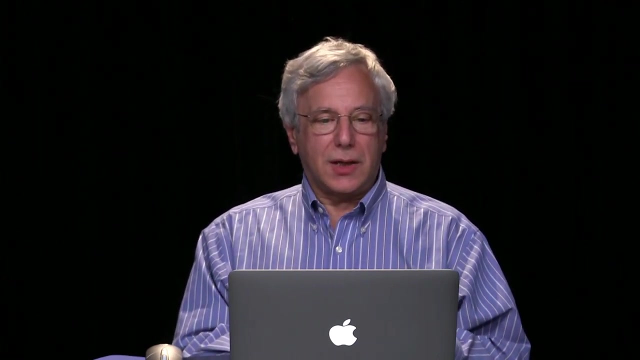 to summarize, is going to contain either just 2, or just 5,, or just square root of 7, or just 0, or alternatively, it can contain nothing. Now, the important thing to remember here is that, while a maybe a float type, 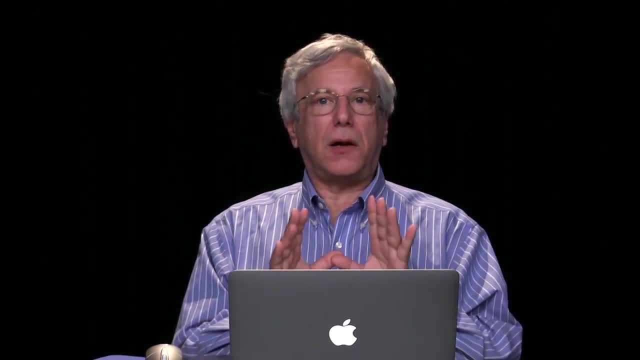 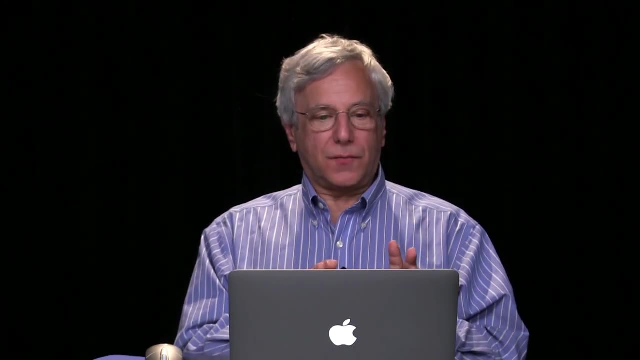 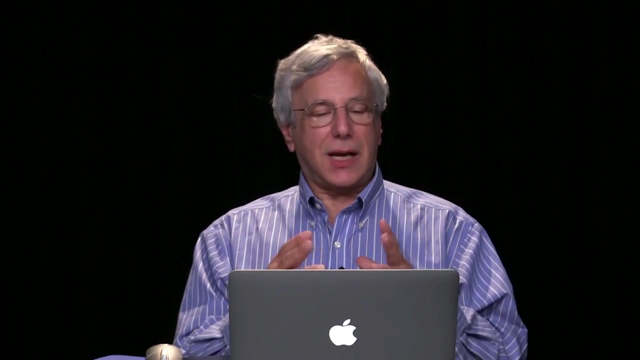 can contain within it a float. it is never exactly the same thing as a float. No, If I have somehow gotten myself a maybe a float thing, a maybe a float thing containing just 7, then that's still a maybe a float thing. 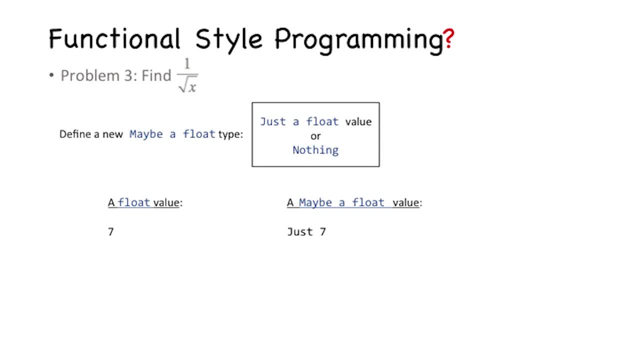 What it contains inside itself is just 7.. It's still a maybe type, even though, yeah, the number 7 is nice and firmly inside there. But anyway, a maybe, a float type is kind of related to a float, but it's not exactly the same as a float. 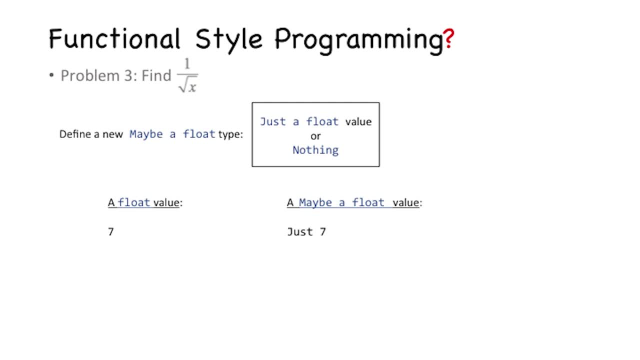 no matter how much I want to think of it as a float. It's important to remember that. How, then, am I going to use this in order to solve the problem, functionally and cleanly, of taking 1 over the square root of x? 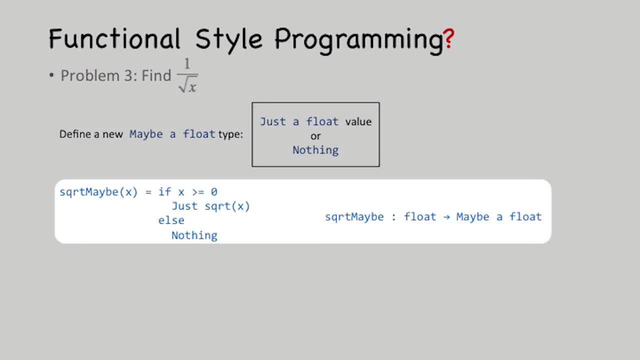 Well, I'm going to define two functions. One of them is called square root maybe, and the other is called reciprocal maybe. And the square root maybe function is going to start with a number. I'll call it x and return for me. 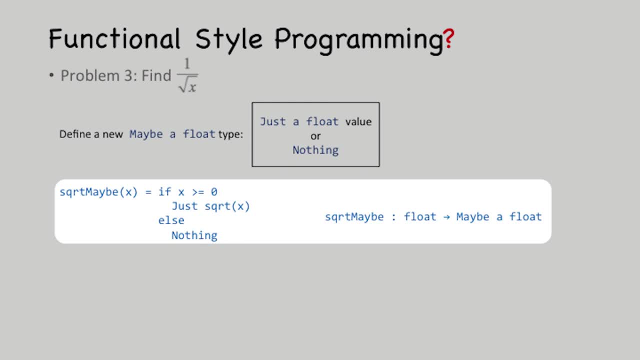 a maybe a float type function. So you see, in blue there it says square root maybe takes a float and returns a maybe a float type object. Now the formula that I've written on this slide for square root, maybe it has an if-else in it. 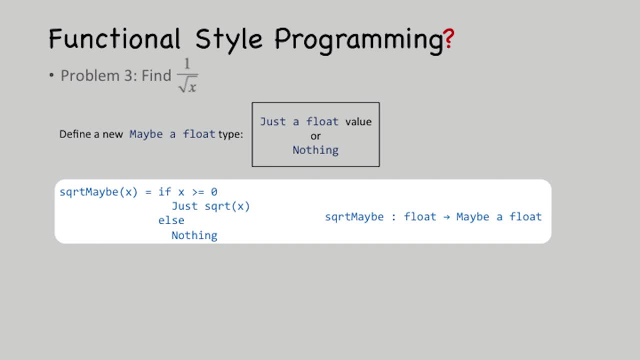 but you know, that's just kind of my shorthand way of defining what I mean by square root. maybe You're not actually going to have to put that in your code, or if you do put it in your code it may not look so much like. 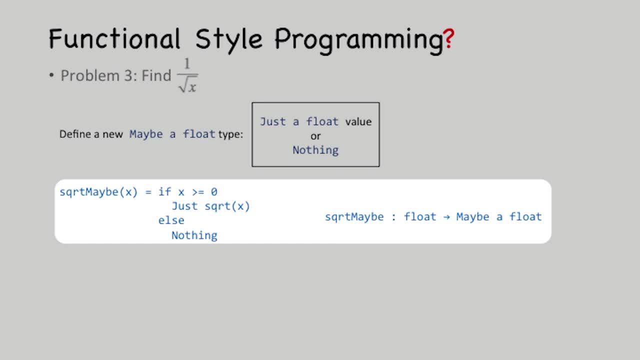 do this, then do that One way or another. what I'm saying there is when I take square root. maybe I'm going to try to take the square root of a number, the honest-to-God square root, and if I do, 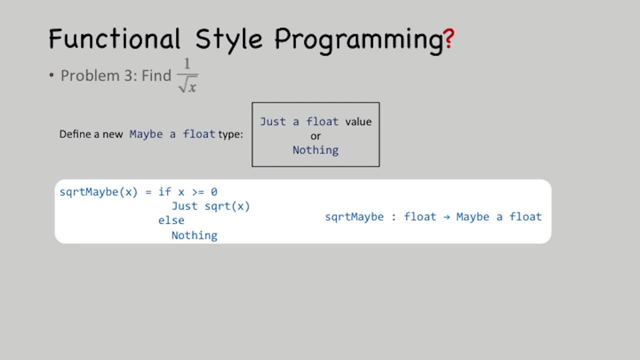 I'm going to get just square root of that number. So if I try to take square root maybe of 4, I'm going to end up in the top part of the if-then-else, I'm going to get just 2.. 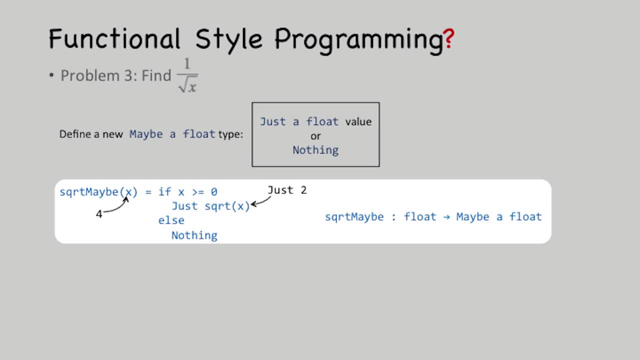 Okay, once again, if I try to take square root, maybe of 4,, I'm going to end up with just 2.. On the other hand, if I try to take square root, maybe of minus 7,, then I'm going to end up with nothing. 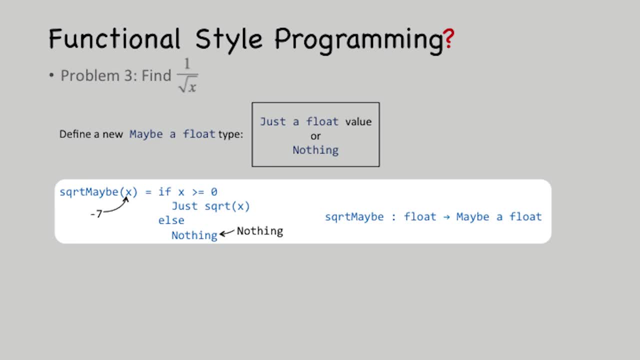 So square root maybe is going to start with a number like 4 or 0 or minus 7, and it's going to end up with a just-type thing or nothing. Okay And reciprocal maybe is similar. Reciprocal maybe starts off with a float value. 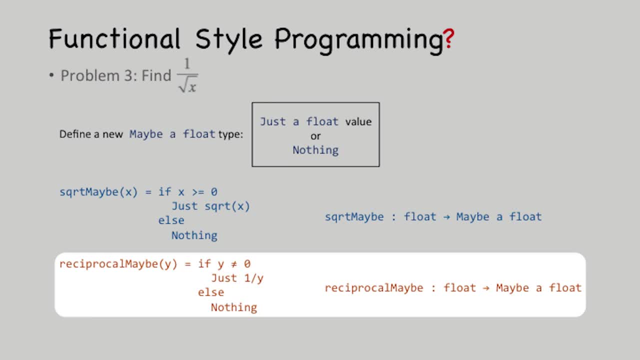 and gives me maybe a float. If y is 7, then applying reciprocal maybe ends up giving me 1 over 7.. Uh-uh, just 1 over 7.. And if I start with 0, then applying reciprocal maybe gives me nothing. 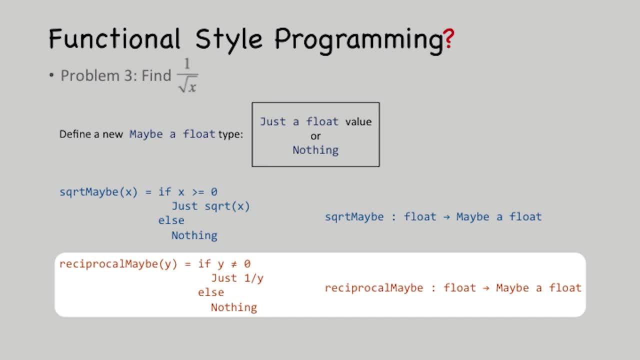 So the question is: is it possible now for me to just take the square root maybe function and call it and apply it to a value such as 3, and then take that result value and feed it into the reciprocal maybe function? And you notice all those question marks that I have on the slide. 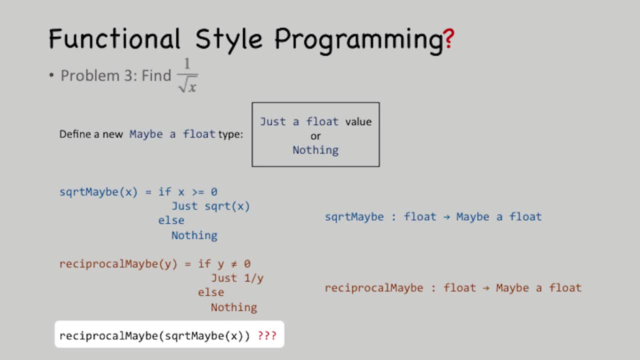 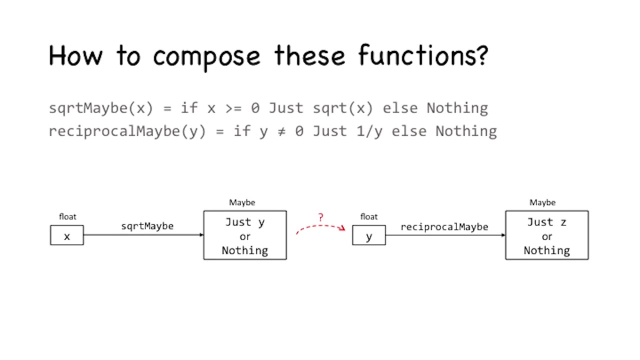 The question marks are there for a specific reason, because the loaded answer to this question is no, you can't do that. Why not A square root maybe application takes a float and gives you a maybe type of thing, A reciprocal maybe application. 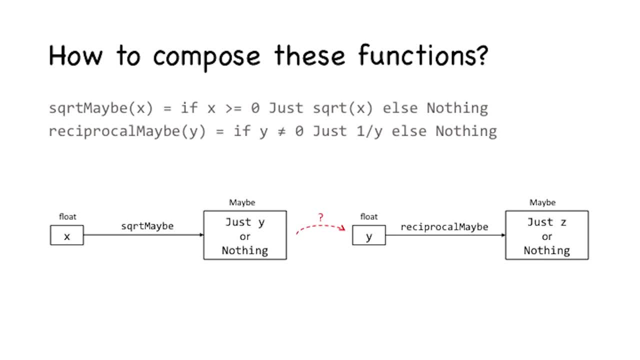 doesn't take a maybe type thing. it takes a float and gives you a maybe type thing. I've got two functions here and they both do some sort of floaty stuff but they don't exactly fit together the way the pieces in a jigsaw puzzle. 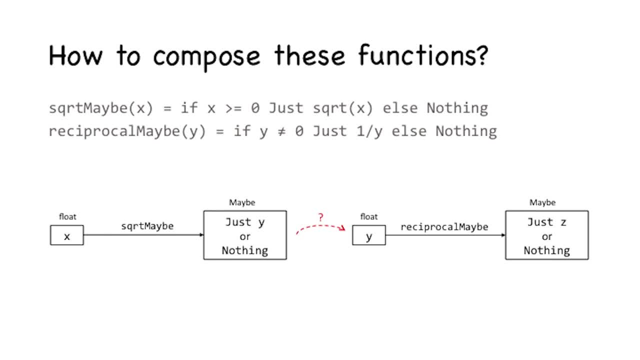 are meant to fit together. You know, I want to take the result of square root maybe and feed it into reciprocal maybe, but unfortunately the maybe, a float type thing isn't exactly the same as a float If it's not something like just 2 or just 7,. 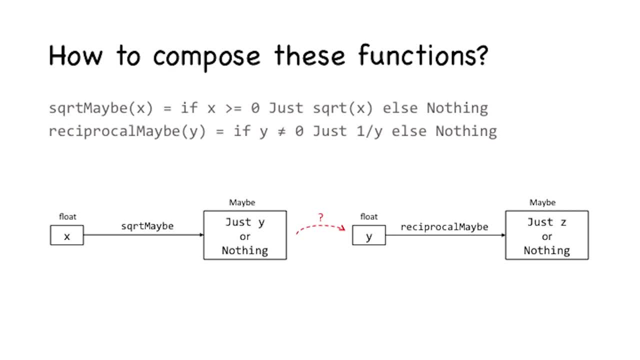 which I sort of think, yeah, that's pretty much a float, then it's nothing, and I haven't got any equipment for feeding nothing into the reciprocal maybe function. You know, now I can make up all kinds of rules about how reciprocal maybe works. 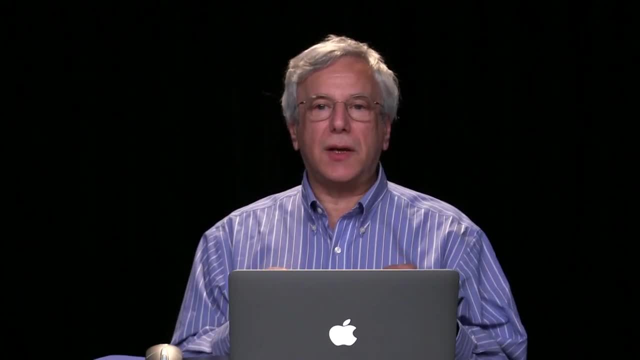 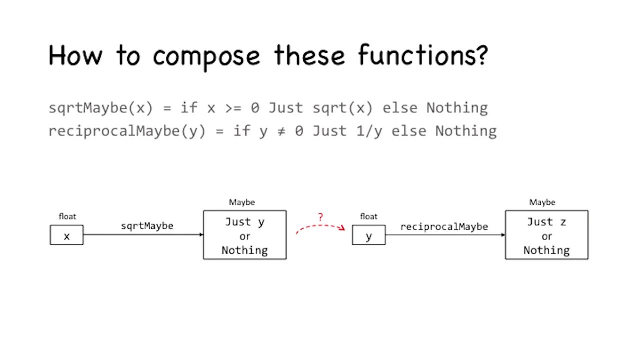 but I'm really better off leaving it like this and doing something slightly different, doing something monadic. What we want to do now is find a way to apply reciprocal maybe to not just a float but to a maybe a float type thing. And if you notice, 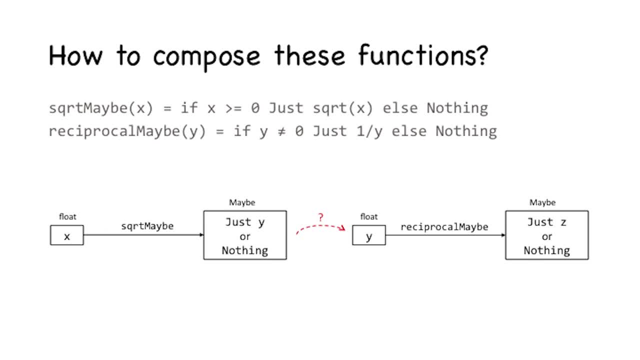 that red arrow with a question mark in it kind of suggests that what I'm going to do is tweak the definition of reciprocal maybe so that it turns- first turns a maybe into a float and then takes that float, and that's not exactly what I'm going to do. 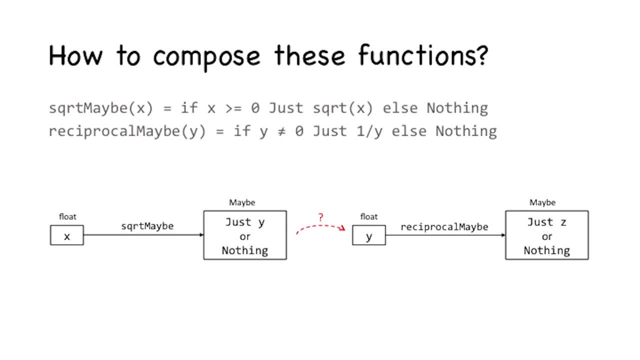 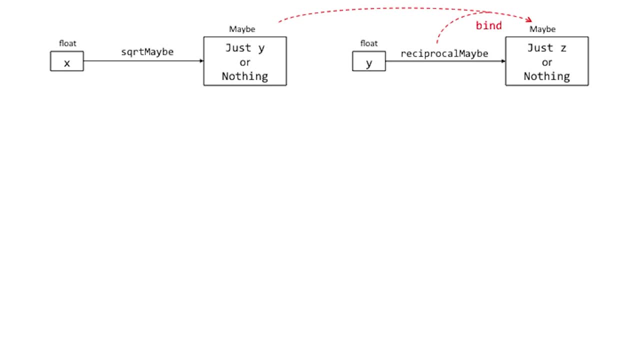 That red arrow with a question mark is kind of going to go away and get substituted for something much better. And what it's going to get substituted- what I'm going to substitute for it- is something called bind. Now, what does bind do? 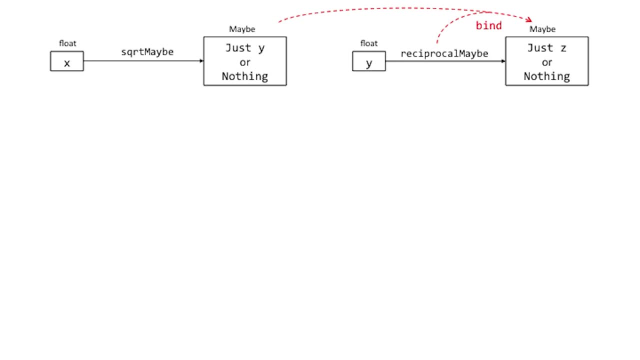 Bind in as general a way as I can, tells me how to start with a maybe thing and also start with something like reciprocal maybe, a function that's meant to apply to an ordinary float, and to come out the other end with a maybe type thing. 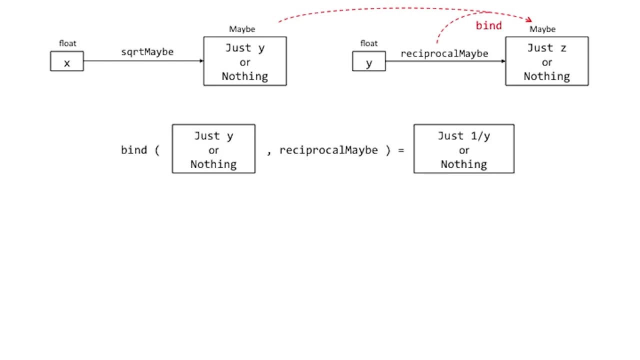 Okay, So bind is going to take two arguments. It's going to take a maybe type thing and a function such as reciprocal maybe, and it's going to tell me how to take those two things, combine those two things and end up giving me a maybe type thing. 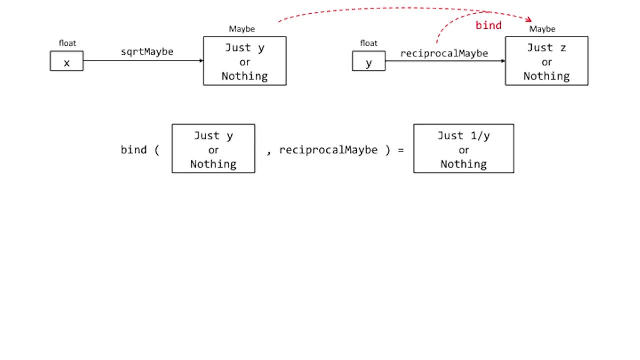 Okay, that's the thing that bind is meant to do. It's got two arguments: one is a maybe, one is a function, and it gives me a maybe. All right, let's be just a little bit more general here. That reciprocal maybe is a certain kind of a function. 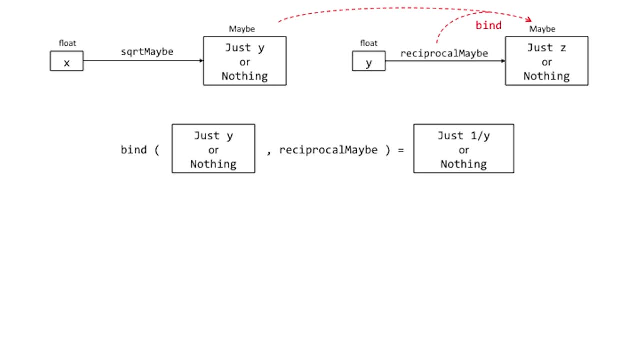 but it's not the only function on the block, It's not the only function that can ever take a float and give me a maybe. There are lots and lots of functions that I might imagine having there. instead of just the reciprocal function, I might want to take the square root again. 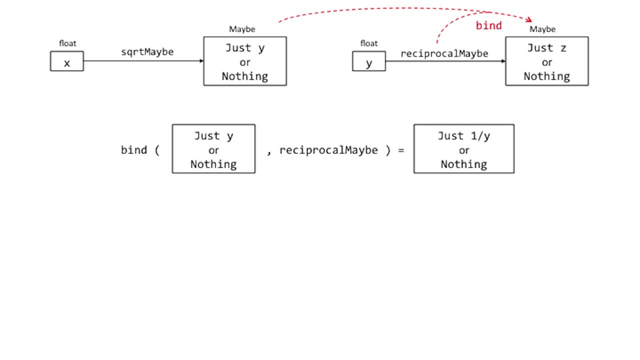 or I may want to, I don't know. take the arctangent or some anything. Any number of things might be substitutable in this expression instead of reciprocal. maybe I have to be a little bit careful, because what I put in place of reciprocal maybe. 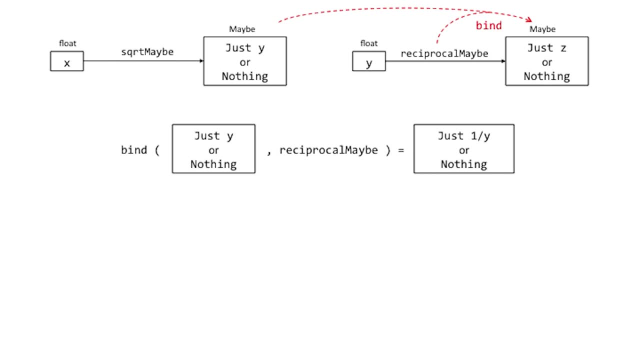 has to take a float and return a maybe thing, But it can be more general than just reciprocal maybe. So when I talk about bind, what I'm going to say is this: This version of the bind function takes a maybe and any function of the correct kind. 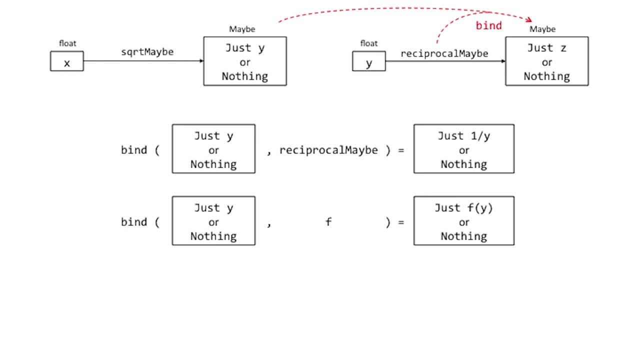 call it f and gives me a maybe back. That's how I'm going to operate Now. what I have to do here is I have to define what bind is going to do, And it's not going to be so terrible, It's going to do pretty much. 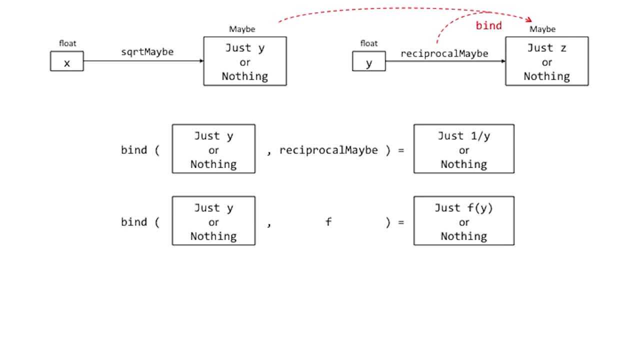 what you would think this bind is supposed to do, For example, with reciprocal. maybe if I bind just 2 and reciprocal, maybe I'm going to get just 1 over 2.. It's going to take the reciprocal, But notice, I start with a just 2. 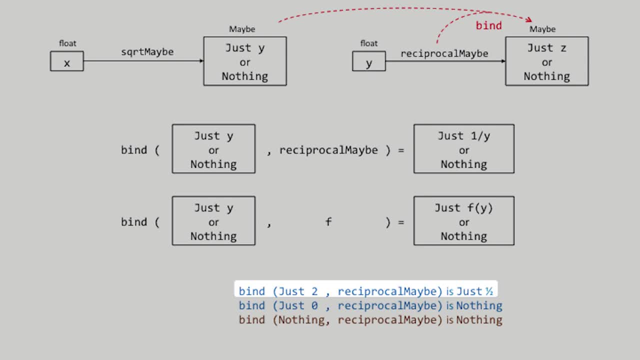 and I end up with a just 1 half. I start with a maybe object and a float and I end up with a maybe type of thing. Okay, what about when I'm applying nothing to reciprocal maybe If I bind together nothing? 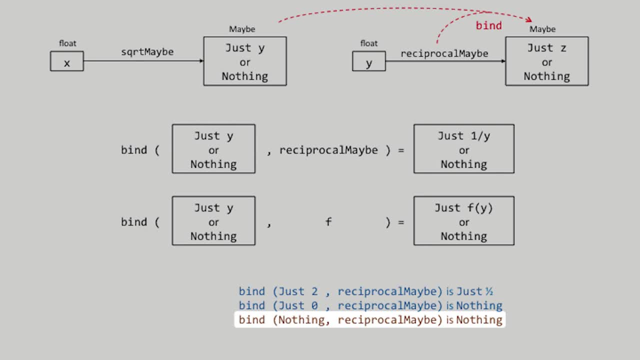 and reciprocal maybe. well, I better darn well get nothing. I can't take 1 over nothing and get something useful. So my general rule for binding together a, maybe afloat with the right kind of function f, is, if I start with just 1,. 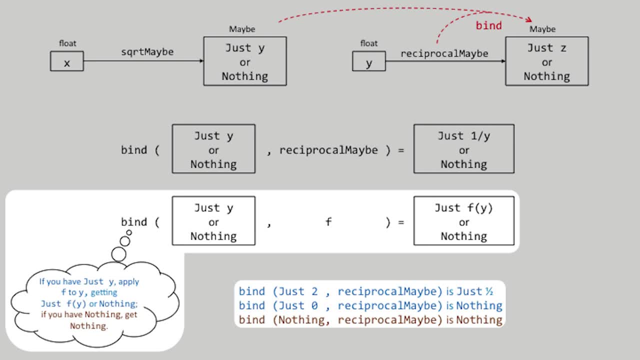 I'm going to apply f to y and I'm going to get just f over y. On the other hand, if I start with nothing, then when I apply f, I end up getting nothing, And that's going to be my general rule. 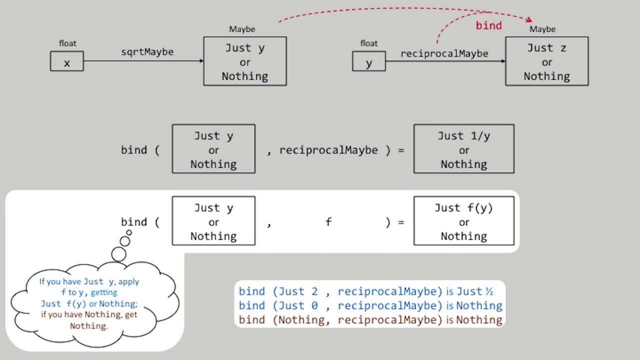 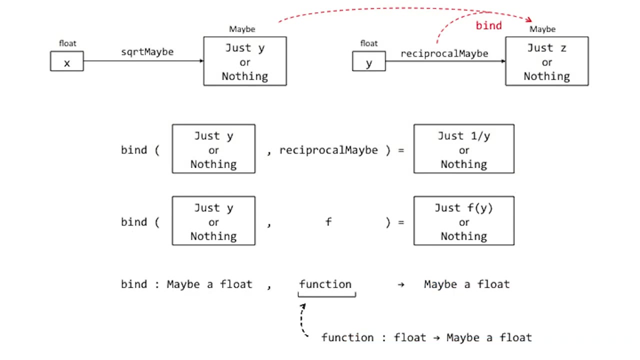 That's going to be the way bind works- at least this version of bind, whenever I start with a maybe object and the right type of function. So let's look at this. What type of an animal is this bind function? Bind takes two arguments. 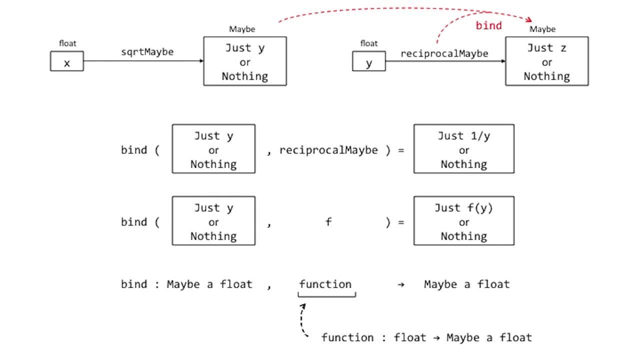 It takes maybe afloat and a function and returns- maybe afloat, And that function has to be the right kind of function. That function has to be the kind of function that takes afloat and returns- well, in this case, maybe afloat. 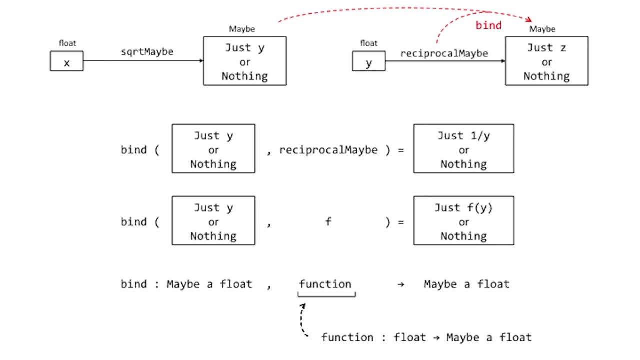 It can be a little bit more general than that. It doesn't have to be maybe afloat, but it has to be a maybe type thing of some sort. That's the way bind is going to work in this incarnation of bind. Once again, what bind is doing. 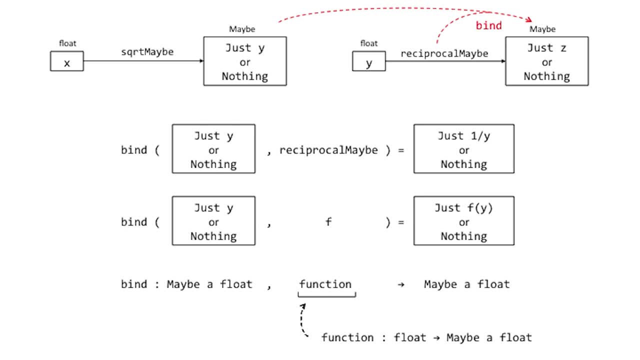 is telling me how to apply something like reciprocal maybe to a maybe object, a maybe thing that I may have gotten from a previous function application. Okay, has this solved the functional style version of the problem for one over square root? Yup, it has. 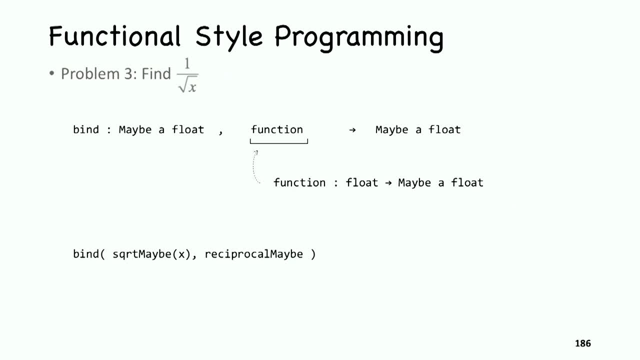 Because if I'm trying to find one over the square root of x now, I can first take the square root maybe of x, that gives me a maybe object, and then I can bind that together with reciprocal maybe. One way or another, I'll either get. 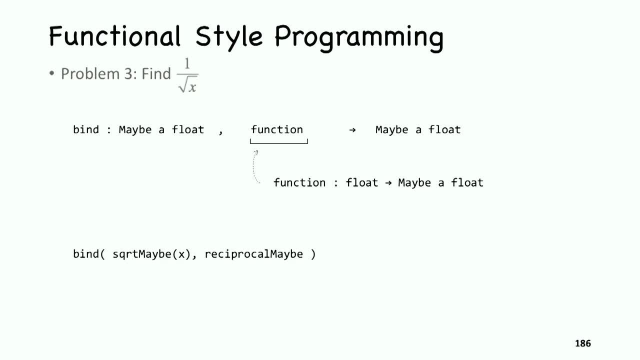 just one over the square root of x, or I might get nothing if it turns out that the square root of x is zero or if the x that I start off with is negative one. But now the error handling the stuff that I handled with is error. 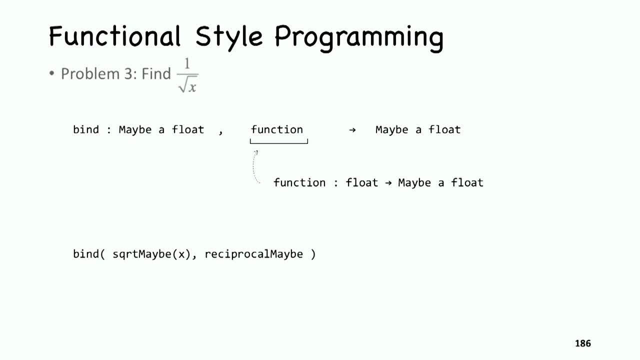 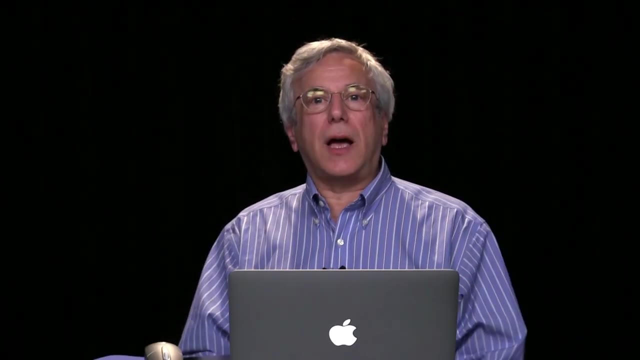 in the imperative style version of the program is swept under the rug with the notion of a maybe and with the notion of bind. Now, sweeping things under the rug, that's an expression that you ordinarily think is not a good expression, but in computer programming, 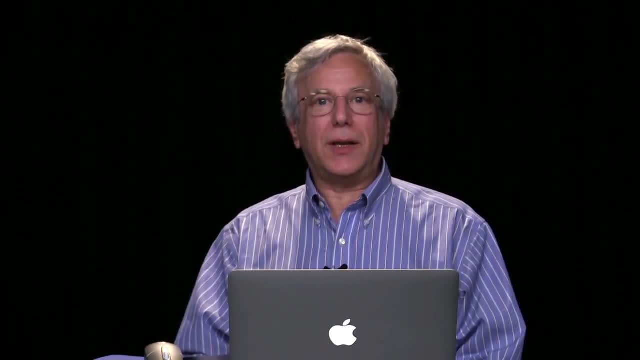 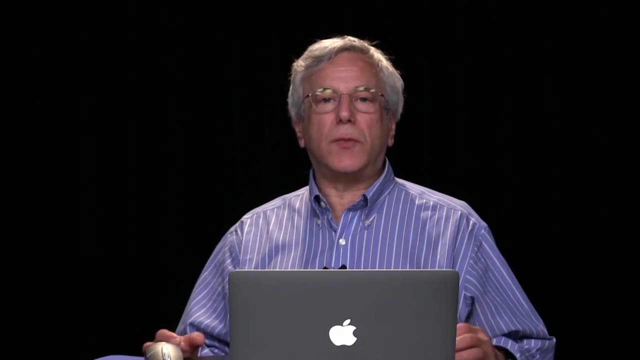 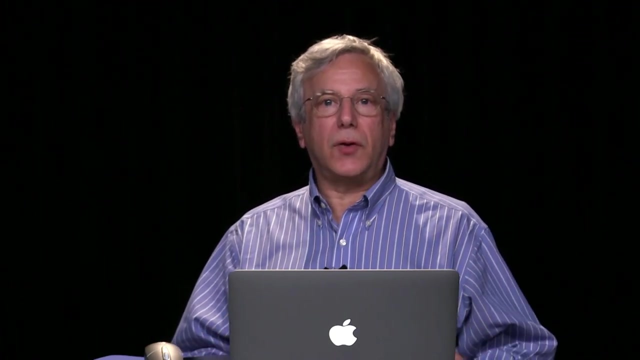 we like to sweep things under the rug. We like to take the complicated parts of a program, the parts that don't have to do so much with the direct logic in the program, and make them be handled automatically, automatically by the programming language. 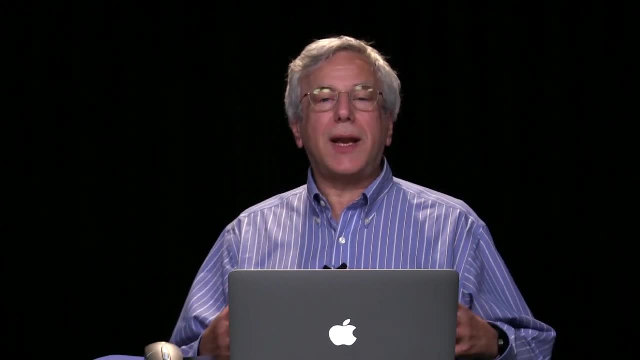 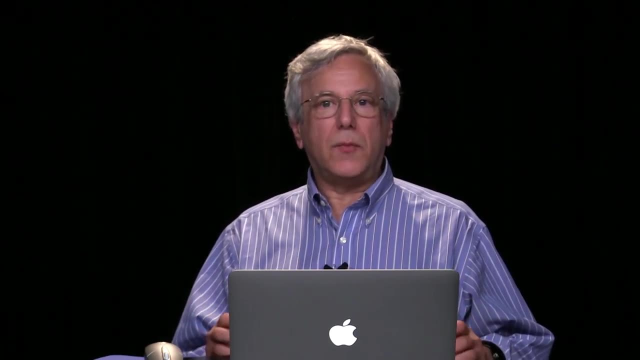 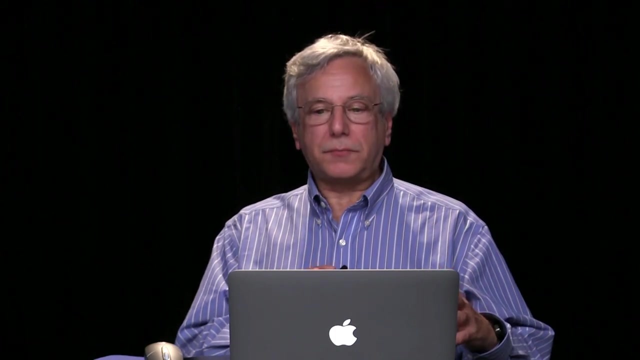 automatically by the runtime, automatically in some way, shape or form. So the fact that we've swept the ifs and the errors under the rug by considering such a thing as maybe a float and bind is a very good thing. Let's take a look at. 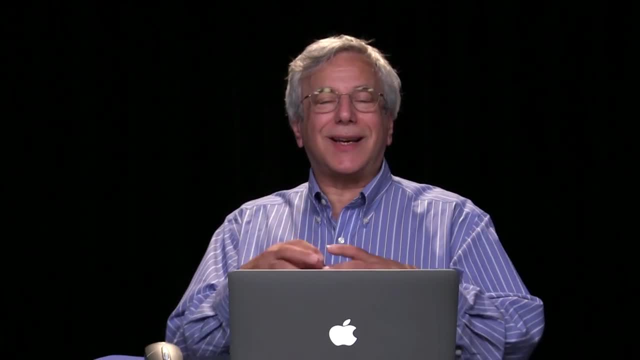 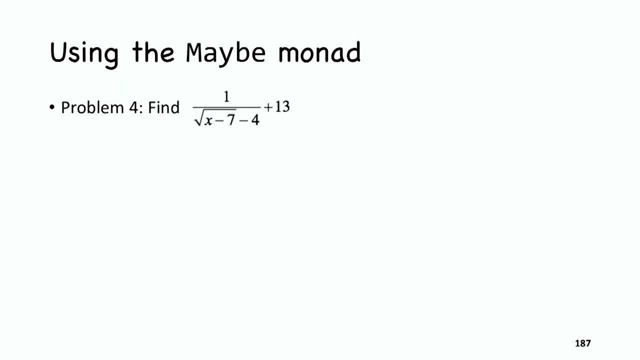 how we would combine this now with just a slightly more complicated computation. I'm going to start by trying to take one over the square root of x, Square root of x minus 7 minus 4 plus 13.. It's not too much more complicated. 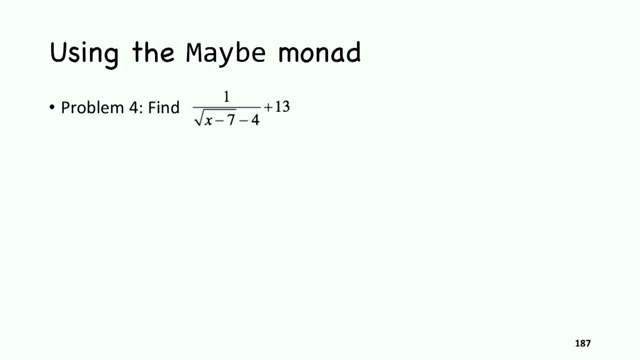 because again, there are really only two places where things can go wrong. I can try to take the square root of x minus 7 and get a negative number, or I can end up with 0 in the denominator and have the whole thing blow up. 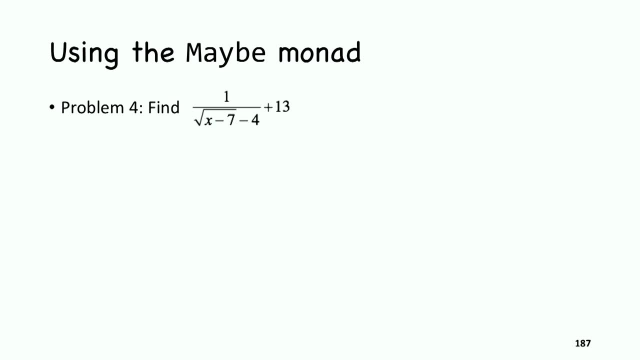 because I'm trying to take 1 over 0. There are really only two things that can go wrong, but it's still just a bit more intricate than starting off with just 1 over square root of x. Okay, in order to solve this problem, 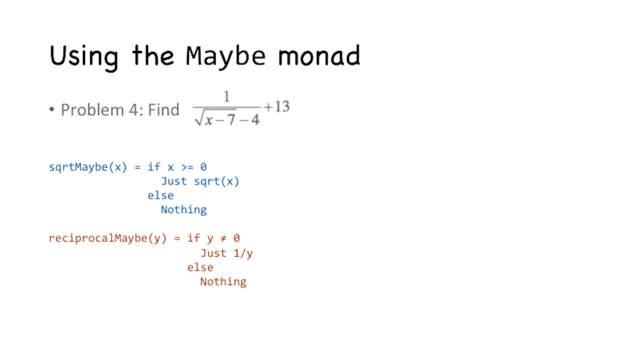 I'm going to have my square root maybe again. I'm going to have my reciprocal- maybe again, but I need two more functions. I need a function that I'm going to call minus 4, maybe, and another function that I'm going to call. 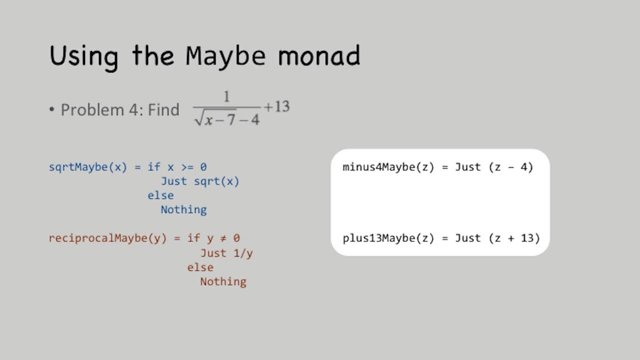 plus 13, maybe My minus 4, maybe. function is well, it's going to subtract 4.. However, it's going to take a float value and return a maybe It's going to return, maybe a float. Notice that on the right-hand side. 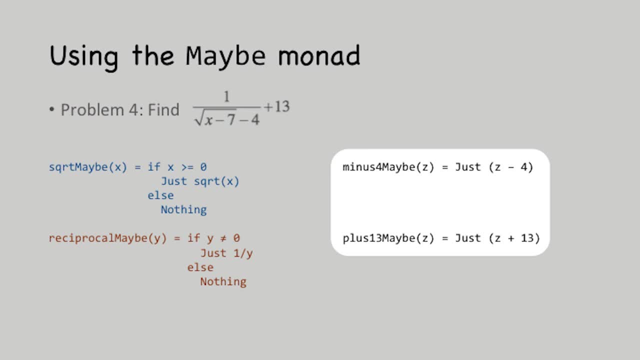 of the definition of minus 4. maybe it doesn't say z minus 4, it says just z minus 4.. So once again I have one of these functions that's shaped in a way so that it starts by taking on the left end. 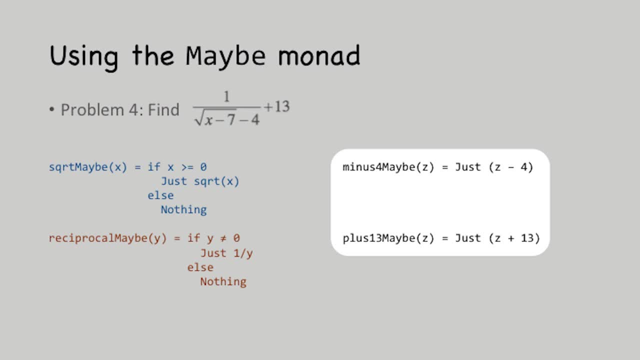 this little float thing and ends up on the right end of the arrow, giving me this bigger maybe type thing, And I'm going to define another function called plus 13. maybe that works in pretty much the same way If I start with 7,. 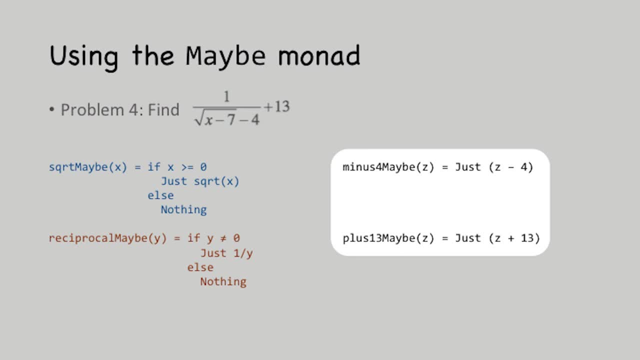 it ends up giving me just 20.. If I start with 0, it ends up giving me just 13.. If I start with minus 7, it ends up giving me just 0.. So now, in order to solve this new calculation, 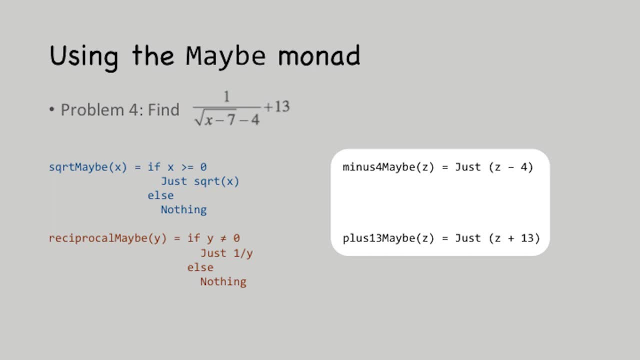 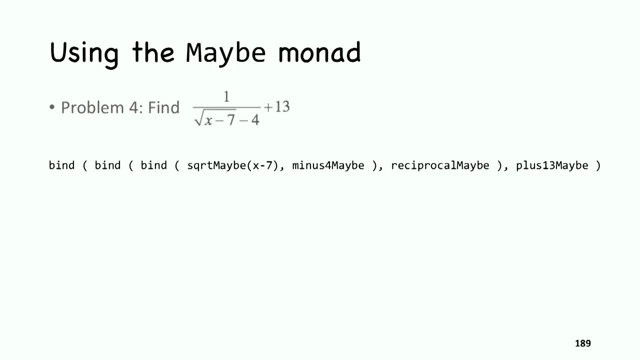 what I have to do is combine these four functions in a row. Hmm, okay, let's see how it's going to be done. I'm going to do bind, bind, bind, Okay. First, I'm going to take the square root, maybe, of x minus 7.. 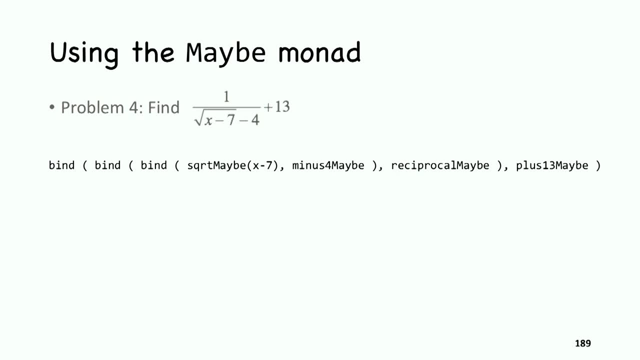 And, by the way, I don't have to fuss about x minus 7.. When I subtract 7 from x, nothing can go wrong. So I didn't bother to create a minus 7 maybe function I could have done that, but 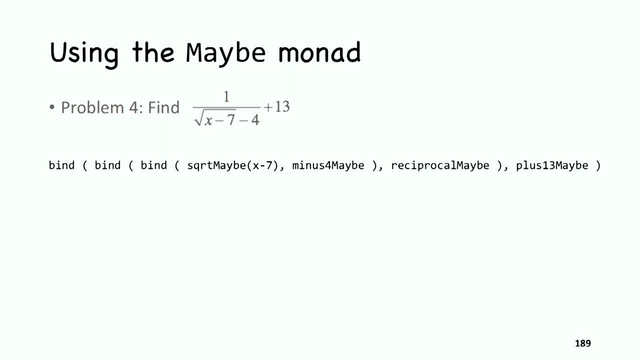 I don't think I would have gained anything by it and just maybe had made the slide longer and harder to read. First I'm going to take x and subtract 7 from it. Then I'm going to take the square root, maybe of that okay. 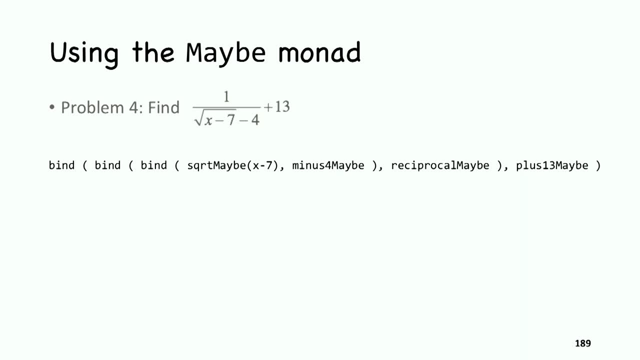 And then I'm going to bind that to minus 4 maybe, And then I'm going to bind that to reciprocal maybe, And then I'm going to bind that to plus 13 maybe. Okay, bind, bind, bind The reason. I've got three binds there. 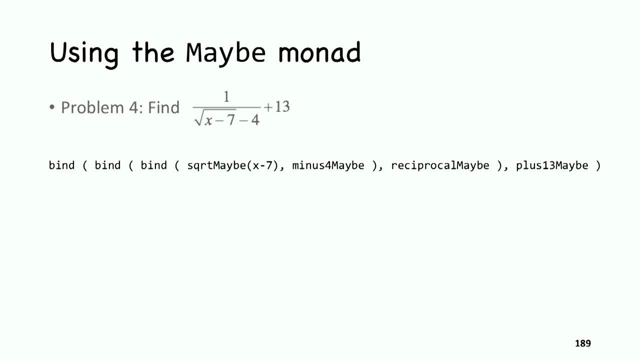 is because I've got so many operations to perform and each one of them has to take a maybe and take it into another maybe. You know what It would be easier here to think of bind not as a function with parameters. I can do that. It's still going to be a function. 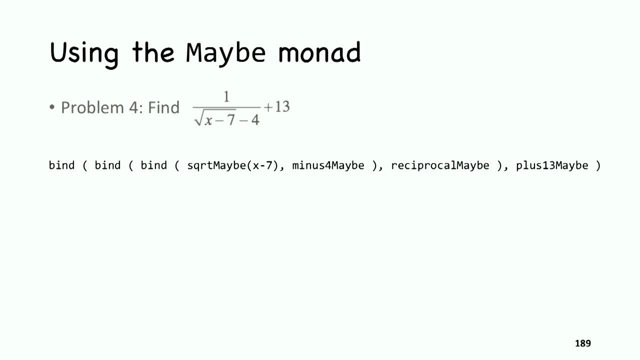 with parameters, But maybe it would be easier to visualize this if I create a binary operator for bind, Something that looks like a plus sign and can be put in between two values. Let me do that. Ha, I just happen to have a slide for it On the bottom. 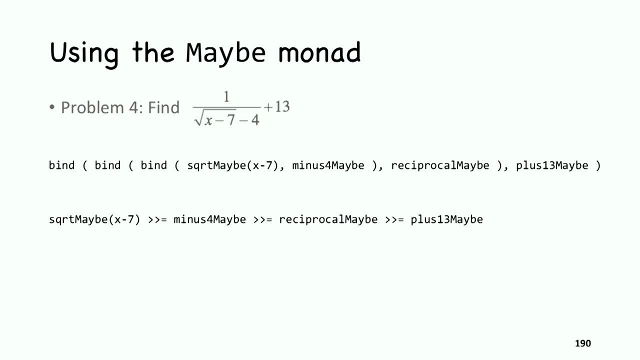 of this slide. what I'm doing here is I'm saying: take square root maybe of x minus 7 and then use that greater than greater than equal sign to stand for infix bind. Take square root maybe x minus 7 and bind it to minus 4, maybe. 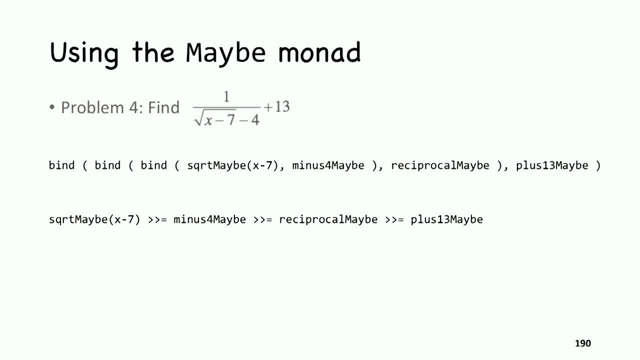 and then bind the result of that to reciprocal maybe and then bind the result of that to plus 13 maybe. The two strings of square root maybes and minus 4 maybes, and everything on this slide have exactly the same meaning. I'm just using slightly. 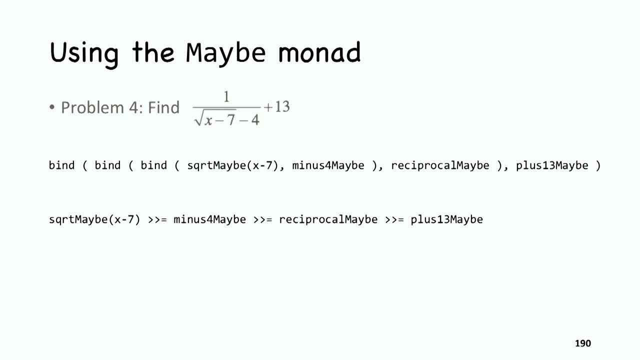 different notation, And the thing that this greater than greater than equal operator gives me is just another way of writing. bind is to just make the expression a little bit more readable, A little bit more compact. Okay, Let's take a look at how it. 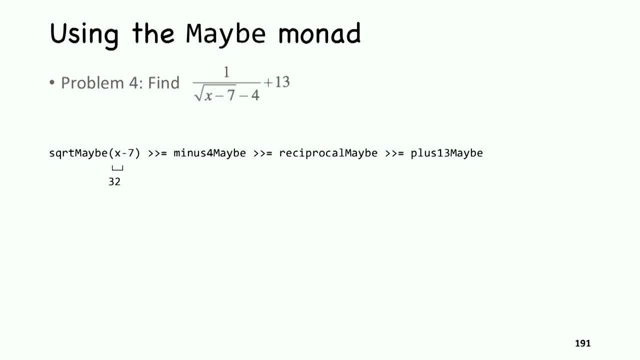 works. I'm going to start with the value of 32 for x. When I subtract 7 from it, I get 25.. So far I don't have any maybes sitting around. No justs, no maybes. But when I apply, 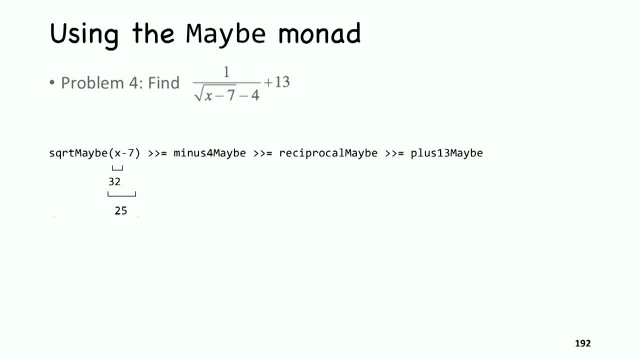 square root maybe to 25, I get the value just 5.. Now the bind operator that comes after that and points to minus 4. maybe that tells me how to combine the function minus 4 maybe with the value just 5.. Okay. 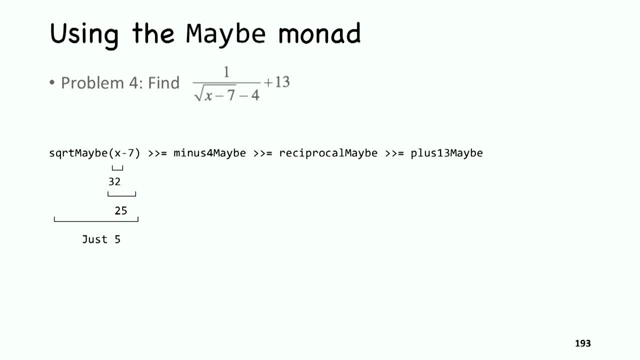 According to the rule of bind, I'm going to end up with just 1.. And now that I've got just 1, I bind that maybe value with reciprocal maybe And according to the rules of bind, when I bind just 1 with 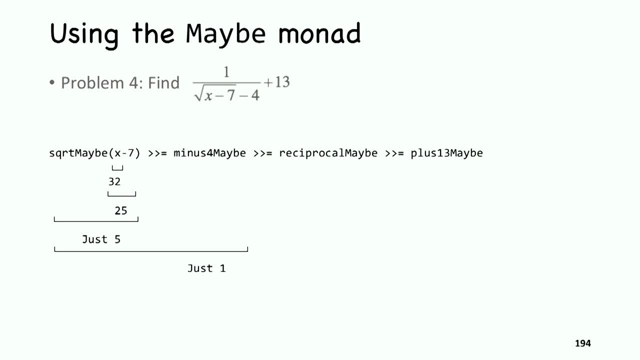 reciprocal, maybe. I get just 1 divided by 1. 1 over 1.. Well, okay, That's just 1.. And then finally I have to bind it to plus 13 maybe. So now I take that just 1. 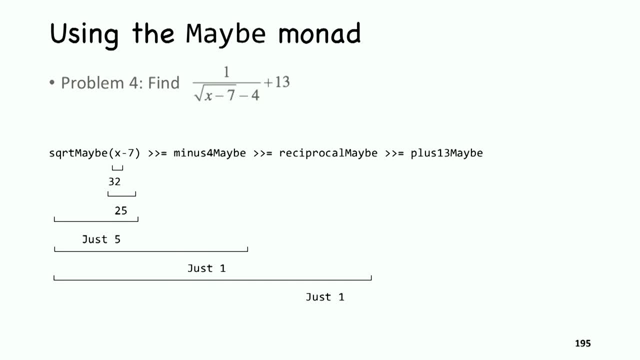 and I apply my bind rule again: Find out what plus 13 gives me. Plus 13 maybe gives me, And what it gives me is just 14.. Very, very nice. Actually, nothing went wrong here. Huh, Wait a minute. Maybe I didn't need this. 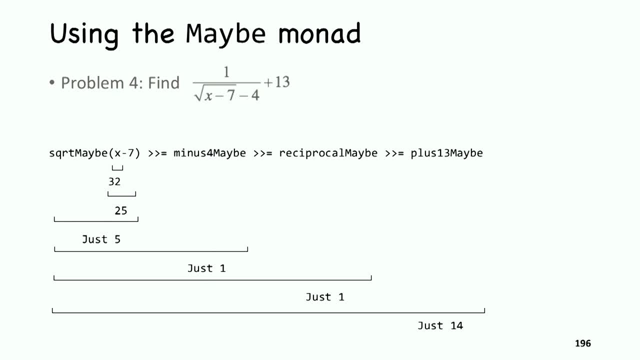 maybe error handling stuff to begin with. Ah yes, There are situations in which I will need it. Let's start, for example, with 6.. If I take 6 and I subtract 7 from it, I get minus 1.. 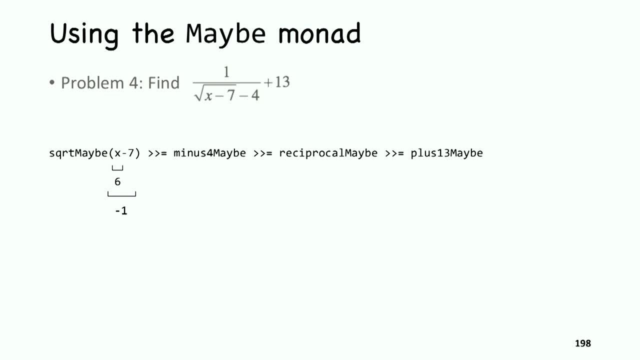 And then I take square root maybe of that. Well, let's see The square root maybe function when I apply it to minus 1, gives me nothing. Sorry, no answer. You didn't get anything there. Now, what does bind? 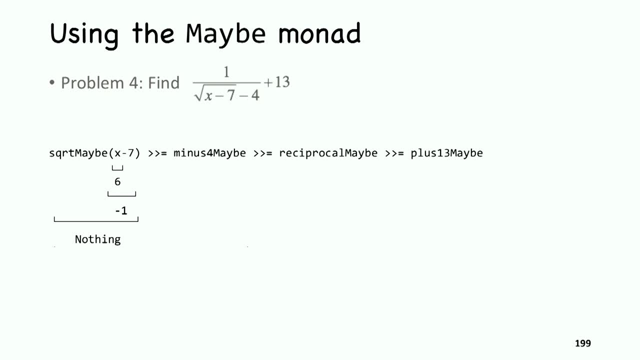 say about binding nothing to a function like minus 4. maybe Bind says that if you start with nothing- in this case on the left-hand side- you end up with nothing, no matter what minus 4 maybe says to do. So I end up here with nothing. 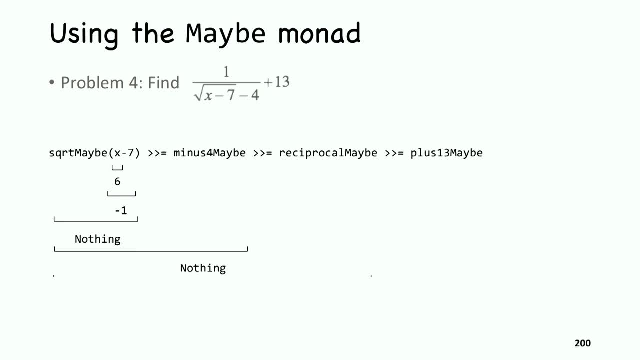 after binding with minus 4, maybe. And again, if you try to bind nothing to reciprocal, maybe you get nothing. And again, if you try to bind nothing to plus 13, maybe you get nothing. Aha, Without having any obvious. 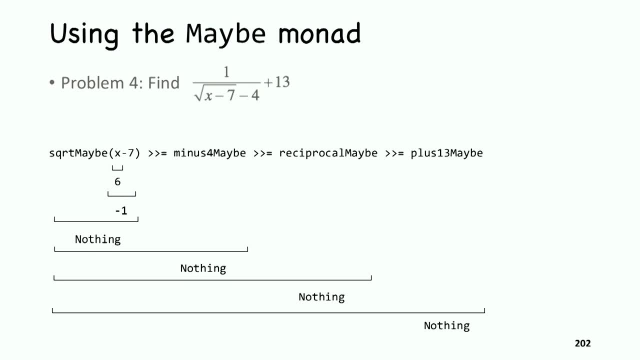 looking if statements in the code, just a string of things with some arrow-like looking operators between them, I end up with the correct answer: error handling and all. Let's try one more situation. Let's start with 23.. Yes, I did hand-pick that. 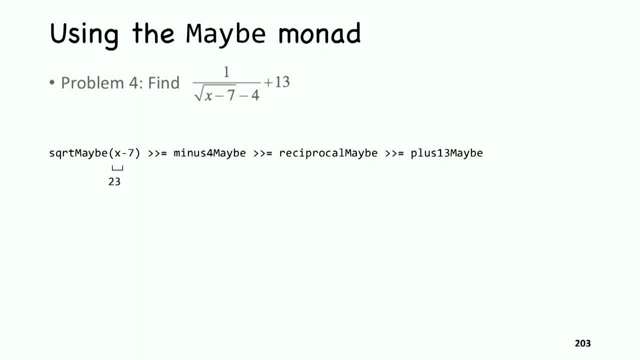 value, because it does something interesting for me. When I subtract 7 from it, it gives me 16.. Okay, what happens when I take square root maybe of that, I get just 4.. That's a maybe type thing. It's a. 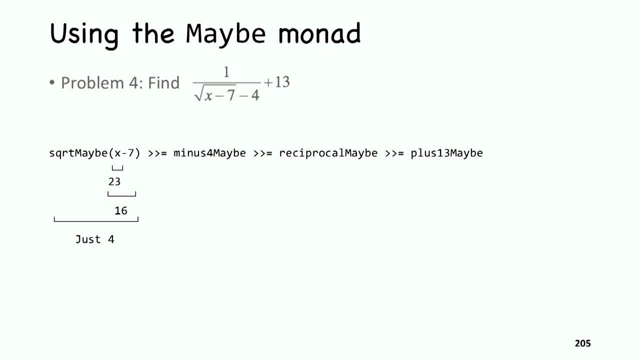 maybe type thing. so I have to bind it to minus 4 maybe. Yep, When I bind minus 4 maybe to just 4, I get just 0. And what happens when I try to bind just 0 to reciprocal maybe I? 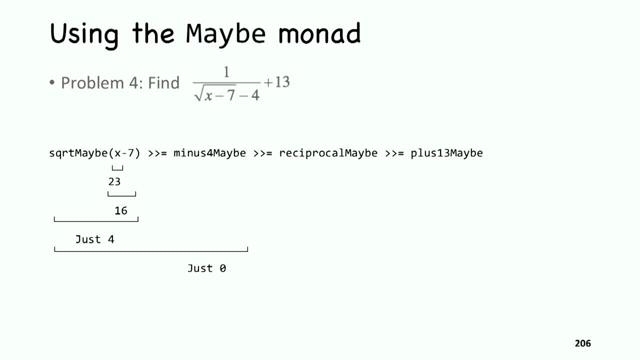 actually do end up binding it, But the binding rule tells me that I get nothing. Because that's the way reciprocal maybe works. Reciprocal maybe ends up giving me nothing because it gets applied to 0.. Okay, Now having gotten a nothing. 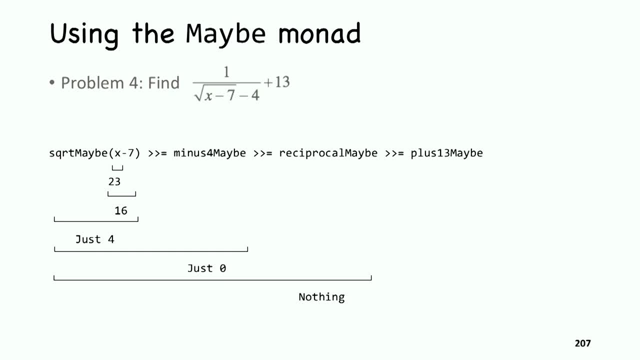 I say: how am I going to bind that nothing to plus 13 maybe? Well, when you bind nothing to any function, then you get nothing back. So again, I've solved the problem. I've gotten nothing, which in this case, 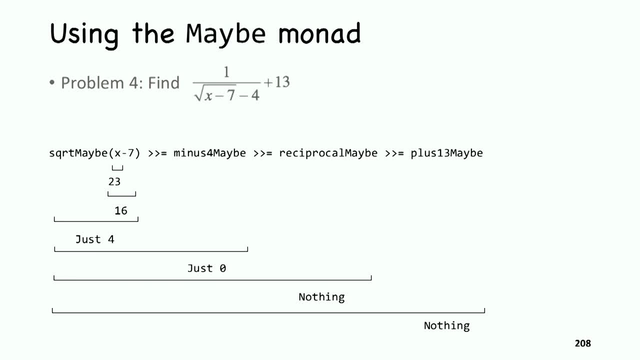 is the right answer. And I didn't use any ifs, I didn't use any loops, I didn't use any exception handling. I just used higher order functions and the maybe monad. This is really cool. Now I once read a book. 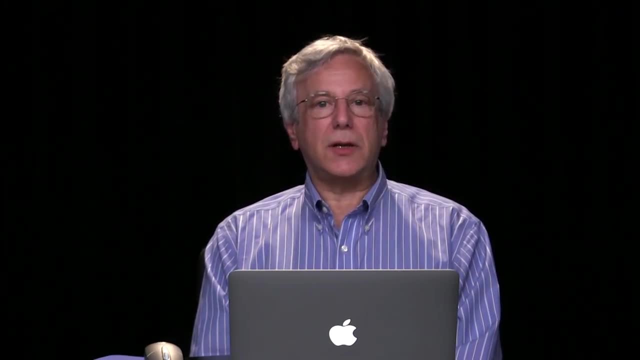 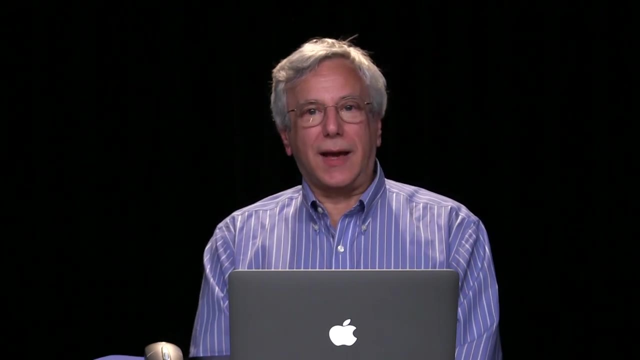 where it said: don't define any new terminology unless you're going to use that terminology more than once. That's very sensible advice. So what about this word monad? And I have this word monad and I apply it to these maybe things. 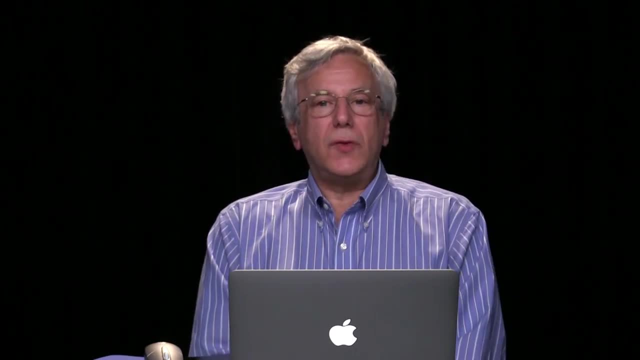 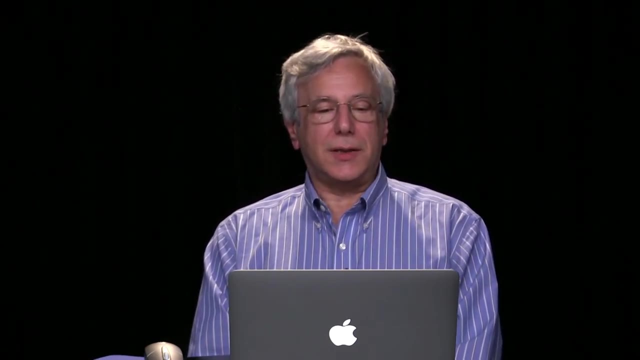 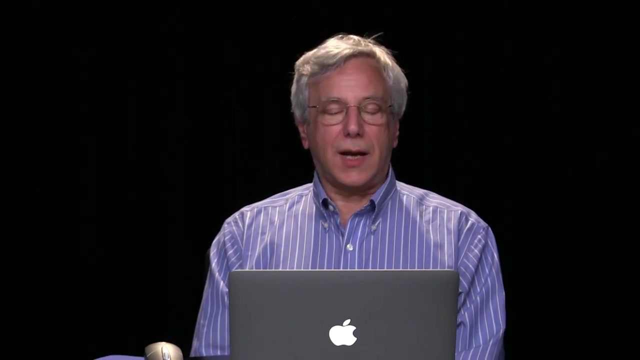 and to error handling, and that's fine. but why bother making up a new name for it? Why bother making up a new name for the bind function if all it's going to do is be applied to these error handling situations? Aha, The notion of a monad. 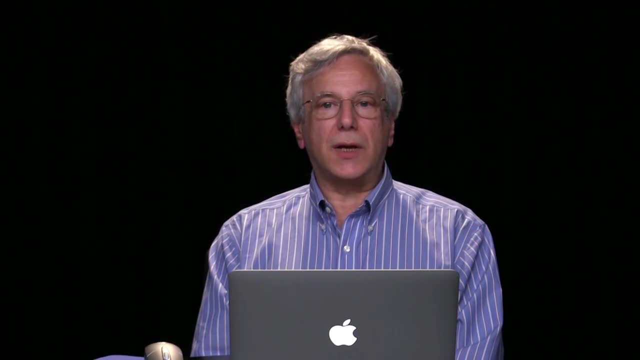 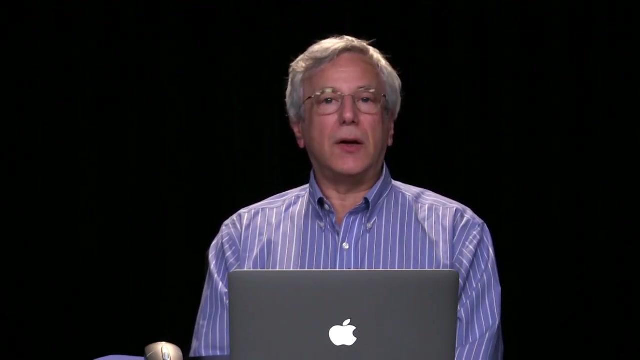 and the notion of a bind function is very, very general. What I'll do in the next segment is use the notion of monads and use the notion of a bind function to get yet another kind of problem solved, A completely different kind of problem solved, One that you 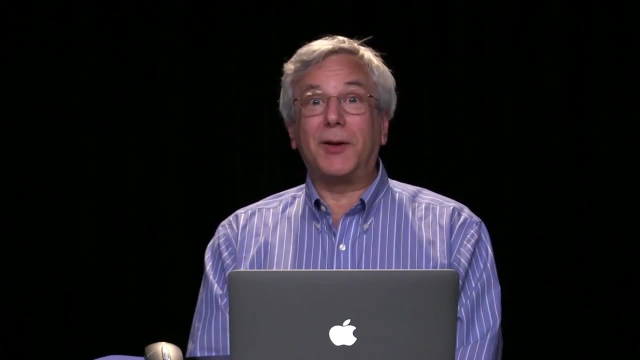 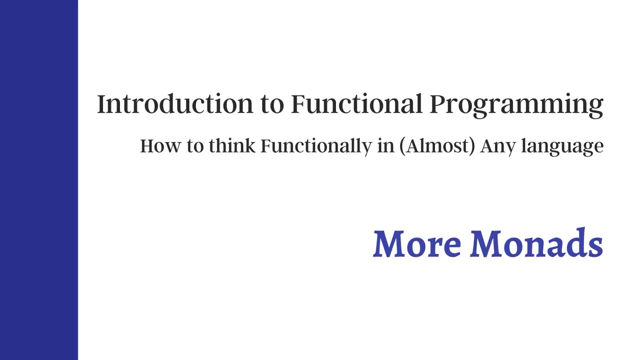 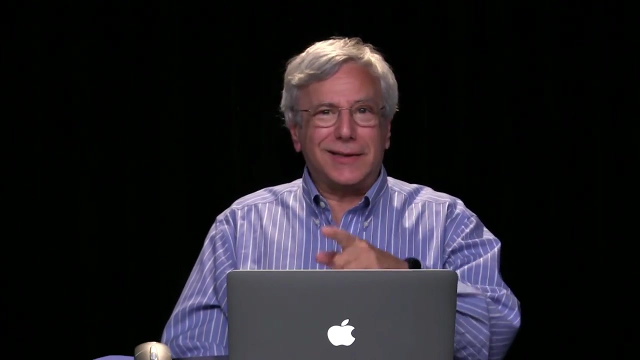 wouldn't think of from the stuff that I've done in this slide. I'm looking forward to it. See you then. In the previous segment, I told you that monads are good for more than just maybe type things, And I was right. Let's take 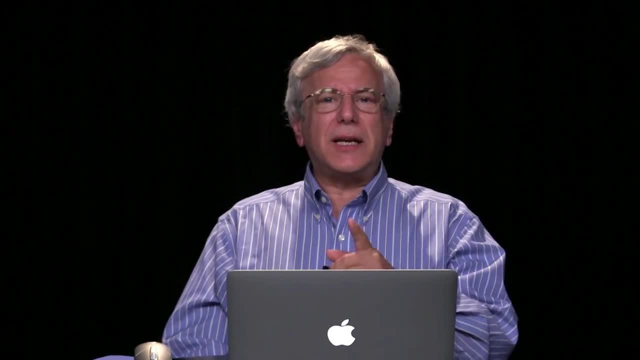 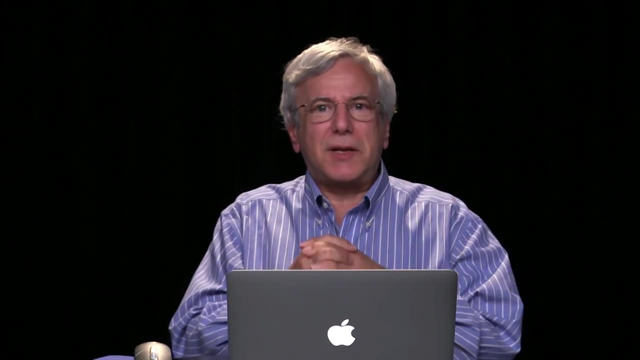 a look at something that doesn't look anything like maybe, but still can make good use of the notion of a monad. I'm not even going to use numbers for this. I'm going to take a person named Ann. What's so special about Ann Well? 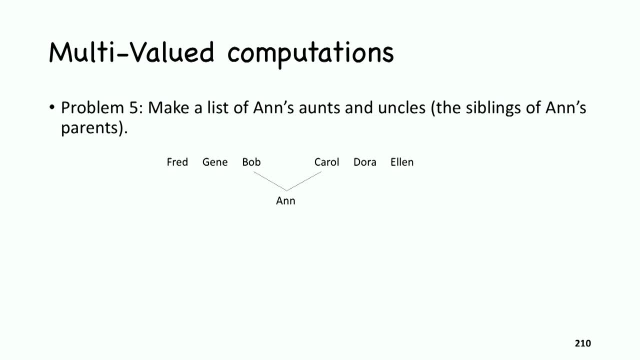 she has a biological father named Bob and a biological mother named Carol, And Bob and Carol, being parts of families, have siblings. So Bob has two siblings named Fred and Gene, and Carol has two siblings named Dora and Ellen. And the problem that faces me- 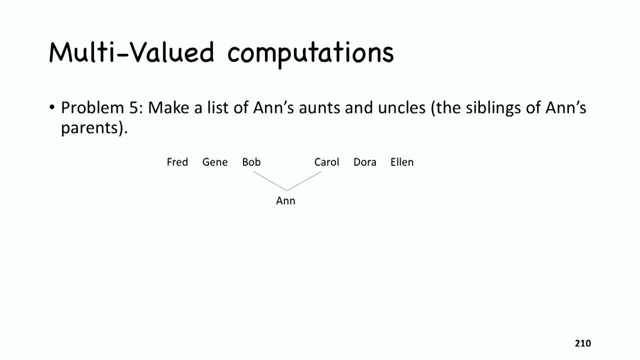 computationally is to find all of Ann's aunts and uncles. Okay, How am I going to do that? I'm going to create functions, Let's do it. I'm going to create a parents of function, and the parents of function is going to take a person. 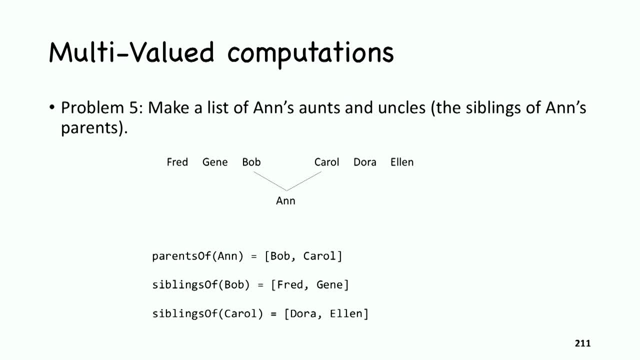 like Ann and it's going to give me a list, such as Bob and Carol, And I'm also going to have a siblings of function And the siblings of function will start with somebody like Bob and give me Bob's siblings, Fred and Gene, Or it'll. 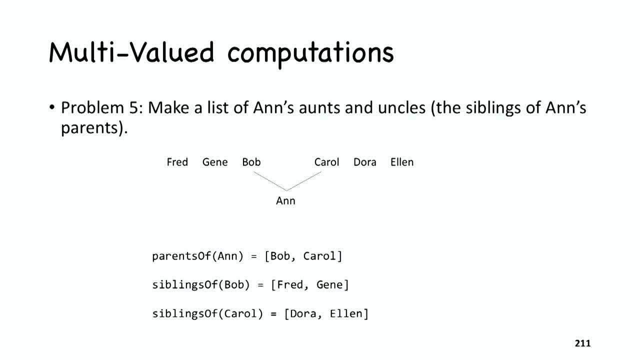 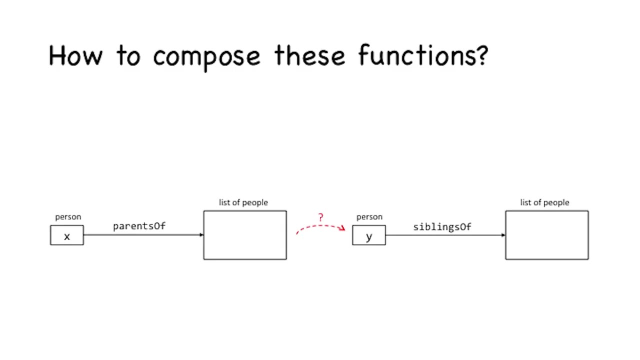 start with somebody like Carol and give me Carol's siblings, for instance Dora and Ellen. What in the world does this have to do with monads? Well, the next slide shows you a diagram that I hope looks familiar. I start with person X. 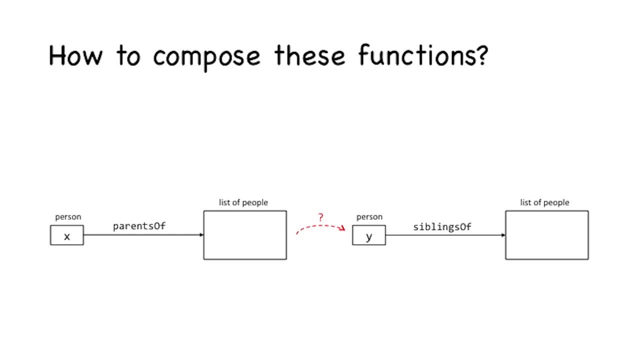 and I apply the parents of function- to get something bigger than X, Bigger than just a person. It's a list of people. Now, if you remember, when I talked about maybe monads, I started with a float and got something that was kind of bigger than a float. 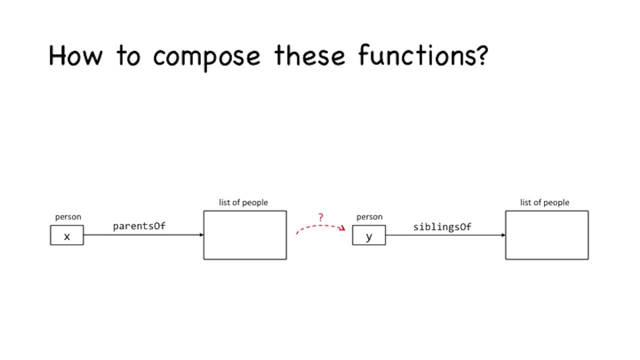 It was just a float or a nothing. I'm doing the same thing here. I'm starting with a person and ending up with a list of people, Something that's a little bit bigger And with the siblings function. I'm starting with a. 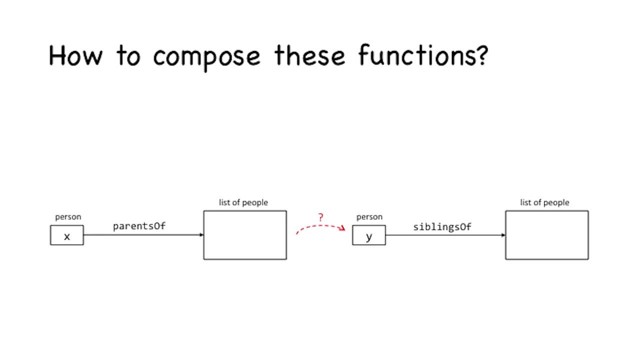 person and ending up with a list of people, And what I want to do again in order to find aunts and uncles, is to first apply the parents of function and then take what I get from that and apply the siblings of function. However, 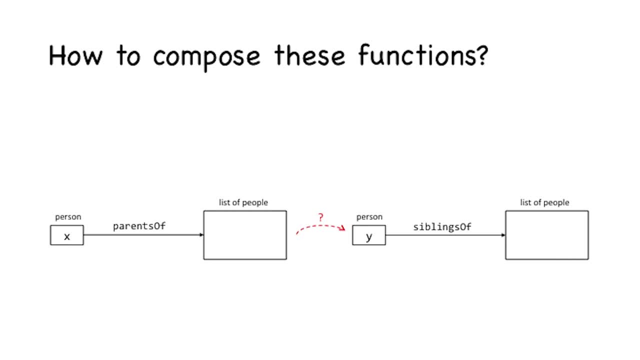 once again I have that red arrow with a question mark over it. How in the world am I going to apply the siblings of function, which takes just a person, and apply that to a list of people? Now, of course, if you're sloppy about types, you just. 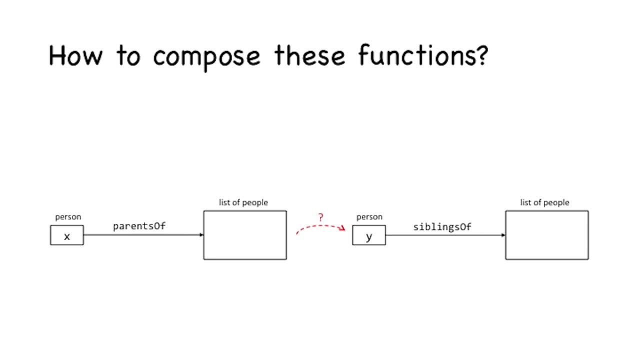 do it In an imperative language, you make yourself a loop. Not a big deal. But I want to be really careful about types, and the reason I want to be really careful about types is number one, because being careful about types pays off in terms of the correctness of 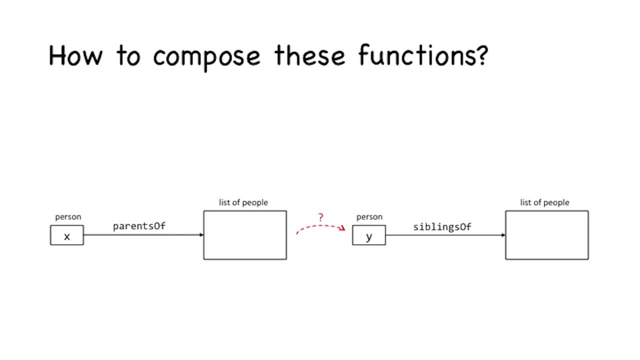 your program, but also because I want to show you that if we concentrate on the types of things, we will find. this is another situation of a monad and the use of a bind function. Let's have a look. I start with Anne and I apply. 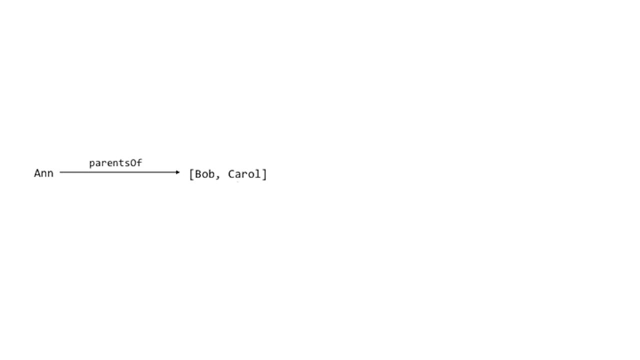 the parents of function and I get her parents, which is a list, not just a single person, It's a list of two people, Bob and Carol. For Bob, I apply the siblings of function and I get yet another list, Fred and. 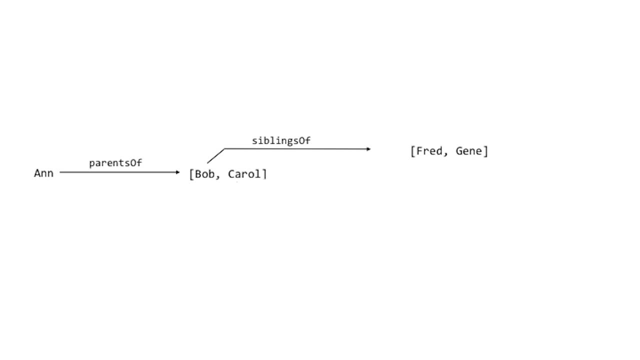 Jean, Okay, list, let's see person to list to list. but wait a minute, I haven't finished getting all of Anne's aunts and uncles. I have to apply siblings of function again. I'm going to apply that to Carol and from there. 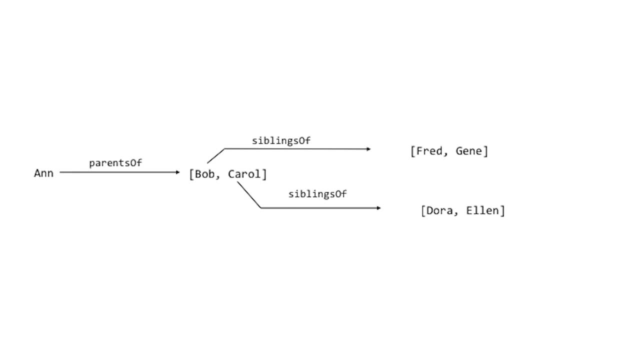 I get another list. so now I've got two lists. I've sort of got a list of lists. yeah, those big red brackets are meant to indicate that the whole thing is a sort of a bracketed list for me and I kind of have to do something about that. 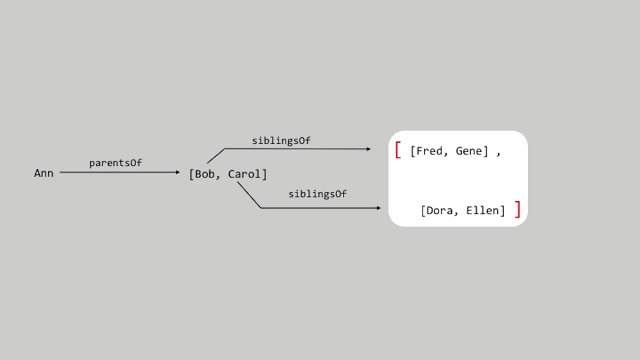 because if you ask me who are the aunts and uncles of Anne, I'm not going to tell you that there were two entities, a Fred Jean entity and a Dora Ellen entity. I'm going to want to tell you that there are four entities. 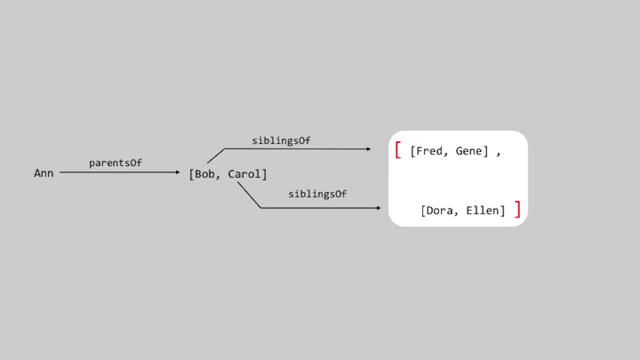 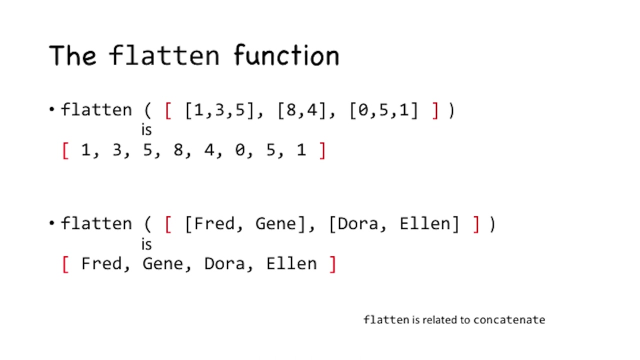 so I want to go from this red looking list of lists to a just plain old list, and to do that I'm going to make up a new function name. I'm going to call it the flatten function. Now, to be painfully honest here, I have to admit. 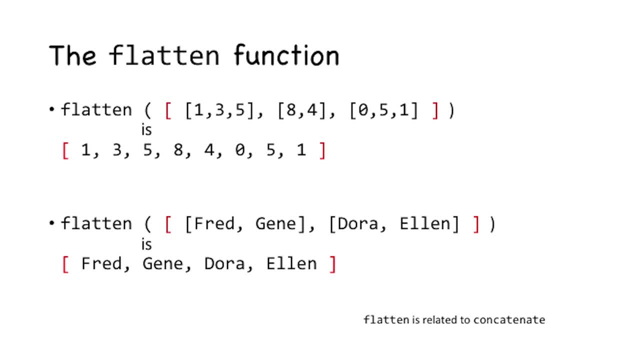 flatten is really well concatenate is flatten in disguise and vice versa. but I'm not going to worry about that similarity here. all I want you to notice is that when I apply the flatten function, my flatten function, to a list of lists, I get a list. 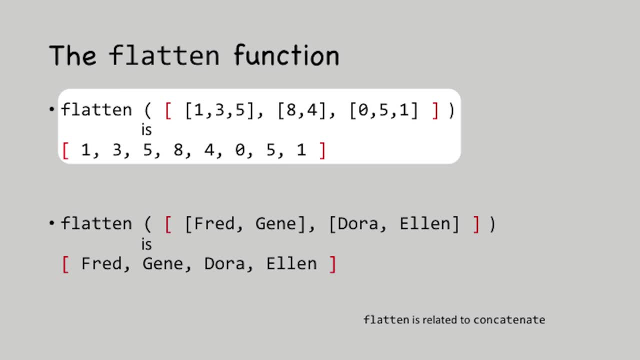 of just plain old things. okay, so if I try to flatten the three lists- one, two, three, eight, four, zero, five, one- then what I get back is just the plain old list with the values one, three, five, eight, four, zero, five one. 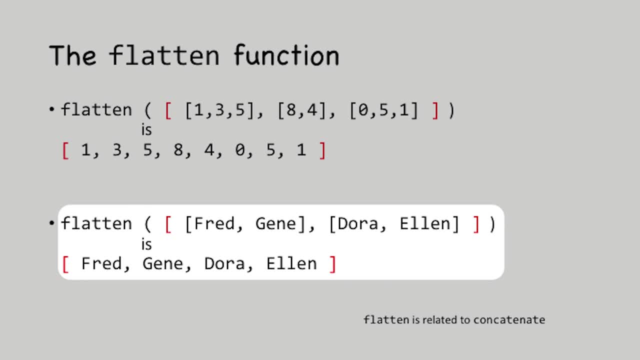 and similarly, if I take the two results of the siblings of function- the Fred and Jean list and the Dora and Ellen list- and if I apply flatten to those, then what I get is a plain old list that has four elements in it: Fred, Jean, Dora. 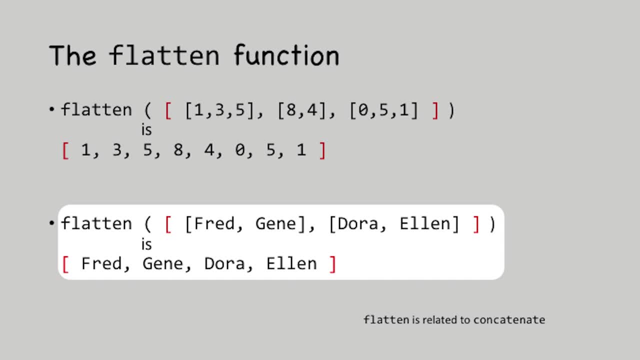 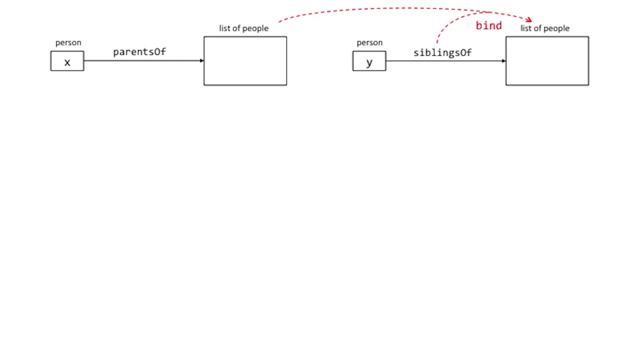 and Ellen. so flatten is going to be the essential tool that I use when I define bind for this scenario. this set of functions, monads. okay, here we go again. this is exactly the same diagram that I had before in my previous segment. 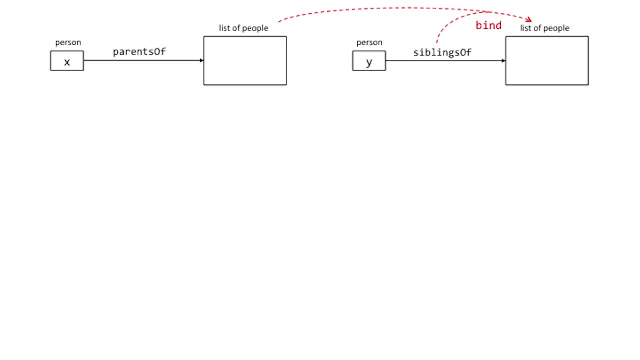 when I was talking about maybe only the labels on the boxes are different. instead of taking the square root maybe of a float, I take the parents of a person and I don't have the word maybe. there I'm not doing a possibly erroneous calculation, instead what I'm doing. 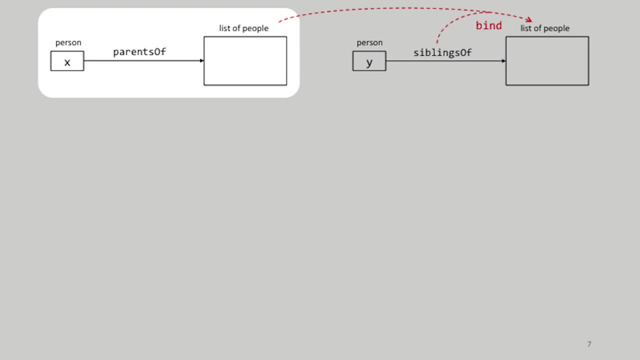 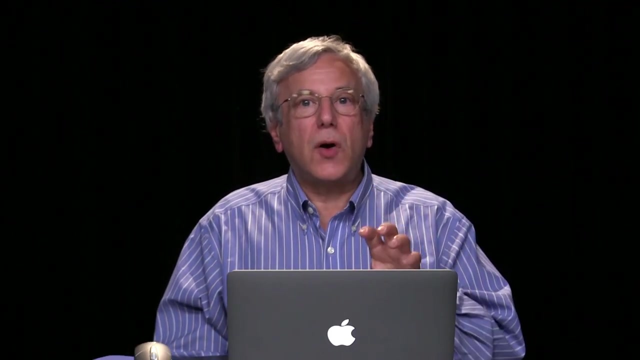 is going from a person to a list of people, a bigger block of stuff, maybe not bigger, but I'm going to something different- and that list of people- yeah, a list- is a monad. I'm going from a person to a monad that contains 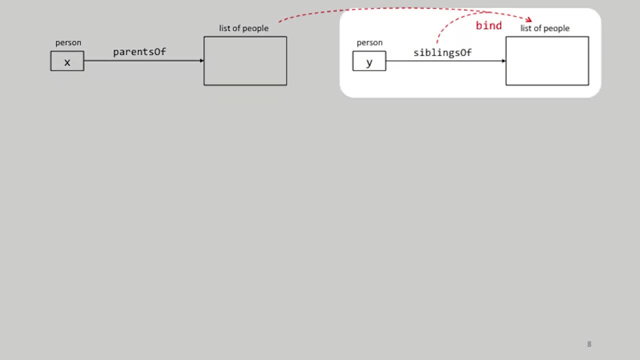 zero or more people. and the same thing with the siblings of function. I start with a person- Bob or Carol- and after applying siblings of, I end up with a monad, a list of people. and now, once again, I'm faced with the problem. 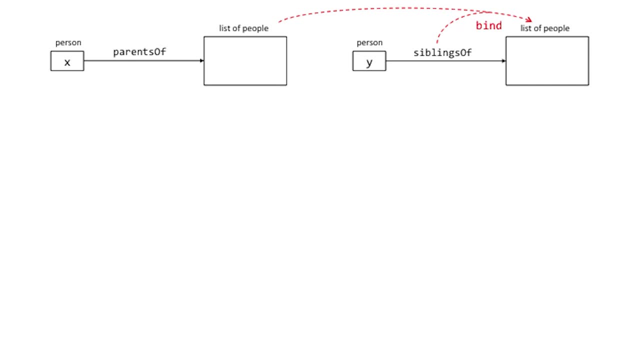 of taking two functions, each of which returns a monadic value, and chaining the functions together, applying the siblings of function after I've applied the parents of function. and to do that, I have to define what I mean by bind. okay, let's keep going bind. 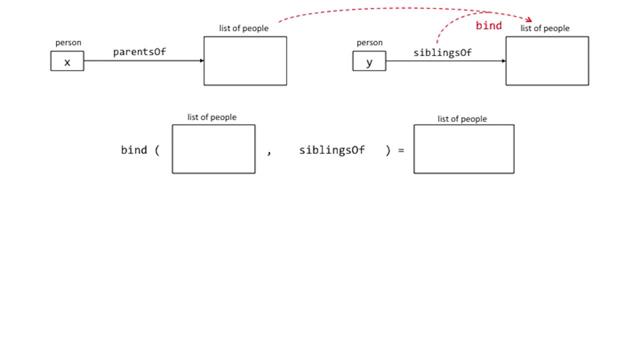 is a function that takes a monad- a list of people and a function such as siblings of- and gives me back a list of people. very cool, hey, why stop here? if I'm going to define bind, why define it only for siblings of? let me define it. 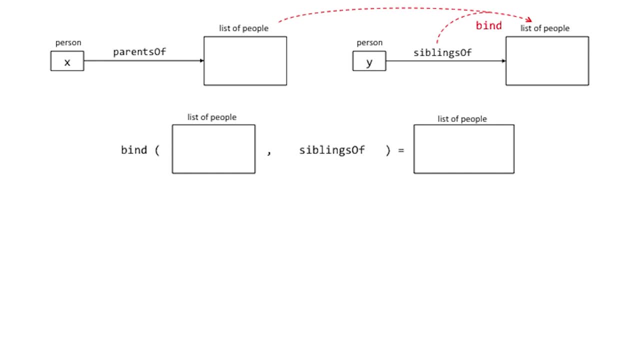 for a function of the right kind, any function of the right kind. I'm going to define bind. that takes a list of people and a function f, and bind is going to give me a brand new list of people and what's going to be the rule for. 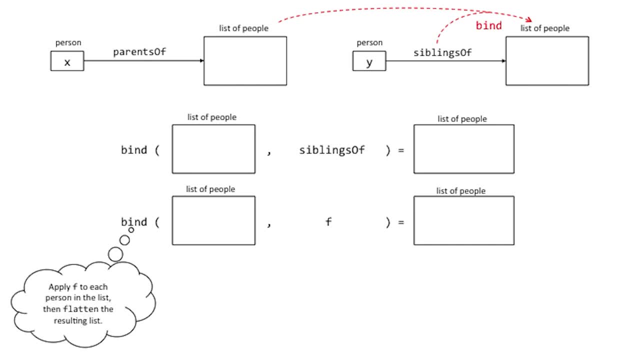 binding. the rule for binding is going to be that I apply f, that function, whatever it is, to each person in the list and then I'll have a list of lists, because applying f to a person gives me a list. the siblings of a person. 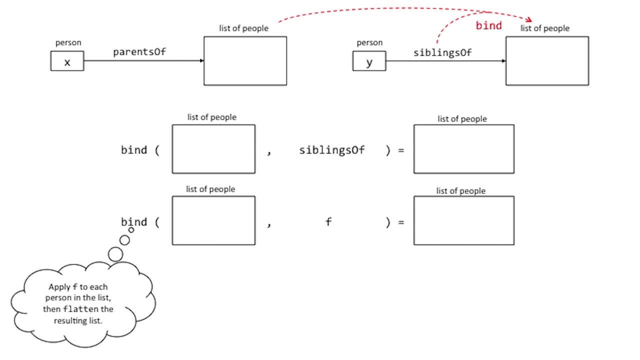 is a list, and then what I'm going to do. so I'll have a list of lists. I will flatten the resulting list of lists. what kind of a thing is bind? bind takes a list of people and a function and returns a list of people. 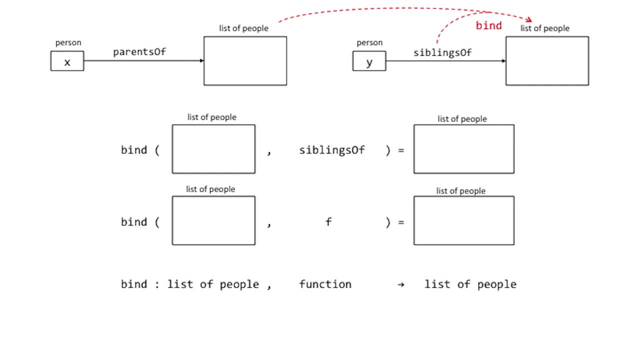 it tells me how to combine something like siblings of with an existing list to get a brand new list and, of course, that function- that f, that thing that I'm saying stands for siblings of- that's got to be a special type of function. well, special. 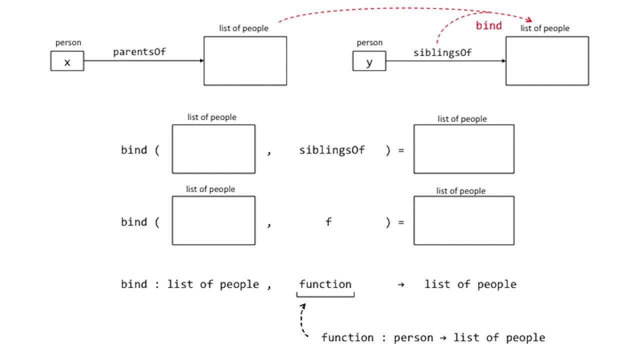 it's got to be a certain have, a certain parameter list, and it's got to have a certain result. the parameter that it has to have is that it has to take a person and it has to return, in this case, a list of people. that's the way. 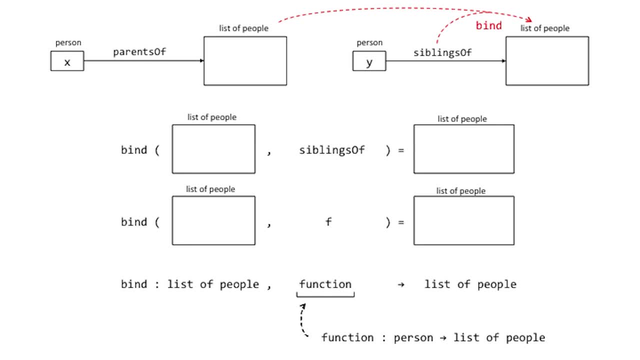 I'm operating here. this is almost exactly the same as the slide that you saw near the end of the discussion of maybe. in fact, what I've done is taken the notion of bind and the notion of list of people and maybe afloat, and found the similarities. 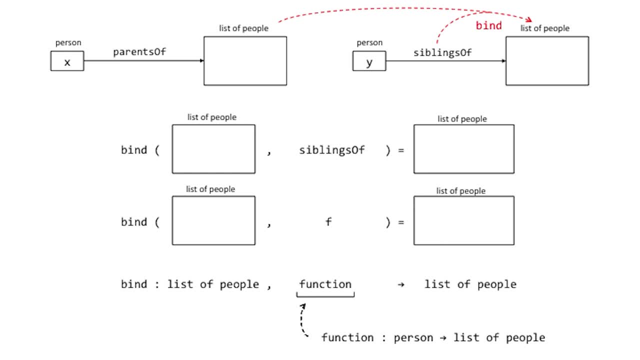 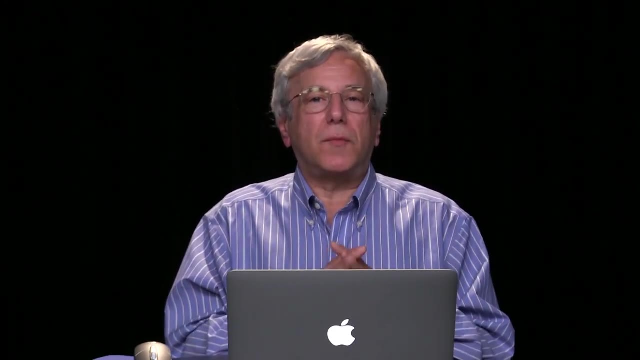 between them. a list of people, then, is an example of a monad, and a- maybe afloat, is an example of a monad. a monad is a type of a thing with a bind operation, and there's maybe another operation or two that a monad has. 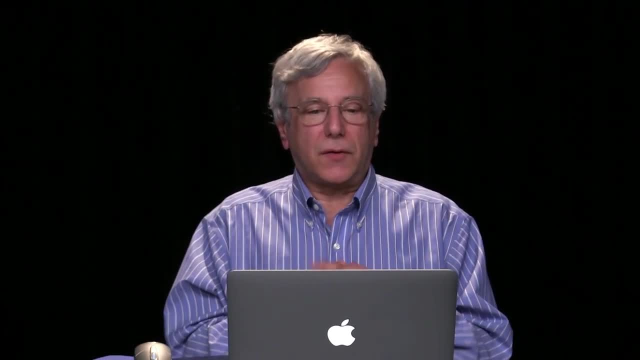 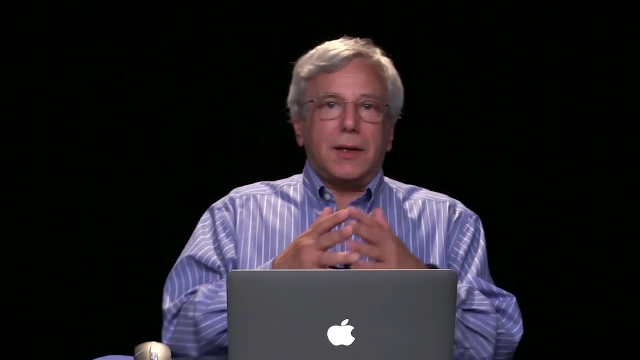 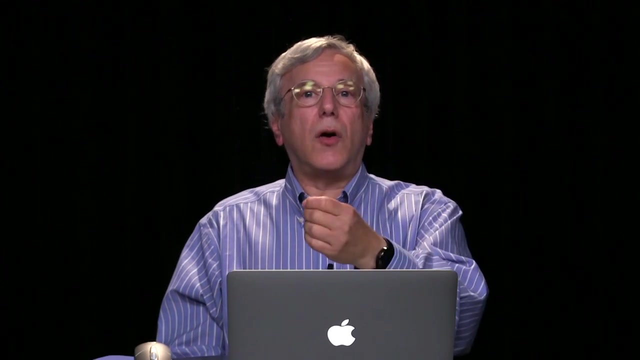 to have, but we'll leave that for further reading. for now, what we've got here is a list monad and a maybe monad. now, in the case of the maybe monad, we started with a float and we ended up with zero, or 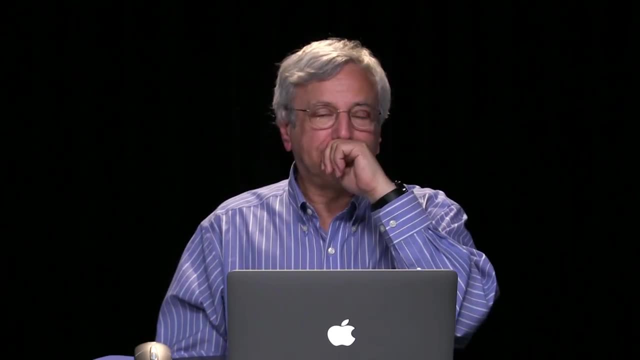 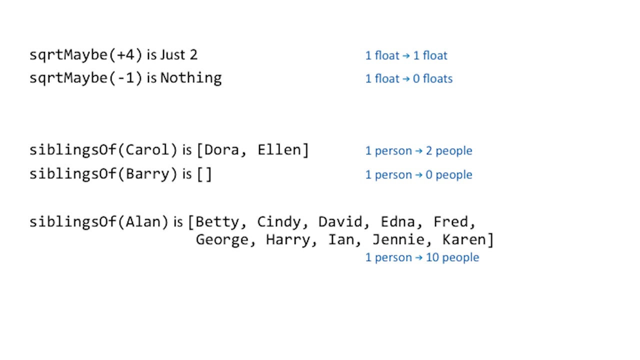 one floats zero or one. in the case of the list monad, we started with a person and we ended up with zero or more people. so when I found the siblings of Carol, I found three people. the siblings of Carol gave me two people, but I could have. 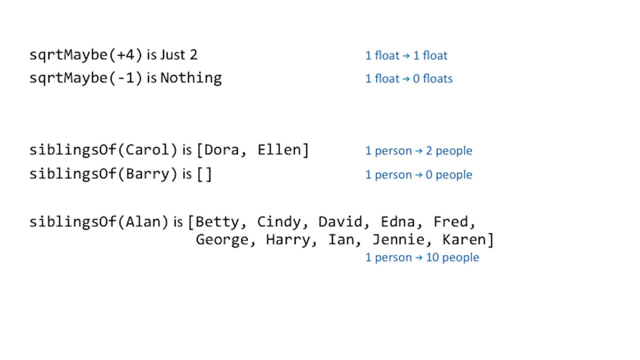 tried to find the siblings of an only child, in which case I would have gotten no people, or I could have tried to find the siblings of someone in a very large family and gotten ten people. we see that similarity here between the maybe monad and the list monad. 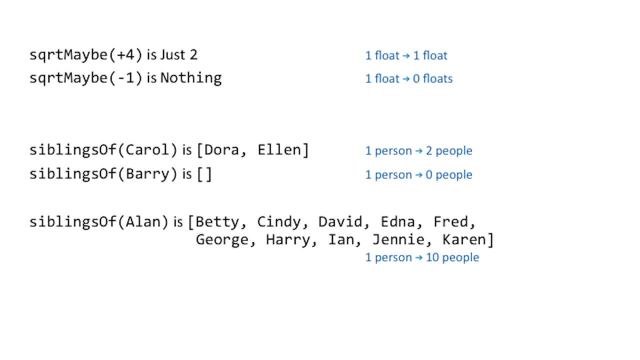 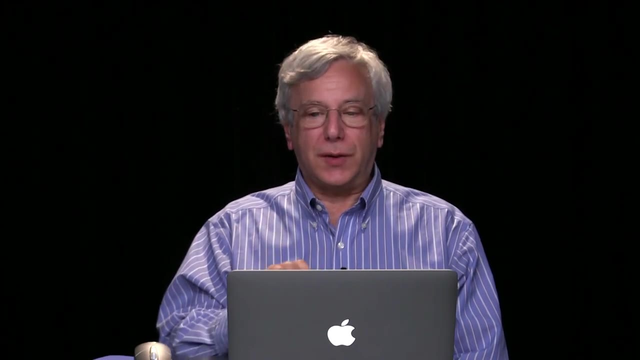 they both start with one thing and end up with some number of things. does that mean that all monads work the same way? no, let's finally try to attack the problem of input and output in the beginning of this course, or very near the beginning of. 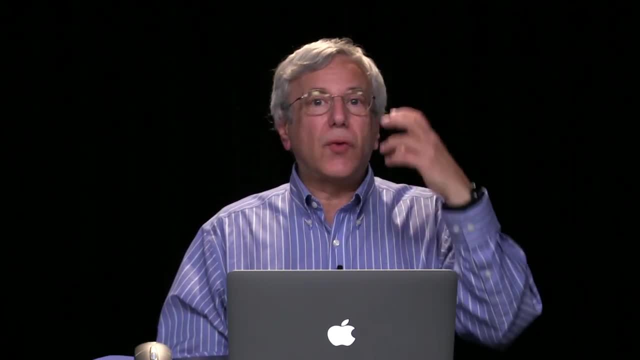 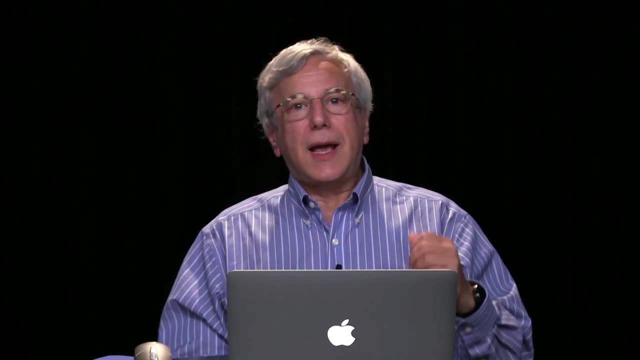 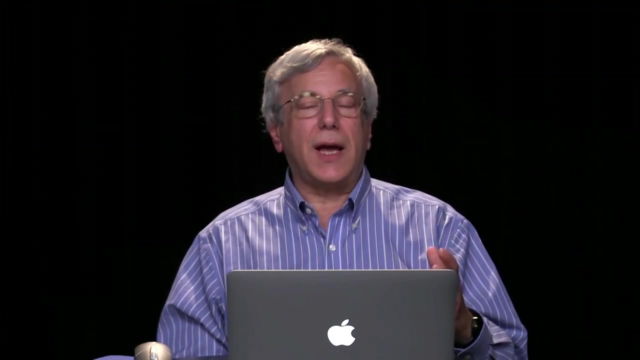 this course, I told you that printing to the screen is a side effect and reading from the keyboard is a side effect, and that some side effects are side effects that we have to live with in life. well, computer scientists have found a way, using monads, to bury those. 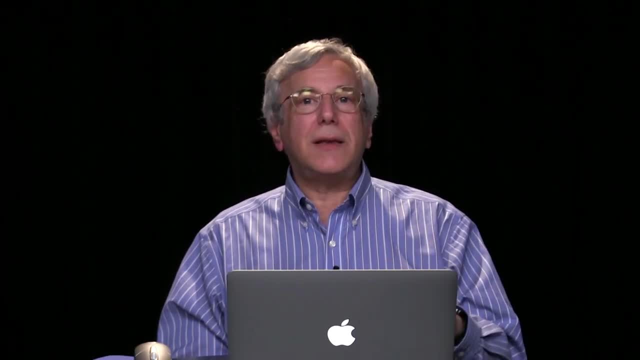 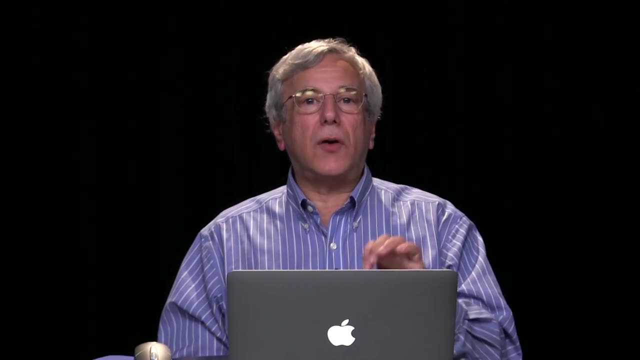 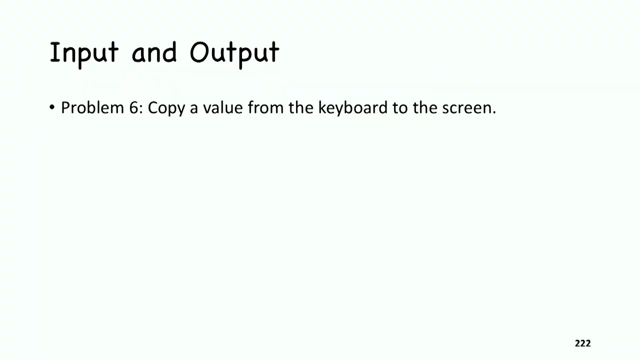 side effects under the rug and to make the expression of a method for solving a problem side effect free, even though it involves input and output. and they've done that using monads. how in the world do they do that? let's take a look at reading. 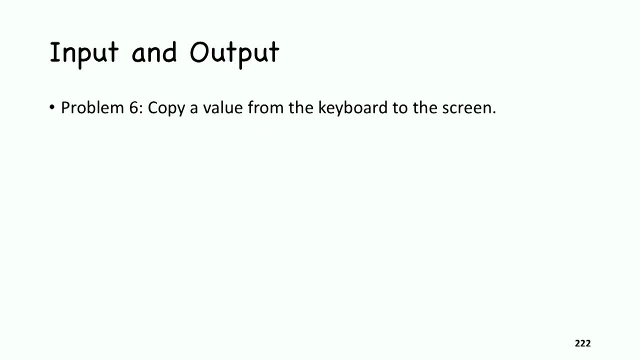 from a keyboard, first in an imperative style, and then I call it a functional style, but really better, it's called a monadic style. let me have a look here. what happens when you read a value from the keyboard? well, let's say that. 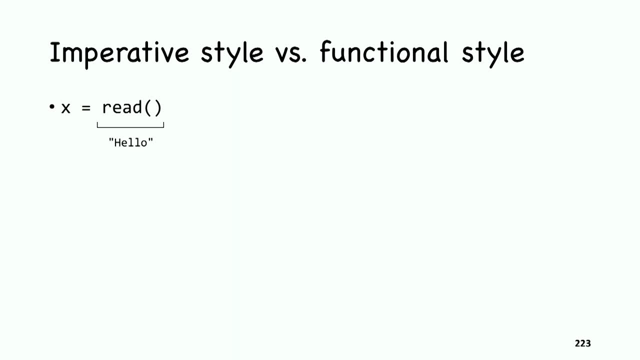 the user types in the word hello and I'm going to denote that by string hello quotation marks. well, if you say x equals read, and by read I mean read from the keyboard, then the words read with parentheses after them. that's an expression whose value is hello. 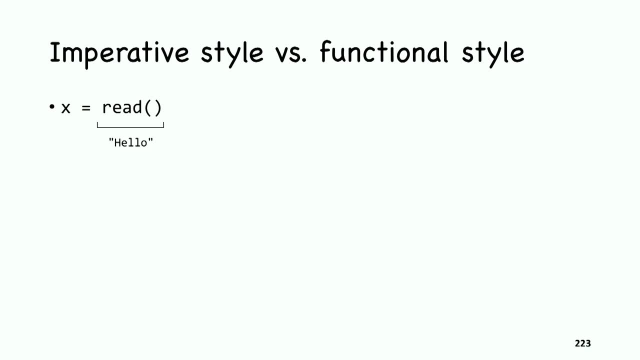 and in the imperative tradition, I can take that string hello and assign it to a variable x. now that means that one time that I call read, it might stand for hello. another time that I call read, that same expression might stand for seventeen, or it might stand for knock, knock. 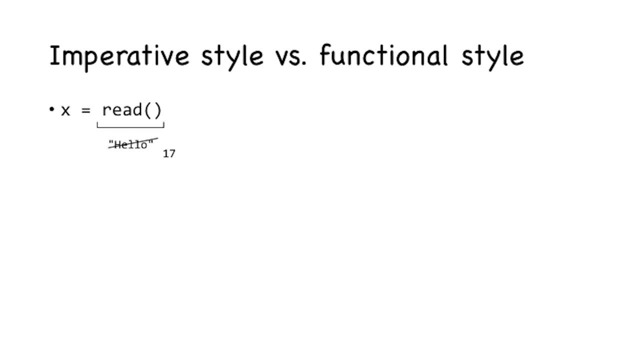 who's there, or any number of different things in a strictly imperative style. a call to read is an expression whose value is whatever the user may have typed in on the keyboard. I'm going to look at read in a different way. yeah, I'm going to have a function called read. 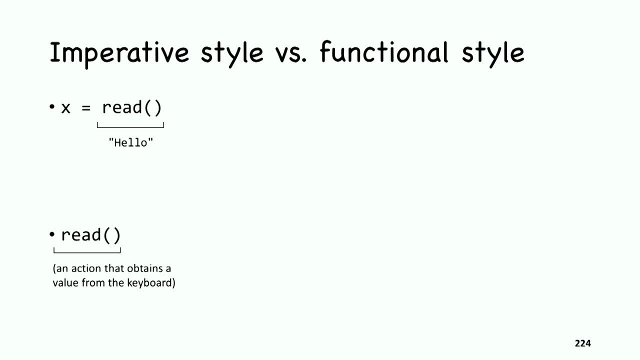 but it's not going to stand for whatever it is that the user types on the keyboard. instead, my call to read is going to stand for an action that obtains a value from the keyboard. now, that action is going to be something that's executed during the run of the program. 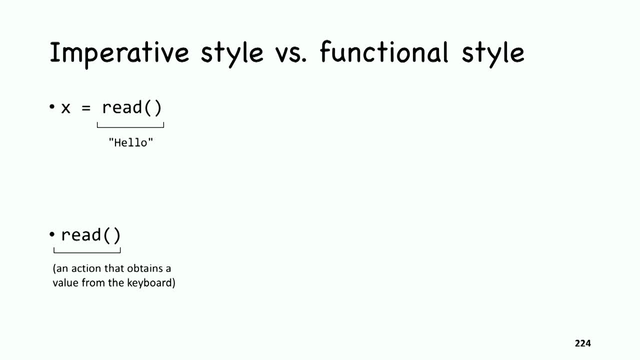 so if I just write down, read in parentheses, it doesn't mean hello, or it doesn't mean seventeen, or it doesn't mean knock, knock, who's there. it means, hey, this thing is an action to be performed. I'm going to call it a run time action. 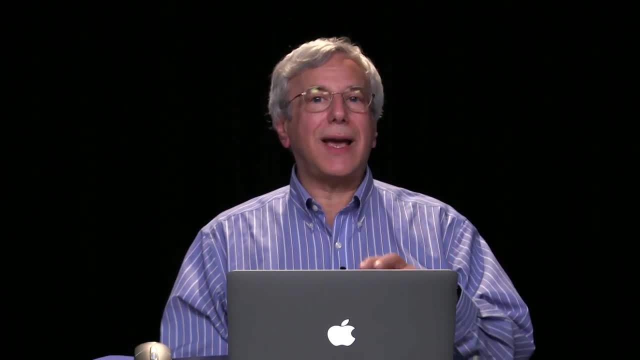 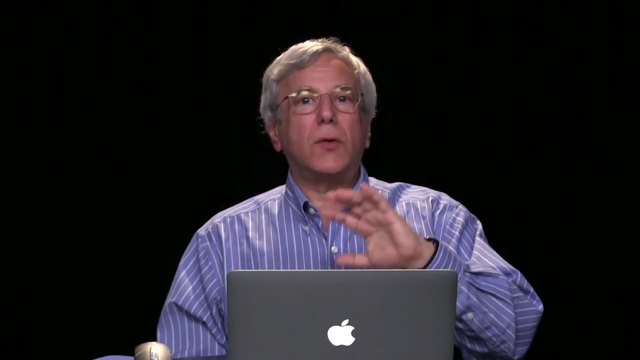 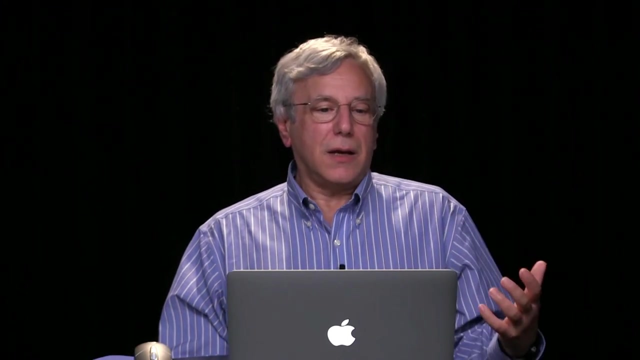 because it's an action that gets performed during the execution of the program. it's not, strictly speaking, part of the micromanagement within the code itself. I don't take the expression read parentheses and try assigning it to a string variable x or to an integer variable x. 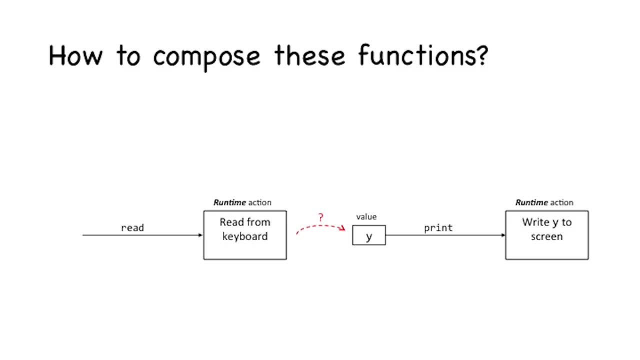 well, what's the picture here? the picture here is: I can have two run time actions. well, in this diagram I have two. I can have many more, but in this diagram I have just two. I have a run time action that reads from the keyboard and another run time action. 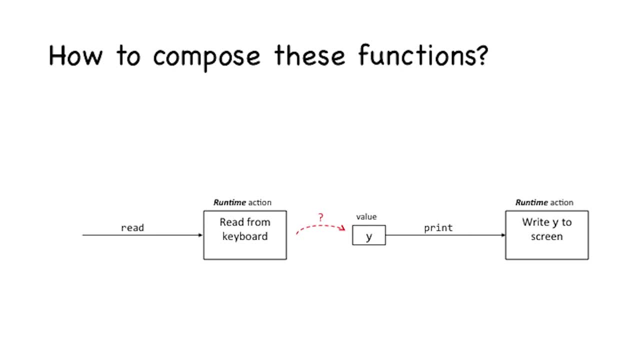 that writes a value to the screen. those again are functions, and they're functions that return run time actions. it might be a little bit abstract, but let's just see. what I've got here is a picture that looks a lot like earlier pictures. there's a big difference, of course. 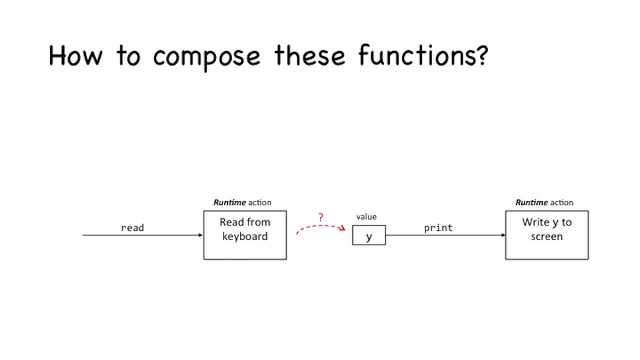 read does not take any parameters as input. it doesn't accept anything. so you don't say read y, or read z, or read x or anything like that. you just say, hey, read, it's a function that doesn't take any parameters as its input values. okay, anyway. 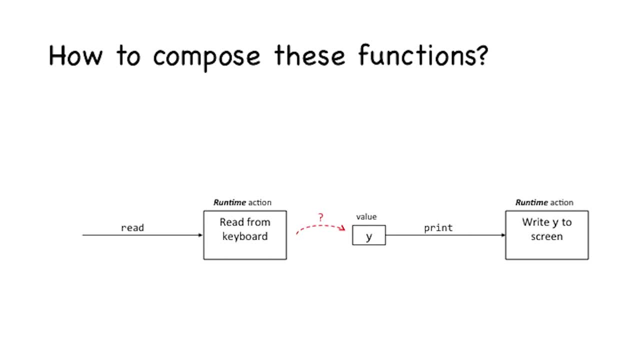 that's a run time action. and now I have another function named print, and what print does is it takes a value to be printed and it creates a run time action which is going to write that value on the screen. once again, I'm trying to chain together the printing. 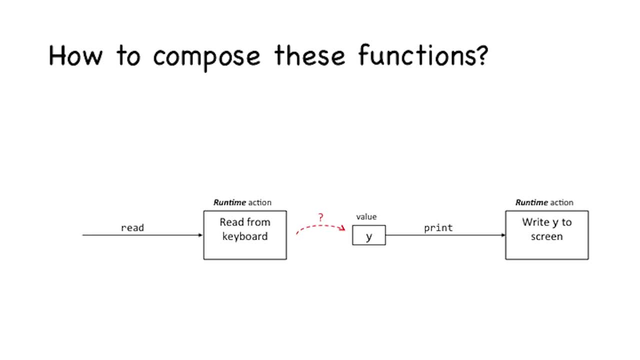 and the reading, and I can't quite make a square peg fit into a- well, in this case, a smaller square hole. okay, I have to find some way with the print function of bridging the gap between a run time action and a value that needs to be. 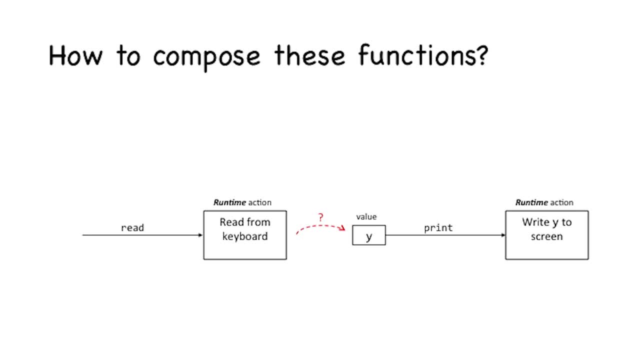 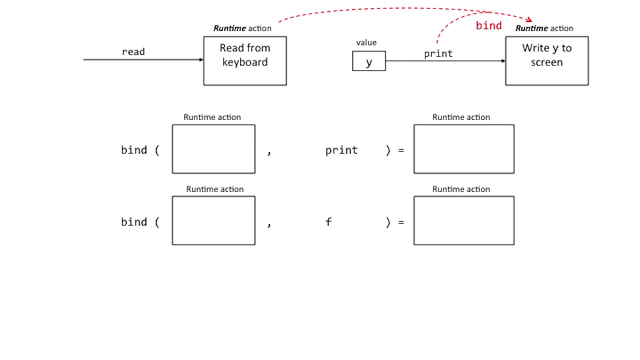 printed and of course I'm not going to somehow try to squeeze the run time action read from keyboard into the value box. instead, I'm going to create the function bind and I've spilled it all out for you all at once on this slide: the bind function. 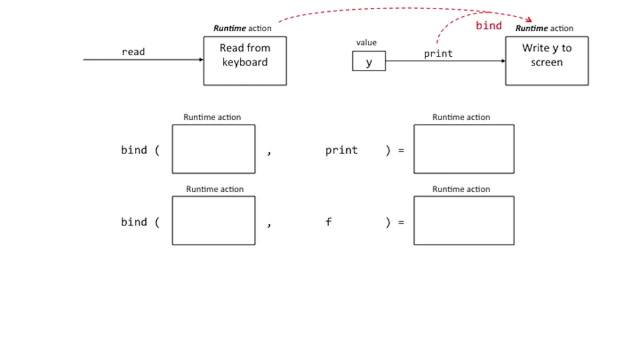 tells you how to bind together the run time action that does the reading from the function that does the printing. the bind function takes two arguments: it takes a run time action and a function like print. hey, it doesn't have to be print, it could be. 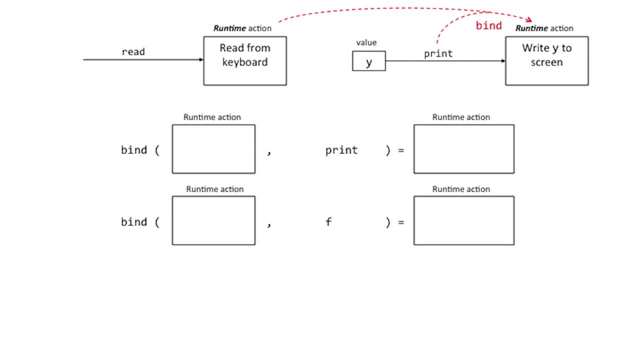 f, as long as f is the right kind of function. so what's the rule for bind in this case? well, the run time action, the action of reading, obtains a value from the keyboard. the binding says: take that obtained value from the run time action of reading. 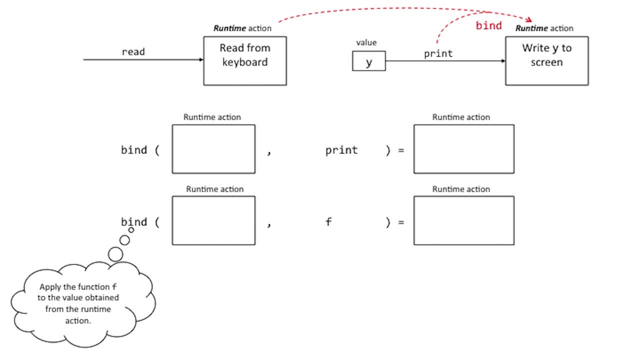 and apply f to it, and what you get from that is another run time action. a run time action that, during the execution of the program, will actually display the value on the screen. again, we have to make sure that the function f is of the right type. it has to. 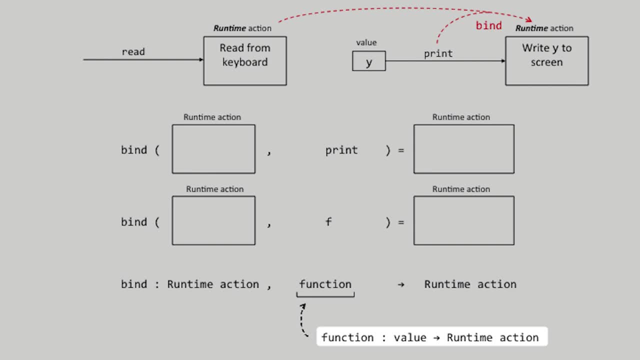 be a function that takes a value like hello and gives you another run time action like display hello. so the bind function, a higher order function, takes two arguments: it takes a run time action and a function and returns another run time action. if you'd asked me before I started, 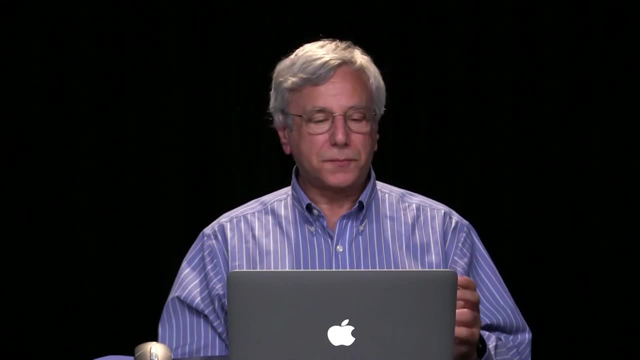 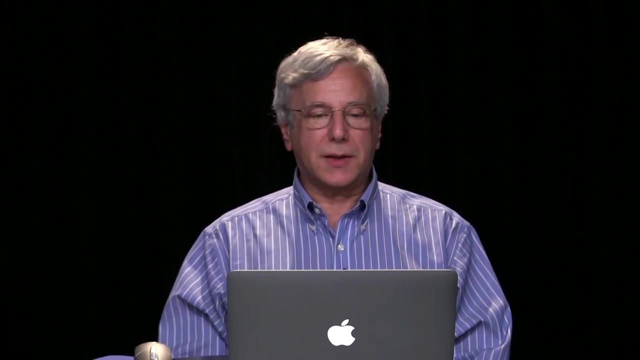 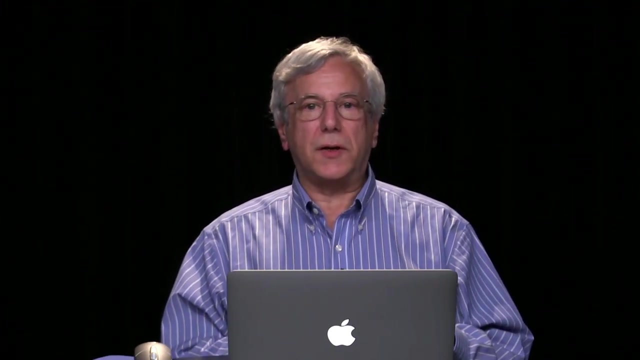 learning about monads. if there was any similarity between, maybe, type things and list type things and input, output type things, I would have said definitely not. but here we see, with the notion of a monad and with the notion of a bind function, that all three of these 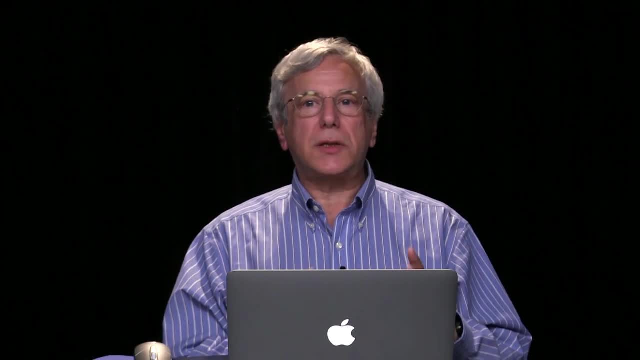 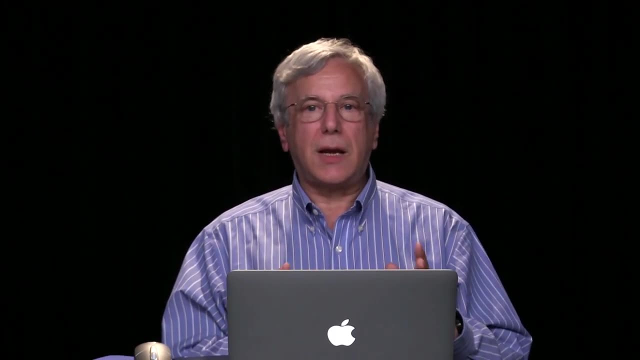 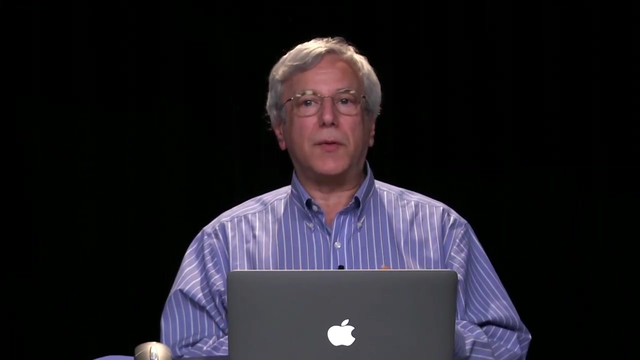 different kinds of computation are similar in structure. well, needless to say, there are monads aplenty and many different ways that I haven't shown here of using things like bind and defining things as monads and solving problems in a very neat way with the monadic structure. 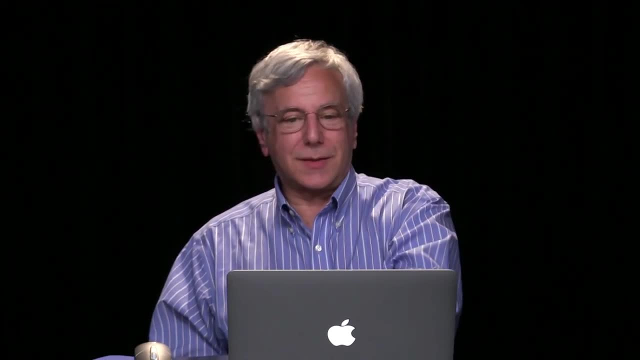 hey, I hope you've enjoyed this course.